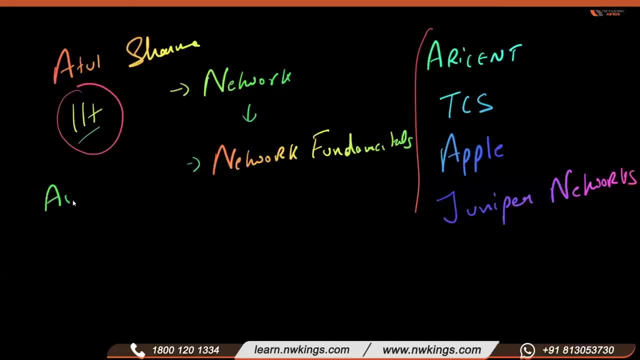 Right. So if you are, if you want to become a cloud engineer like AWS, Azure, or if you already have a good experience, but you are not able to crack your interviews because of what we call that lack of basic fundamentals, right, Some guys have good understanding of configurations of router and switches, but they don't have good understanding of the basic stuff like how things works. So we are going to discuss about that. 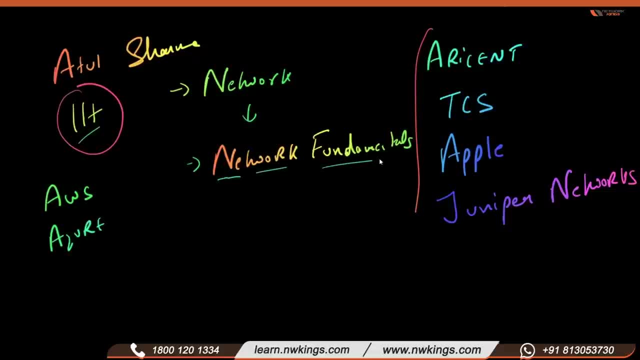 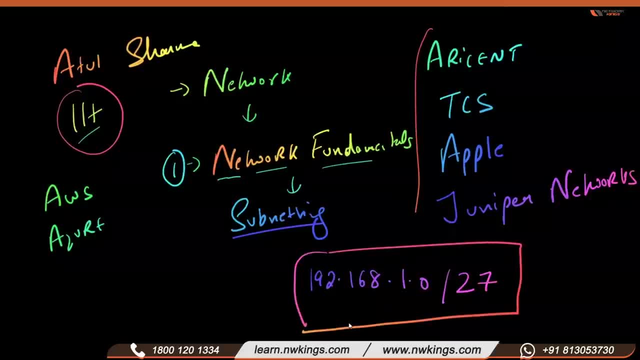 you divide this class into two parts. I just want to create a network with this network with two parts. What would be the slash value? If you know subnetting, just tell me this answer. Okay, leave it, So they got a homework. Okay. 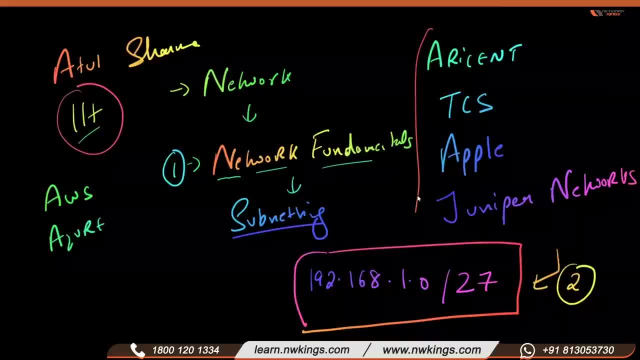 yeah, few guys are good with submitting, i think. but it's a session for everyone, right? it's not for just okay. so we will cover network fundamental submitting also. so i'm adding a submitting, so we will cover one day submitting. so those who are comfortable in submitting they can skip this. 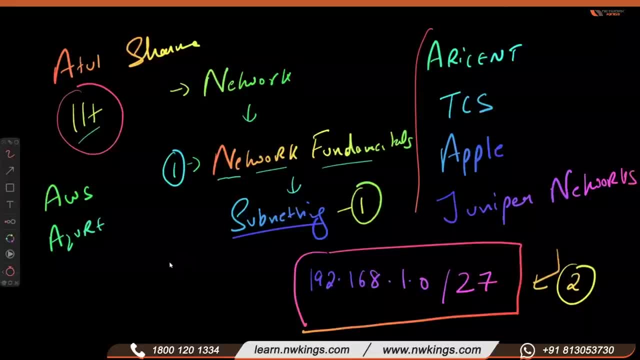 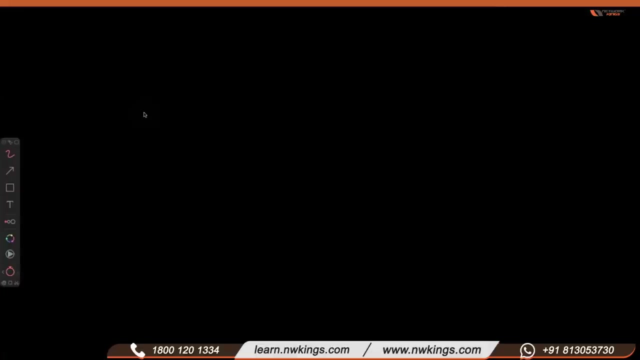 session: okay, and third day again. we are going to do some basic practicals like how to configure a router or how to configure a switch. okay, and let's see how it will be okay. so now i'm starting with the network fundamentals. okay, so let's start okay. 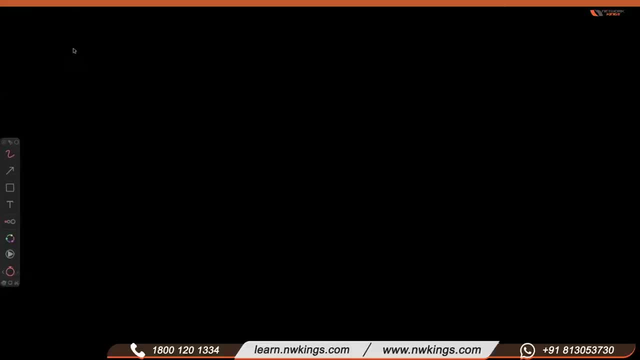 so i'll start with: what is network? so what is network? so, guys, you can always put down your answers in the chat. so what is network so like? if two computers are connected, they are all. this is also a network, right? so computer a is connected to computer b so they can share the things with each other, they can send. 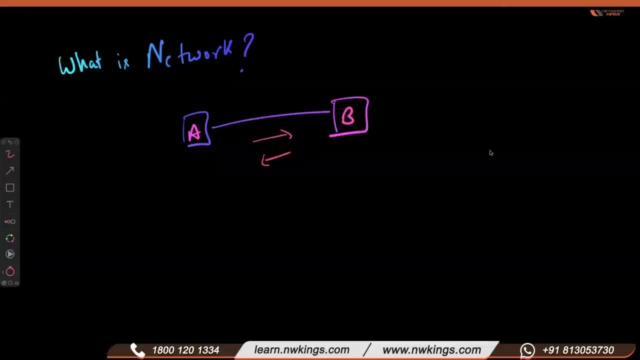 files to each other. so this is a network also, right. and if multiple computers are connected? suppose four computers or four devices are connected with a device which is known as what? yeah, so four devices are connected with a device that is known as switch. okay, so this is also a network when four computers or four devices are connected. 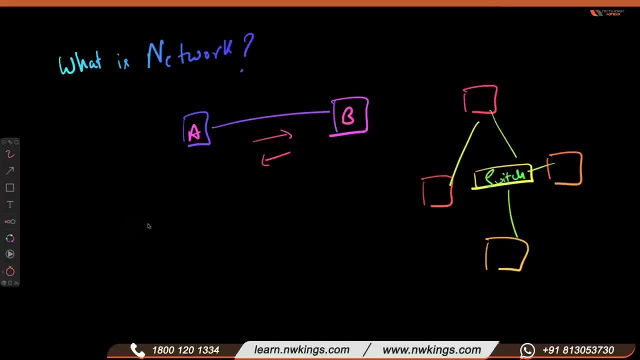 together. that is also a network, right. and when we talk about like, uh suppose i'm sitting in india right now and you will be taking this session from us, okay, so I'm in India right now and you are in US, so you, so we are also connected, right, what? but? 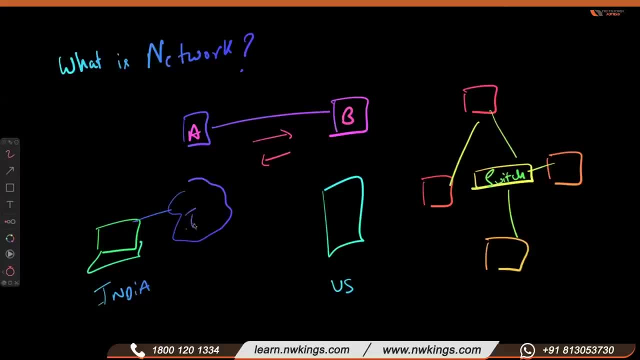 how we are connected. we are connected with service provider Network. okay, so you have your own ISP. suppose you have 80 NT and in India I'm using maybe atl or geo or whatever, right, so all these ISPs are connected together with a cable, or you can say that a fiber cable, that is, Submarine cable. 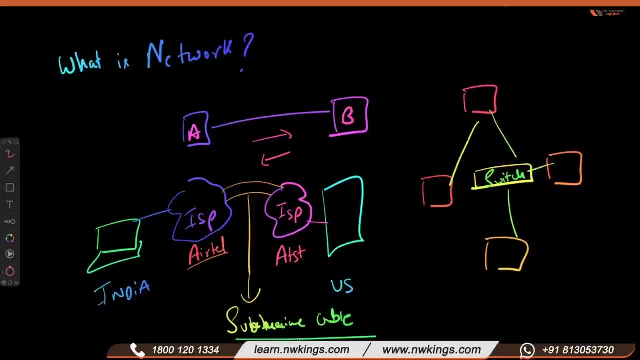 Submarine cable. okay, so what is Submarine cable? I'll show you all these things. okay, so this is also a network. so means network can be like two computers are connected together and computer, uh, and Network can be like a four or five computers are connected, uh, so computers, PCs, laptops. 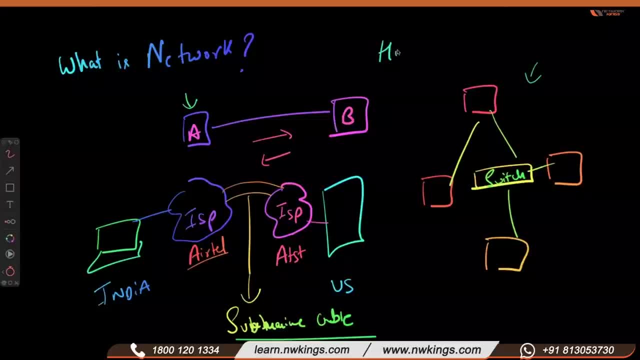 mobiles can say anything, any host, so we can say that host. so what is host? so host? basically any device which gets the ip address is known as host. so pc is host, laptop is host, server is host. so when we say host in networking, so host means the any device which gets the ip address, that is host. 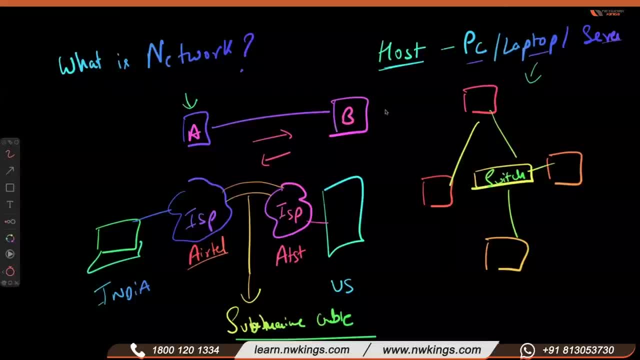 okay, so pc, laptop servers, all these machines are your host. okay, so now. so got my point right. so this is network, and what is networking then? so this is network, so what is networking? right, so it networking, or you can say the networking. so networking means when they actually they are going to share the data. so suppose, uh, you are. 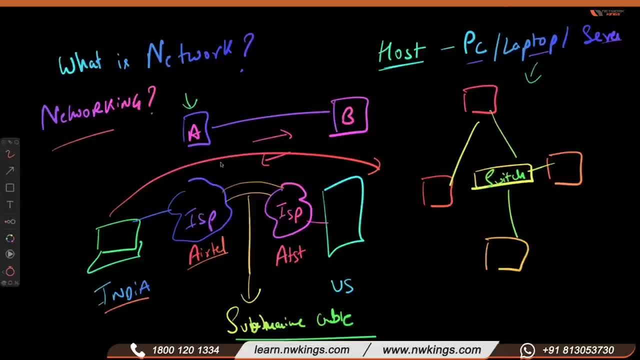 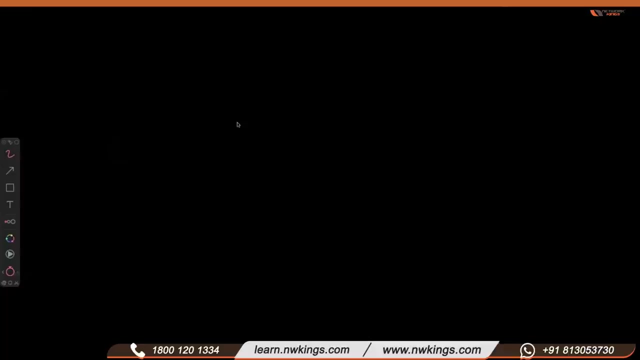 watching my screen right now. so we are sharing resources with each other. so sharing of data and resources is known as networking. okay, so sharing of data and resources in a network is known as networking. yeah, the basic i'm covering. okay, so now in network we have a like. 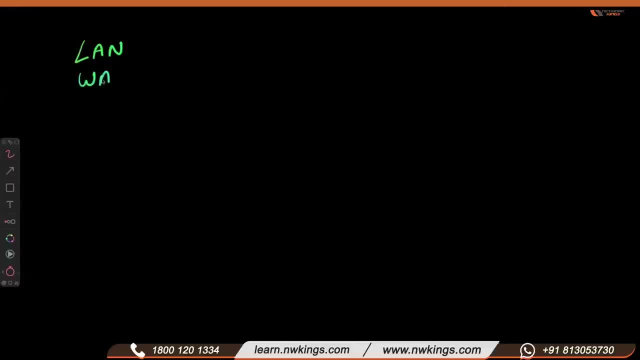 in industry we call this lan and van. so don't just uh, read the books with man pan and there are a lot of other networks, so just simply learn these two terms: lan and when. so what is lan and when? so lan is local area network, okay, and what is when? that is wide area network. 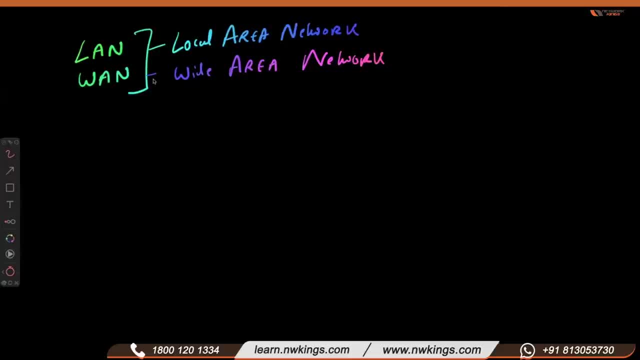 so these are only just the terms, trust me. but when you will be in the industry, you will not be figure out. this is van or lan, what exactly? but yes, in a simple term, suppose you are, you have your own office and let's say, this office is in Mumbai. okay, so this? 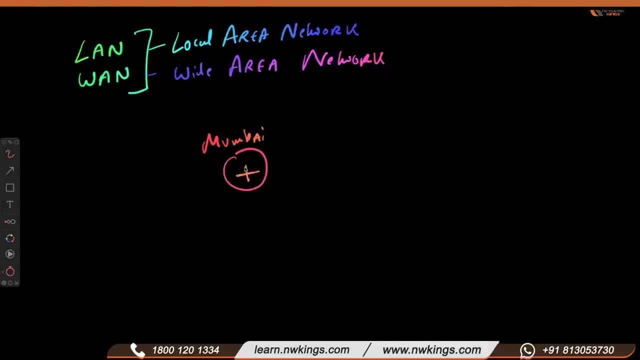 device. this icon is of a circle with this like four lines. so this is a representation of a router. okay, so this is a representation of router. so why I am adding a router here in Mumbai? because maybe I have another router in Chennai, okay, okay. so why we have two routers? because 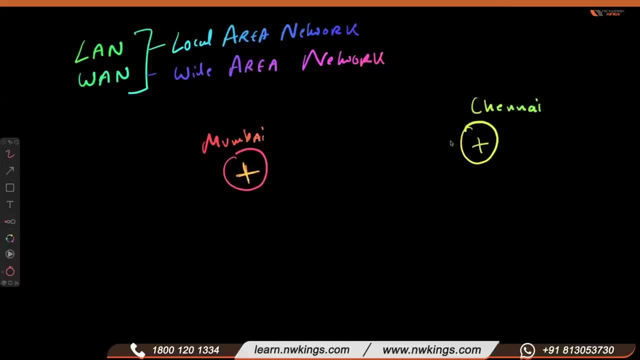 when we connect with the different networks, we need a device that is known as router. so what is router? so, when you want to connect two different networks, so I will write here: router so when you want to, when you want to connect two or more networks and which are different, right? so when you want to connect two or more different networks. 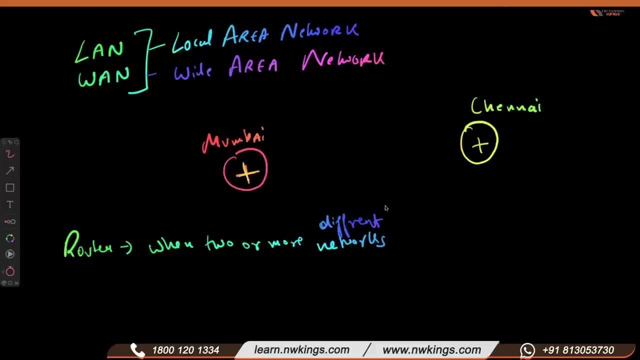 okay, so different networks, then we use this router. so let me take an example. suppose you are sitting at home, you have a broadband router right now and router is connected with internet. okay, so you have your own mobile phone laptops, okay, which are connected with the router. okay, so my these devices or these pcs are connected to 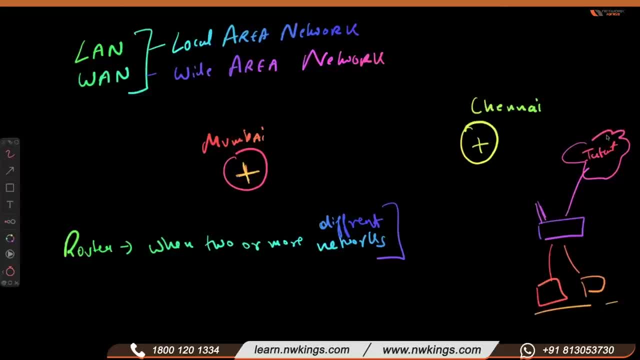 internet. so internet is what internet is: a network of networks. so what is internet? because a lot many companies and users are connected. that is internet. so internet is nothing but a network of networks, a very big network which is a combo of small networks, big networks. so you can simply say that internet is network of networks. right, yes, it's interconnection. 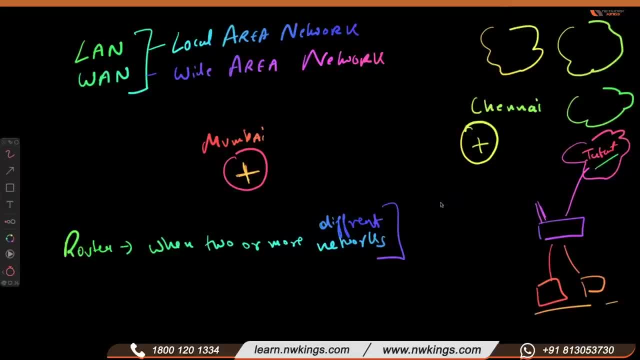 of network. correct, right. so this device, router, is helping you out to connect outside your network. so this is the role of router when you connect with the different network. this is the reason we all have a router at home. when we get the broadband connection or any type of connection got it. so this is the 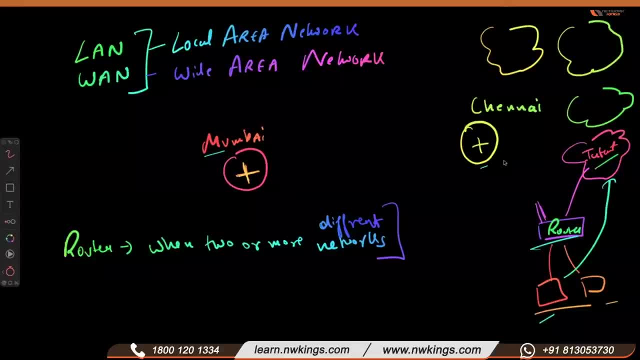 reason when you have your branch in mumbai and you have another branch office in chennai, so you in you, if you want to connect both the locations, so you need a hardware device that is known as router. okay, got it. so router is what? when two or more different networks are connected together? 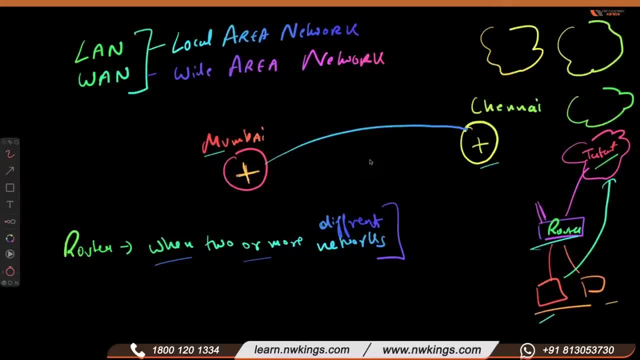 they actually need a device that is router. okay, got it. so below this network, below this router, okay, so we have a device that is. you can say that simply. that is a device which is a switch. okay, so switch has a lot of ports, like four ports, eight ports. 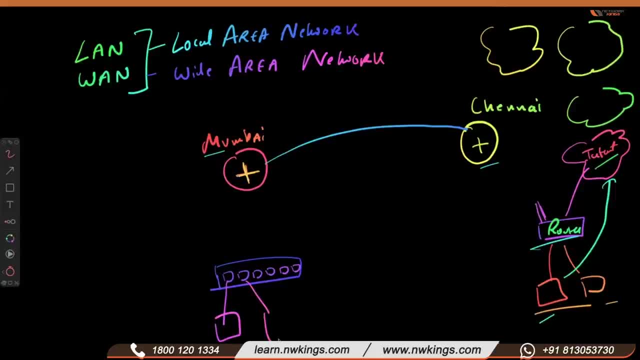 so it has a ports where we can connect our computers, servers, printers or any type of network device, and this switch is actually connected with your router. okay, so this area, or this area, you can say that this is a lan network. right, and chennai also have same type of. 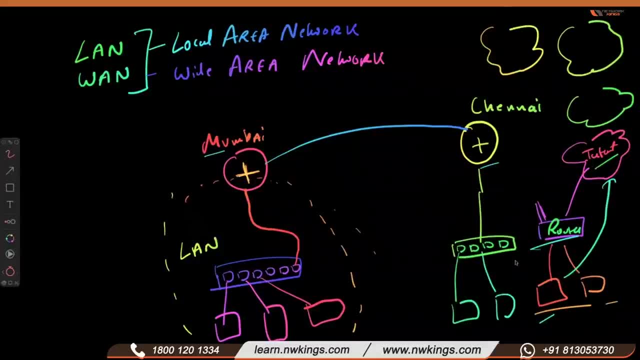 terminology that we have a switch. all my computer servers are connected together and that is also a local area network. and this we can say that this is a wide area network, and now when? so this wide area network doesn't mean like we are connecting two locations only. 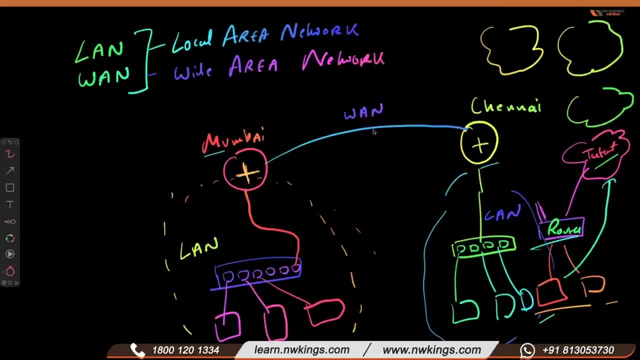 that is when. so when can be of two thing, uh, two types: that is private and one is public. okay, so public means internet and private means your private connection. so public means internet and private means your private connection. so when you are paying. see, it's a very simple thing, just understand. 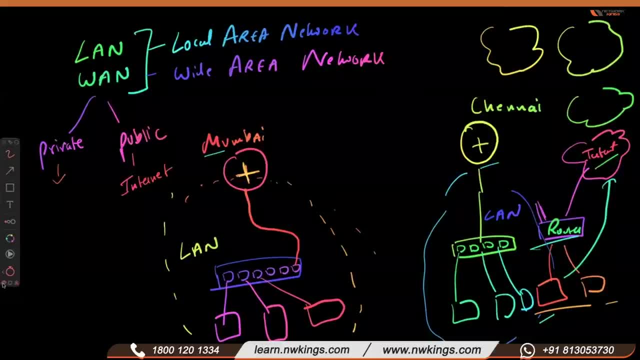 so when you are not getting, or if you don't want to pay a lot, you can just use internet connections. suppose mumbai device just hold on. yeah, so mumbai device is connected with internet and chinese is also connected with the internet right. so now, with the help of internet, you are actually connecting your mumbai and chennai. that we can. 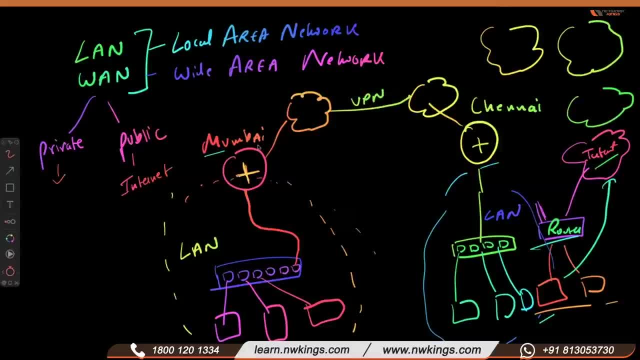 say that this is a vpn. okay. so when you want to connect mumbai and chennai location with internet- because in mumbai we also have internet, in chennai we also have internet- right. so when you want to connect to your branch office's headquarters, at that time we can say that we need to create a vpn connection. 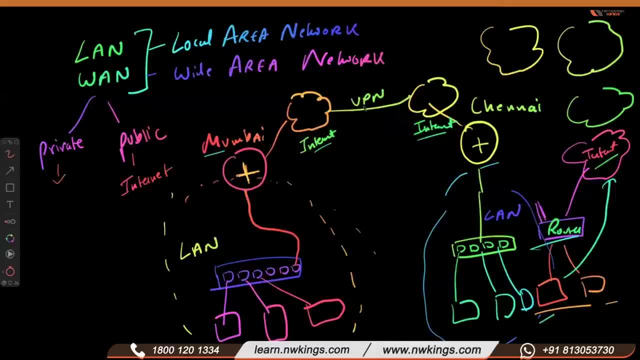 between mumbai and chennai. that is your public van, so this type of network is known as public van. when you are actually using public resources and connecting your locations, got it? say yes in the chat. yeah, i'll explain what is a switch, don't worry. okay, good, yes, okay. so when we are going to connect with the help of internet, that is known as public 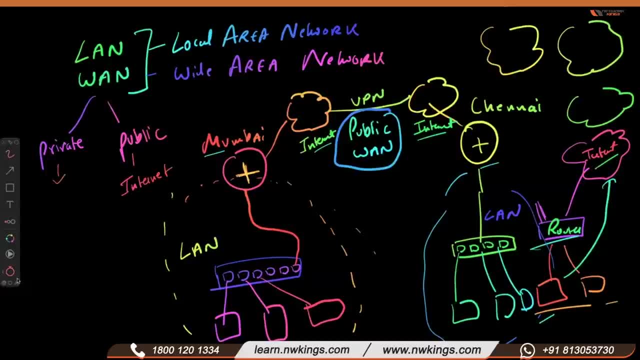 van and when we have enough money that we and we want secure connection, we can use a dedicated, dedicated line that is known as private one. but yes, we don't have enough funds to you know, we don't have enough money to connect with the public van, invest a cable between mumbai and chennai. so who is going to make or create a connection for you? 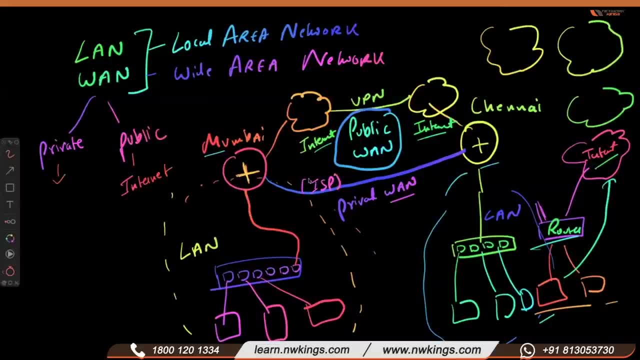 isp. so in both the, in both the networks in private van your isp will be same for on both the ends. like in mumbai also you are using atl and in chennai also you have to use atl. then only you atl can create a virtual connection or a hardware connection lease line. there are a lot. 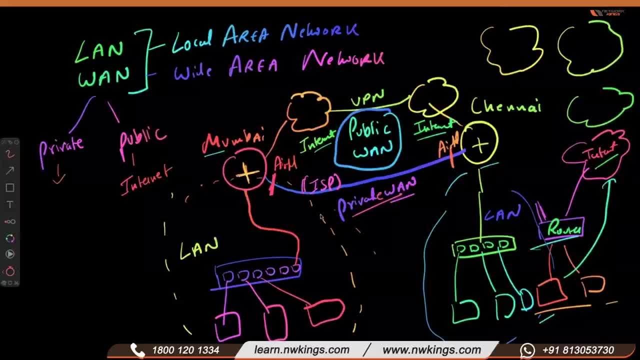 a lot many type of isp connections available right like mpls, l2 vp and l3 vp and there are a lot of other uh connectivities. that is too advanced right now for you, so just understand one thing, like in van, we have two type of connections: private and public. 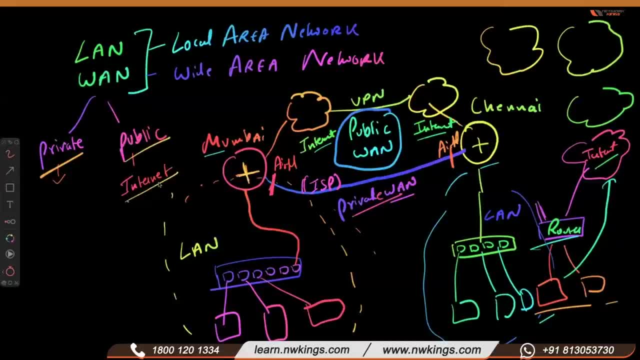 so when we connect all our offices with internet, okay, so that is public van. and when we connect all our offices with the dedicated line, with a high cost cable or really leased line, you can say that leased line, okay, so that type of connection, you can say that private, so private is costly. 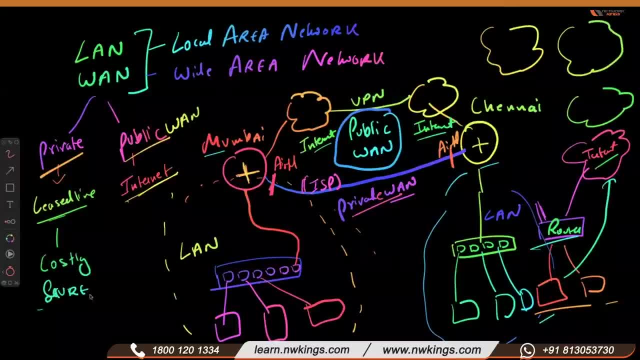 and secure. but so it's a secure connection because nobody is uh in between the connections, but in public van it's internet. it's not costly, it's a cheap connection, but yes, it's not secure. so this is the reason we have to use advanced technologies like vpn, ipsec or other type of 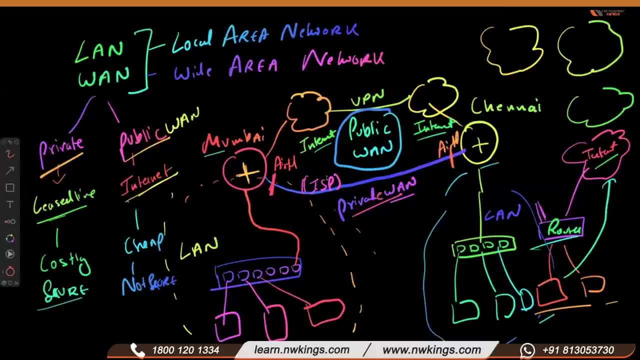 things, so that i'll discuss. okay, so that is the difference between local area network and wide area network. so local means the network which is behind your router, or you can say that downside, downstream, uh, like all your switches, routers and all. so this is the lan network. when 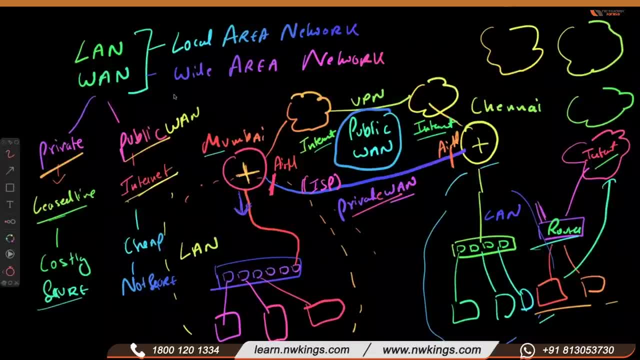 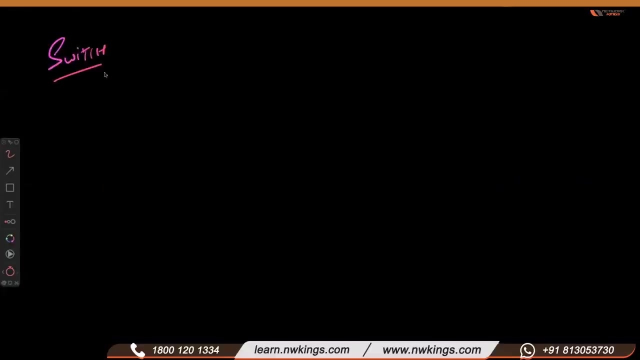 you are going from outside your network, that is when wide area network, so you can simply say that: so this is my wide area network, okay, yeah, so let's move on. so i'll explain what is a switch. okay, so let's see. so switch is a device which is used to connect two or more. 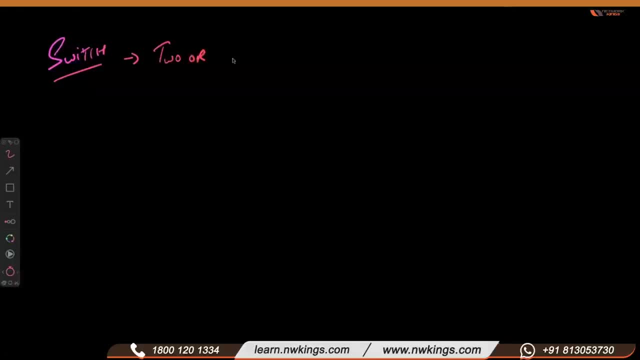 host or two or more computers. so what you will do when you have two or more computers like, uh, let's take an example, suppose we have, we are four guys and we want to play a land game. okay, so we want to play a land game, like a counter strike, call of duty and anything. 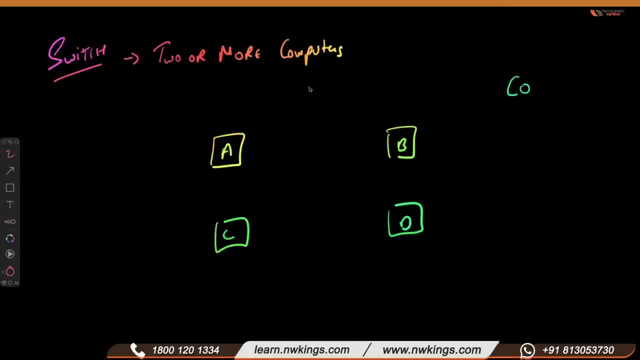 okay. so we want to play a land game like a counter strike, call of duty and anything like that. okay thing, right, we want to play together what exactly we will do. so either we can have, we can create, uh, we can connect with the wi-fi or something, but or simply we can buy a switch from market which? 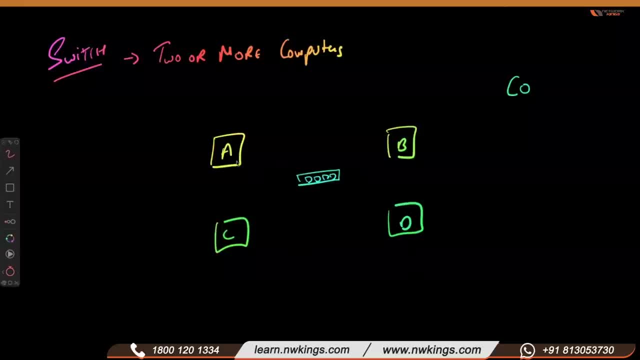 is hardly uh 10 to 15 dollars, right, and we will connect all our devices with this device. this is a switch, but we in market, when we buy switches from amazon or from any website, it starts from 10 and like we have a very big companies like cisco, juniper, hp, aruba and lot, many big companies. 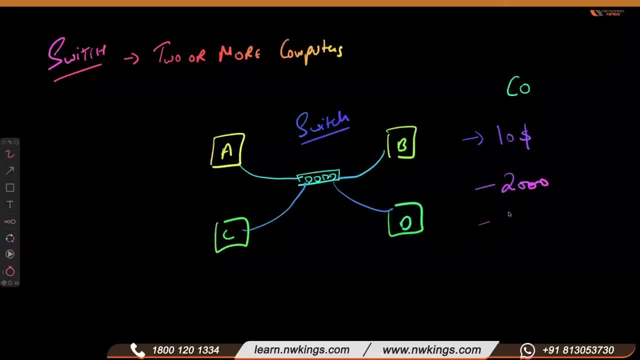 they have two thousand dollar switches. they have twenty thousand dollars, which is. but what is the difference between this ten dollar and two thousand dollars? basically features features. so in a normal 10 switch, when this device, uh, wants to communicate with b, the information will pass on to d also, c also. so this happens with the local switches with. 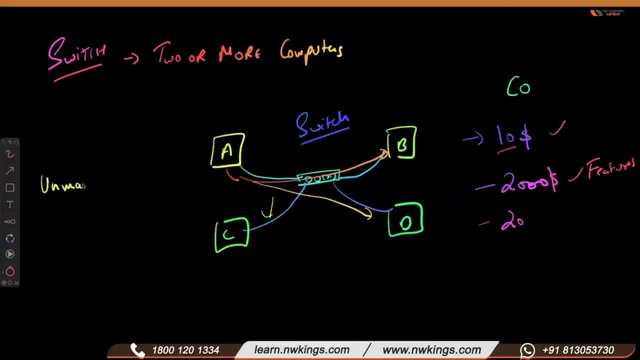 which are known as unmanageable switches. so unmanageable switches are nothing, just extension to the devices like, uh suppose, a power switch right at your home or at your office, or extension board, what we call. so you have a one power socket. so what you will do when you want to connect multiple devices? you will. 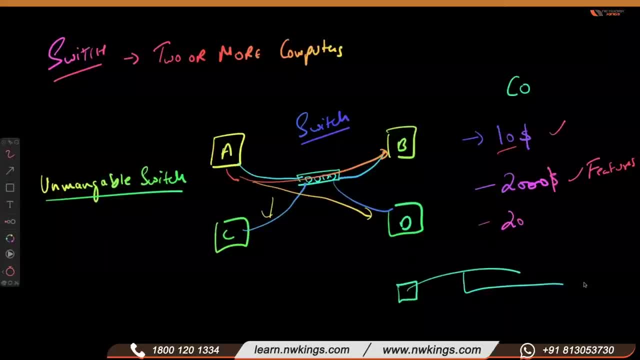 order a power surge right or a power extension board where you get multiple ports and you can put your charger, laptop charger and other things right. so the same it- this unmanageable switch- is extension so that you can connect multiple devices. but when we talk about manageable devices, 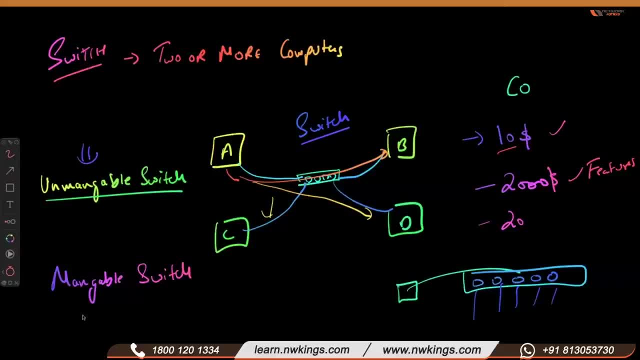 manageable switches so they have a lot of functionalities, like vlan is a concept which comes under manageable switch. so all your industry- uh, companies or big firms- actually uses manageable switches so that it we can create a lot many or we can use a good features in these manageable switches, but in unmanageable switches we hardly get any feature. okay, yes, you can say 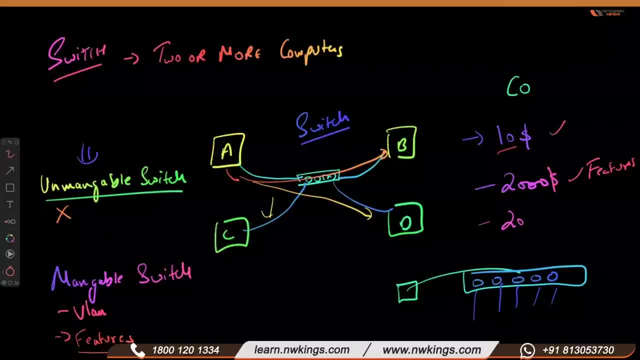 that it works like a hub, right, but it's not a hub right now because hub is obsolete technology. nobody uses hub right now. guys, can you please stop your video? you, okay, okay. so switch is nothing when we want to connect devices in a company we use actually. 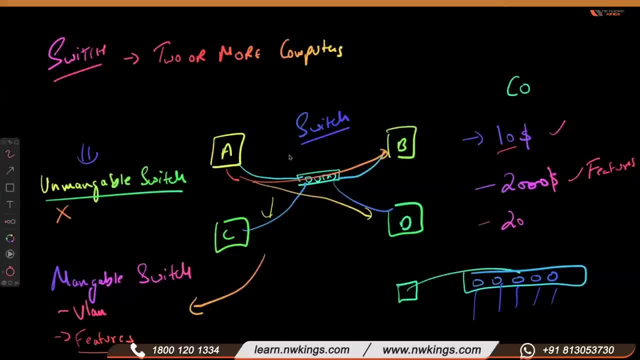 manageable switches and when we just want to play games or just want to use at our home offices or a very small offices, we can use unmanageable switches. so now in switches we have this term l2 and l3. so what is this l2 and l3 switch? 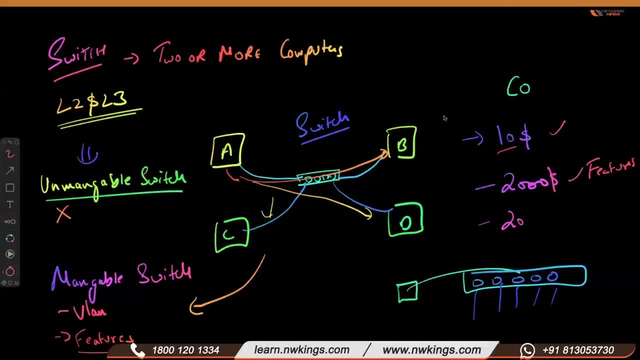 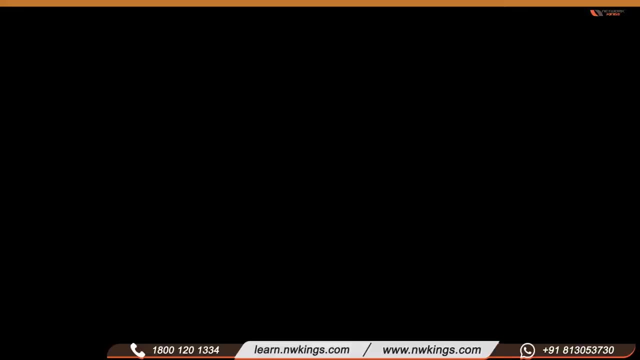 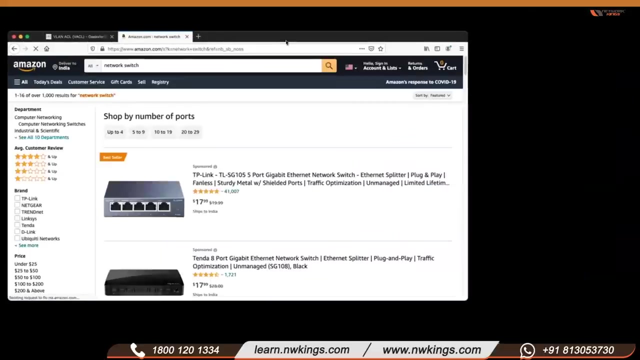 okay, so l2, l3 switch. i'll explain later, because before knowing this, you should know about the osi model. what is the example of unmanageable switch? i'll i'll show you something, just hold on. okay. okay, so i'll show you. see, this is an unmanageable switches, so you can see. 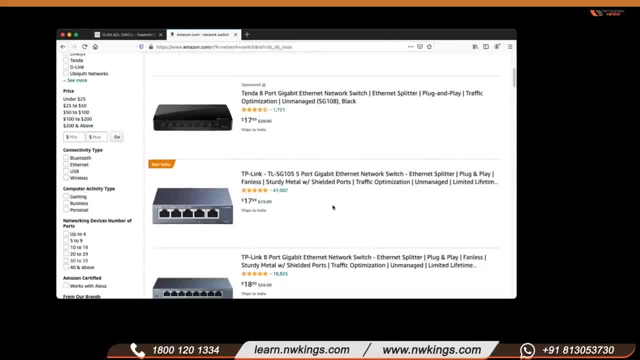 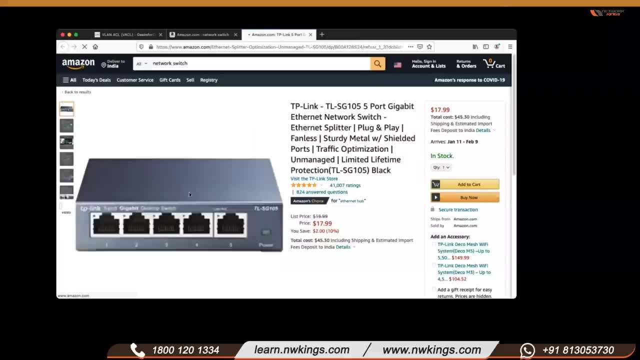 it hardly cost 10, 15, 20, 17 device which will allow you to use those kind of lock to access those individual devices. so once here, let me just conscience take a look here. can i just let me set it up a couple times, help you to connect four to five machines so you can see. so it's a 17.99, 18 dollar device. 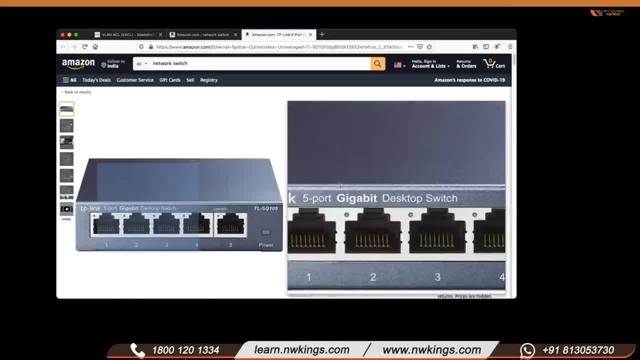 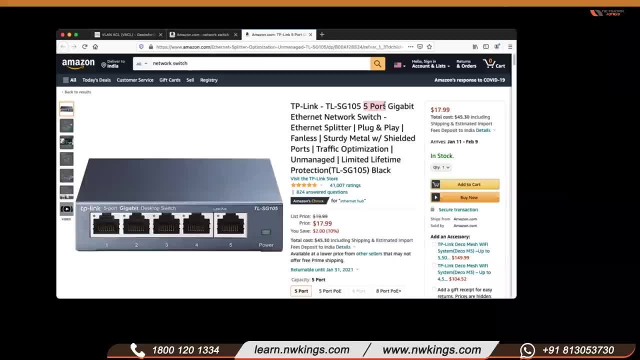 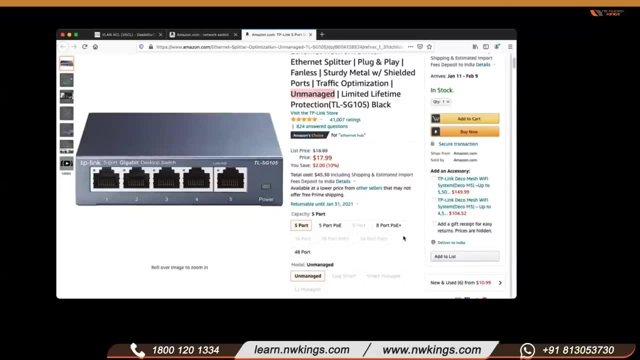 which will help you to connect at least approximately four to five devices. so you can see five port. so it means you can plug almost five devices in this device. and this is unmanaged- you can see here unmanaged. so in industry you can have around 24 port, 8 port or 48 port also, so you 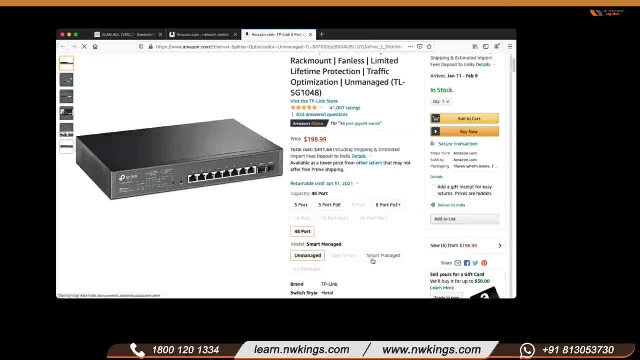 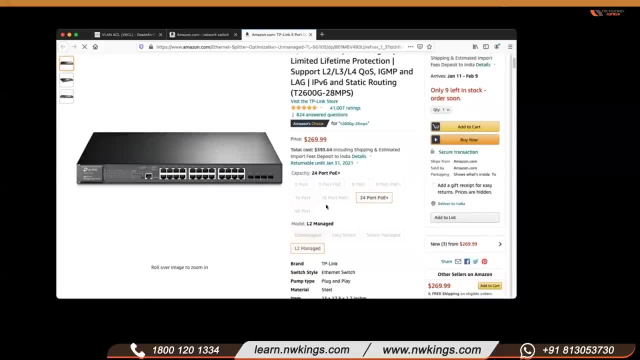 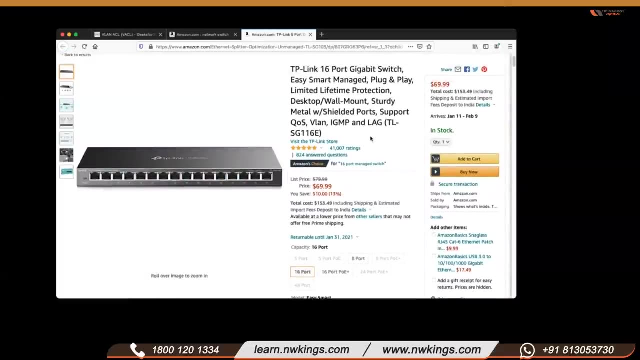 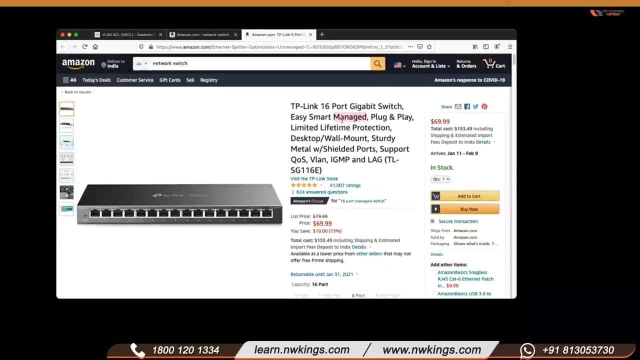 can able to connect 48 devices. so that is unmanageable device. that is very like you can say that cheap or like cost effective, but from industry point of view this is not acceptable because it doesn't have too many things. okay, yeah, but you can see here it's managed, but somehow it's a smart managed or. 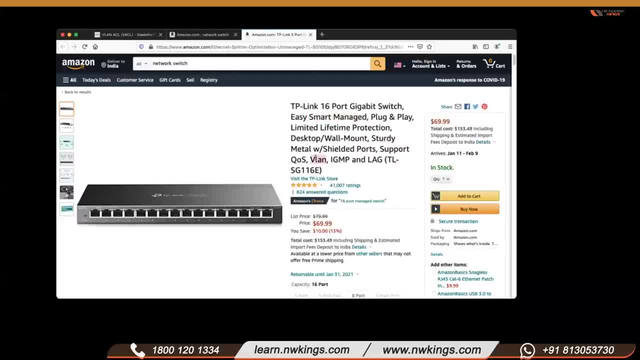 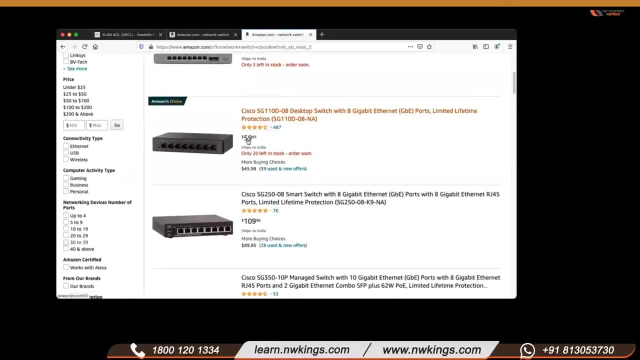 partially managed. so it is giving you option of vlan. but if you go and buy the cisco switches which are or hp switches, so they are very costly. so these- even cisco makes very small devices nowadays- okay, but this is hardly at 60 dollar. but when you go into the industry side it will. 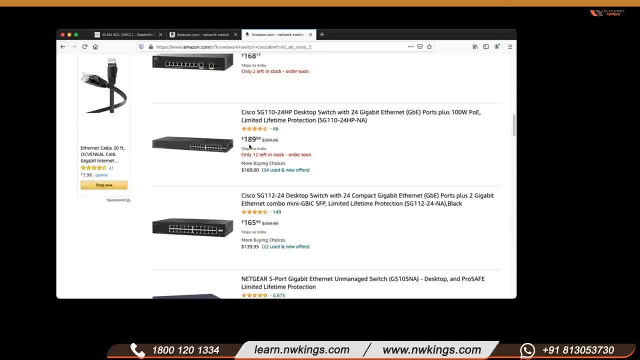 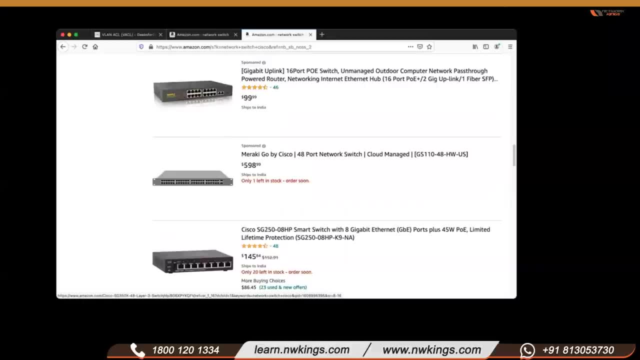 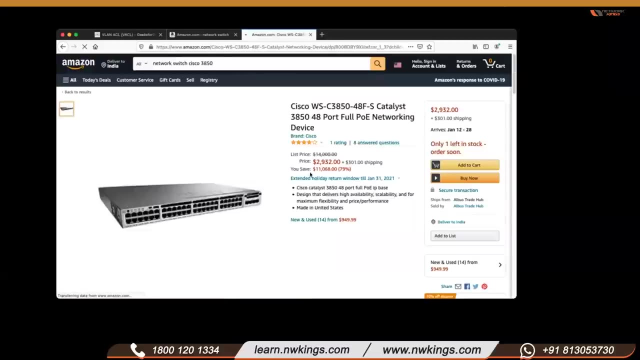 cost more, or maybe a thousand dollars, or maybe you can see this. so i'll show you one device that is 3850, so that model is 3850. okay, so cisco has a device that is also a switch that will cost around 3000 plus or maybe. uh, and maybe this is a new or you can see, the actual price is fourteen thousand. 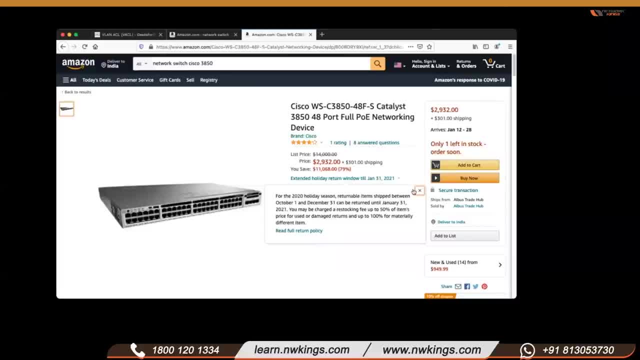 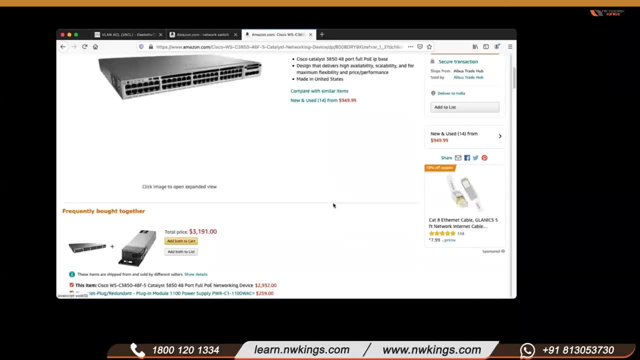 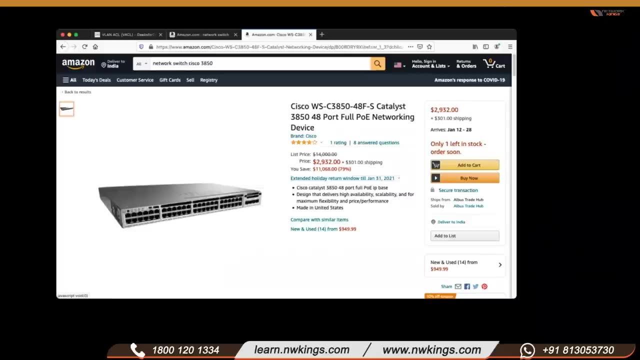 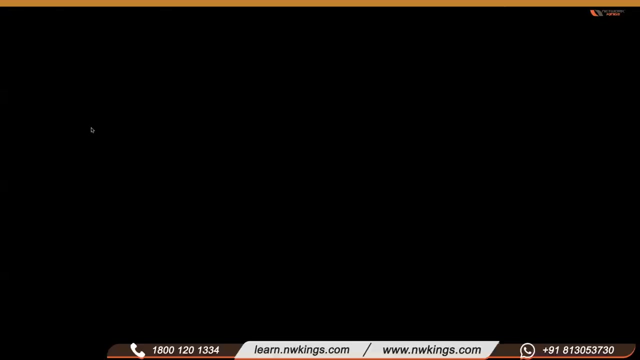 dollars. maybe this is the old one or refurbished one. okay, i'm audible, guys. okay, great, thank you. okay, so this is the difference between managed and unmanageable. okay, so i'm giving you some real examples by showing some images and with amazon. so what's the difference actually? so unmanageable is the difference between managed and unmanageable. 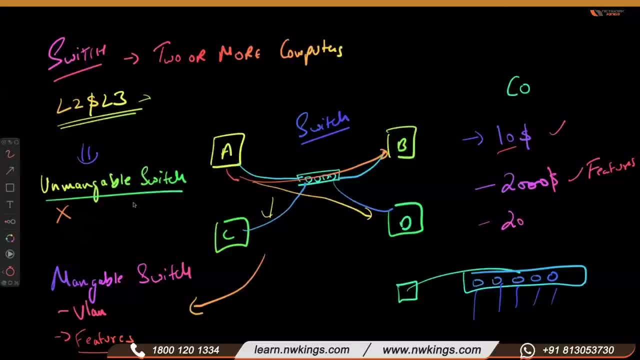 is like very basic functionality just to get the work done. but in manageable switch we get vlan features and lot other things. so this is the difference between unmanageable and manageable, because people actually ask me when they do, uh, what exactly they ask? they ask, sir, what? what is the difference between this? 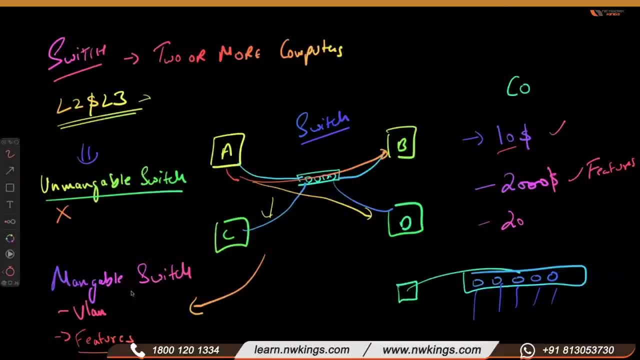 10 or 20 switch and with two thousand dollar devices, because they have more functionalities they have, and what type of functionalities that you will dis, that will be discussed later on. yes, so it goes with the router also. so if you have, uh, let me show you. yeah, so now let's. 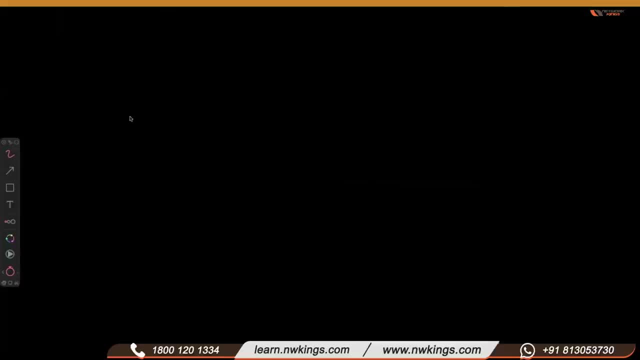 so let me take a snapshot so that i okay. so now let's take a look at this router. so router is also like you can say that it's a manageable or unmanageable, but it's better to call this uh when we have this device at our home, so we actually 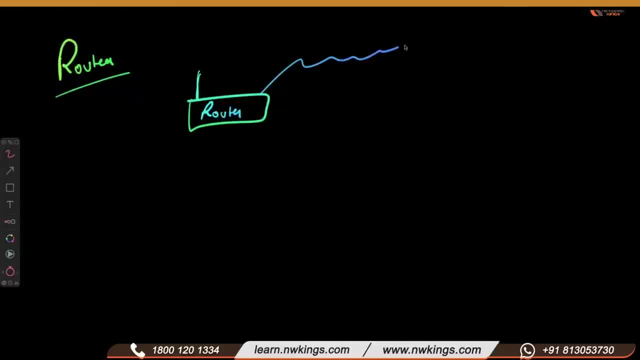 think that this is a router. suppose you have a broadband connection, but this is not a router. this is a, actually a device which is a combo of a router, modem, these type of technologies, and this is what we call adsl device or dsl device. okay, so it. what is adsl? that is a symmetric digital subscriber line. suppose you got a. 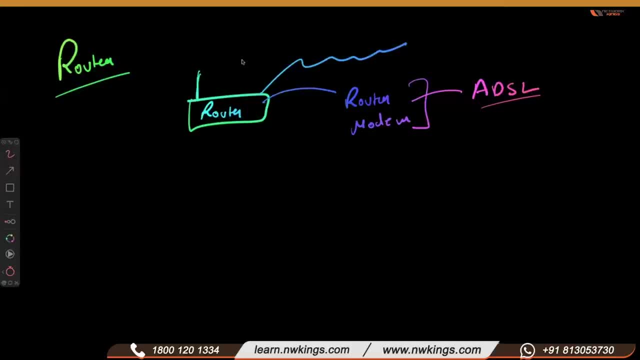 connection from at&t, or maybe you got a connection from atl in india. okay, any from any isp. so the type of device you are looking at right now is a digital subscriber line. now, maybe that device is not a router, so that is a adsl because it has a functionality of modem. 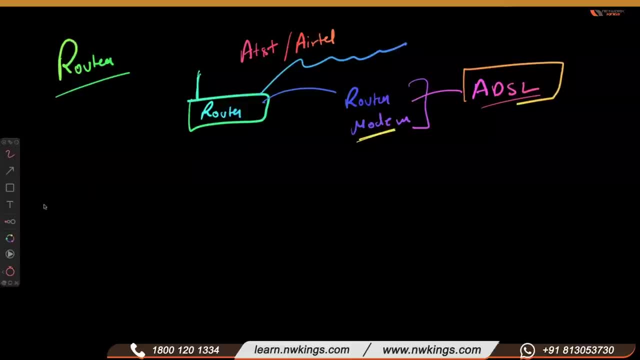 so why we use modem, by the way. so let me explain you. what is modem? so modem is actually doing modulation. so what is modulation? and modem also does the demodulation. and what is this demodulation? so when we get the registration, so when we get the registration, so we get a moving data. 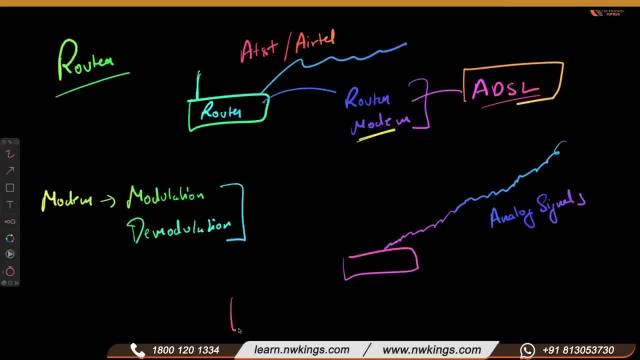 of the data. we will not be able to see any data in the data in the main network, so we will only see the data when it is in the main network. so for that we have to do a modulation of information and we can also see that it is. 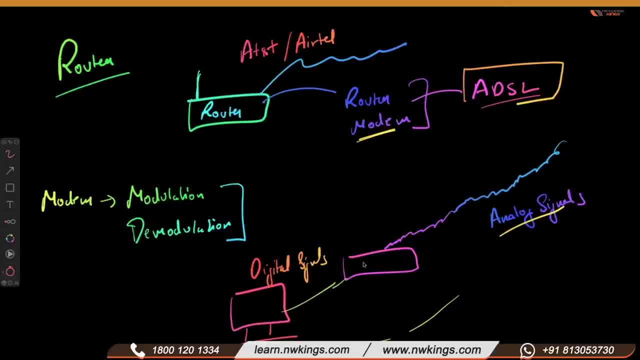 the data. it will be able to see the data and you can also see the signals. you can measure the data to see what type of signals they are coming in- the form of analog signals, right, so when the signals are coming to your device, and your computer understand which signals: digital signals. 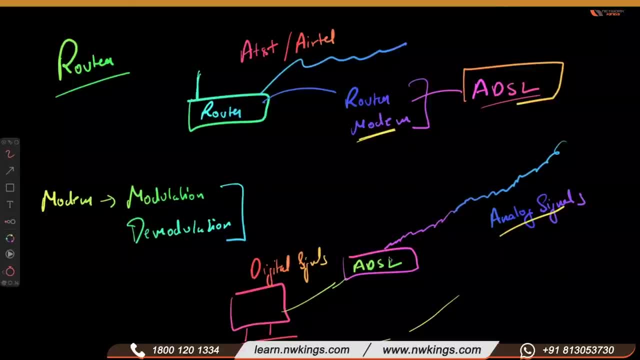 down one device that is adsl. so this device is actually converting your analog signals into digital signals and sending those signals in the form of zero and one and computer understand those signals and the same way it is giving back digital signals and adsl is converting these. 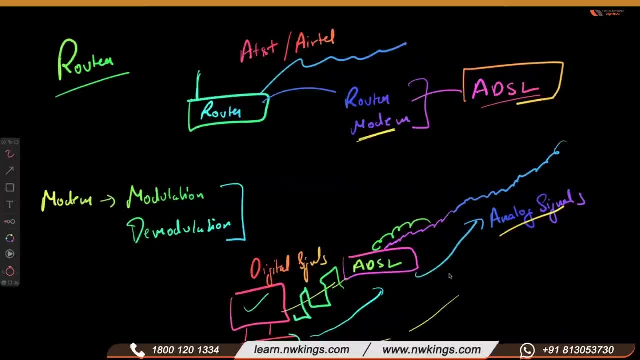 digital signals again back to the analog signal. so this is modem and this modem is actually integrated into this device adsl. and now adsl has one another functionality: router, because this device is actually created for multi-purpose router modem. it has a three, four ports outside also, like it has a small switch inside also. 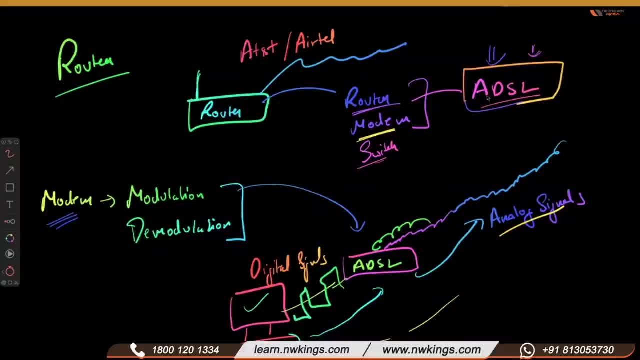 and this is very cheap device which is used by isp to provide the internet connectivity. yeah, it goes with the fiber also, your fiber modems actually converting your light signals, because when you have a fiber or fiber type of modem, the signals are coming in the form of light, right, so that is optical. 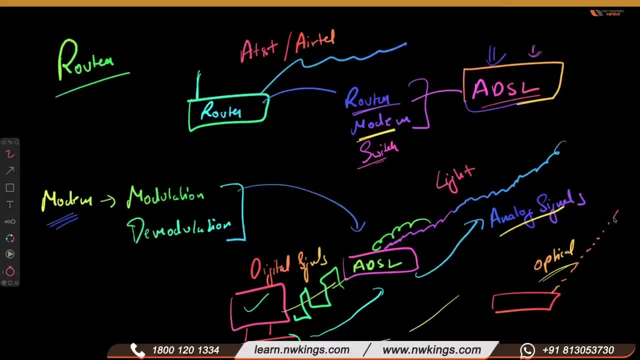 transmission. so when we get any type of communication within the form of signals, that we call this optical, but your computer does not understand these type of things, so we have to convert this into digital signals or electrical signals. so this is what fiber modem does. so fiber modem is converting your light signals into 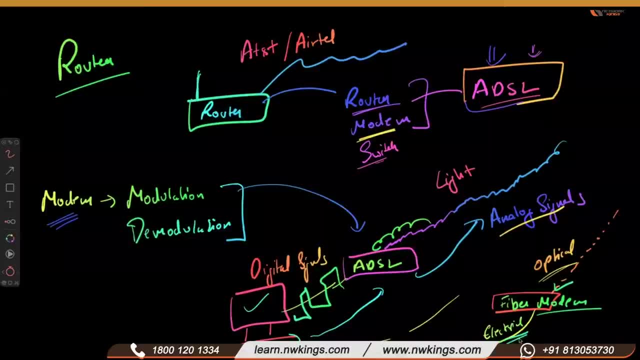 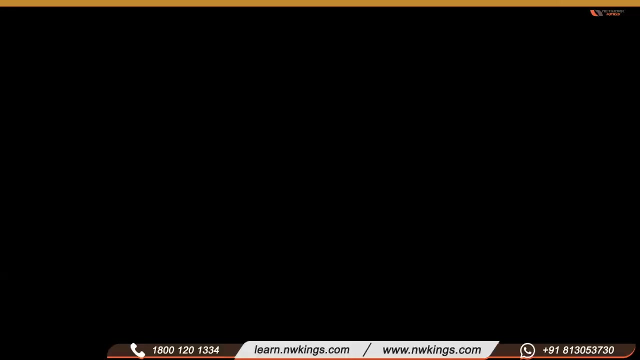 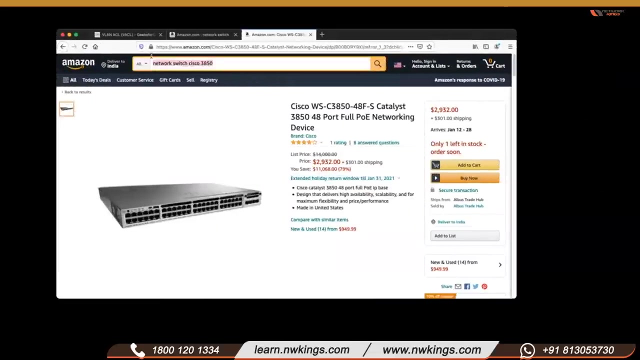 electrical signals. got it? yeah. so himanshu has a question. sir, i have a wi-fi router. these are not wi-fi routers, basically. so if isp has given you something, i'll show you with the example again. okay, just hold on. yeah, so again, see, when we buy adsl. 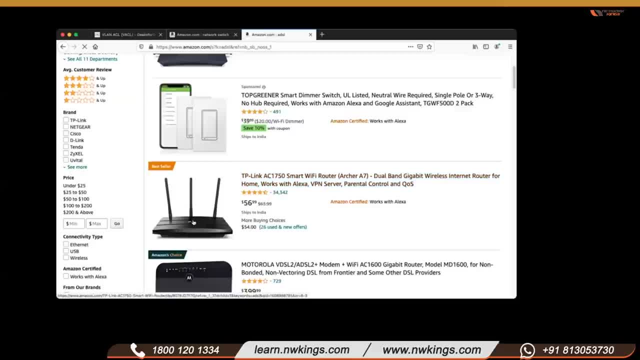 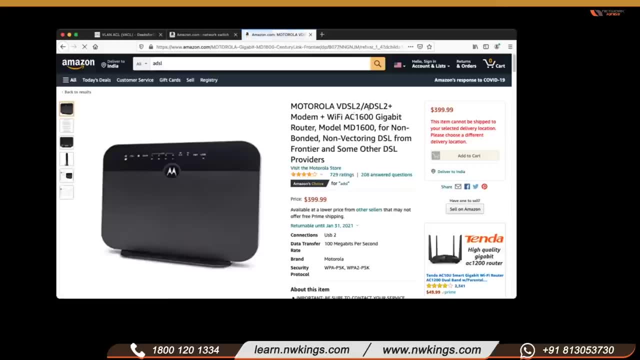 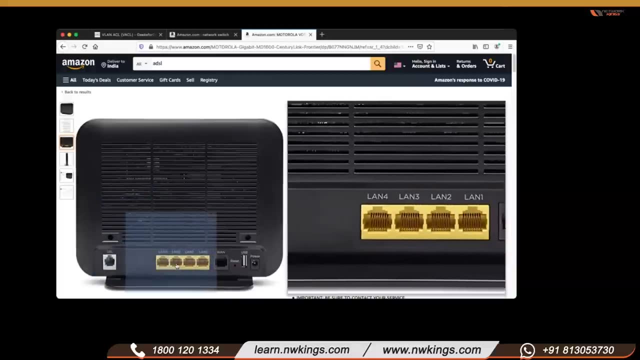 so this type of device is like a router, but it has adsl functionality also, like you can see, this modem. so this is a moto motorola device or with wi-fi. everything is inside and it has a lot. see, you can see the ports. so it is a switch also because it has around four or five ports, so that you can. 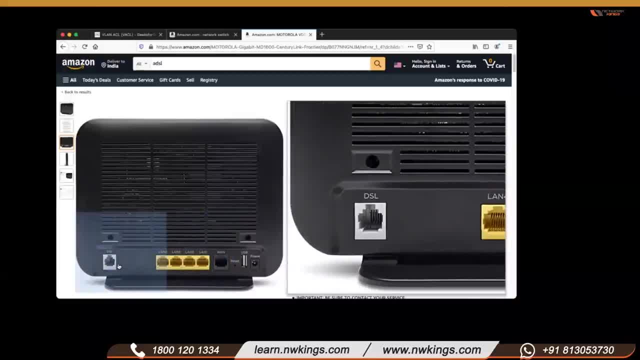 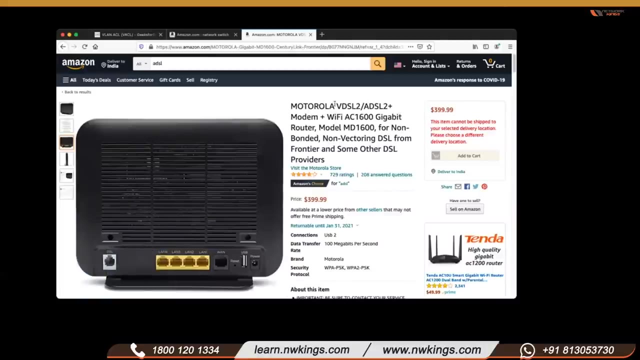 connect to your devices and it has a dsl cable also. this dsl is when we have phone connectivity, uh like from any of the service provider. this, all that cable, is actually giving you analog signal and this port is actually converting your analog signals to digital. okay, so this is adsl device. 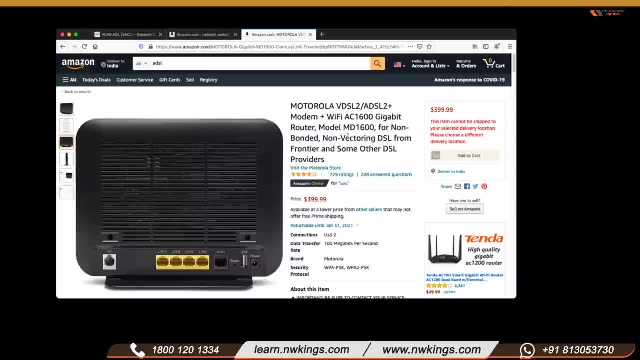 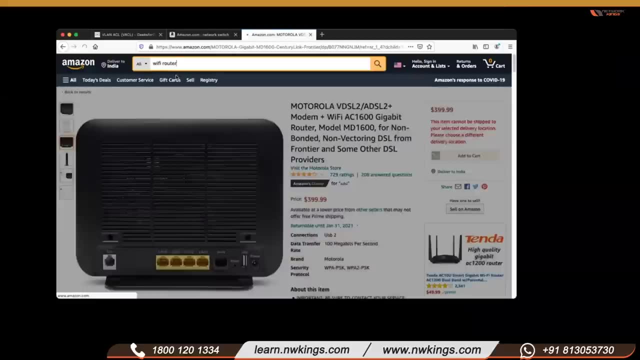 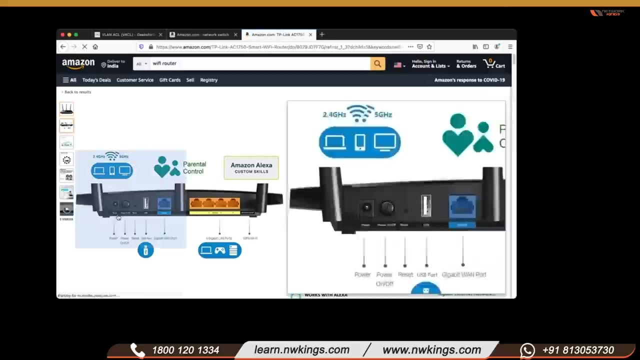 okay, adsldsl, so this is actually a combo of router, modem and somehow switch also okay. and when we get this wi-fi router, okay, so these type of devices like wi-fi router- and let's check the ports, guys, so you can see, here we have only internet cable, but this type of port is not like dsl. 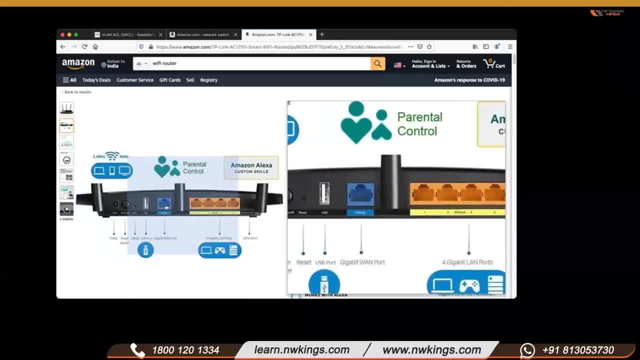 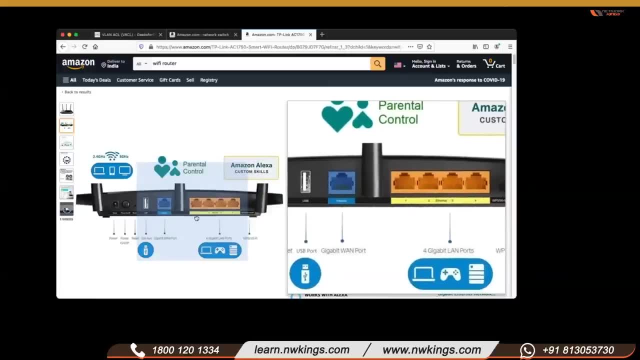 so it means when you are, when you are putting any connectivity here or any type of connection, so isp should give an ethernet link to you. then only you can use this type of device. okay, so what we are going to do is we are going to connect our adl sound to this device. 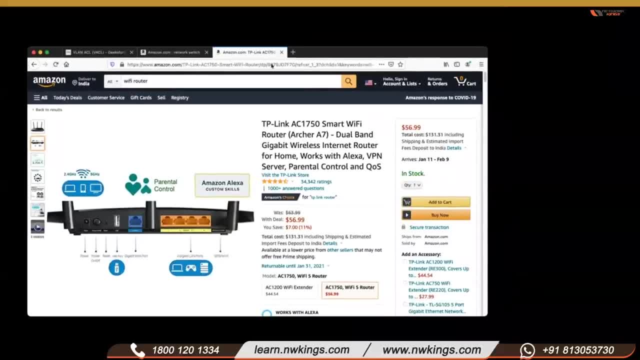 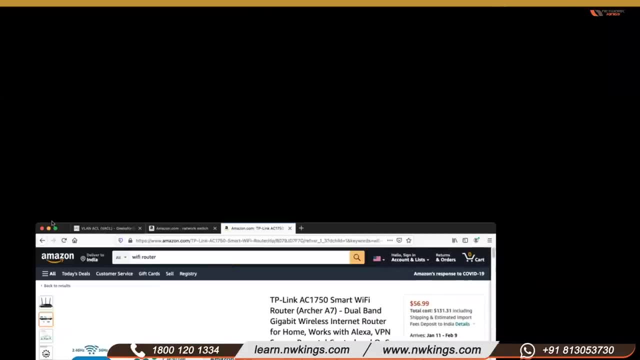 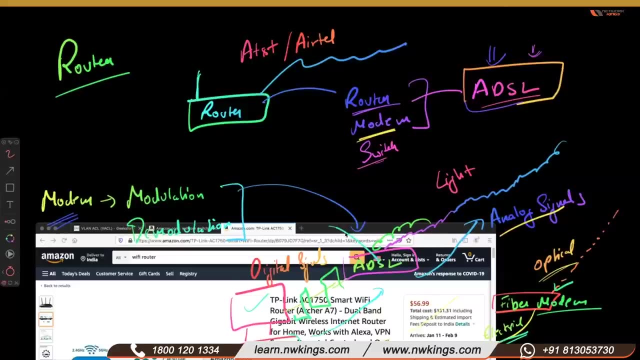 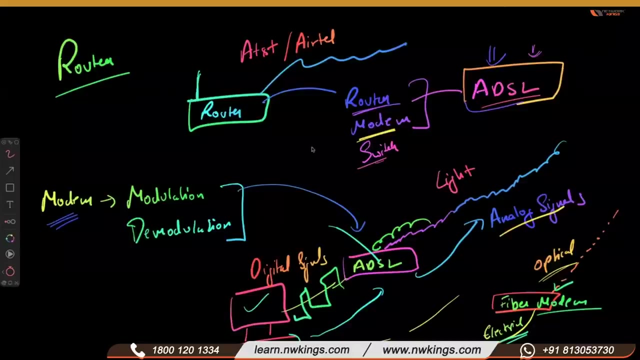 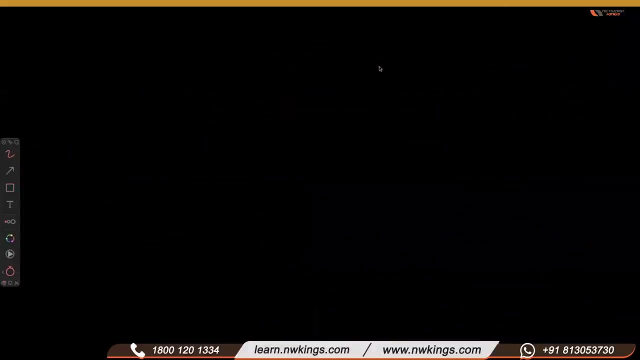 It means let me show you, Okay So, what I was trying to say. okay, so like, okay, so ISP. what is ISP, by the way, Internet Service Provider? okay, So ISP is giving you connection And you have this device, which we call this ADSL. okay, 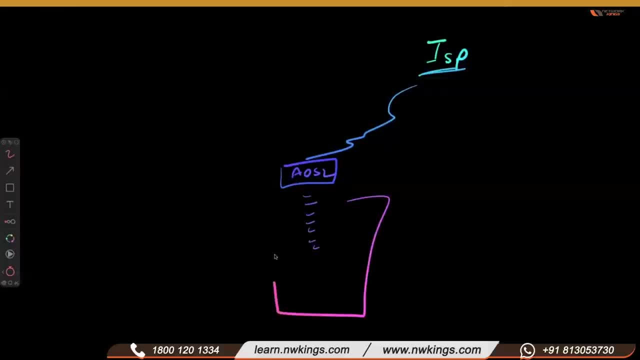 It has a Wi-Fi, but it has a limited range. It only goes up to like maybe 100 square feet area. But you have a big home, Big house, And you want to send these signals to another part of the room. So what you will do, you will put a Wi-Fi router here. 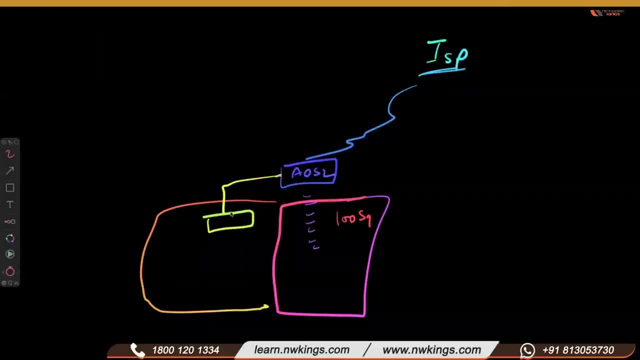 which we have seen right now. So we can just put down one cable and we can place a Wi-Fi router here to extend the range basically. So ADSL is required when you are getting the connectivity in the form of either this type of cable we use to use this PST. 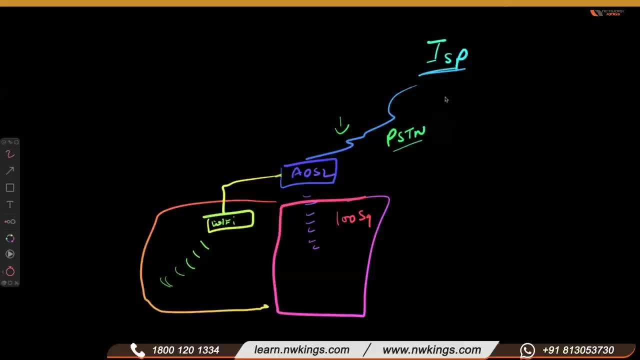 and cable, like public switch telephone network cable, either in the form of fiber. So when you are going to get the fiber connectivity, we are going to use fiber modems, okay, And so ADSL fiber. sometimes ISP gives a direct Ethernet connectivity also. 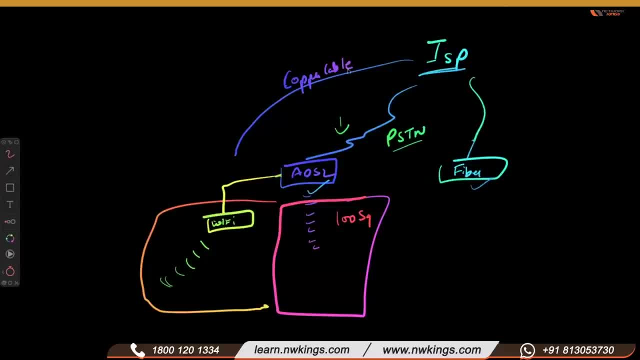 Or what we call this copper cable. Sometimes I have seen this, but it's not common. So this is PSTN. PSTN is common and fiber nowadays is common. Yeah, thanks, Nikhil. Yeah, fiber modems. I explained. 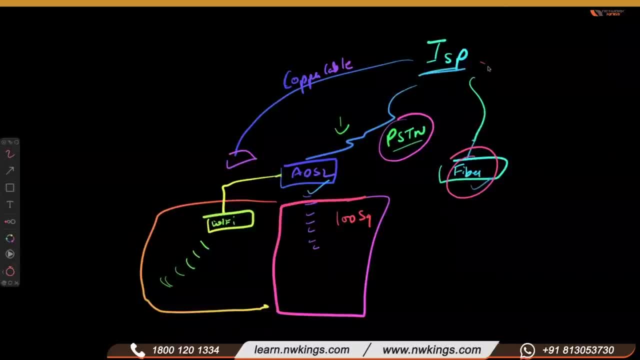 like when any device or any ISP is sending, because light has more speed, right? So when we are sending data in the form of light, right? this fiber modem is actually converting your, your light signals into electrical signals, Because your computer still don't understand what we call this light optical signals. 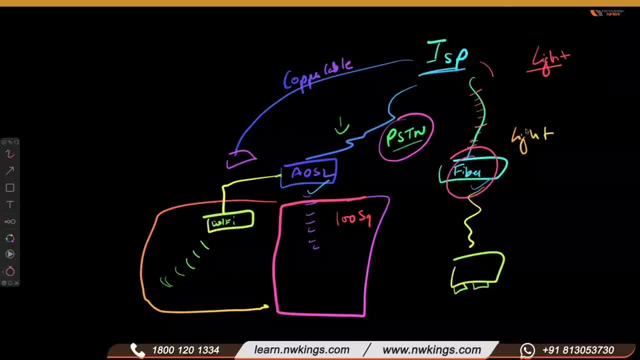 Because your computers does not have that type of chips, those who understand light signals. But when you go into this corporate world, your router actually gets fiber cable directly into the port Means. we can place fiber cables inside our router. we can place fiber cables inside our router. 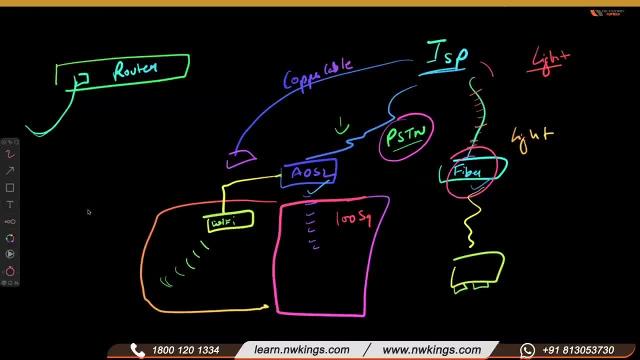 we can place fiber cables inside our router. so how? why we can't put fiber cables in computers? because the router do these type of routers or any high-end devices, or, nowadays, servers or servers also. so they have a small chip that is known as SFP. so this chip is known as small form. 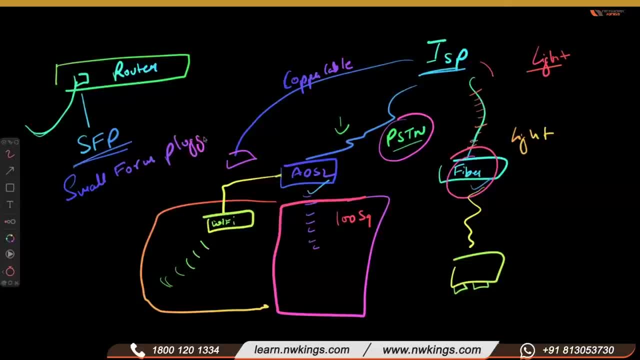 pluggable adapter. so this chip is like a small modem which is helping you out to convert your light signals into electrical signals to the router. are you getting now? so this works like a small modem which actually converge, converting your optical signals into electrical signal. this is the work done by SFP. so 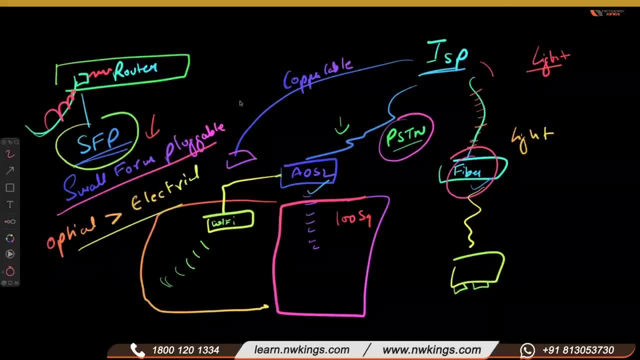 this is the reason we have SFP type of chips inside the router. if you have not seen it, ignore right now. we will see later on. okay, by but high-end devices can like in a server, in a routers we can place fiber cables directly because of this small chips, SFP. 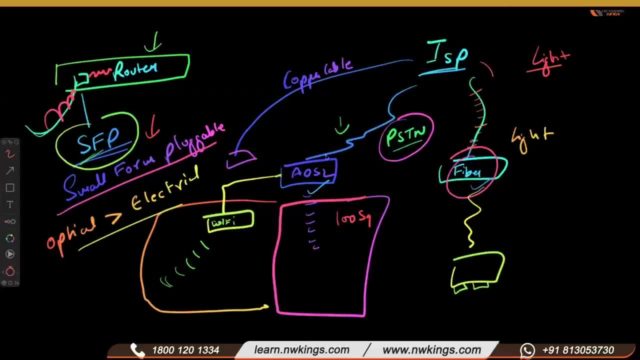 the man should that you have to figure out a DSL, you get, you are getting a DSL, you have four ports outside a DSL and you can just connect a Ethernet cable to your Wi-Fi router and put that device into bridge mode or any type of mode. it will show you the all. 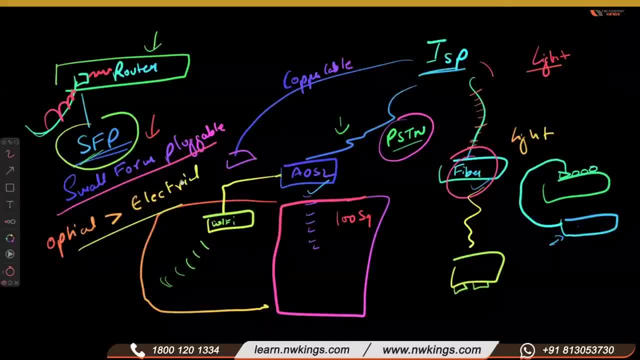 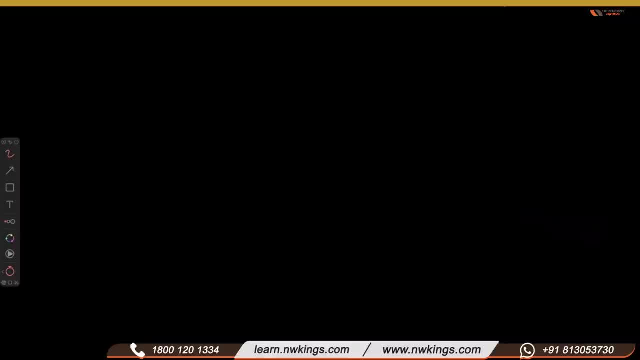 the functionality Wi-Fi router. okay, clear, just say yes, SFP is a small form pluggable adapter. I'll show you what is SFP again. I'll give you real examples of this chip. so this chip is a small form pluggable adapter. I'll show you what is SFP again. I'll give you real example. 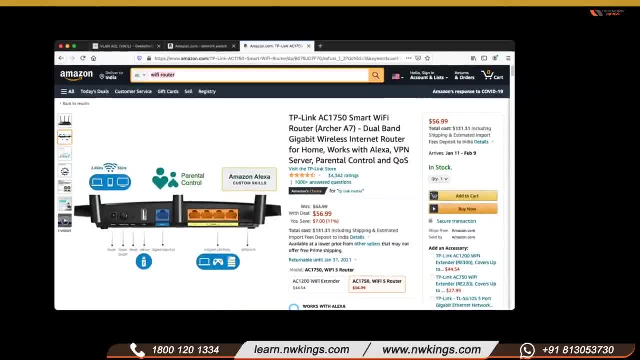 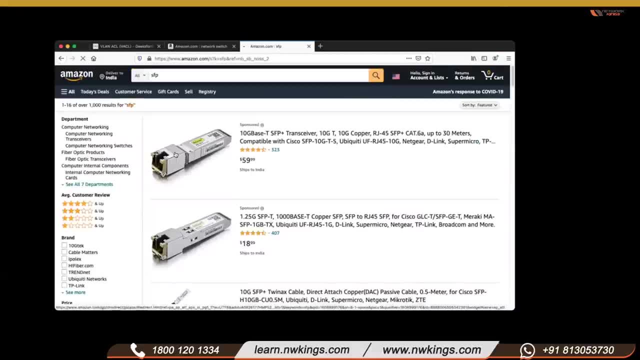 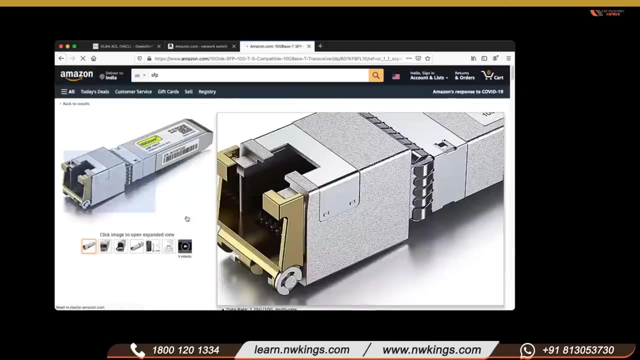 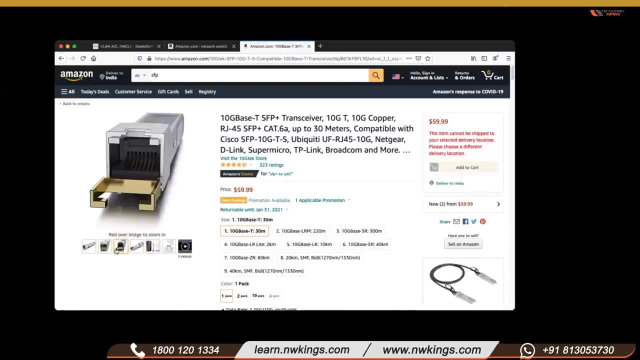 also okay. so I'll show you what is SFP: SFP- okay, so SFP is actually a small chip, or you can say that it's a small part. okay, so we're. so. this part is actually. we are putting this part inside the servers, routers- so that it can convert optical. 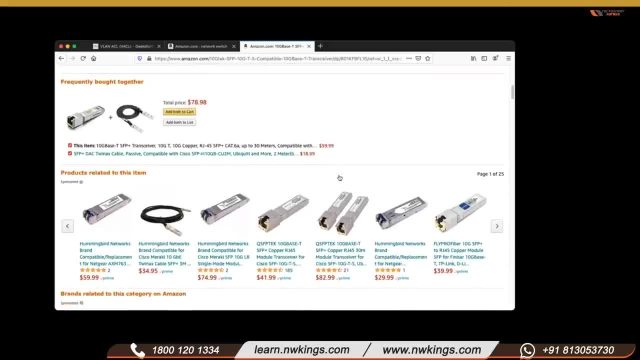 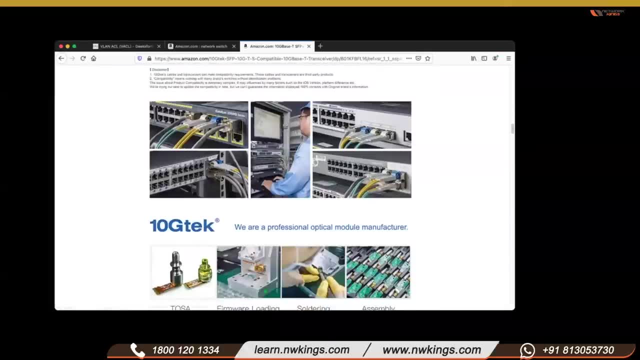 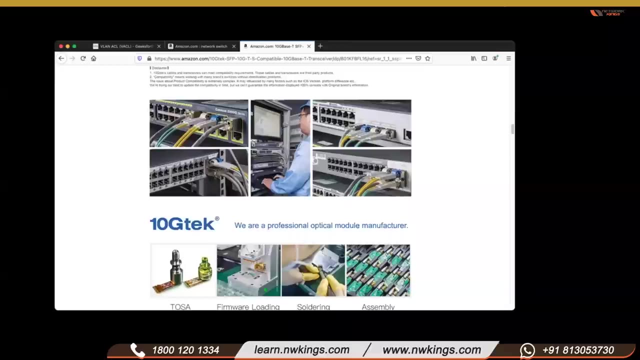 signals into electrical signals because we can't put optical signals directly into the devices. so you can see here all the Cisco devices or all other company devices are using these type of ports. we are not putting directly fiber cable into the device because we are putting this SFP first and then we are 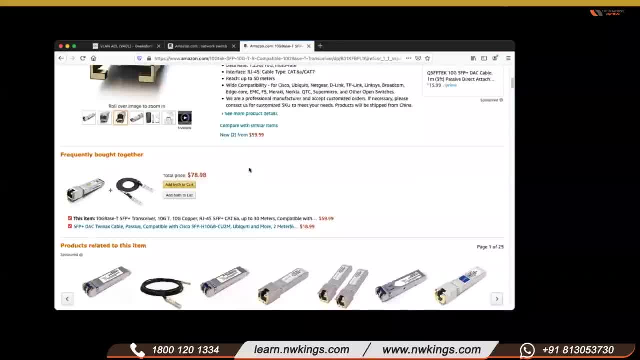 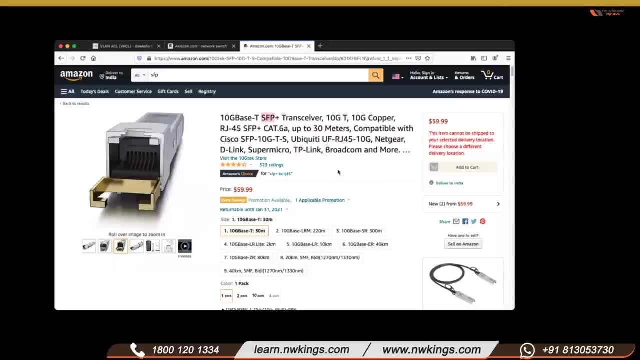 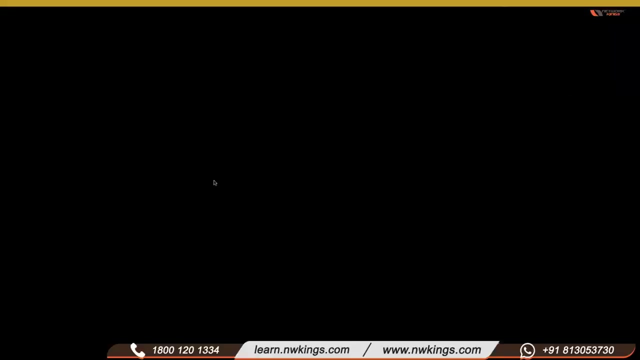 putting or adding the cable. clear: what is the SFP plus? SFP plus means 10 GB, SFP is 1 GB, SFP plus is 10 GB and this is the and this is the with you and this is the. okay, you, okay, you okay. 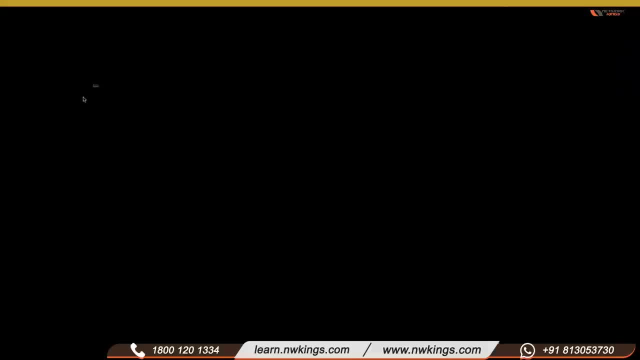 okay, fundamental class okay, yeah, so so I have explained you what is a router switch also. okay, I'll show you something interesting so that I always show to my students. so just hold on, no, Avinash. so Avinash Avinash is asking something that it has 250 computers like. 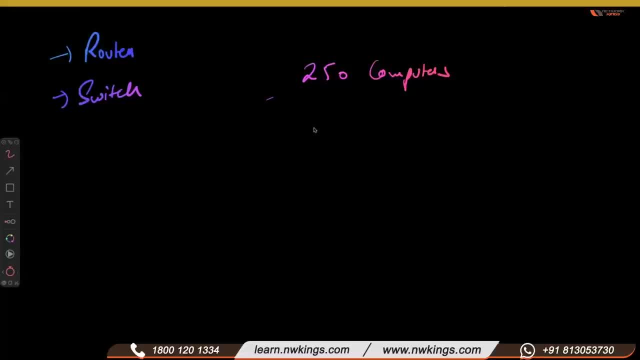 250 computers. okay, so all these computers are actually suppose these are 250 computers. okay, so all these computers are actually suppose these are pieces. okay, so all these pieces have one chip, that is known as all machines. all laptops have one card, that is known as an IC card. so that is network. 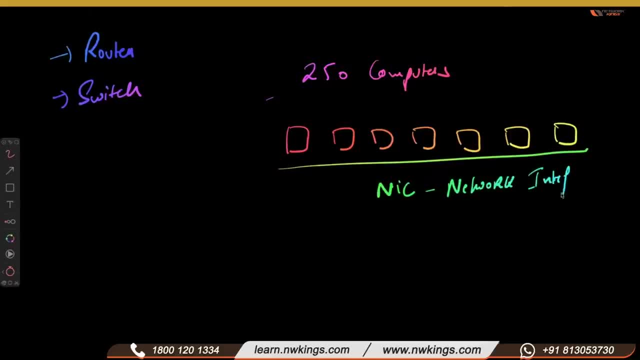 interface card so you can check your laptop. right now you may be having some port where we can put down the cable, or maybe you have wireless right? why? maybe you all you should have this wireless card. so all these chips are known as an IC with an IC. so either we have wide NIC where we can put down our cable and we have 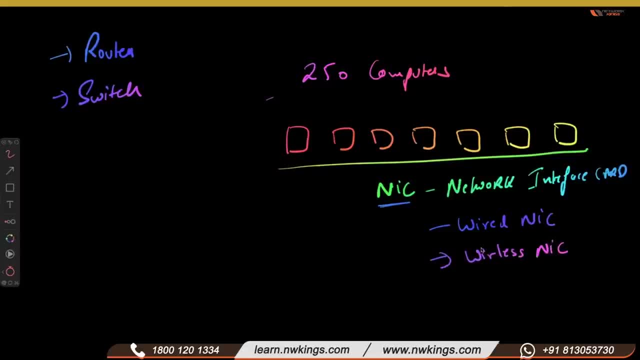 wireless NIC. so what is this NIC? NIC is a chip or any type of part which is actually helping you to connect your computers with the network. okay, so you're adding the network cables into the computers and where we are presenting it with a, you know, aized computer. 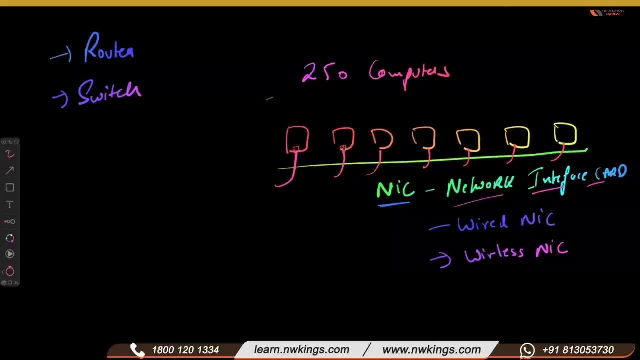 So let me explain this a little bit. Okay, you can see that here. you can see here that it has св4 works. there's no work and are adding these cables in a small uh like. this chip is nowadays integrated in the motherboard, so we don't have to add this, but a few years back we need to buy a separate card to install. 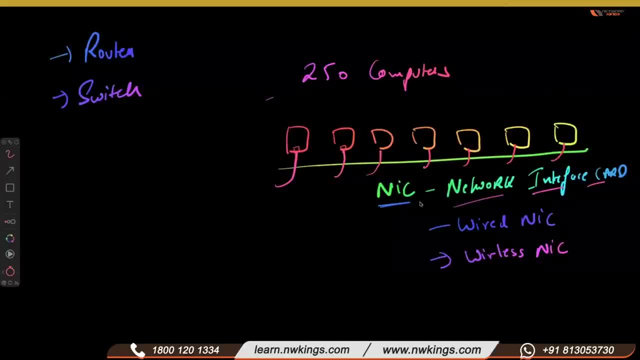 in the pieces, but nowadays it's pre-installed into the motherboard. okay, yeah, yeah, nic card is basically your ethernet port. yes, when we say we have ethernet port in our laptop, that actually means it. it's a nic. and do you know that you? your computer does not have any mac address. 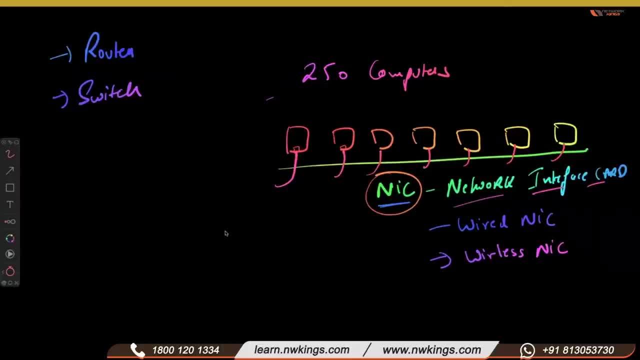 your nic chips have. it means if my laptop has wired. nic means and wireless nic and a bluetooth adapter, bluetooth and ic. bluetooth means also nic. so it means if i have three things in my laptop, it means how many mac address we will have three mac address. okay, because this this mac address when we say mac address, so this is not a address. 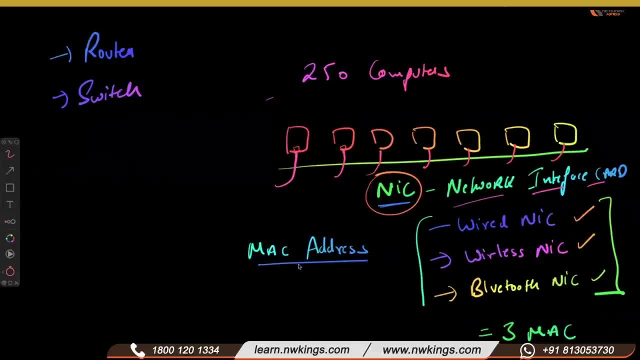 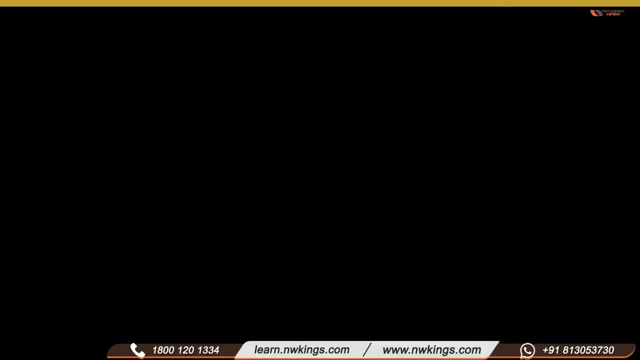 which we are giving to any computer or machine. this is a hardware address, which is actually address of these chips. either it is a bluetooth, wireless or void, okay. so if somebody is asking you how many mac address you have in your laptop, just count the nic, okay. so, nic, you can count, or you can check with the help of which command ipconfig. 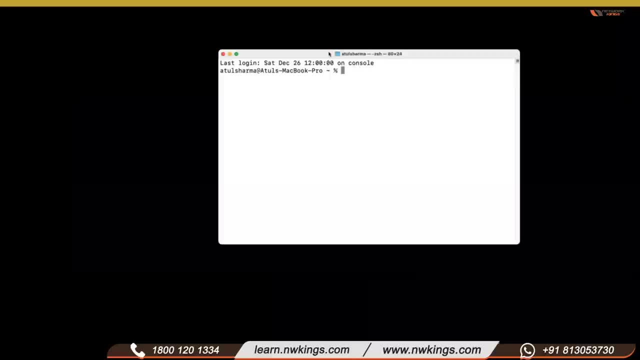 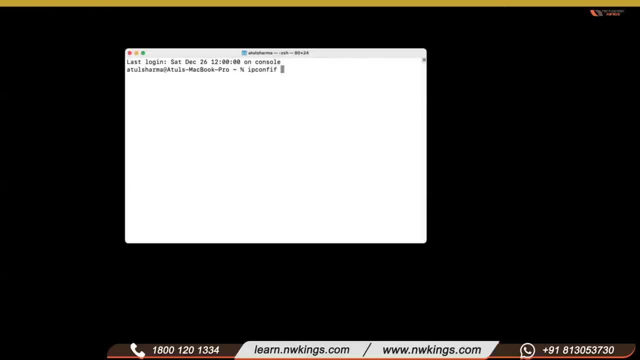 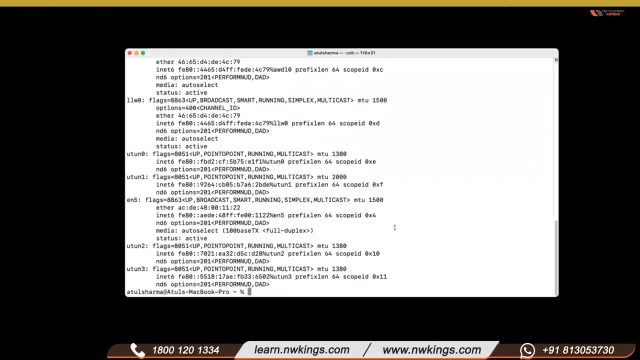 okay, so i'm using macbook here, so i can. so if you are using windows, you can type ipconfig right now and you can see all the details. or your, uh, your, yes, your, nic. so i'm in linux and in macbook we have if config. okay, so in if config. 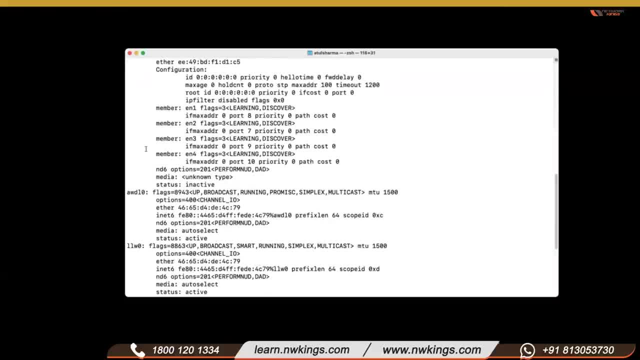 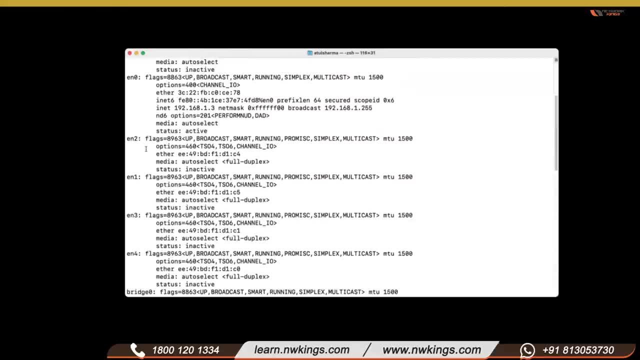 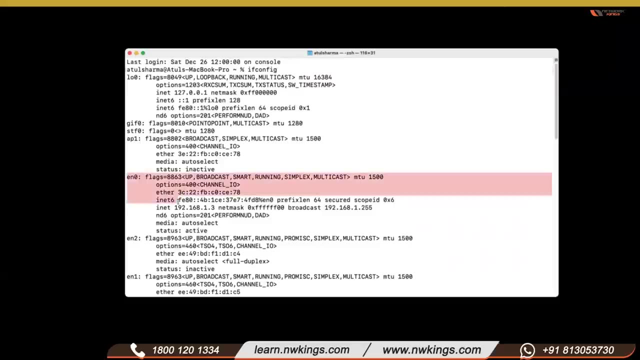 so you can see a lot many ports here, because some are virtual ports. okay, virtual means uh that is created just for uh for the virtual purpose, like vmware, and all right. so you can see here en0. so my computer is getting this ip address right now: 192 1968 1.3. 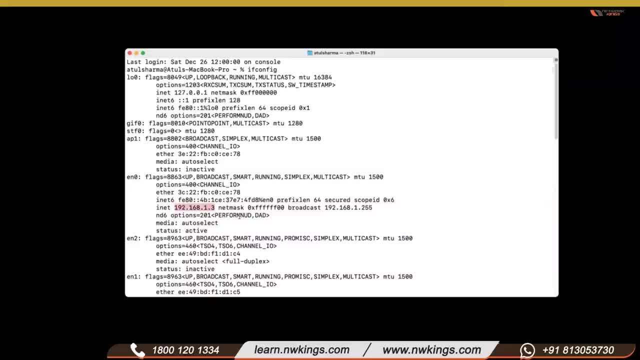 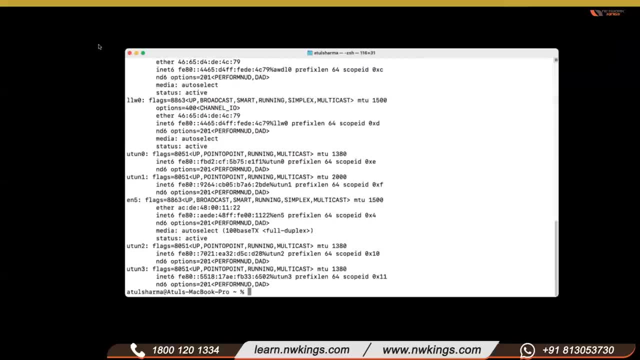 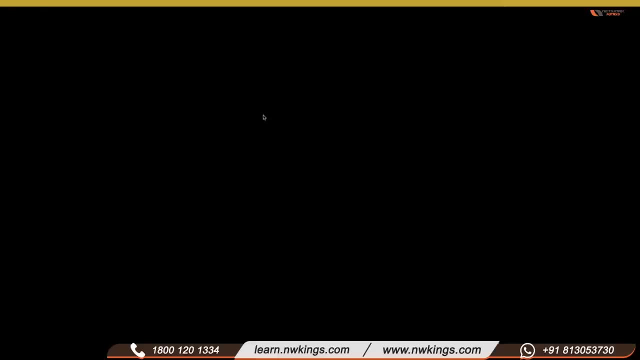 okay, so you can use ipconfig okay, yeah, yeah, i'll explain mac address, don't worry. okay, you can also go to macbook in youtube. you can do that and say when you are in macbook and say: if i want to do my apk, let me go to macbook. 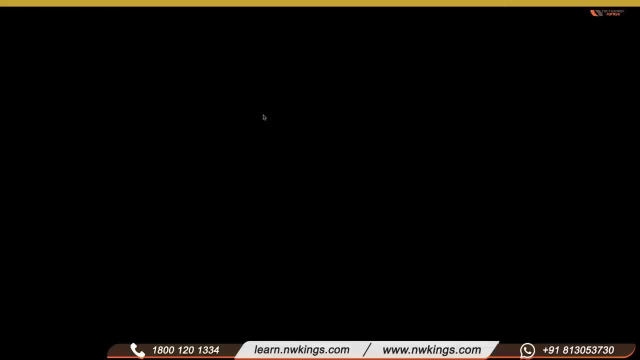 or if you are into macbook, um, you can use to do my ip address. let's say, if i wanted to be a hybrid but you are using macbook. let's say, if i was using macbook, this would be my ip address. let's say, if i wanted to be a hybrid at that time, yeah, 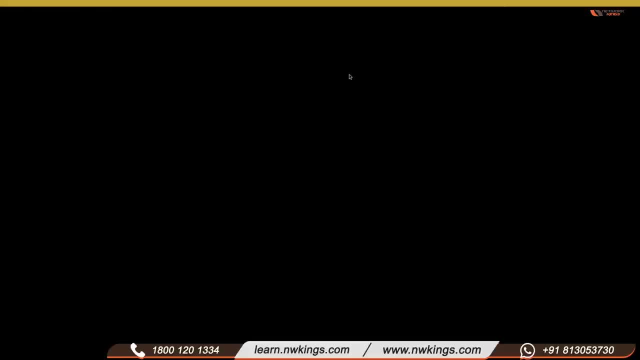 i don't want to go to macbook. i can go to macbookничinis, for example, and i can see the position of macbook. so it's written in macbook, okay. yeah, so i was discussing the question. so we have around 250 computers, remember. 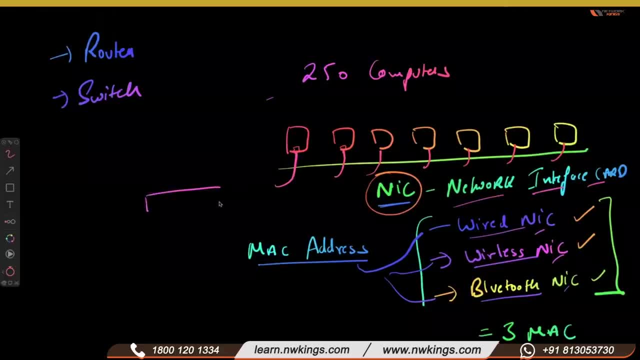 yeah, so when we have all these devices are connected with the help with the device, we call this switch. okay, all the cables are going inside this device. this is switch right. so these suppose these type of nic have a speed. uh, nowadays we have. we got one gbps, but 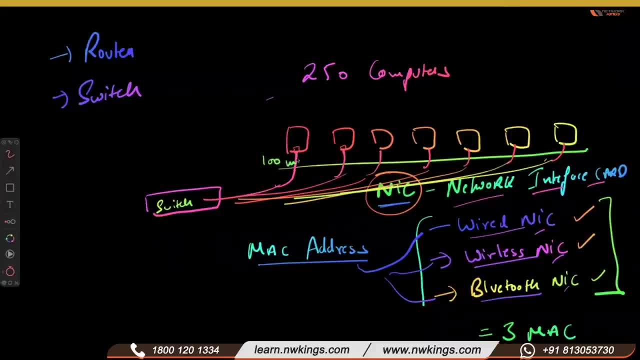 a few older laptops have 100 mbps, so suppose all the ports. so do you know what is kbps, gmbps and all these things? so just a quick overview. so we have zero and one. these are known as bits. okay, so when we have eight zero ones, when we count, eight zero or ones, either it would be. 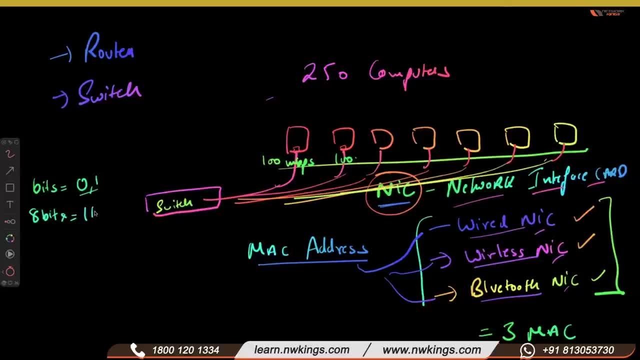 zero or one. that eight bits are known as one byte, so like zero one, zero, one. one one, zero, zero. so what is this? this is one byte, okay. so when we have eight zero and ones computer understand this, one byte, okay. and when we have one zero, two, four bytes, when we have 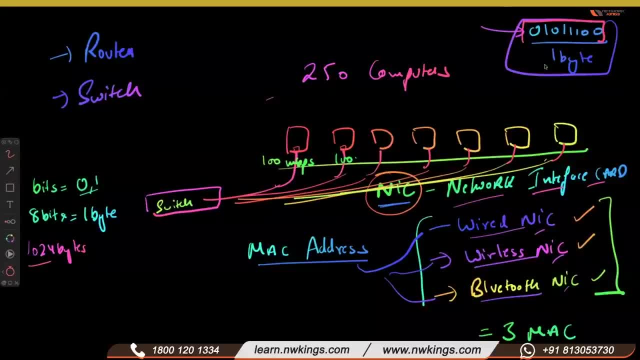 combo of this is a group which is byte. when we have one zero, two, four similar zero ones, that is known as one kilobyte. okay, obviously, then you know kb. and when we have one zero, two, four kb, we say this, what we call this: one mb, megabyte, and then we have gigabyte, terabyte, petabyte, hexabyte. 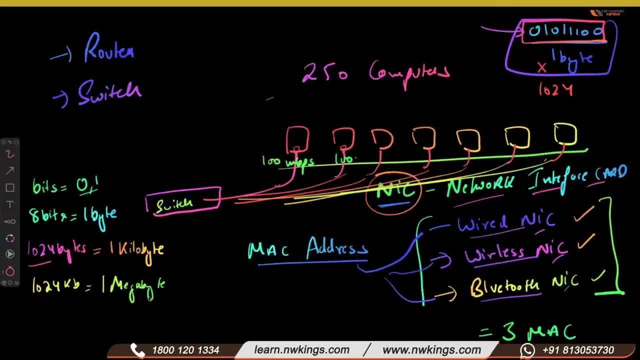 hexabyte, zettabyte, a lot of many bytes. okay, so you can check this on google, but yes, you understand this. bits, eight bits is one byte and one zero two, see one. uh, i was taking one interview few years back and just i asked one: what is one byte? 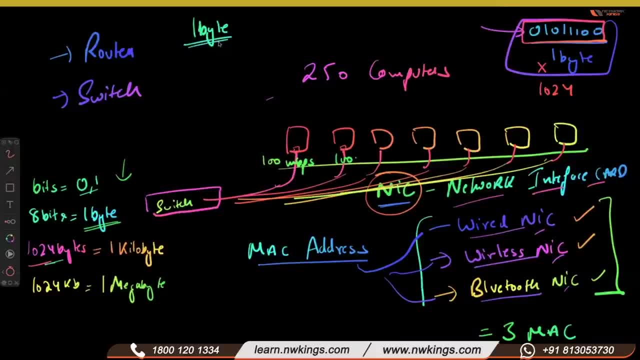 so even that person can't able to give that, and so he was saying eight bits. so i was just asking: what is eight bits? so that was a actually answer. zero ones are actually bits, right, so zero and one are bits. so it happens sometimes. you know, but you can't in interviews you got. 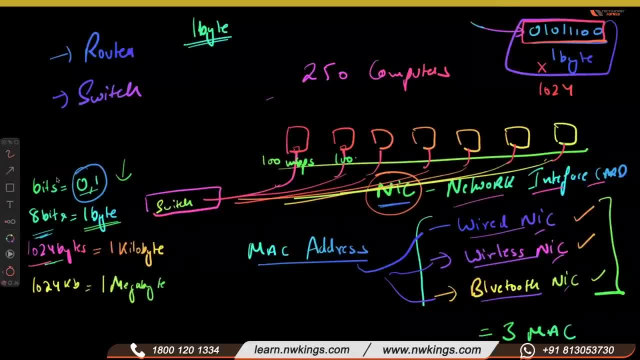 black and white. so it happens sometimes, you know, but you can't in interviews. you got black and white, okay, so so now, if all my devices are 100 mbps, right, so how much throughput they will get? what is throughput means how much data they can send or receive. maximum 100 mbps if my computer has. 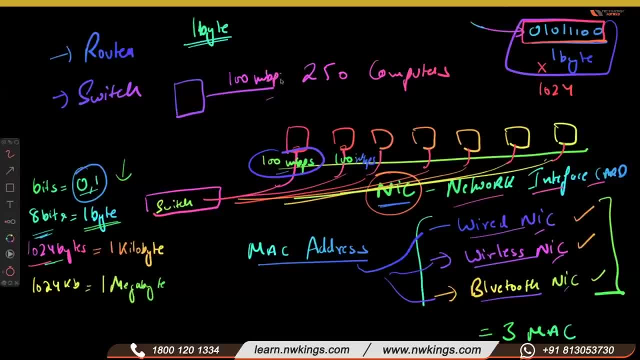 100 mbps. what is the maximum throughput? throughput means how much data i can send or receive. what is the maximum throughput? throughput means how much data i can send or receive. that is throughput. so how much data this device maximum send or receive? 100 mbps. right, that is the. 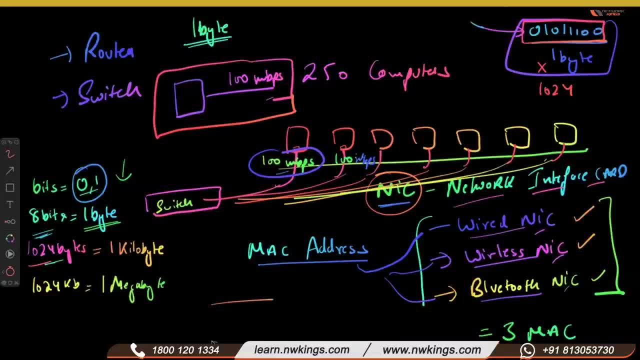 same example. uh like, uh, we are. we have a pipe from where we are transferring water or something right, so we can. uh, when the pipe is broad, then we can send or transfer a lot of water. but we can send over water by giving small preserve packs, but when the pipe is smaller we can. 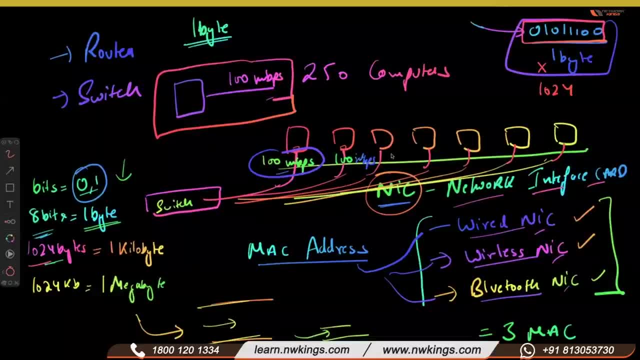 share small amount of water, right? so this is what i'm trying to explain this. all, all your computers are like 100 mbps. they can only get maximum 100 mbps and you got a internet connection of 1 gbps. tell me how much maximum speed these computers will get? tell me. 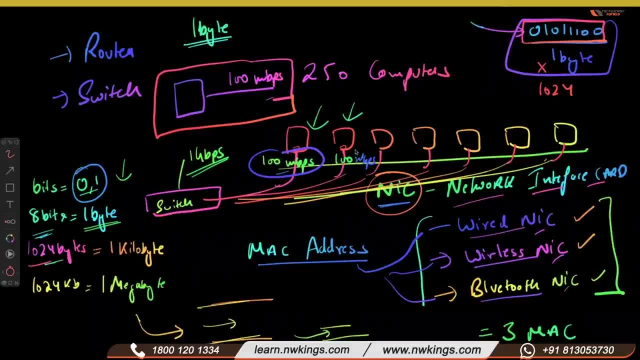 you have 1gbps internet connection. one gbps connection, how loved face the half, a 100 mbps. can you please be kind to me because because i'm turned off, because it is pessoal to end chain internet connection, but your computers have 100 mbps, so what would be the maximum speed you will? 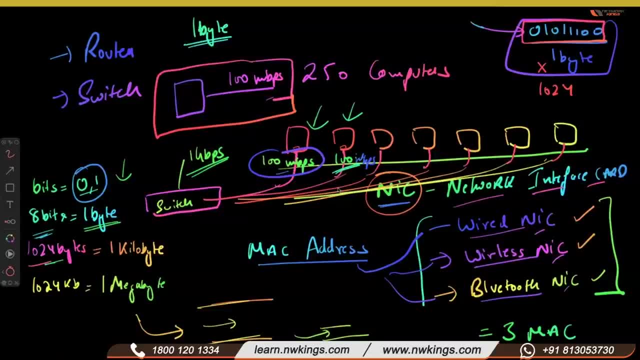 get. yes, correct, 100 mbps, right. so that is exactly throughput means. and let's take another example. let's take another example: when you have one gbps, all your ports have one gbps, but they are using 100 mbps connection. so what would be the maximum speed these devices will get? 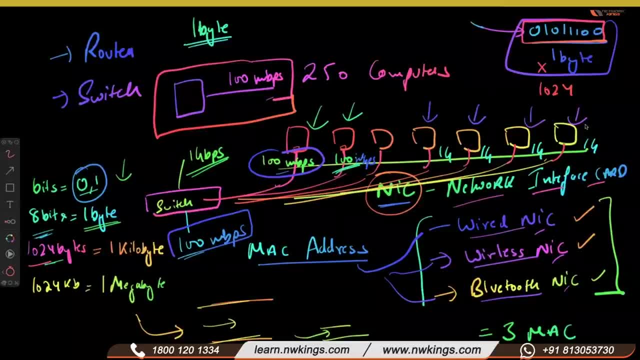 again 100. right, because you are going to internet. but when they are sending data to each other, they are sending data to each other or they are sharing data between them- how much data or how much throughput they will get? yes, one gbps. correct, correct, very good, cool, clear, okay, good. 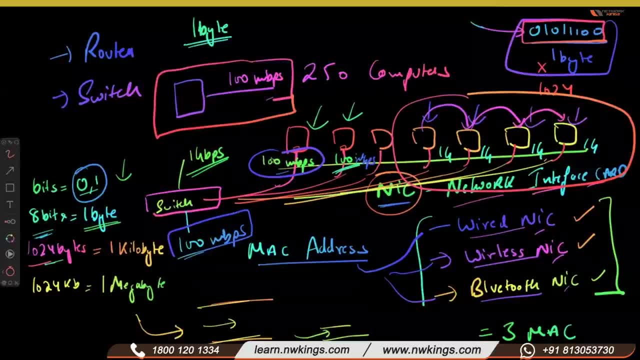 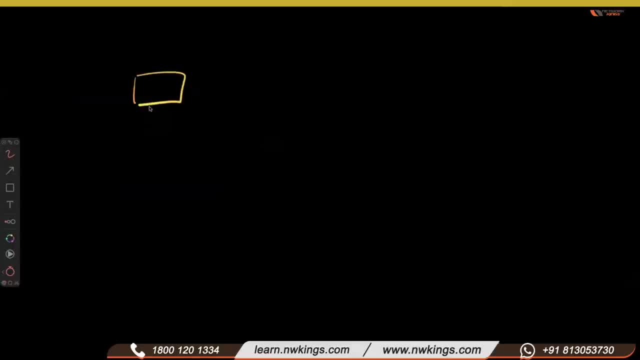 okay, so explain again. okay, so explain again. okay, don't worry. so i was saying so. this is my computer, okay, okay, so i'm getting internet connection of one gbps, but i have a chip in my computer which is only supports 100 mbps. that is so 100 mbps- sometimes we call this 100 mbps fast. 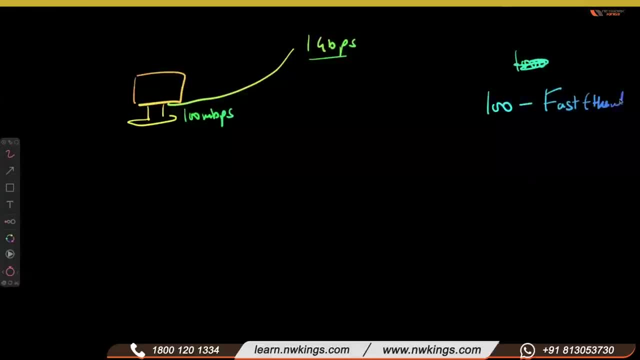 ethernet. so i'm getting internet connection of one gbps, but i have a chip in my computer. okay. so when we use one gb or one gb connection, so we call this one gigabyte or giga ethernet. okay. and when we have 10 mbps speed, which is very obsolete, but we call this ethernet. 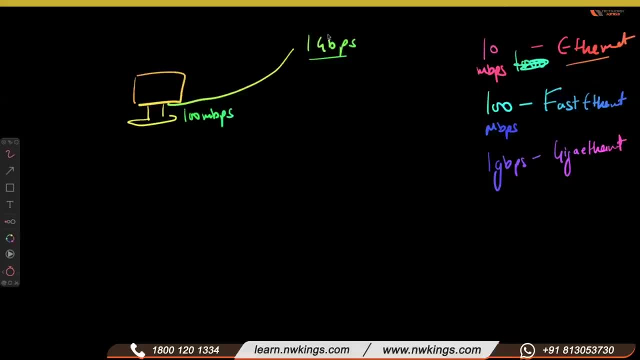 okay, ethernet. so i'm asking: you have an internet connection of one gbps. you have a device here which is giving you whole one gbps, but your computer supports 100 only. okay, so you can't have speed more than 100 mbps. so i'll give you one another example. so 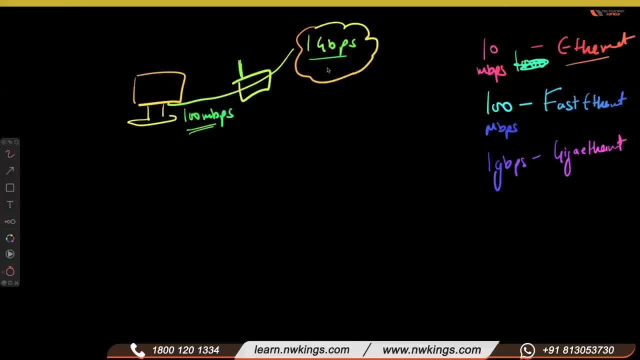 all devices should have good speed, right? suppose you have one gbps, okay, and your computer has one gbps, but you have a device which is giving you whole one gbps. so you have a device which is giving you whole one gbps. so you have a device which is giving you whole one gbps. so you have a device which is only supports 300 mbps. 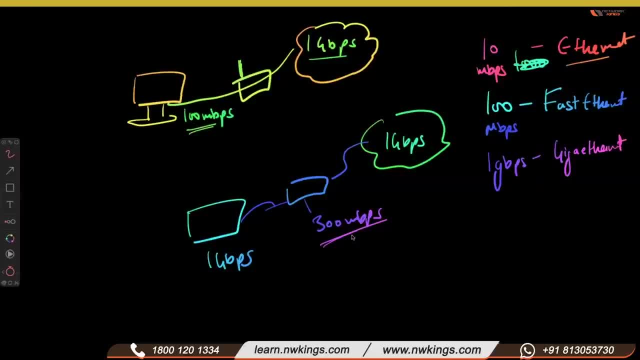 which is only supports 300 mbps, which is only supports 300 mbps. so tell me how much speed you will get. so tell me how much speed you will get. so tell me how much speed you will get maximum 300 right. maximum, 300 right. 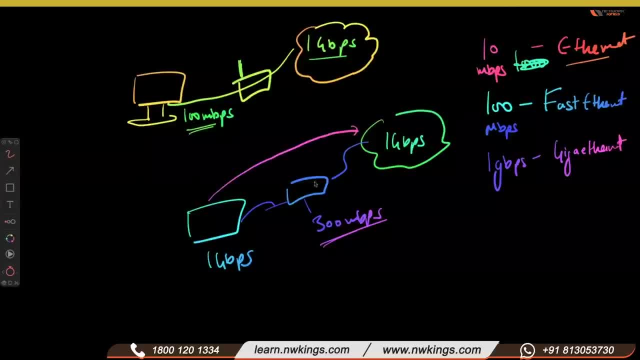 maximum 300. right because? because, because between the transmission, between the transmission, between the transmission: if any device have low bandwidth, it, if any device have low bandwidth, it, if any device have low bandwidth, it means you are going to get the same, means you are going to get the same. 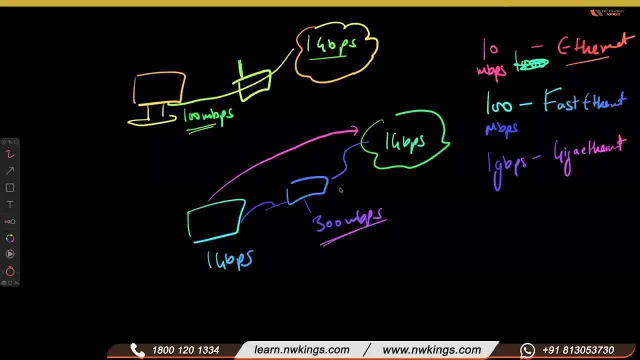 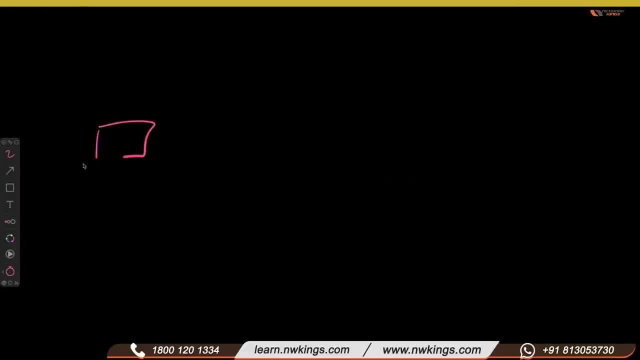 i'll show you one thing. i'll show you one thing. so just let me show you one thing. suppose, so just let me show you one thing. suppose, so just let me show you one thing. suppose you have very good laptop. you have very good laptop. you have very good laptop, right, macbook, and you have one gbps port. 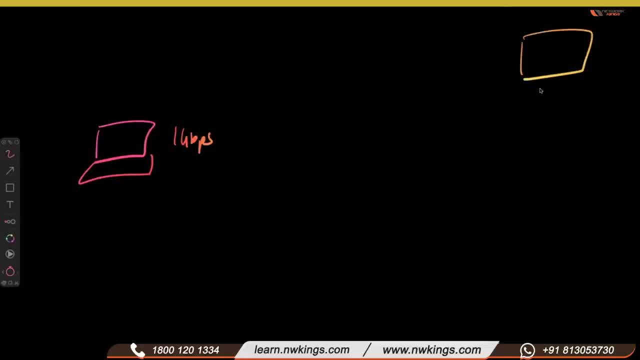 right macbook and you have one gbps port. right, macbook and you have one gbps port. you got an internet connection also. you got an internet connection also. you got an internet connection also. uh suppose 100 mbps okay. uh suppose 100 mbps okay. 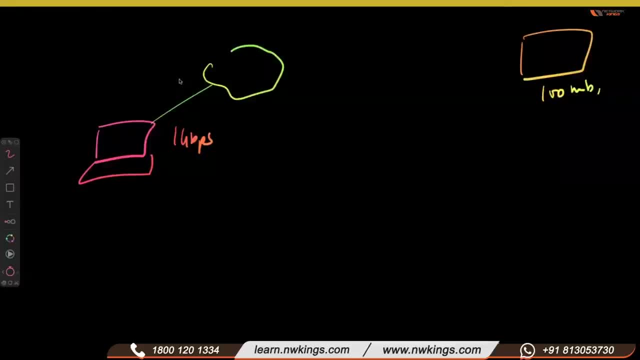 uh suppose 100 mbps. okay, you got an internet connection of 100. you got an internet connection of 100. you got an internet connection of 100 mbps. okay, so you are paying 400 mbps. mbps- okay, so you are paying 400 mbps. 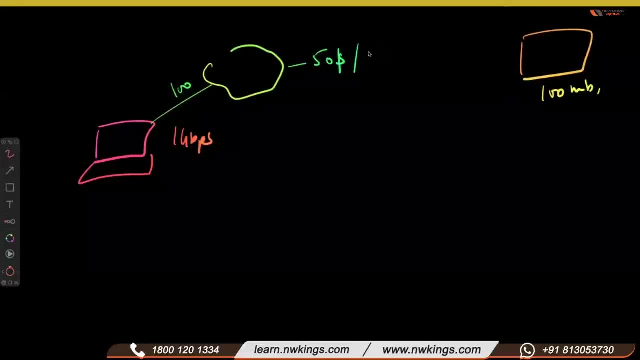 mbps okay, so you are paying 400 mbps plan. suppose you are paying 50 dollars plan. suppose you are paying 50 dollars plan. suppose you are paying 50 dollars or approximately 2000 indian currency, or approximately 2000 indian currency or approximately 2000 indian currency. so you are paying for this internet. 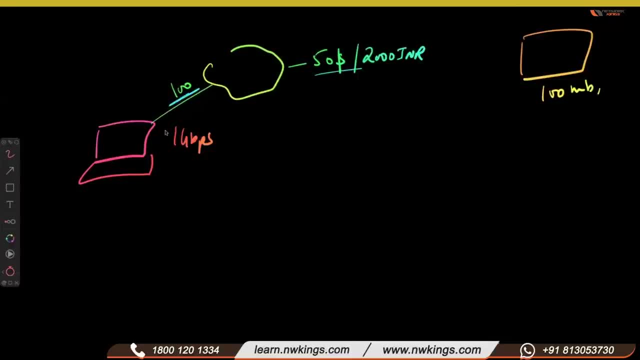 so you are paying for this internet, so you are paying for this internet connection, but you think that connection, but you think that connection, but you think that you are getting 100 mbps connectivity. you are getting 100 mbps connectivity. you are getting 100 mbps connectivity. okay, and when you are watching a video, 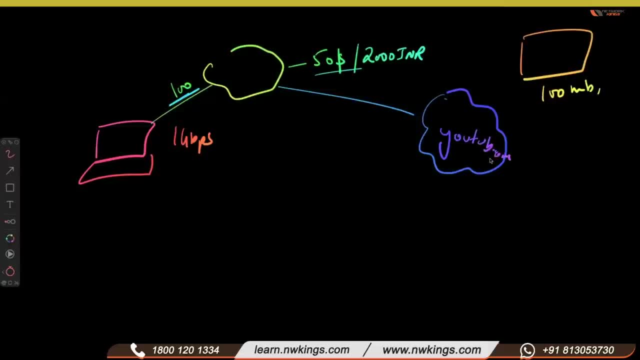 okay, and when you are watching a video: okay. and when you are watching a video from youtube, from youtube, from youtube, but you are getting a delay means it, but you are getting a delay means it. but you are getting a delay means it keeps on buffering, keeps on buffering. 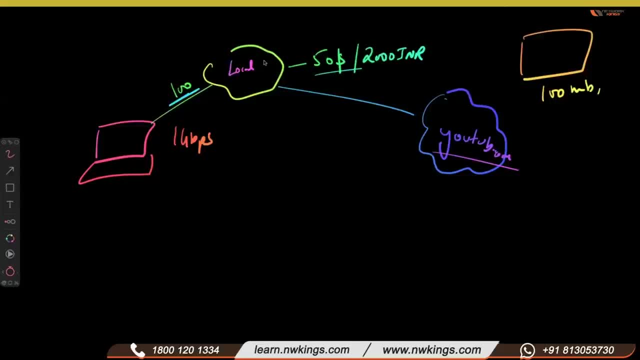 keeps on buffering and you always complain to this local isp and you always complain to this local isp and you always complain to this local isp. man, you have given me 100 mbps, but my man, you have given me 100 mbps, but my man, you have given me 100 mbps but my i'm not able to watch this youtube in. 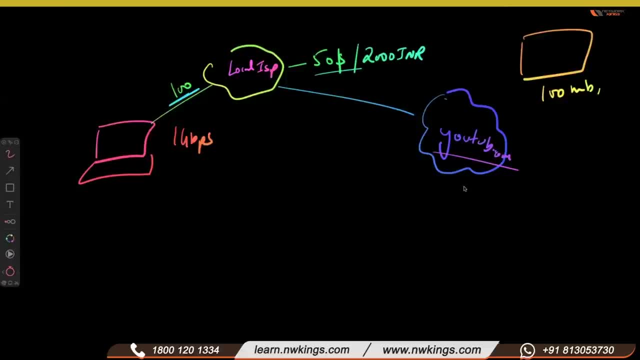 i'm not able to watch this youtube in. i'm not able to watch this youtube in 720 pixels or 1080, 720 pixels or 1080, 720 pixels or 1080. why? why? why? because maybe this local isp giving you, because maybe this local isp giving you. 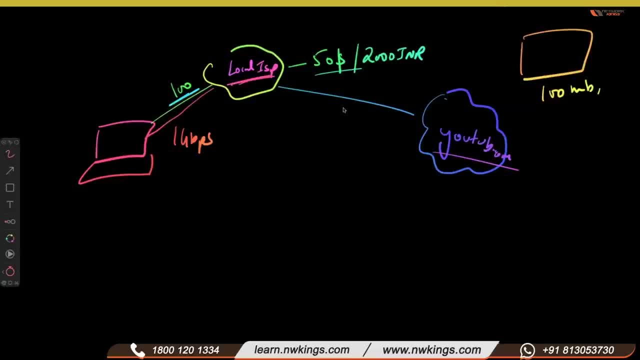 because maybe this local isp giving you 100 mbps link here, 100 mbps link here, 100 mbps link here, but maybe they have a 100 mb or maybe low, but maybe they have a 100 mb or maybe low, but maybe they have a 100 mb or maybe low bandwidth link over the internet. because 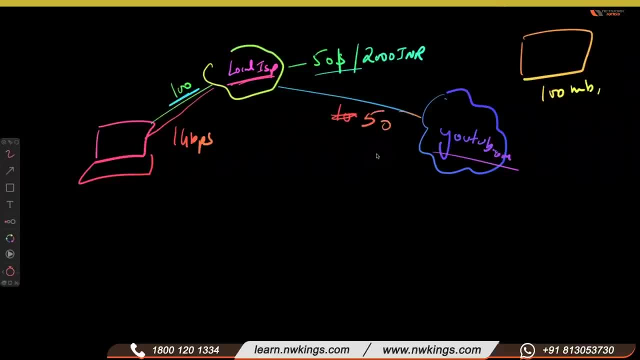 bandwidth link over the internet. because bandwidth link over the internet, because they are also taking connection from, they are also taking connection from, they are also taking connection from somewhere, somewhere, somewhere. so this is the trick actually played by. so this is the trick actually played by. so this is the trick actually played by local isp. 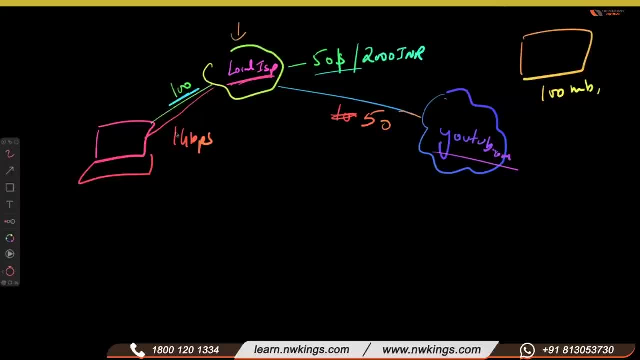 local isp, local isp, right. so they say one gbps 100 mbps, but right. so they say one gbps 100 mbps, but right. so they say one gbps 100 mbps, but uh, when you actually do the speed test, uh, when you actually do the speed test, 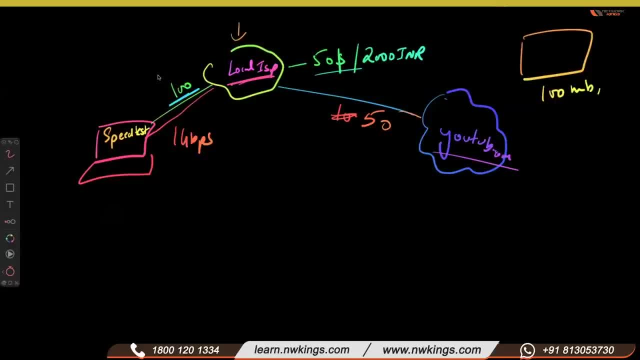 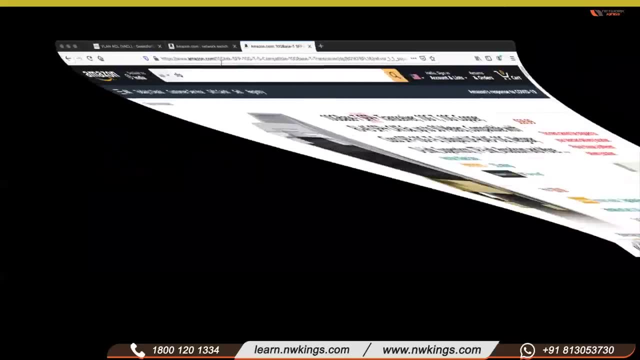 uh, when you actually do the speed test, they go to their server only. um, i hope i'm trying to explain this, so, um, i hope i'm trying to explain this, so, um, i hope i'm trying to explain this, so i'll show you exactly. i'll show you exactly. 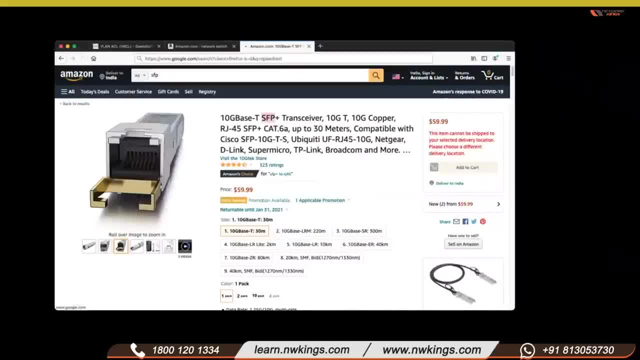 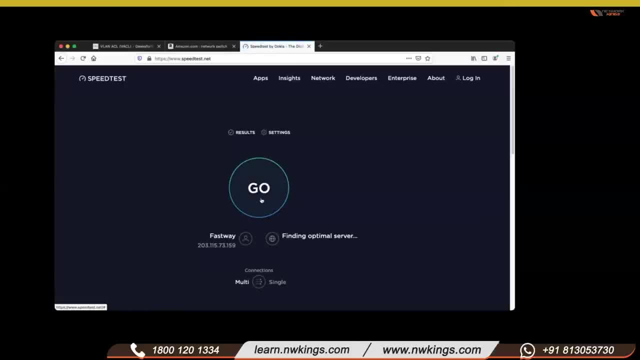 i'll show you exactly. okay, i'm going uh with speed test. okay, i'm going uh with speed test. okay, i'm going uh with speed test, okay, okay, okay, so i'm checking speed test. so, by the way, i'm in north india, right? so, by the way, i'm in north india, right? 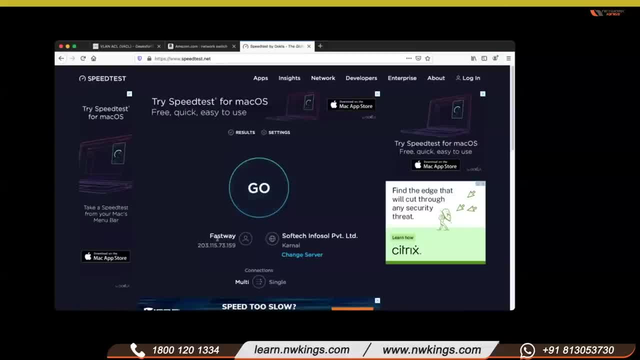 so, by the way, i'm in north india right now, in chandigarh. okay, now in chandigarh. okay, now in chandigarh. okay, so i'll check. this is a small isp, i'm. so i'll check. this is a small isp, i'm. 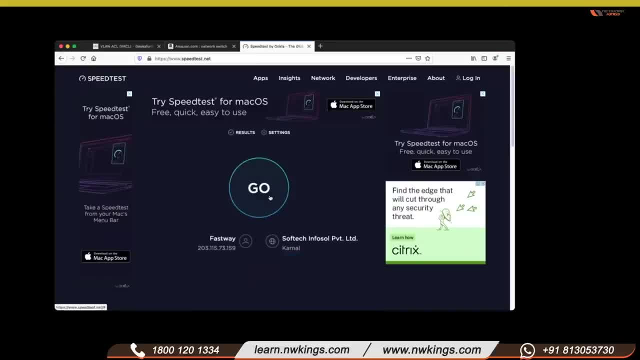 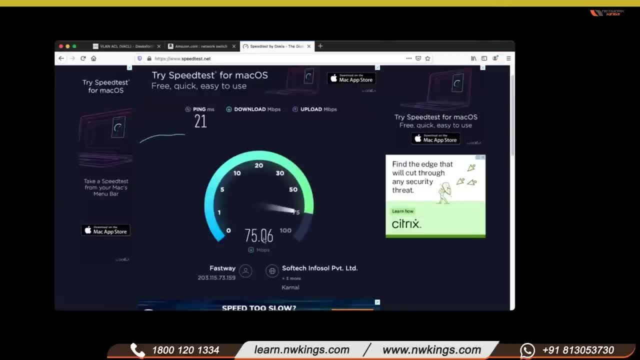 so i'll check. this is a small isp. i'm using fast way, using fast way, using fast way. okay, so let me check the speed. go. so it, so it, so it. it's giving me 70, 80, even i'm teaching. it's giving me 70, 80, even i'm teaching. 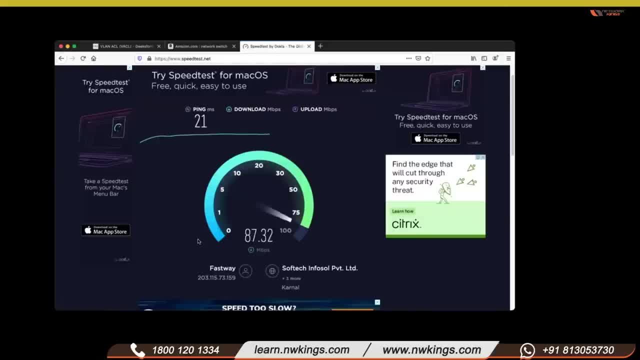 it's giving me 70, 80. even i'm teaching right now with zoom. so this is the right now with zoom. so this is the right now with zoom. so this is the reason it's giving me 80, 90 and all reason it's giving me 80, 90 and all. 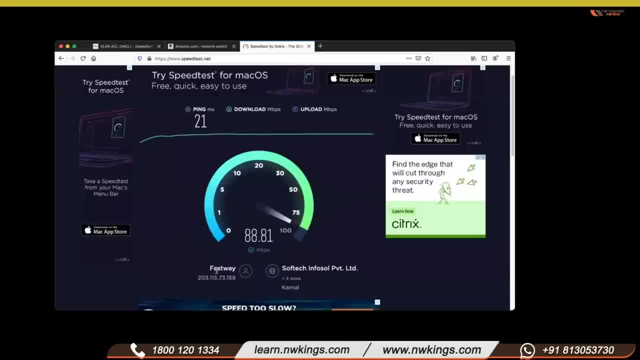 reason. it's giving me 80, 90 and all it means from uh. my, it means from uh, my, it means from uh. my. isp is giving me around 90 mbps and isp is giving me around 90 mbps and isp is giving me around 90 mbps and upload speed also 90- 200 mbps. 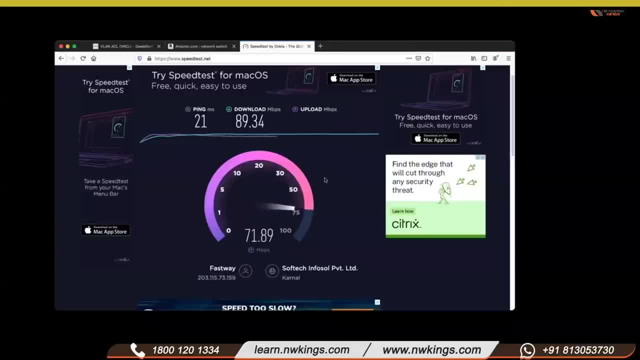 upload speed also 90 200 mbps. upload speed also 90 200 mbps. right are you getting now? right are you getting now? right are you getting now? so you always go and check, okay, and so you always go and check, okay, and so you always go and check, okay, and they show you the speed test, but exactly. 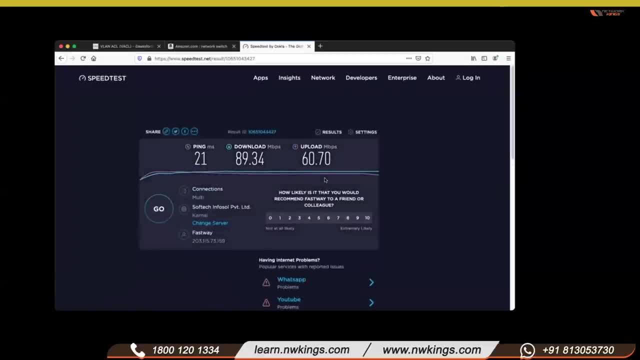 they show you the speed test, but exactly. they show you the speed test, but exactly it doesn't mean you are actually getting it. doesn't mean you are actually getting. it doesn't mean you are actually getting 100 mbps over the internet, 100 mbps over the internet. 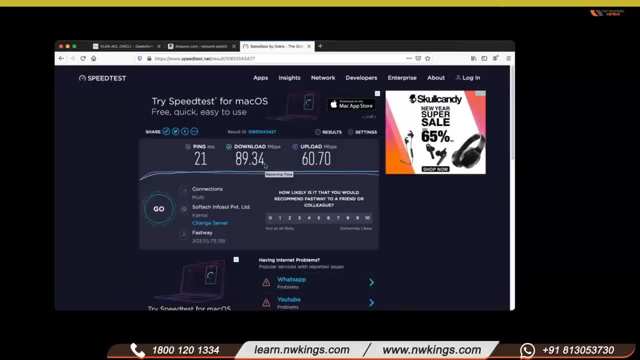 100 mbps over the internet, so this is just a marketing gimmick by. so this is just a marketing gimmick by. so this is just a marketing gimmick by isps. i'm actually isps, i'm actually isps. i'm actually opening their secrets. okay, no issues. 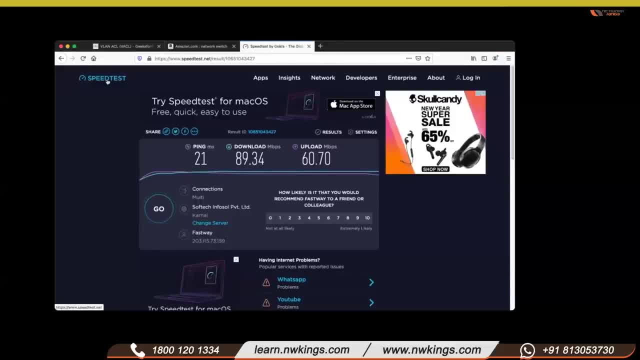 opening their secrets? okay, no issues. opening their secrets- okay, no issues. so 100 mbps- here we are getting 90. so 100 mbps- here we are getting 90. so 100 mbps- here we are getting 90. but again, i'm going to speed test, but 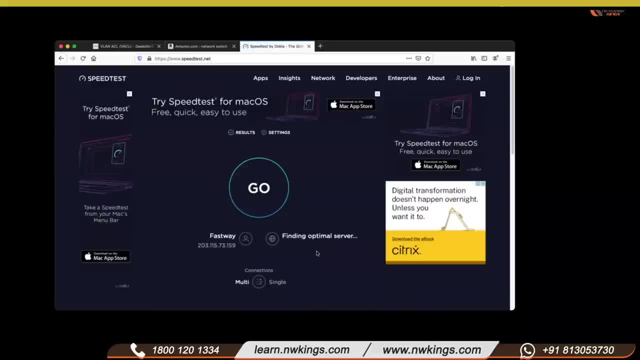 but again, i'm going to speed test, but. but again, i'm going to speed test. but i'm too, i'm going to choose another. i'm too, i'm going to choose another. i'm too, i'm going to choose another server. maybe it's in bangalore, or maybe. 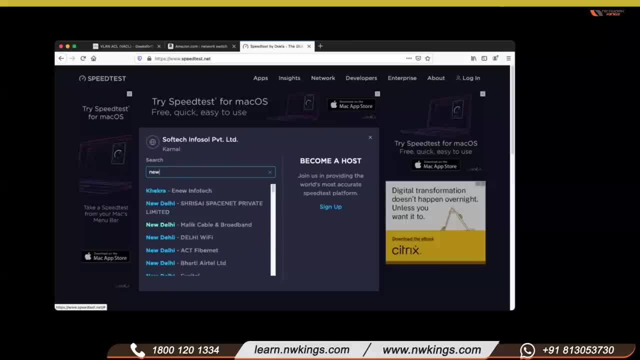 server. maybe it's in bangalore, or maybe server maybe it's in bangalore or maybe somewhere, somewhere, somewhere. or maybe let's check in new york, or maybe let's check in new york, or maybe let's check in new york, let's test one, any server in new york. 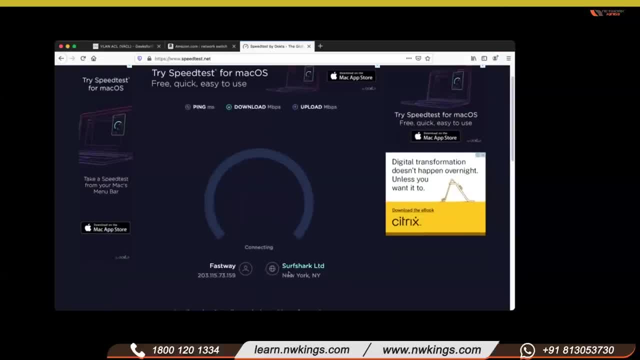 let's test one any server in new york. let's test one any server in new york. so let's test, so let's test, so let's test how much speed actually. so you can just how much speed actually. so you can just how much speed actually. so you can just check the speed outside india and you. 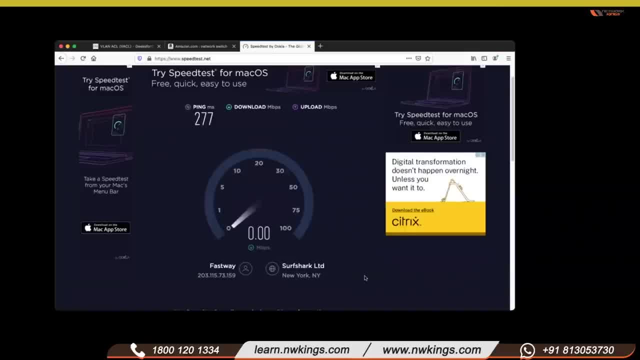 check the speed outside india and you check the speed outside india and you will be actually getting that speed only, will be actually getting that speed only, will be actually getting that speed only. so you can't go more than that. so you can't go more than that. 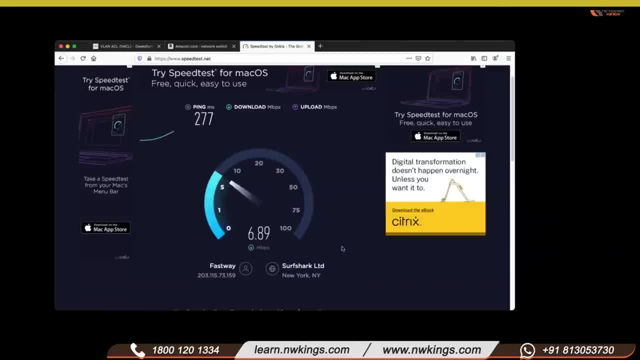 so you can't go more than that. so, so, so, let's see, it's going good, it's going good, it's going good. might be my isp is good, might be my isp is good, might be my isp is good. right, but it it. uh see, if new york is giving me. 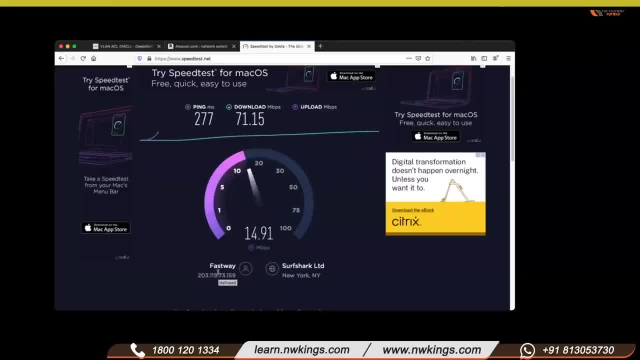 but it it, uh see if new york is giving me. but it it, uh see if new york is giving me seven, eight minutes. my isp is good. this seven eight minutes, my isp is good. this seven eight minutes, my isp is good. this is how you check your isp. 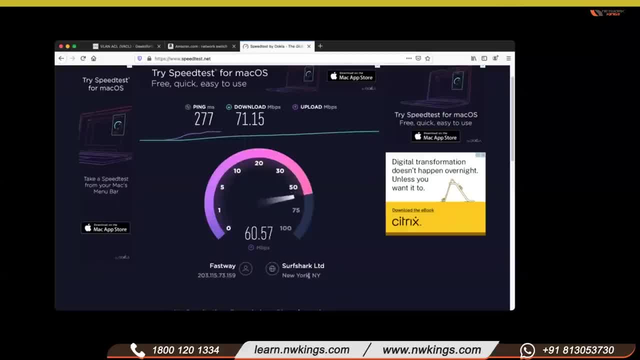 is how you check your isp. is how you check your isp. so just check with another country isp. so just check with another country isp. so just check with another country isp or any location, and you will find this or any location. and you will find this or any location and you will find. this actually gives me. 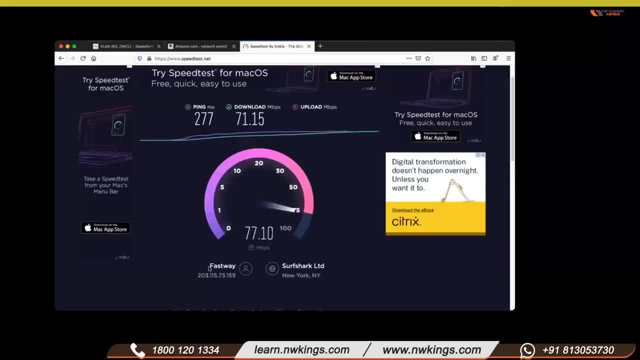 actually gives me, actually gives me yes, so my is better because i'm i have yes, so my is better because i'm i have yes, so my is better because i'm i have around three connections at my home, around three connections at my home, around three connections at my home, and i'm using this one because this is. 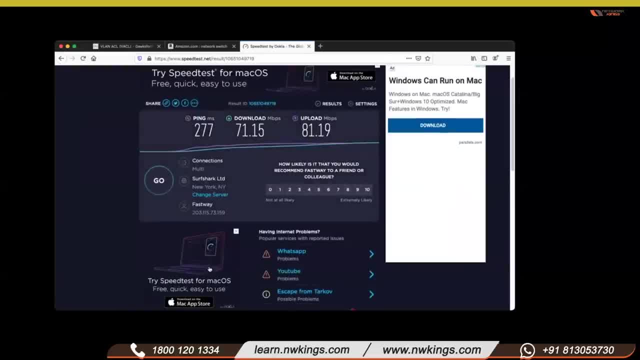 and i'm using this one because this is, and i'm using this one because this is the best one. okay, okay, okay, now you got the point what i'm i was. now you got the point what i'm i was. now you got the point what i'm i was trying to say. 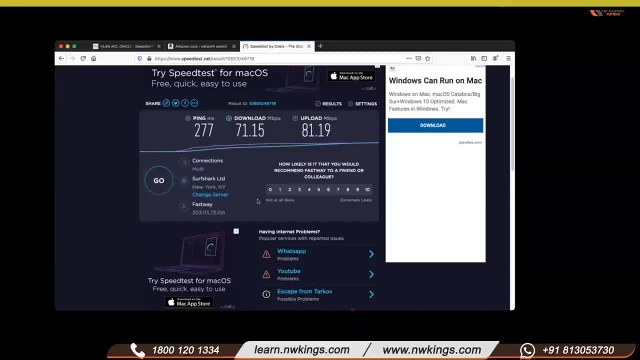 trying to say. trying to say: if you are getting low speed over the, if you are getting low speed over the, if you are getting low speed over the different servers, it means different servers, it means different servers, it means the bandwidth is choking somewhere. the bandwidth is choking somewhere. 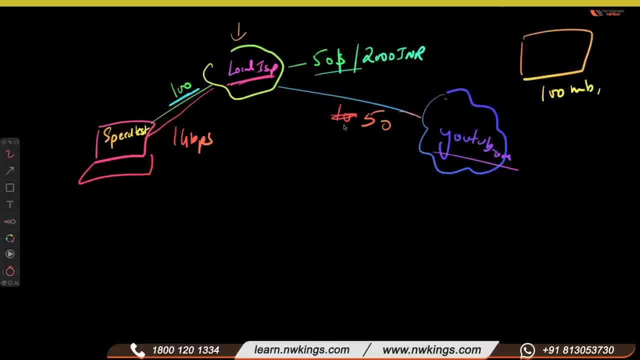 the bandwidth is choking somewhere. okay, okay, okay. might be isp have low bandwidth plan. might be isp have low bandwidth plan. might be isp have low bandwidth plan. so this is so. this is so. this is you guys need to check, okay, cool, okay, guys, let's take a five. 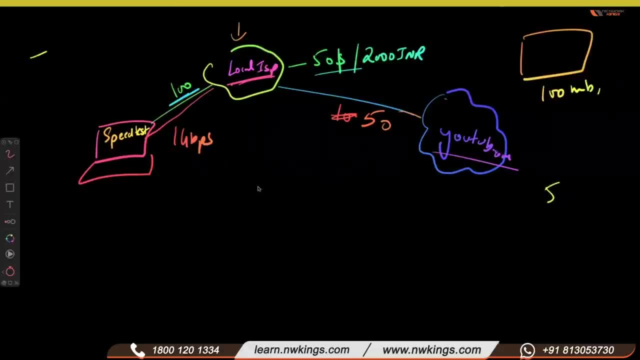 okay, guys, let's take a five. okay, guys, let's take a five to to to. so this: these sessions are of two hours. so this, these sessions are of two hours. so this, these sessions are of two hours. okay, 9 pm. okay 9 pm. okay, 9 pm to 11 pm. 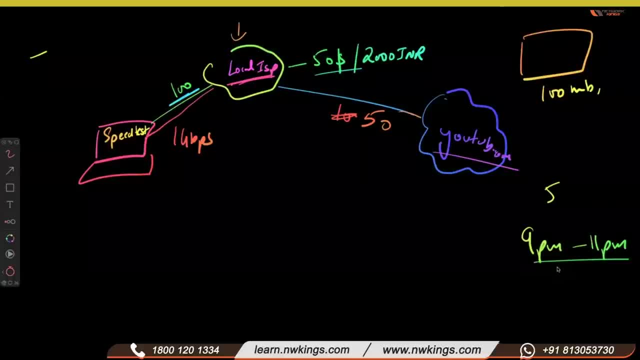 to 11 pm to 11 pm, okay. so i don't think you will mind if i okay. so i don't think you will mind if i okay. so i don't think you will mind if i am going to take 5 to 10 minutes break. 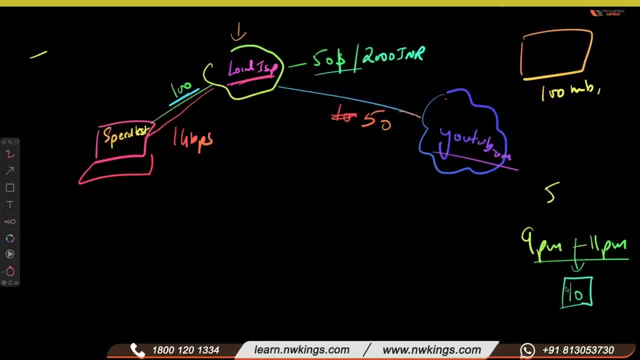 am going to take 5 to 10 minutes break. am going to take 5 to 10 minutes break because, because, because i have not done my dinner yet, so i am. i have not done my dinner yet, so i am. i have not done my dinner yet, so i am going to take 10 minutes break, okay, so. 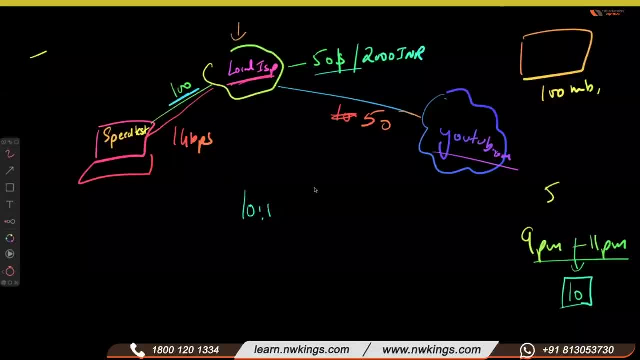 going to take 10 minutes break. okay, so going to take 10 minutes break, okay, so we will meet at 10. we will meet at 10. we will meet at 10. 12, okay, 12, okay, 12, okay, yeah, yeah, so have your dinner and come. 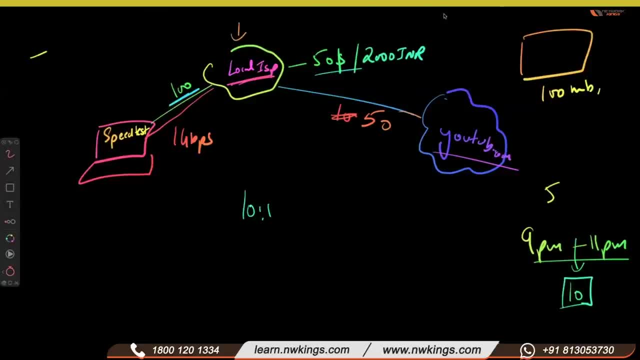 yeah, yeah, so have your dinner and come. yeah, yeah, so have your dinner and come back in 10 minutes, back in 10 minutes, back in 10 minutes. so i'm just so, i'm just so, i'm just going to pause this recording, okay, great, and i'll explain you how to access the. 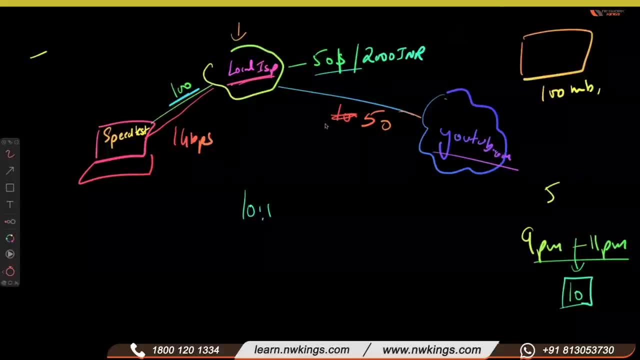 and i'll explain you how to access the and i'll explain you how to access the lab also. okay, okay. so what exactly we are going to? so what exactly we are going to to do, we are going to connect two machines and we will see how they are going to share files with. 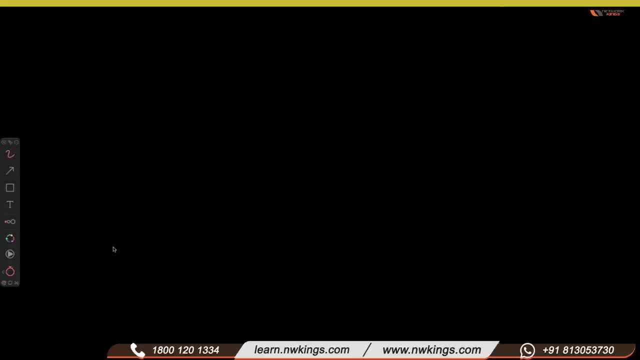 each other. okay, so we are going a very we are going with the first practical. okay, in the first practical or first lab, what we are going to do, so, like my two computers will be connecting with a cable and i'm going to assign ip address here and i'm going to assign one ip address here and before assigning the ip address, 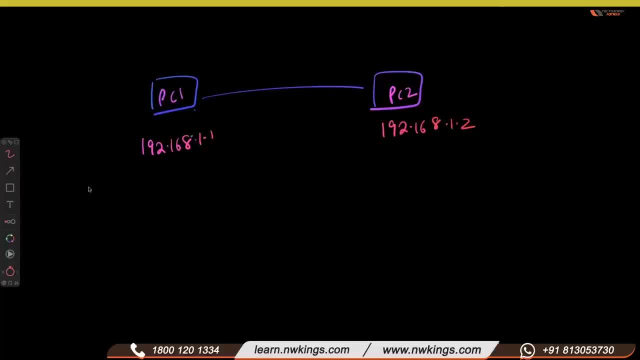 so i'm going to explain you one thing. uh, that is ip address classes. so just remember one thing: we have three classes: class a, b, c, d, e. we will discuss so. when any ip address start from one or between one to one, two, six, you, just you need to match the first part, that is first is network part. i'll explain. 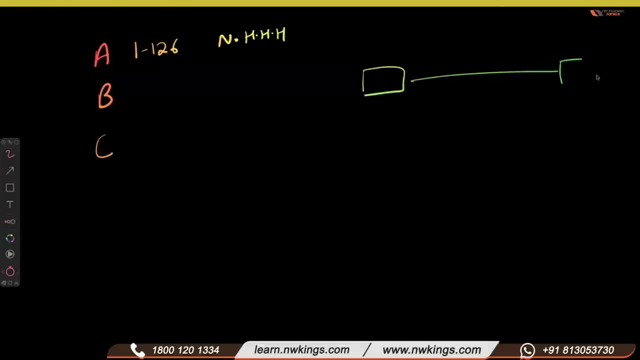 so if two computers are connected together, they have ip 1.1.1.1 and this computer is having 1.1.1.5. so in class a any ip address start from between 1 to 126. we just need to check the first part. 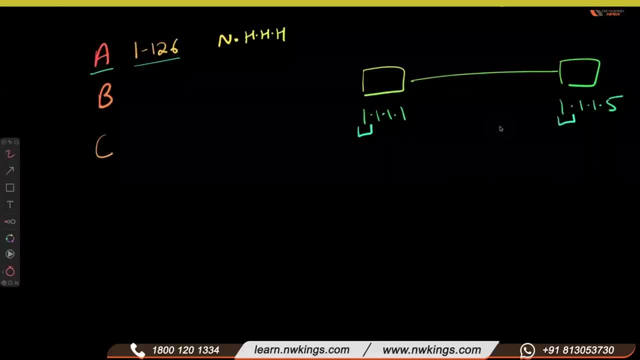 so tell me: they are matching or not. yes, yes, so it means they will communicate with each other. what if i'm going to give 1.1.1.1 and here 2.1.1.1, so our is the first pair, first octet or first part is matching. no right, so they will not communicate. 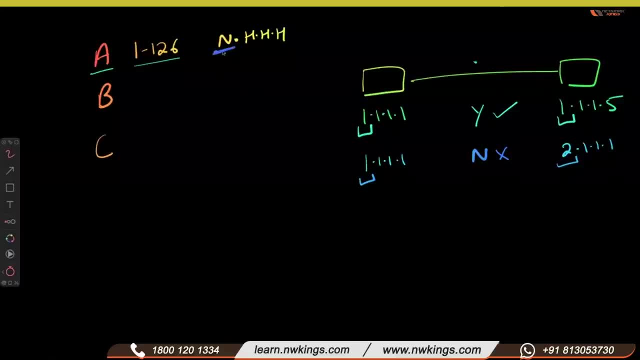 they are not going to communicate with each other because our first network part in class a, between 1 to 126, by default is this: we can change these things. that terminology is known as subnetting. okay, that we will discuss later on. so in b, when the ip address is between: 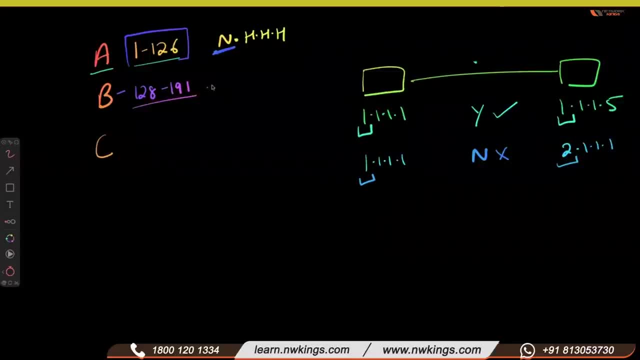 128 to 191. so we need to check how many parts we need to match. two parts, guys, two parts only. it means when we have ip 150.1.1.1 and here we have 150.2.1.1 or 2.7.. 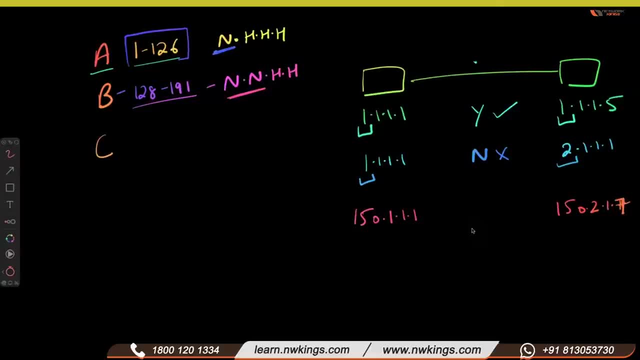 so tell me, are they going to communicate with each other? yes, routing is a different. i'm just asking two about two computers first. ah See, in class B need to match two things. So just check if two things or first two parts are matching. 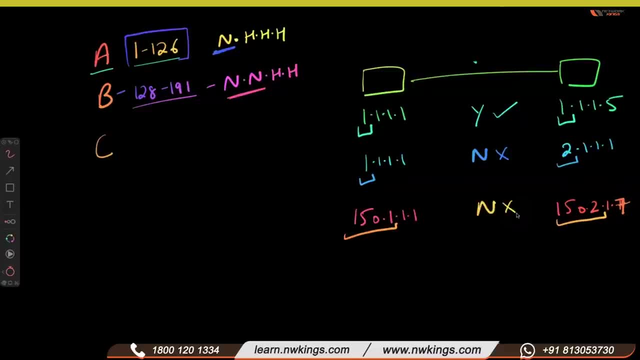 No, Big no. They will not communicate. They are not going to communicate with each other. Why? Because my first two octets are not matching. My network bits are not matching. It means they are not in my network. This is the power of network bits. 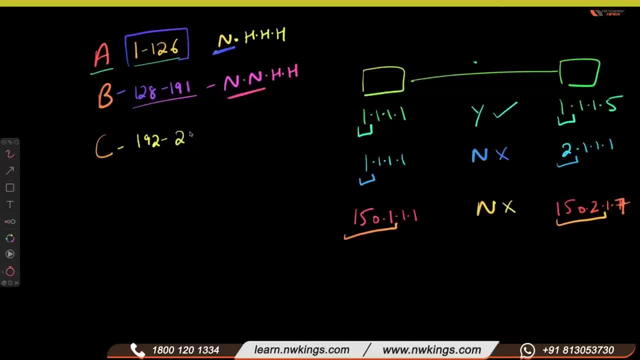 In class C we have 192 to 223.. So that is three network part. It means we need to match three portion. So suppose I got 192, 168, 1.1, which is very common IP. 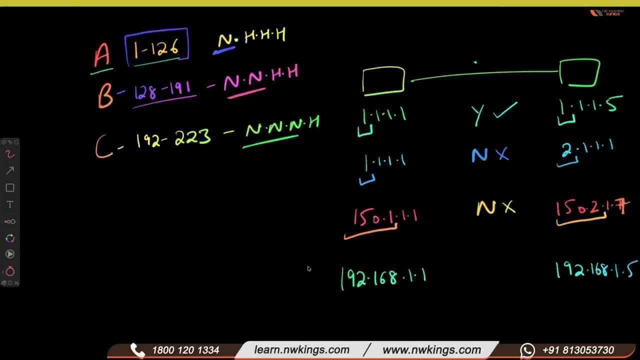 192, 168, 1.5.. This is class C, where we are going to match three network bits. So tell me if they are going to communicate, Yes, And what we will do to communicate In Between these ones. 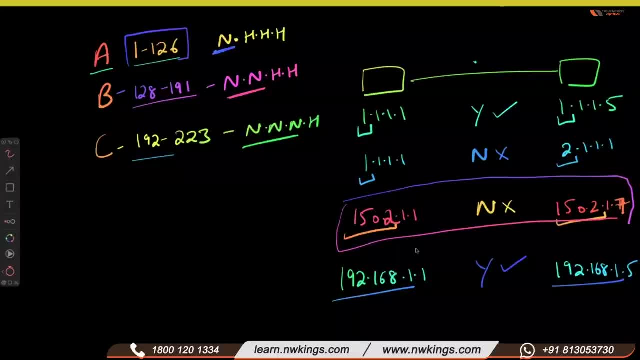 So what we are going to do, Either we will make this two, or either we will make both 150.1.. Right, Then they are able to communicate with each other. So this 127, which is not here- that is for loopback testing or loopback IPs. 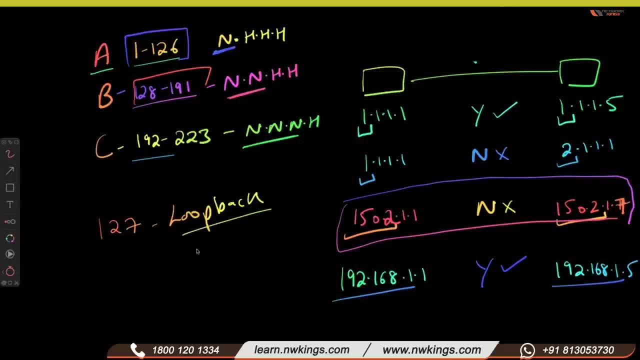 That is for self-owned IPs or local host. It means all your computers. when Windows starts, it appears a logo. All the services are in background, Or all the services inside your machine, Because your laptop machine itself has server for your machine. 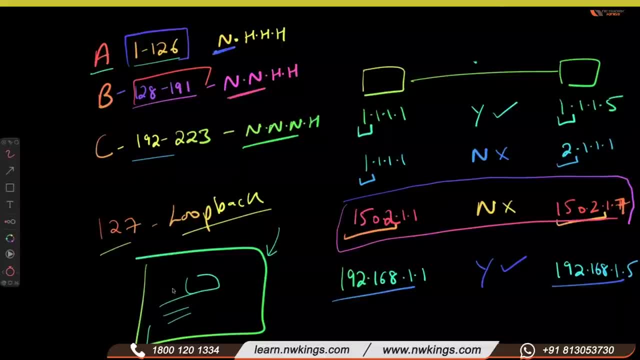 Because you are getting all the images, all icons of the files. So that is a self-host IP or self-hosted IP address. That means these are your IPs. Okay, So means your internal IPs, which are not accessible or accessible. 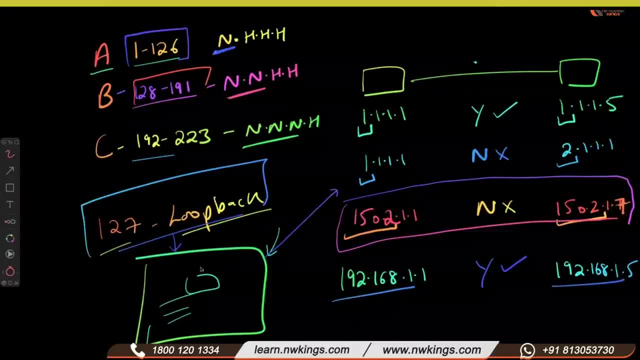 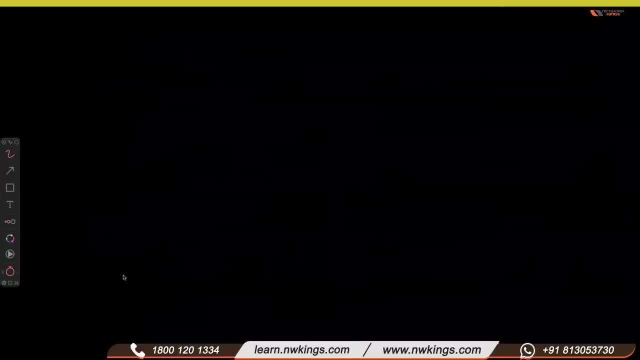 Okay, All from outside, Like it says sole, you can say that, Right, We can't transfer Until and unless you have black magic tricks. Okay, Bad joke, Let's go with the lab. So labs, I will explain later on. 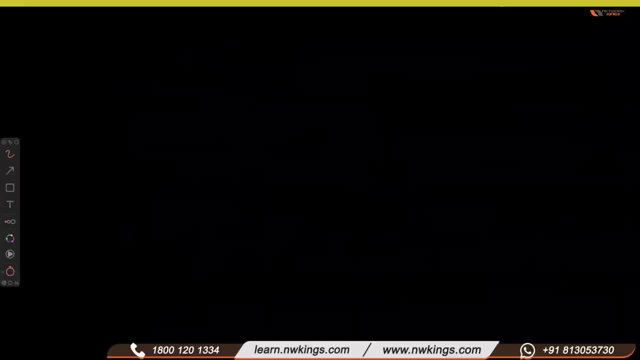 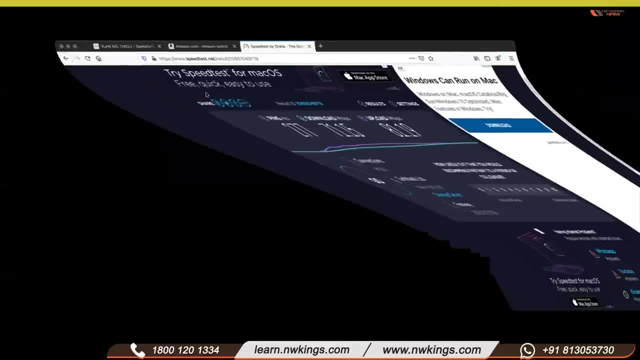 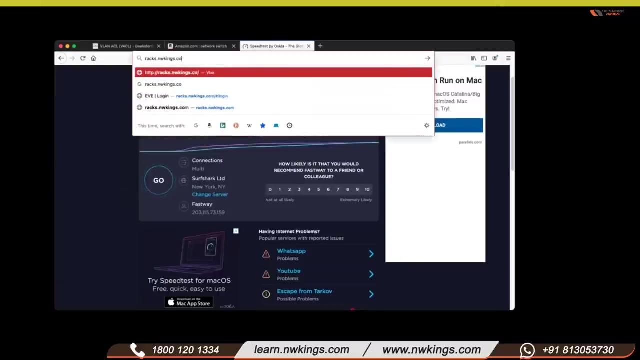 Just first do the lab first. Okay, to access the labs, we are going to use racksnwkingscom. Here is the trick. I am going to use one port number, 8081.. I think this is the 8086, sorry. 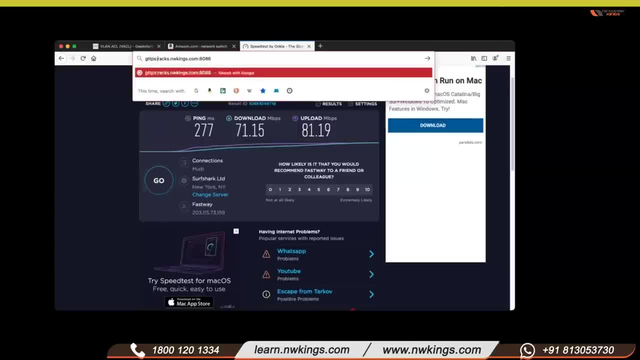 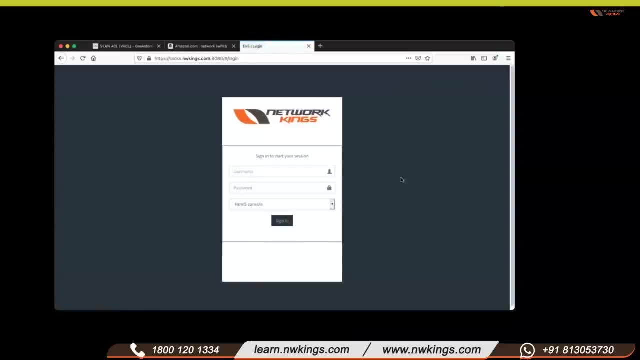 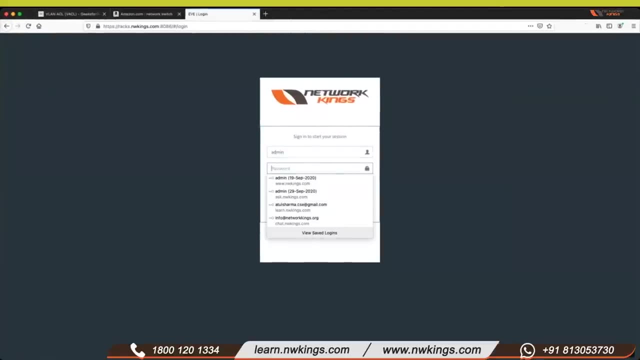 Okay, And I am going to use HTTPS here. Okay, So you will be getting an email very soon to access the server. So we have installed EVE engine on top of our servers so that you can access the lab, Okay. 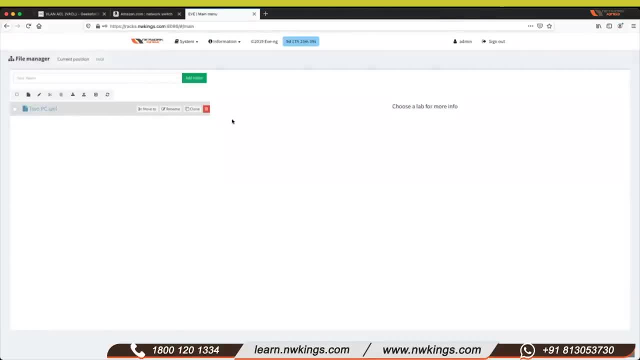 So I have already made a lab here, two PC When you are going to log in. so you are going to get this lab first, lab here. Okay, So open it. You don't have to do anything. Just these two PCs are my two window machines. 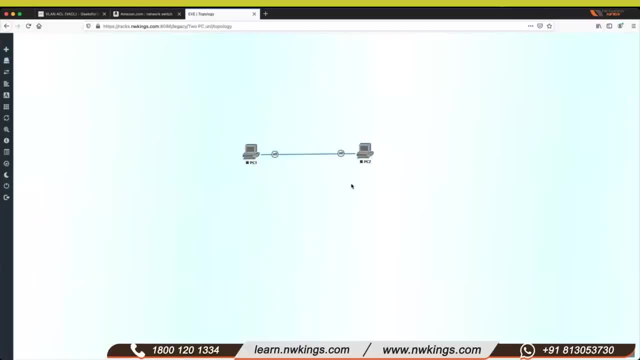 Looks good. Or should I change the icons? Okay, It's good. So now I am going to click on PC1 and I am going to start this Start And I am going to click on another PC- Start. Okay. 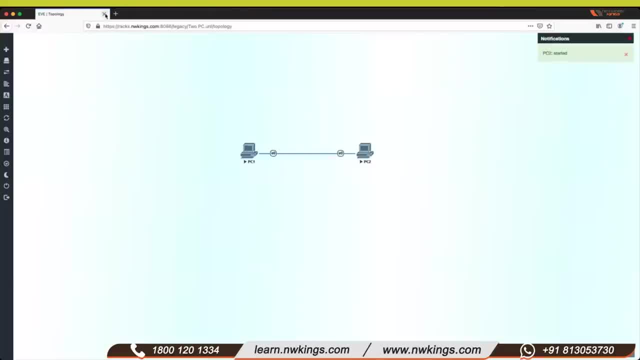 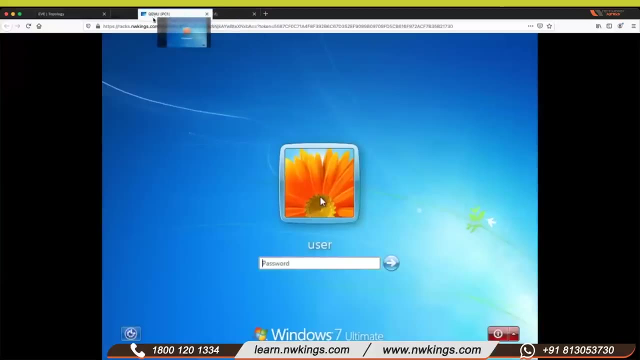 And just click on the PC PC1. And I am here starting my lab. I am going to log in to Windows 7. And in another PC, also PC2.. So my two PCs are opened here, Cool Right. 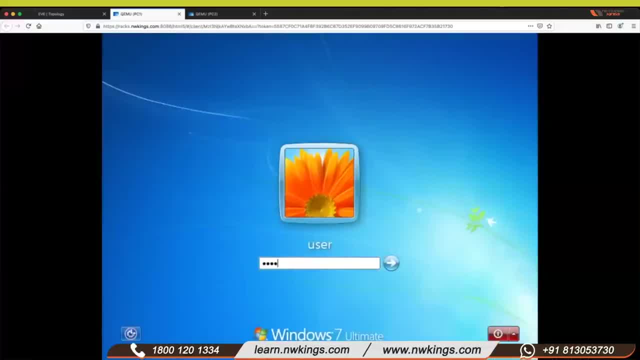 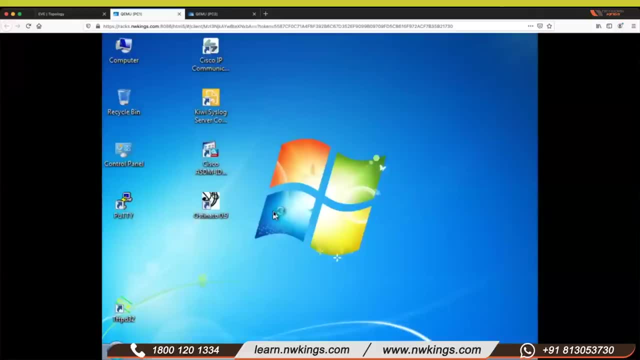 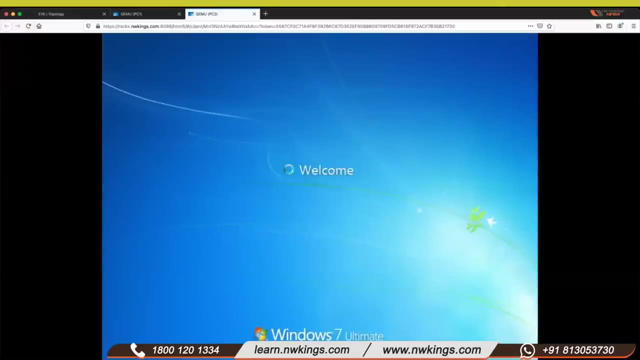 So the password is test123.. Okay, T in upper case: Test123.. Remember it When you are going to do the lab. it will help you. Okay, here I'm going to log in test 1,, 2,, 3.. So my two PCs are here. Yes, it's fast, obviously. 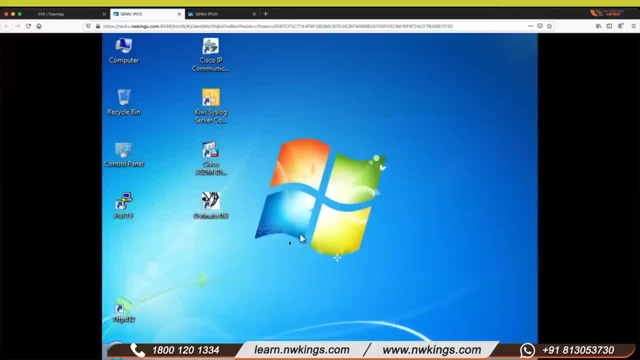 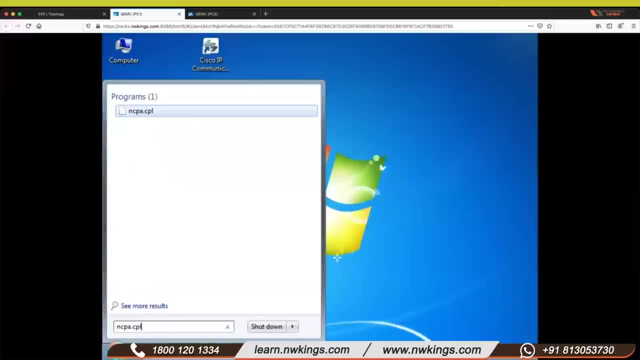 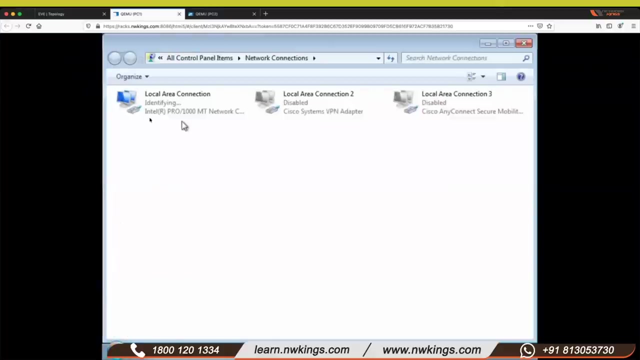 So how we are going to give IP address. So in Windows, I'm going to give you one shortcut, that is ncpacpl. You can write down this shortcut: ncpacpl. Okay, ncpacpl, enter it And we are connected with this local area. connection means the. 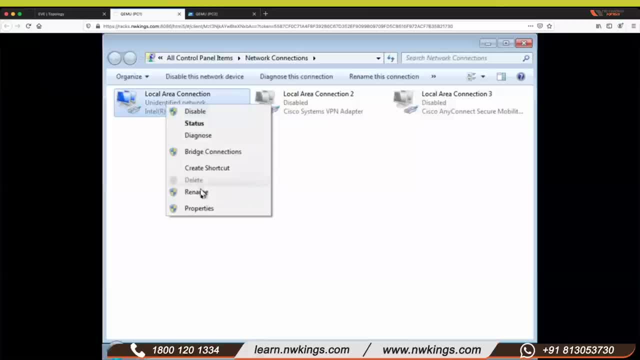 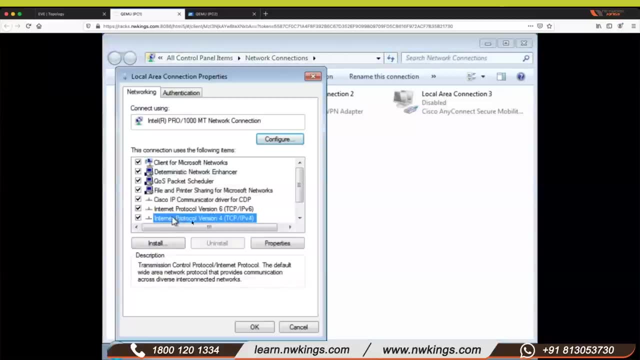 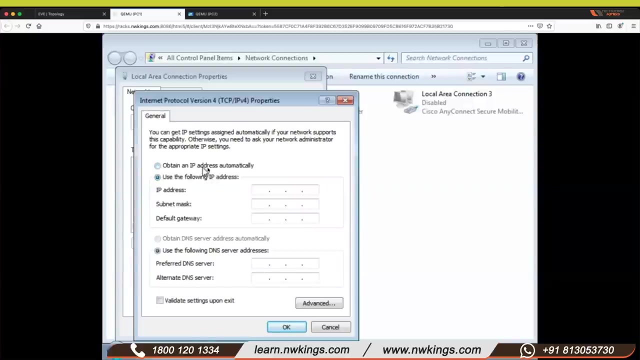 port. So right click on this and properties And here you can see internet protocol version 4.. We are using version 4 right now. Okay, and click on properties And here we are going to assign the IP. So this is the option here: obtain an IP address automatically. It means when you connect with 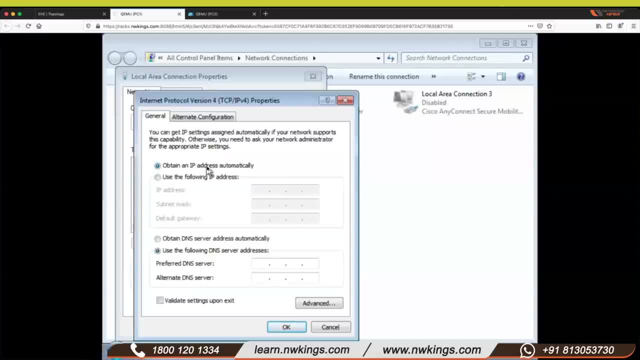 the Wi-Fi or any type of router or any device, it actually gives you IP address automatically. That is DHCP. So we'll discuss DHCP later on, But here we are going to assign the IP, So I'm going to use a class A11111.. Okay, And here we got by default automatically. 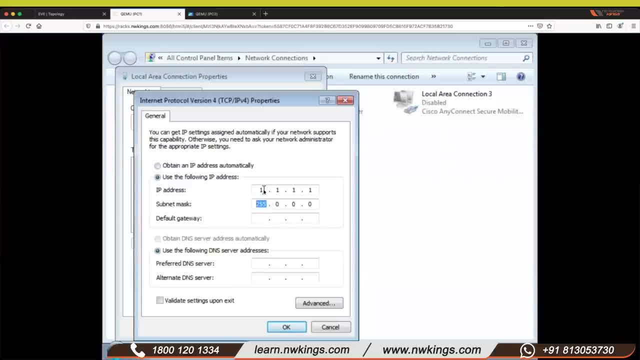 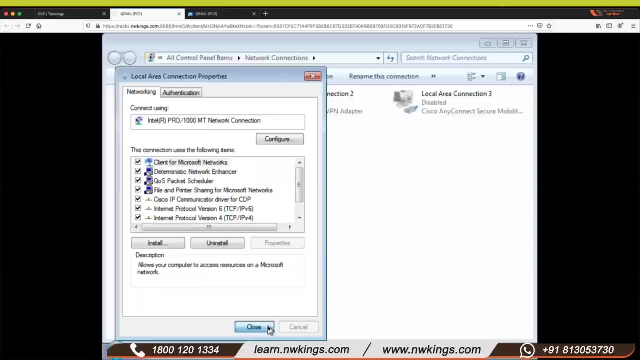 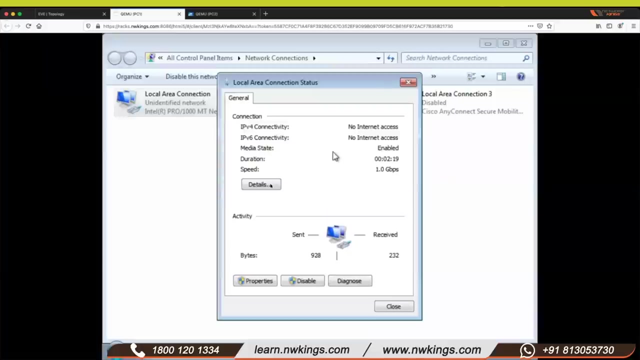 subnet mask This 255, it means just need to match the first part. Okay, when we have 1255, where it means we need to just check the first part. So in first PC I have given 1.1.1.1.. Okay, close And let's check: the IP address is configured or not. Status and. 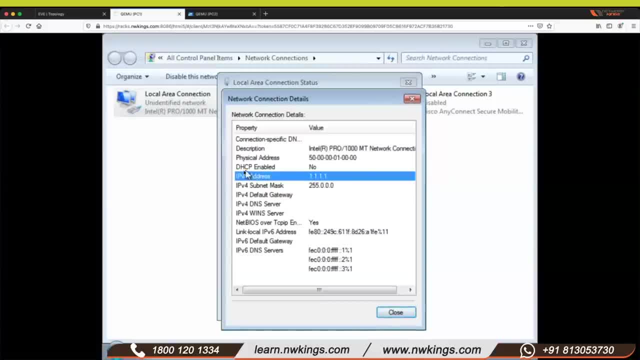 the details Here we can see DHCP is enabled. No, because we are going to use DHCP, So we have configured the IP address manually. So you can see here: 1.1.1.1.. Okay, So this is my first PC IP address. 1.1.1.1.. Close it And in another PC tell me which IP address. 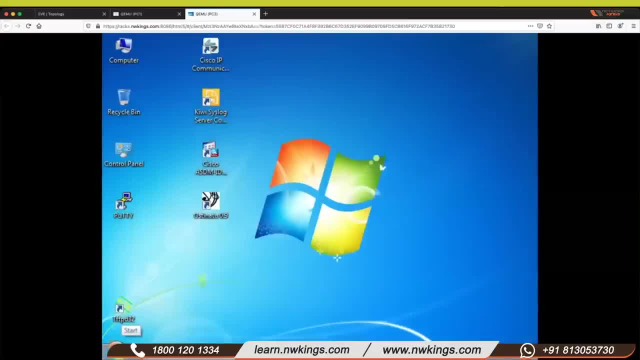 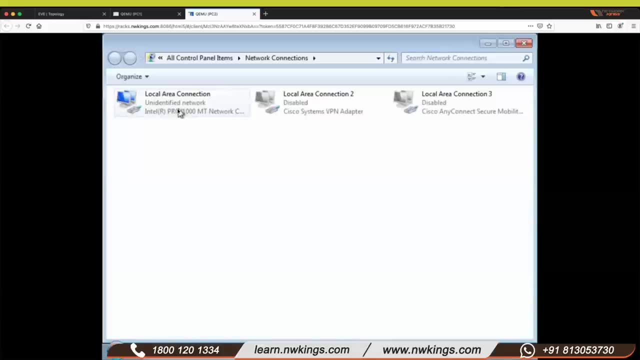 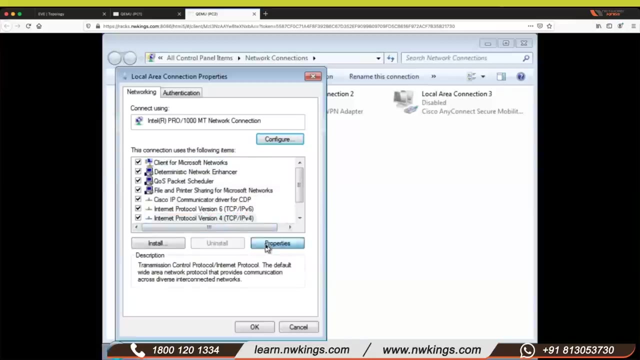 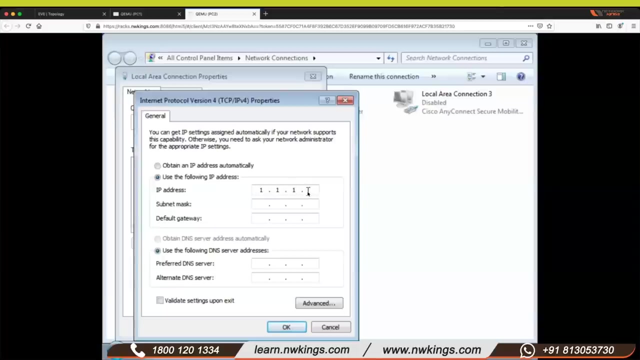 should I use? Can I assign 2.1.1.5?? Okay, So in the second system I'm going to give properties and inside the properties I'm going to give: Yeah, I'm going to use 1.1.1.. 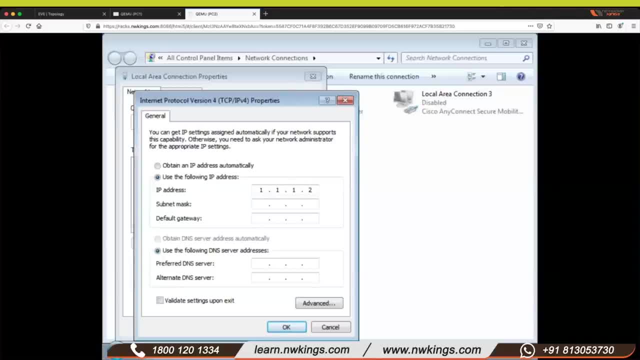 Let's take 100.. Or let's make it simple: 1.1.1.2.. Okay, again, 255.. It means my first computer and the second computer is having 255, where it means I'm going to check the first portion. 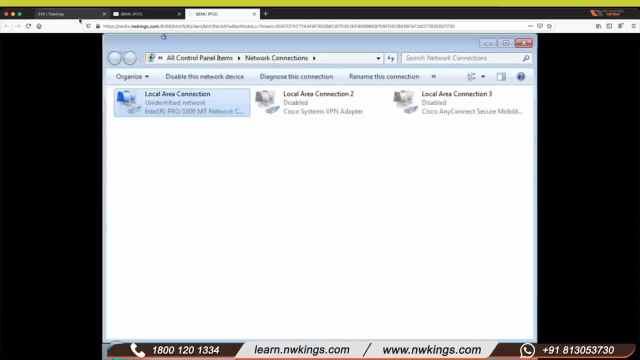 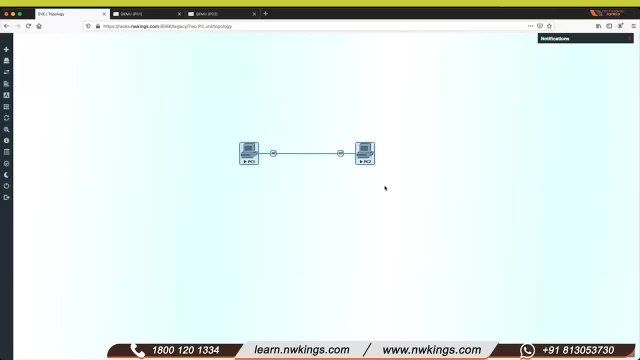 So if both the portions are the same, then I'm going to check the first portion. So if both the portions are the same, then I'm going to check the first portion. So if both the portions are the same, it means both my PCs are in same network. Kevin, I'll explain. 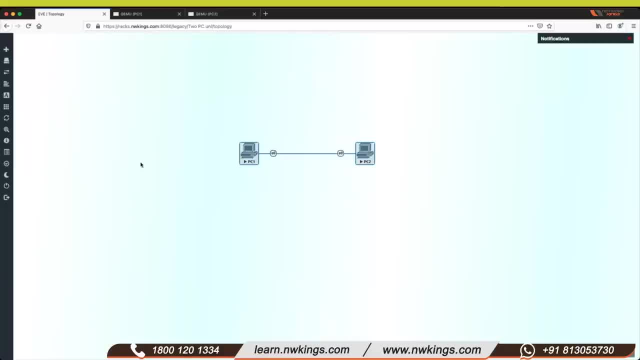 IPv6 later on, its little advance right. So first go with the IPv4.. And this is how exactly we train. The difference between IPv4 and IPv6 is: IPv4 is 32 bit and IPv6 is 128. bit means it's a combination of IPv4 and IPv6. So the difference between IPv4 and IPv6 is: 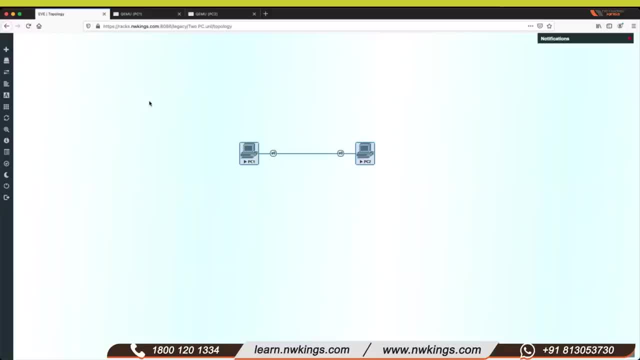 keeping constant. IPv4 were 1 and IP ST黨. We can assign a lot many IP addresses in IPv6, but in IPv4, we have limited range. so IPv4 is now almost collapse, or what we call that: all most utilized. So this is the reason we have IPV 6 now. I see Sila explain so. 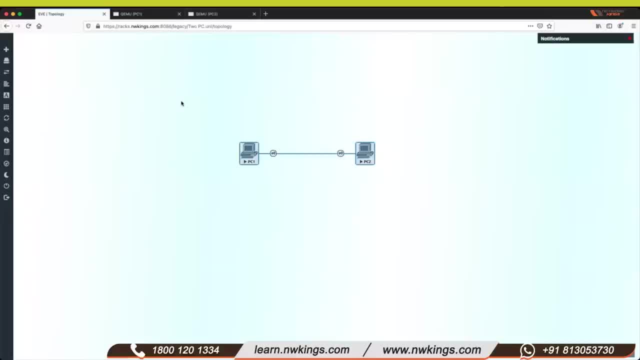 So both the pieces. just see the practical guys first. Okay, let's go to a hol piano, Anybody else, And they can't just thunderstorm. the shop functions in ärbleando now. Is that a goofy idea. Why can't anyone ever have others? No thanks, I don't think this. 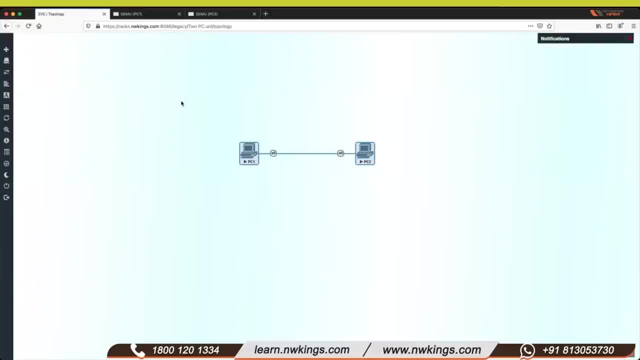 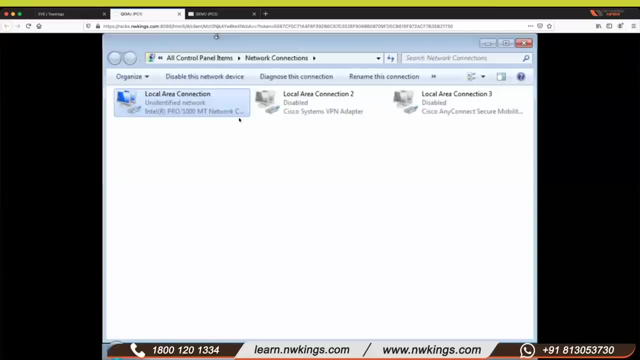 is Just forget. Basically, if everyone has Orbit before, I can do this one. I shot here me now out of lack of internet access. Whatever they love weird, Let's run that off. I think does not have no connection to의 so. so both the pieces, just see the practical guys first. okay, so might be we'll learn something maybe. 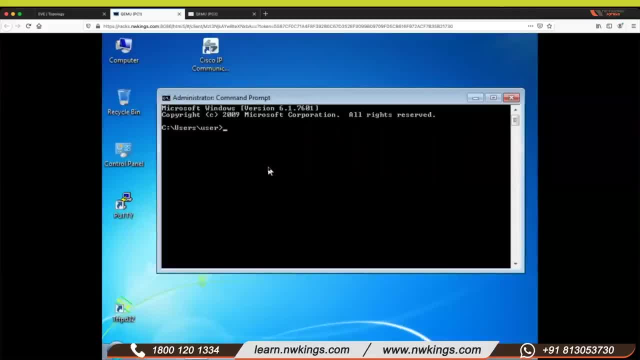 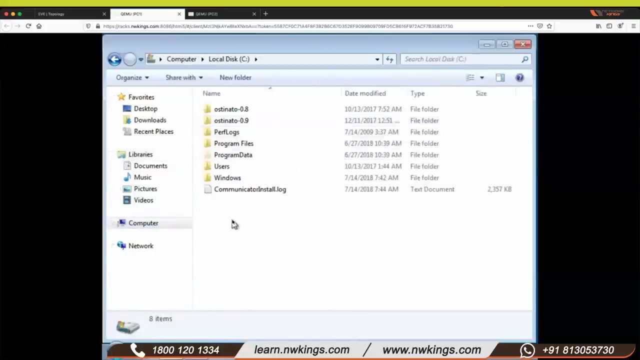 it's very basic, but obviously it's a fundamental class, right, so i'll use i i'm going to show you something. so i'm in c directory. let me go inside c. so i i'm in c drive right now, so you can see this is my c drive, right, right? so i'm going to create a. 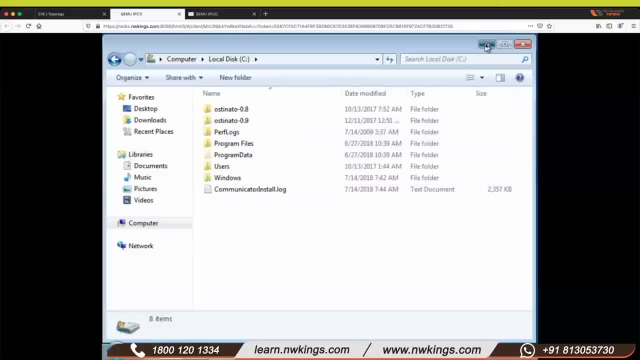 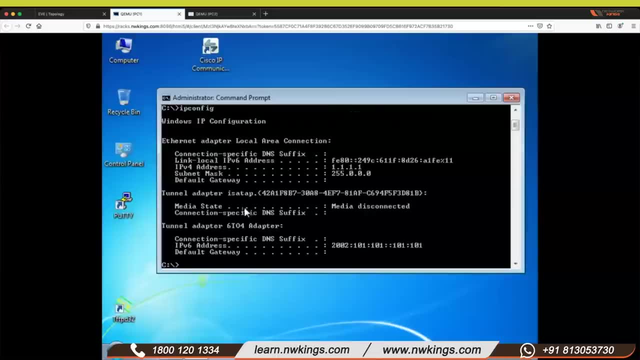 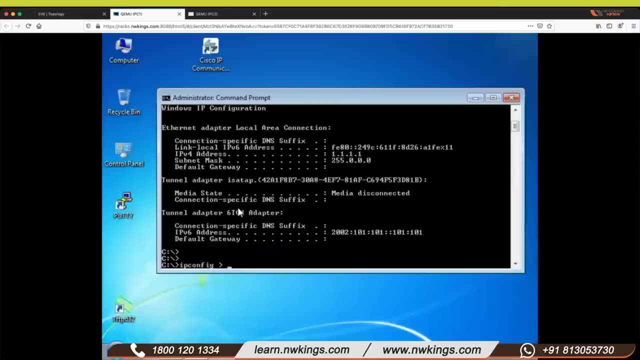 one file here or no need to create here. i'll show you something. so there is a command call ip config where you can see all your ip address. but i want to just get all this output in one file. so i'm in c drive, i'm just using this symbol and i'm putting this into one dot txt. 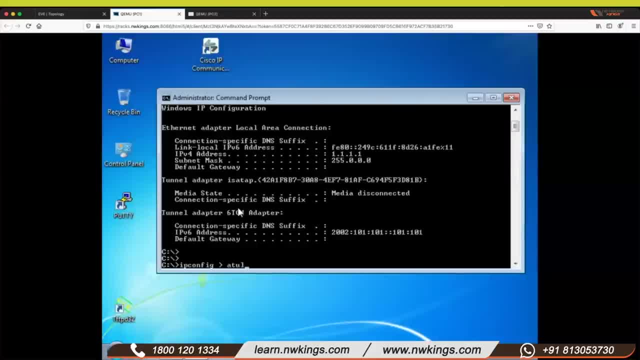 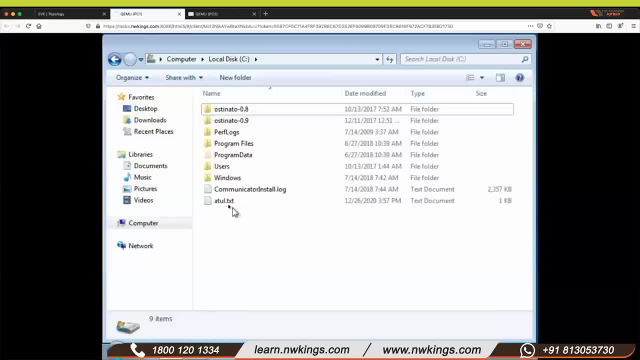 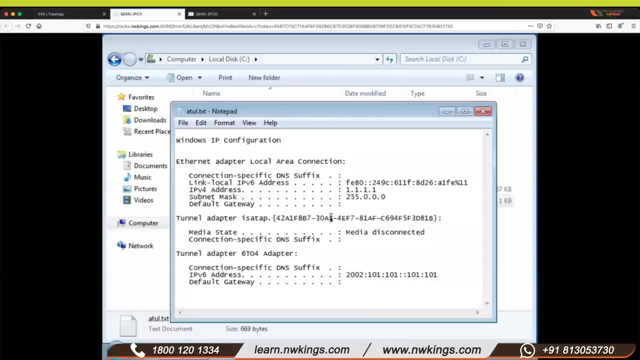 or this any name? uh, suppose atul dot txt. so in c drive let's see if there is a file- yes, we can see here atul dot txt, and let's open it and we got all the details. even windows sometimes behaves like, behaves like linux, right? so my computer is 1.1.1.1. 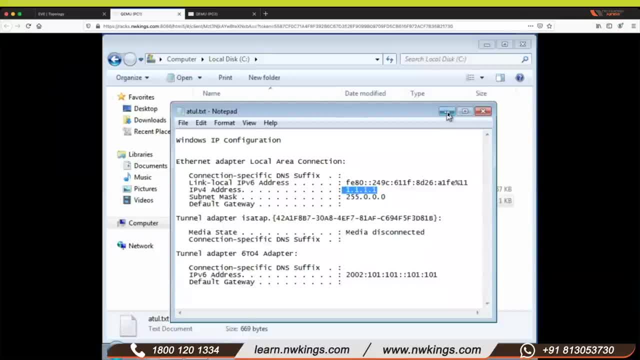 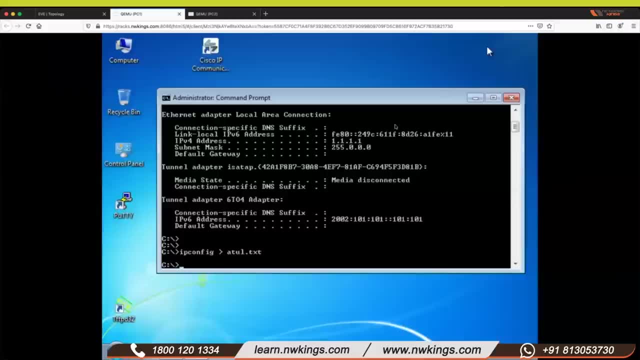 okay, and here you can see all ethernet adapter and all. okay, so i'm in c drive right now. so i'm in c drive right now. so i'm in c drive right now. great, okay. so let's check how to test if my another pc is connected to pc1. so how we are. 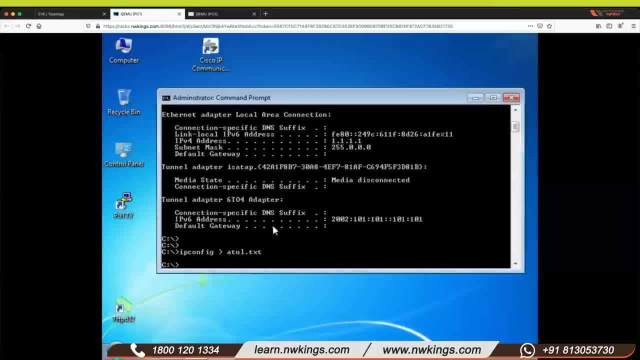 going to identify. pc1 is connected to pc2 now. so there is a tool called ping, so ping stands for packet internet gropper or okay. so this ping is a tool to test the connectivity between two devices or either hundred of devices. so i'm in c drive right now. so i'm in c drive right now. so i'm in c drive. 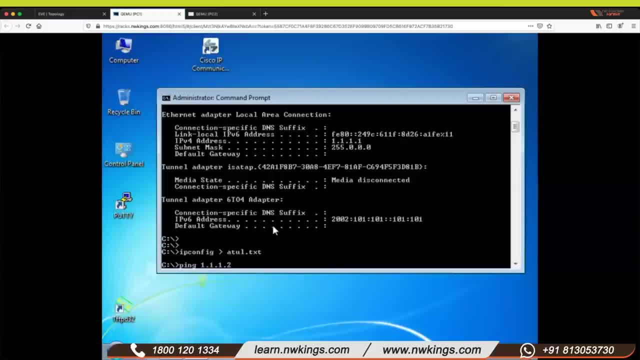 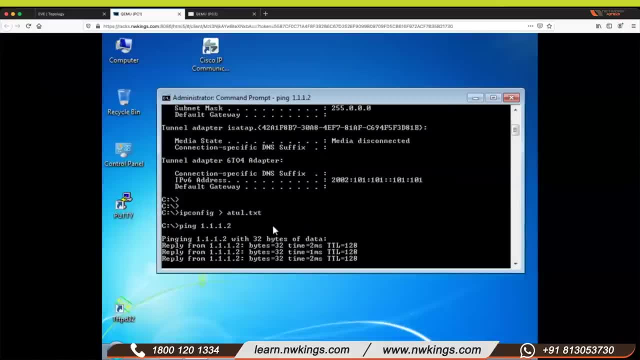 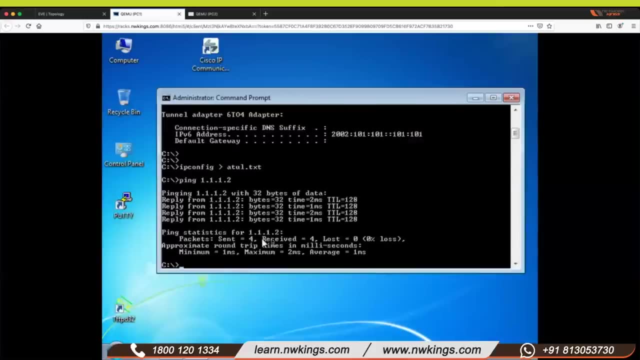 also so. 1.1.1.2. we need to send this ping request so you can see we are getting four replies. it means we have sent four packets, we got four replies. it means zero percent loss. it means we are connected with this device. this is how we come to know this. these two devices are connected now. 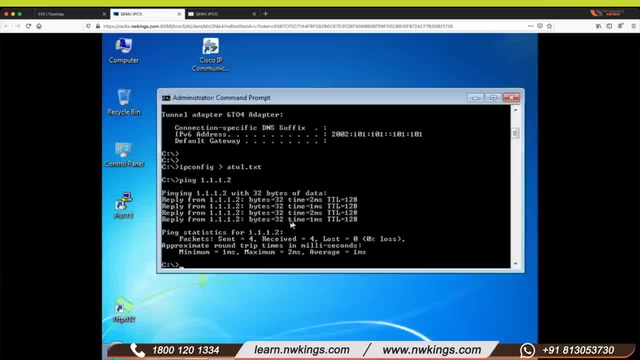 so what is ttl and time and all? i'll explain. so first of all i'm saying: uh, i'm, i'm by default i'm sending 32 bytes of packet, so ping is a packet. okay, so i'm sending four packets and i'm getting four packets. reply: it means so my two pc are connected, i'm sending four ping requests. this is. 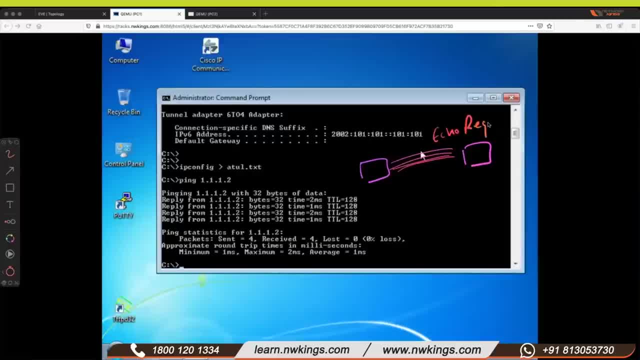 This is known as echo request. We call this echo request. Okay, And how computer understand this is echo request. There is a code in it And that code is basically 8.. So this is a type code. So how my computer understand, it's a request. 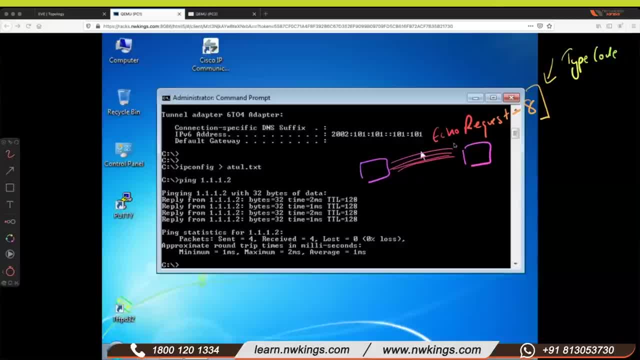 Because when we send this echo request- Echo is a type of message we are sending from PC A to PC B With a code that is echo request type code 8.. That means it's a request And B is going to reply with all four replies here. 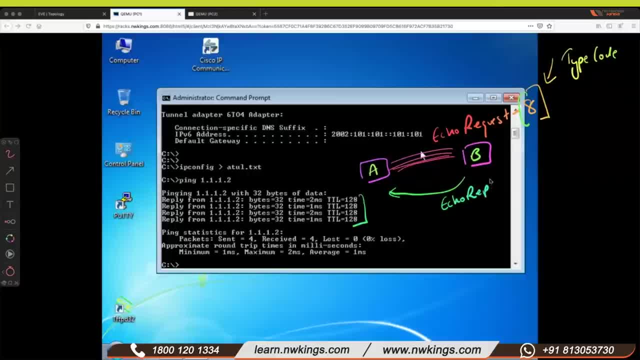 So that is echo reply. For every request we are going to receive one reply. It means we are sending four packets, It means we are going to get back four replies And the echo reply code is 0.. So that is the type code of echo reply. 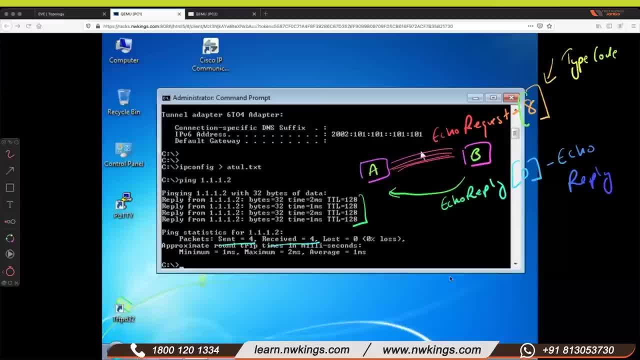 So this is how your computer understand When they are getting, Because computer is getting 0: 1.. All the data in the form of 0: 1.. So how it is getting it's echo reply or echo request. Because when we are going to write this 8 into this binary form, 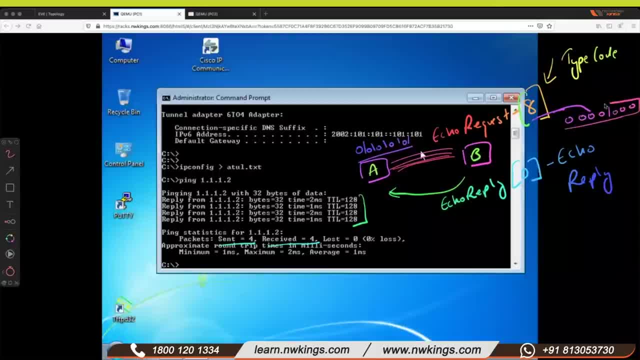 Like kind of this. So when these type of 0- 1's are coming from another device, It means we are getting a request And we need to send a reply back With all 0's, Okay. So if it's getting more complex, 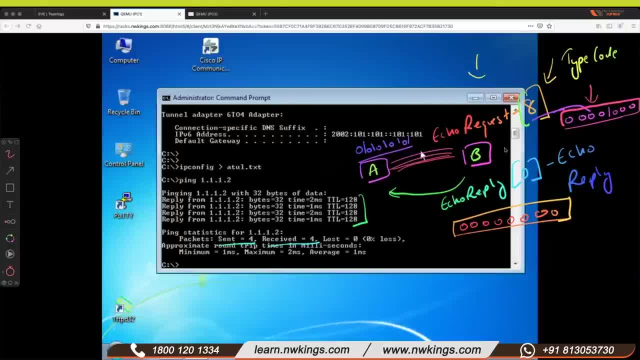 You can just simply understand. It's a ping packet, We are sending request And we are getting reply back, And this is a tool to check the connectivity between two devices. So by default, we are sending what type of size, By default when we are sending data. 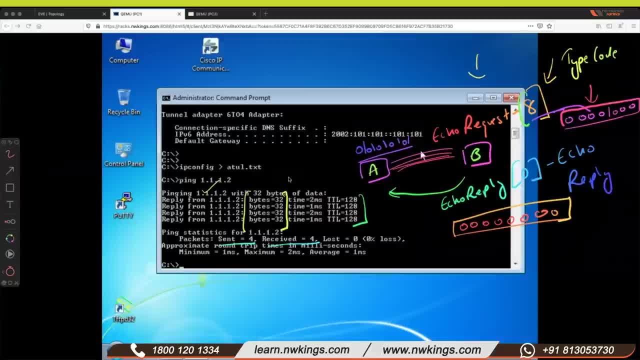 We are sending 32 bytes of packet And we are getting a reply back. Okay, Yes, I see Yeah. And in how much time? we are getting reply back? in 2 millisecond. 1 millisecond This time represents how much time my computer is sending data to another device and device. 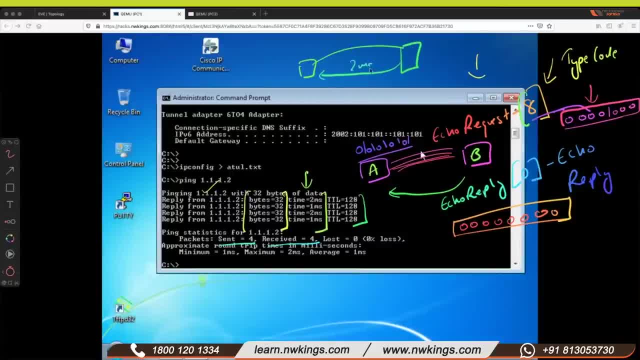 is sending reply And this reply is coming in 2 millisecond. Second reply: I got in 1 millisecond, Okay. Third reply: I'm getting in 2 millisecond. So it varies Right, Sometimes it 2 millisecond. 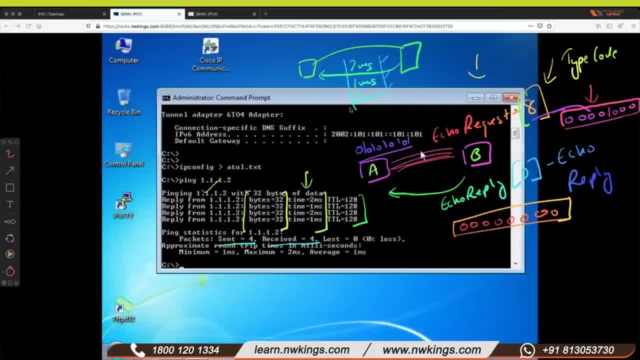 3 millisecond, 4 millisecond. It depends on the location. Also, if you are pinging googlecom, obviously you are going to get more time because Google servers are at different location. We call this latency, We call this time. 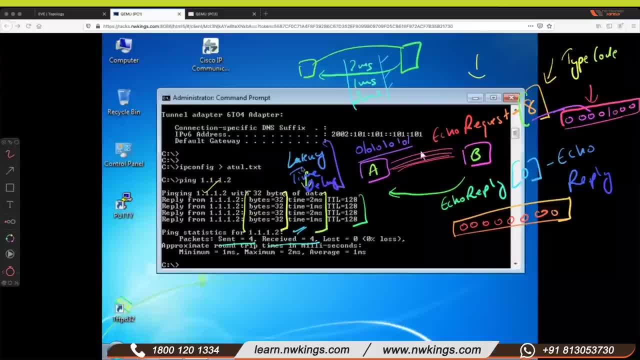 Also, you can say that delay, You can say that in network language, delay, latency time. All these are common or same thing. So what is TTL over here? That is time to live. Time to live. Suppose we are sending a ping to any device but it's not actually present in my network. 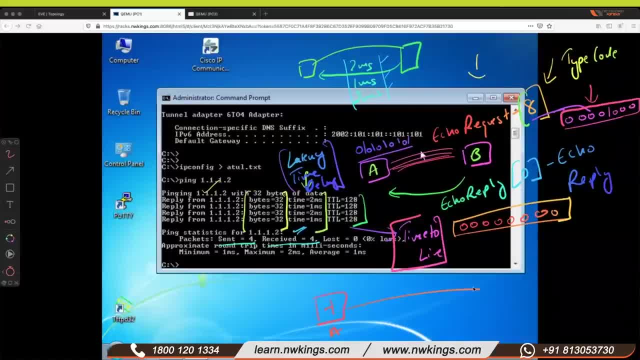 Suppose you are sending requests from PCA to any device which is not in network. Okay, Over the internet, it actually over the internet. data is very important when you are pinging googlecom But mistakenly you are pinging some another IP which is not over. that IP is not available. 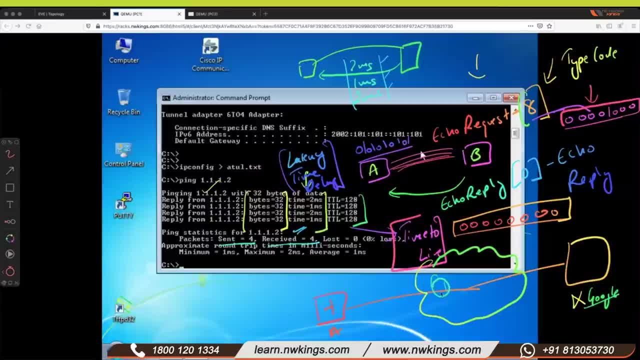 in the internet. So actually, what happens your routers? if you are sending ping request, your router is going to decrement this value. with one Suppose you are sending request with 128. The first router will make it 127.. The request is going with another router. 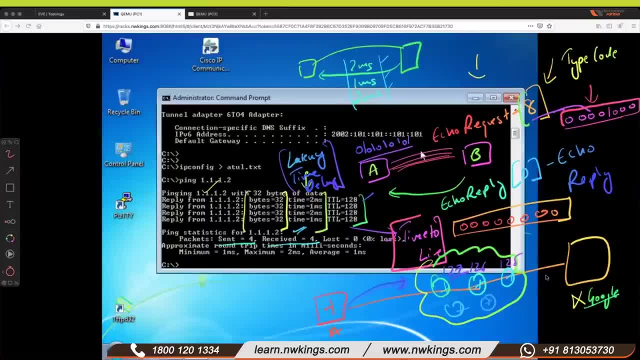 126, 125.. So if location is not identified, if location is not in my network or any anywhere in the network, that packet will be discarded or dropped when the TTL value will be zero. So TTL is just like expiry date, Okay. 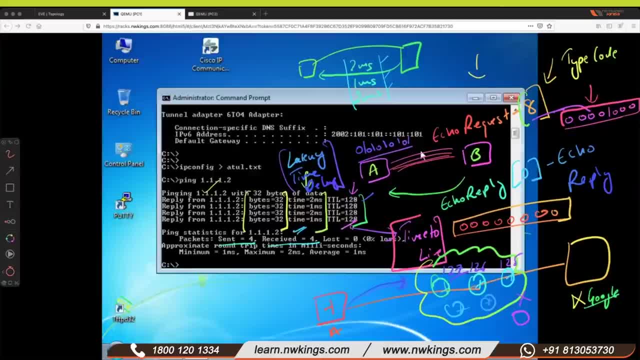 So if I'm going to, I'm going to send a limit with the 128,. it means, if we don't get this IP address within the 128 routers, I'm going to drop this packet. Got it Why we have this TTL value? Because if we don't have TTL, the packet will keep revolving in our network and it will create internet loops. This is the power of TTL value: If we don't have anything in internet, it is going to discard it or drop. After roaming to 128 routers. 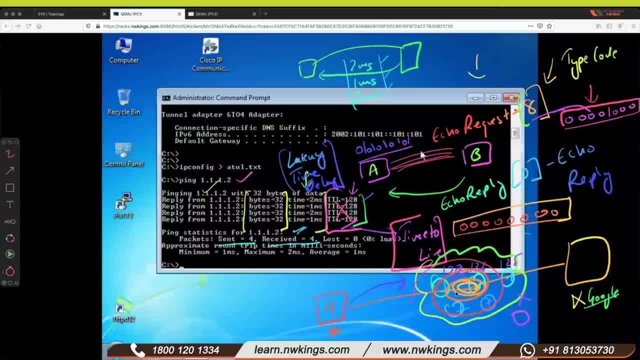 Yeah, Okay, Cool. Are you getting these things? Okay, Cool, Okay. It means TTL value is like expiry date. If we don't get in 128 routers, I'm going to drop this packet. So that has TTL value. 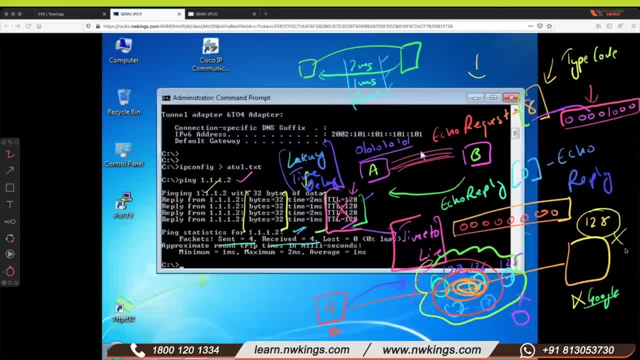 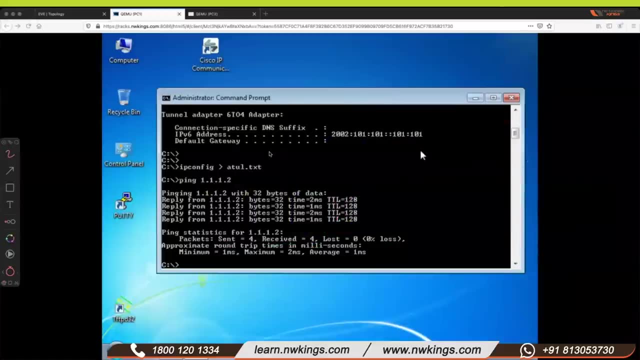 Okay, So my both PCs are connected with each other. Latency means a delay. Okay, If you are pinging from India to USA, definitely it is going to take time. That is latency. So 0% loss doesn't mean you will have drops when you have high latency. 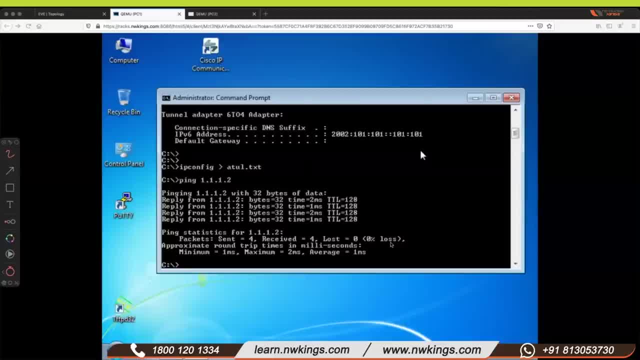 It means yes, when the packet is coming from very long distance. sometimes packet drops and it will show you lost here. Okay, So now what I'm going to do. I'm going to share one folder in PC1 and let's see if PC2. 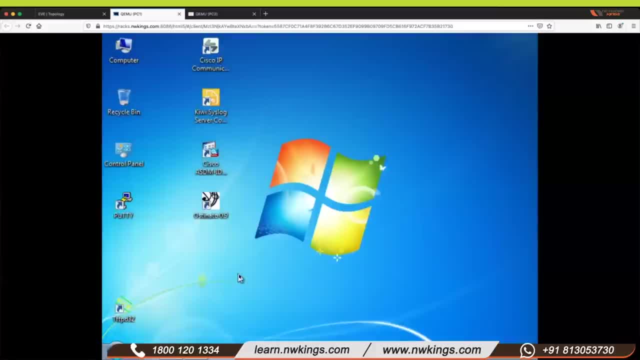 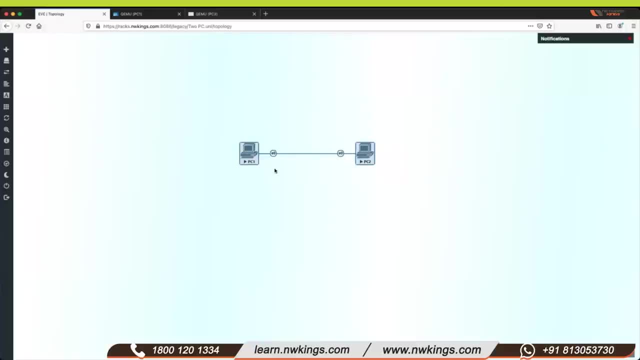 can access it. Okay, So this is the first thing we are doing. See, when two computers are connected together, that is a network, right? I explained you. I've explained you. This is: somebody is asking what ping actually command do. 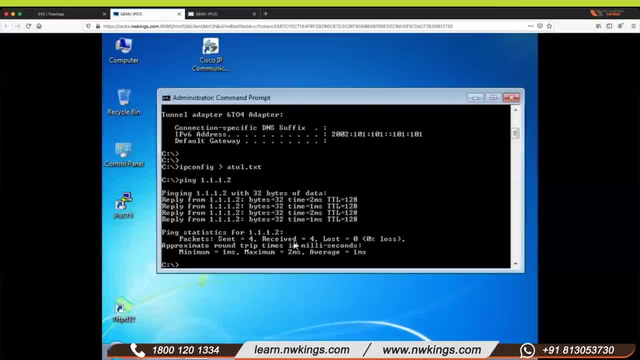 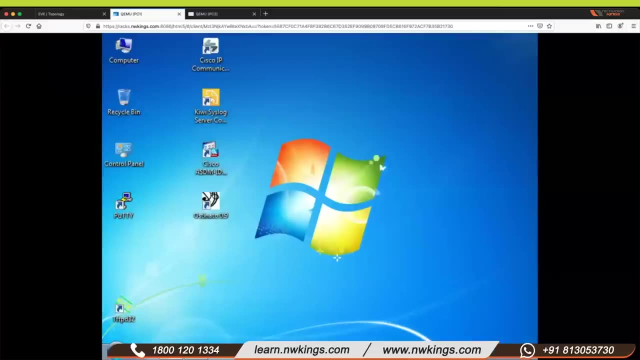 Ping is actually to test that another devices is connected to me or not. If I'm getting reply from another computer, it means both the devices are connected to each other. Okay, Can share files now. So let me share one file in PC1.. 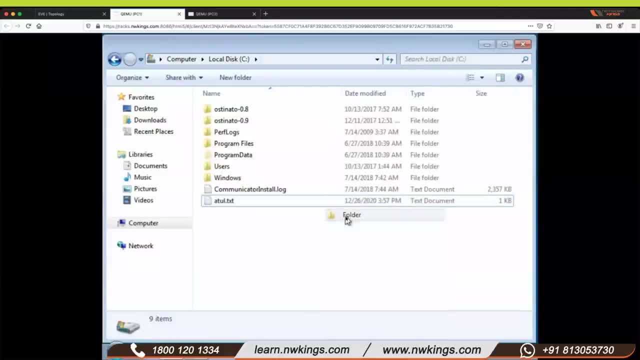 I'm going to create one folder, Okay, Suppose, I'm sure. Okay, So let's make a folder cabin here. Okay, So I'm adding this file in cabin So you can see, and let me just copy paste multiple times. 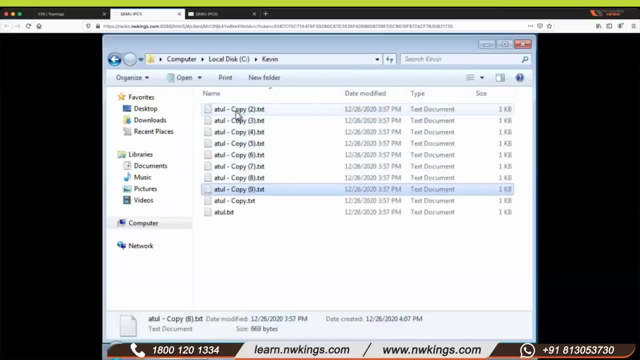 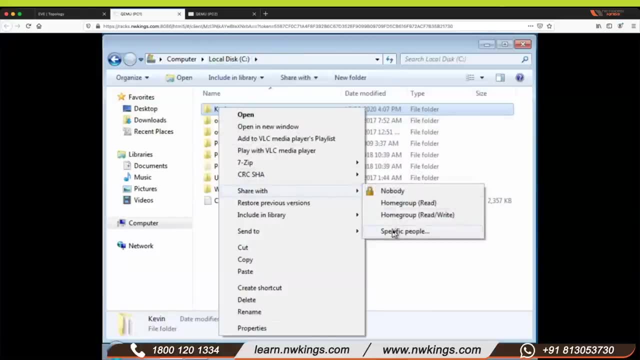 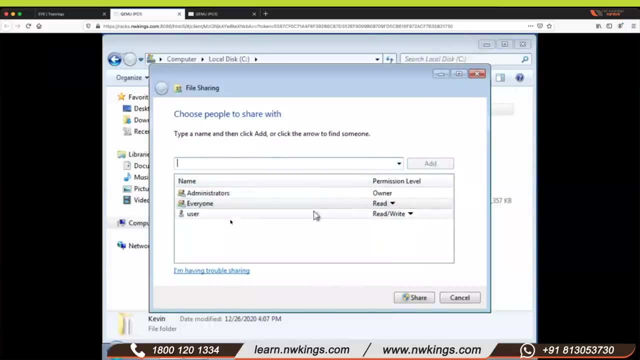 So this folder has multiple files. Okay, So I'm going to share this folder, share with specific people and I'm going to add everyone and I'm going to add: Okay, Just click here, Everyone add, share and share it. So now this cabin folder is shared. 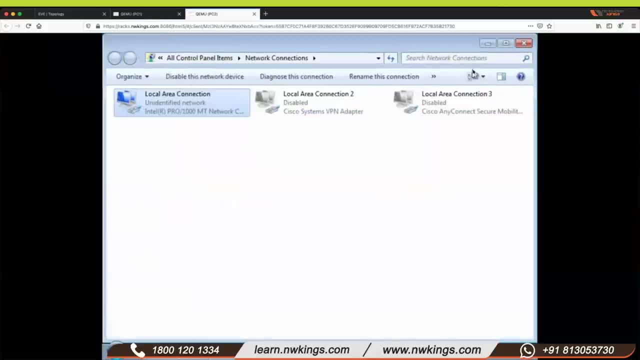 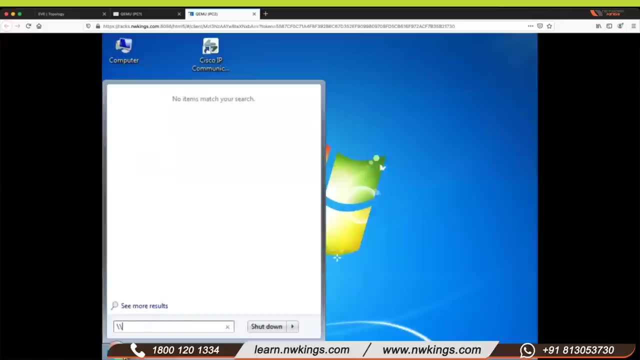 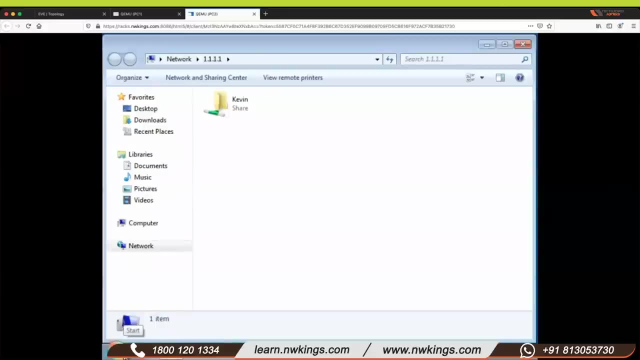 How to access from another computer. Now it's very simple. Just type here double slash and I'm going to type the IP address of foster device. Boom, We go the folder right. So you can see 1.1 in my network has shared the cabin folder and I'm going to copy this. 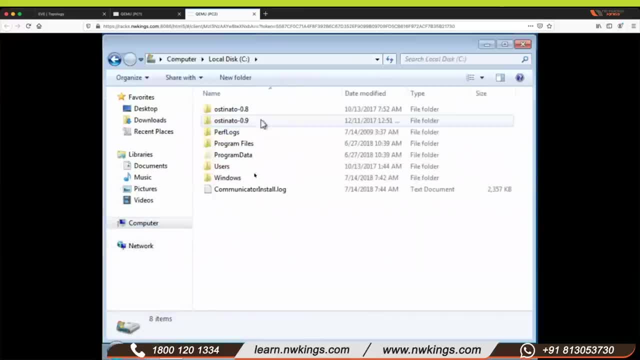 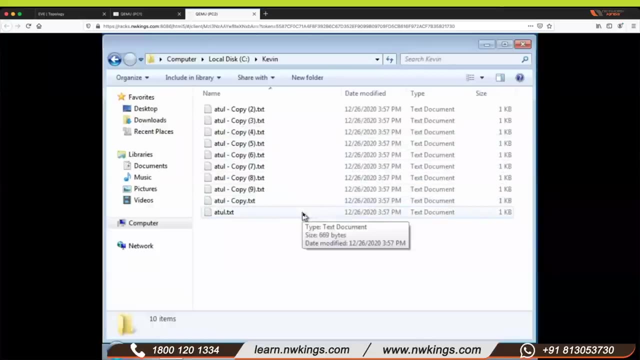 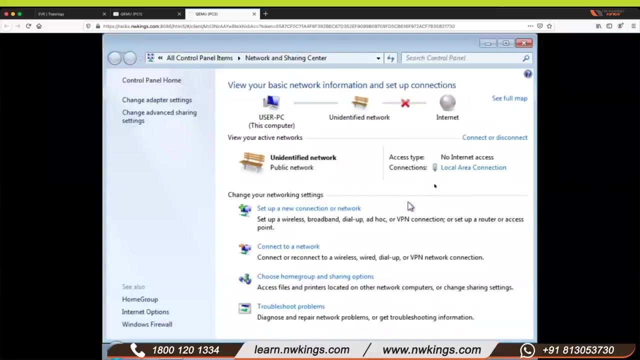 or we can Save, See in C drive. We don't have folder I'm going to paste here. So this is how we exactly transfer the files from one computer to another computer, Got it? Sometimes what happens? Uh, like you need to check your properties also, like advanced sharing settings. 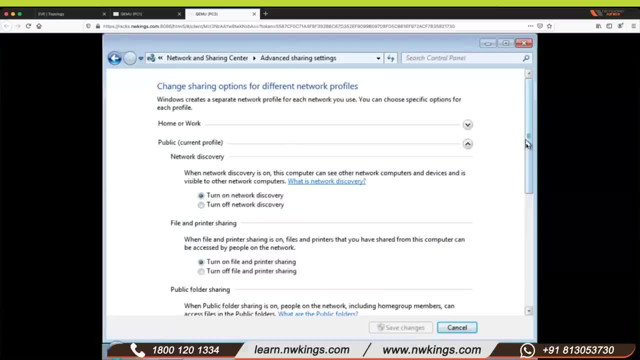 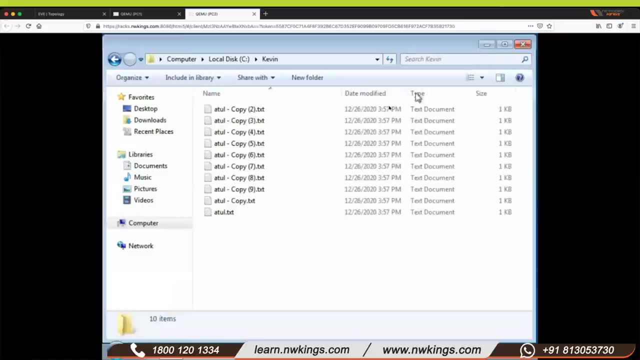 Sometimes your turn network discovery on file sharing. These are off, So you need to enable these ones. Then only you can access the folder, If you are not able to access from your real devices. sometimes, uh, like firewall is blocking or something is happening. 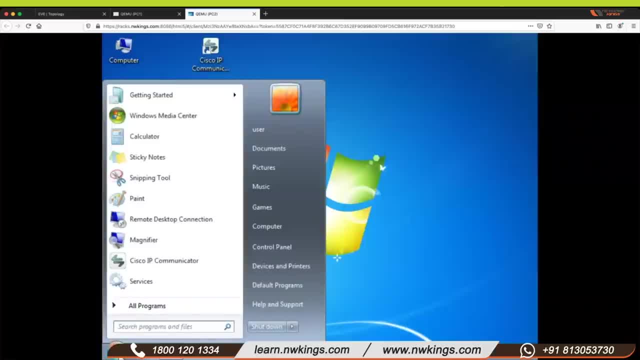 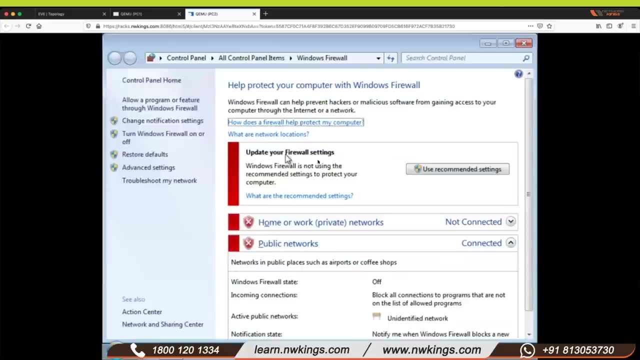 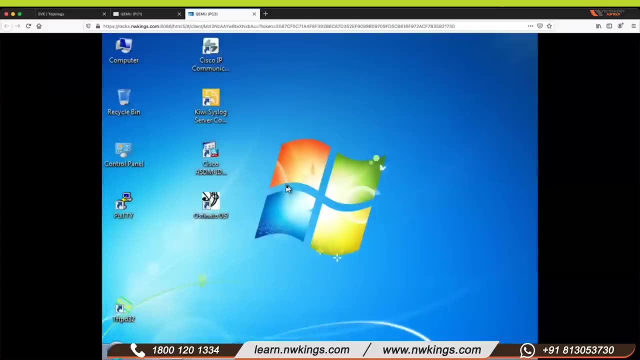 You need to figure out. Okay, Yeah, obviously. So sometimes you need to disable this windows firewall. Sometimes it is restricting you to share, So I have already disabled it. Okay, So this is how, uh, like, uh, you are going to do the first lab. 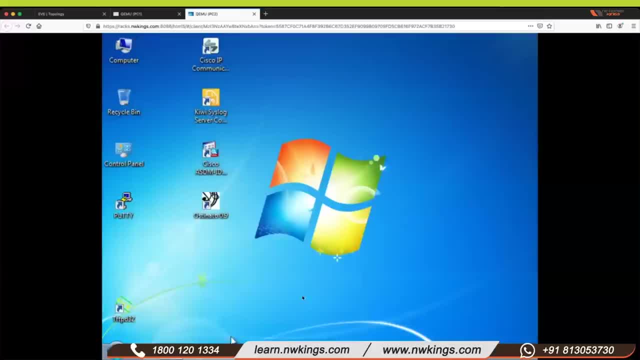 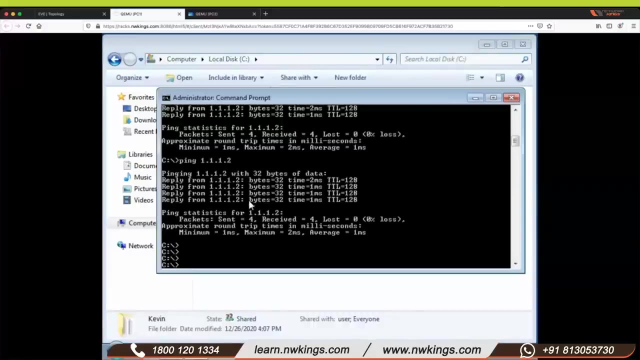 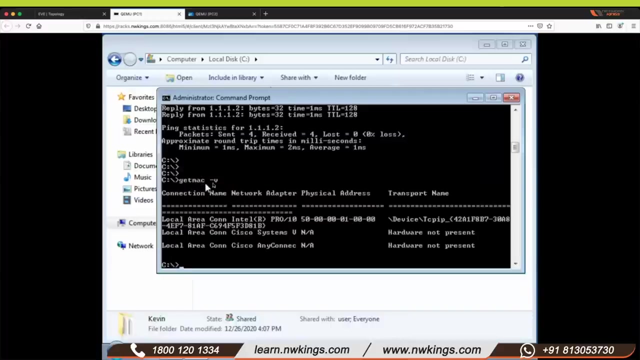 So this is for PC one, and let me show you a few other things. Okay, So there is a. so when we want to get the Mac address Of this device, there is a command command called get Mac hyphen V. So if you want to see all your Mac address, there is a command: get Mac hyphen V. 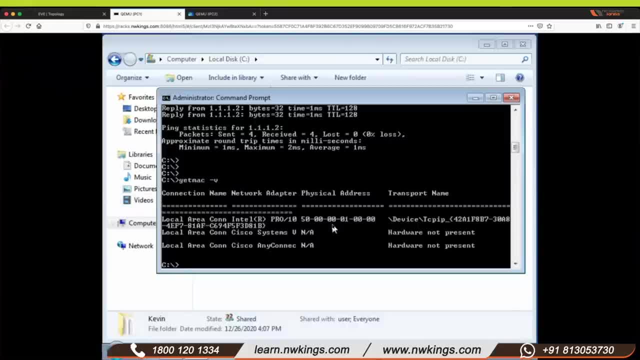 There is a command, also IP config, slash all. But if you want to see all your network adapters, Mac address. so this is the physical Mac address. You can see here: 50 dot 0, 0 0, 0.. So this is the Mac address. 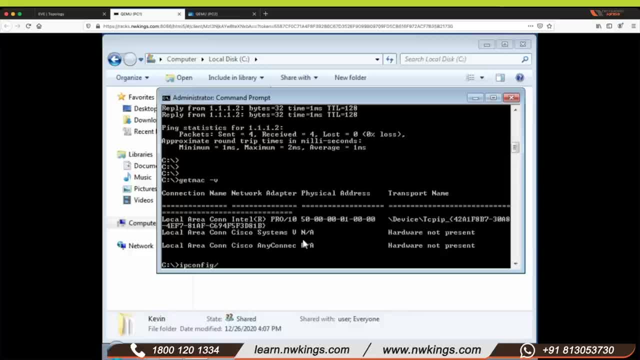 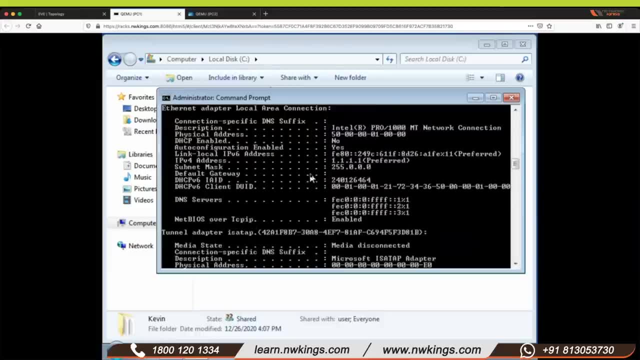 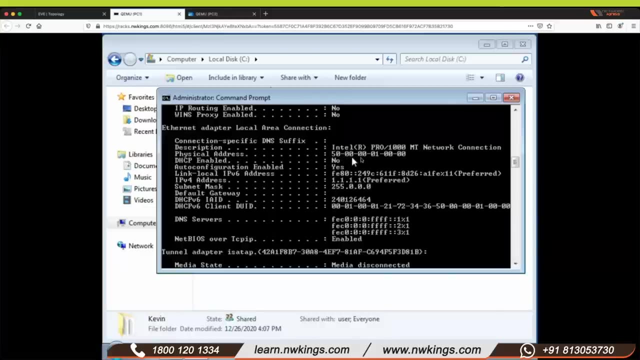 And there is another thing like IP config slash all. So it will also display you the Mac address. So you can see, here I'm using some this technology, Intel empty network. So this is my Mac address: 50 0 0, 1 0 0, 0.. 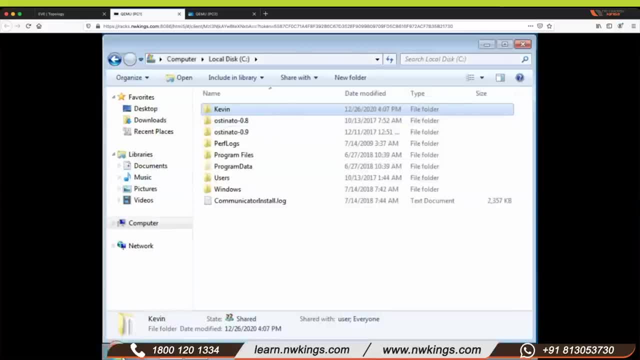 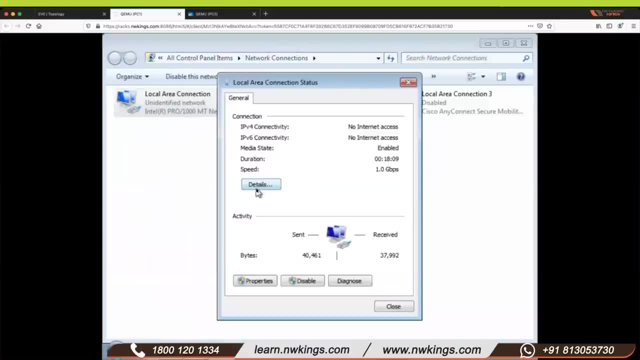 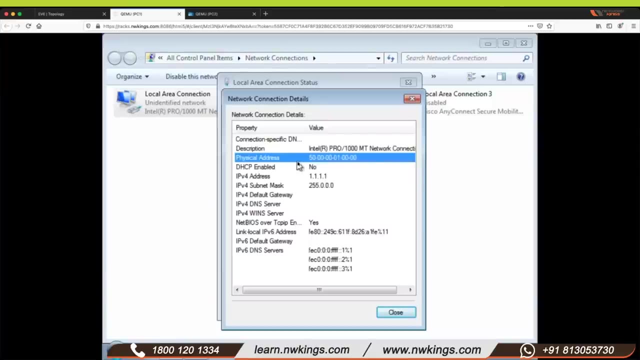 And if you want to see in a very simple way, so just again go to that N C P a dot C P L And I'm going to click over here status Details And here also you can see your physical Mac address. 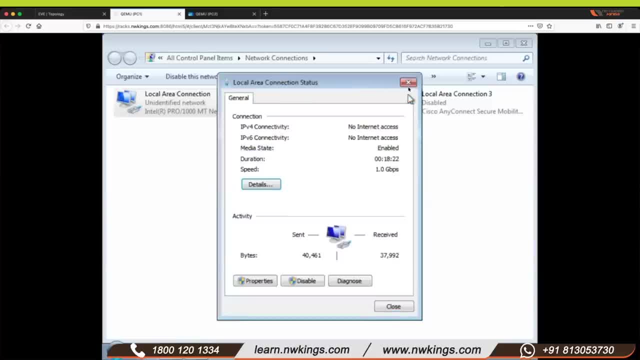 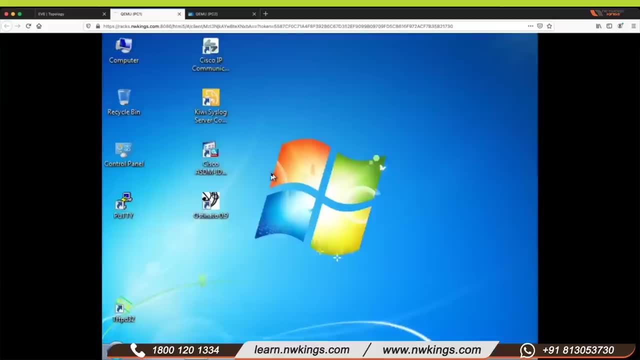 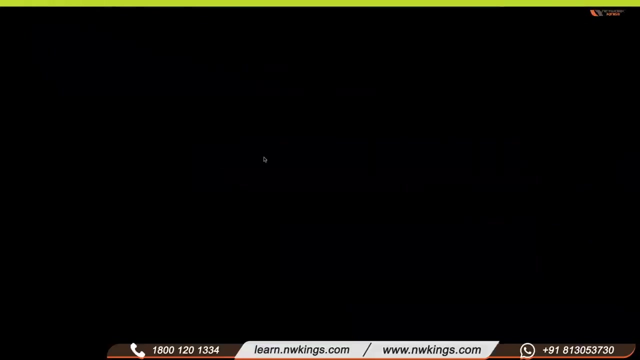 Okay, cool. So now yours uh homework would be like you can check with the class B, class C, Okay, Okay. So I'll show you something today. So what is IP address basically? So IP address is basically Okay. 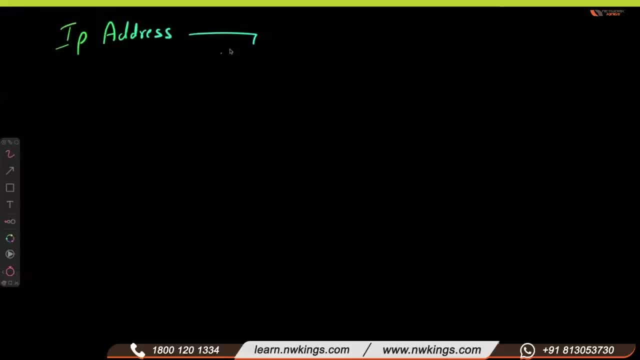 Okay, Okay, Okay, Okay, Okay, Okay. So IP address is of two types. One is IPV4.. And when we have, we have YPV6.. So this is 32 bit IP address. It means it's a combo of 32 zero ones and it's a combo of 1, 28 bits. 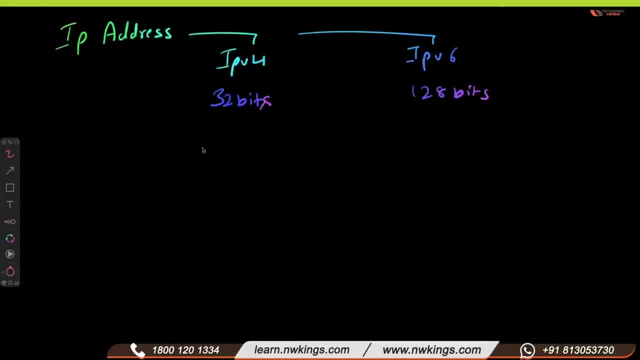 You remember bits, right? So zero and one is bits. So IPV4 is in the form of four groups, four groups, Okay, And that is into decimal format, like IP addresses, 204.. dot one, dot one, dot one. this is a decimal format. when we see ip version four, it represents into: 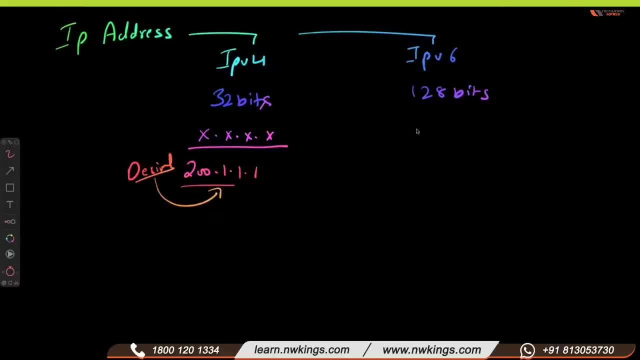 the decimal format and in ipv6 we have a groups, eight groups, eight groups, and here, oh like group is known as octet, and each group is of eight bit. all groups are is of r of 8 bit, and here each group is of 16 bit. so 16 into 8 is 128, right, so 16 bit group. 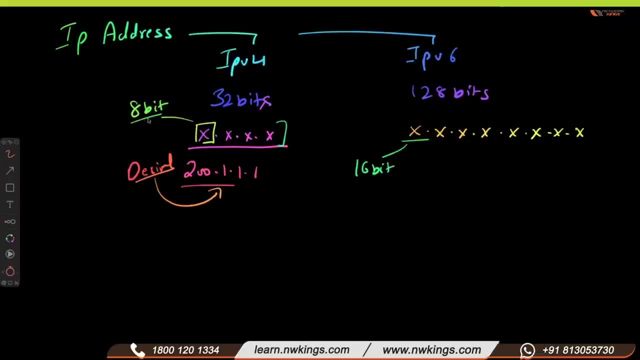 and here we have 8 bit group and 4 groups. so 4 into 8 is 32. so if you plus all 8 bits- 8, 8, 8, 8- you are getting 32 bits. and here we are: we have 16 groups and 8 groups. it means 128 bit. 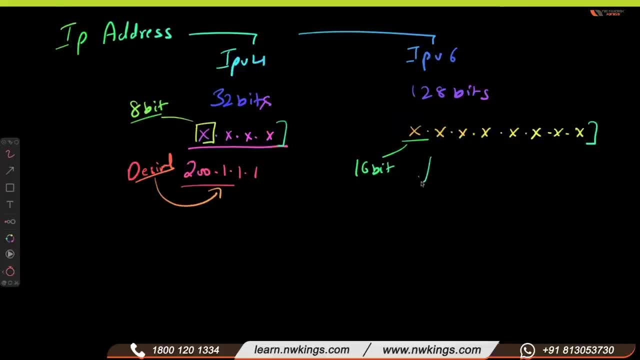 okay, and here uh, the ip address looks like this: 2 0 0, 1, 1, 2, 3, 4, 0, 0, 0, 0, kind of 0 0 0, okay it it's. it's actually big address, so i'm trying to just 3, 4, 5, 6. 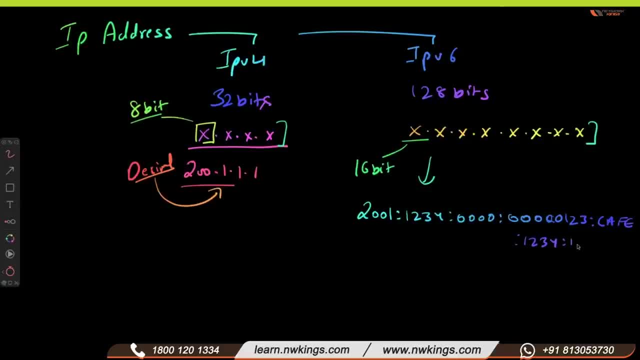 okay, this type of address- very big address, you can see it's very short and easy to remember. okay, this type of address- very big address, you can see it's very short and easy to remember. here it's complex, but, yes, there is a way to shorter this address also. okay, so we can place. 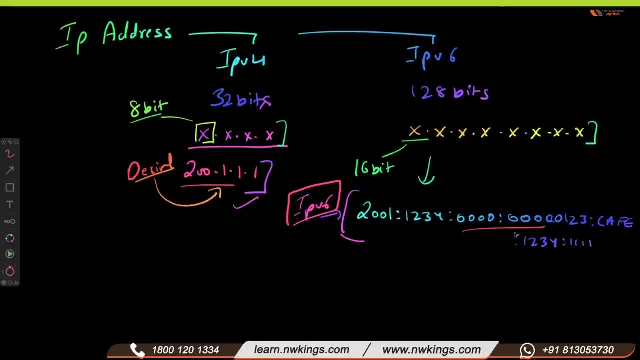 double colons instead of zeros. okay, so we will discuss this later on, okay, but ipv6 looks like this address and you can see some cfe, abcd and all these terms. this is known as hexadecimal. why we use ipv6? because we have a short address and we can place double colons instead of zeros. 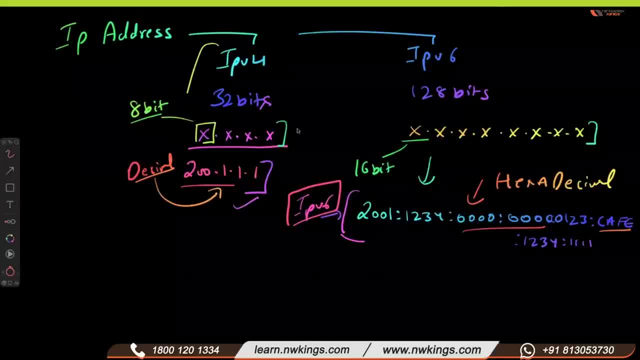 because we have a short address and we can place double colons instead of zeros. if, when we add, you can see the couple dot alt p and we can name them. if, when we add, you can see the couple dot alt p and we can name them now. 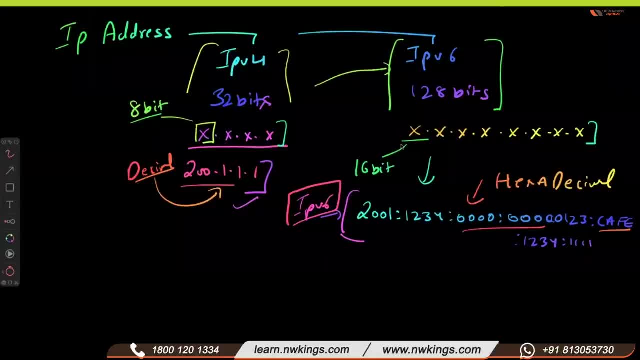 because the only difference, the sub setting you have between serializ- and this is the reason why the ipv6 belongs here- approximately, hmm, okay, if we add. so if you learn this computer, and then what i want so to start learning beloved heres is some common thing that I want: mineralize. you have to understand. it is very direct, you have to. 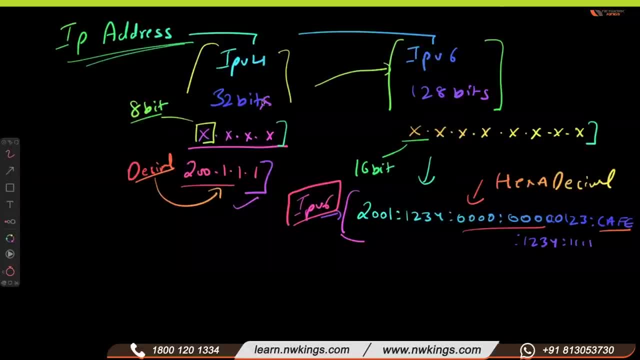 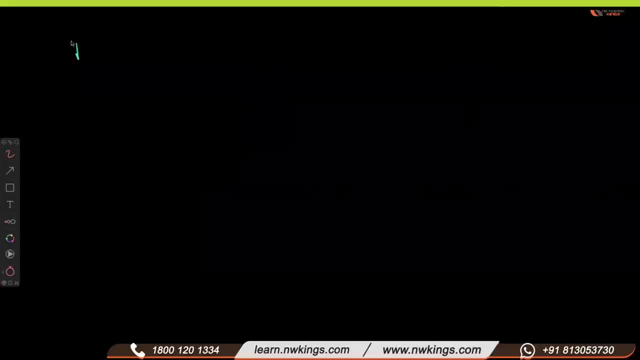 understand. it is very direct. you have toose understood this. you have to understand its circuit to decimal, all other things. so just a quick intro. I'll give you overview about what is decimal to binary and why it's important. I'll show you, trust me, if you already know this thing, but still you. 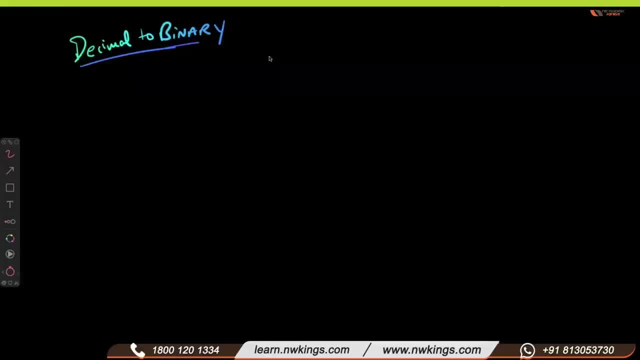 are going to learn something new today. suppose we have IP address 192, 168 dot 1, dot 1. so this is a decimal format. your computer does not understand decimal format. your computer understand binary. so these things we are learning from our school days: that computer understand binary. 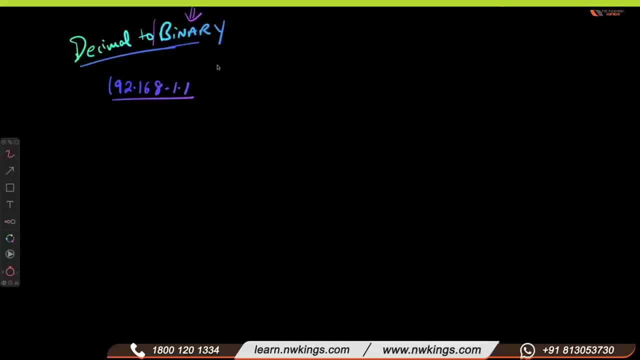 language, machine language, right? so how computer is going to understand this IP address? we also need to understand that thing. so, IP address, I told you this is of 32-bit and each group is of 8-bit. every group is of 8-bit. and how we represent this, because 0 and 1, how many values are the? so 0, 1 it. 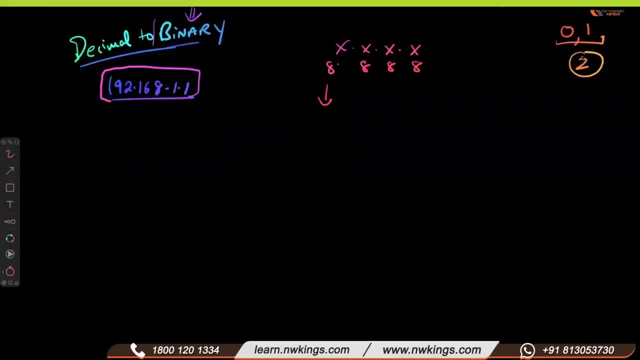 means this is a 2 right, it's 2 values. so this is this is the reason we always take the combo of 2, so we can take to the power of a to represent 8 bits. how we are going to represent it: we start with the power of 2, from right to left, to the power of 0. 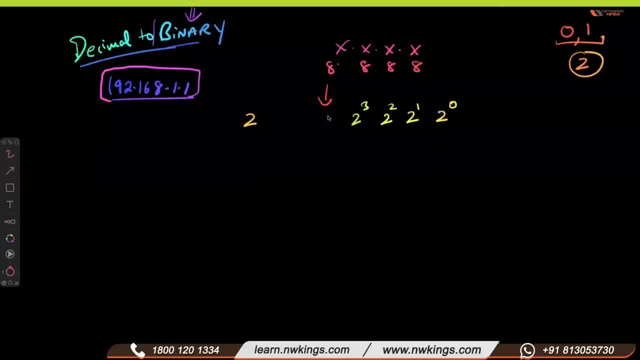 to the power of one, 2 the power of 2 to the power of three, 4, 5 to the power of 6 to the power of 7. so if you know these things, that's good. so 2, the power of 0 is 1 to the power of 1, is 2 to the. 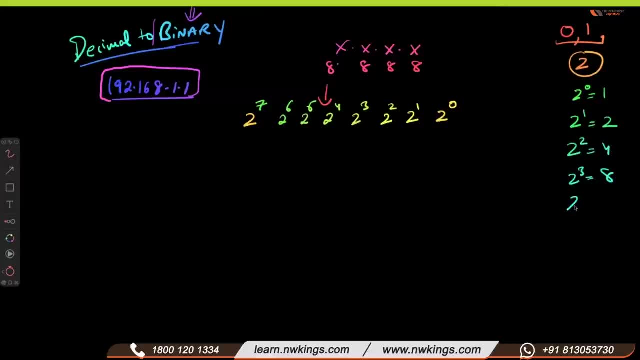 power of 2 is 4, 8, 16, 32, 64 and 2. the power of 7 is 128. right, and so this will take us to the power of 7, to the power of 8 is 255.. So now, if I want to write 192, so I am going to write first. 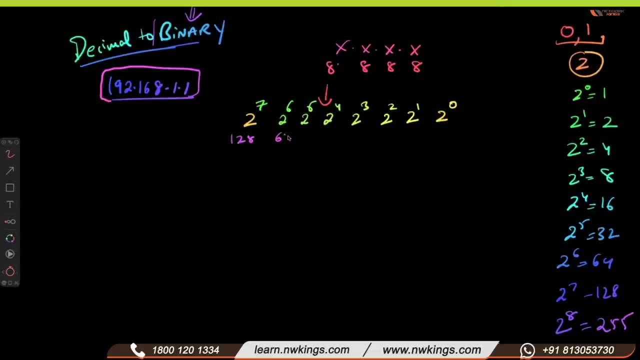 all these values here, like 128. You can just note down. if you want to pen down this, you can pen down 4,, 2, 1.. So how I am going to make 192?? Very simple, Just take group of. 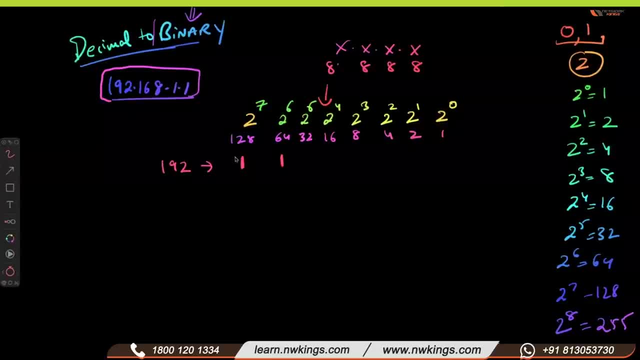 128 plus 64.. 128 plus 64 is 192 and put all the values which we are not using, 0.. Yes, Very simple, right? So just take for 168,. very simple, just take 128 plus 32.. 128, 32. 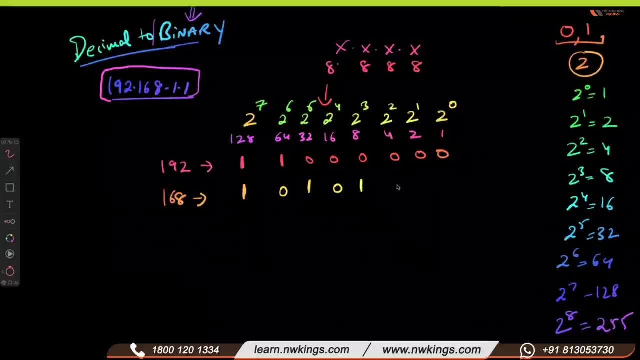 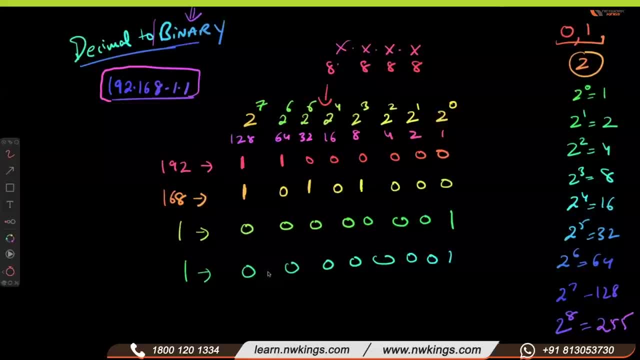 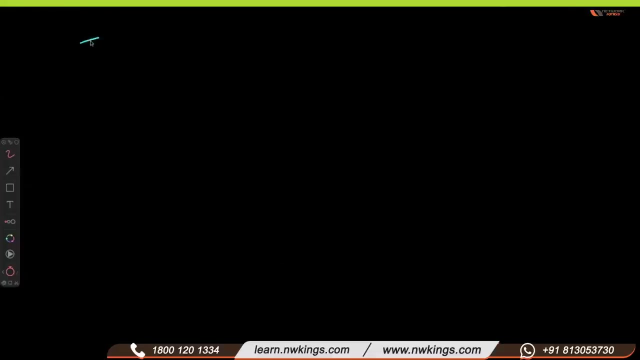 0, 1.. If you understand, just type yes in the chat section. Okay, cool, Now I am going to show you why we have classes in IP version 4.. Okay, Let's go ahead. Yeah, So now there is an organization known as INA Internet. 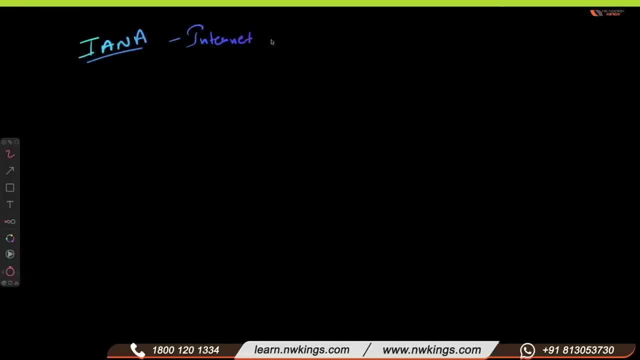 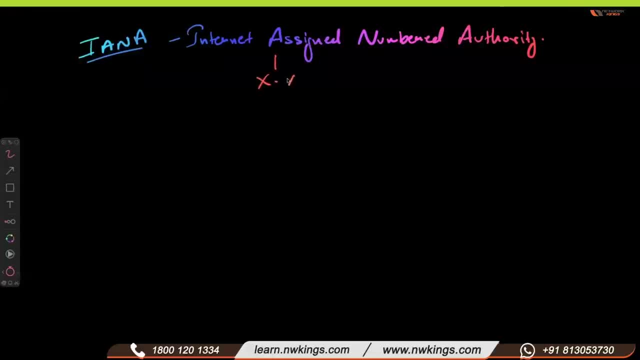 thing here. Like we are going to take one octet, Like we have four groups, We are going to write the same here to the power of 7,, 6,, 5,, 4,, 3,, 2,, 1, and 0.. So just write down the values 128,, 64,, 32,. 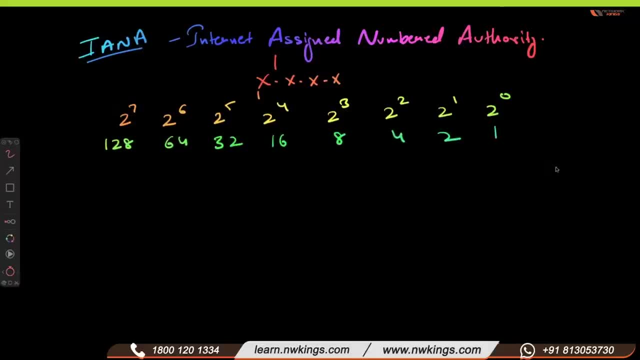 16,, 8,, 4,, 2,, 1.. Okay, So let's play the game. So what INA has introduced? it actually made the groups like: in the first group we are going to take all values 0. So it means what value I am. 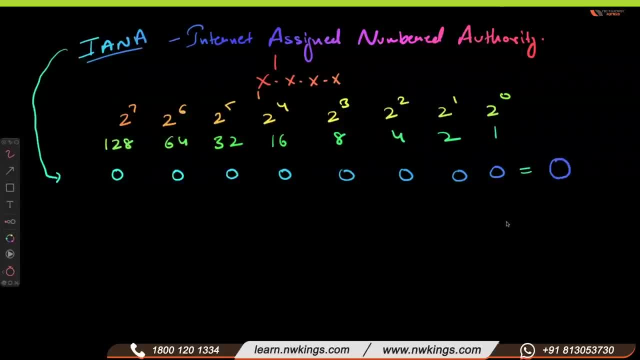 going to get here 0,. right In the second group. I am going to take 1 here and rest. all my values will be 0. And it means if we have 1 here, it means I am going to get 128 here. 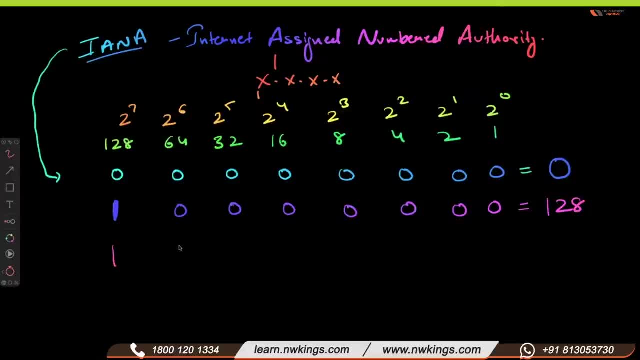 Okay, And in the, in the third group, we are going to add two 1s. It means what value we are going to get: 128,, 64,, 192.. And here we have three 1s and we are going to get 224, right, And in the another part we are going. 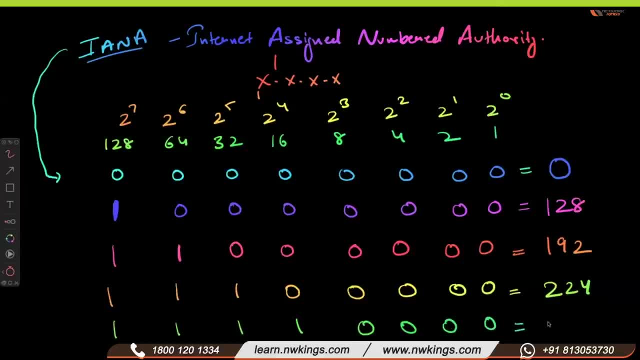 to take four 1s, 240. And what would be the maximum? if we plus all values, we get what value? 255. And what comes before 240,? guys, That is 239.. What comes before 224,, 223?? What comes before? 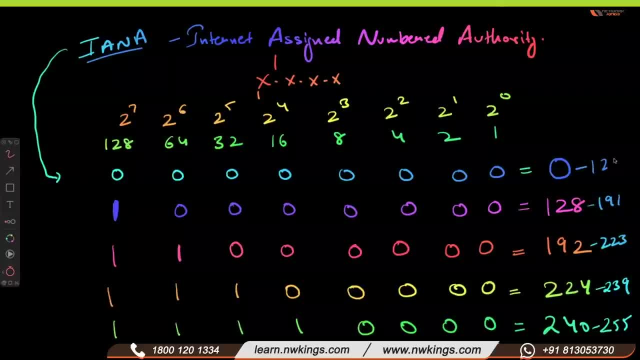 192, 191? And what comes before 127?? This is A, B, C, D, E. Enjoy, Okay. Okay, This is how INA formed IP addresses, And you don't have to cram every time. Just remember this. 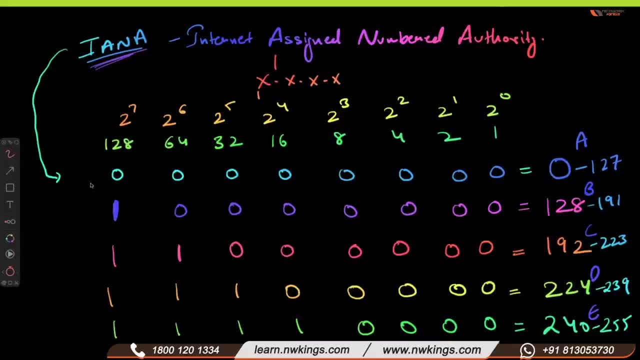 formula And it's very simple: In the first group we are taking all 0s. When we plus all 0s we get 0. And here in the second group, in A class, all values are 0. In B class, just take one. group C. 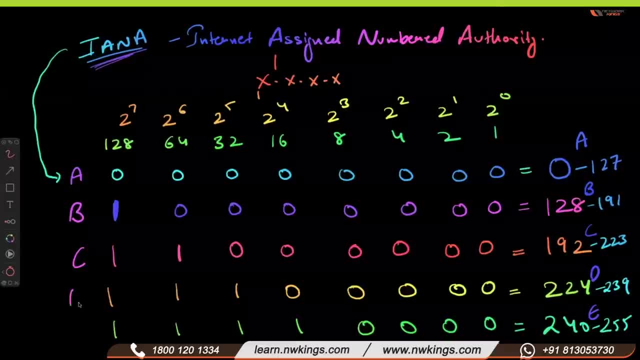 we are going to take two 1s. In D we are going to take three 1s. In E class we are going to take four 1s. So that is the actually representation of. Yeah Might be some of you are thinking like I have gone through to hundreds of books. This formula is not in the books, or maybe over the internet. 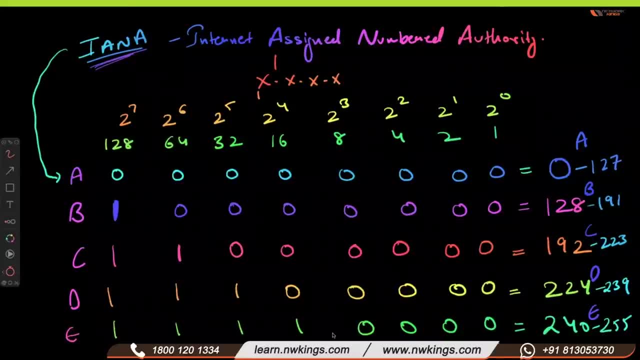 How tener knows these things. Or might be there are, But it actually 127 is actually Class A, but we don't consider this. 0 and 127 are reserved. So 0 and 127 is reserved. So how i got to know is that when we also ask questions about ourselves why we have to do it all to one who has no idea. 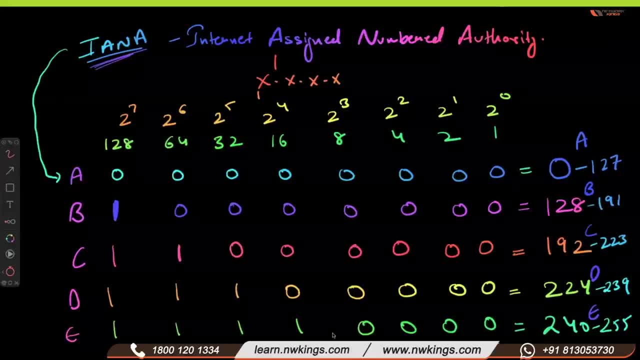 Like I am not like a genius or something, Hollywood, Because I've been listening to how we interact first, like in the sense of how we behave in anyaretti, where students just we're sommes-verses, or how you behave. Yeah, there is a whole lot that's going on here about this thing. 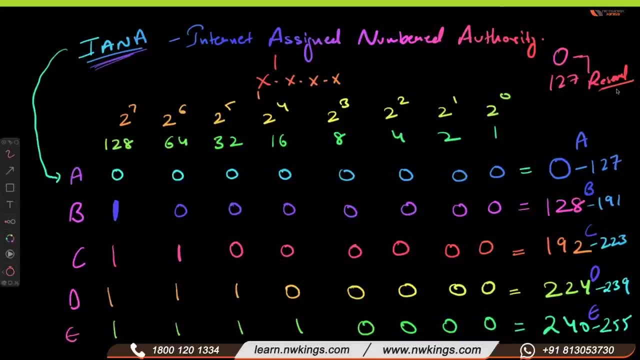 And, like you just call, here we connected. It works because we're from the other community too. when i was in college, i was like i used to think in this regards, like why they have made the classes right, so we always remember the classes, but we only like used to cram, but this is the exactly. 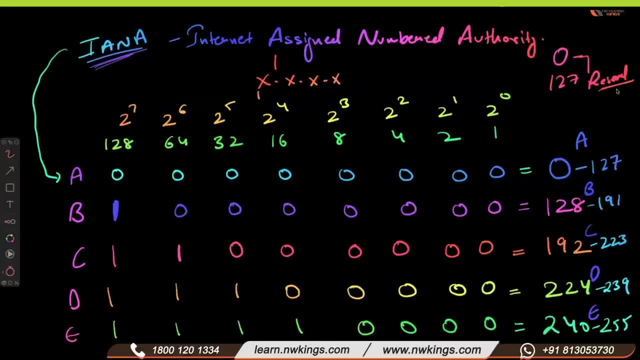 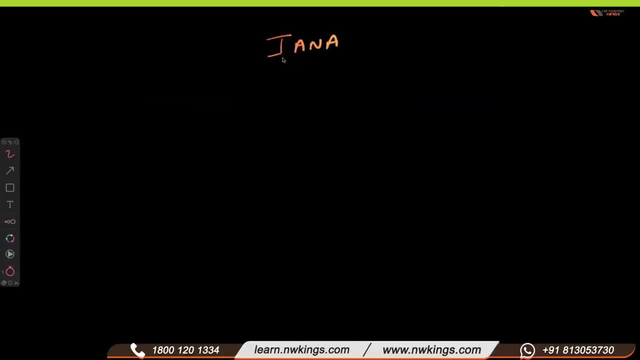 reason? okay, and do you know this? like, if you want to buy ip address, you can't directly go to aina. so aina has formed far ah, what we call this rirs. so aina has regional internet registries, so these are known as regional internet. 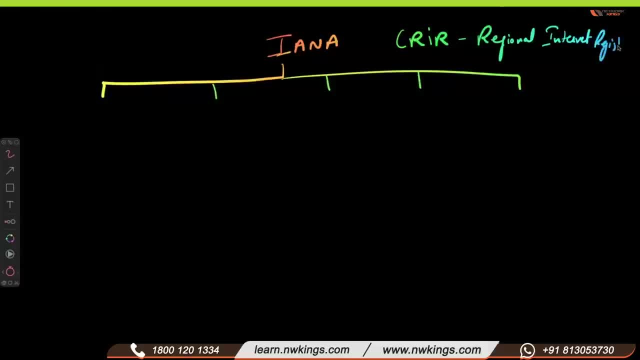 registries, registries. so first registry is like america registry for america erin, for asia that is apnic, for latin america that is latinic, for russia that is ripe and for africa that is african. so this is by continent, wise right. and if, uh, i'll discuss about apnic because i belong to this. 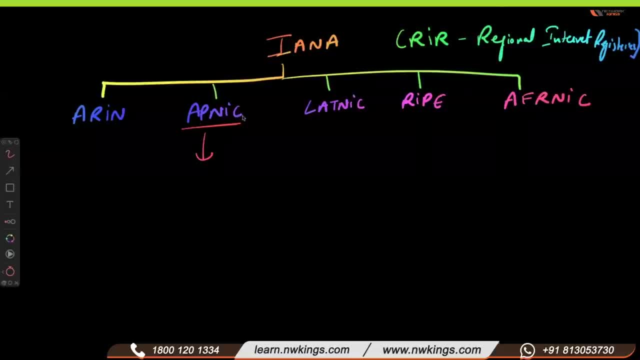 so that is asia pacific network information center. okay, asia pacific network information exchange something, so you can just check it or google it. so i highly recommend you this to go on. so if i want to buy ip address in india, so this: i want to go directly to apnic, not to aina. 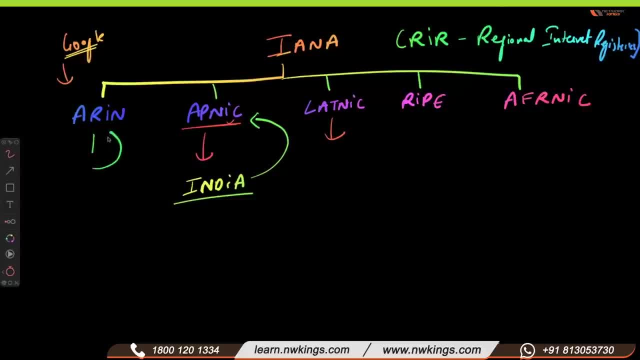 if i want to buy a ip address in america, i will contact erin. yeah, aina is not a go. yeah, it's a kind of government body, but now it's uh like, uh, what we call this. it's for all kind of it's a government body but it's organization now, or like. 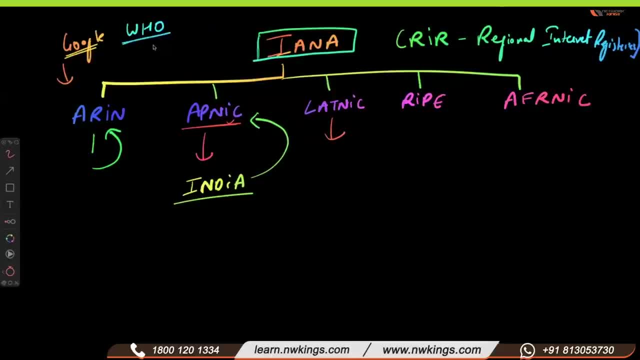 like: uh, what we call this wh, it's a or a government, or it's a global organization, right, so it's like that kind of yeah, centralized, okay. so i had an apnic latinic, ripe african. so america registry information numbers, asia pacific network information center- latin. 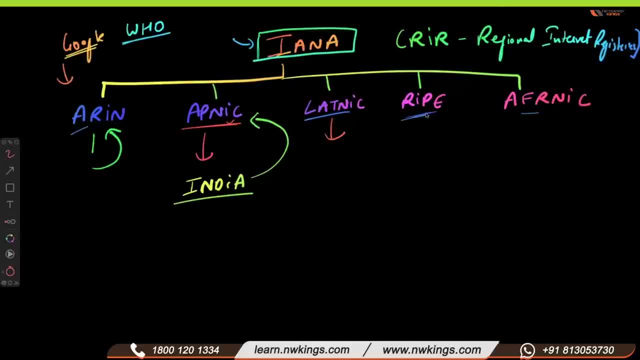 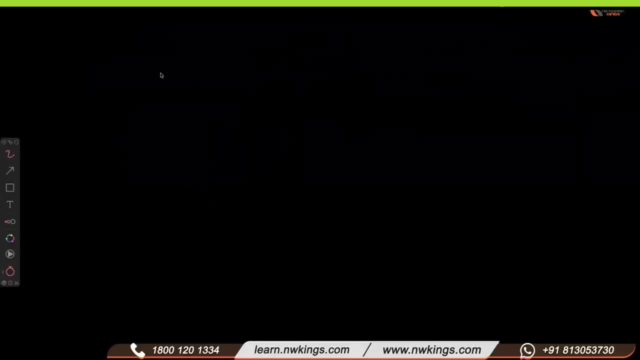 america network information center, so that stands for resux internet protocol exchange. that stands for africa network information center, so that stands for resux internet protocol exchange. that stands for freqa network information center. okay, so go and check it. so now, uh, one question that arises from where we are getting internet. like, uh, i'm getting internet from one isp, that is atl. 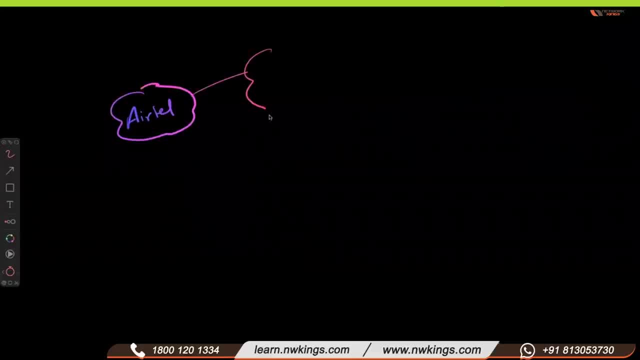 but from where atl is getting the connection? maybe from different isp? maybe let's take atnt. from where atnt is getting the connection? you must be thinking that, uh, maybe they are taking connection from uh somewhere or some kind of isp. it's not like that. so internet, i told you, internet is a network of networks. so atl, atnt, sprint when they are. 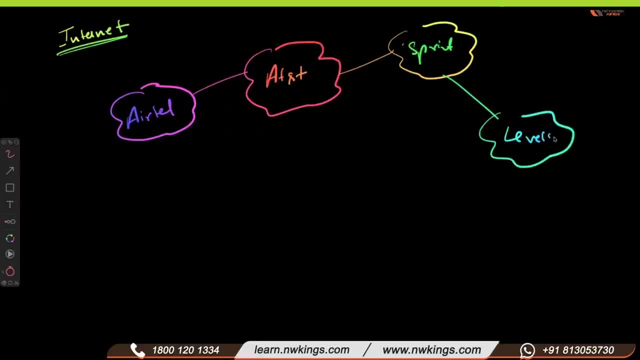 actually connected each other. when all the isps in the world, like tata, uh, like telstra, all companies or all like all isps are connected together, they are actually making internet. so internet is not coming from anywhere, right, it's a combination of all the networks are connected. 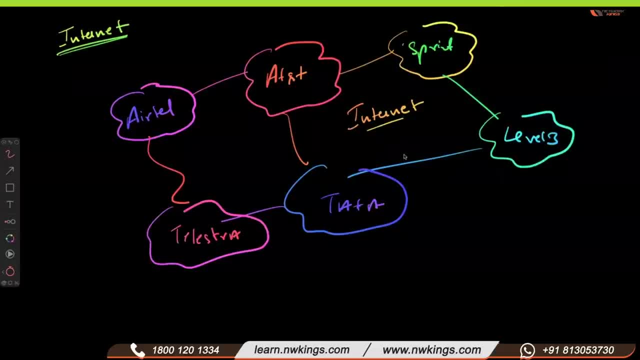 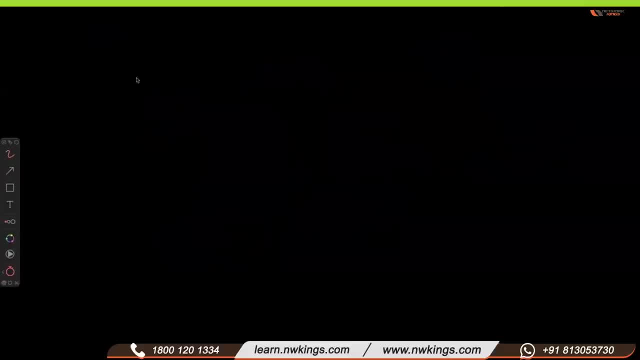 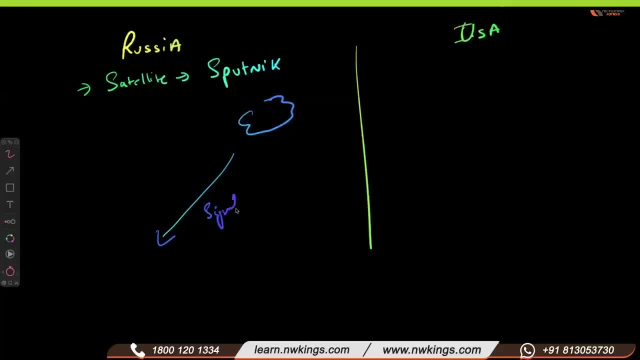 space and they are getting signals. and when they are getting signals somebody is jealous. and they actually made two organizations, that is, that is a darpa and nasa at the same time means it can be a delay between them, but they actually started two organization. you already know this right. so darpa is defense advance research project agency. 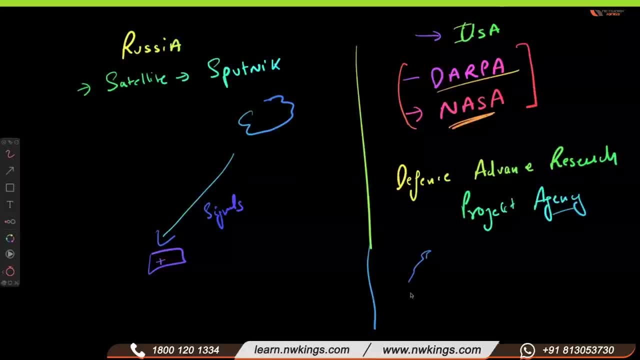 so actually, what they have done? so they have, like in usa, they have underlay the cables to connect multiple defense sites. okay, maybe new york, maybe, uh, somewhere like another areas of us, right, the laws and all texas and all. so all the areas are like under uh, like the cables are under uh. these cities are connected for the connectivity between army. 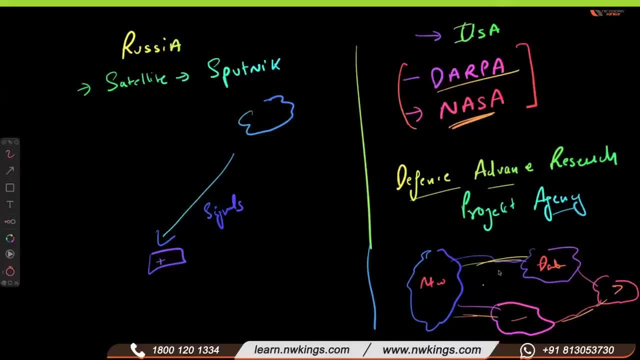 projects, or maybe something is going with right. so basically, this group is made to create a network so that all the cities or all their armies can communicate with each other. so when this project got famous, they actually released a public version of it that is known as advanced research project agency, that is, arpa. they formed another arpa. 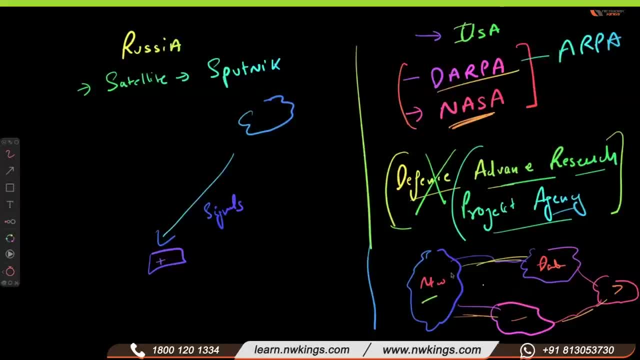 okay, so arpa means when they launch this, they asked, like, when we create a big company or big, like, suppose i'm a builder, okay, i'm making a very big, uh, uh, like i'm making 1000, 1000 flats or maybe bigger or big project. so i'm going to ask investors to put down their 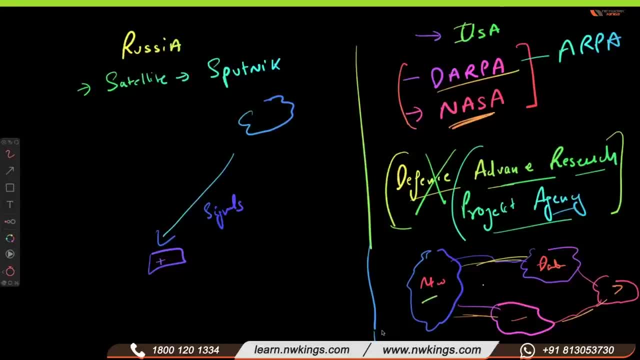 money in my project right. so when advanced research project agency came, like some investors, like those are known as now isps- like they came into picture and they invested to put down the cables to connect the cities, like when people are actually investing to create a big network- now they are known as. tier one isp. so what is tier one isp? those who actually actually invested in the cables. so that is known as tier one isp. so there is a like to become a tier one isp. tier one isp is like the king of isps, you can say that. so tier one isp is actually giving. 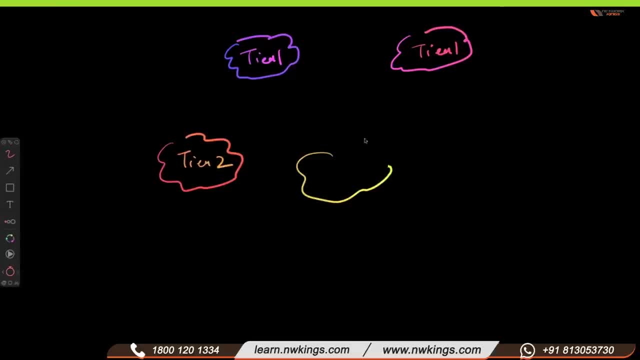 connections to tier two isps. there are a lot of tier two isps in the world. also, all they are taking connections from tier two for the backup they're taking from multiple tier ones and these tier 2 isps are giving connections to the local ones. 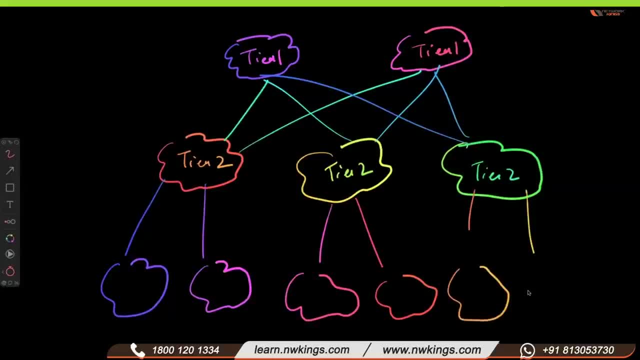 which are known as tier 3 or local isps. so these are tier 3 or we can call these local isp. so these are very small isps, like maybe you have in your hometown but it's not in another cities. tier 3 and users can connect to these ones also. these ones also, and these ones says who are tier. 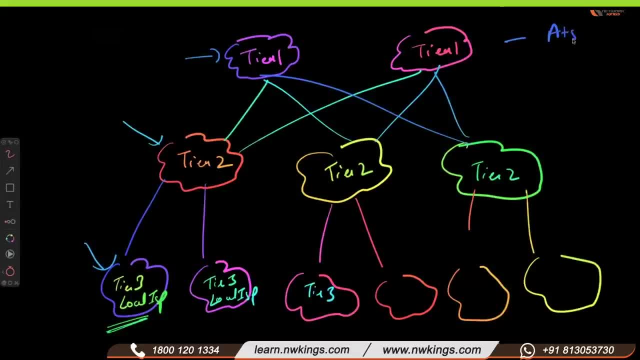 one like i remember few names, like at t level, three okay sprint comcast cables. so these are from all us. so in canada it's, i think, rogers cable, or maybe right in ua australia's telstra. in india only one name, tata communications. uh, japan, and all they have singtel. 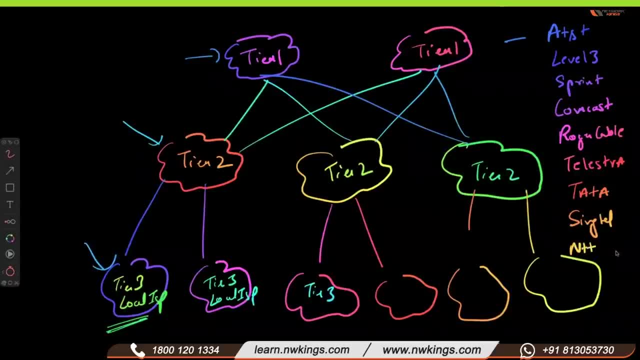 like there is another one entity, communications, so you can just google it: tier 1 isp, you will have around 15 to 20 names. means only 15 to 20 isps in the world are actually investing in big projects, and that big projects actually they are investing in most of submarine cables. 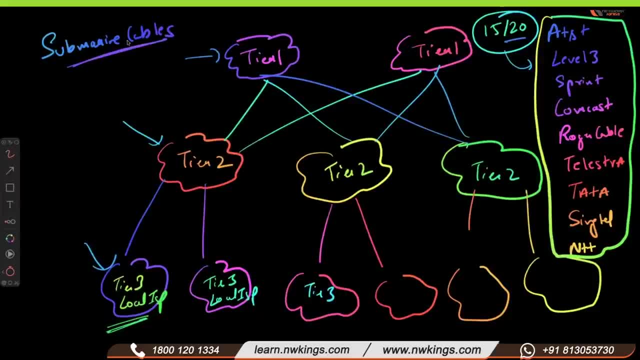 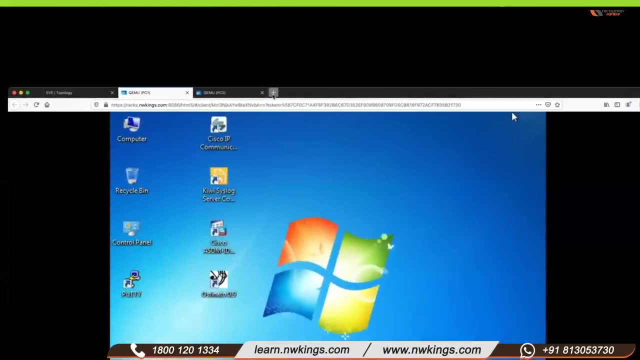 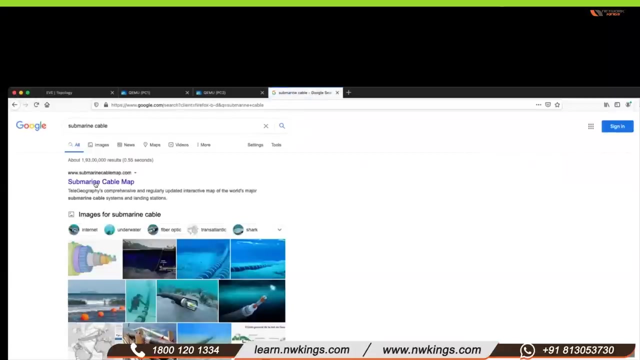 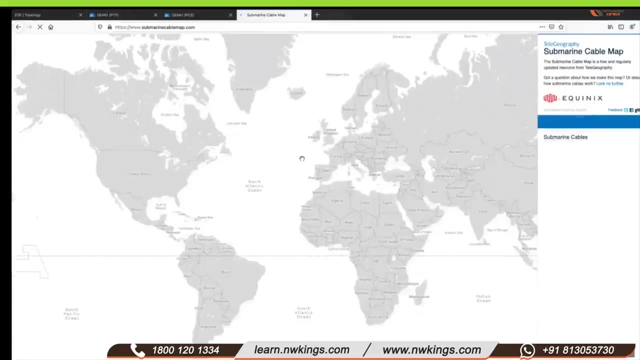 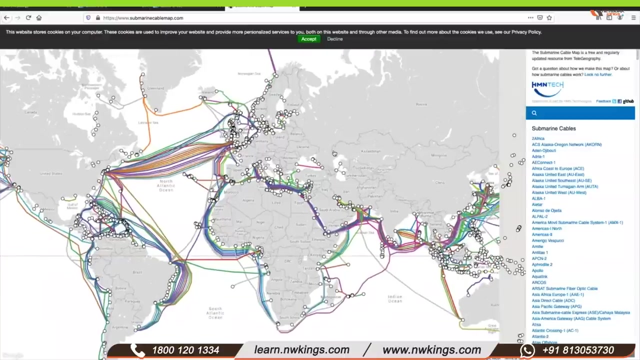 so i will show you the last thing of this class today so that you will have good dreams of submarine cables. so i am going with the map: submarine cable. okay, just go and check this website. so all these are cables under c, which is actually connecting all of us to have this zoom session. 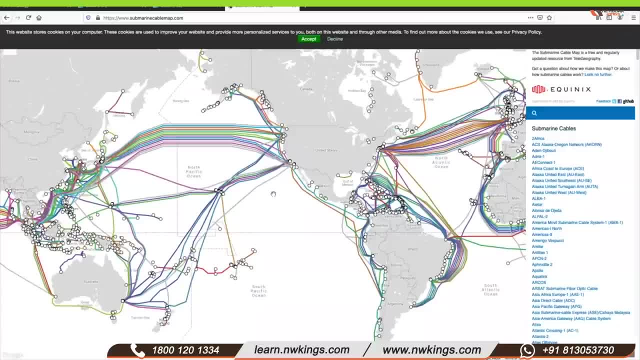 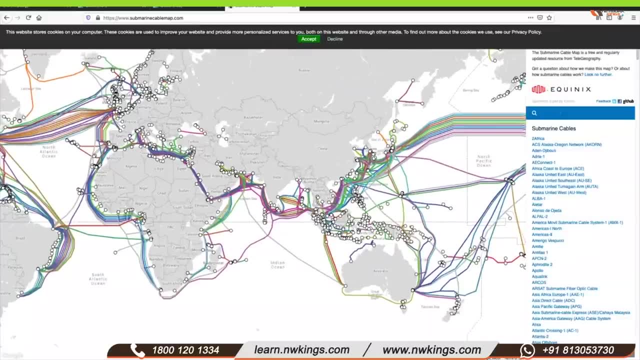 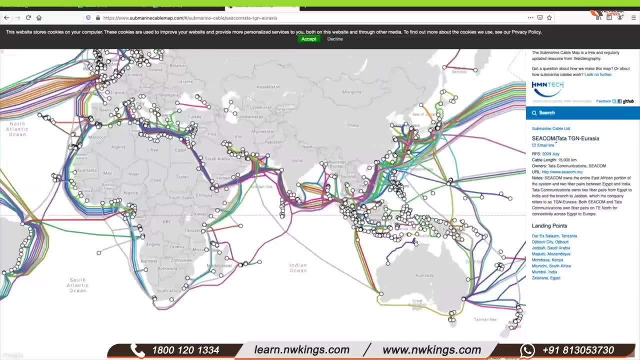 this is the main purpose, okay, so. so all the countries are connected and if you check tata here, so there is a lot of list here. so i can just click on the list and you can see. this is a cable which is known as cd. so if you click on this you will see that this is the whole list of the cd's. 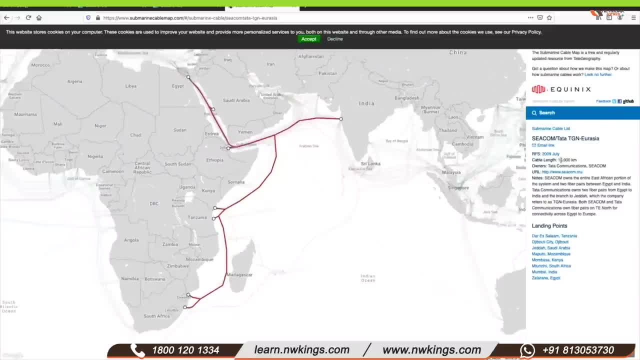 which is known as ccom, which is actually a 15 000 kilometer cable which owned by tata. so i can check another. so why tata is tier one? i am showing you why tata is tier one. because they are not actually. tata is from india, by the way, obviously most of you know, uh, but yes, why tata is tier one? i mean, 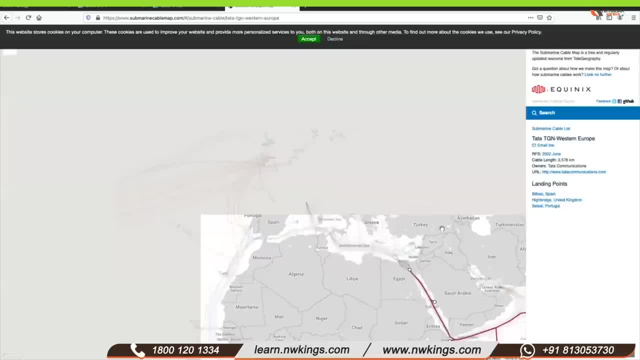 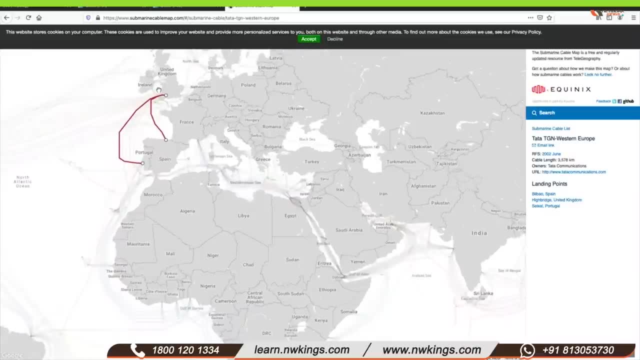 i am giving you example because they have. they are not actually only investing in connecting india- even we are, even tata is from india- but they are actually connecting uk to france, spain and portugal also. so you can see, this cable is a tata tg in western europe cable and it's not 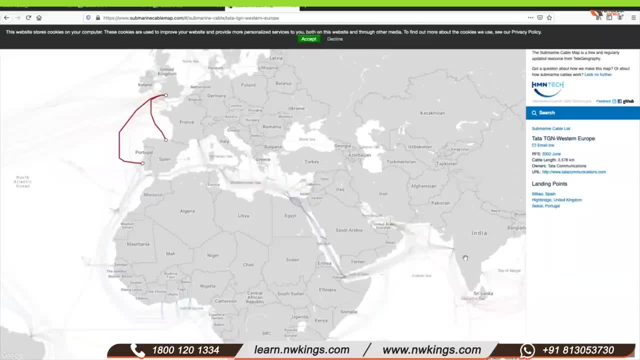 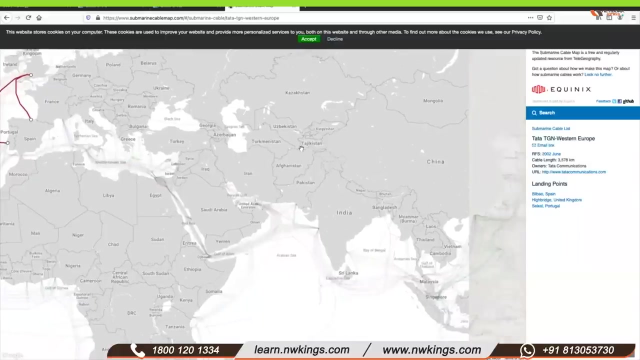 coming to india. so everyone used to think tata must be deploying, or this, adding, these cables for india. no, tata is a like an investor. this is the reason they are known as tier one isp right, so this is how we check and if you want to see any particular location, or any, if you are from, 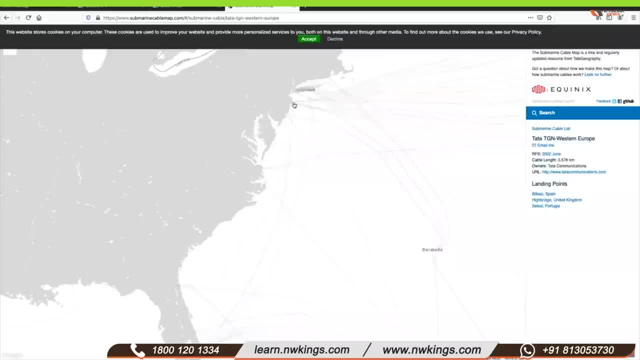 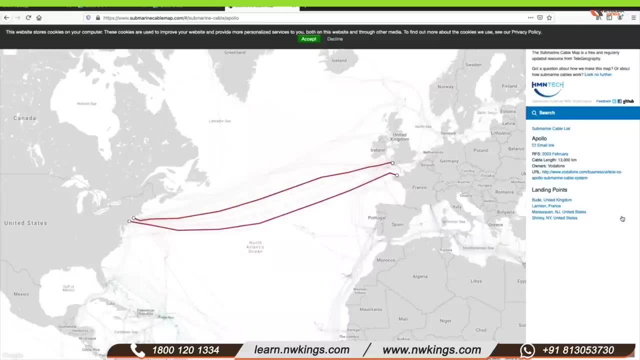 usa and all. so you can see these are sub c points so you can check any of the cable. this cable is implemented by vodafone and vodafone is, by the way, from uk and but this cable is between uk, france and us. it's very interesting map. you can always 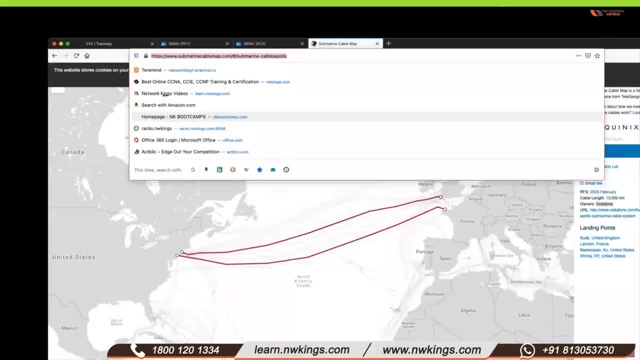 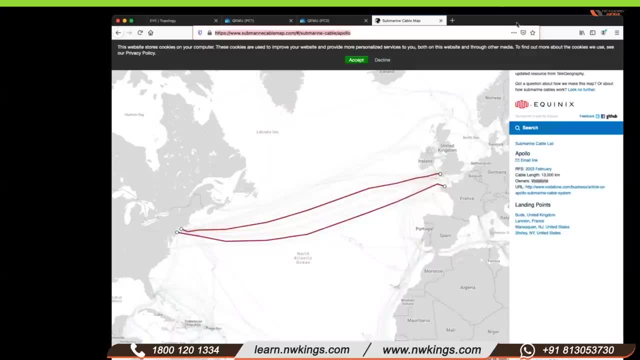 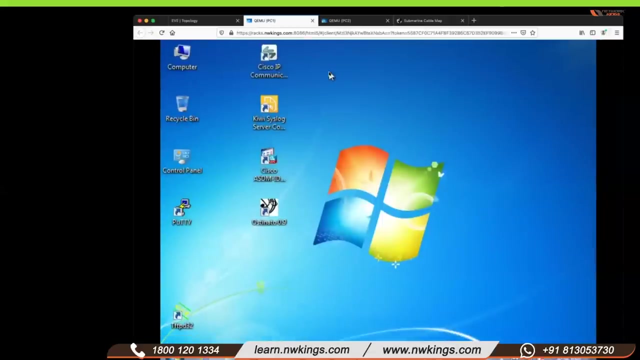 check this, okay. so, guys who came late in this session, and if you want lab access, you can just put down your email id and we are going to create. obviously see, when we asked for the registrations, we got around 340. obviously we have only 100 seats for the lab right and- and this is a testing we are doing for our 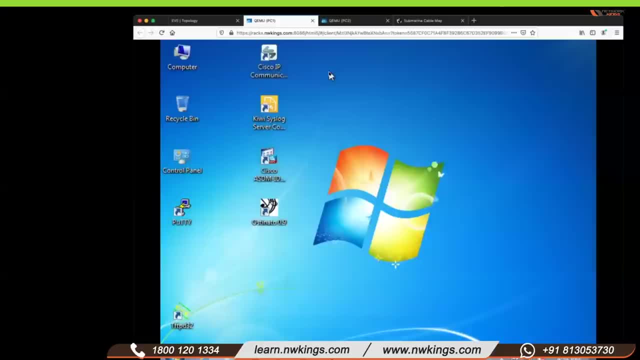 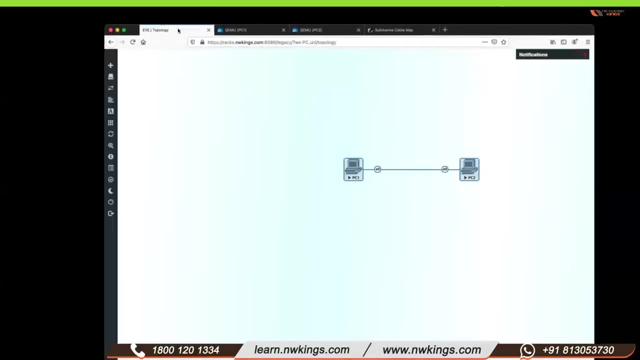 racks. so this is a testing we are doing for our racks. so this is a testing we are doing for our racks. so yeah, so don't type again and again if you have already typed your email address and okay. so i think it's uh, enough for today. we can't learn cci today or ccna in one class, so it takes time. 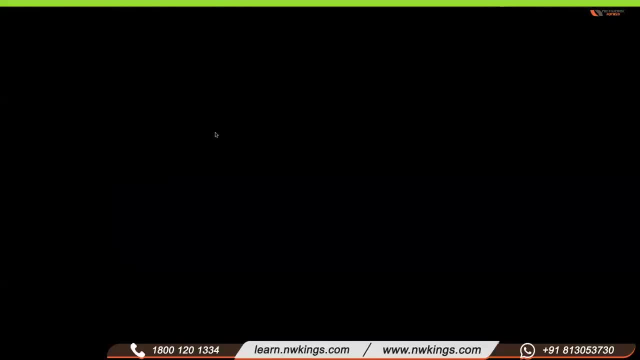 but first we need to create interest in this network field. then only we can go up to the link in thewietwerzland in this network field, then only we can go up to the top level. trust me, if you really love this technology, you can have like thousands, uh, or maybe like, if i talk about usa, you can. 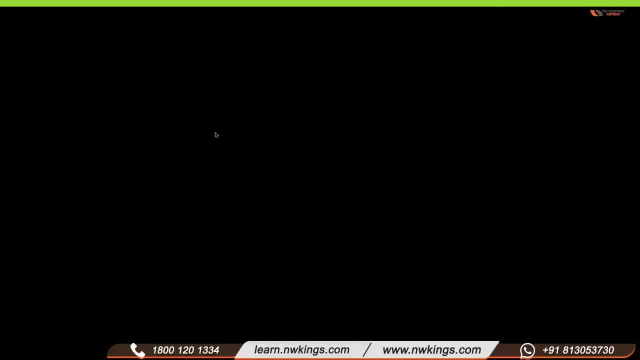 go up to 150 or 2 lakhs dollars up to in in- not as a fresher, but it takes time. in india also, like you can go up to 50 lakhs, 60 lakhs also in this particular field, but it takes time. you can't jump to 50 lakhs package within one year or two years. it takes time, right. 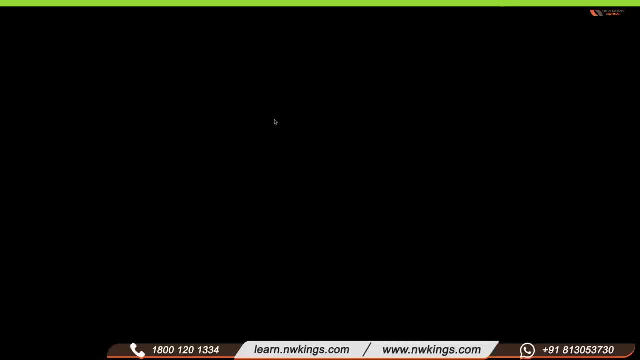 so i'll show you, or i'll give you one career uh strategy also- what exactly you need to learn in 2021. obviously, 2020 is going, so we will discuss about 2021 plan also, right, and i'll give you the step by step things because, uh, like, i have a good exposure and if you 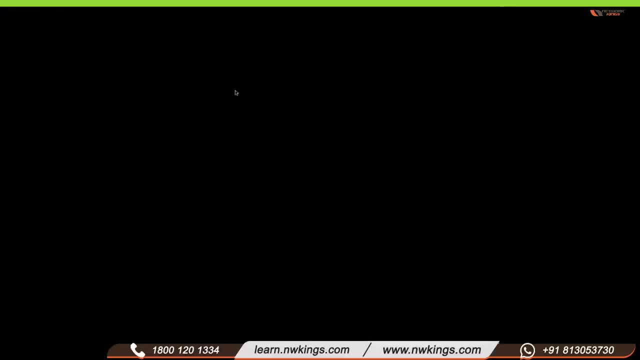 have. obviously everyone needs guidance. without guidance, you can't learn right. yeah, okay, so definitely, from tomorrow we are going to see another things and we are going to configure basic router setup, also in these sessions, and i'm going to complete tomorrow's video and i'll see you in the next one. bye. 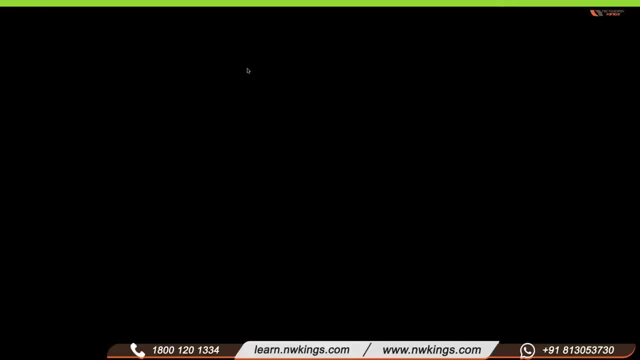 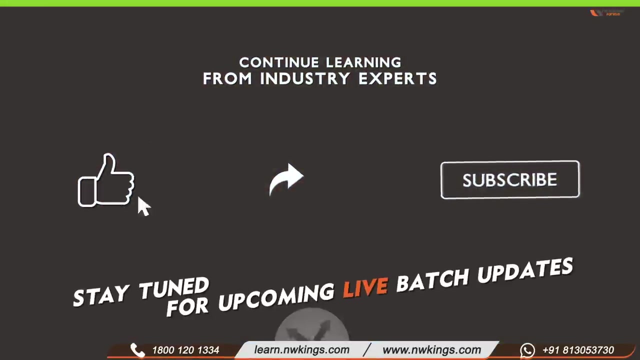 tomorrow subnetting or maybe see whenever i go into my sessions. i i never plan my sessions. i go with the flow. so somebody is asking my qualification, so it's better you check linkedin so you can hi. you are watching the recording from one of our live session. hit like share and subscribe. 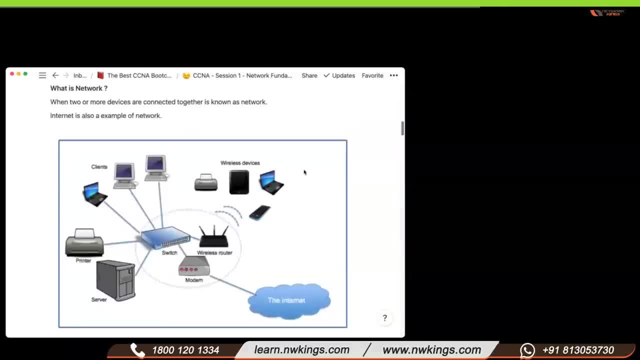 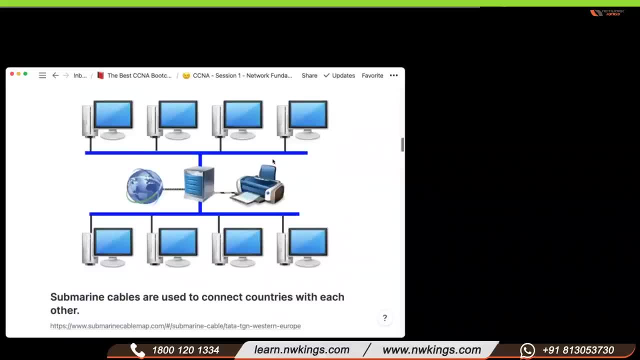 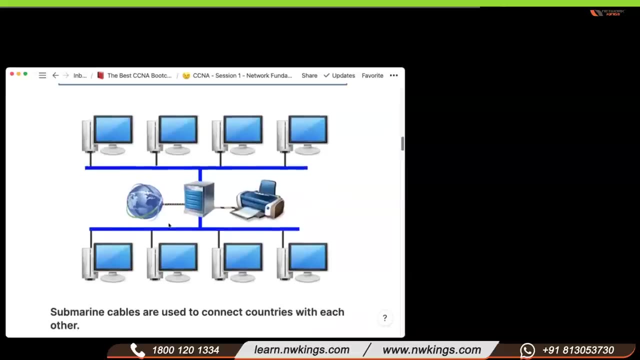 for more future updates. so i have explained you what is a network? when two or more devices are connected together, is a network right and like. you can connect to your computer printers or laptops in a network and that is also in it. that is also known as network, and one when 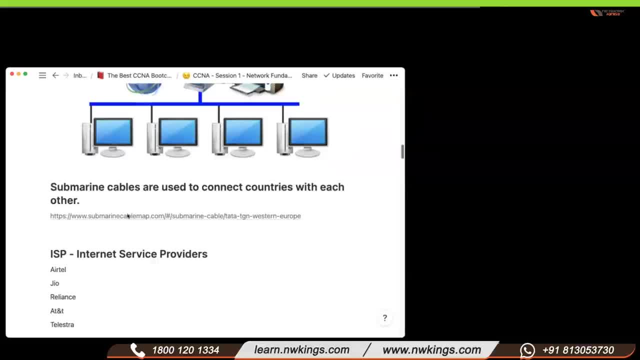 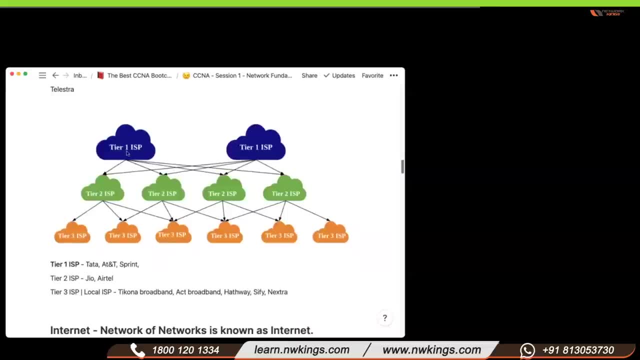 all, uh, all of the service providers are connected together with submarine cable and all. so that is also a network. so i have also explained you that there are tier one isps in the world which are giving connections to the tier two isps and further tier three isps are taking connections. 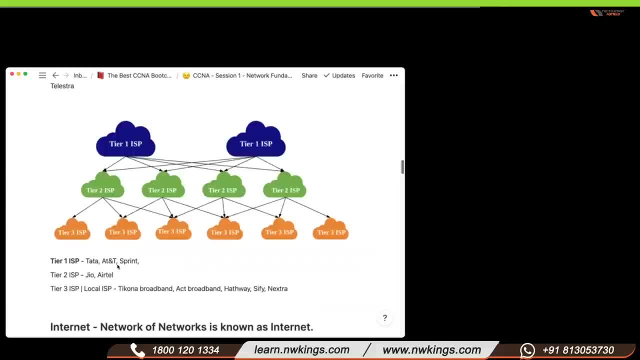 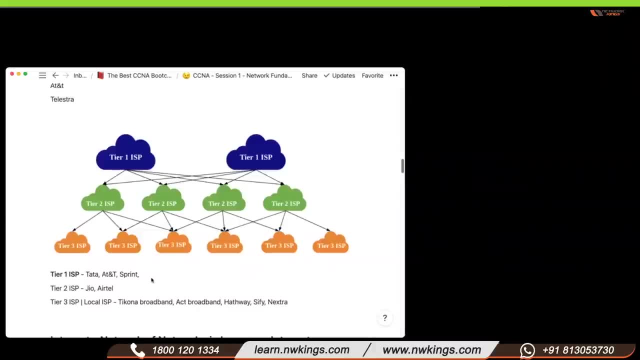 from tier two isp, right. so tata, at&t sprint. the bigger isps are known as tier one isp, those who actually invest in the submarine cable, right. and tier two isps are like, uh, the normal ones. like in india we have geo atl and all these are tier two isp. so i'm audible, right guys? 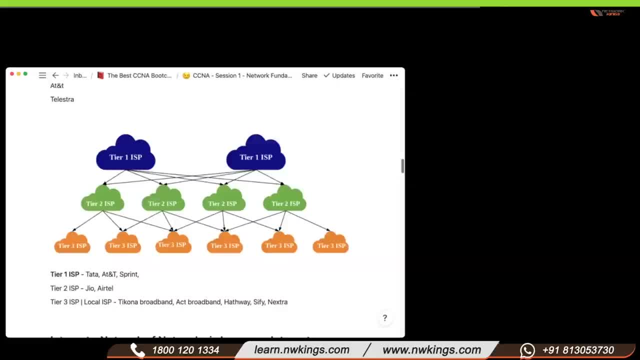 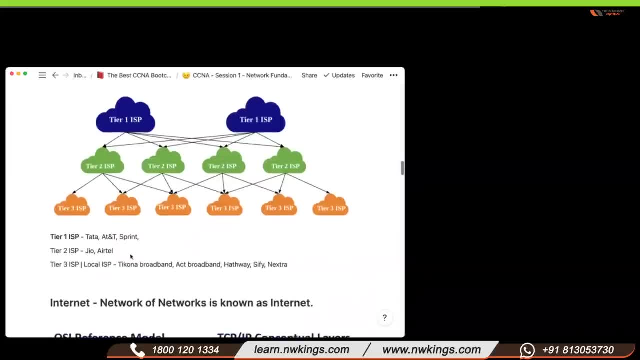 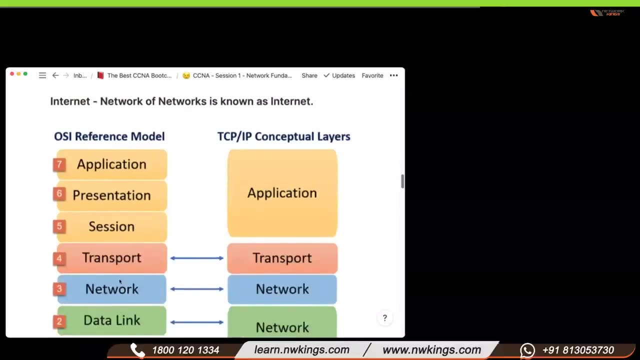 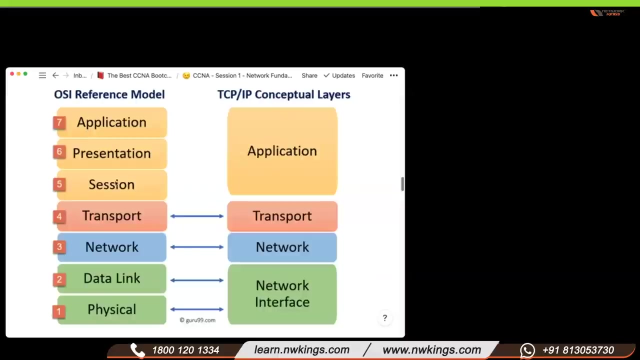 no, this is not a youtube live, this is zoom live only. okay, yeah, so we are going to discuss today that osi model and tcp ip. so, uh, first of all, we need to remember these layers. so, starting from top, that is application presentation session- transport, network, data and physical right, and we are not actually using osi model in real networks. 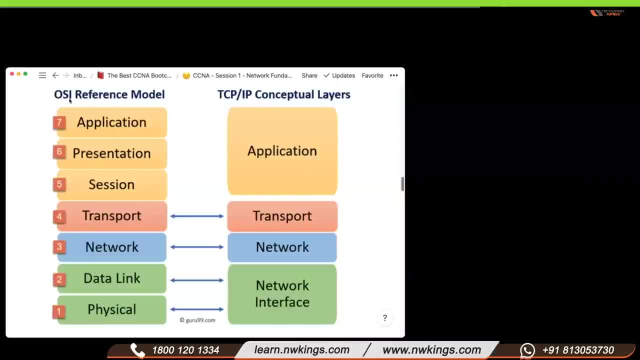 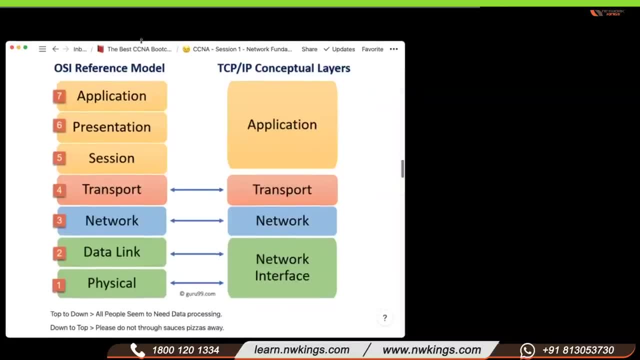 because osi is a reference to the osi model, so we are not actually using osi model in real networks. this is the reason osi's model is known as reference model, just to understand about networks and how actually packets travel from one source to destination. we actually learn osi model even in 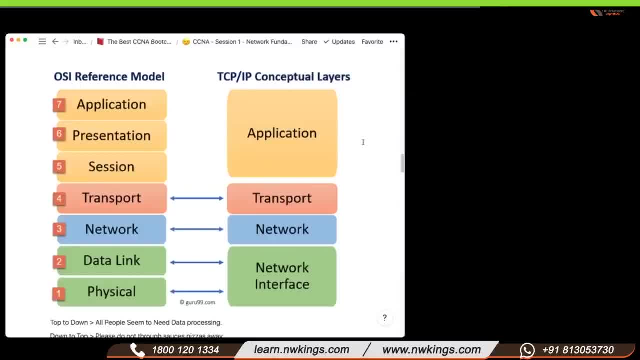 the cisco books or even any vendor books. you will understand osi model first and in real world we are actually using tcpip. so the combination of application presentation session layer is application in this tcp ip and in transport we say transport, uh, the same in tcp ip also. here we have network. here 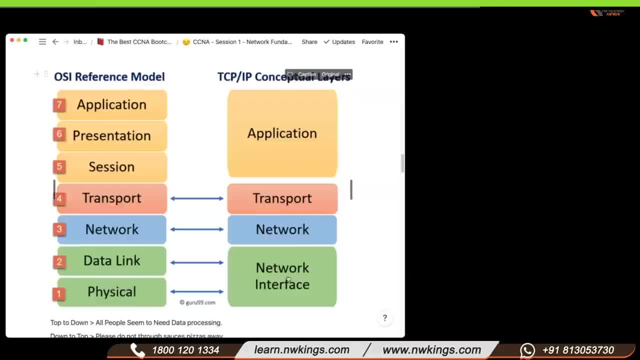 also we have network and the combo of data link and physical. we can say that network interface. but now the tcp ip is also updated. it means so. it means data link layer is known as data link layer and physical is known as physical. so earlier tcp had four layers but now we have tcp ip updated version. 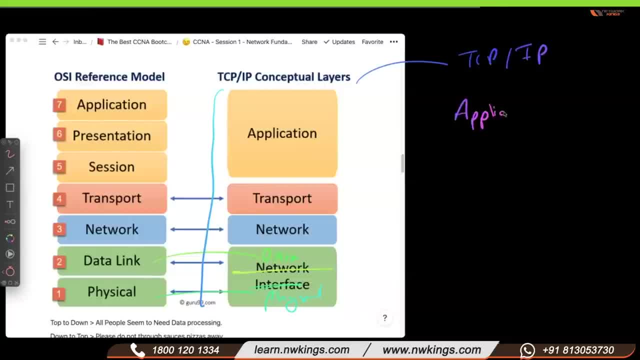 in which we have five layers. first is application- okay, so transport, that is transport. we have network, we have data link layer and last we have physical layer. so in now, that is in tcp ip, we can say that we have around five layers: application, which is actually the combo of these three layers. application presentation session. 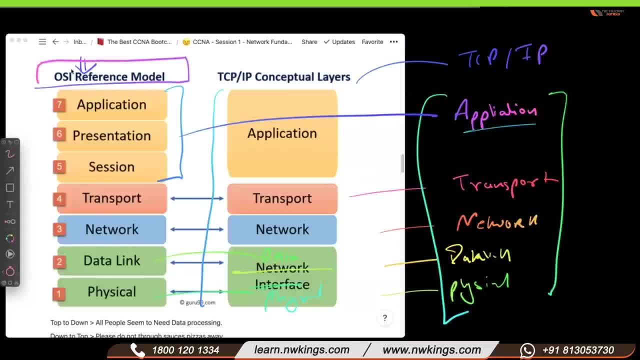 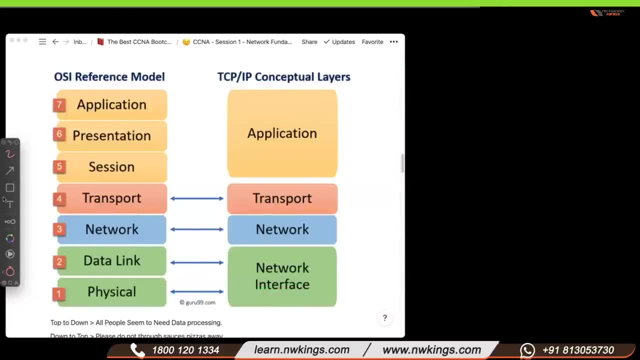 uh. when we want to learn it networks, then we always learn with the oversea model and if you understand osi model, then tcp i? p will be very easy to understand. okay, so we'll be starting with the osi model with uh and check tcp ip also. okay so, but yes, we need to understand first this osi model. 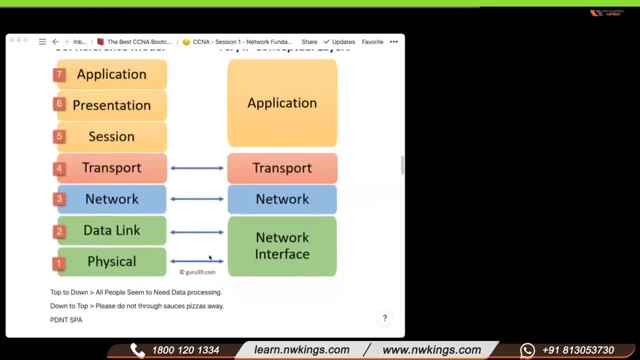 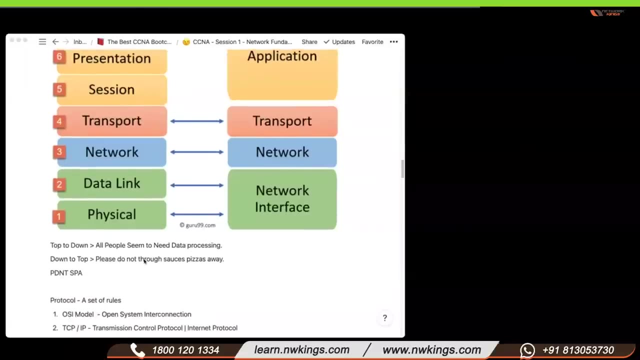 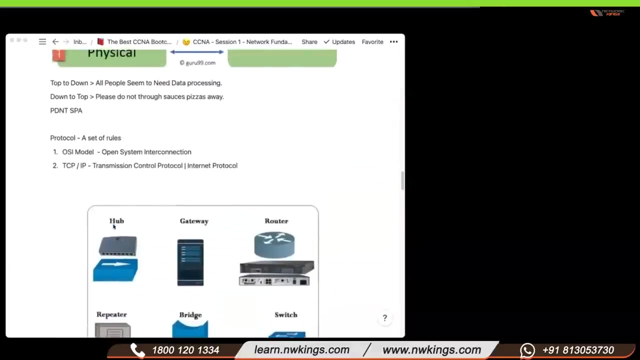 so there is a allies to learn this, like all people seem to need data processing, like all people seem to need data processing. or you can say that please do not throw sauces, pizzas or hey. so it's just allies so that you can understand or learn the layers in order. okay, so what? so? every 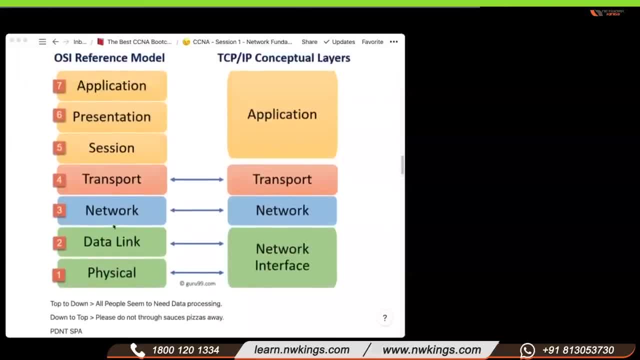 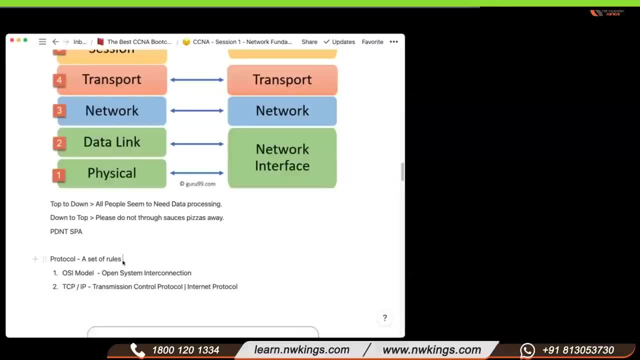 time when we learn about it networks, there is a term called protocol. so what is this protocol means? so protocol means a simple set of rules, right? a protocol is known as set of rules, like: suppose you are driving a car, you need to follow some rules, right? so the government. 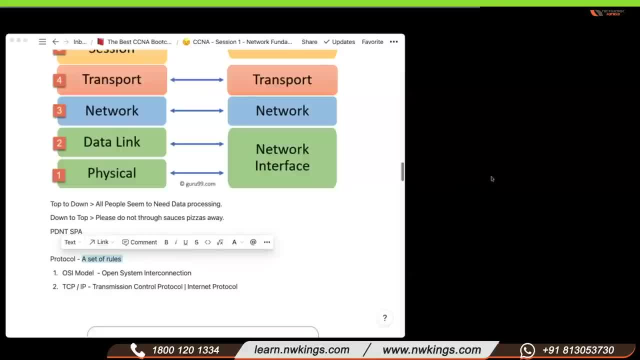 of that particular country has already made some rules that you need to drive, or at the right side or the left side, right. so there are rules, right. so the rules we have over the internet also. these rules are actually known as protocols, like when we say transport, tcp, ip or these protocols. so 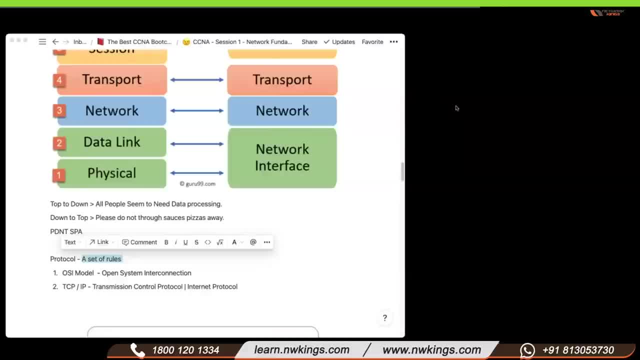 these are actually rules. if anybody wants to go over the internet, they need to follow the rules, like all windows machines, all macbook, all routers- which is all- are following the same rules. that is tcp, ip. okay, got it. chintan, stop asking me lab questions. i am ask me when we will complete this session. okay, so don't distract me here. yeah. 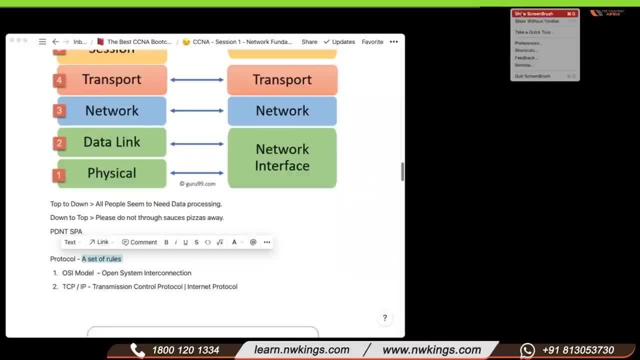 so what i was saying? so like to reach internet or to follow, so osi model tcp, ipr rules, so that we can follow the internet rules. so these are known as protocol. so, like all these four, five routers are sharing the information with each other, so they are following some rules, right? so these rules are actually known as protocols. 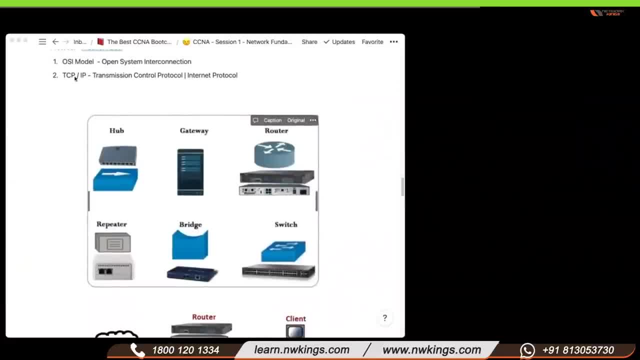 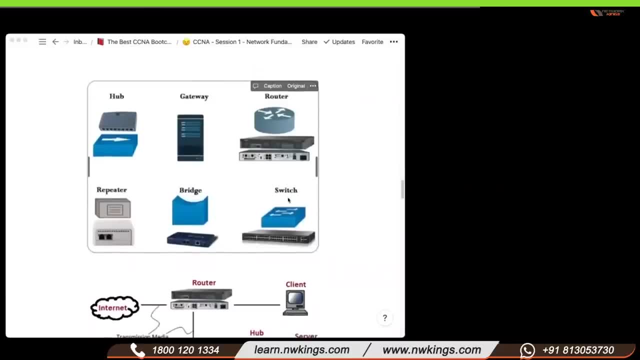 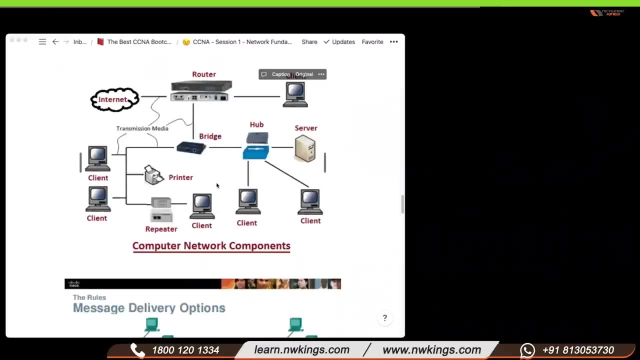 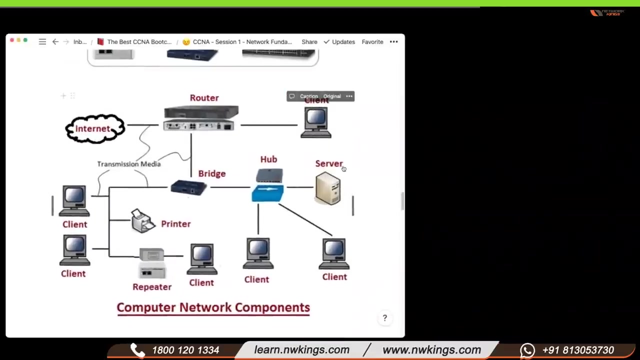 so we have, like, which rule we are following? everyone is following nowadays tcp, ip, so people are following these ms using code. so this is this Van corrupted, so this is actually the root of the operating system, right? so this is which are fine. so, like over here, and we have placed the device that is known as a router. so why we are, why we have router. 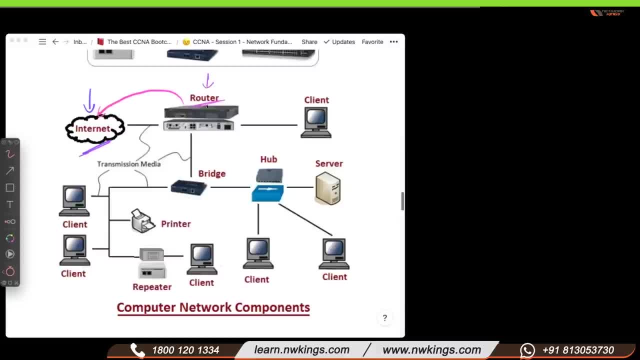 here so that we can connect to the different world means to connect with different network. we need a router. so these client means your computers, laptops or any device, and these servers are actually connected with hub. so hub is a obsolete device. nowadays nobody uses hub, so we have, instead of, 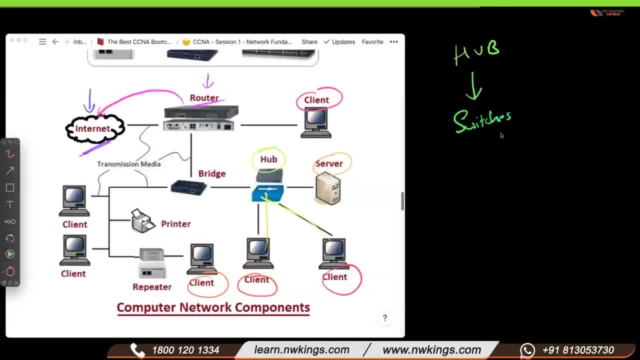 hub we use is switches. so switches are better than hub because, like it's it, it works only on signals, but switches actually understand about the mac address and other functionalities like switches are better than hub. you can say that. okay. so this is a simple representation. that router is actually connecting to the internet and all your hub or these. 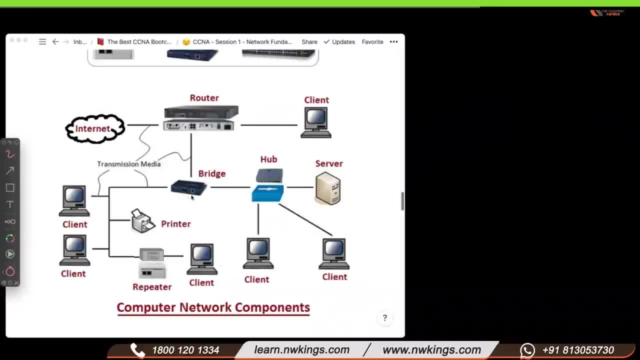 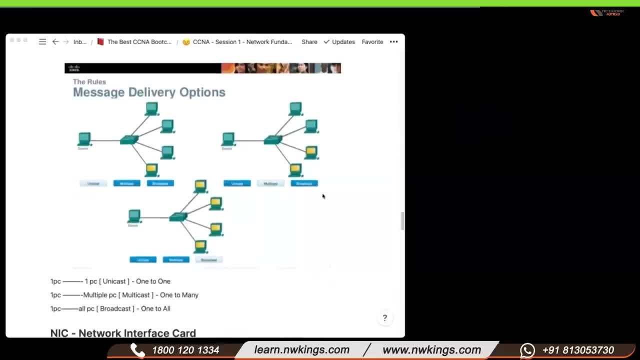 type of devices are actually connecting your machines together. so that is a little bit old one. yeah, so there are. so what is the difference between hub and switch? yeah, so i was explaining that. so when, like few computers are sending data, okay, so hub is just like your power extension. 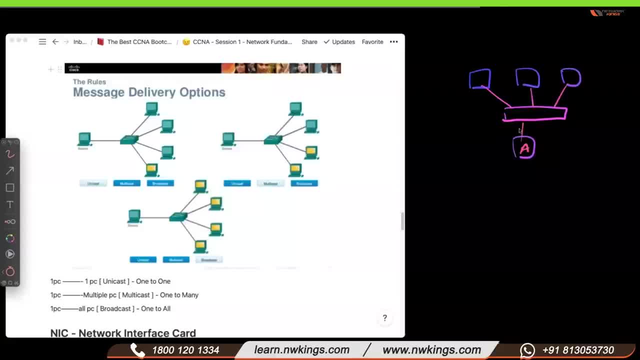 device. so if a computer is sending data to b, it will also go to c, for you see, here it is regardless of whether it is c or d also. so hub always do broadcast, because it works on signal. so if you sent any signal it will go to everyone. so that is hub. 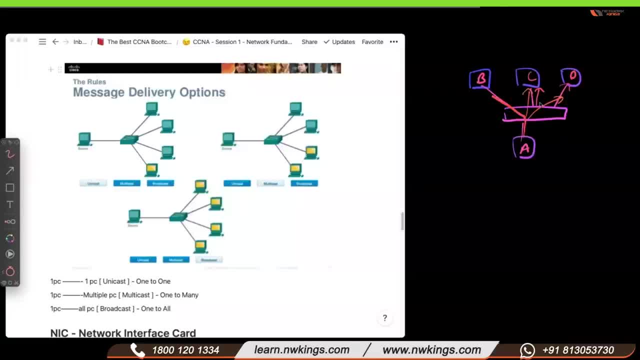 hub, it actually does not learn mac address. okay, so in when we use switch so switch actually makes one table inside the switch so that is known as mac address table. so whenever you send data from a to b or c to d, so when we are sending data a to b, so a computer mac address will be stored, b computer mac address will be stored. 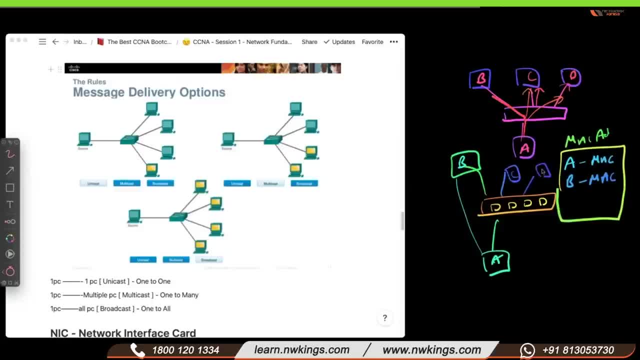 so next time when data is sending or when data is going between a and b, so because switch knows the mac address, switch knows the address of that b device, so it will directly go to b device, so it will not send to c and d. okay, so this is the difference between hub always do broadcast. so 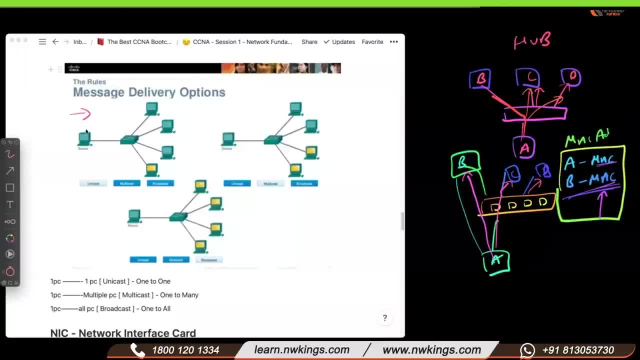 what is broadcast. see this image. so when my computer- one computer- is sending data to one device, that is unicast- okay. when one device- either it is router or any device- sending to multiple devices, that is known as multicast- okay. and when my device is sending data to everyone, 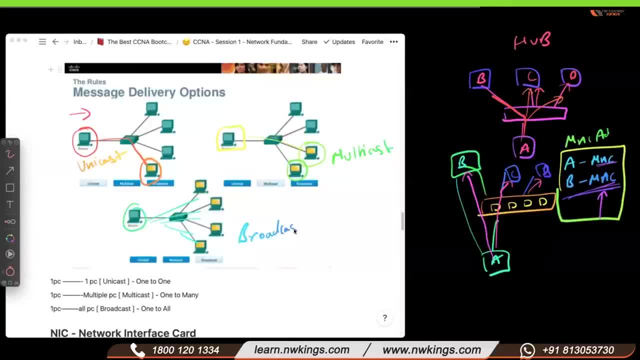 that is known as broadcast. so in simple terminology, hub always does not send data to any device. that is unicast. so when my device is sending data to multiple devices, that is unicast. so when my device is sending data to any device that is unicast always do broadcast, because hub never store any mac address. it works on signals. so this is known. 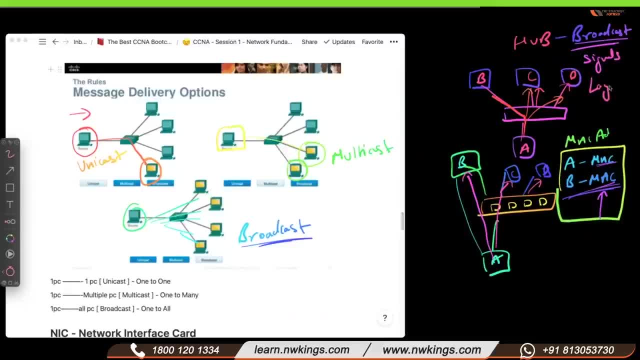 as uh like we can also say that it it's a layer one device. so what is layer one? so in osi model, layer one is known as physical layer, which works on signals, connectors and all yes. so it's like a dummy device. it does not store anything, right when we talk about switches. so switch actually store. 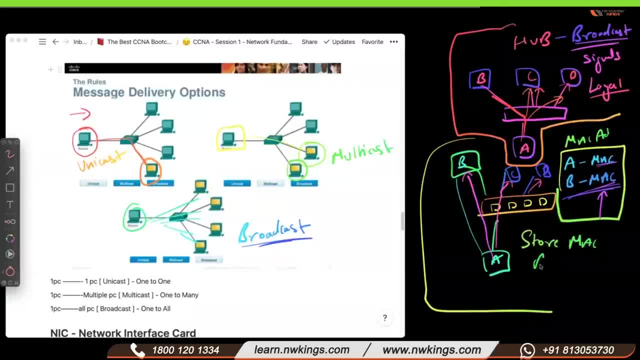 the mac address. so when we talk about switches, so switch actually store the mac address. so when we talk about switches, so switch actually store the mac address. so when we talk about switches, so when we talk about switches, so switch actually store the mac address. so store mac address. so this. 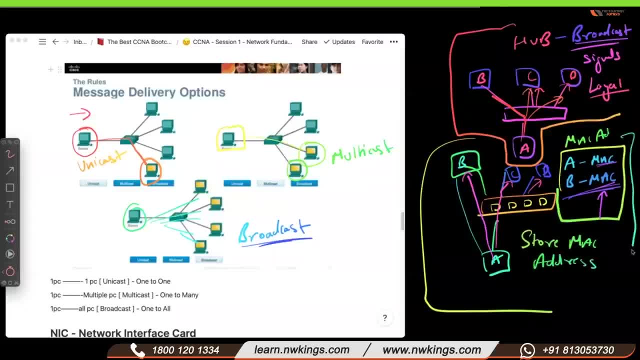 the mac address. so this the mac address. so this is the reason it is known as a it's intelligent is the reason it is known as a it's intelligent, is the reason it is known as a it's intelligent device, whenever device, whenever device, whenever data is going between a to b or c to d. 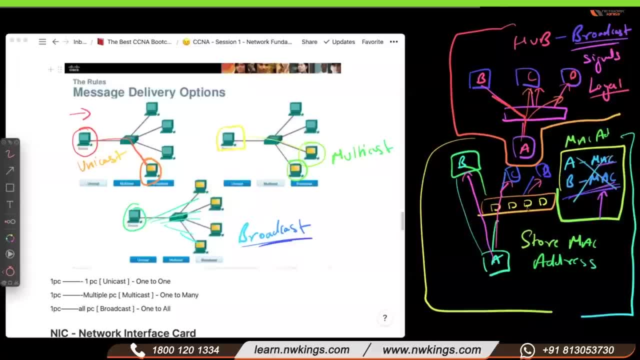 data is going between a to b or c to d. data is going between a to b or c to d, so it checks the mac address. if we don't, so it checks the mac address. if we don't, so it checks the mac address. if we don't have any entry, then it is going to send. 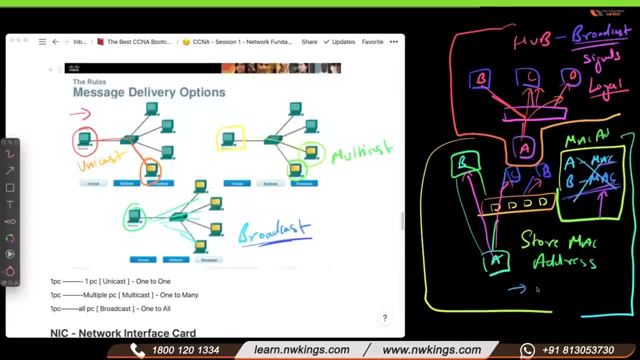 have any entry, then it is going to send. have any entry, then it is going to send broadcast, but one time it will. you can broadcast, but one time it will. you can broadcast, but one time it will. you can say that initially it sends broadcast. say that initially it sends broadcast. 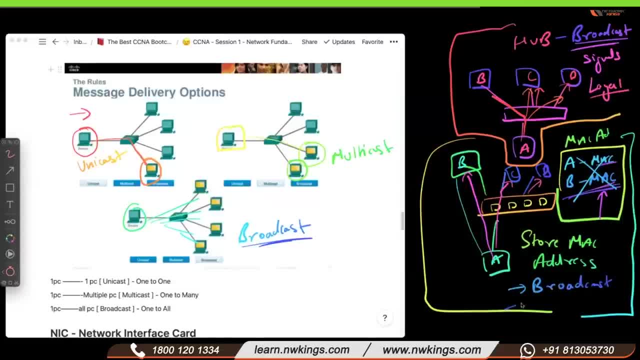 say that initially it sends broadcast because initially we don't have mac, because initially we don't have mac, because initially we don't have mac address table, but when data is address table, but when data is address table, but when data is like going between the devices it makes. 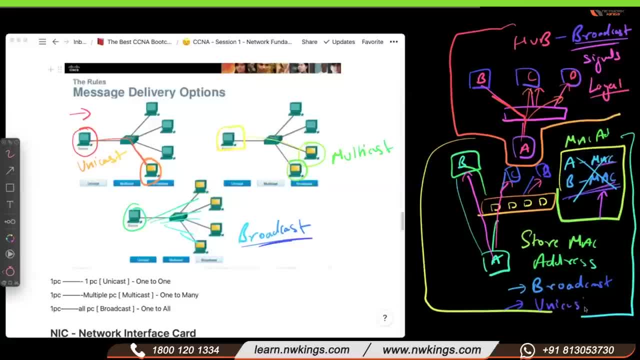 like going between the devices it makes, like going between the devices: it makes a mac address table and after that it a mac address table, and after that it a mac address table, and after that it sends unique cast, sends unique cast, sends unique cast. so so so if i'm sending data a to b first time, i'm 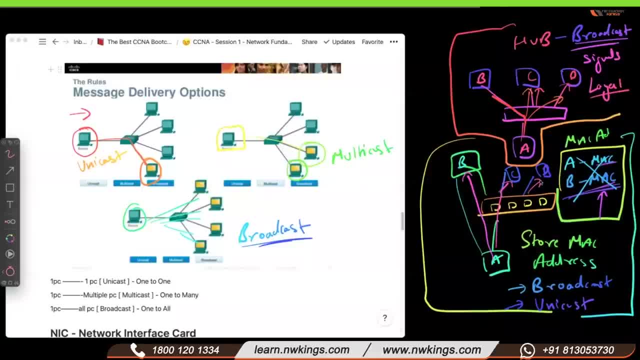 if i'm sending data a to b first time, i'm if i'm sending data a to b first time, i'm going to send broadcast. the packet will going to send broadcast. the packet will going to send broadcast. the packet will go to c and d also, but next time. 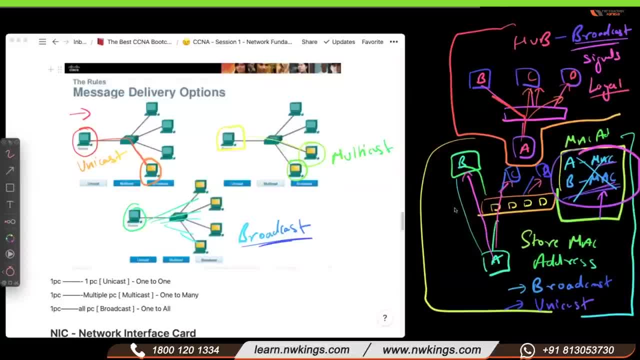 go to c and d also, but next time go to c and d also, but next time when we have mac address table, when we have mac address table, when we have mac address table, when next time i'm going to send data, when next time i'm going to send data. 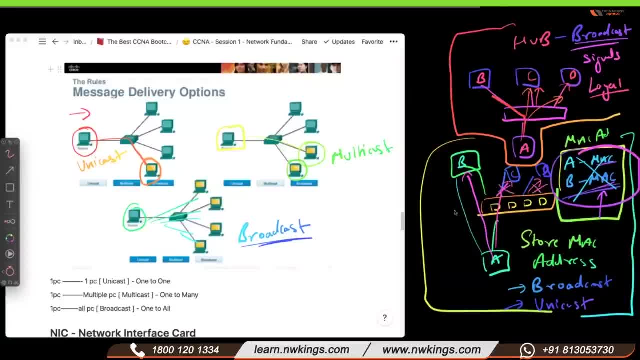 when next time i'm going to send data between a and b, i'm not going to send between a and b. i'm not going to send between a and b. i'm not going to send data to c and d, because that will be data to c and d, because that will be. 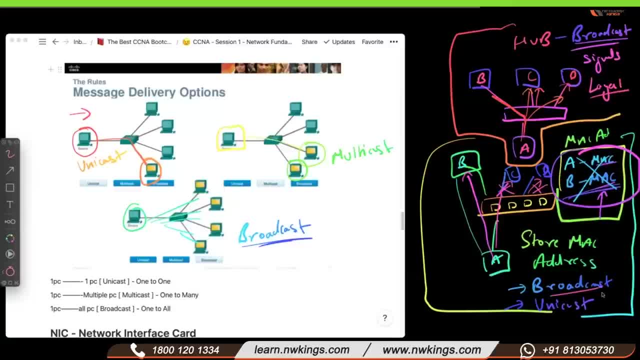 data to c and d, because that will be unicast, so initially unicast, so initially unicast, so initially, till the time we don't have mac address, till the time we don't have mac address, till the time we don't have mac address, we will send broadcast and once we get, 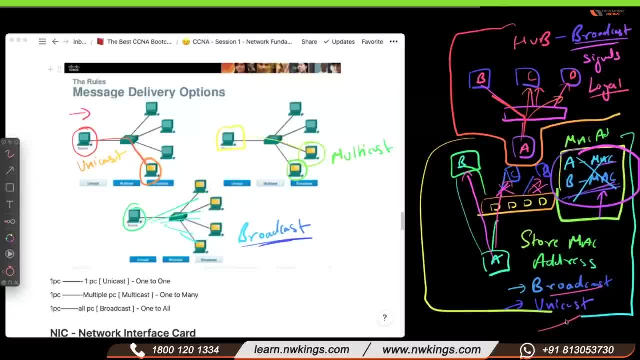 we will send broadcast. and once we get, we will send broadcast. and once we get the mac address, we send unicast the mac address. we send unicast the mac address. we send unicast. okay. so this is the difference between. okay, so this is the difference between. 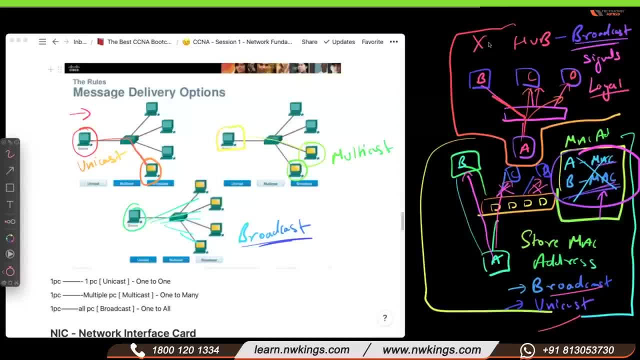 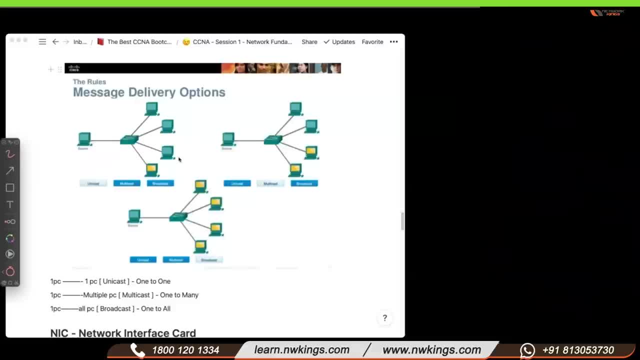 okay, so this is the difference between hub and switch. so we don't use hub, hub and switch. so we don't use hub, hub and switch, so we don't use hub nowadays. by the way, okay, yeah, so i have explained to this network. yeah, so i have explained to this network. 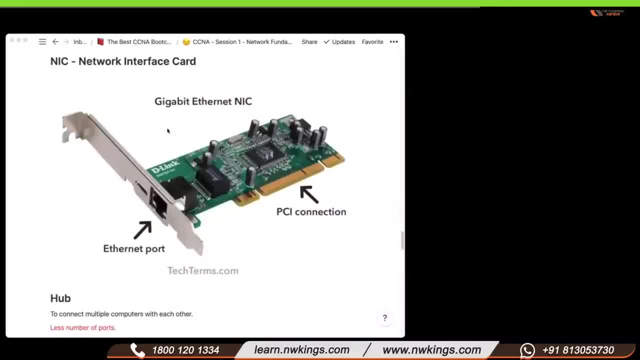 yeah, so i have explained to this network interface card, it interface card, it interface card, it. it's a chip basically and we put this: it's a chip basically and we put this: it's a chip basically and we put this nic card in the nic card in the. 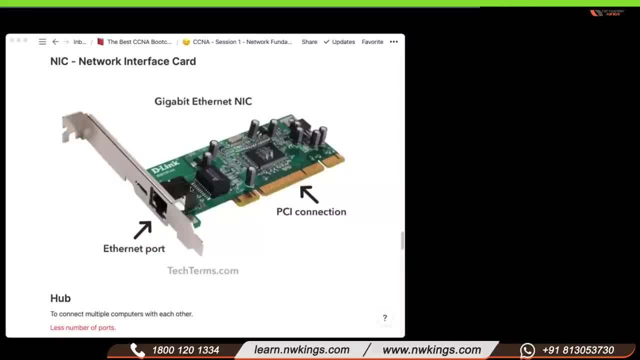 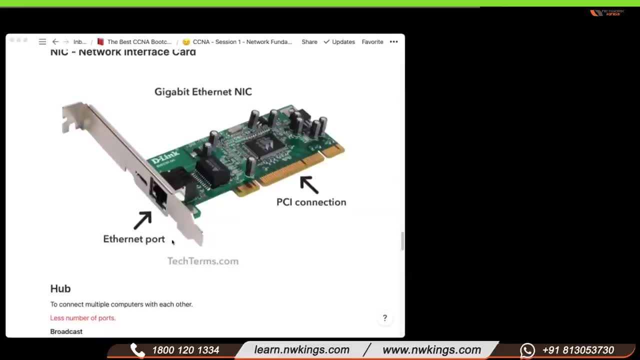 nic card in the like motherboard pci slot, like motherboard pci slot, like motherboard pci slot. but nowadays all machines like computers but nowadays all machines like computers, but nowadays all machines like computers: laptops, laptops, laptops, they have integrated ethernet chips, or they have integrated ethernet chips, or they have integrated ethernet chips or nic card inside the machines. 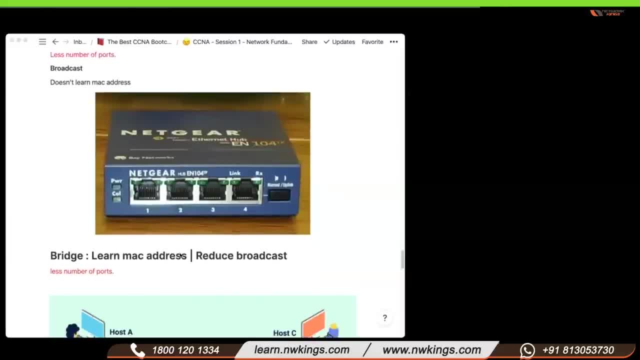 nic card inside the machines. nic card inside the machines. so this is the image of hub, but nowadays, so this is the image of hub, but nowadays, so this is the image of hub, but nowadays we don't use this, we don't use this, we don't use this devices and hub actually have like uh in. 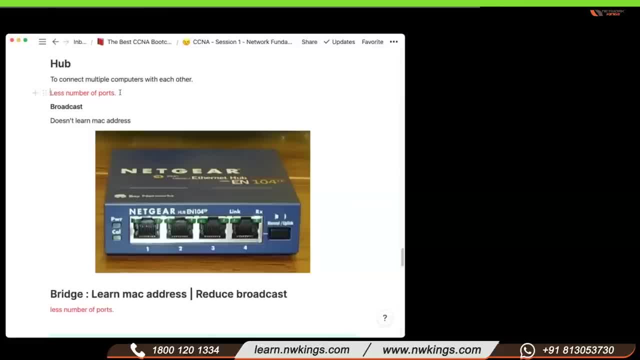 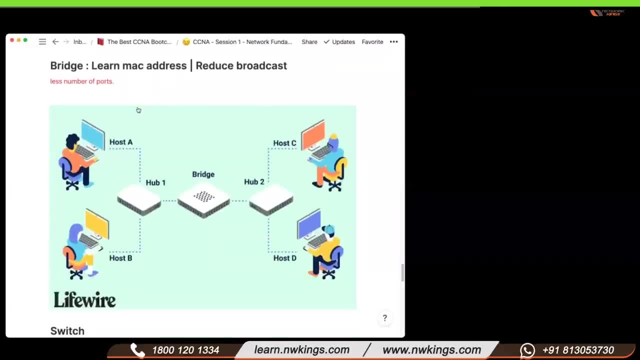 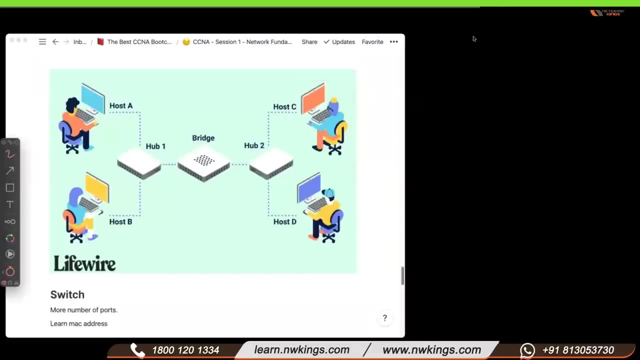 devices and hub actually have like uh in devices and hub actually have like uh in hub, hub, hub. we used to have this less number of. we used to have this less number of. we used to have this less number of ports, ports, ports, okay, and and and reduce the broadcast because bridge. 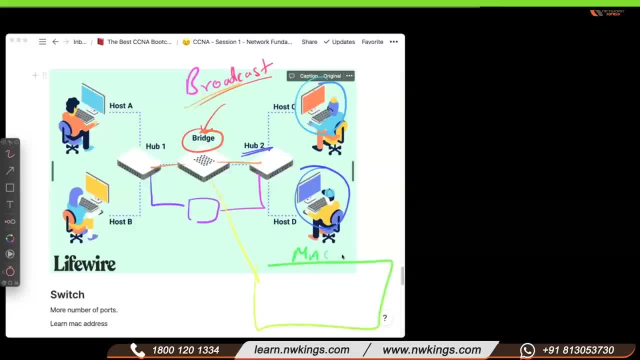 reduce the broadcast because bridge. reduce the broadcast because bridge was the device which actually store the, was the device which actually store the, was the device which actually store the mac address, mac address, mac address. so it actually not eliminate it can. so it actually not eliminate it can. 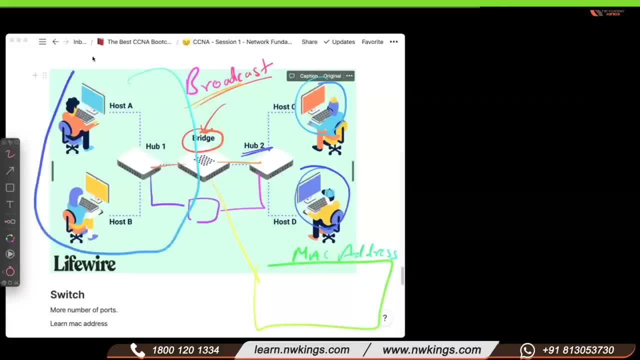 so it actually not eliminate. it can reduce the broadcast, so like whenever. reduce the broadcast so like whenever. reduce the broadcast, so like whenever any packets are going, it will go into. any packets are going, it will go into. any packets are going, it will go into this area only. 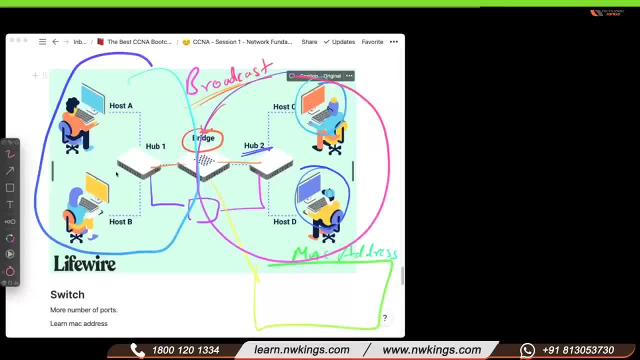 this area only, this area only and this area only like this- okay but. and this area only like this- okay but. and this area only like this: okay, but bridge also is an obsolete device. bridge also is an obsolete device. bridge also is an obsolete device because the combination of hub plus. 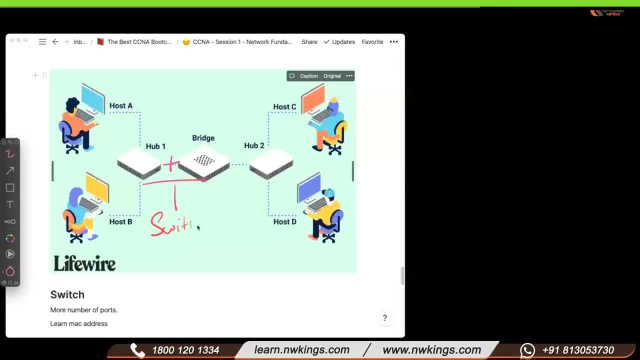 because the combination of hub plus, because the combination of hub plus bridge is now known as switch. okay, so hub was to connect multiple. okay, so hub was to connect multiple. okay, so hub was to connect multiple devices and bridge is to devices and bridge is to devices and bridge is to actually. 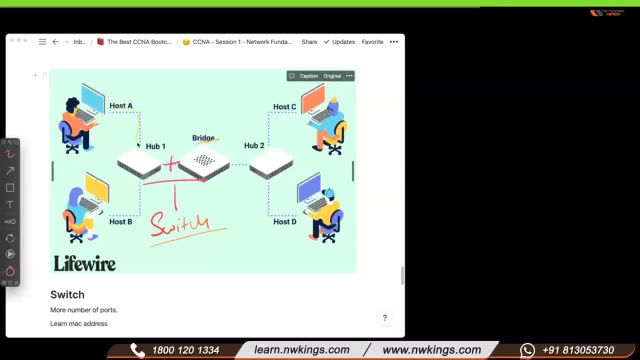 actually actually reduce the broadcast, reduce the broadcast. reduce the broadcast because whenever any host a is sending, because whenever any host a is sending, because whenever any host a is sending data, so bridge will store the mac address data, so bridge will store the mac address data. so bridge will store the mac address of host a and sending data to host c. 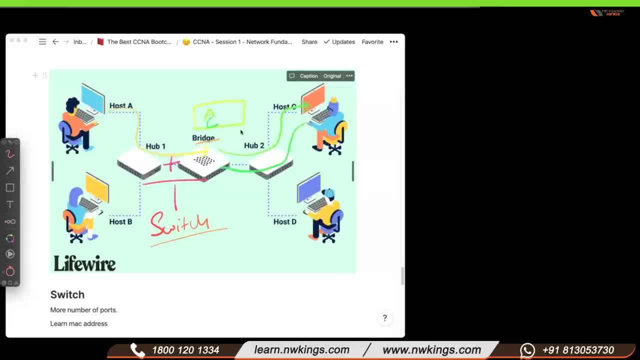 of host a and sending data to host c of host a and sending data to host c. host c will reply and we will store the host c will reply and we will store the host c will reply and we will store the mac address of host a and c also. so next, 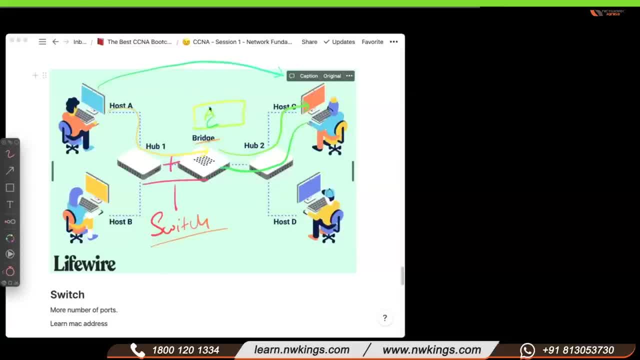 mac address of host a and c also. so next mac address of host a and c also. so next time, when we are sending data between time, when we are sending data between time, when we are sending data between host a and c, host a and c, host a and c bridge will show us the mac address table. 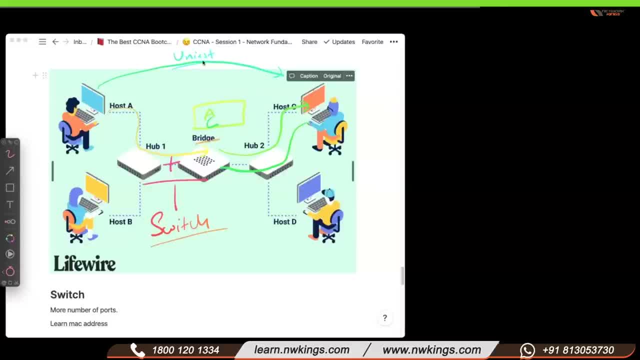 bridge will show us the mac address table. bridge will show us the mac address table and we are going to send the unicast. and we are going to send the unicast and we are going to send the unicast, kind of packet, kind of packet, kind of packet, so that we can save the bandwidth. 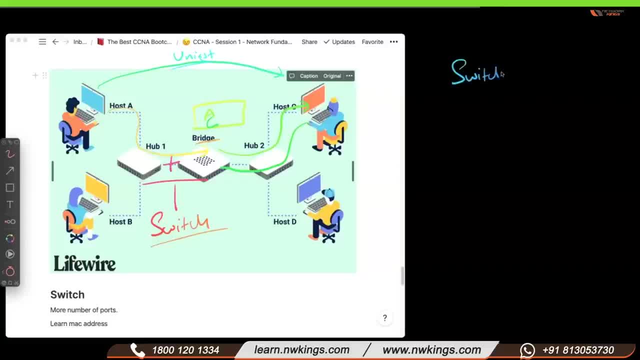 so that we can save the bandwidth, so that we can save the bandwidth, yeah so, yeah, so, yeah so, uh, switch uh, switch, uh switch is like, is like, is like successor of this device that is known successor of this device that is known successor of this device that is known as bridge. 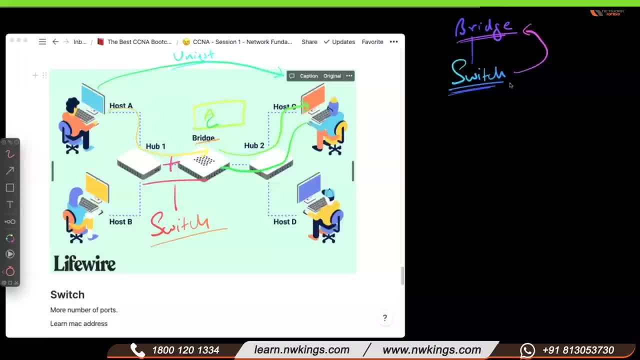 as bridge, as bridge. so switches was bridge, you can say that. so now bridge is. you can say that. so now bridge is. you can say that. so now bridge is known as switch with multi, known as switch with multi, known as switch with multi. many ports in bridge we used to have. 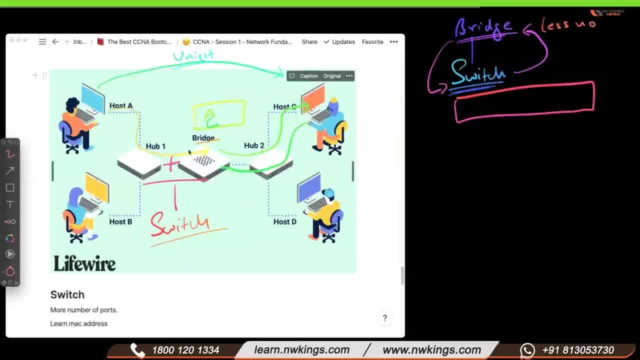 many ports in bridge. we used to have many ports in bridge. we used to have less number of ports because the device less number of ports because the device less number of ports because the device made to connect the hubs, made to connect the hubs, made to connect the hubs right so you can see connected hub here. 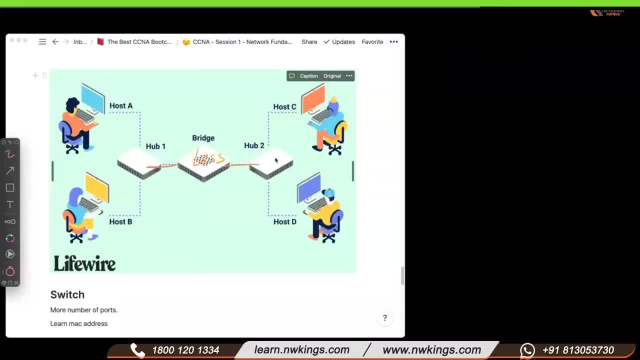 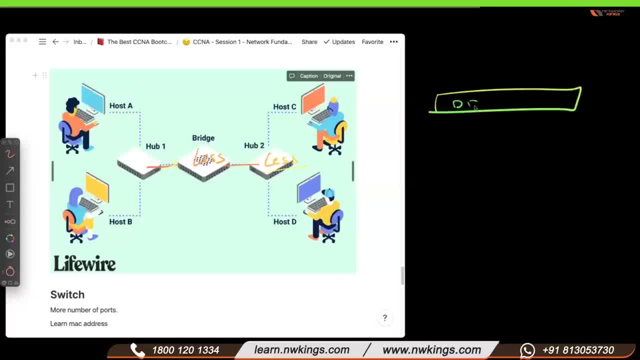 even hub was having less ports. but the combination- you can say that hub has a combination. you can say that hub has a combination. you can say that hub has a lot of, lot, of lot of like four port v in switches we have. like four port v in switches we have. 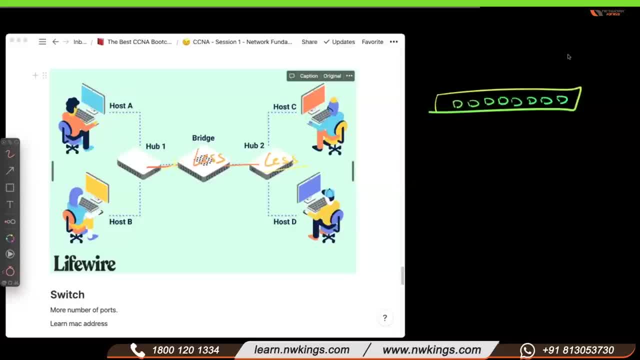 like four port v in switches. we have eight port 16 port 32 or 24, eight port 16, port 32 or 24, eight port 16, port 32 or 24, not 32, 24, 48 like that, not 32, 24, 48 like that. 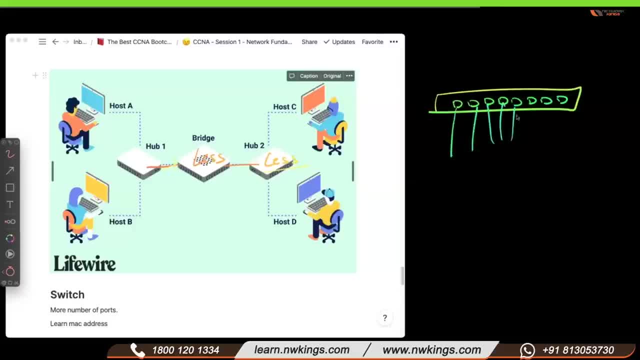 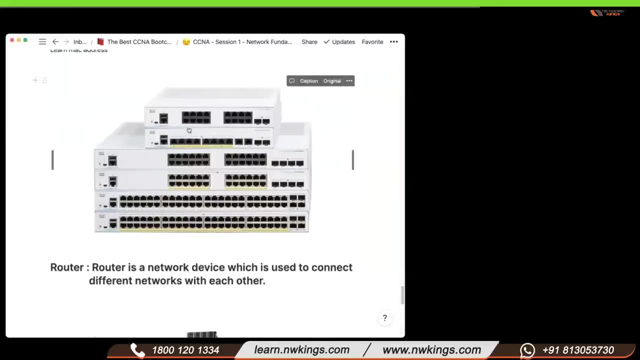 not 32, 24, 48, like that. okay, so now this device understand mac. okay, so now this device understand mac. okay, so now this device understand mac address on every port. okay, cool, so these are the switches actually. so these are the switches actually. so these are the switches actually. nowadays, cisco has, like you can see, 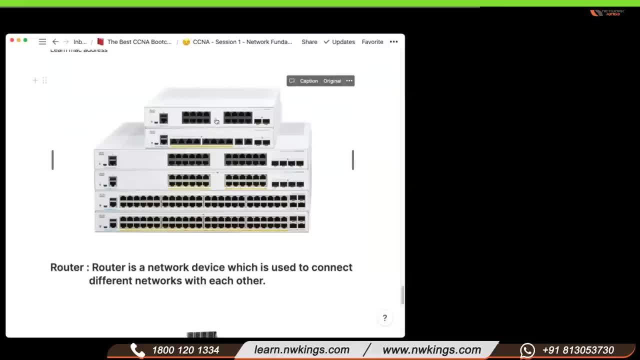 nowadays cisco has, like you can see, nowadays, cisco has, like you can see, this, this, this. so this is a. so this is a. so this is a 16 port switch- the upper one, and a 16 port switch, the upper one, and a 16 port switch, the upper one, and a. the below one is 24 and in the last one, 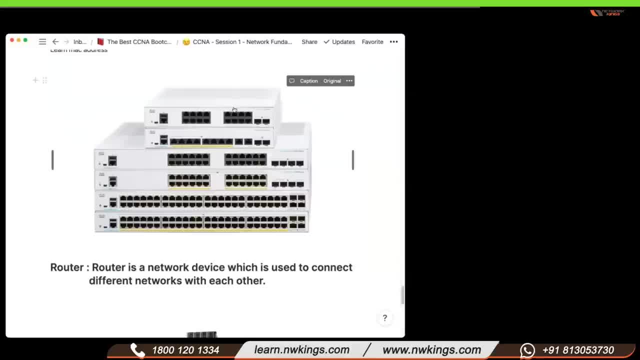 the below one is 24 and in the last one the below one is 24 and in the last one we have, we have: we have 48 port switches, so that actually 48 port switches, so that actually 48 port switches, so that actually switches cost actually varies on the. 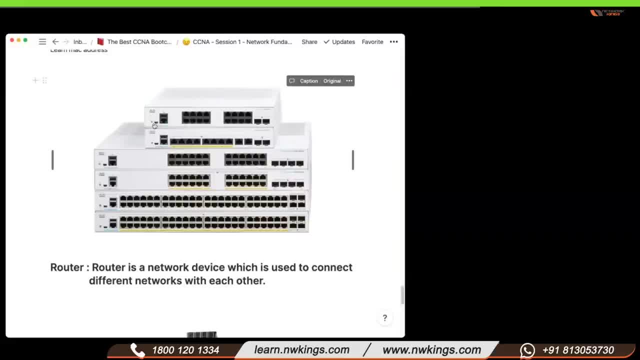 switches cost actually varies on the switches cost actually varies on the density of ports also. density of ports also. density of ports also, like how many ports we have in switches. like how many ports we have in switches. like how many ports we have in switches- maybe 16 ports, which is 100. 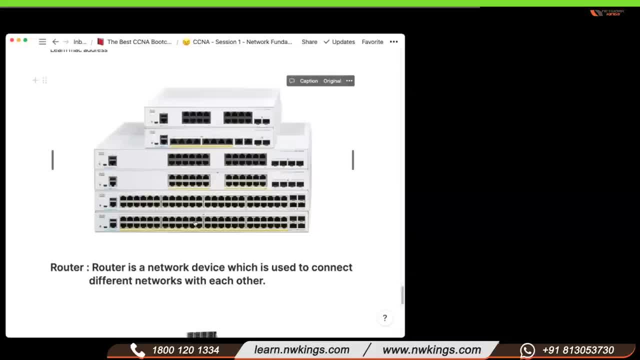 maybe 16 ports, which is 100, maybe 16 ports, which is 100, and 24 is 150, and maybe 48 will cost and 24 is 150, and maybe 48 will cost and 24 is 150 and maybe 48 will cost around 200. it depends on which model you 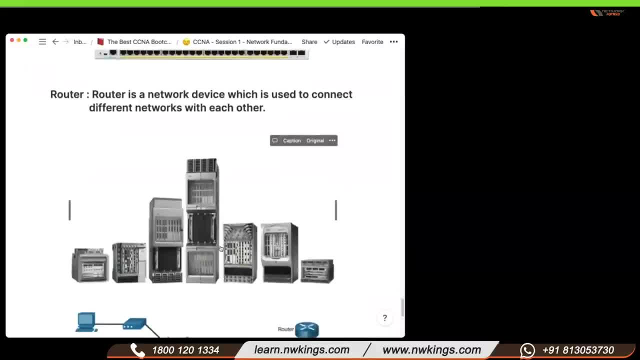 around 200. it depends on which model you around 200. it depends on which model you are buying. are buying, are buying. so now comes the router, so again router. so now comes the router, so again router. so now comes the router, so again. router is a network device which is used to 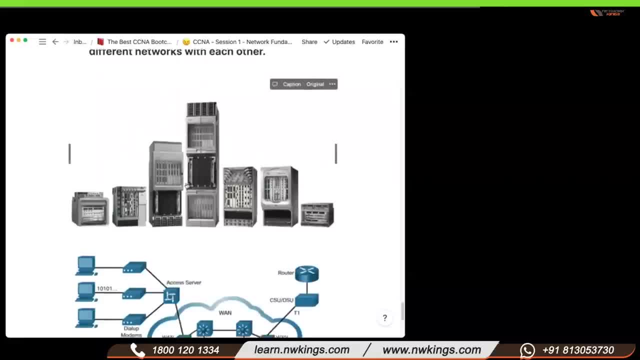 is a network device which is used to, is a network device which is used to create different networks with each, create different networks with each, create different networks with each other. so in other, so in other, so in when we talk about routers, we don't have. when we talk about routers, we don't have. 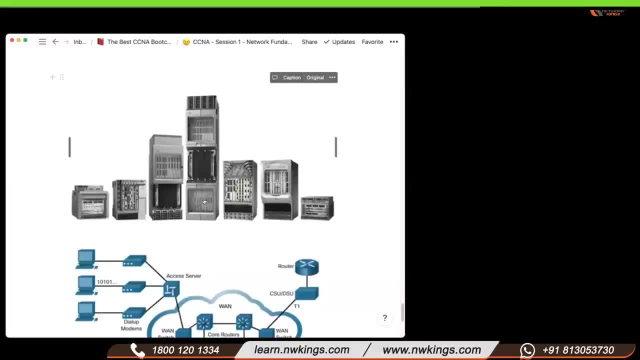 when we talk about routers, we don't have the small routers. so you can see this: the small routers. so you can see this, the small routers. so you can see this big router over here that is used by big router over here, that is used by big router over here that is used by big companies, or you can say that used by. 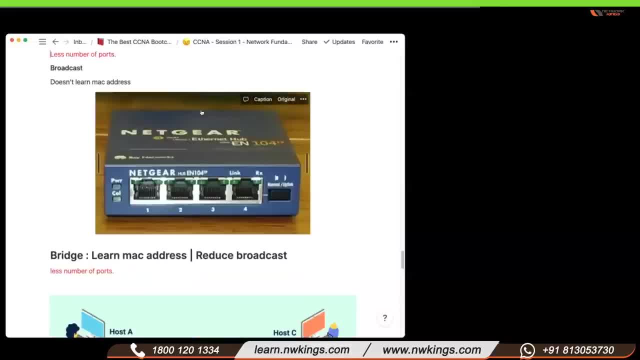 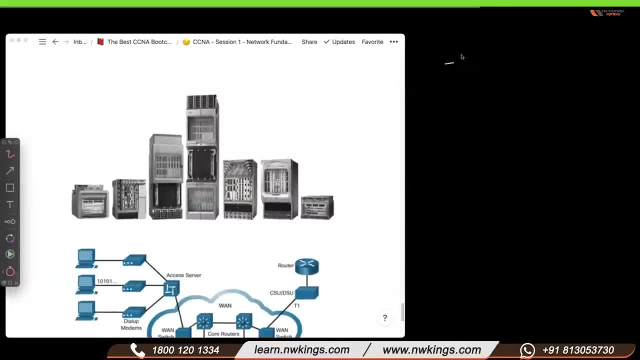 big companies. or you can say that used by big companies, or you can say that used by service providers, service providers, service providers. okay so, yeah, just yeah. so when we talk about the: yeah, just yeah. so when we talk about the: yeah, just yeah. so when we talk about the normal cisco devices we have around, 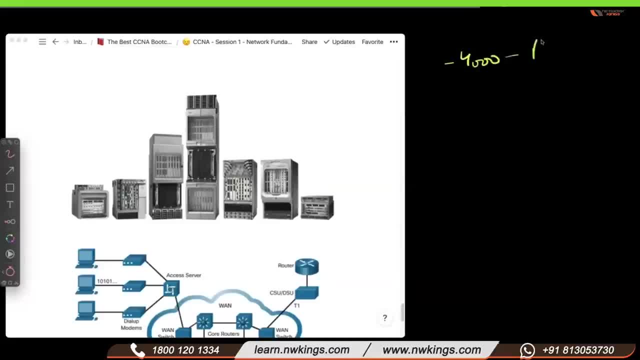 normal cisco devices. we have around normal cisco devices. we have around 4000 series, 4000 series, 4000 series- okay. 4000 series is like branch routers- okay. 4000 series is like branch routers- okay. 4000 series is like branch routers- okay. and these routers are not very. 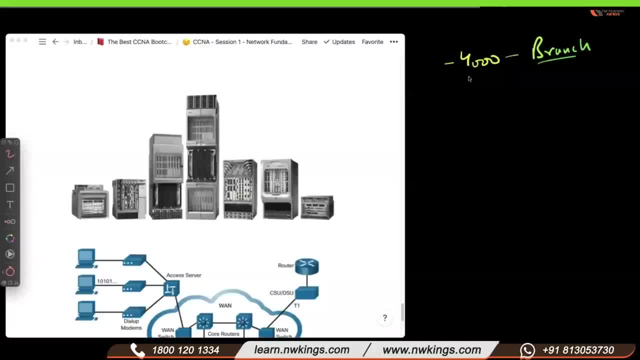 okay and these routers are not very okay and these routers are not very uh uh uh costly, but yes, it's the starting range costly, but yes, it's the starting range costly, but yes, it's the starting range of cisco, of cisco, of cisco in market, the devices we have, of router. 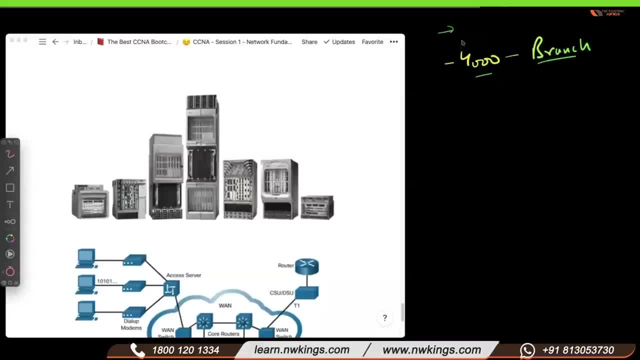 in market the devices we have of router in market, the devices we have of router. so again, this device is very costly in. so again, this device is very costly in. so again, this device is very costly in terms of the local routers, or terms of the local routers, or 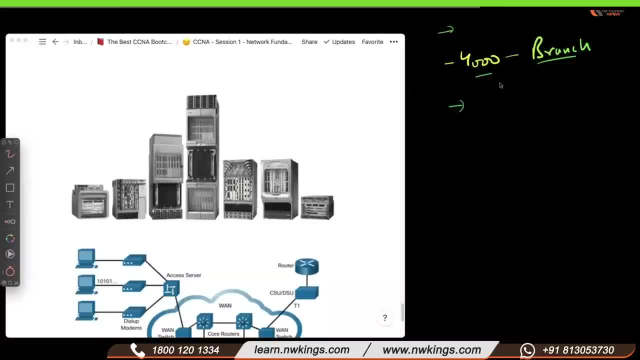 terms of the local routers, or uh any local company routers, right so, uh any local company routers, right so? uh any local company routers, right so these are. these are, these are known as branch routers and these known as branch routers and these known as branch routers, and these routers are like cisco asr routers. 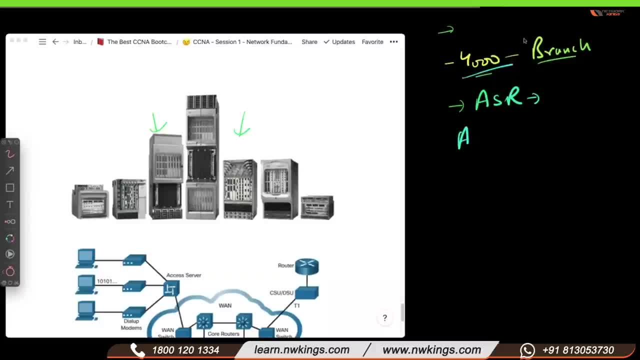 routers are like cisco asr routers. routers are like cisco asr routers: aggregation service routers, aggregation service routers, aggregation service routers. so these small routers are known in cisco. so these small routers are known in cisco. so these small routers are known in cisco isr integrated service router. 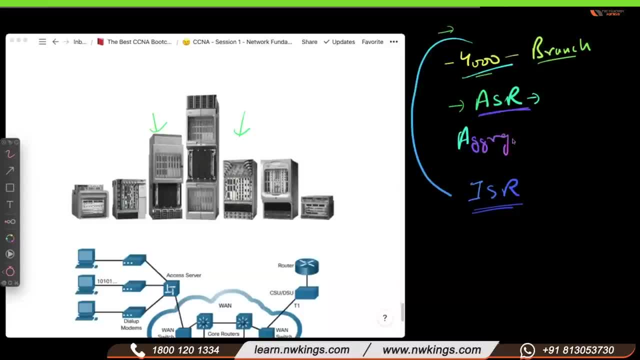 isr- integrated service router. isr- integrated service router. when we talk about asr, that is aggregation. when we talk about asr, that is aggregation. when we talk about asr, that is aggregation. service router, service router, service router, aggregation service routers. and isr is aggregation service routers and isr is. 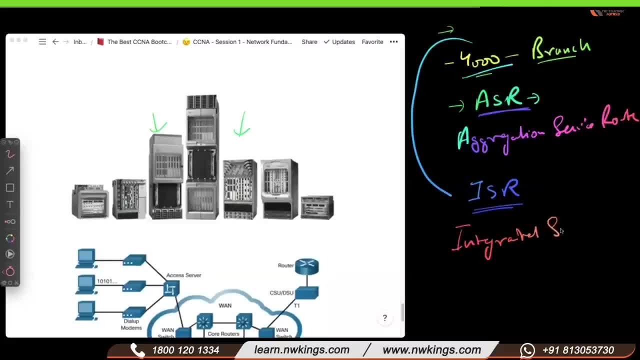 aggregation service routers and isr is integrated service routers. okay, so this is okay, so this is okay. so this is the category isr- asr and cisco has uh, the category isr- asr and cisco has, uh, the category isr- asr and cisco has, uh, i think, one another category, that is. 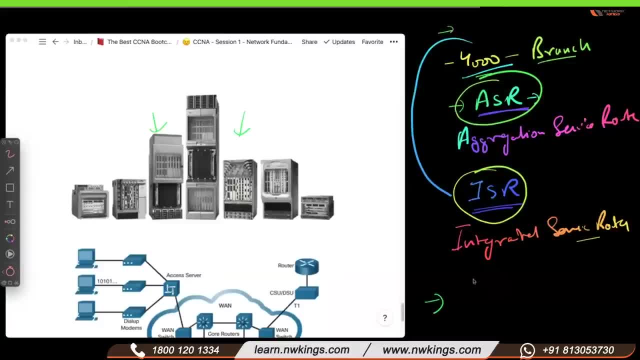 i think one another category, that is. i think one another category, that is i, i, i forget the name, forget the name, forget the name. yeah, csr, yeah, csr, yeah, csr. what was the full form of this carrier? what was the full form of this carrier? what was the full form of this carrier? segregation route or something right. 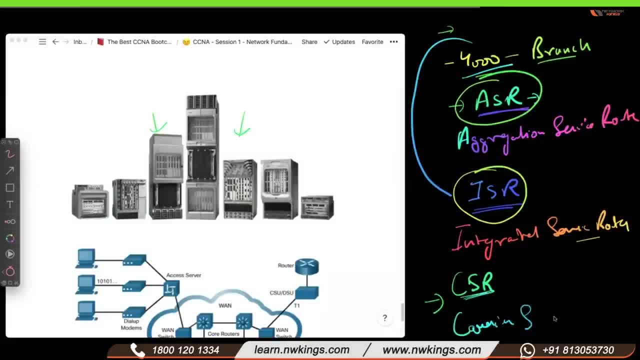 so that was career segregation, or so that was career segregation, or so that was career segregation, or something router segregation, or you can something router segregation, or you can something router segregation, or you can check or google it. so these are the check or google it. so these are the. 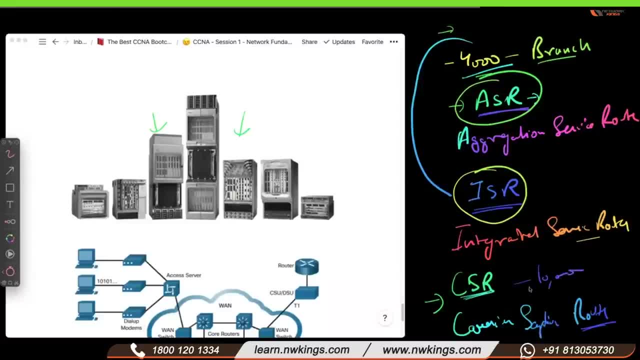 check or google it. so these are the biggest routers like ten thousand series, biggest routers like ten thousand series, biggest routers like ten thousand series, eleven thousand big series. so again these eleven thousand big series. so again these eleven thousand big series. so again these are used by service providers. 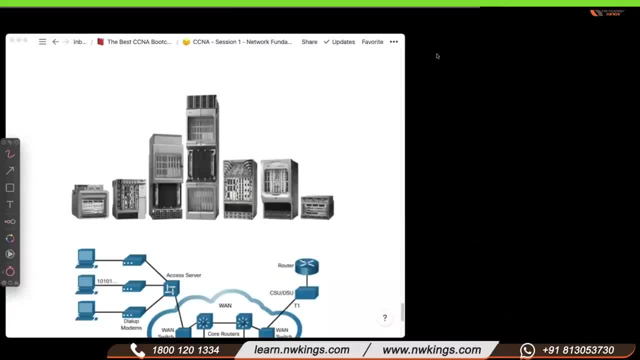 are used by service providers are used by service providers. okay, so same it goes with another vendor. okay, so same it goes with another vendor. okay, so same it goes with another vendor. like, like, like juniper and all, so they have ptx series, juniper and all, so they have ptx series. 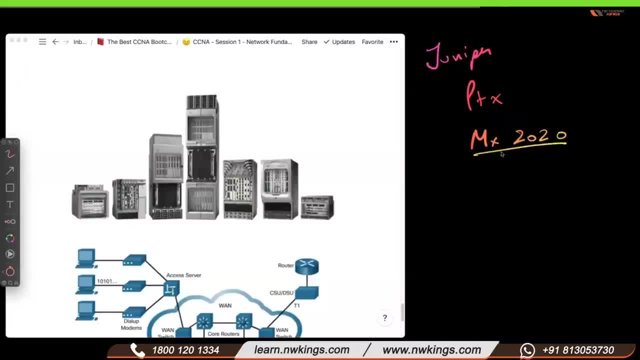 juniper and all. so they have ptx series, they have mx, they have mx, they have mx 2020 is the biggest device right. ptx 2020 is the biggest device. right, ptx 2020 is the biggest device right, ptx 10 000. 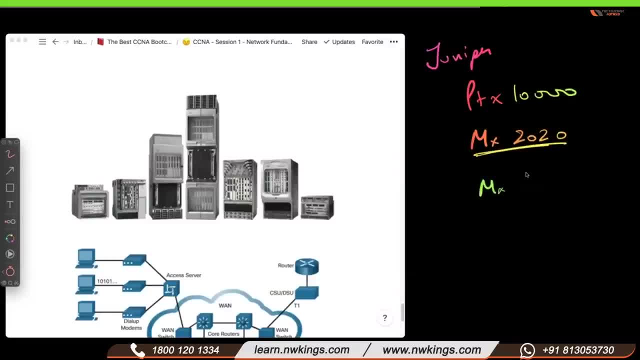 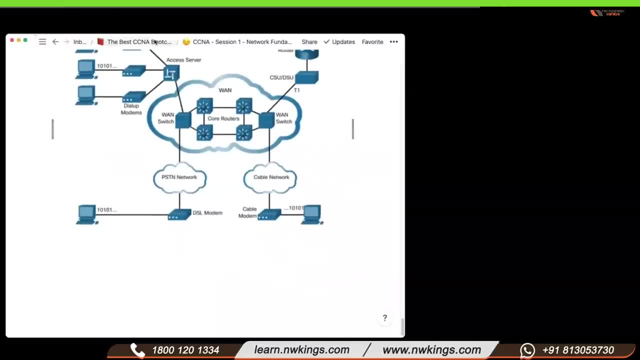 10 000, 10 000, or like the smaller ones are like, or like the smaller ones are like, or like the smaller ones are like: uh, uh, uh, 560 and all 560 and all 560 and all, okay, okay, okay, so, so, so, these are the model names. 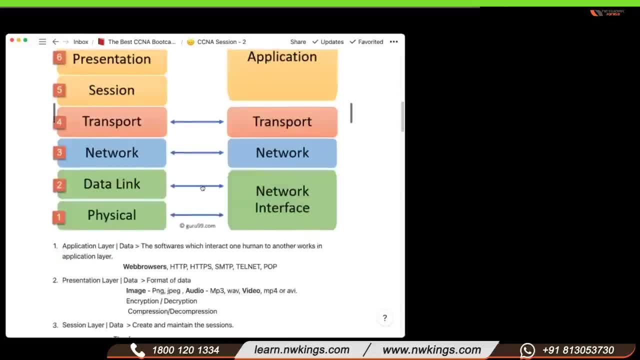 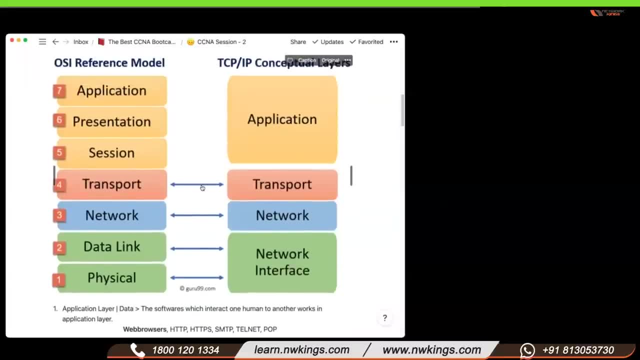 okay, let's come back to osi model now. okay, let's come back to osi model now. okay, let's come back to osi model now. okay, so that was just a quick reviews. if okay, so that was just a quick reviews. if okay, so that was just a quick reviews. if and if anybody joined. 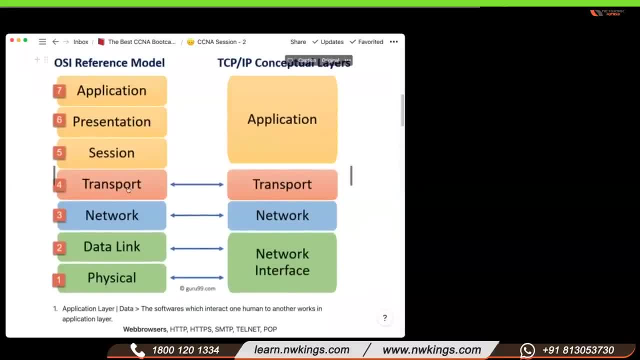 and if anybody joined, and if anybody joined uh session from today onwards, uh session from today onwards, uh session from today onwards. so yesterday we have covered these things. so yesterday we have covered these things. so yesterday we have covered these things like network fundamentals routers, like network fundamentals routers. 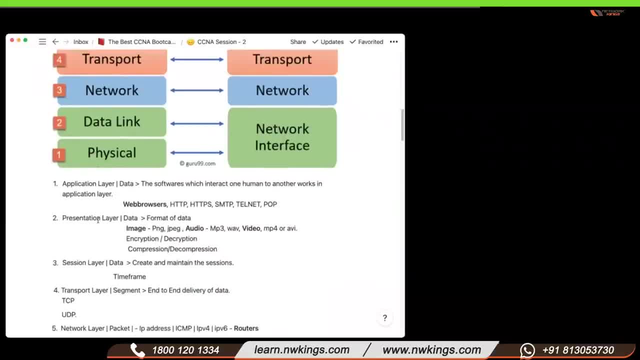 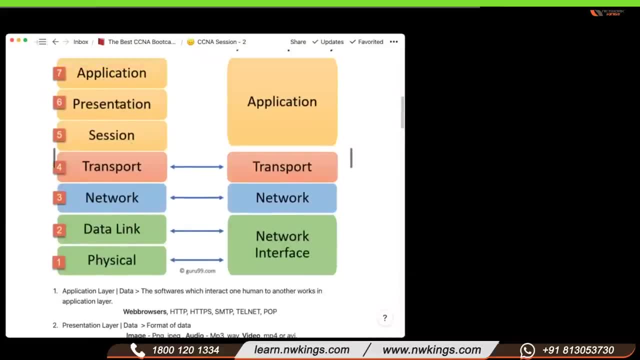 like network fundamentals: routers, switches, switches, switches and all yeah and all, yeah and all, yeah, so, so, so let's start with the application layer. let's start with the application layer. let's start with the application layer. what will happen, what will happen, what will happen and what exactly this layer means. 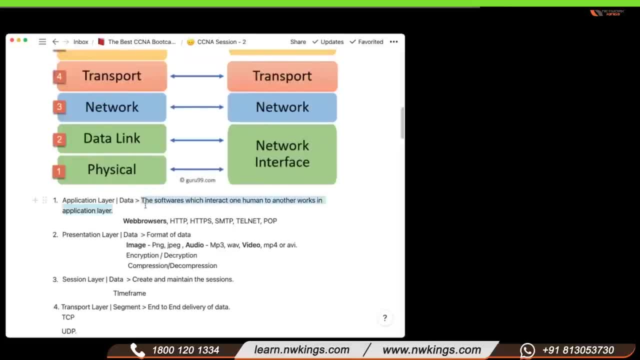 and what exactly this application so application means, and what exactly this application so application means, and what exactly this application so application means, um any softwares which interact one human to um. any softwares which interact one human to um. any softwares which interact one human to another. 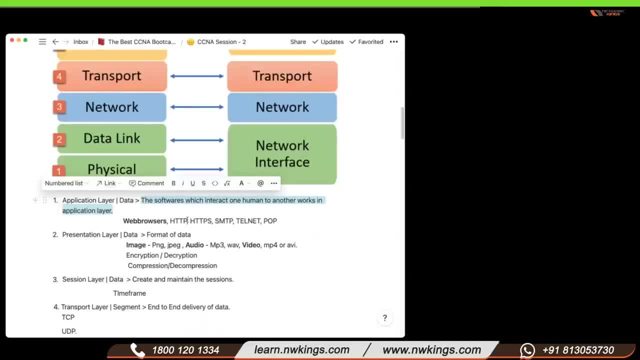 another. another is comes under application layer. is comes under application layer. is comes under application layer. like your uh web browser uses http. like your uh web browser uses http. like your uh web browser uses http. https protocol- right. so when you use https protocol, right. so when you use 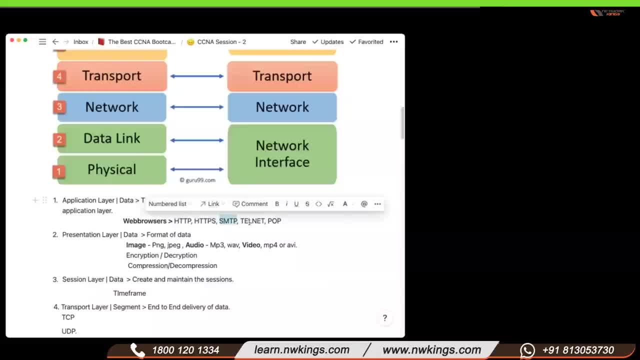 https protocol right. so when you use http https, when you are sending email, http https, when you are sending email, http https, when you are sending email telnet or telnet or telnet, or so all these protocols comes under. so all these protocols comes under. so all these protocols comes under application. 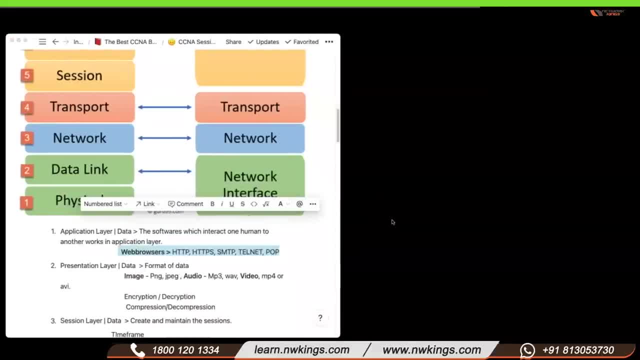 application application: okay, okay, okay, yeah, yeah, yeah, okay. so there are many protocols. i'll discuss. okay, so there are many protocols. i'll discuss. okay, so there are many protocols. i'll discuss in detail, in detail, in detail. okay, this application, but just understand. okay, this application, but just understand. 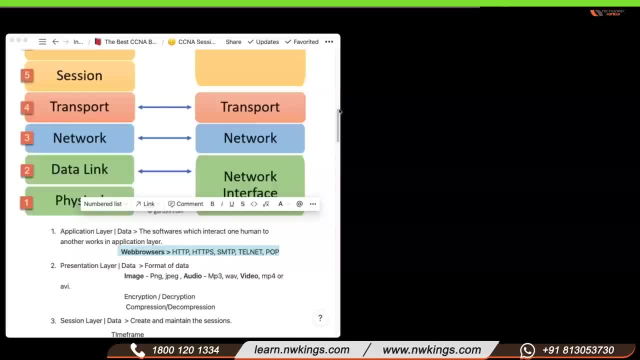 okay this application, but just understand, if anybody wants to communicate with, if anybody wants to communicate with, if anybody wants to communicate with another user from if another user from, if another user from, if one human to another. you can say that one human to another, you can say that. 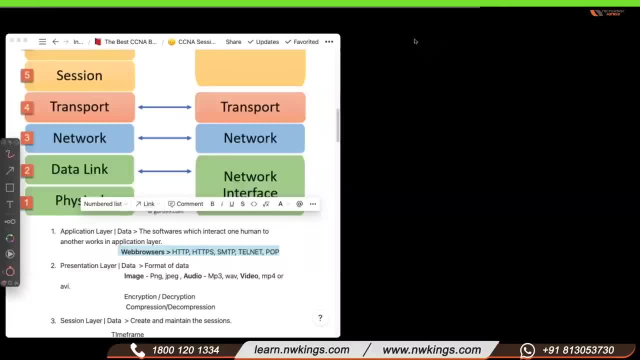 one human to another. you can say that: so they are going to use some thing. so they are going to use some thing. so they are going to use some thing. right, i, you want to access website, you right i? you want to access website. you right, i? you want to access website. you will use http. 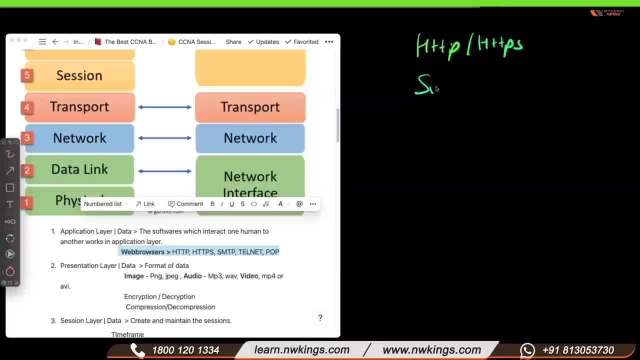 will use http, will use http or https. you want to send a email you. you want to send a email you. you want to send a email. you will use simple mail transfer protocol. will use simple mail transfer protocol. will use simple mail transfer protocol to send a email, to receive email you. 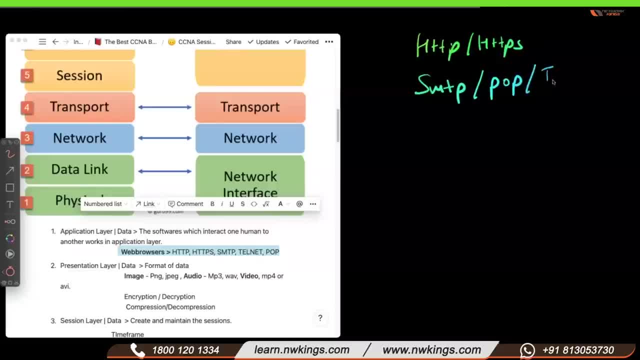 to send a email to receive email. you to send a email to receive email. you will use. will use. will use pop post office protocol. or there is pop post office protocol or there is pop post office protocol, or there is another protocol- imap- another protocol. imap- another protocol. imap- internet message access protocol. so these 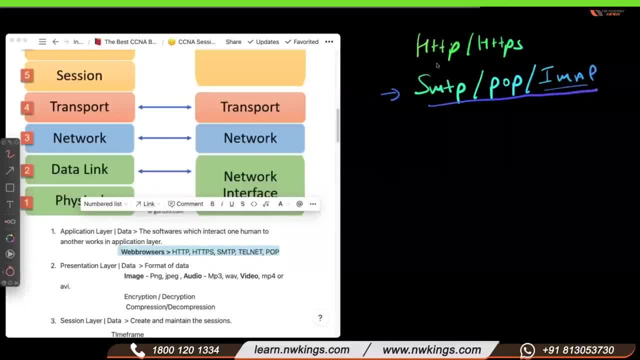 internet message access protocol. so these internet message access protocol, so these all protocols are used by emails. all protocols are used by emails. all protocols are used by emails so that you can send or receive the, so that you can send or receive the, so that you can send or receive the emails. 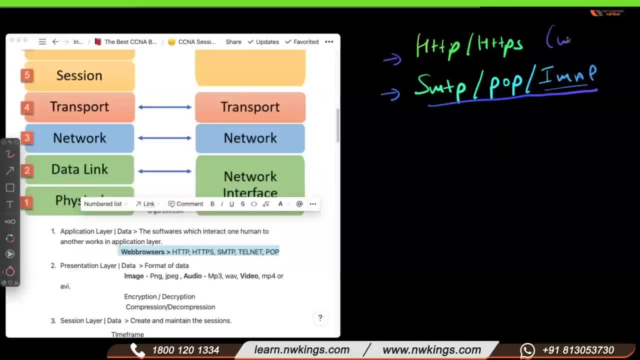 emails, emails. so these two protocols are used for. so these two protocols are used for. so these two protocols are used for www world wide web, so that you can access www world wide web. so that you can access www world wide web. so that you can access the websites right. 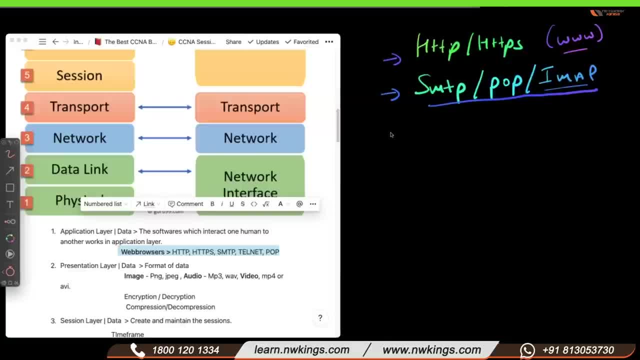 the websites right, the websites right. so there are a lot of protocols which. so there are a lot of protocols which, so there are a lot of protocols which falls under application layer. so falls under application layer, so falls under application layer. so, whenever like file transfer protocol to 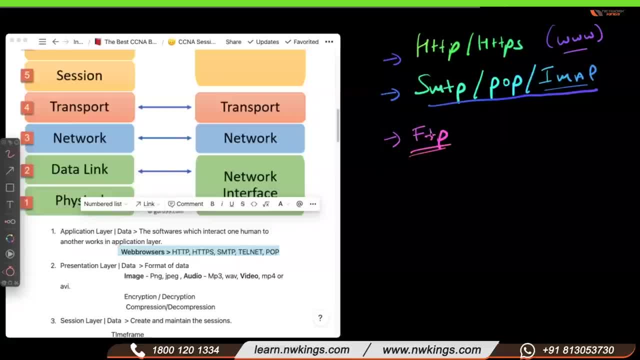 whenever like file transfer protocol to whenever like file transfer protocol to send files, send files. send files to the server. we use ftp. okay, so these to the server, we use ftp. okay, so these to the server, we use ftp. okay, so these protocols and if you want to access, 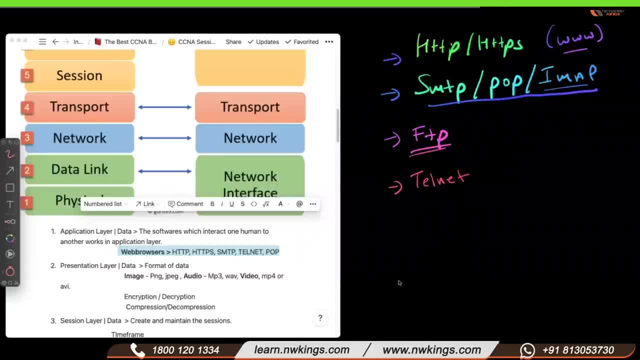 protocols and if you want to access protocols and if you want to access any device remotely, any device remotely, any device remotely. so you are in india right now and you so you are in india right now and you so you are in india right now and you want to access a router which is in usa. 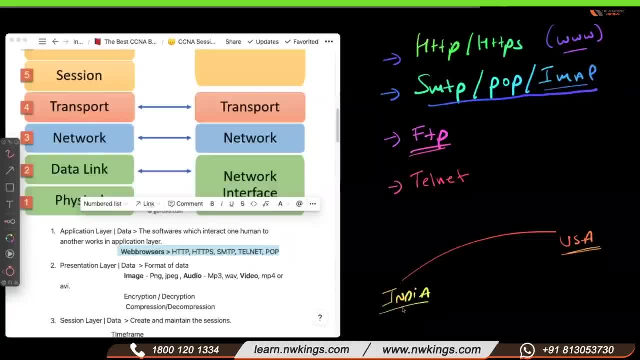 want to access a router which is in usa, want to access a router which is in usa, so so, so you are in india, so you are working as a. you are in india, so you are working as a. you are in india, so you are working as a network engineer for any us company from. 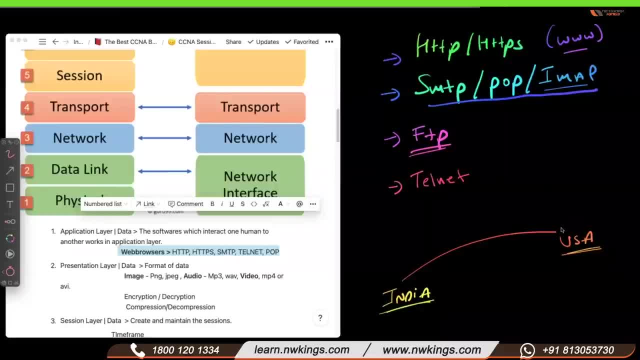 network engineer for any us company, from network engineer for any us company from here, here, here, so you can directly access the router. so you can directly access the router, so you can directly access the router from here, from here, from here. okay, so that is telnet and there is a. 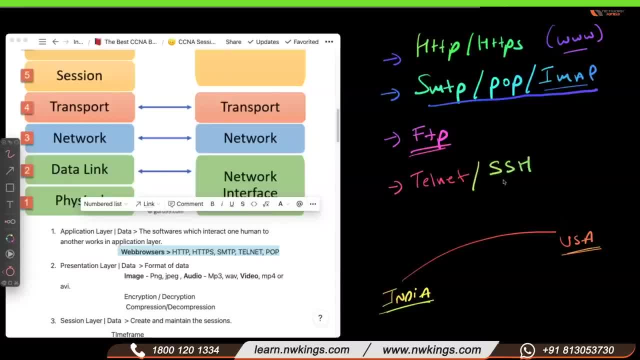 okay, so that is telnet. and there is a okay, so that is telnet. and there is a secure, secure, secure version of it that is known as ssh. so secure version of it that is known as ssh, so secure version of it that is known as ssh. so that is for to remotely access the. 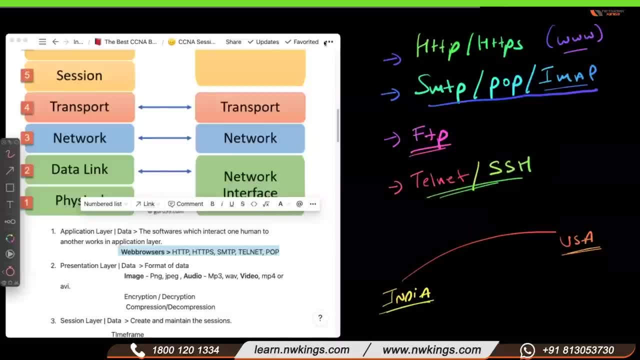 that is for to remotely access the, that is for to remotely access the devices, devices, devices, right, right, right, yeah, yeah, yeah, so these all, so, these all, so these all, if you see, if you see, if you see, from application point of view, all we are, from application point of view, all we are. 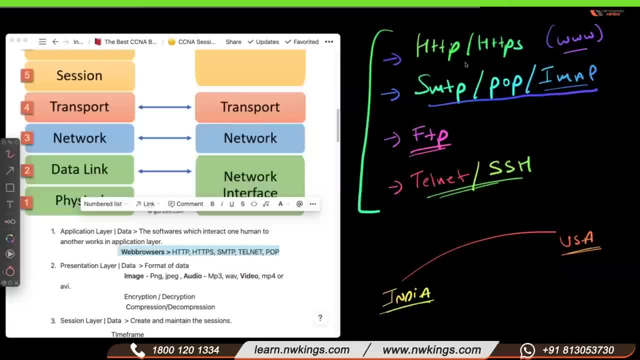 from application point of view. all we are doing, we are doing, we are doing. we are using these application for sharing data, using these application for sharing data, using these application for sharing data. so we are accessing the websites we are. so we are accessing the websites we are. 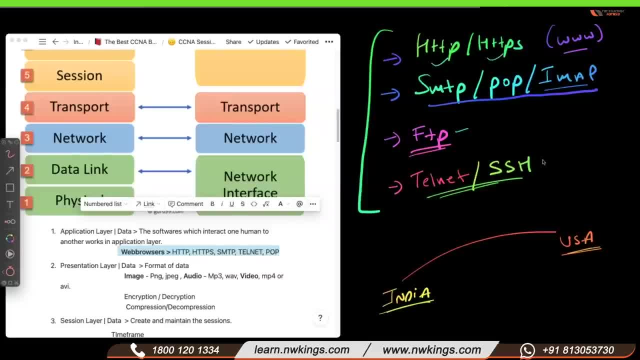 so we are accessing the websites, we are sending emails, we are sending files, we sending emails, we are sending files, we sending emails, we are sending files. we are actually accessing the routers, actually accessing the routers, actually accessing the routers- switches or maybe the servers from switches or maybe the servers from. 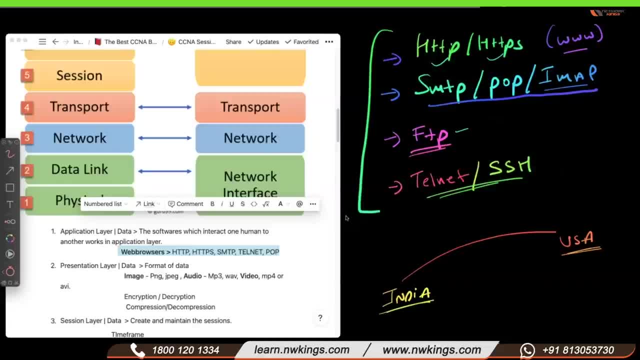 switches, or maybe the servers from internet. so these all falls under internet. so these all falls under internet. so these all falls under application layer, application layer. application layer so any softwares or any protocols which so any softwares or any protocols, which so any softwares or any protocols which interact one human to another, or maybe. 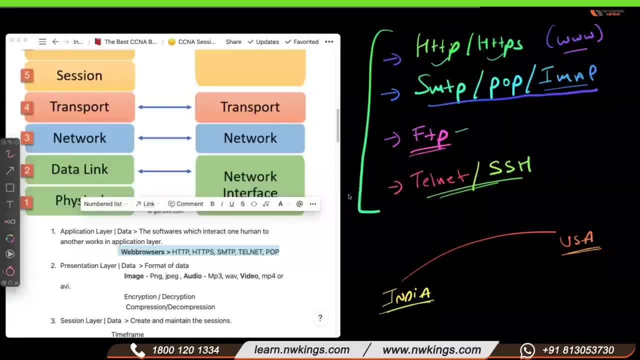 interact one human to another, or maybe interact one human to another, or maybe you are interacting. you are interacting. you are interacting with any, with any, with any protocol. or you are sending data protocol, or you are sending data protocol, or you are sending data somewhere, so you are actually false. 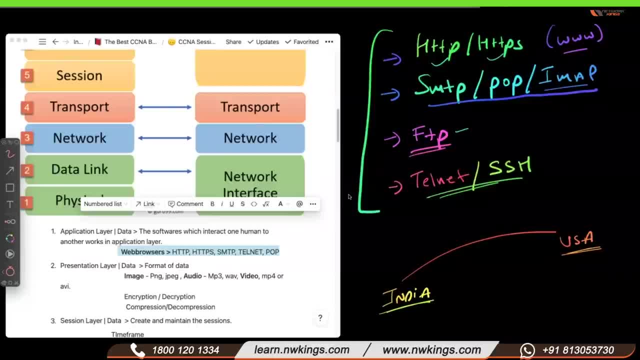 somewhere. so you are actually false, somewhere, so you are actually false. these protocols comes under application. these protocols comes under application. these protocols comes under application, layer, layer, layer, okay, okay, okay. so now the second, so now the second. so now the second one is, or you can say, the sixth layer. 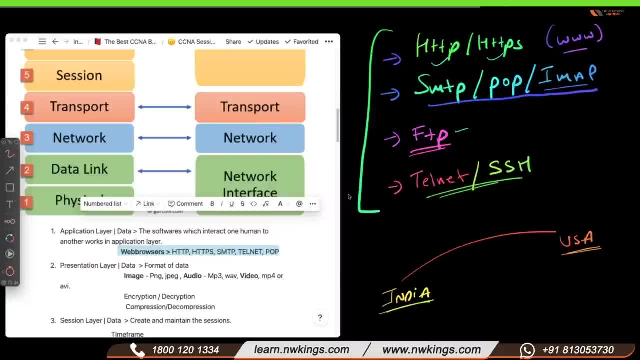 one is, or you can say the sixth layer. one is, or you can say the sixth layer, because seventh is the application layer, because seventh is the application layer, because seventh is the application layer from top to bottom. sixth layer is from top to bottom. sixth layer is from top to bottom. sixth layer is presentation layer. 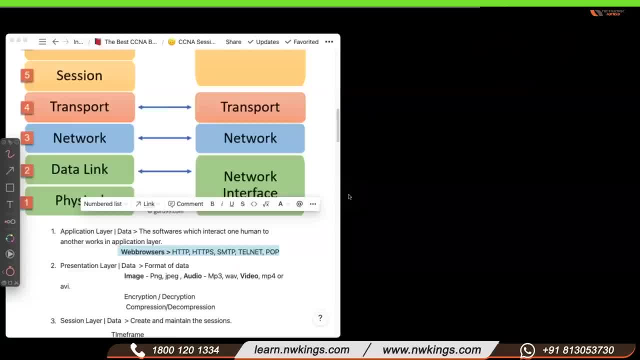 presentation layer, presentation layer. so what does this presentation layer do? so? what does this presentation layer do? so what does this presentation layer do? so presentation layer actually tells so. presentation layer actually tells. so presentation layer actually tells about the format of data, about the format of data, about the format of data. so what is this format of data? so format. 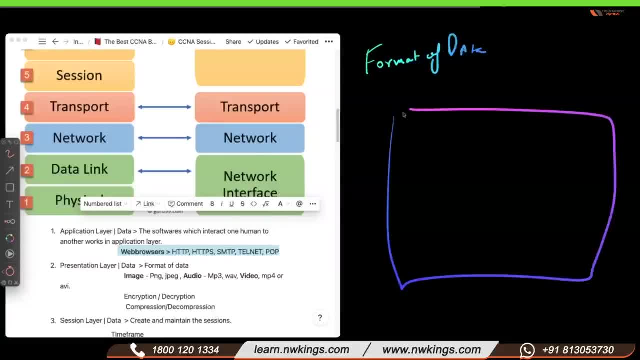 so what is this format of data? so format. so what is this format of data? so format of data, means of data. means of data means: when you see a web page, either it is a when you see a web page, either it is a when you see a web page, either it is a googlecom. 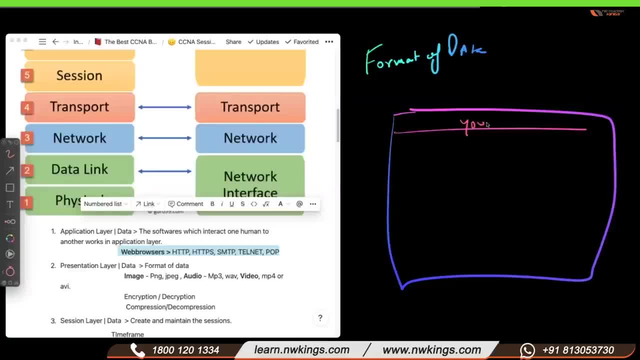 googlecom, googlecom, youtubecom. so let's suppose youtubecom, youtubecom. so let's suppose youtubecom, youtubecom. so let's suppose youtubecom. okay, so you see images. okay, so you see images. okay, so you see images. thumbnails of videos. you are watching a thumbnails of videos. you are watching a. 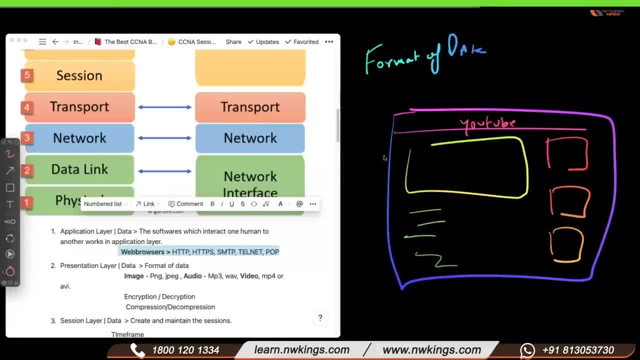 thumbnails of videos you are watching: a video over here, video over here, video over here, comments and all. so the data you are comments and all so the data, you are comments and all so the data you are actually seeing right now. so actually seeing right now, so actually seeing right now. so the data is coming from youtube server in. 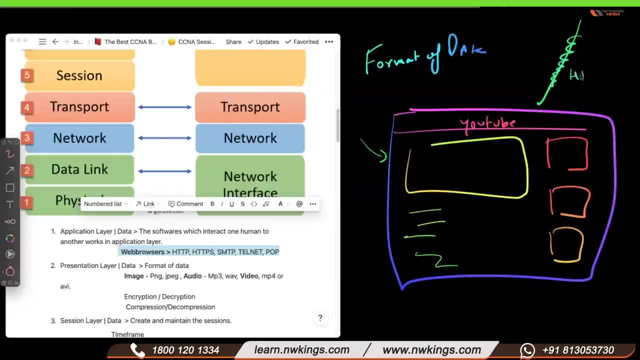 the data is coming from youtube server. in the data is coming from youtube server in the form of some code or some, the form of some code or some, the form of some code or some html or some type of format. but it is html or some type of format, but it is. 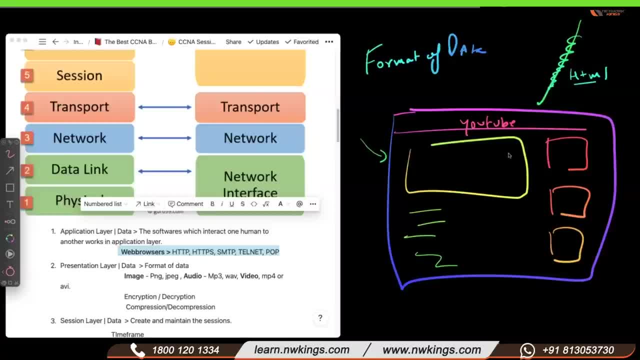 html or some type of format, but it is actually actually actually showing you in your format, right? so showing you in your format, right? so showing you in your format right. so because directly video is not coming, so because directly video is not coming, so because directly video is not coming, so maybe the urls or maybe. 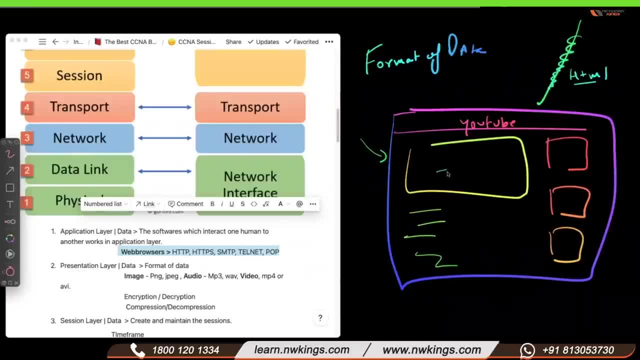 maybe the urls, or maybe, maybe the urls or maybe, uh, the links of videos are coming. so, uh, the links of videos are coming. so, uh, the links of videos are coming, so that it is that, it is that it is. keep on. the video is going to buffer. 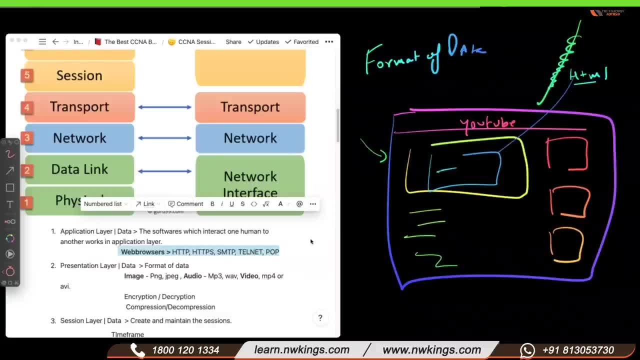 keep on. the video is going to buffer. keep on, the video is going to buffer from the servers, right so i. what i'm from the servers, right so i, what i'm from the servers, right so i. what i'm trying to say means the data you see on. 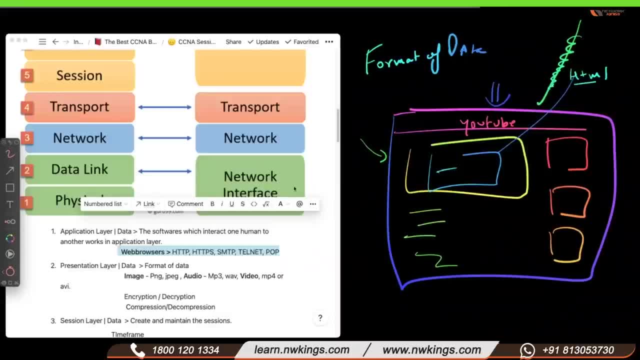 trying to say means the data you see on. trying to say means the data you see on your screen is actually your screen, is actually your screen, is actually uh converted, or you can say that this uh converted, or you can say that this uh converted, or you can say that this presentation layer helps you. 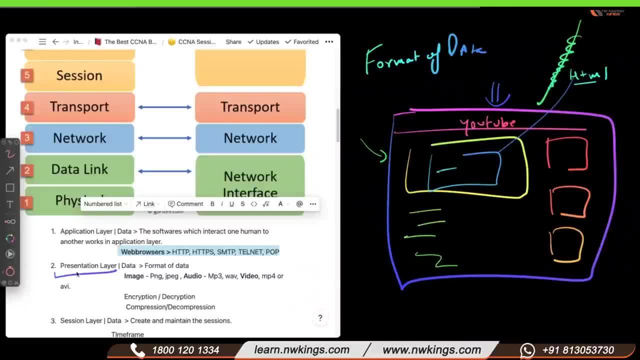 presentation layer helps you. presentation layer helps you. helps us to, helps us to. helps us to show the representation of data. show the representation of data. show the representation of data, or that or that or that. like images in multiple formats like png. like images in multiple formats like png. 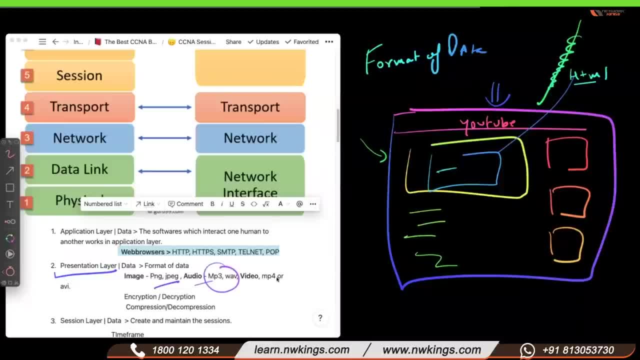 like images in multiple formats, like png, jpg, audio, jpg, audio, jpg. audio is in multiple formats. video is into, is into, is into the presentation layer responsibility. the presentation layer responsibility. the presentation layer responsibility to show the data in the correct format. to show the data in the correct format. 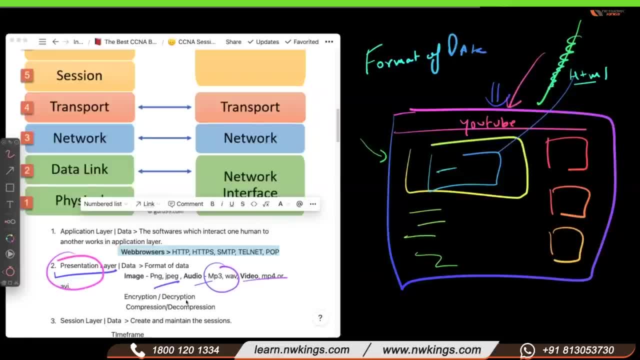 to show the data in the correct format so that you will understand, so that you will understand, so that you will understand, okay, and it is also responsible for okay, and it is also responsible for okay, and it is also responsible for this encryption, decryption, because, if this encryption, decryption, because, if 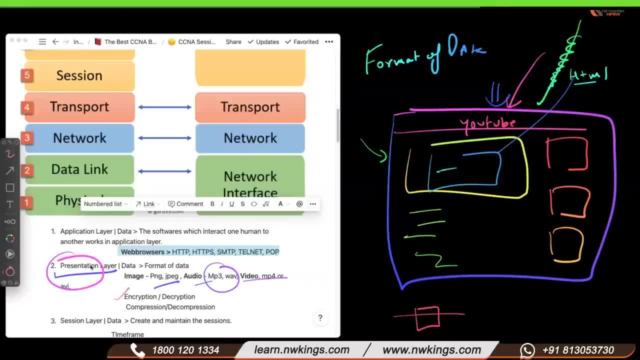 this encryption, decryption, because if you want to encrypt any file or folder, you want to encrypt any file or folder. you want to encrypt any file or folder. the presentation layer is responsible. the presentation layer is responsible. the presentation layer is responsible. again, this is a reference model to just 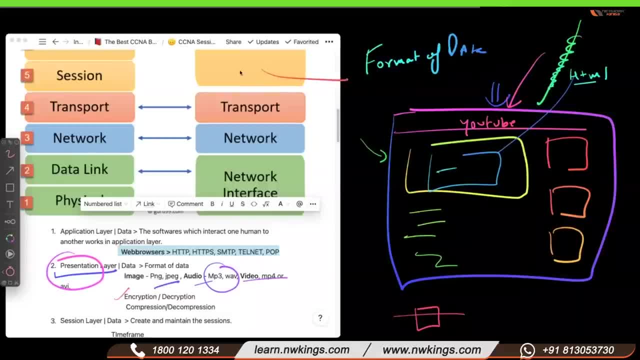 again, this is a reference model to just again, this is a reference model to just understand. but in real world all comes understand, but in real world all comes understand. but in real world all comes under application layer, because all three under application layer, because all three under application layer, because all three layers. 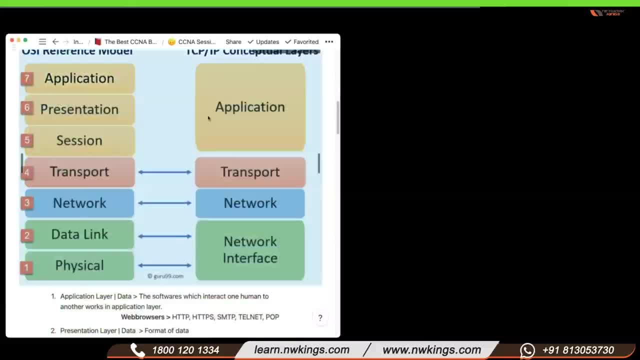 layers, layers, all three layers, all three layers, all three layers. right is known as application in real right, is known as application in real right, is known as application in real world. so when you say in real world, the world, so when you say in real world, the world, so when you say in real world, the format of data is actually taking care. 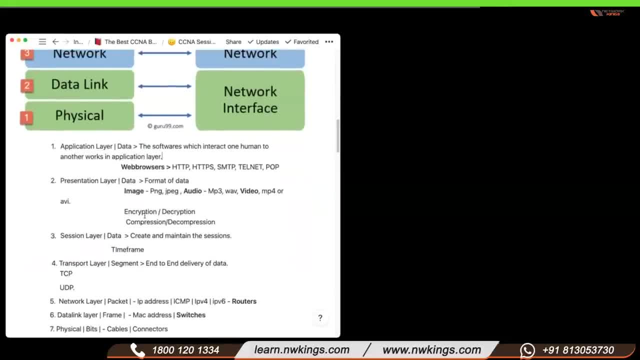 format of data is actually taking care, format of data is actually taking care by application layer, by application layer, by application layer- okay, but here, when we discuss a osi, okay, but here, when we discuss a osi, okay, but here when we discuss a osi model, it falls under presentation layer. 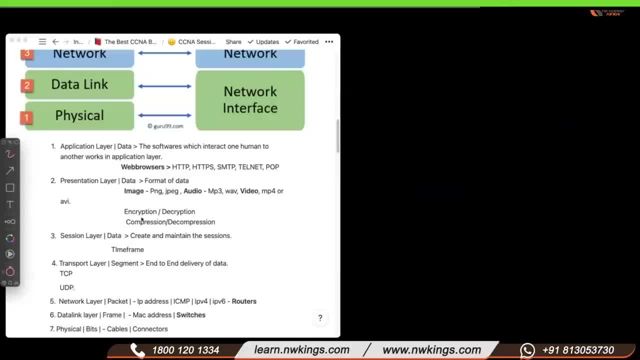 okay guys, okay guys, okay guys. so when now the data is also so, when now the data is also so, when now the data is also uh like this in this presentation layer, uh like this in this presentation layer, uh like this in this presentation layer, presentation layer is also responsible. 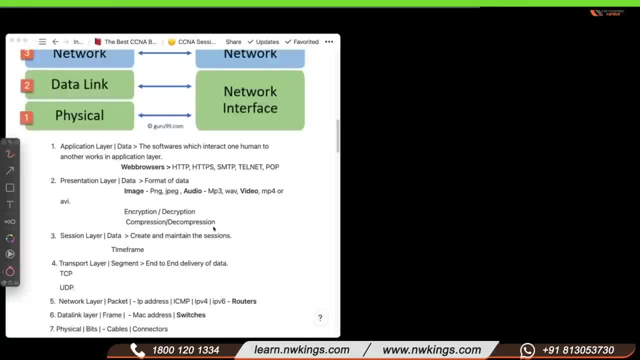 presentation layer is also responsible. presentation layer is also responsible for compression and decompression. means for compression and decompression. means for compression and decompression. means to reduce or increase the size of the. to reduce or increase the size of the. to reduce or increase the size of the files. 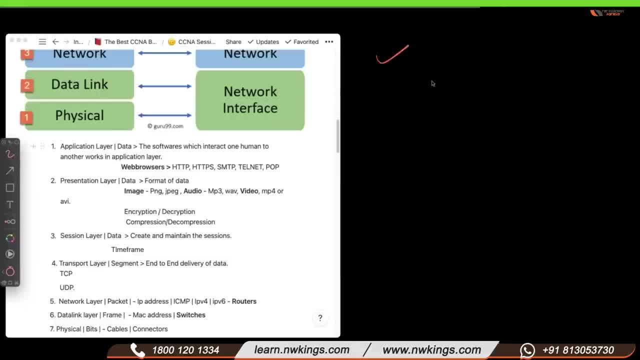 files, files. so these two layers, so these two layers, so these two layers done right. so applications means the done right. so applications means the done right. so applications means the applications which interact one human to applications, which interact one human to applications, which interact one human to another, in presentation layer just. 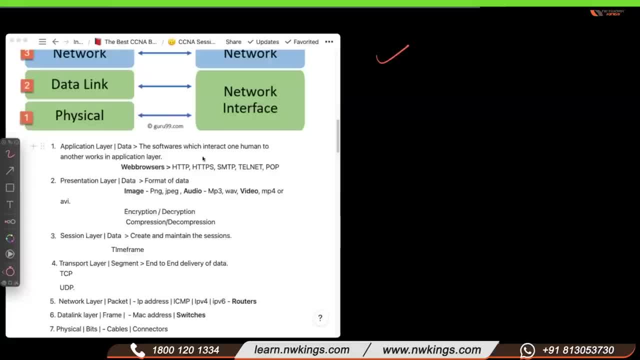 another in presentation layer. just another in presentation layer. just remember the keywords. remember the keywords, remember the keywords, just remember the keywords. the keyword is: just remember the keywords. the keyword is: just remember the keywords. the keyword is: here the applications or the software, here the applications or the software. 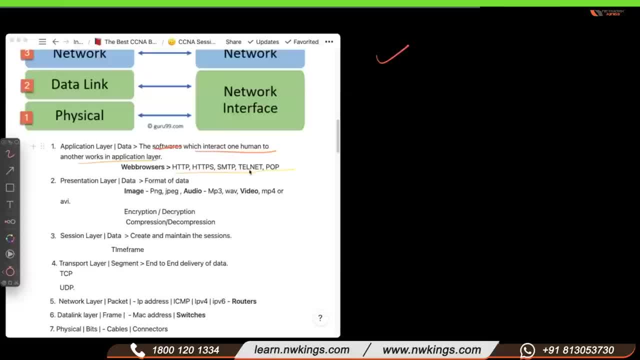 here the applications or the software which interact one human to another, or which interact one human to another, or which interact one human to another, or maybe you can learn the protocol names. maybe you can learn the protocol names. maybe you can learn the protocol names and in presentation layer, the keyword is: 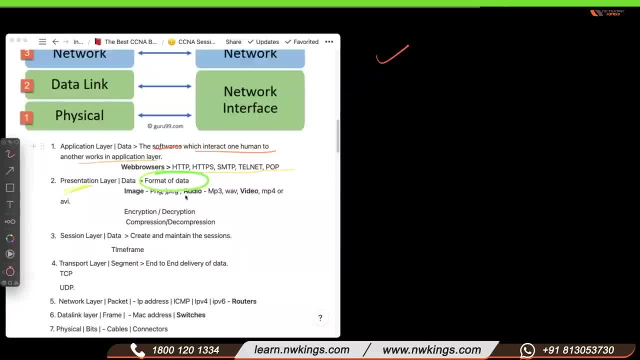 and in presentation layer, the keyword is: and in presentation layer, the keyword is: format of data. so just remember the format of data. so just remember the format of data. so just remember the format of data, format of data, format of data, so when the data is, so when the data is. 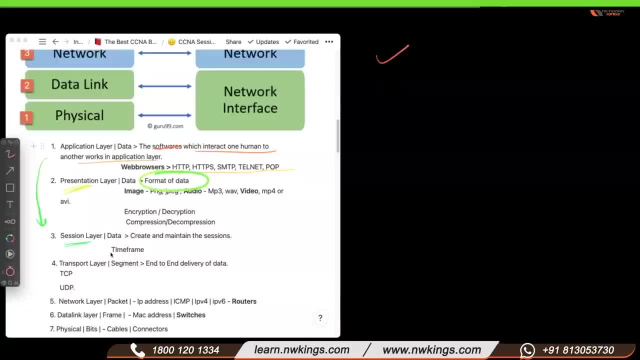 so when the data is moving to session layer, so session layer moving to session layer, so session layer moving to session layer, so session layer is actually is actually is actually creating and maintaining the sessions. so creating and maintaining the sessions. so creating and maintaining the sessions. so whenever you open any bank bank website, 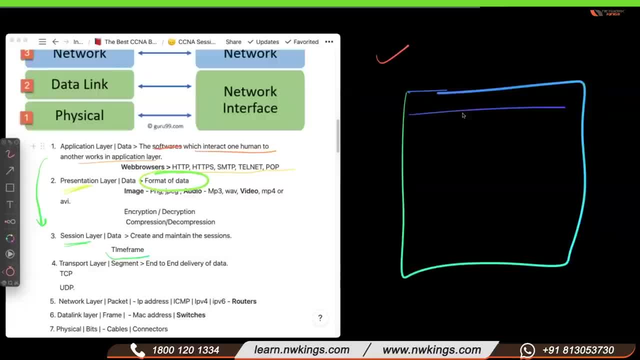 whenever you open any bank bank website. whenever you open any bank bank website, right, right, right, so it has a time limit. so if you don't so, it has a time limit. so if you don't so, it has a time limit. so if you don't use your, 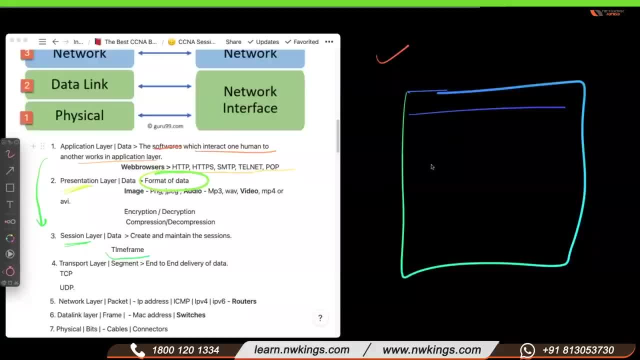 use your. use your like if you are away from keyboard. like like. if you are away from keyboard, like like if you are away from keyboard. like for for for almost five minutes or 10 minutes. right, the almost five minutes or 10 minutes. right, the almost five minutes or 10 minutes. right. the session will automatically log out. 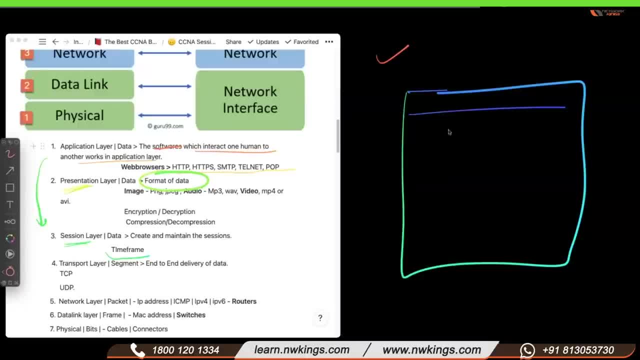 session will automatically log out. session will automatically log out if you are not. if you are not, if you are not using your screen, or you are not using using your screen, or you are not using using your screen, or you are not using mouse pointers or anything- mouse pointers or anything. 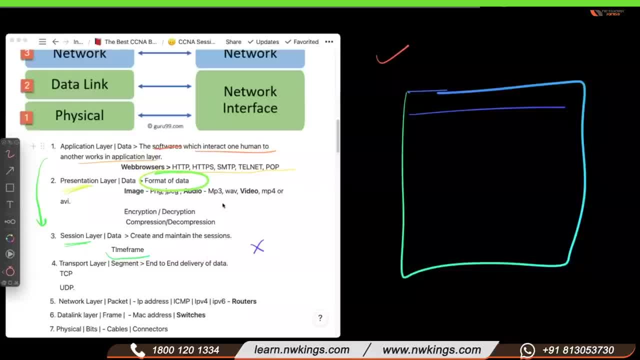 mouse pointers or anything, so the session will log out automatically. so the session will log out automatically. so the session will log out automatically. so why? because this session layer is so? why because this session layer is so? why? because this session layer is controlling that, controlling that, controlling that time frame. so whenever developers 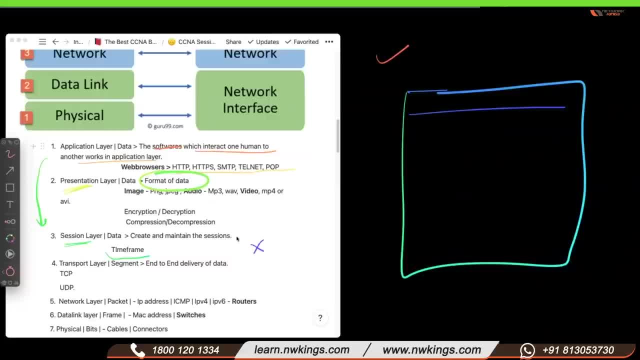 time frame. so whenever developers time frame, so whenever developers actually makes websites or applications, actually makes websites or applications, actually makes websites or applications, they actually code, they actually code, they actually code that time frame with the session layer, that time frame with the session layer, that time frame with the session layer algorithms. 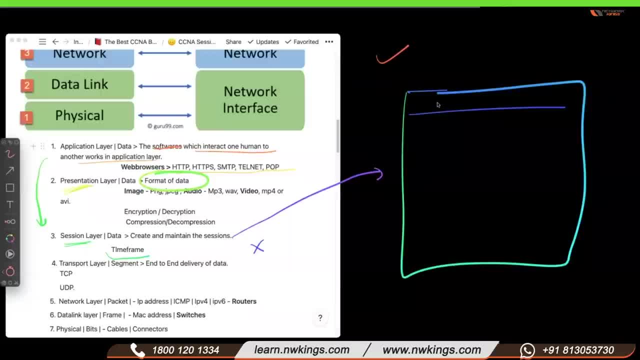 algorithms, algorithms. so suppose, if i'm- uh, let me okay, suppose i'm, let me okay, suppose i'm, let me okay. suppose i'm using one bank. suppose hsbc bank. okay, using one bank. suppose hsbc bank, okay, using one bank, suppose hsbc bank, okay. so in this bank i'm not able, i'm not. 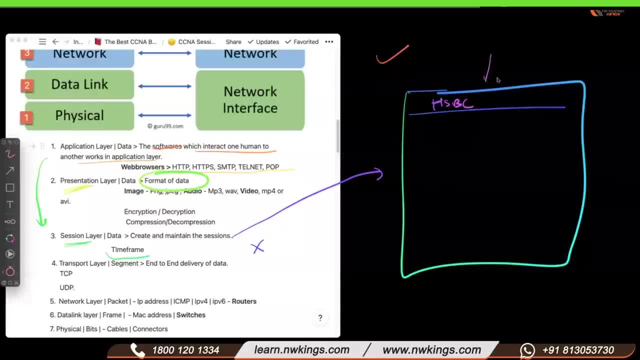 so in this bank, i'm not able. i'm not. so in this bank, i'm not able. i'm not. using this screen for almost 10 minutes. using this screen for almost 10 minutes, using this screen for almost 10 minutes. so hsbc website is actually coded with. 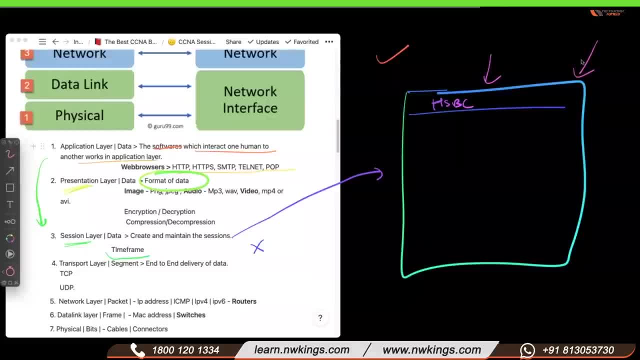 so hsbc website is actually coded with. so hsbc website is actually coded with like by developers. it is in like by developers. it is in like by developers. it is in it. it's integrated with some session. it. it's integrated with some session it. it's integrated with some session programs. 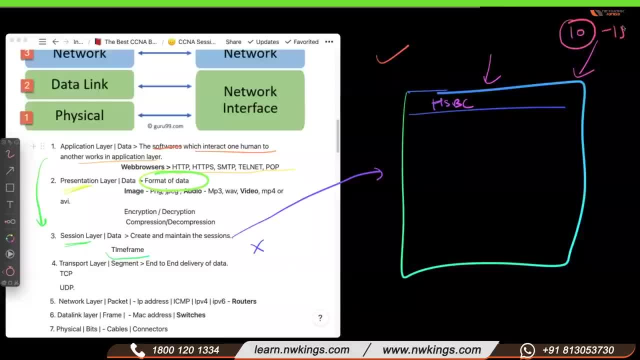 programs: programs: like the session will log out after 10. like the session will log out after 10. like the session will log out after 10 minutes or maybe 15 minutes. so all falls minutes, or maybe 15 minutes. so all falls minutes, or maybe 15 minutes. so all falls under this session layer. so session. 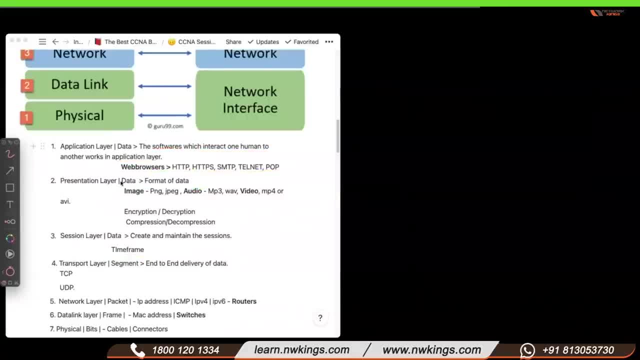 under this session layer, so session under this session layer. so session layer means layer means layer means the time frame in which the session will, the time frame in which the session will, the time frame in which the session will be be be controlled. this session layer actually controlled, this session layer actually. 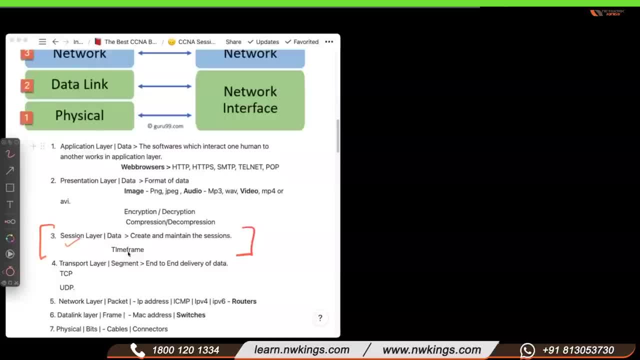 controlled. this session layer actually create and maintain the sessions with. create and maintain the sessions with. create and maintain the sessions with the time frame, the time frame, the time frame. okay, so all three layers clear, so okay. so all three layers clear, so okay. so all three layers clear. so application means the softwares or the 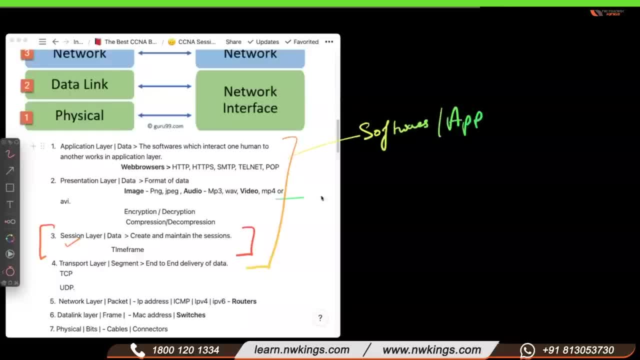 application means the softwares, or the application means the softwares or the applications. in this. we actually in this, we actually in this. we actually takes care of format of data, takes care of format of data, takes care of format of data. this is the keyword and in session layer, 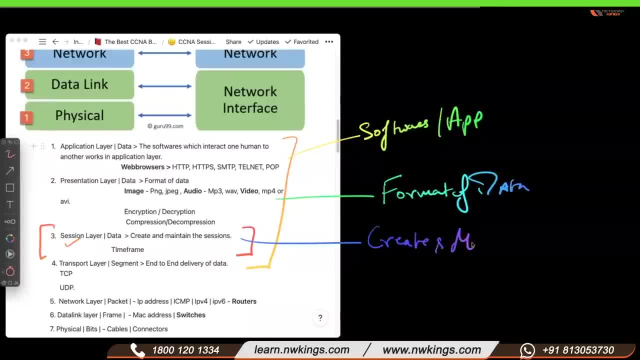 this is the keyword and in session layer, this is the keyword and in session layer, we actually, we actually, we actually create and maintain the time frames. yes guys, nobody is responding in the. yes guys, nobody is responding in the. yes guys, nobody is responding in the chat chat. 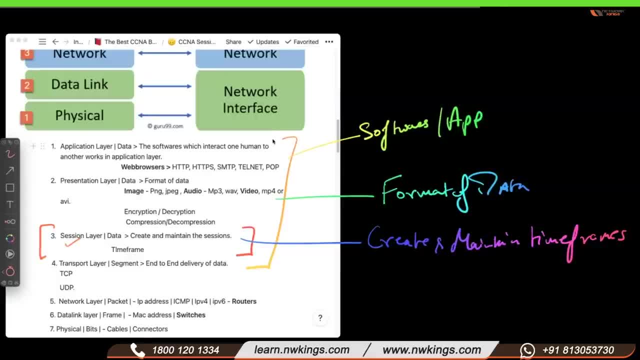 chat. what happened? hello, hello, okay, snmp will, snmp will, snmp will determine, snmp will determine. discuss that is an network management. discuss that is an network management. discuss that is an network management protocol, protocol, protocol. okay, great, okay, great, okay, great, okay. so all three. 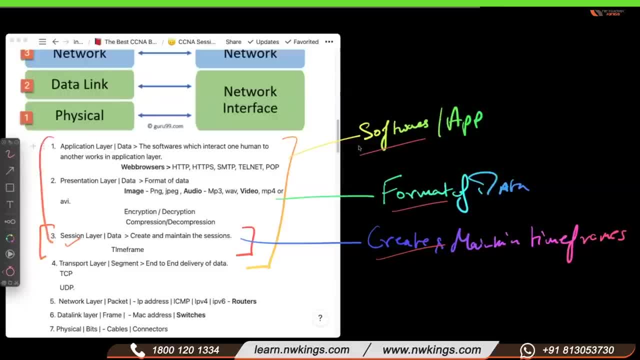 okay, so all three. okay, so all three falls under, falls under, falls under these three and all three layers are in these three and all three layers are in these three and all three layers are in real world. they are known as real world. they are known as real world. they are known as application layer. 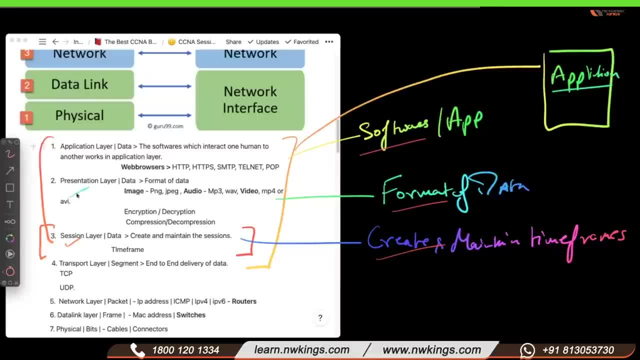 application layer, application layer. so you will not find actually. so you will not find actually, so you will not find actually presentation layer or session layer or presentation layer or session layer or presentation layer or session layer or application different in real world. application different in real world. application different in real world because in real world all falls under 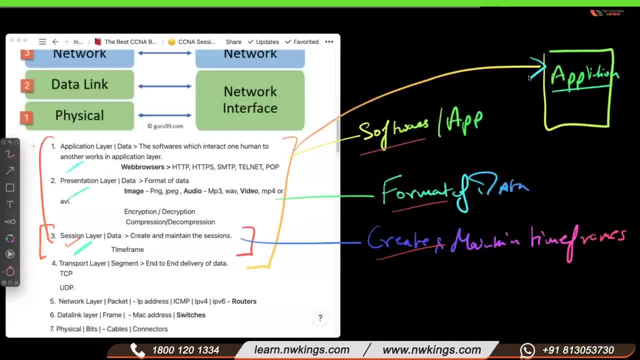 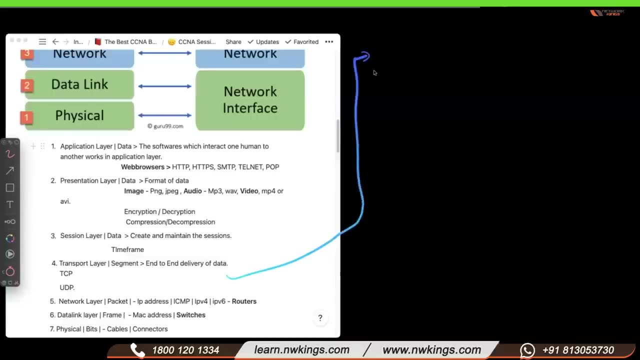 because in real world, all falls under, because in real world, all falls under one layer, that is application. one layer, that is application. one layer, that is application. okay, okay, okay, clear, so now, so, now, so now. this is very important layer of, this is very important layer of. 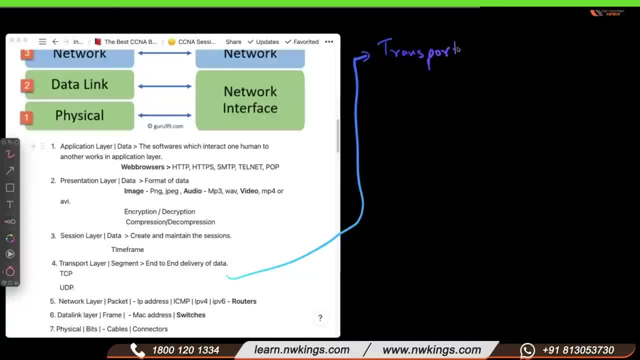 this is very important layer of, so that is transport layer. so now, when we discuss about three layers, so now when we discuss about three layers, so now, when we discuss about three layers, so the data is in which format data, so the data is in which format data. 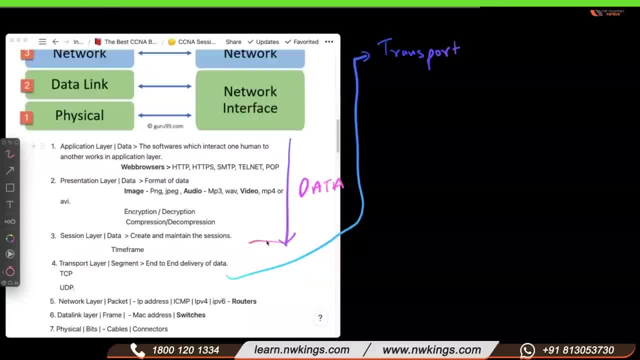 so the data is in which format data? so now, when the data comes to transport? so now, when the data comes to transport. so now, when the data comes to transport, layer, it actually layer, it actually layer, it actually converts the data into segments, converts the data into segments. 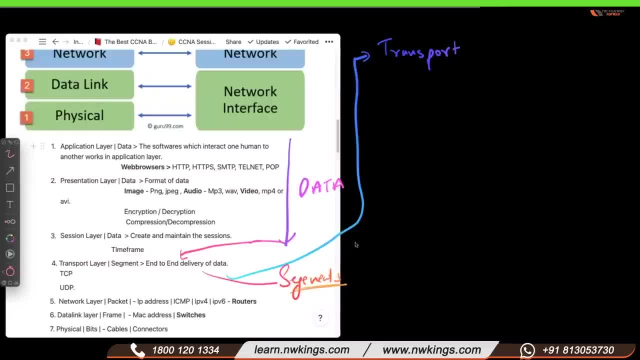 converts the data into segments. it means it will divide the data into it, means it will divide the data into it, means it will divide the data into multiple, multiple, multiple chunks or parts, chunks or parts, chunks or parts. so, whenever, so, whenever so, whenever, from above level, above layers, we are 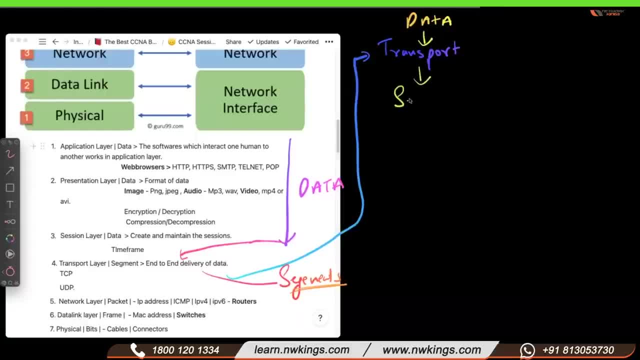 from above level above layers. we are from above, level above layers. we are getting data, and transport layer is getting data and transport layer is getting data, and transport layer is actually converting these packets into actually converting these packets, into actually converting these packets into segments, segments. segments, okay means you are getting a data. 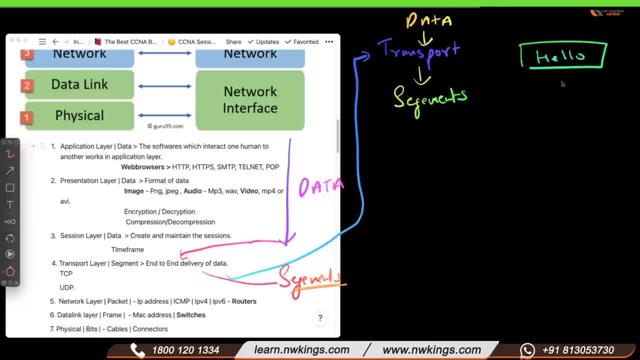 okay means you are getting a data. okay means you are getting a data. okay, suppose this is data. okay, suppose this is data. okay, suppose this is data, not just hello. i'm just giving an example, not just hello. i'm just giving an example, not just hello. i'm just giving an example. so when the data is going to transport, 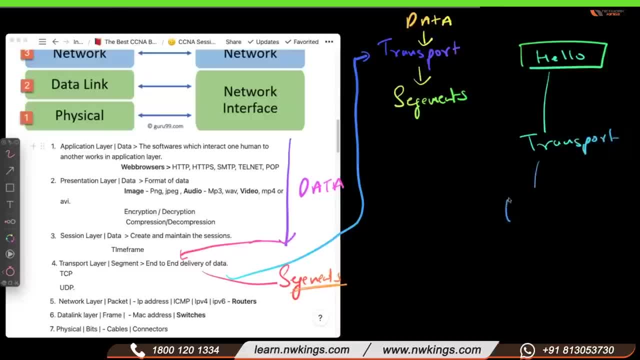 so when the data is going to transport, so when the data is going to transport layer, it is actually segmenting the data layer. it is actually segmenting the data layer. it is actually segmenting the data into, into, into multiple parts, multiple parts, multiple parts like this: 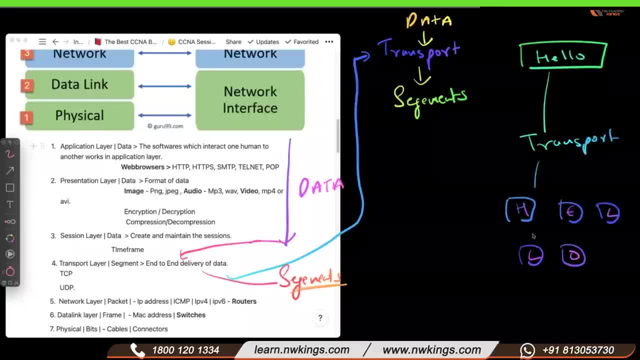 like this, like this. so again, hello is very small. so i'm just so, again, hello is very small, so i'm just so again hello is very small, so i'm just explaining you what is happening. so the explaining you what is happening, so the explaining you what is happening, so the data is actually converting and so this is. 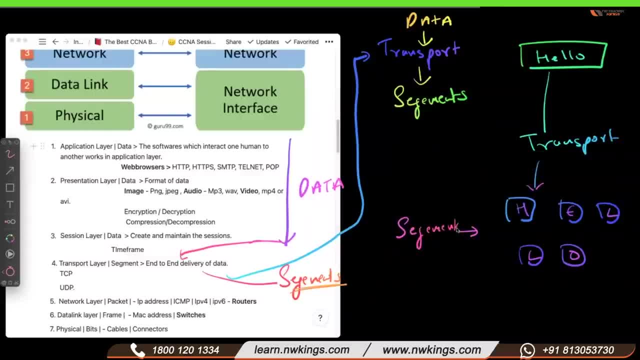 data is actually converting, and so this is data is actually converting, and so this is known as segmentation, segmentation, segmentation, segmentation. okay, and also this transport layer is okay, and also this transport layer is okay, and also this transport layer is responsible for sequencing, responsible for sequencing, responsible for sequencing. what is this? sequencing, sequencing? 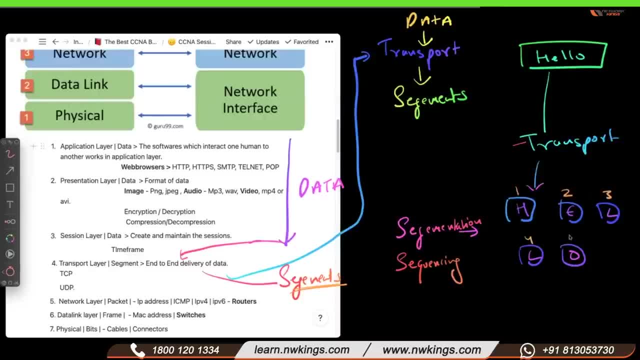 what is this sequencing sequencing? what is this sequencing sequencing? so it will actually add the number on, so it will actually add the number on, so it will actually add the number on the data, the data, the data. why? because when data is going from one. why because when data is going from one, 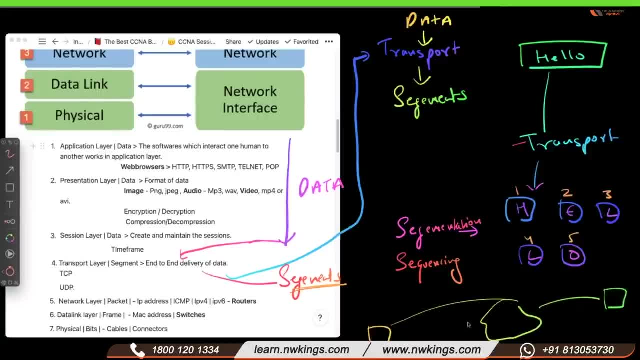 why? because when data is going from one pc over the internet to any another pc over the internet, to any another pc over the internet, to any another device, device, device over the internet or over the internet, or over the internet or in your lan network, in your lan network. 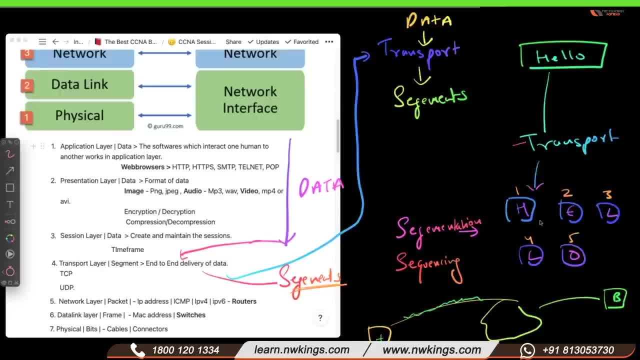 in your lan network, anywhere, anywhere, anywhere. so the data is traveling. so might be so the data is traveling. so might be. so the data is traveling. so might be. there is a chance, there is a chance. there is a chance. the packet will be, the packet will be. 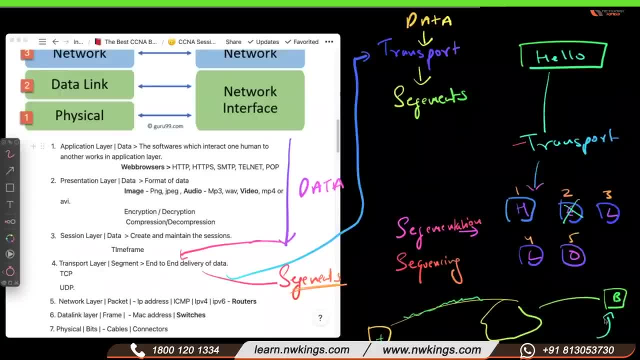 the packet will be dropped, dropped, dropped, and when the data is going to be, and when the data is going to be and when the data is going to be. so b will check. okay, i got one, so b will check. okay, i got one, so b will check. okay, i got one. three, four, five. i haven't received the. 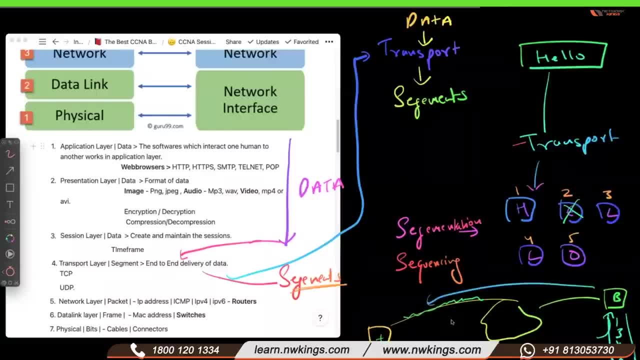 three, four five. i haven't received the three four five. i haven't received the second number sequence. second number sequence. second number sequence. can you please retransmit? can you please retransmit? can you please retransmit? can you send me again? so in this transport. 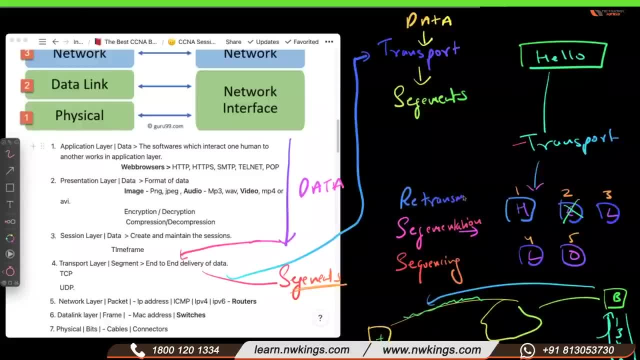 can you send me again? so in this transport, can you send me again? so in this transport layer, we actually layer, we actually layer, we actually do retransmission also. okay, so transport layer is responsible. okay, so transport layer is responsible. okay, so transport layer is responsible for. 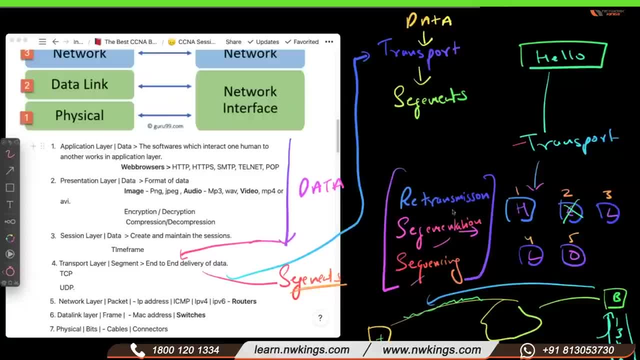 for for multiple things. so like sequencing multiple things. so like sequencing multiple things. so like sequencing segmentation, retransmission. all this segmentation retransmission, all this segmentation retransmission, all this stuff, but transport layer actually stuff. but transport layer actually stuff. but transport layer actually divided into two protocols. 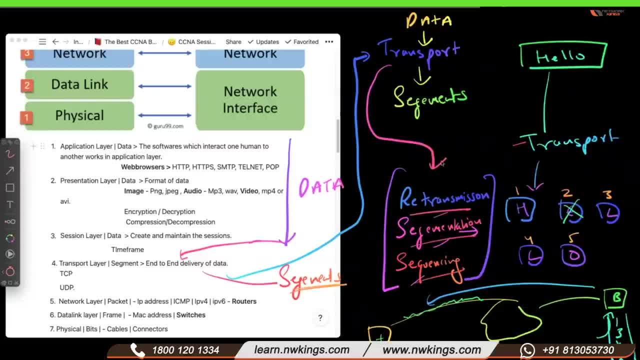 divided into two protocols, divided into two protocols. so all this retransmission segmentation, so all this retransmission segmentation, so all this retransmission segmentation, sequencing: all comes under tcp sequencing, all comes under tcp sequencing, all comes under tcp. yes, nickel, correct sequencing is. yes, nickel, correct sequencing is. 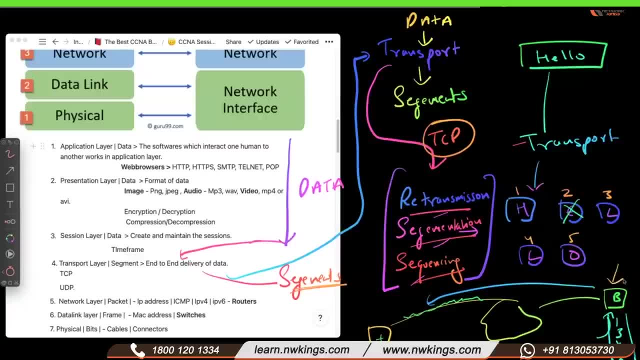 yes, nickel, correct sequencing is. used so that we can assemble or reassemble. used so that we can assemble or reassemble. used so that we can assemble or reassemble the data at the destination end. okay, so that is the overview. now let's. okay, so that is the overview. now let's. 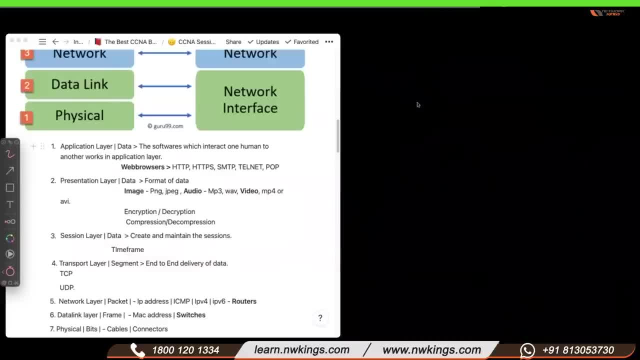 okay, so that is the overview. now let's start start start transport layer. okay so, in transport transport layer. okay so in transport transport layer. okay so in transport layer. i have explained you: the data is layer. i have explained you. the data is layer. i have explained you. the data is divided into segmentation. but before 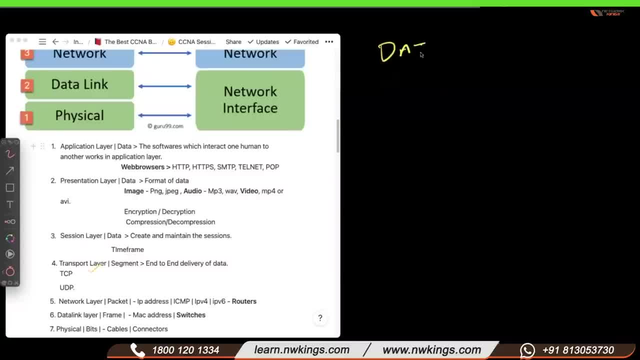 divided into segmentation, but before divided into segmentation, but before doing that. so the now data is coming doing that, so the now data is coming doing that, so the now data is coming from above layer, from above layer, from above layer. okay, so now you can just say that we 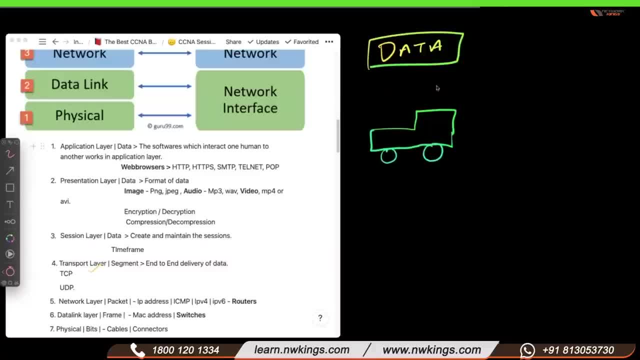 okay, so now you can just say that we okay, so now you can just say that we have, so the data is going. so the data is going, so the data is going in. we have two trucks over here in. we have two trucks over here in. we have two trucks over here, so one truck is known, as you can say. 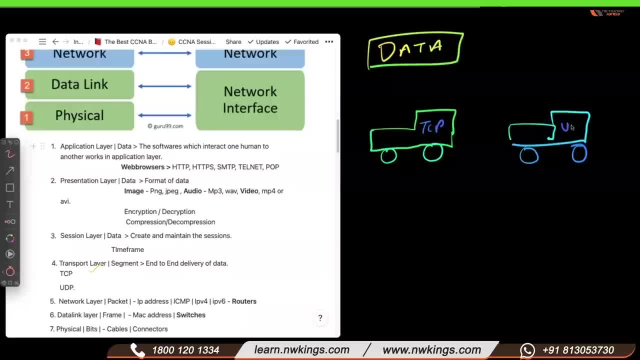 so one truck is known as you can say. so one truck is known as you can say that it's a tcp, that it's a tcp, that it's a tcp and this is a udb, and this is a udb and this is a udb. so now data either, if data is going. 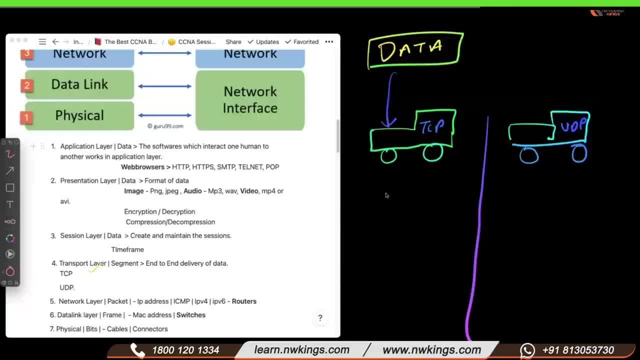 so now data. either if data is going, so now data, either if data is going with this, with this, with this proc, what will happen proc? what will happen proc? what will happen? so, whenever we send any data with tcp, so whenever we send any data with tcp, so whenever we send any data with tcp, whenever. so this 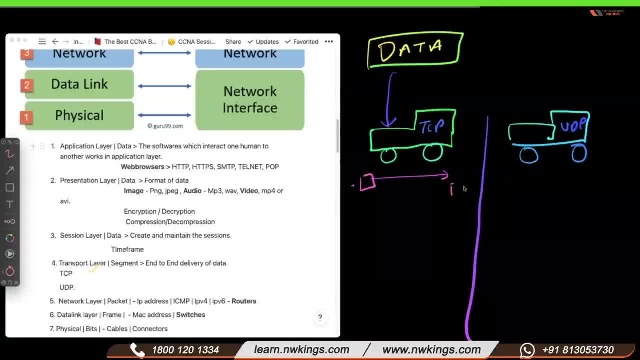 whenever so this, whenever so this, any packet is going from source to any packet is going from source to. any packet is going from source to destination. so the destination is going destination. so the destination is going destination. so the destination is going to send, to send, to send us back a receipt that is known as. 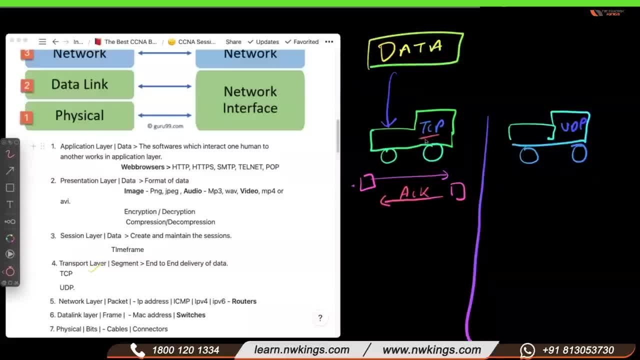 us back a receipt that is known as us back. a receipt that is known as acknowledgement means if the data is acknowledgement means if the data is acknowledgement means if the data is going with this, going with this, going with this guy. okay, it is going to take or it is. 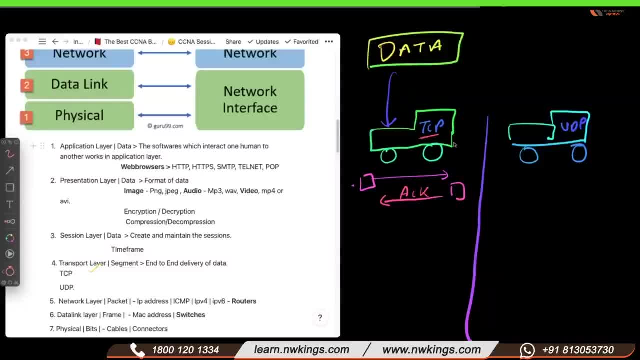 guy, okay, it is going to take. or it is guy, okay, it is going to take, or it is going, going, going, uh, and coming back with the receipt, uh, and coming back with the receipt, uh, and coming back with the receipt that i have delivered the data, that i have delivered the data. 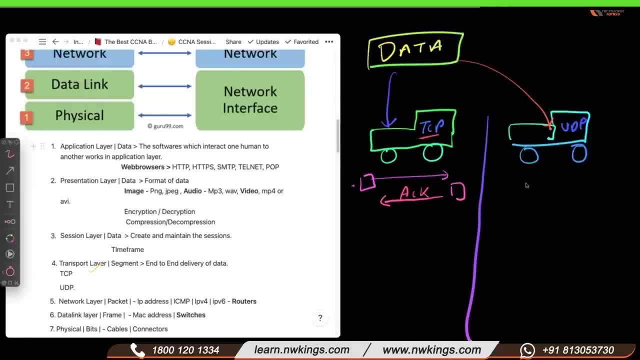 that i have delivered the data. but when data is going with this, but when data is going with this, but when data is going with this with the udp, we are just sending the with the udp, we are just sending the with the udp, we are just sending the data, but we are not going to. 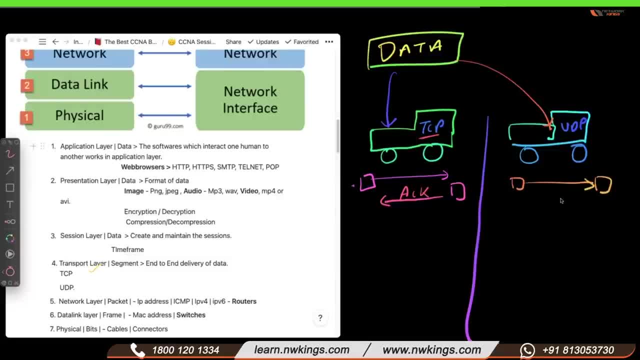 data. but we are not going to data, but we are not going to get back the receipt of whatever we are. get back the receipt of whatever we are. get back the receipt of whatever we are sending. so it means whenever we sending. so it means whenever we sending. so it means whenever we send data with the tcp. so tcp stands for. 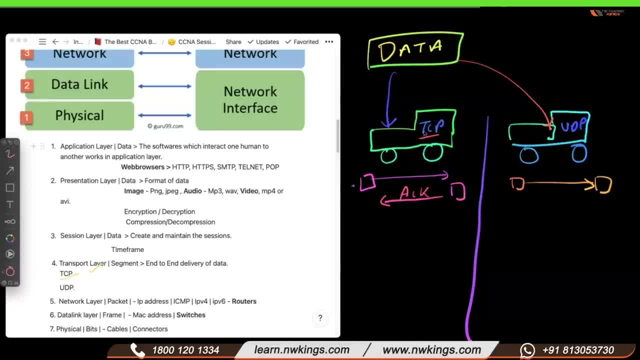 send data with the tcp. so tcp stands for send data with the tcp. so tcp stands for trans trans, trans mission control protocol, transmission mission control protocol, transmission mission control protocol, transmission control protocol. and udp stands for user control protocol. and udp stands for user control protocol and udp stands for user datagram protocol. 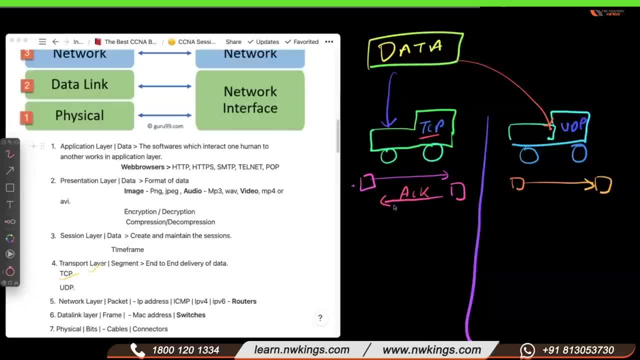 datagram protocol. datagram protocol, so whenever data is going with tcp, so whenever data is going with tcp, so whenever data is going with tcp, so it actually takes care of, so it actually takes care of, so it actually takes care of acknowledgements. so tell me if anybody 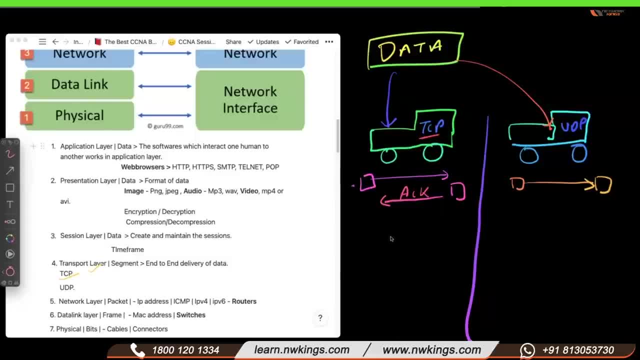 acknowledgements, so tell me. if anybody acknowledgements, so tell me. if anybody is coming with the receipt is coming with the receipt, is coming with the receipt. who is more reliable, tcp or udp? who is more reliable, tcp or udp? who is more reliable tcp or udp data? so this is reliable where this? 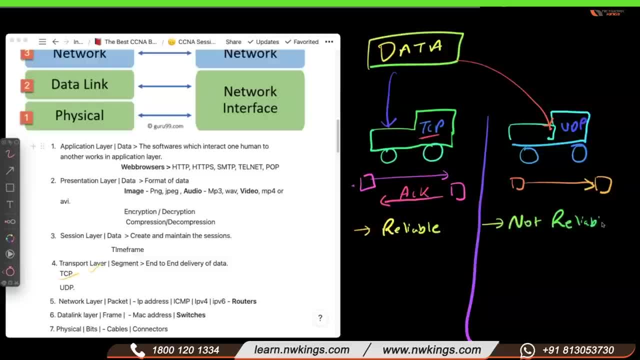 data, so this is reliable where this data, so this is reliable. where this person or this person or this person or this dudp truck is not reliable. right, and if data is, and if data is and if data is lost, if suppose we are sending data one lost, if suppose we are sending data one, 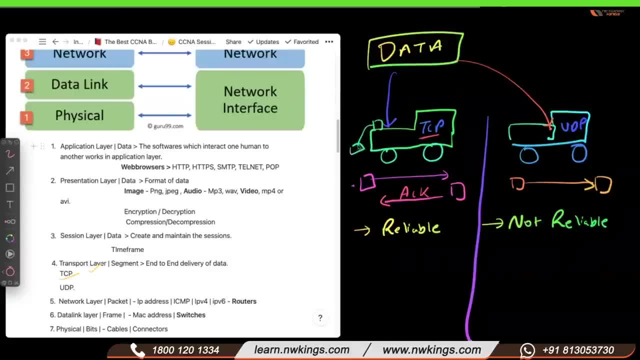 lost. if suppose we are sending data one box dropped box, dropped box dropped somewhere in the road or somewhere, so somewhere in the road or somewhere. so somewhere in the road or somewhere. so the vendor is actually take or count the. the vendor is actually take or count the. 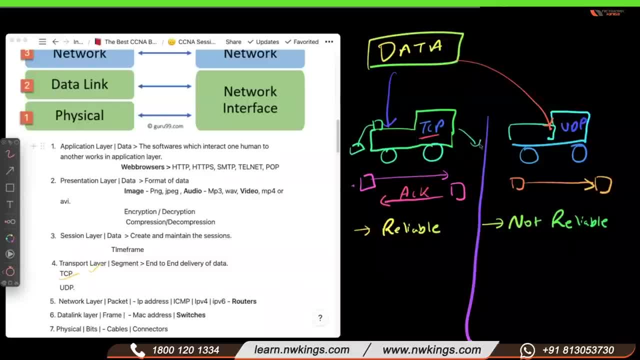 the vendor is actually take or count the boxes. how many boxes we got boxes? how many boxes we got boxes, how many boxes we got right? and it actually says oh right. and it actually says oh right. and it actually says oh, please send me one box again, or maybe. 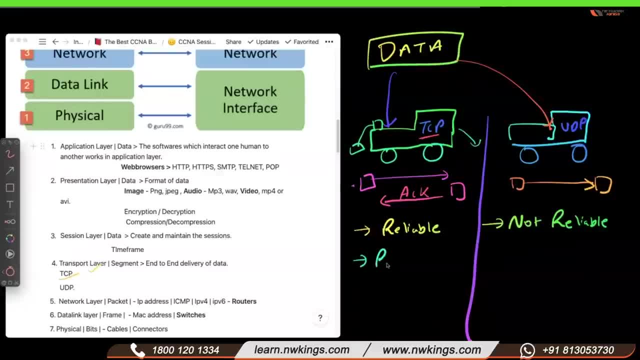 please send me one box again. or maybe please send me one box again. or maybe the box is broken or something, so it is the box is broken or something. so it is the box is broken or something. so it is going to retransmit the data, going to retransmit the data. 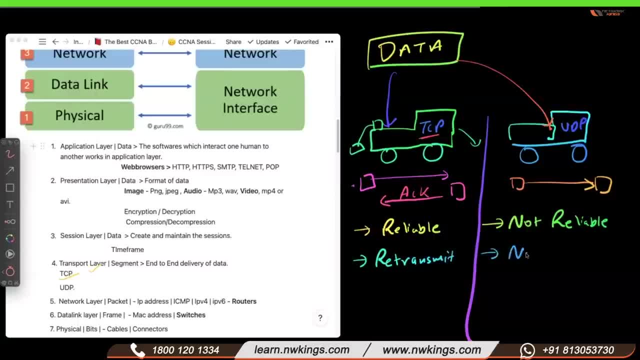 going to retransmit the data, so we don't have any retransmission. so we don't have any retransmission, so we don't have any retransmission over here, over here, over here, no retransmission, no retransmission, no retransmission. so 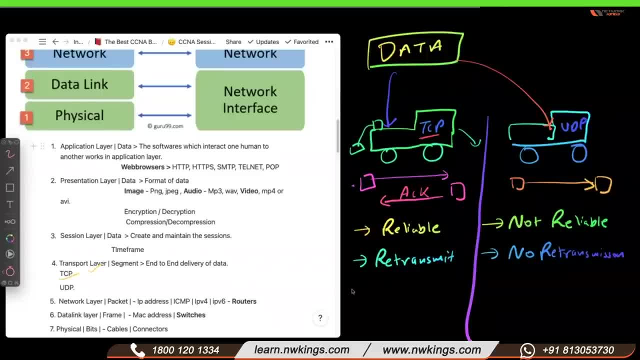 so. so if data is dropped or discarded, or anything is dropped or discarded, or anything is dropped or discarded or anything happened with the data, it is going to happened with the data. it is going to happened with the data, it is going to retransmit the data. 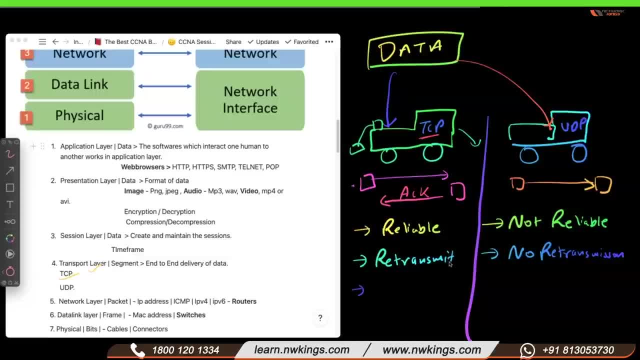 retransmit the data. retransmit the data. yeah, yeah, yeah, so this is known as. so this is known as: so. this is known as. it always believes in connection, it always believes in connection, it always believes in connection. so this is so, this is so. this is in network language, it is known as: 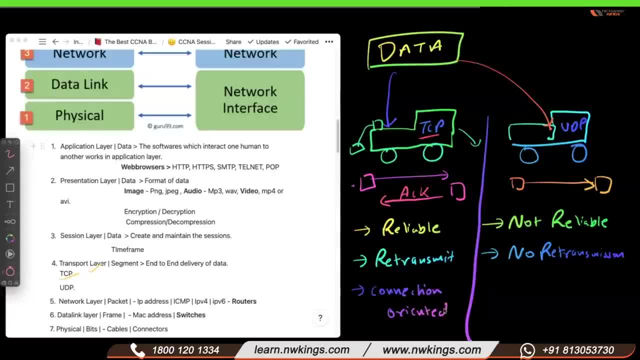 in network language it is known as: in network language it is known as connection oriented, connection oriented, connection oriented, because it always believes in making, because it always believes in making, because it always believes in making connection. but this is connectionless, right so udp, right so udp, right so udp. so there is a term called fast in udp. 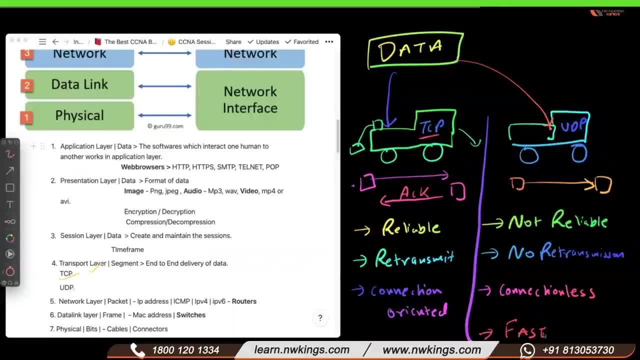 so there is a term called fast in udp. so there is a term called fast in udp. but nowadays our internet history, but nowadays our internet history, but nowadays our internet history is super fast, is super fast, is super fast. so we don't have to say that tcp slow or 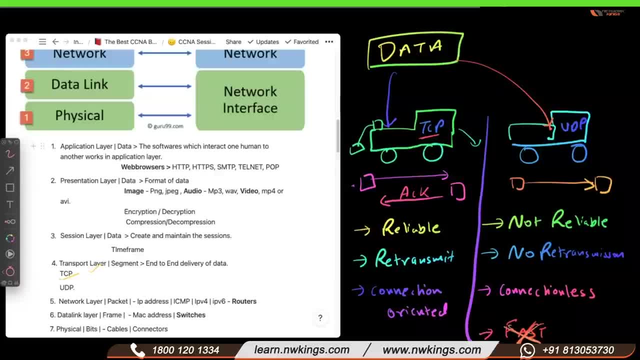 so we don't have to say that tcp slow, or so we don't have to say that tcp slow or fast or something, so you, you can skip fast or something. so you, you can skip fast or something. so you, you can skip this line, this line, this line. it looks like very childish if we speak. 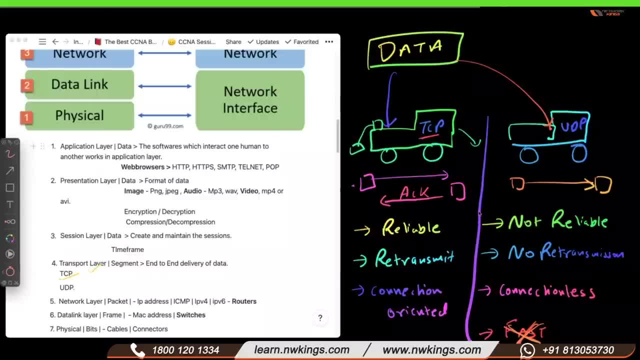 it looks like very childish if we speak. it looks like very childish if we speak like this is fast or slow like that, like this is fast or slow, like that, like this is fast or slow like that, because, because, because, now, yes, you can say yes, correct. now, yes, you can say yes, correct. 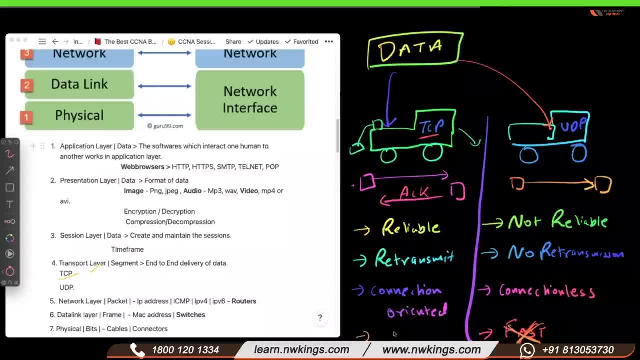 now, yes, you can say yes, correct, so, so, so, so you can say so. so, uh, like one guy sharath has given a. uh, like one guy sharath has given a. uh, like one guy sharath has given a. we don't actually send a lot of many. 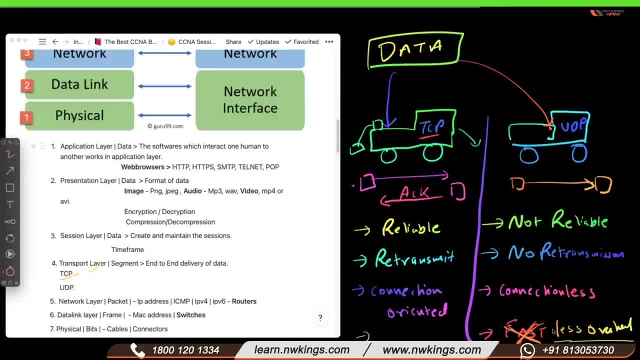 we don't actually send a lot of many, we don't actually send a lot of many things. so it means things, so it means things. so it means: uh, there will be less size of the packet. uh, there will be less size of the packet. uh, there will be less size of the packet in comparison to tcp. 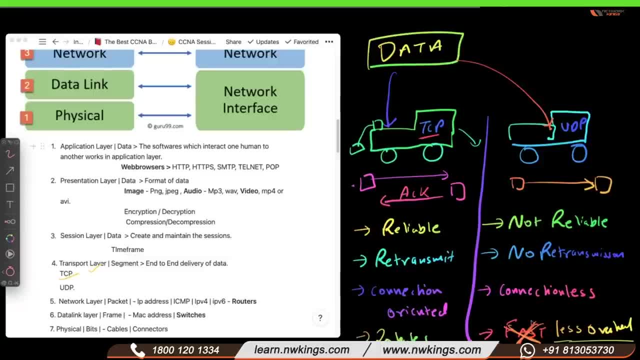 in comparison to tcp, in comparison to tcp. so tcp takes 20 bytes, so tcp takes 20 bytes. so tcp takes 20 bytes. and udp takes how many bytes? i think eight. and udp takes how many bytes? i think eight. and udp takes how many bytes? i think eight. right. 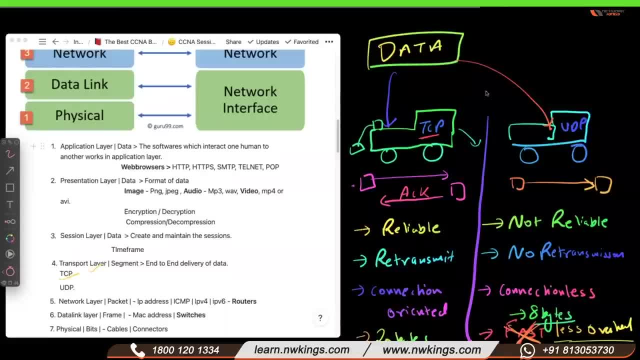 right, right, eight bytes. so any data, any small box or any packet. so any data, any small box or any packet. so any data, any small box or any packet going with udp. it is going to take going with udp. it is going to take going with udp. it is going to take eight bytes. 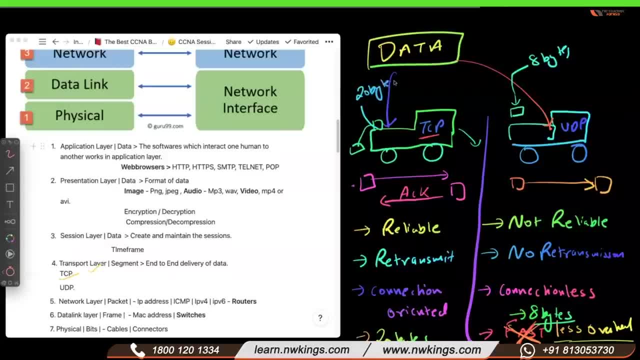 eight bytes, eight bytes. and in tcp we are going to take on every and in tcp we are going to take on every and in tcp we are going to take on every packet. i am going to packet, i am going to packet, i am going to place my address. that is 20 bytes. 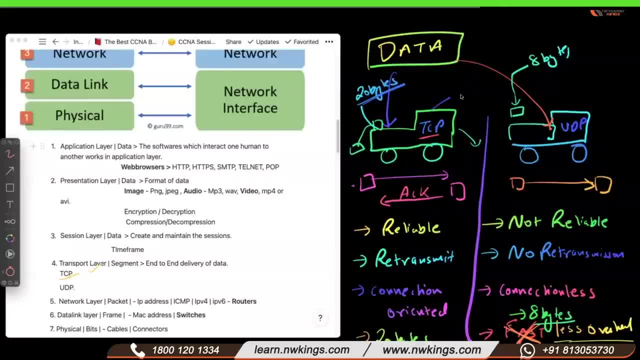 yeah, so tcp. uh, there is a protocol number. yeah, so tcp. uh, there is a protocol number. yeah, so tcp. uh, there is a protocol number to it. tcp protocol number is six to it. tcp protocol number is six to it. tcp protocol number is six because this, these both protocols, falls. 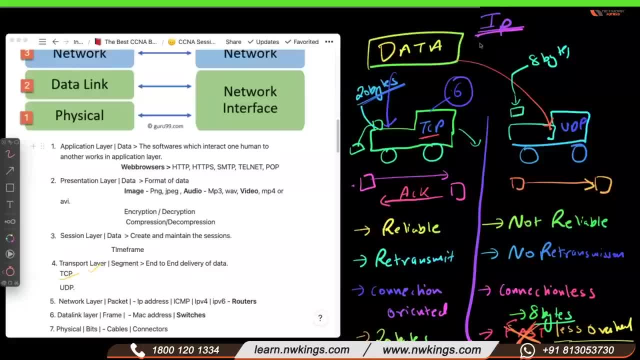 because this, these both protocols falls, because this, these both protocols falls under ip, under ip, under ip, so ip is the biggest or main protocol. so so ip is the biggest or main protocol. so so ip is the biggest or main protocol. so i tcp works under ip and the protocol. 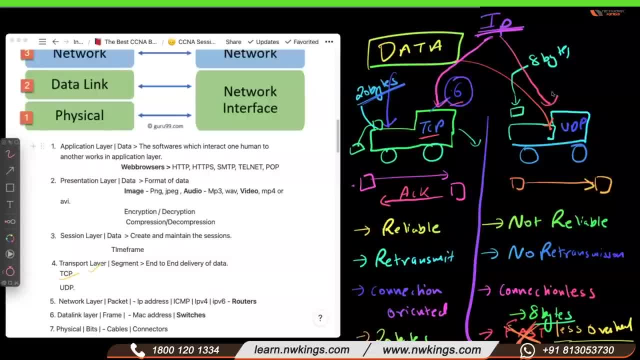 i tcp works under ip and the protocol i tcp works under ip and the protocol number is six, number is six, number is six and udp works also under ip. that protocol and udp works also under ip. that protocol and udp works also under ip. that protocol number is 17.. 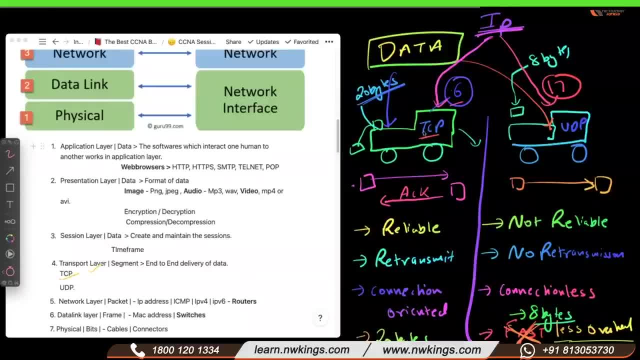 again. repeat okay, so see in again. repeat okay, so see in again. repeat okay, so see. in transport layer we have two protocols: tcp transport layer. we have two protocols: tcp transport layer. we have two protocols: tcp and udp and udp and udp. so whenever we send data from tcp, we 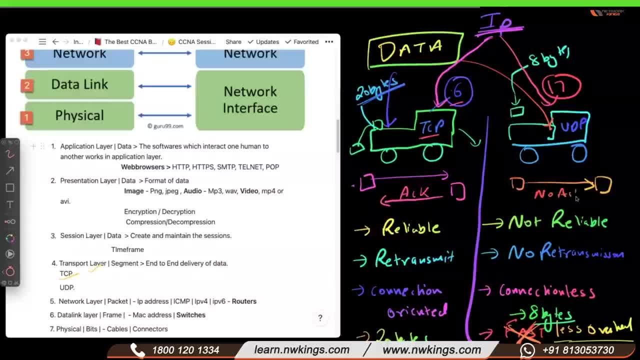 so whenever we send data from tcp, we so, whenever we send data from tcp- we always get acknowledgement, always get acknowledgement, always get acknowledgement. so this is the reason it is reliable, and so this is the reason it is reliable, and so this is the reason it is reliable and it is not reliable. 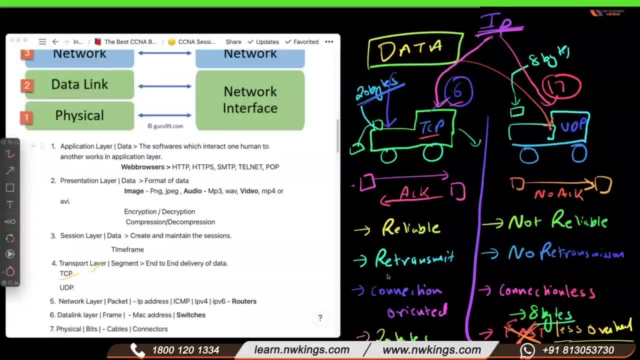 it is not reliable. it is not reliable. so whenever anything happens with any, so whenever anything happens with any, so whenever anything happens with any packet, it is going to retransmit it. packet, it is going to retransmit it. packet, it is going to retransmit it. and here we don't have retransmission. 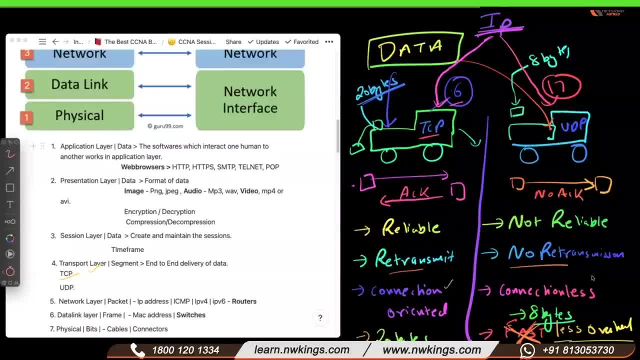 and here we don't have retransmission, and here we don't have retransmission. so this is the reason we also say that. so this is the reason we also say that. so this is the reason we also say that it is connection oriented, and this is. 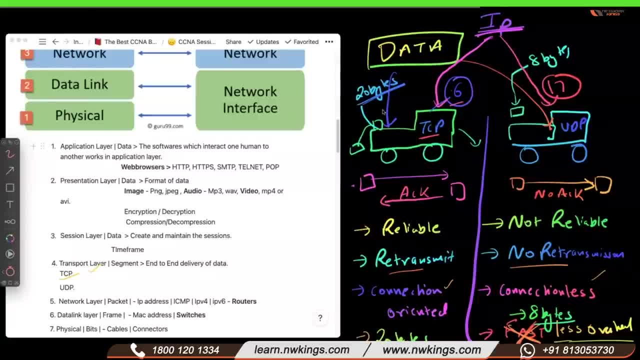 it is connection oriented and this is. it is connection oriented and this is connectionless, connectionless, connectionless. so tcp takes, so tcp takes. so tcp takes 20 bytes to add information and udp 20 bytes to add information and udp 20 bytes to add information and udp takes only 8 bytes to add the udp. 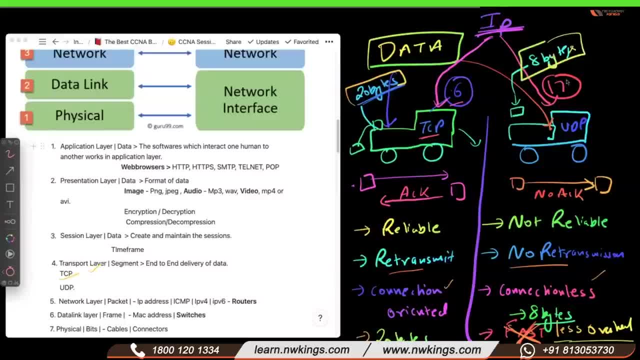 takes only 8 bytes to add the udp. takes only 8 bytes to add the udp. information, information, information. so what is that information that is port? so what is that information that is port? so what is that information that is port numbers? numbers, numbers. we add port numbers here. 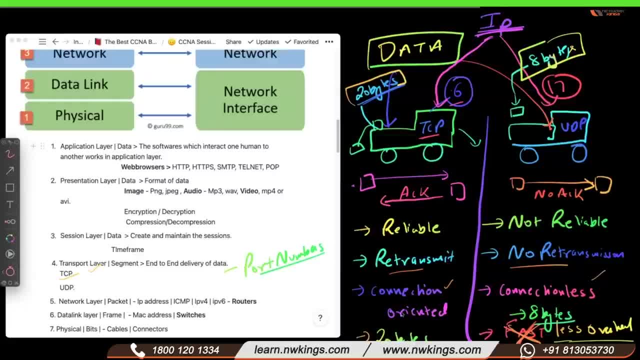 we add port numbers here. we add port numbers here. so the bytes: i am talking here 20 bytes. so the bytes: i am talking here 20 bytes. so the bytes: i am talking here 20 bytes, 8 bytes. it actually adds 8 bytes. it actually adds. 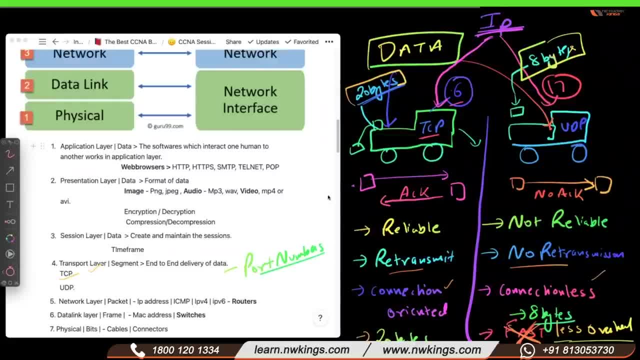 8 bytes. it actually adds port numbers, port numbers, port numbers. okay. so suppose you are sending data. okay, so suppose you are sending data. okay, so suppose you are sending data from your computer, from your computer, from your computer. so computer, a computer is going to add. so computer, a computer is going to add. 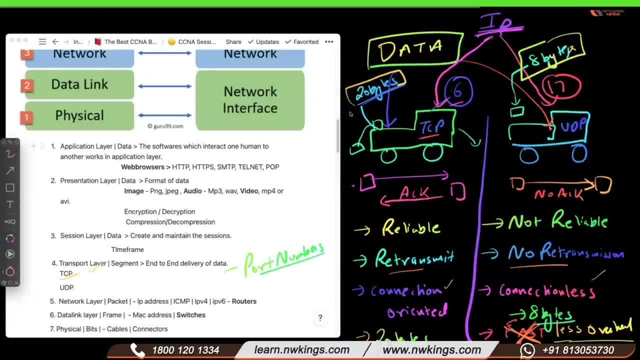 so, computer, a computer is going to add one port, one port, one port and destination port will be like you and destination port will be like you and destination port will be like you are going to https and all are going to https and all are going to https and all. so it is going to add the port number. so 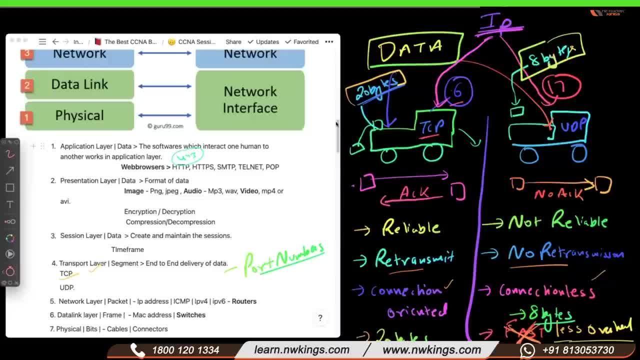 so it is going to add the port number. so, so it is going to add the port number. so we will discuss this, we will discuss this. we will discuss this also. so just understand this in transport also. so just understand this in transport also. so just understand this in transport layer right now. 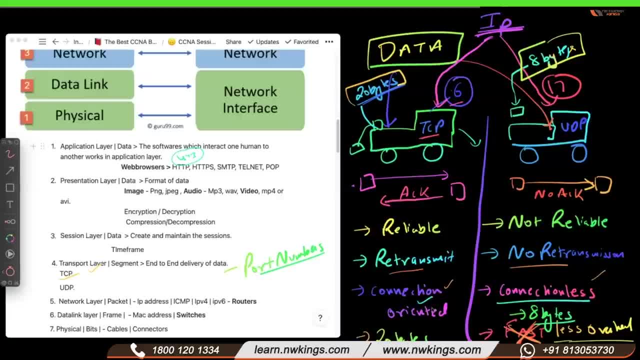 so connection less means connection. so connection less means connection. so connection less means connection. oriented means: it all believes in oriented means. it all believes in oriented means, it all believes in connection making, connection making, connection making. it is going to retransmit it and it it is going to retransmit it and it. 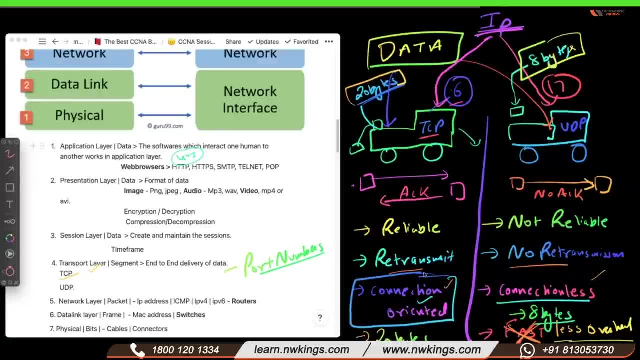 it is going to retransmit it. and it always means connection oriented means always means connection oriented means always means connection oriented means it always believes in making connections, it always believes in making connections, it always believes in making connections. connectionless means if anything happens. connectionless means if anything happens. 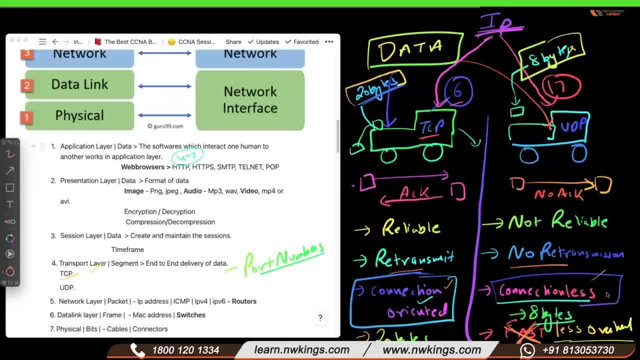 connectionless means: if anything happens, or packet has dropped, we are not going to, or packet has dropped, we are not going to. or packet has dropped, we are not going to. retransmit and all retransmit and all retransmit and all. so this is the reason you can say that 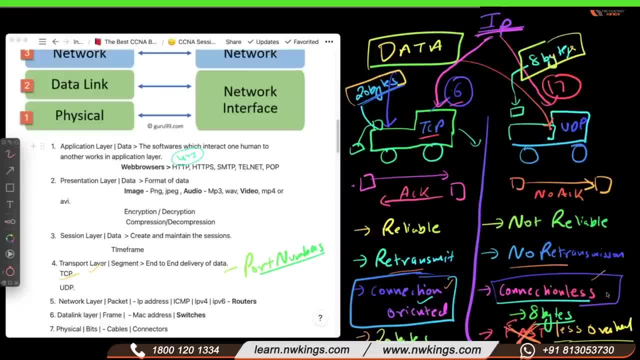 so this is the reason you can say that. so this is the reason you can say that it's connectionless, it's connectionless, it's connectionless. yeah, not trusted. yeah, so we don't. yeah, not trusted. yeah, so we don't. yeah, not trusted, yeah, so we don't. this is not reliable or not trustworthy. 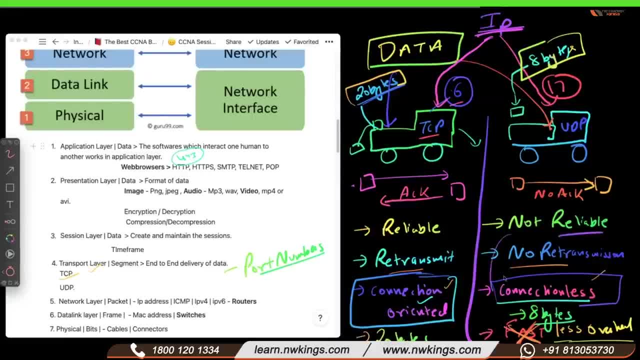 this is not reliable or not trustworthy. this is not reliable or not trustworthy. connectionless, connectionless, connectionless- it's just a synonym of this. you can say: it's just a synonym of this. you can say: it's just a synonym of this. you can say: they. 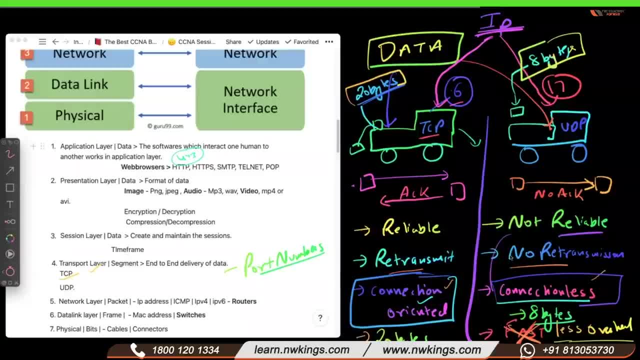 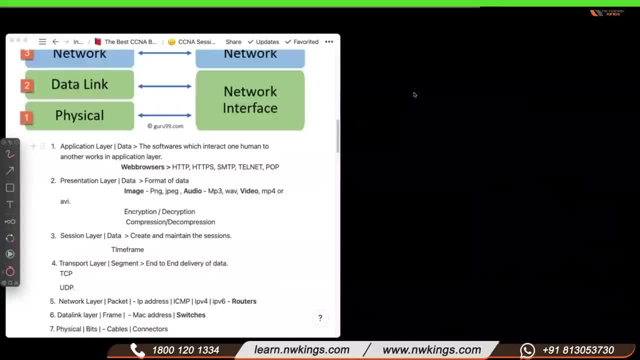 they, they, reliable. okay, so what we have learned so far? okay, so what we have learned so far, okay, so what we have learned so far, the data, the data, the data is coming is coming, is coming, and data is coming to transport layer and data is coming to transport layer. 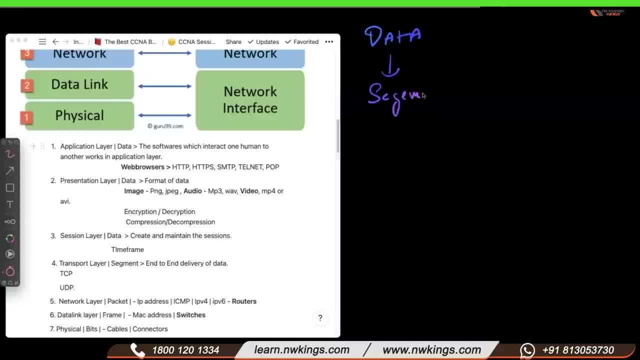 and data is coming to transport layer. transport layer is transport layer. is transport layer is actually converting those into, actually converting those into actually converting those into segments, segments, segments, right, right, right. so which layer is converting transport? so which layer is converting transport? so which layer is converting transport layer? 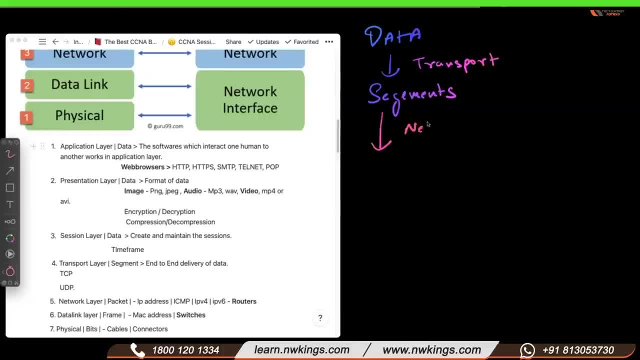 layer layer: okay, so now the data is moving to which. okay, so now the data is moving to which. okay, so now the data is moving to which layer layer layer, network layer. so now segments is actually converting into packet. means converting into packet means converting into packet means the data. 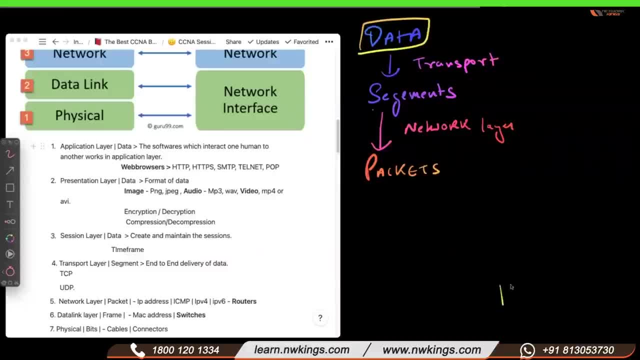 the data. the data is here, it's like a gift trap. you can say: is here, it's like a gift trap. you can say: the data is here, it's like a gift trap. you can say: that data is here, so on top of it. that data is here, so on top of it. 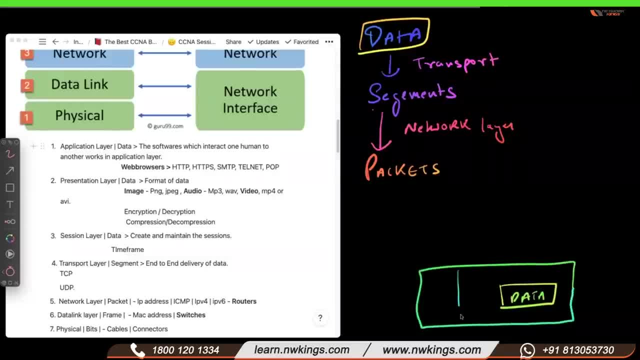 that data is here, so on top of it we are going to add extra header. that is like we are going to add extra header. that is like we are going to add extra header. that is like source port number, port number: okay. source port number, port number, okay. 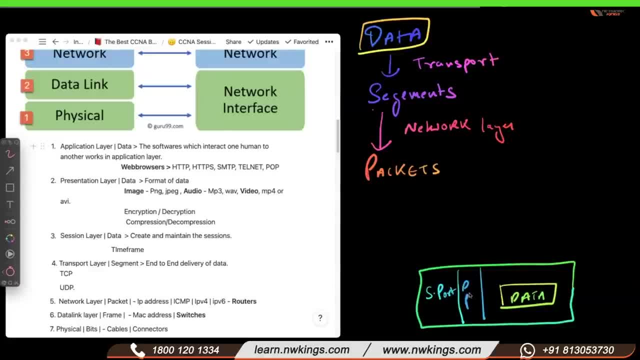 source port number, port number. okay, source port number, destination port number. source port number, destination port number. source port number, destination port number. and this hole is known as segment and this hole is known as segment and this hole is known as segment, so that is known as encapsulation also. so 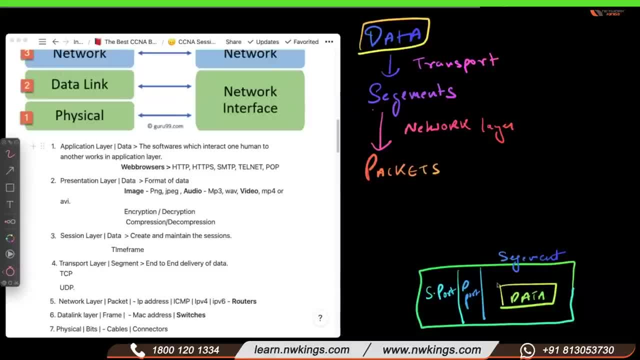 so that is known as encapsulation also. so, so that is known as encapsulation also. so whenever you add something, that is, whenever you add something that is encapsulation, or whenever you remove something, that is a decapsulation- okay, so data is actually going inside a segment and now on top of it, we are going to add extra few things. that is known as 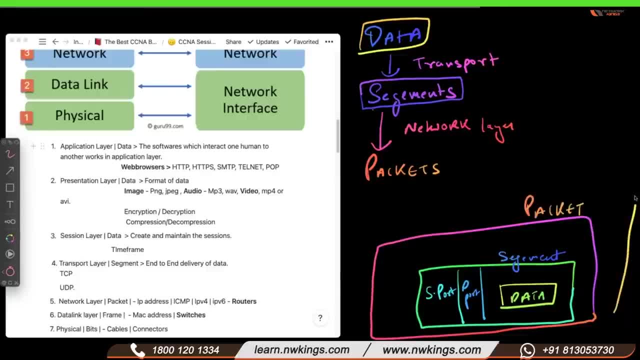 now packet, on top of it we will have another thing that will be known as frame. okay, so packet will have source ip, destination ip, and frame will have source mac address, destination mac address. there are a lot of okay, okay, so i'll explain in more appropriate way. so i'm just giving you idea. 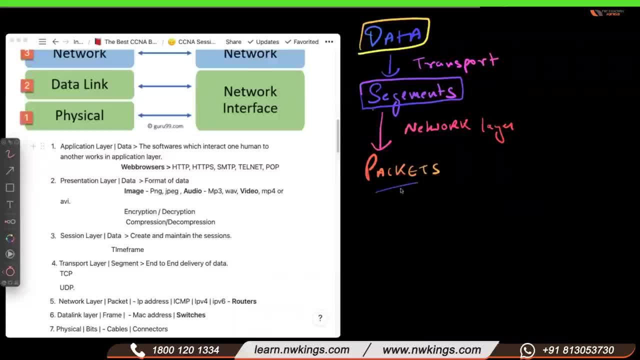 yeah, so packets. so in network layer all your routers and all your packets will have source ip, destination ip and frame will have source mac address. all works under this network layer and packets actually adds the source ip and destination ip. so whenever we talk about the ip address, this segment actually adds the port numbers. 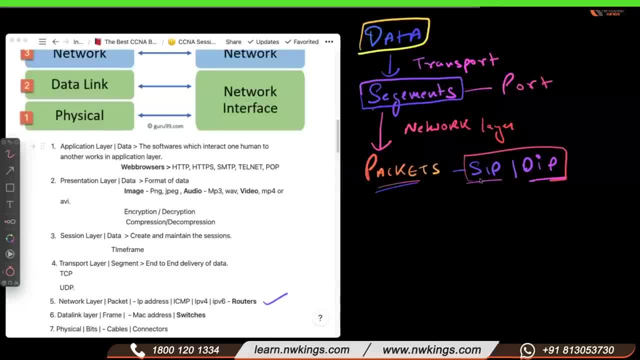 and packets, we add the source ip, destination ip. end-to-end delivery means it is going to take care of all the responsibility of sending data from source to destination, because the transport layer is going to take care of all the responsibility of sending data from source to destination. 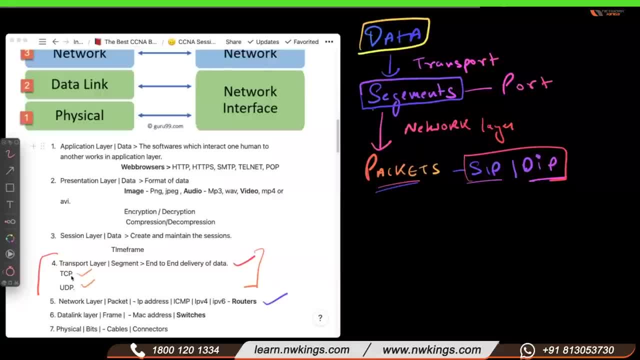 is choosing which protocol is going to carry forward your data. so this is the reason we have written here: end-to-end delivery of data. okay, so packets is now moving to another layer, that is, packets are going to convert into frame and this. which layer is doing this data link layer. 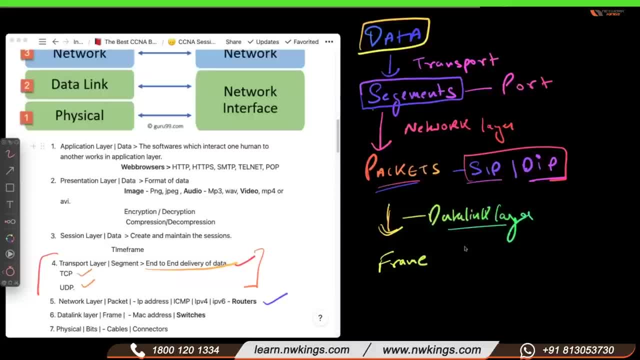 so data link layer or like in network layer, your routers works here and switches works on this layer. okay, and frame is actually adding what information? like? in segments we have port number, in packets we have source ip, destination ip, and in the frame we have source mac address and destination mac address. okay, and all your frame is now going to convert. 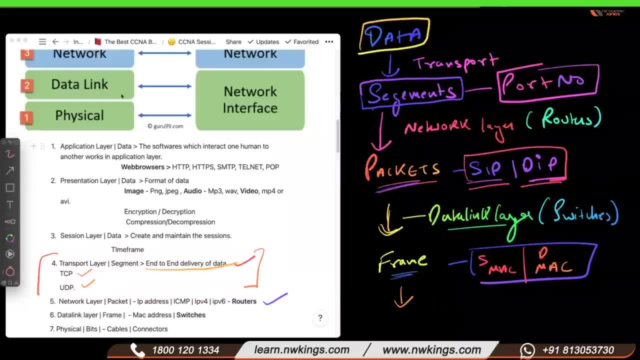 into signals because your computer is going to send data right. so all data is going from top to bottom. so now just see from. this is a computer, just understand this is a computer. now. physical layer means your nic card is going to convert into zero and form. that is. 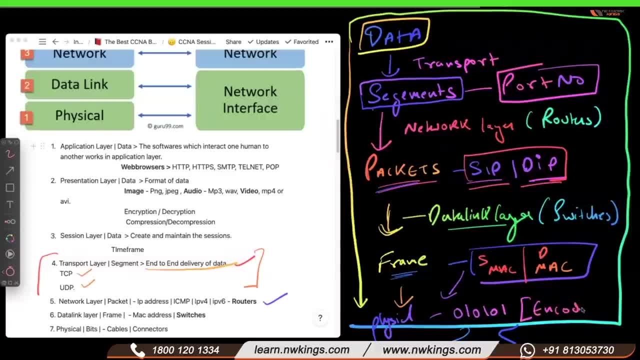 known as encoding. encoding means converting or encoding. decoding is converting the data into 01 format and converting them ión to signals, so that this computer is sending data to another computer. okay, so this whole process is known as encapsulation, and also the data is going over the cable now and whenever. the second device. 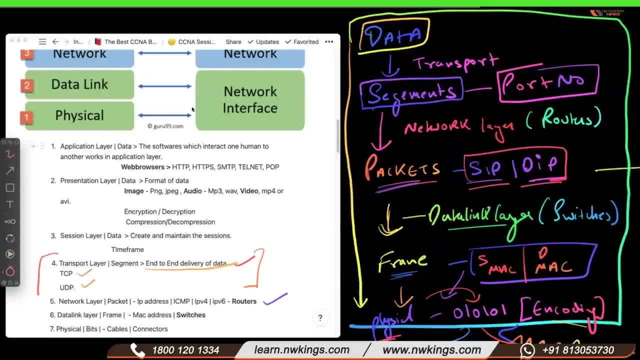 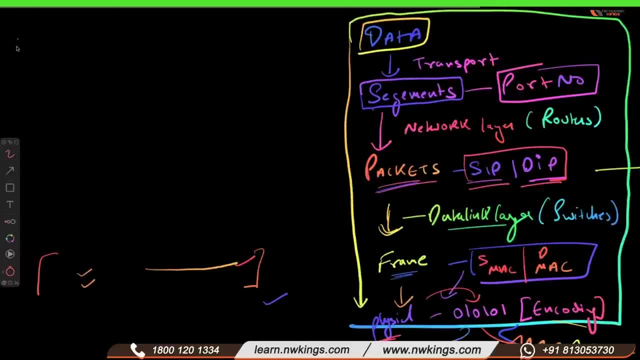 which is over here right side. you can't see, just understand or we can place here, just hold on. yeah, so now data is coming into another pc here. let's take example: so now data is going zero one form again. here we have physical layer, so we got zero ones. it is now physical. 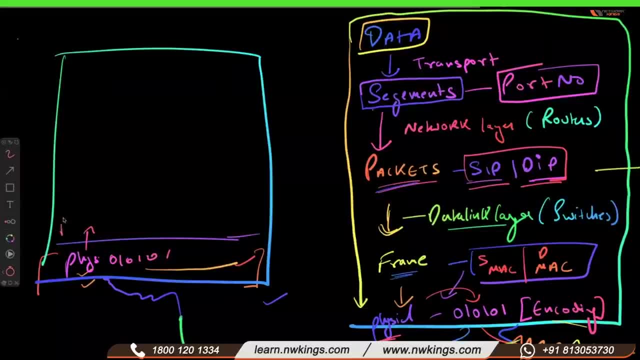 layer is giving data to data link layer. so data link layer is actually converting this into frame. it will check the mac address address information. okay, so computer will check its mac address. so this computer is suppose b, this is a. okay, so the when we open this frame we get what packet? so when we in 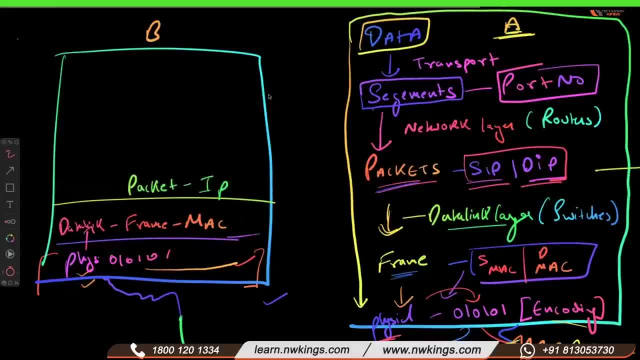 packet. we will check the ip address. so the packet is for my device or not. okay, if a device ip address or the packet ip address match with this computer address, it means this is this computer information or this packet came for this computer only. so packet when we open. 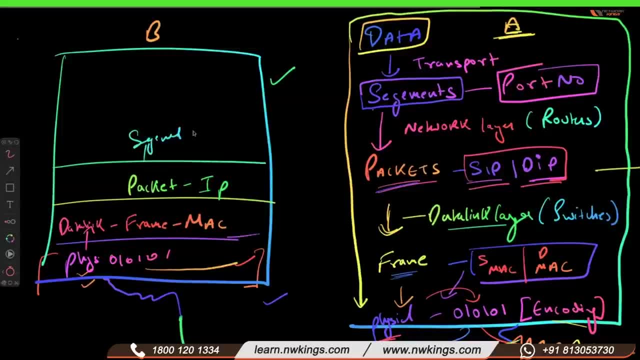 the packet, we will receive the segment in segment. we check the port number, which application this computer is trying to access, which application, and when we open the segment we get what data. so this is how it works. okay, cool, i'm not explaining in very complex way, i'm just trying to explain in a very layman language. 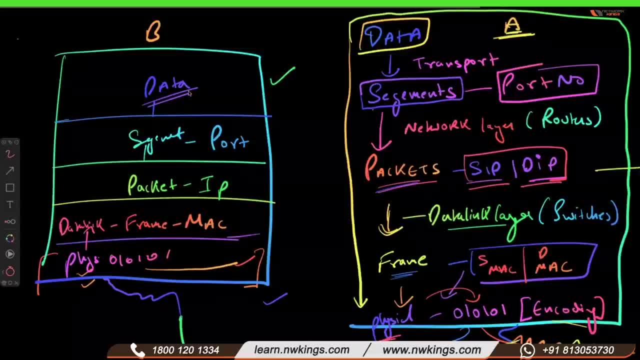 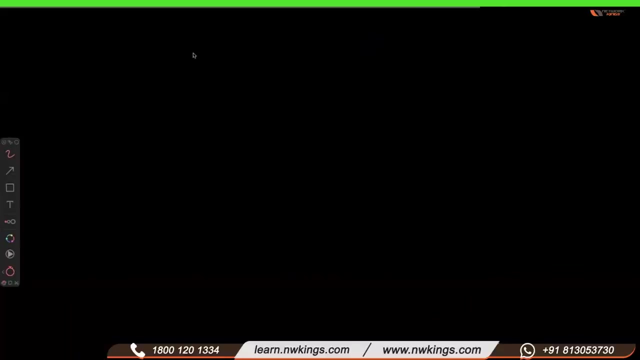 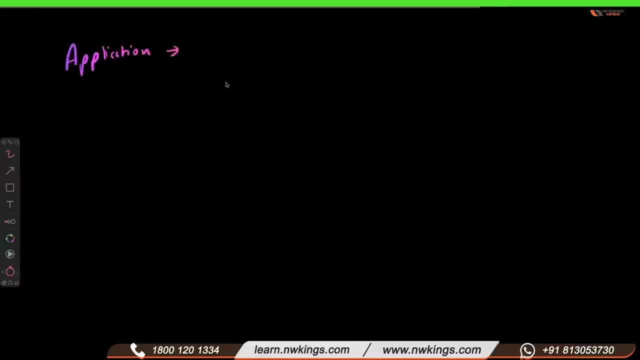 remember with the one human to another human, or you can remember with the keyword all applications, or like http user, it is the same as the one human to another human in the protocol, or if you are using the one human to another human and you want to refer to this, or if you want to use the one human or not. so 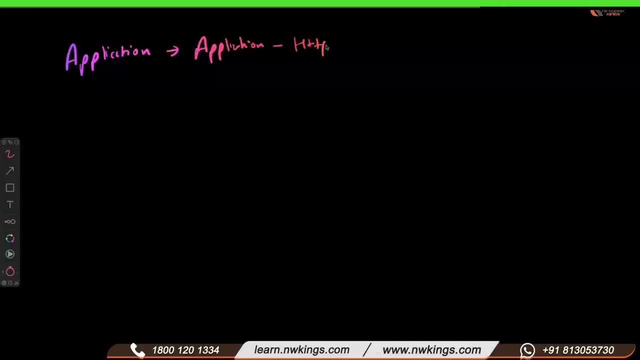 http, smtp. all comes under s this, okay, application software which help interact one human to another human. okay, very basic. so in presentation layer, what was the keyword? format of data? right, format of data. so when we talk about the like compression here, compression, decompression, encryption, decryption all falls under in this layer. so when we go, the data is going to session. 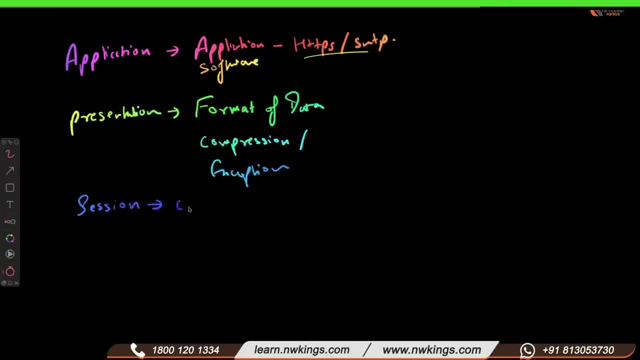 layer. so what is the responsibility of session layer? create and maintain the session. create and maintain the session, okay, okay. so when we talk about the format of data: right format of data. so when we talk about the format of data, right format of data, okay. and when data is going to transport layer. 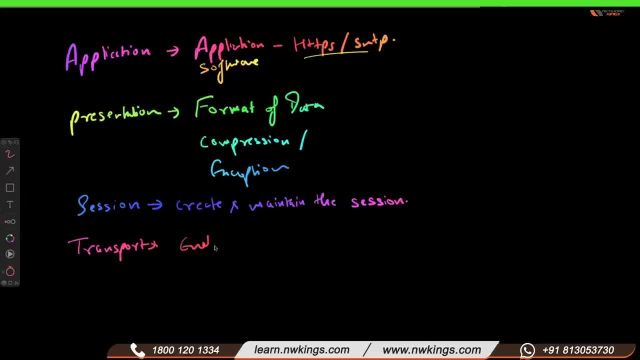 so transport layer is responsible for end-to-end delivery of data, means it is going to take care of all the delivery part. end-to-end delivery of data with the help of two protocols, tcp and udp, so where tcps always send acknowledgements, where udp does not send acknowledgements. 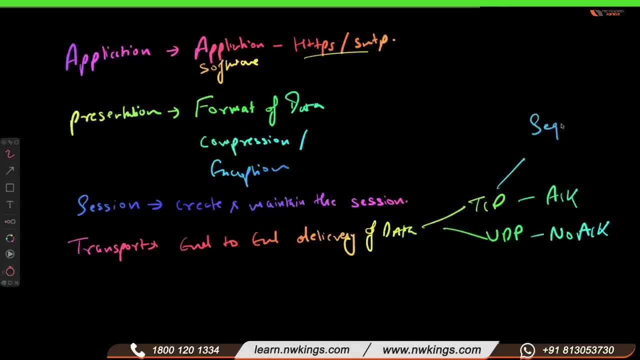 so tcp has a sequencing: okay, put down the number over the packet. okay, segmentation: divide the data into parts, retransmission, so all faults, all these work under transport and now the data is moving to. here the data is known as data, so now data is known as segment here, right, so now the data is moving to. 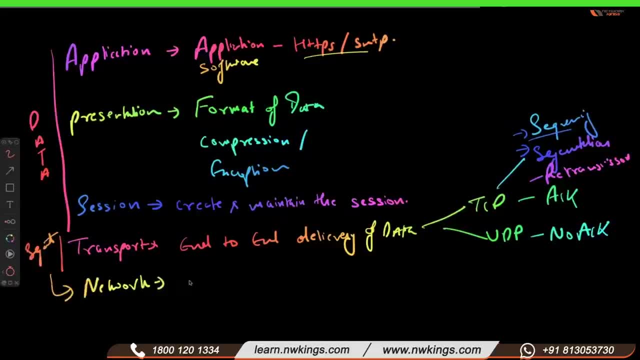 which layer, network layer. so where we are going to add what add? ip address. here we are going to ip address, so ip address, either it would be ip version 4 or ipv6. so network layer is going to add the ipv4 or ipv6 any any. 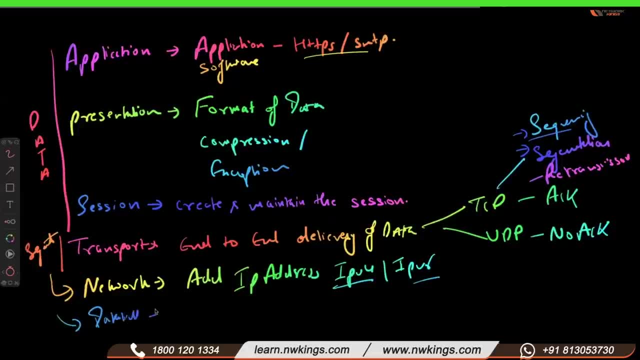 which you are using. so in data link layer we are going to add what? add mac address. so mac address means the chip hardware address of nic. okay, and the physical layer is actually converting your all data into zero one, zero one, zero one. so that is encoding, okay, clear. 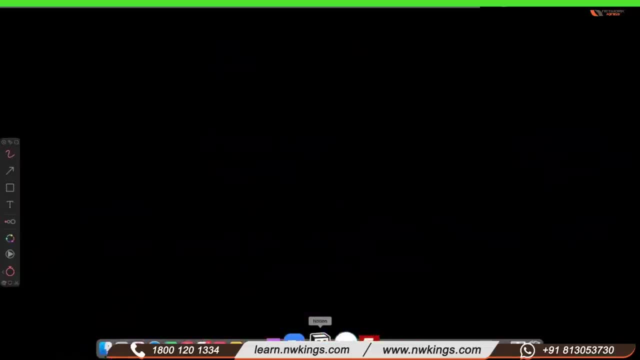 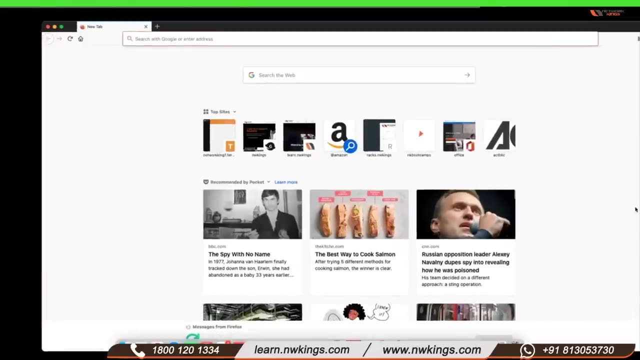 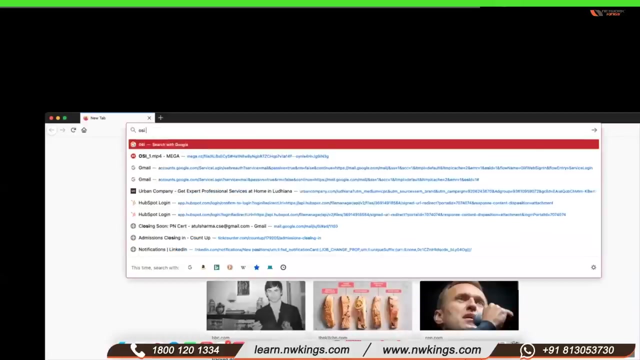 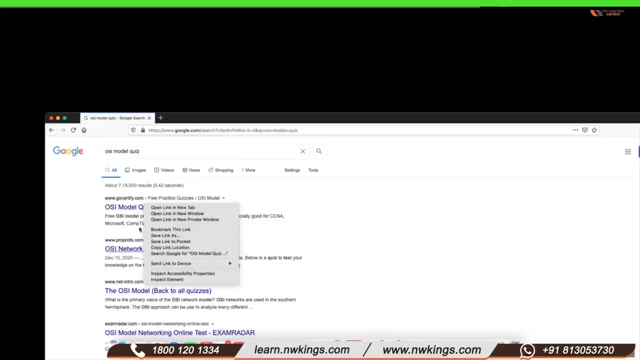 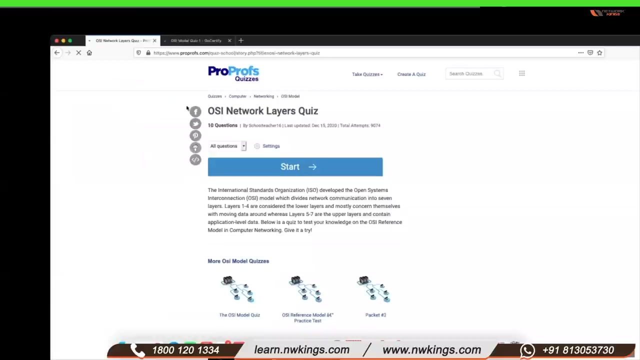 got some confidence or not? okay, so let's do a small quiz. osi model quiz- just check from over the internet. okay, so we can open this one. let's do a small quiz. so if you're a user, so if you're our client, you can see that we have two these types of support. 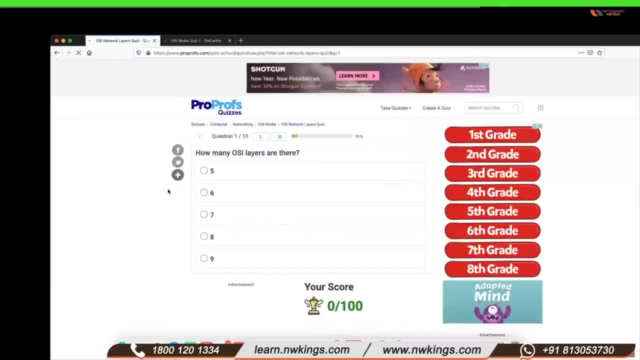 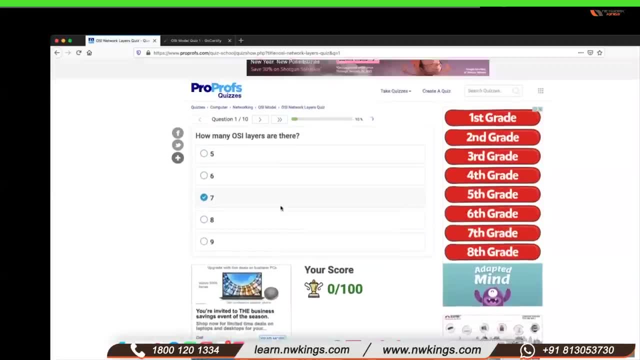 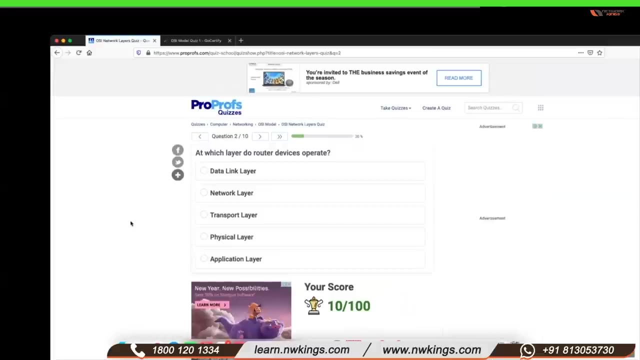 so if you want to let your client get our support from the site, the first option is to chilab app, and if you can wait until then, let's say our clients come to our site. perhaps you want us, for example, to now crack our service code because 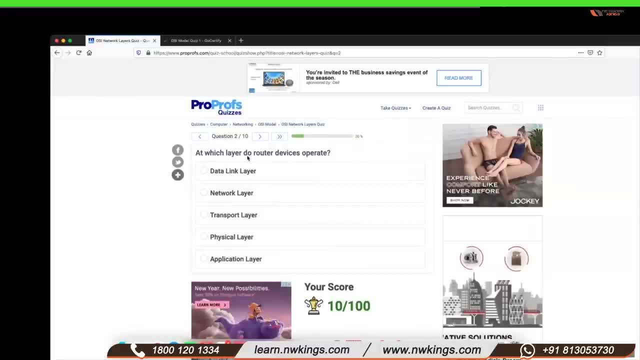 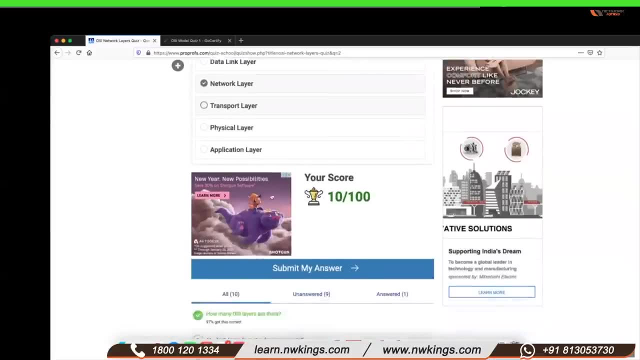 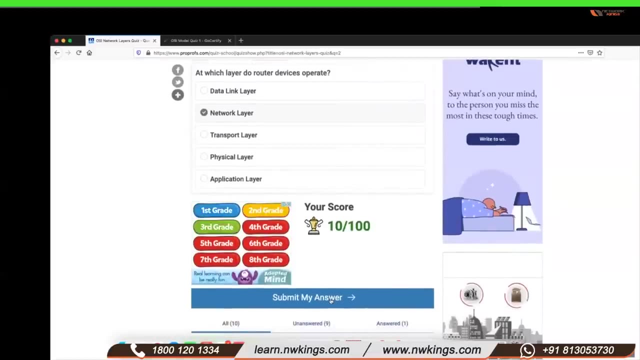 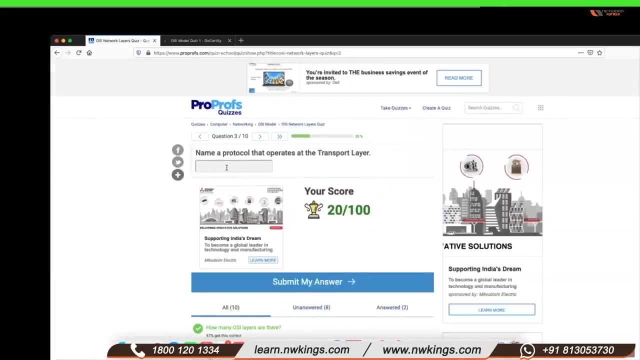 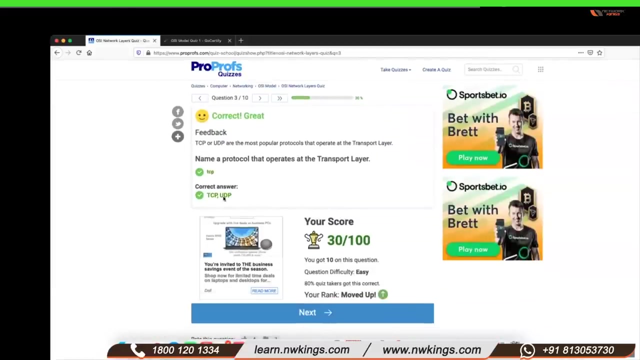 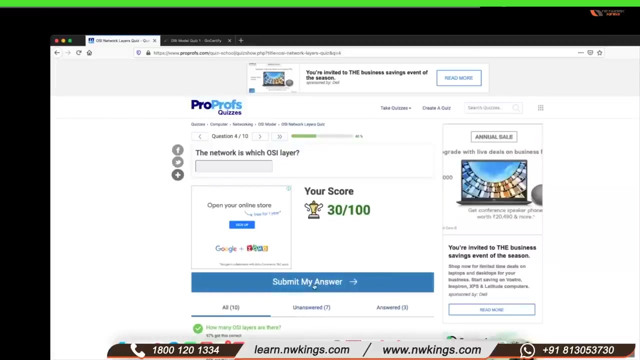 we cannot allow companies to tag between seven systems just like this. yes, ip address where we have ip address. yeah, network layer: okay, name a protocol that operates a transport layer. so i told you two protocols: tcp, so i'll write down tcp. yeah, so you can uh. so either you can write udp also, so both works under. 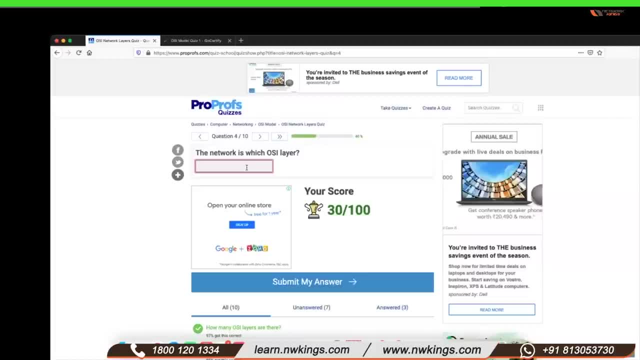 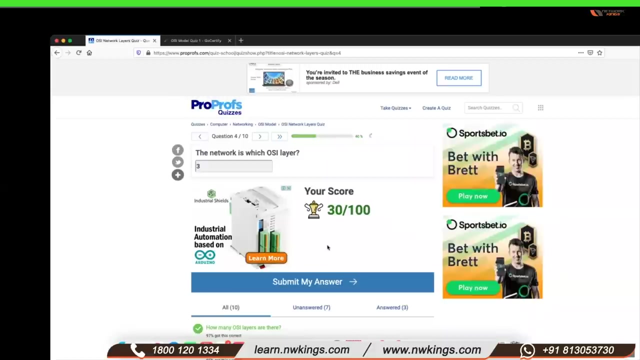 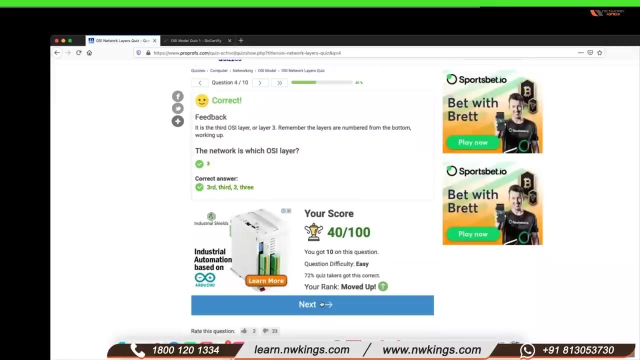 so the network is which osi layer network layer is known as which layer layer three. write three, third, or maybe just write down: let me write 3, hopefully it will be yeah, so you can write third, 3, 3 or third, something like that. ok, so which layer manages the? 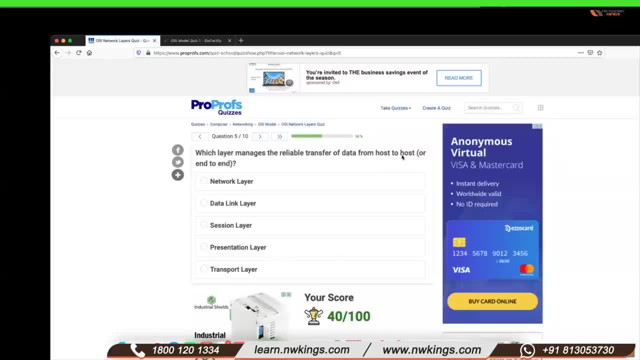 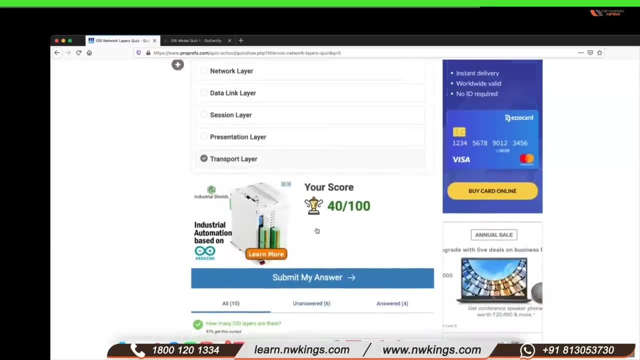 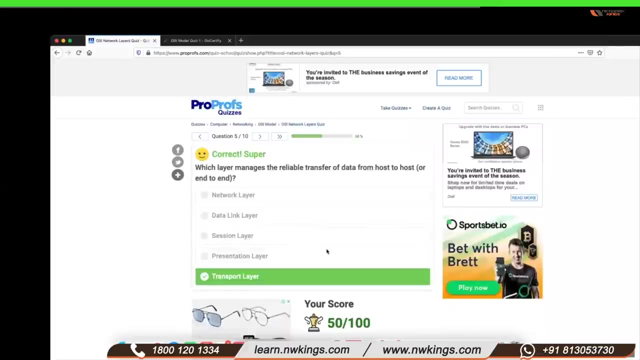 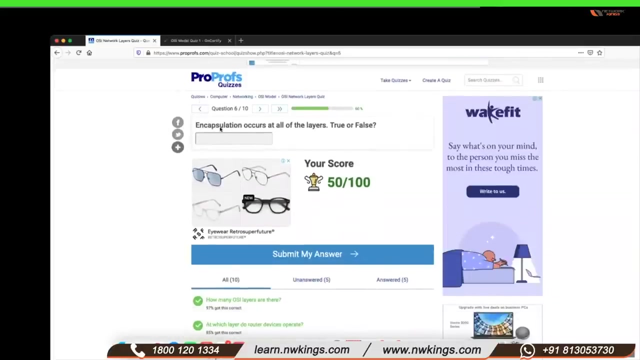 reliable transfer of data from host to host means end to end, which is actually taking care of delivery of data transport. we don't have option of TCP, so we have to choose transport, cool right. so tell me, really encapsulation. so tell me encapsulation. I told you encapsulation occurs at all layers, true or false. 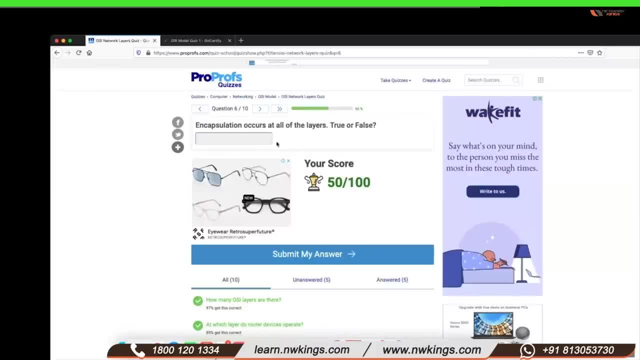 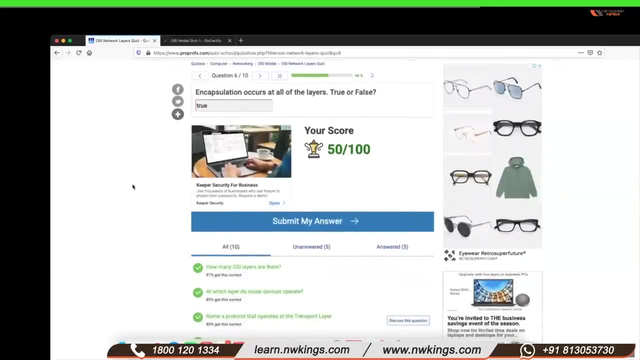 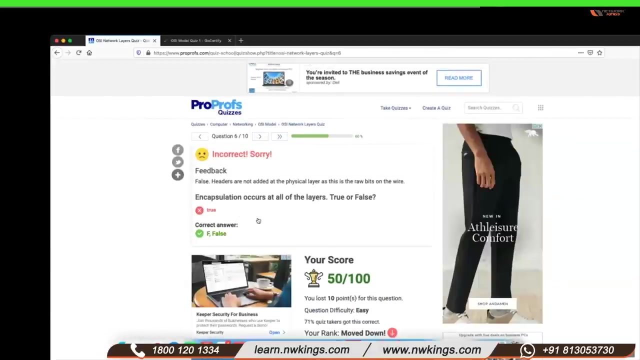 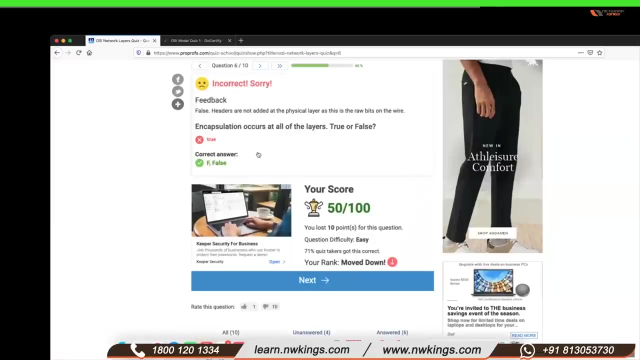 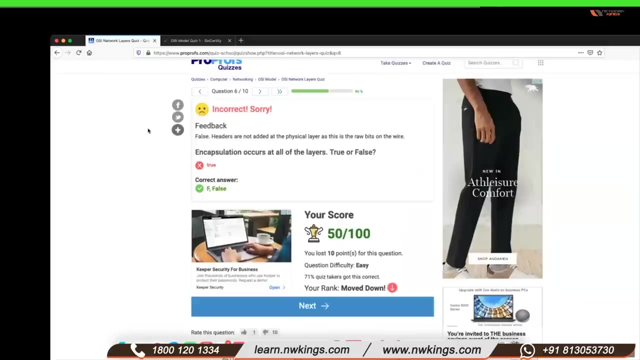 true or false? true, right, I told you that adding anything and every layer is adding something. oh, but we got false. why? because few layers I are actually not adding, because this question is regarding osa model and i told you: uh, in real world we have application, so maybe. so it's a tricky question. encapsulation actually occurs when we add port numbers, when we 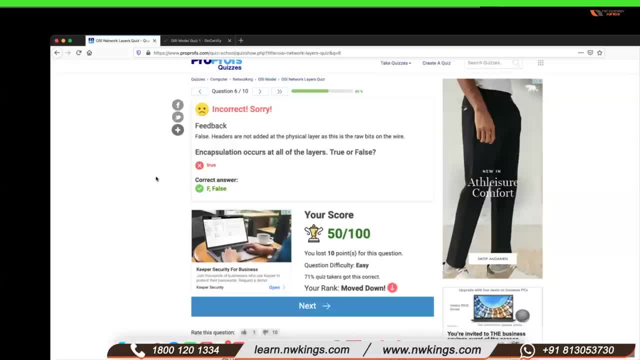 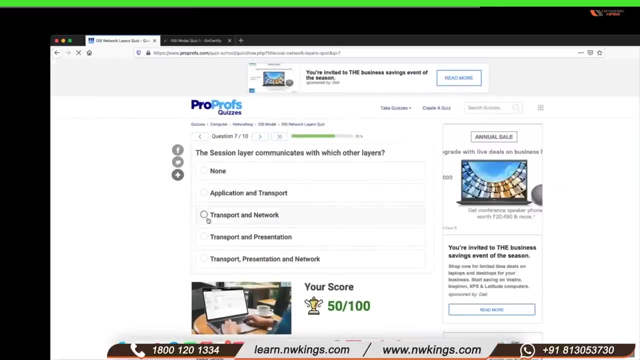 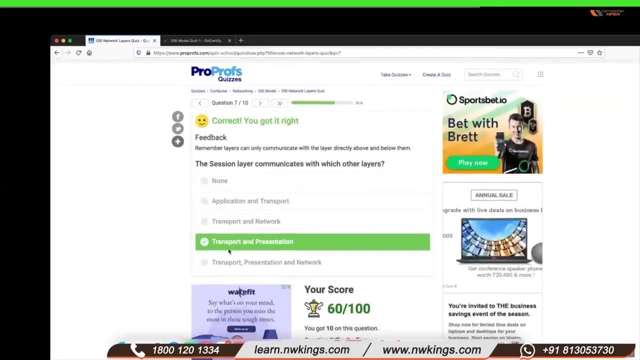 add ip address, mac address in, like physical network data and transport. okay, so the application layer is not adding something, so maybe this is the reason, but no issues. the session layer communicates with which other layers. so session layer is between which layer, transport and presentation. so i think this would be the answer. yeah, correct, so the session layer is between 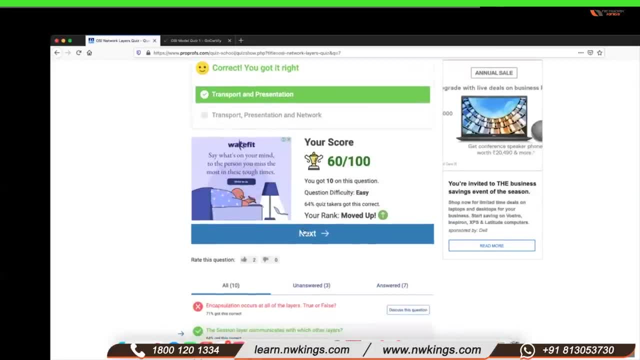 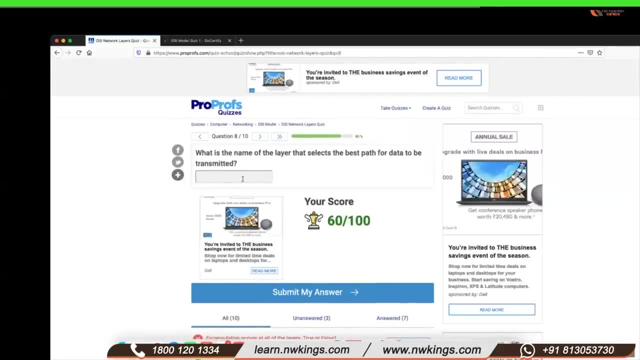 transport and presentation. so the question was like that, only so. what is the name of the layer that selects the best path for data to be transmitted? i think i have not explained. this means actually the device router actually selects the best path. so tell me which layer or which router works on which layer network. 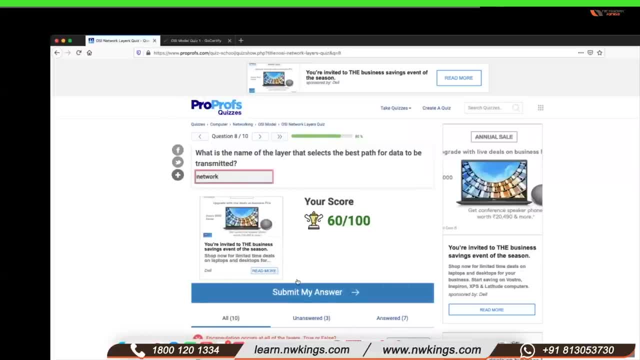 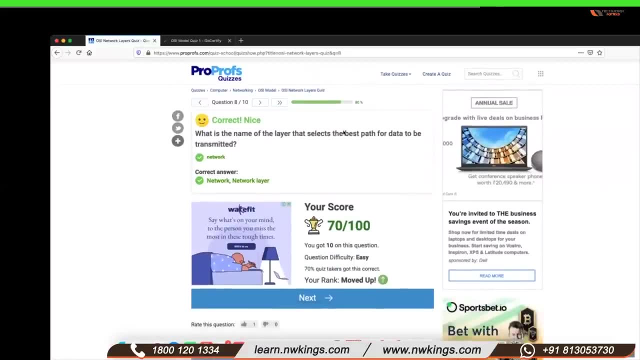 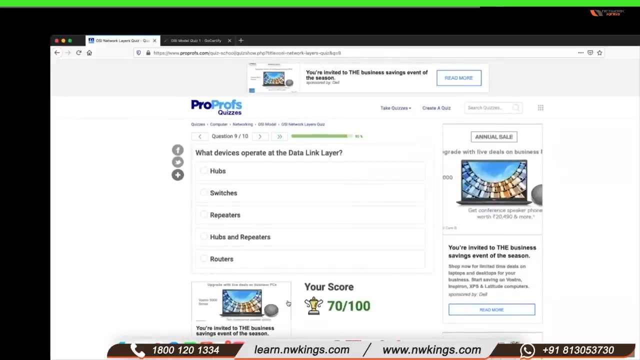 i think this would be the answer. okay, yeah, correct network. so router, actually, router chooses best path if you want to go to googlecom. right, sharmaji? what exactly you are saying? so data link layer works on which layer? okay, so which devices actually work on data link layer? 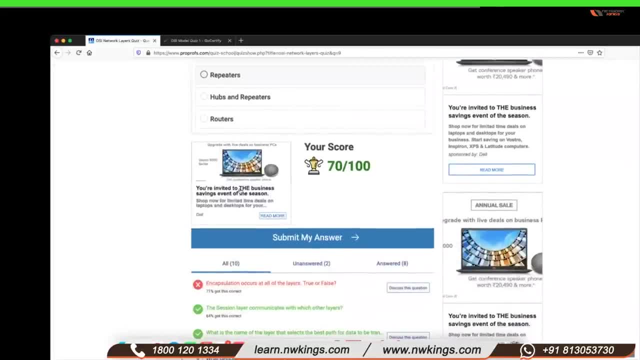 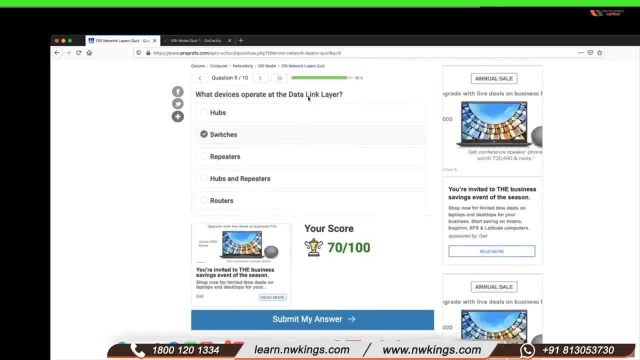 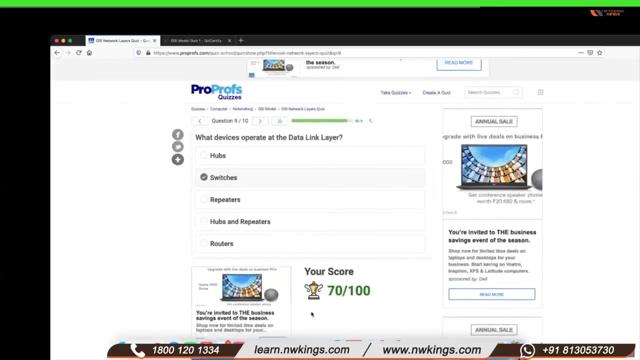 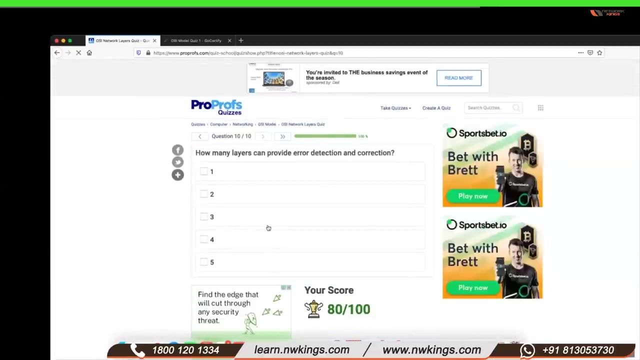 which operates with the mac address. that is switch, not hub. hub works on physical layer with the signals. data link layer takes care of mac address and i have explained that a mac address switch is stored at table. that is known as mac address, right? so that is some error correction detection. so error correction, i think works on this. 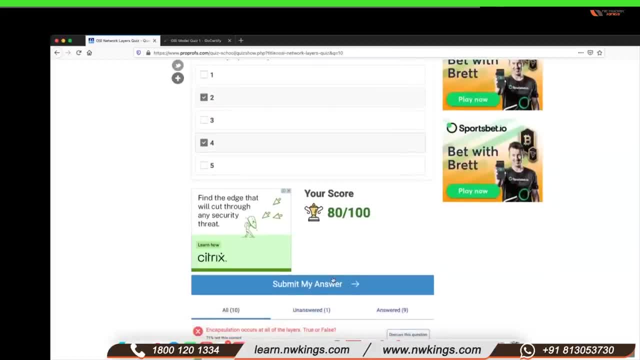 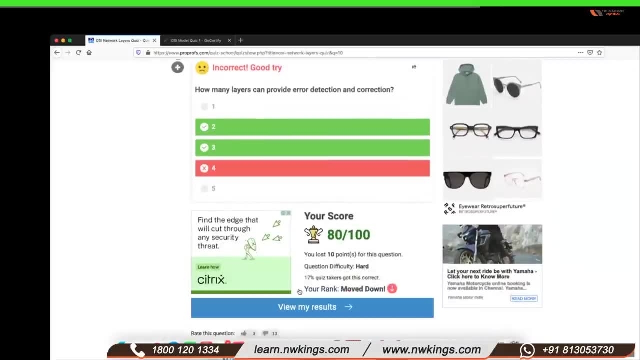 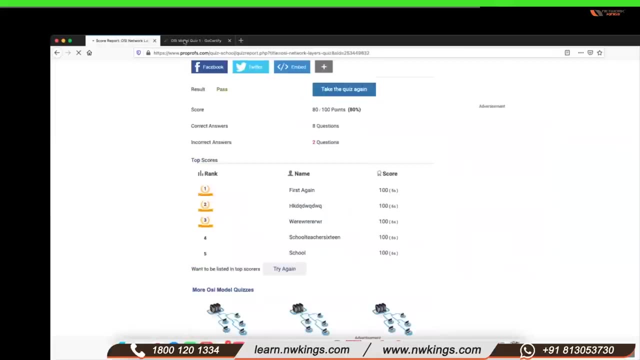 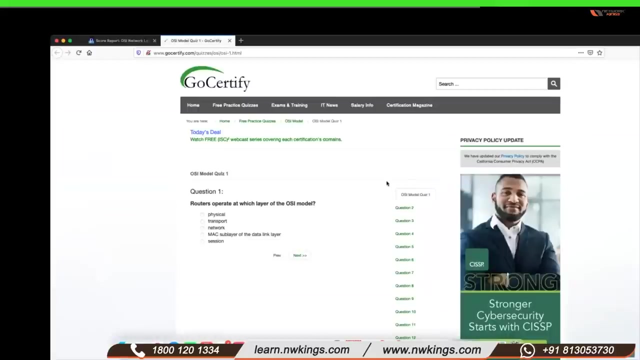 layer two, layer, layer four, maybe layer two, three, something. yeah, two, three, okay, so we have done. we got around eight to nine questions correct, so again you can check. so means what i'm trying to say, like at least you got now when you will see osi model questions you 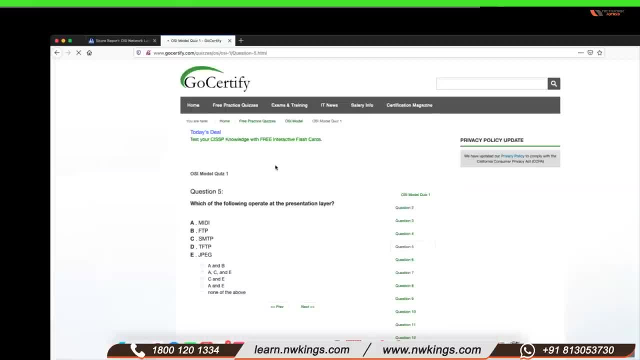 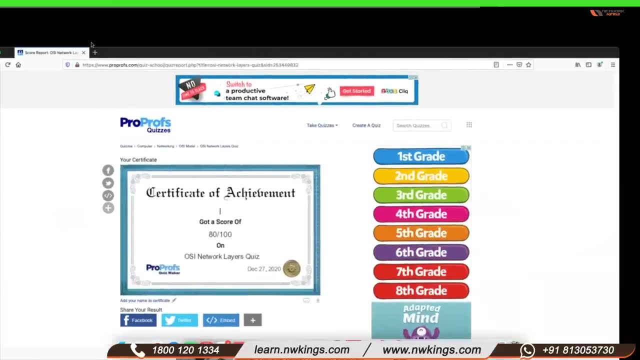 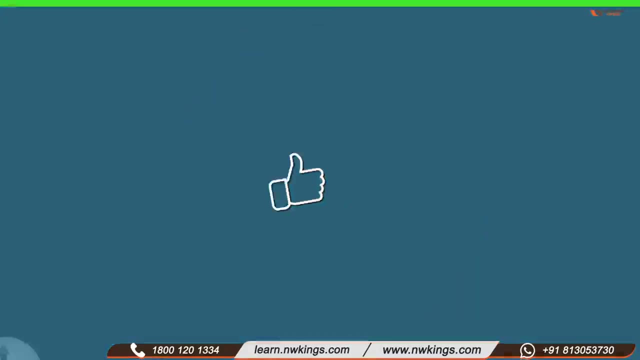 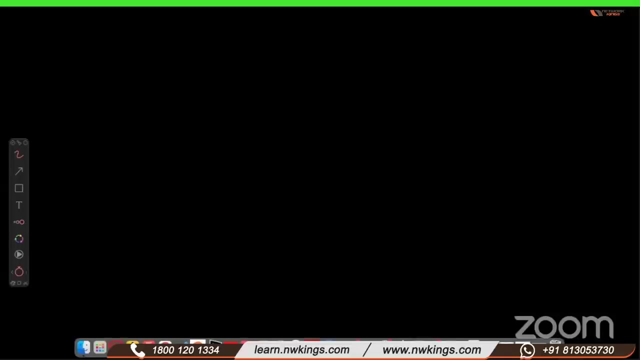 will not. you will not be completely blank. if you really want to give any exam like ccna or anything, okay, or maybe the comptia network plus hi, you are watching the recording from one of our live session. hit like share and subscribe for more future updates. so we will not waste time, let's. 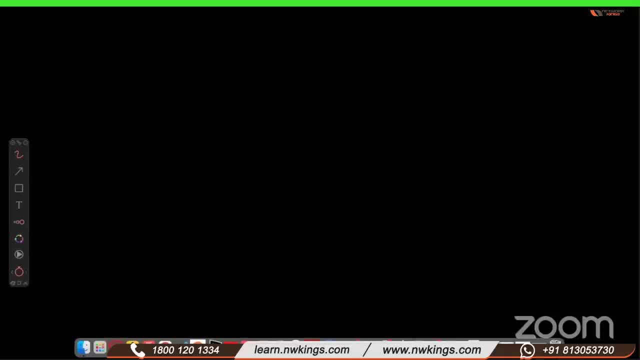 learn the ip address. but before learning ip address you should know how ip address like evolved or kisne usko banaya. okay, so this batch i'm going to take in mixed language. i'll going to like: uh, don't worry, if you are, if you understand hindi, definitely. 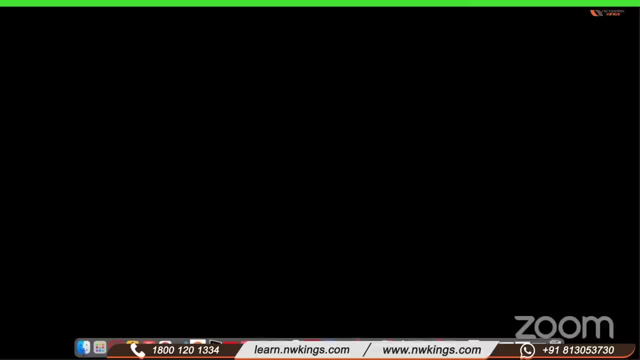 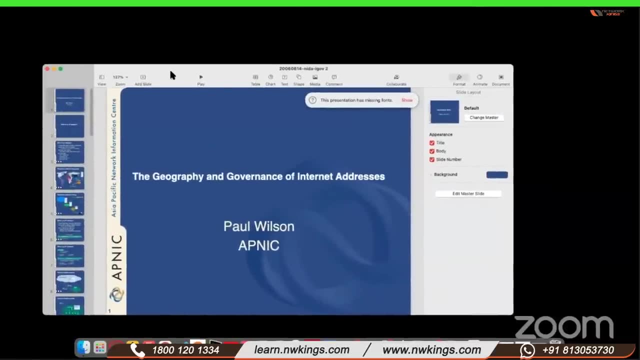 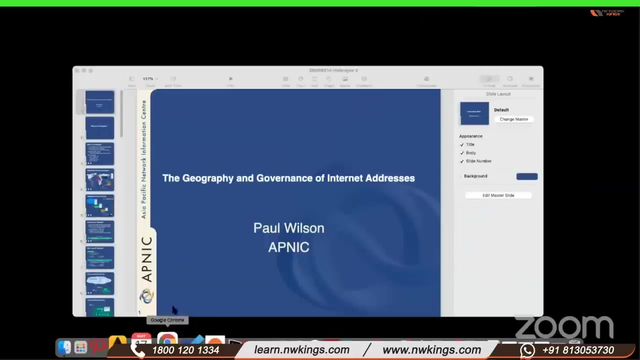 you can also understand this. so hindi english me mix rakhunga, don't worry, okay. so, guys, first of all, you need to learn about one company or organization that is called aina internet, assigned a number authority. okay, so do one thing. how to get the document? so just. 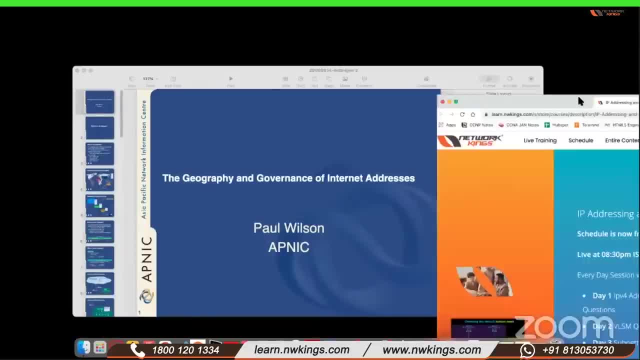 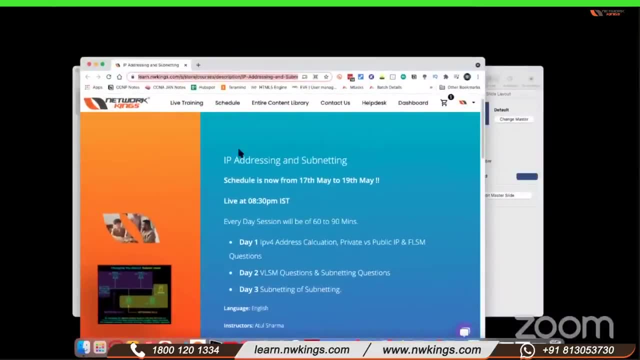 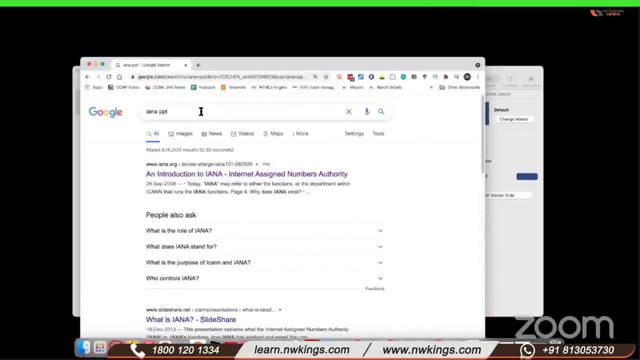 okay, so this is the link you can join from here: ip addressing and submitting: okay, so aina, ppt. okay, just search this and you will be getting one ppt or pdf document. just search. i, a, n, a. what is i? n a internet assigned a number authority. okay, so i'm not directly starting submitting. you should understand. 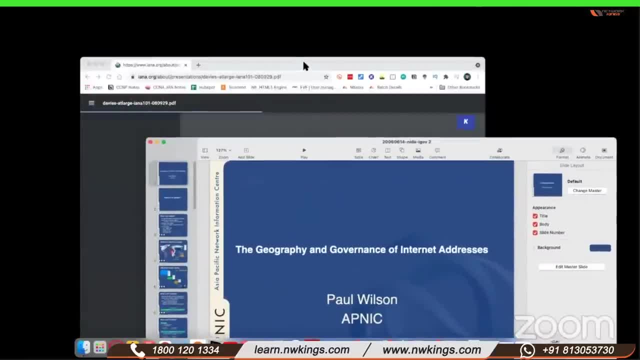 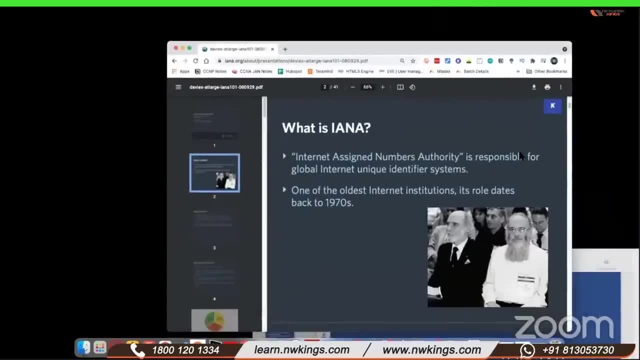 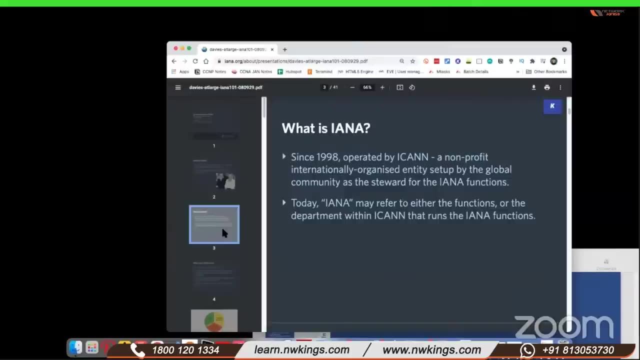 what is aina and why it is like started ip addressing and all okay, let's back to some the okay. so what is aina? so it's internet assigned number authority. very simple, okay. so aina is actually operated by i can okay, and this is another organization which is a non-profit organization. 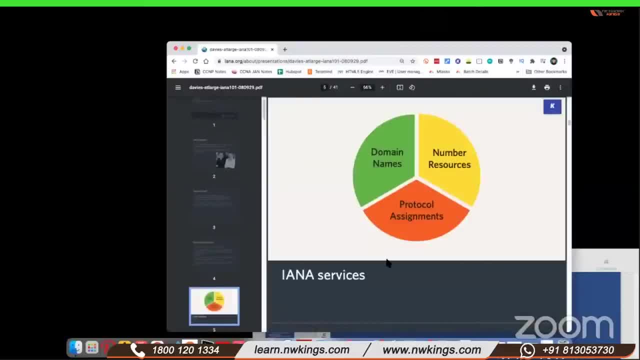 and what aina do. so aina is taking control of three things: domain names, number resources and protocol assignments. okay, so means all domain names, like if you buy any domain name like googlecom, facebookcom, so the this is called domain, and this all controlled by aina. number resources, like ip. 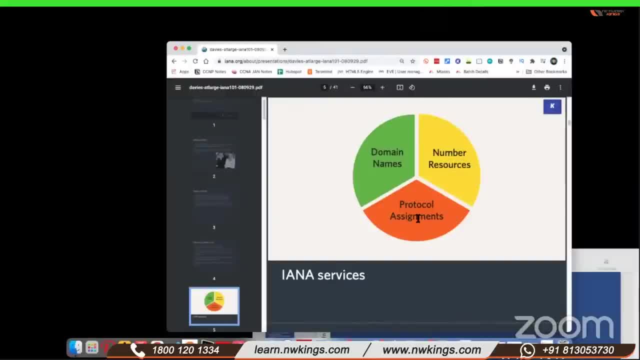 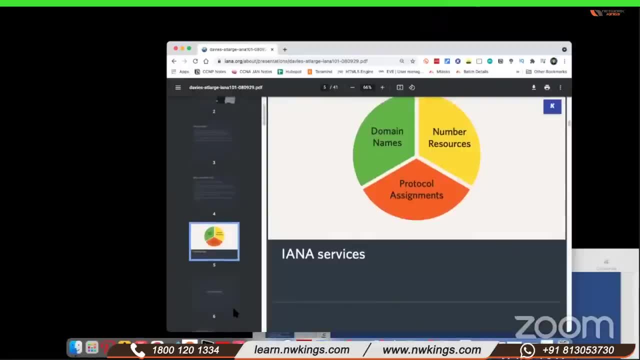 addresses will be also controlled by aina and the protocol number, like ftp port number 21, simple mail transfer protocol port number is 25, all this also controlled by aina, so please remember aina. so aina is a very big organization which controls domain names, protocol number and number. 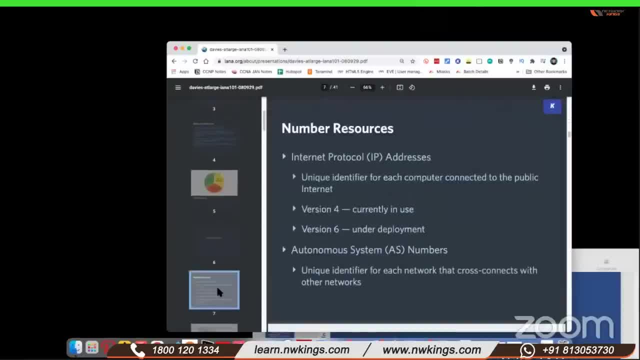 resources. okay, so this you will not get in any book, definitely. so what is number resources like if ip address, if we talk about ip address, so number resources, may ip address? okay, so in ip all, version 4, version 6, so this is what we call ip address. right, and one another address comes. 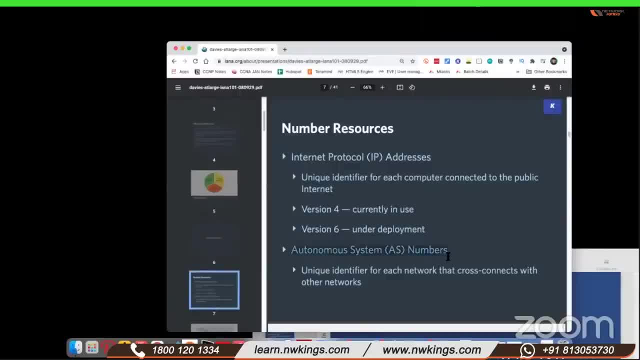 autonomous system number. if you learn bgp or some kind of system number, you will get a number address. okay, if you are a beginner, like if you have not done even your cc, so just it's like a number where every company have their own number. okay, it's like a company unique number, you can say that. 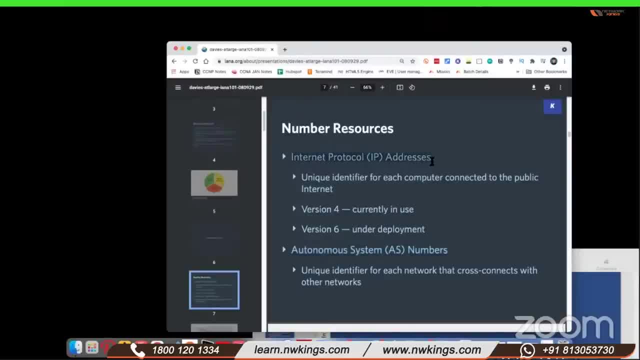 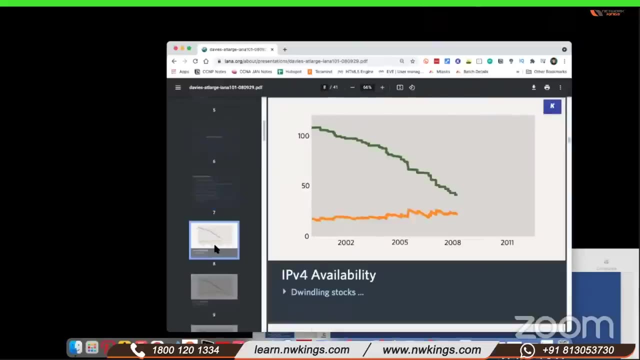 and another is internet protocol address, which is available in two address: version 4 and version 6. so version 4 or version 6, you must have heard of it. there are two types of ip address, okay, and one is autonomous number which companies use. okay, so let's talk about, so slowly, what, what is happening? ip version. 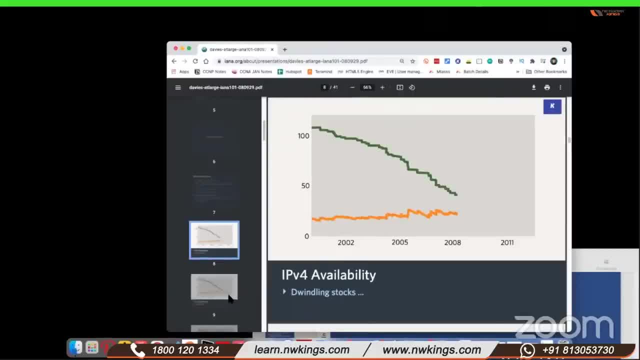 4 is actually uh like, uh getting exhaust, meaning it is getting exhausted slowly. so ip version 4 is getting exhaust. so this is why ipv6 is also in trend. most of the big companies are using ipv6 also nowadays, like geo reliance. geo is using ipv6, okay, so ipv6 is a very 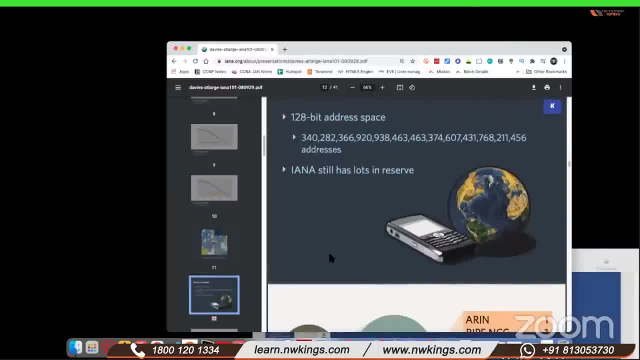 big number. but here this workshop is for ip version 4, strictly because we need to learn the subnetting, because 80- 90 companies are still using ip version 4. but i am going to conduct another workshop, maybe after a few days, for ipv6. maybe i'm not sure, but let's complete this first. okay, so now, what is aina? 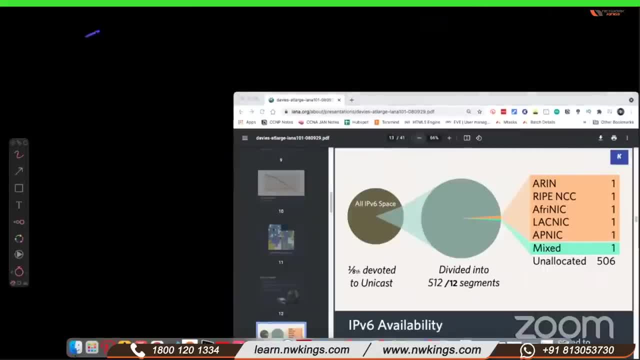 so i told you, aina is internet assigned number, authority, right. so aina has five or another organization which is called airin, so these are called rir. so aina k small, small departments, so which we call rir. so aina has subdivisions called airin, ripe apnic. 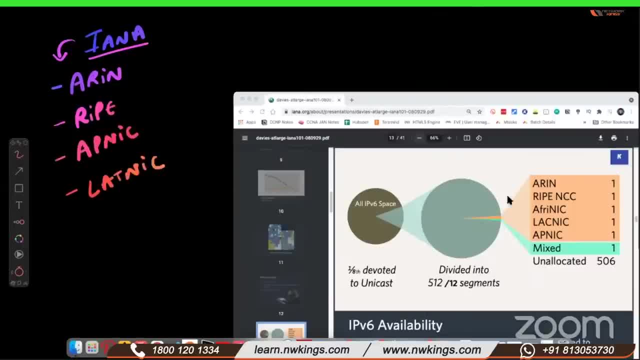 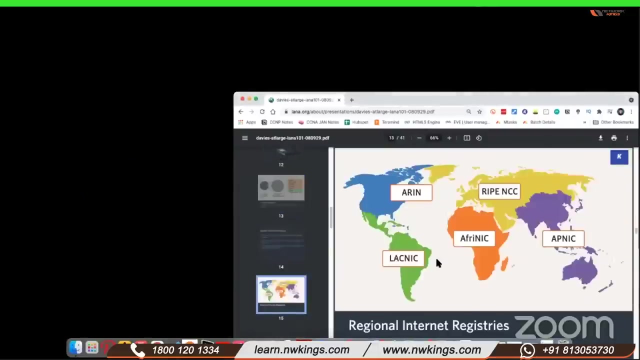 latinic one another. uh, this is latinic, the ppt is wrong. see, aina ppt's are wrong. man, what is happening? so another? so what is this? so every big, big organizations means, uh, all countries, we aina can't handle. so this is why aina divided into different, different continents. okay, so you can see apnic. 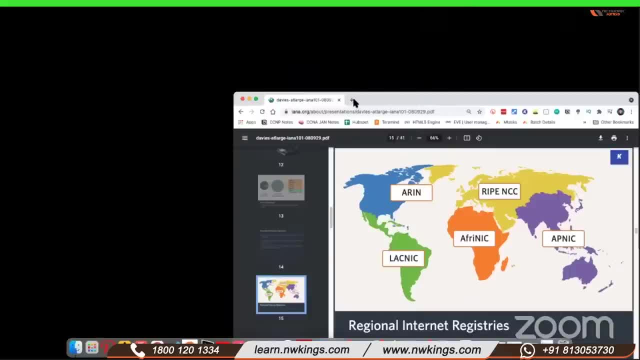 that is asia pacific network information center. if you want to buy ip address, you will not buy forum directly, aina, okay. so i told you who manages iip addresses. all dns entries, all protocol number and all ip addresses managed by aina. okay, clear everyone. please say yes in the chat. 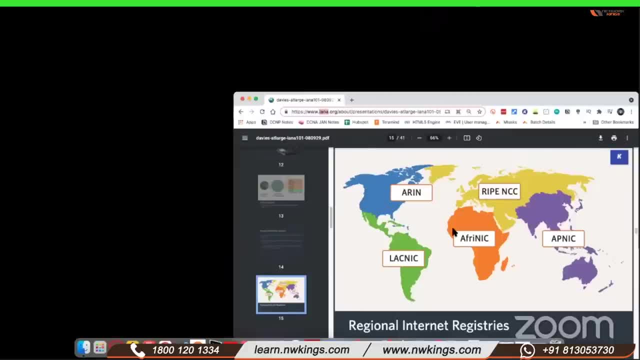 if anyone has any doubt, you can ask me. yes, everyone clear, all going good. yes, abhishek ajit robin deep. all okay, say it. okay, you are writing in chat. yes sir, yes sir, yes sir, okay, any doubt? no, sir, no sir, all good, all good, thank you okay. okay, so air in laconic, africanic ripe apnic. 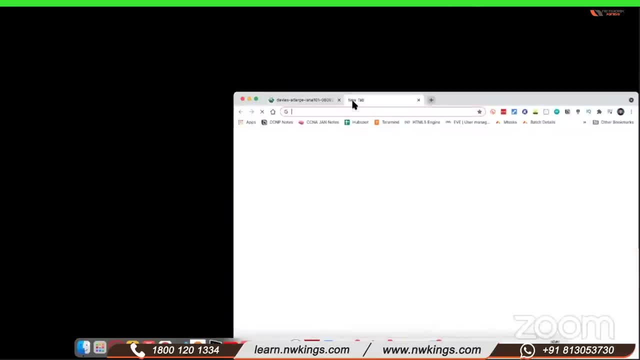 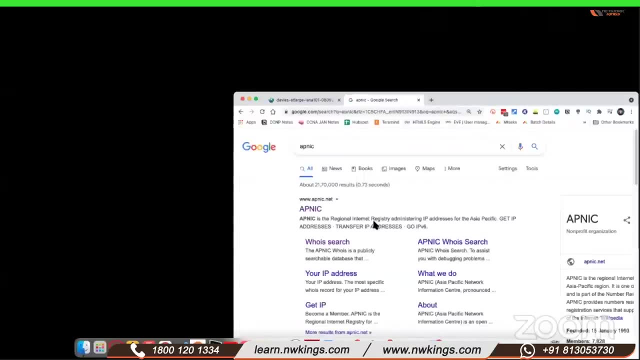 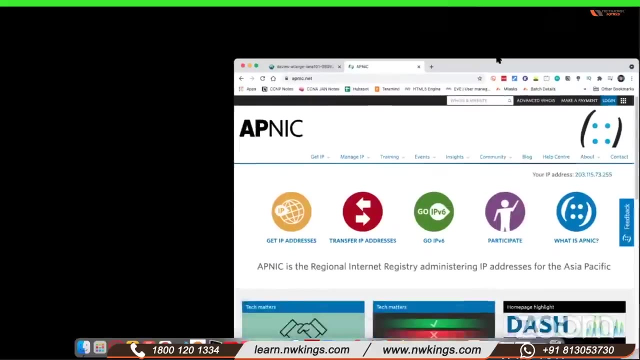 okay, so this is asia pacific network information center. you can check one by one apnic. so if you are from india or from any other asia country, you have to buy the ip address directly from apnic. so you can see apnic, asia pacific network information center. so this is in australia. 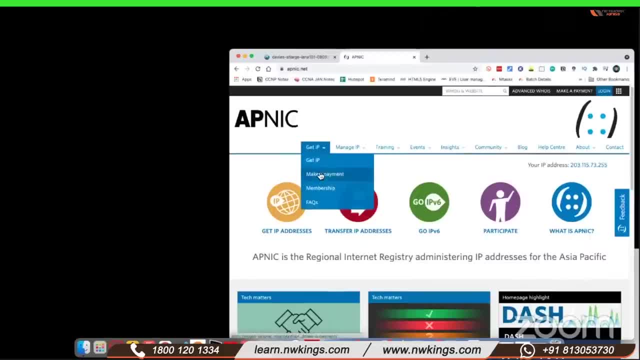 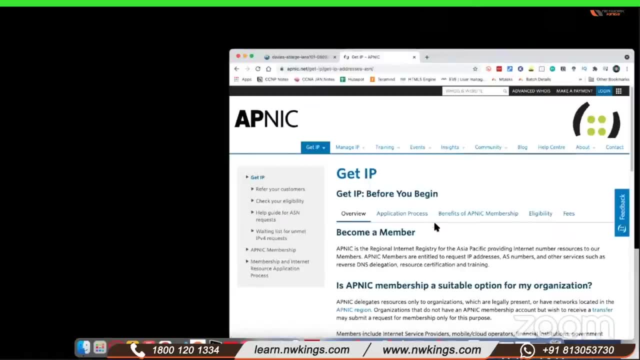 so they have office in australia. so now, if you want ip, you can see, make a payment, get ip. okay, so when you get a broadband connection, when you get internet connection, you don't pay to apnic. why? because your service provider is already paid the fees. so when you install broadband at home, you don't pay for ip. 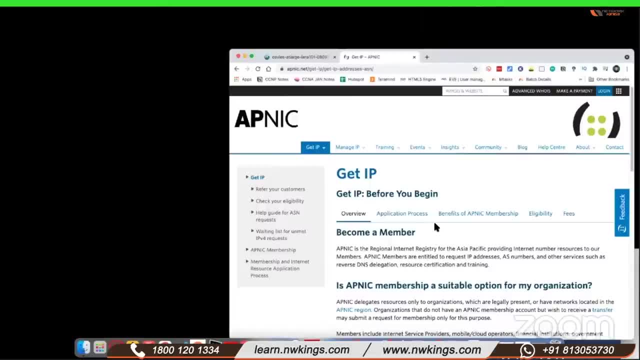 right, because isp is giving you its own ip, so isp is giving your his ip addresses to you. this is why you don't have to get from apnic. but if you are a very big organization, organization, if you are a very big organization, uh, you need more than 256 ip address. if you need 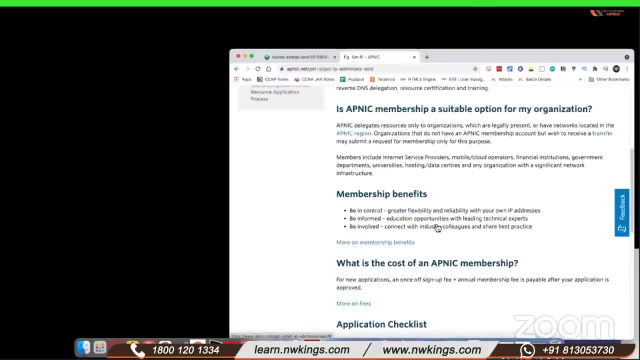 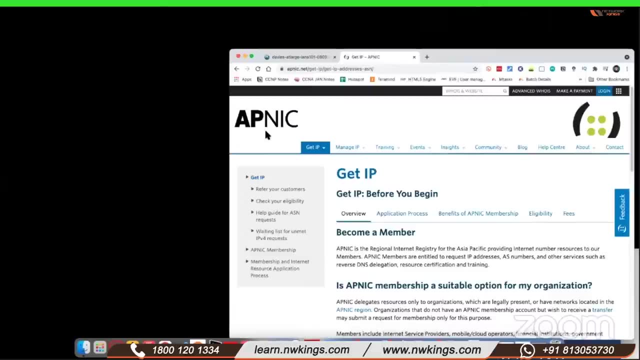 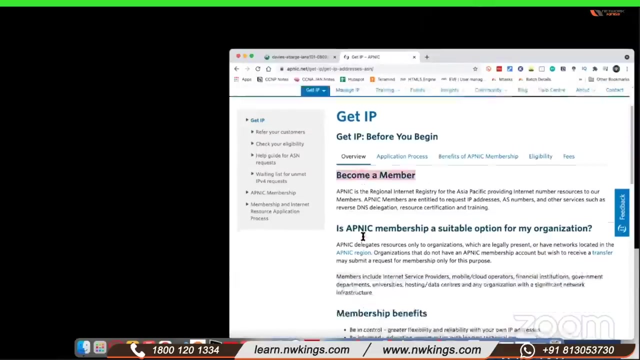 more than 250, 256 public ip address, then obviously you have to buy it from apnic clear. yes is, yes, is 10, 20, 50 IP address. you will buy from ISP clear, yes, sir, yeah, yeah, clear, okay. so you have to be a member. then, uh, like there is a fees, it's not free, okay. so start your application now. so there. 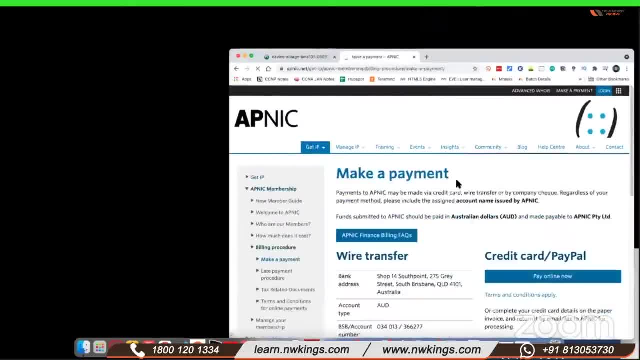 is a fee, uh, so you can check what is the payment mode, how to get IP address and all. so you can see all the details here. so generally, uh, 250 IP address is approximately 500 Australian dollars every year, so 500- 600 dollars every year. you have to pay IP address if you want 256 or some IP like. 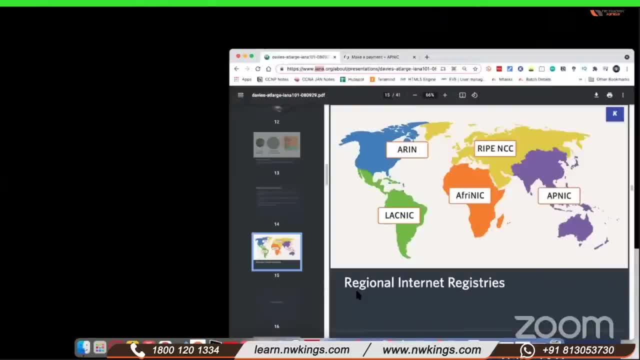 that, okay, so that is overview. so this is called regional internet registries. if you are from America, you will buy from America registry internet numbers. if you are from Africa, that is Latin America. sorry, Afrinic is for Africa, this is for Latin America and this is for Europe. okay, so 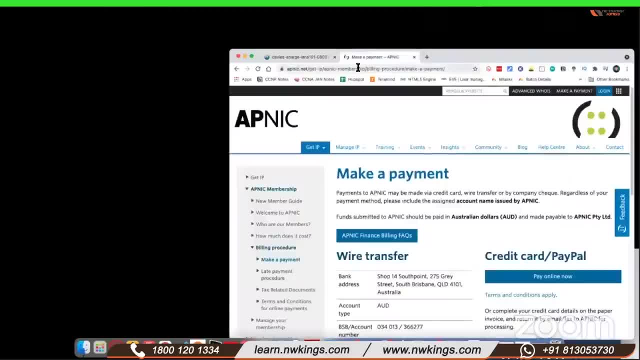 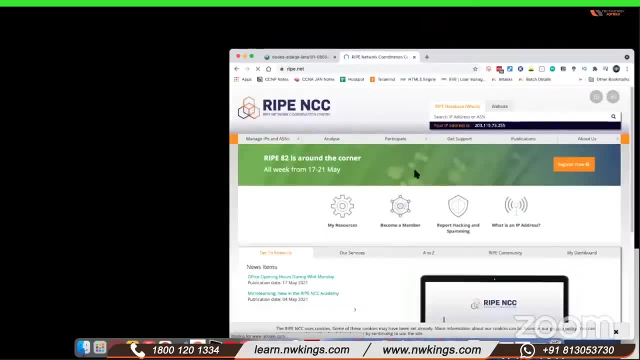 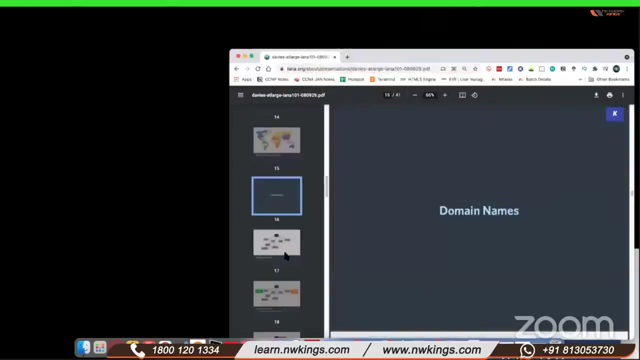 you can check one by one on Google and you will want to know if you want IP from ripe, then definitely you have to go to right network coordination center. so if you are from Europe or any country in Europe, you have to buy it from here. okay, so all all are five RIR, so let's move on. okay, so IP address, and after that I now also 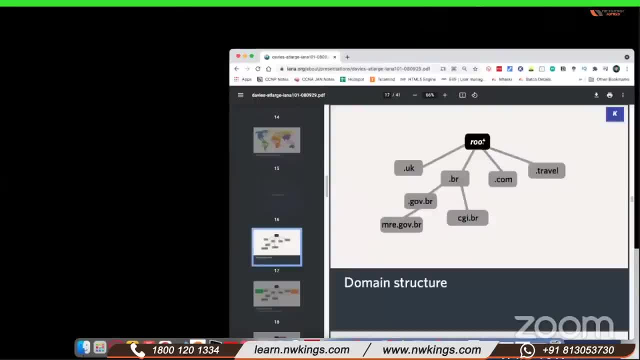 maintain the DNS numbers. so the main, the domain structure is like that: root root. all the big numbers are inside this root something. so you can see there are two numbers, which is called cc, tld, country based top level domain. tld means top level domain and dot, com, dot, travel, this. 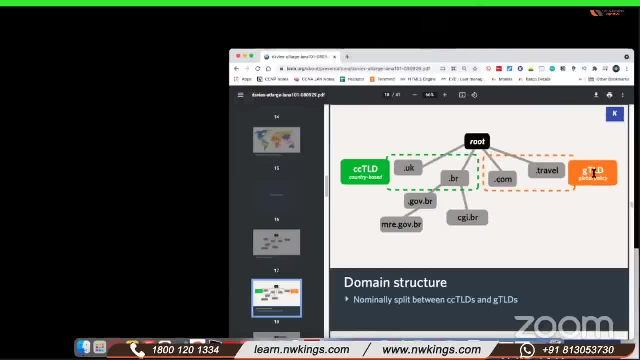 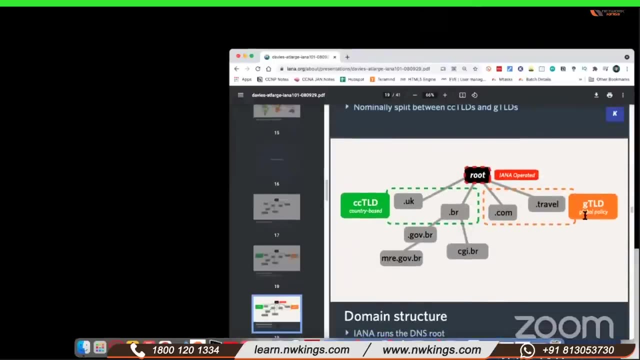 is for global policy. okay, suppose you buy dot com, this comes under global policy. and if you buy dot uk, dot i n, dot government, dot education, so these are like country based, specific. okay, so who operates this? global policy? numbers like dot com, dot travel, dot net. so all these domains are operated by Aina. 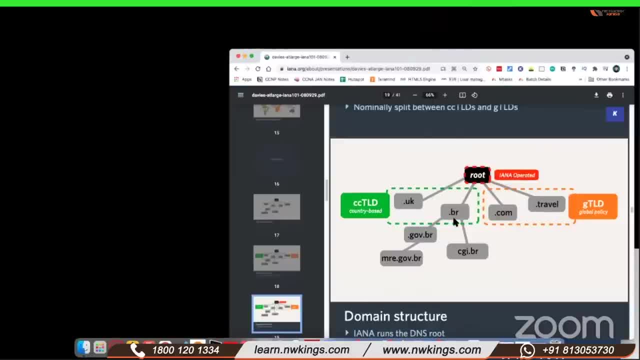 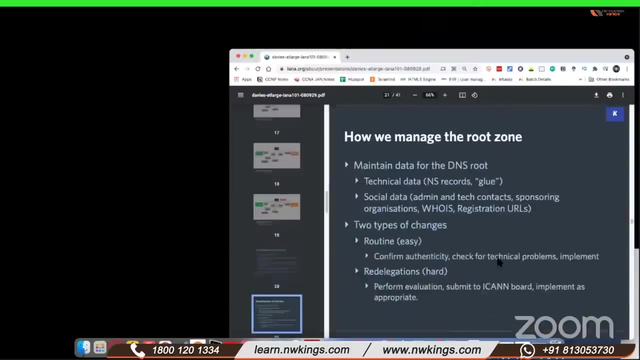 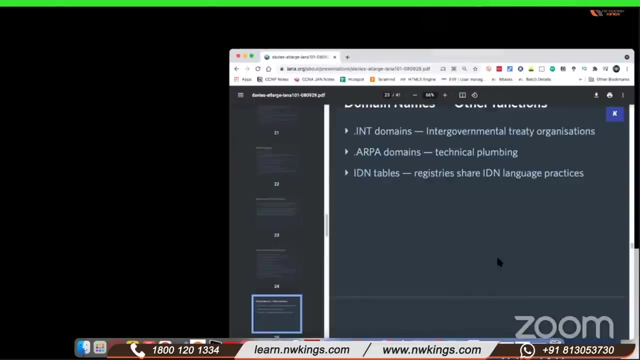 managed by Aina, but all dot uk, dot Brazil or dot I and all are controlled by countries. okay, all are controlled by country DNS servers, not by Aina. so I know is a very big organization again. okay, so this is all basic things I'm you might be will not get directly. I am showing you from the I now. okay, it's like very big. 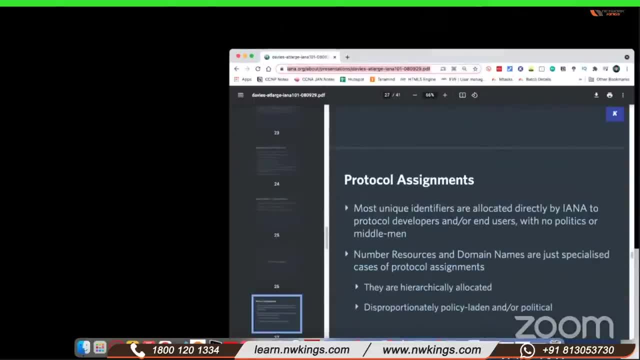 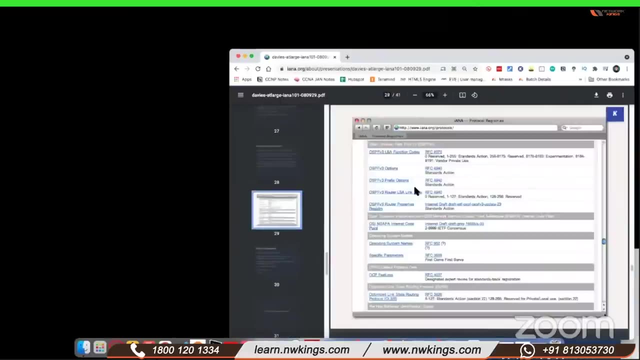 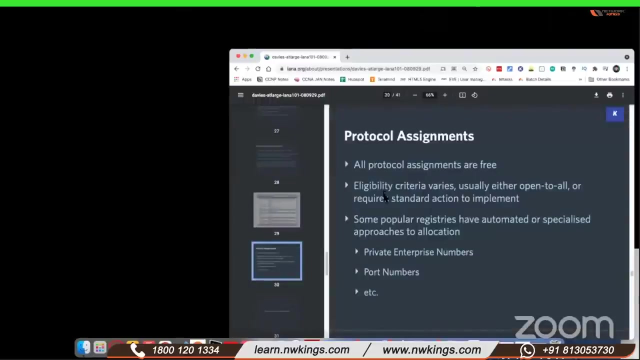 organization and you can still download this ppt also, so match at my link. yeah, so we will definitely come to submitting, don't worry. okay and uh, protocol numbers like the protocol number FTP and all these protocol numbers are also assigned by Aina. okay, port numbers or these numbers also assigned by internet assigned number. 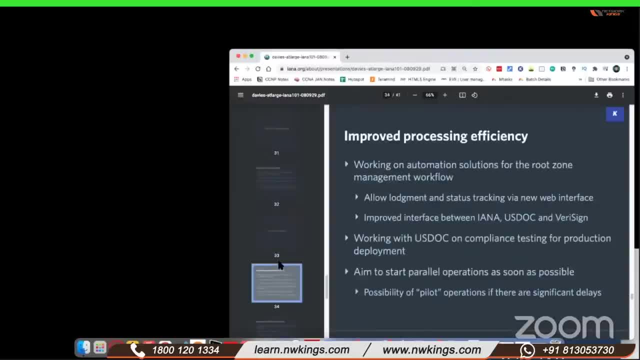 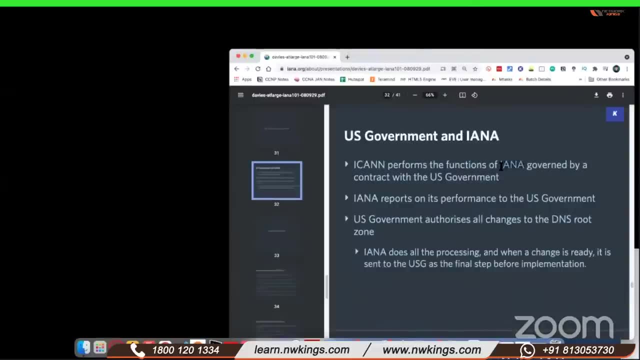 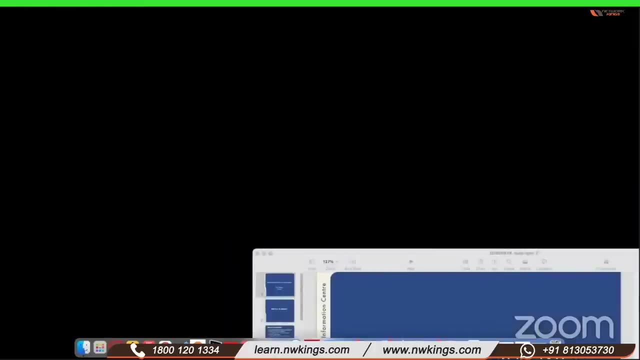 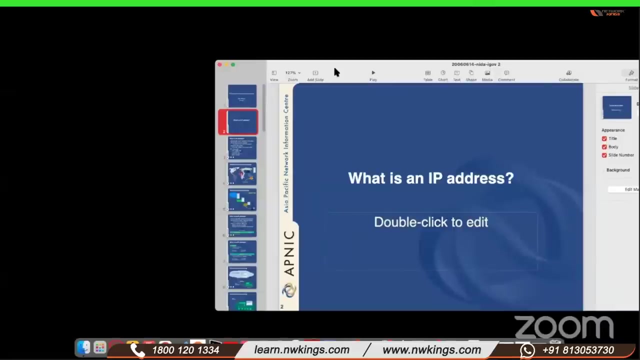 authority. sir, registered port number is also assigned by Aina. yeah, yeah, yeah, all registered ports are registered by Aina. only. okay, sir, okay, yeah, okay. so this is all. now you come to know, like, what is Aina? yes, yes, yes, okay, because IP address is all managed by Aina. this is why you should understand what is Aina and when. 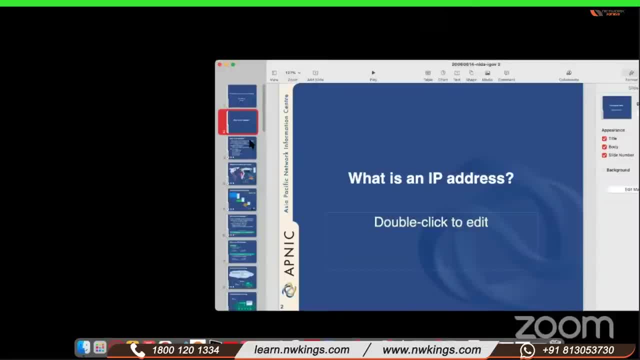 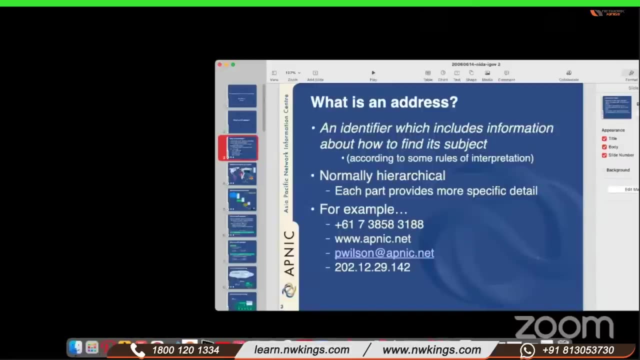 you will be going to join any company as a network engineer, cloud engineer, system engineer, Linux, whatever. so you should know, like, how to get IP address, how IP address work. this is why I have IP address is a unique identifier means a unique idea of every device, so it's like a unique identifier. 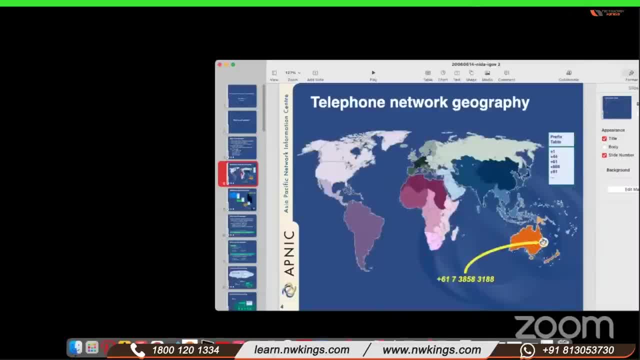 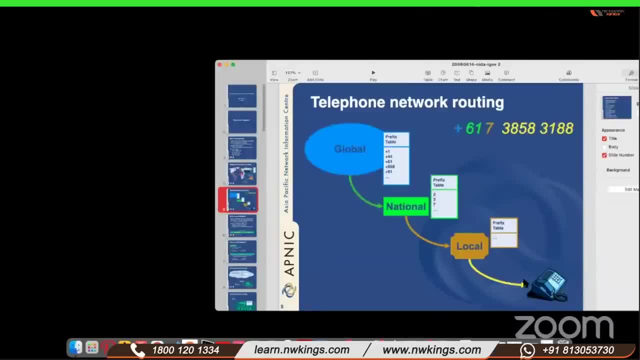 every device in this world needs IP address to talk with another device. okay, so like if you call someone- suppose you are calling from India to Australia- okay, you need a country code, then again a national code, then you type the number. so same like you dial someone and the another person get a. 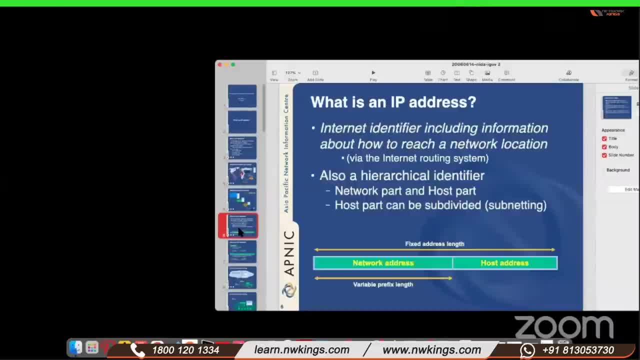 call so that you guys can talk to each other. so same like IP address is a unique identifier, like internet identifier, but full form is IP address. okay, IP address, okay. so all internet routing system, all internet devices works on IP address. so let's talk about in short: so what is IP address? 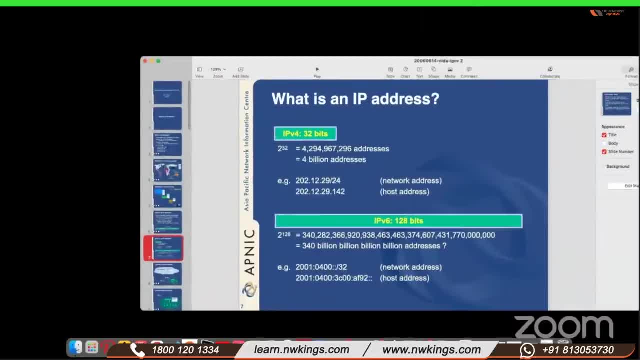 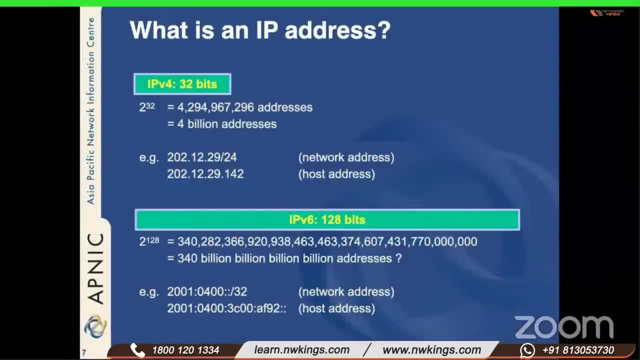 it's a very big number, so it is available in two variants: IP version: okay. method of broader screen: huh so, and guys, I don't actually read ppt is this is not my style, but still it's very good, informative ppt, so let's understand. so now you can see. IP version 4 is 32-bit, which comes around 4. 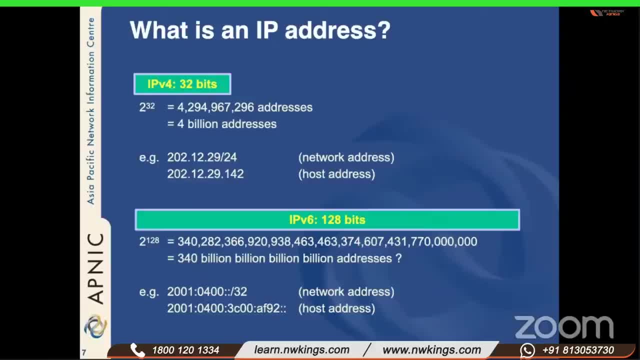 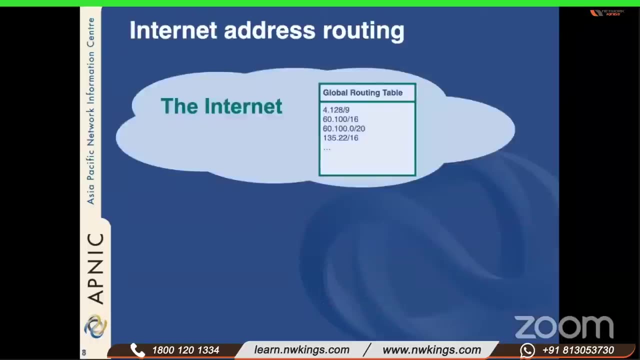 billion addresses, but this is almost exhausted. and now ipv6 have almost 340 billion, billion billion IP address. you can't even count that. it's a very big number. some people call this undeclian also. so now what is happening? internet has very big, big number routers, okay, all internet has a very big 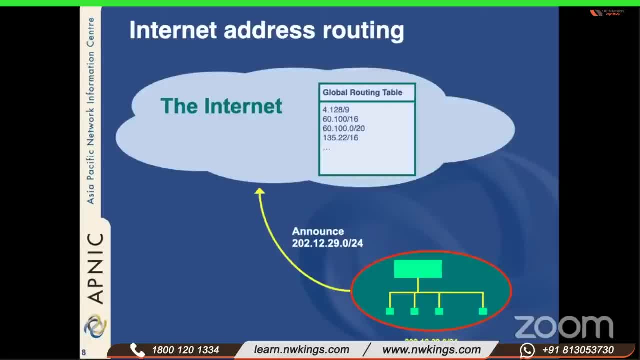 routing table. so why we need IP address? all internet has a table called global routing table. it is also known as BGP table. there is a protocol which is very famous- BGP border Gateway protocol- simple language. internet has a table called global routing table and when you announce your routes, 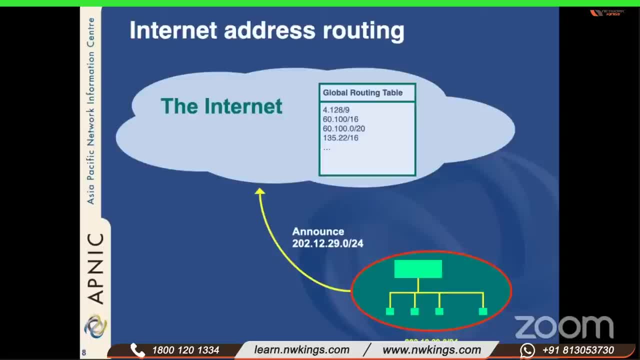 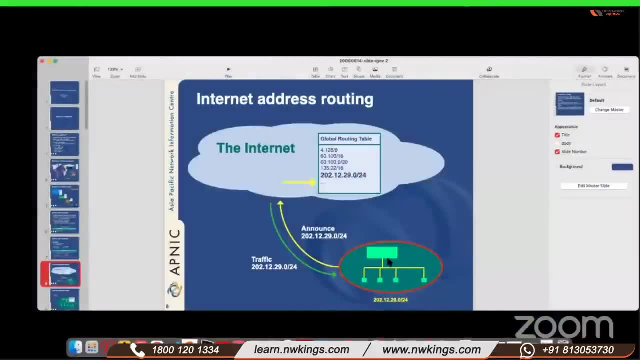 what is announced. you can see there is a small green color circle with red line border. just see the downside ticket. so you can see here. suppose this is your company and you have few servers, like you have a. you are a company like Facebook or any company, or maybe you are yatracom or railwaycom or 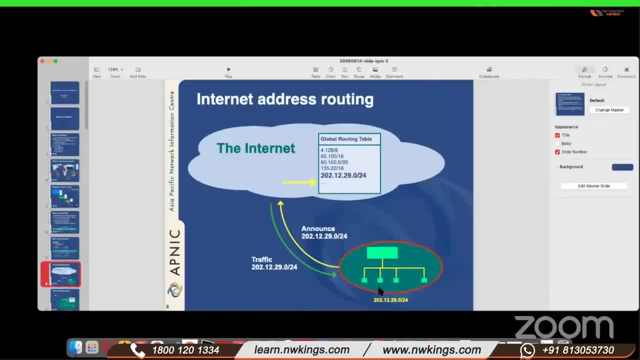 any website you name it suppose you have your servers, so you have to share your IP address. you are, you get this IP address from where apnic, so from where you bought this apnic and you are going to announce you are going to share your IP addresses with global routing table. why, when you 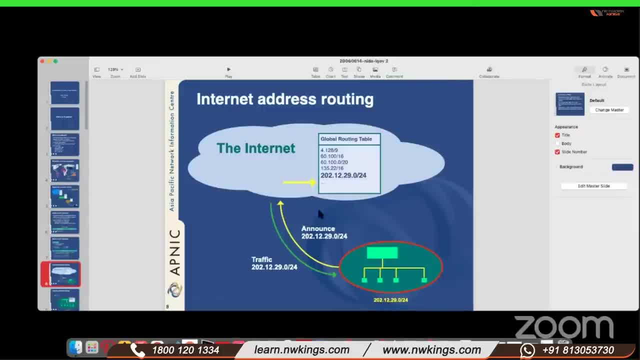 announce this: 20212. so this is IP address. when you announce, then whole internet will come to know. you have some servers, so when you put your IP addresses in the global routing table, then only whole world can access you. this is called routing. when you announce, so how to share your routes to? 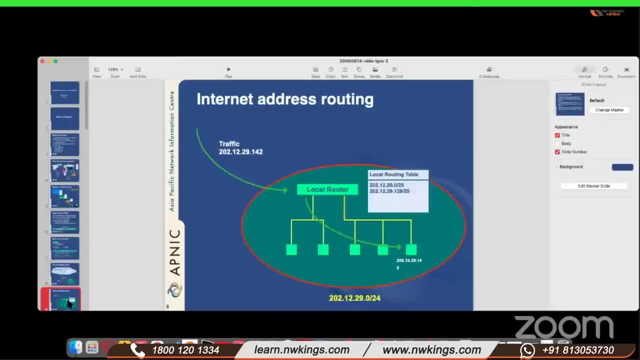 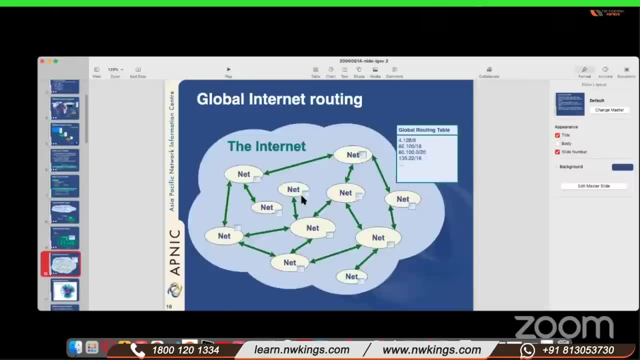 internet you have to use a router. Ok, so, in short, you are going to push your information to a router, then router is going to share your information to the global internet. so you can understand like this: one router and it will go, because internet is a network, of network. so what is internet? internet? 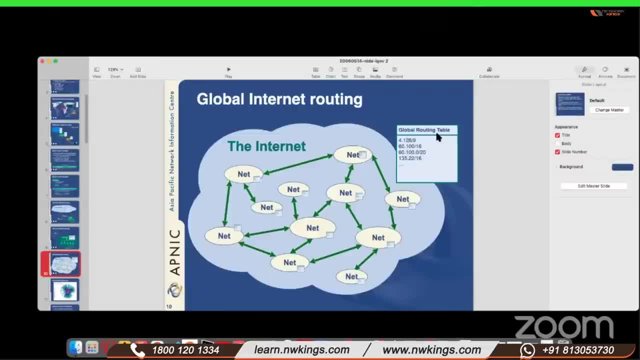 is network of networks which are managing global routing table. all big companies, routers, have global routing table. this is why, if you sit, if you take atl connection, if you take geo connection, you can open googlecom, facebookcom. so few sites are blocked because they have their own internal. 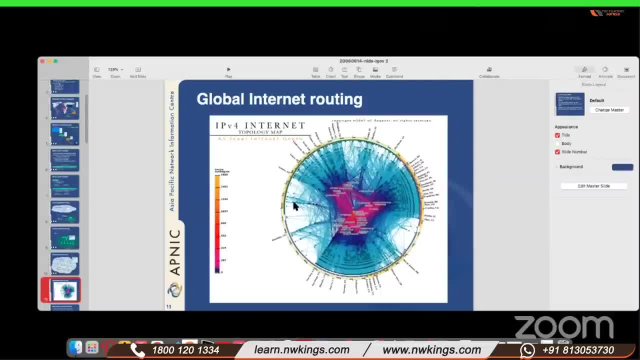 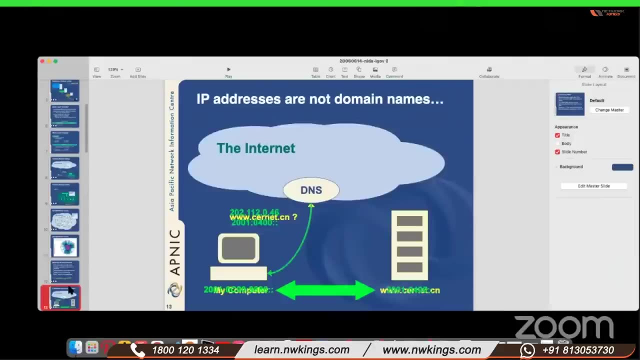 firewalls. so this is ip version 4 internet map. almost it is exhausted and it is a old ppt, so still you can understand the boss of exhaust, okay. okay, so remember: ip addresses are not domain names, so domain name is your website name, like googlecom, facebookcom. that is domain name and ip. 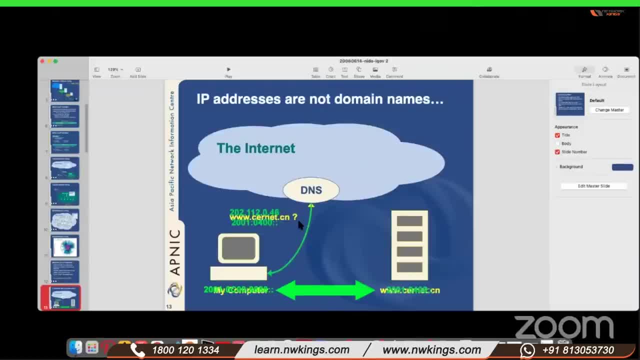 address is your, like 202. any number is called ip addresses, right 101 dot any four decimal number. if you have seen somewhere like 190 to 168 and when you see any open website like googlecom, facebookcom, that is domain name. okay, so that's all, so you can see where do i. 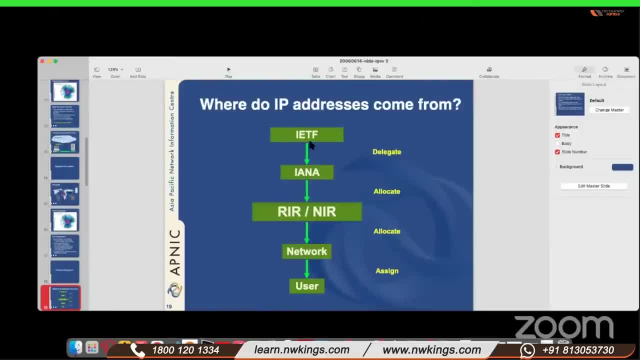 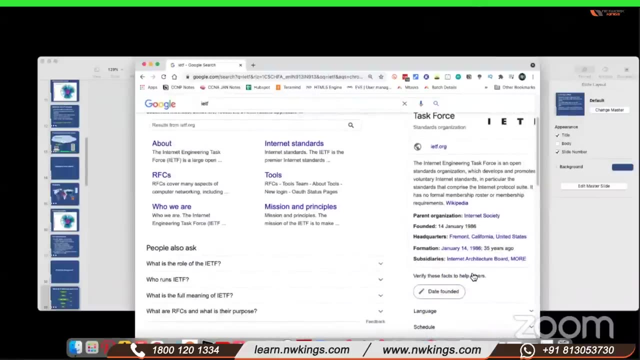 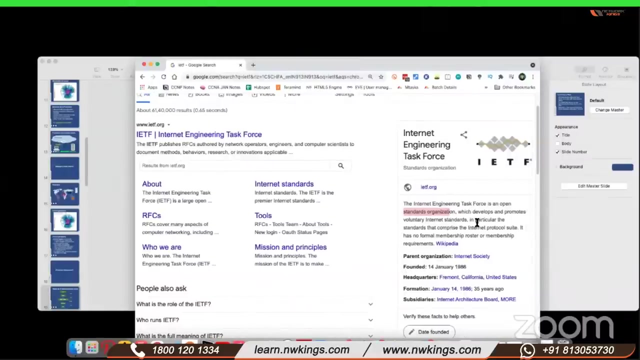 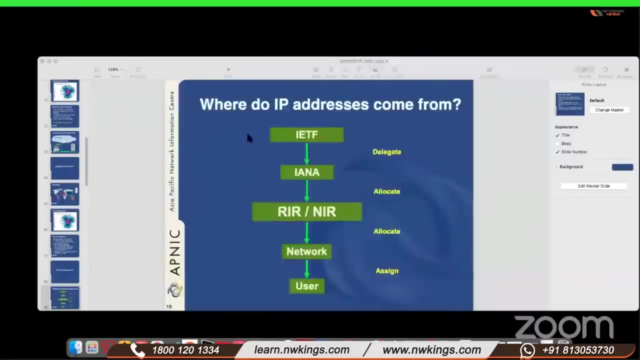 paid iraq Merci far mainly made for its open standard organization which develops and promote internet standard organization. our ike over here. we teu also okay, so that is ietf. then they give to aina. so then after that i have explained, aina gives to. 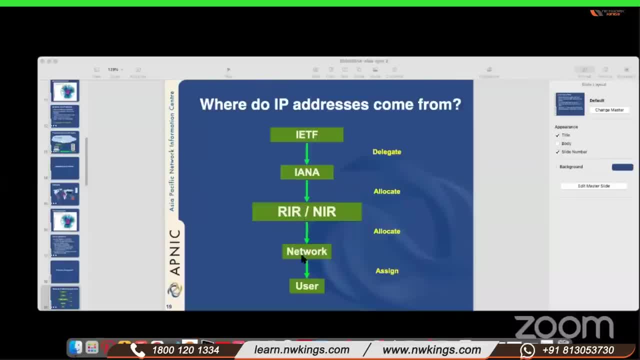 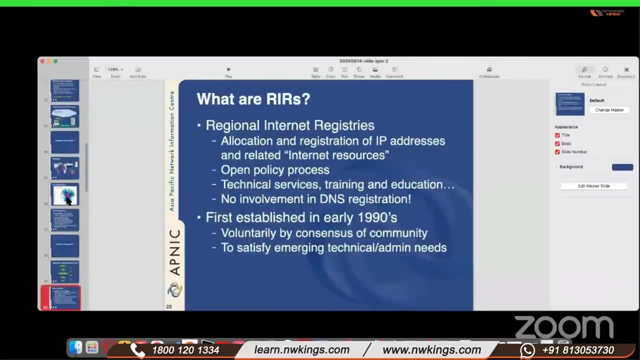 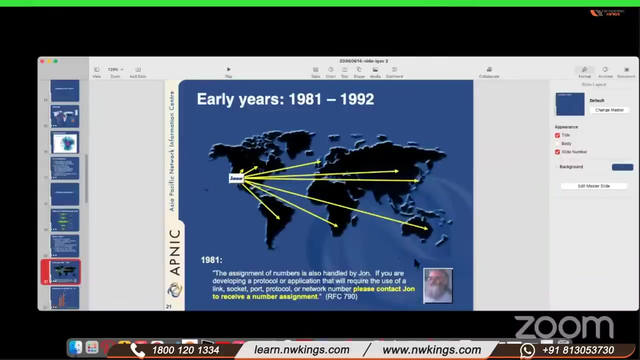 regional internet registry, then it gives to service providers or any company and then user gets the ip address. yes, everyone, any question. yes, all good, thank you. yes, i got it okay. good, okay, let's move on. okay, so when aina started, right, so just it's like a funny story. only one guy used to manage. 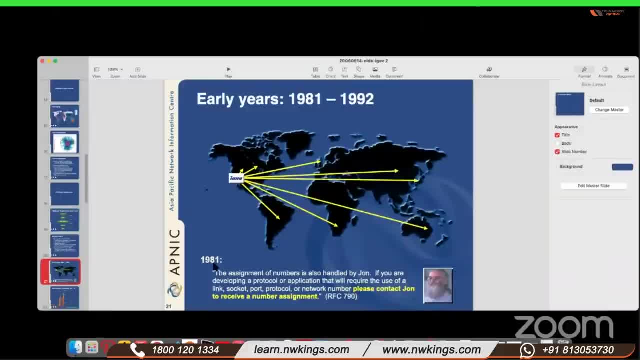 the ip addresses. if in 1981, if you want to get any ip address, port number, protocol, call then on the website. it's like please contact john to receive a number assignment. so that is like long back, 30 years back, 30, 40 years back, almost okay. so only one person who? 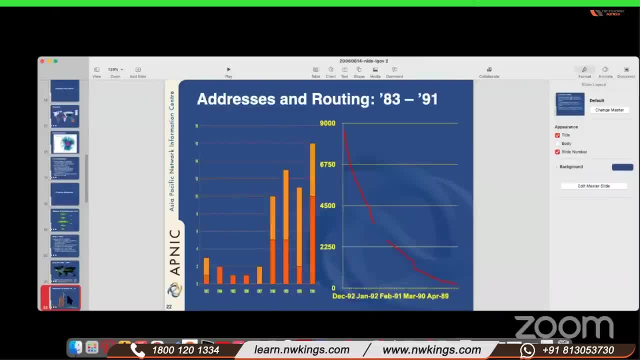 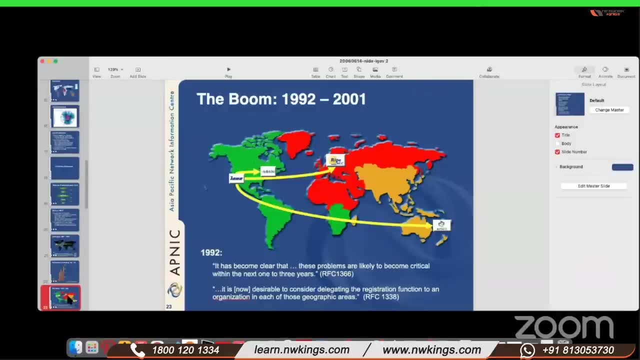 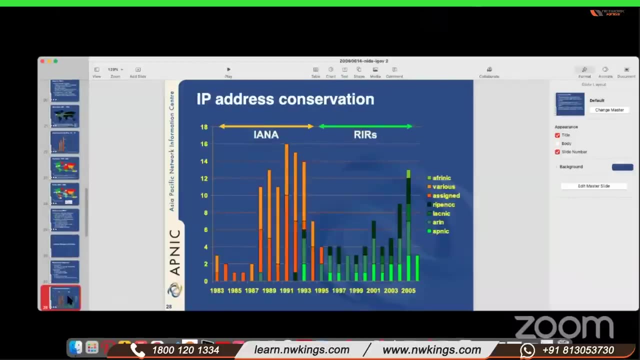 used to manage the ip and protocol numbers. then slowly, slowly, users are increased, routing tables are increased. this is why they have divided the network into different, different regional internet registries, and this is how this is what we call internet now. okay, so i know. so you have. 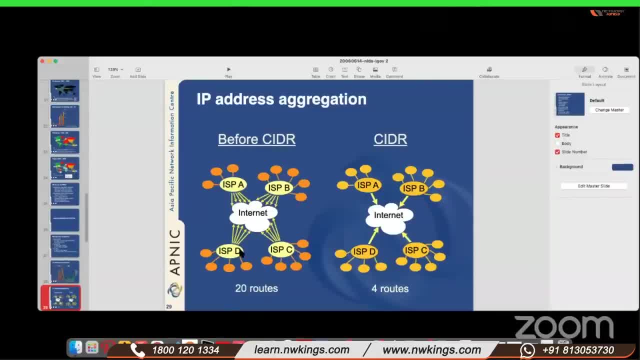 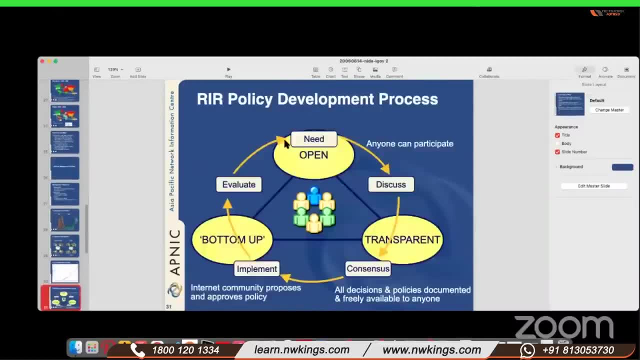 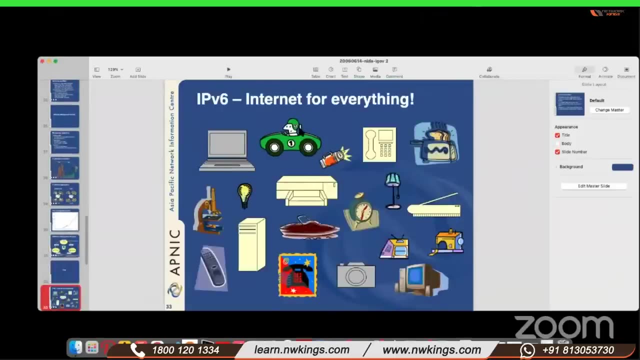 like many service providers are getting a lot of routes. okay, this is also called cidr. i'll explain that cidr. so uh, so let's start. it's better. let's start the ip address now. so ipv6, a very big number you can assign. yeah, so ipv6 is a very big number, like you can give ip addresses to any object in this world. 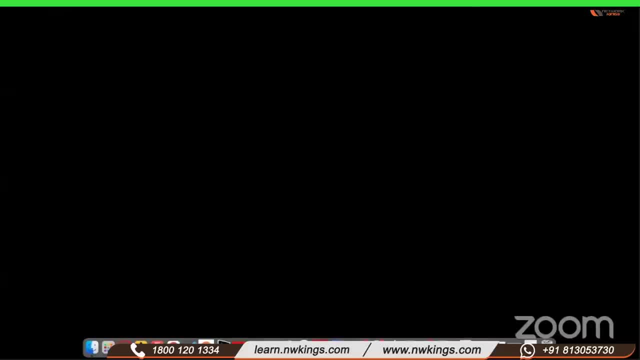 thanks, okay, this i was discussing aina, so now, now let's understand how aina divided the number. okay, so, first of all, guys, please open your notebooks and just let's understand what is the decimal to binary. okay, just complete these three days workshop, you will be mastering. 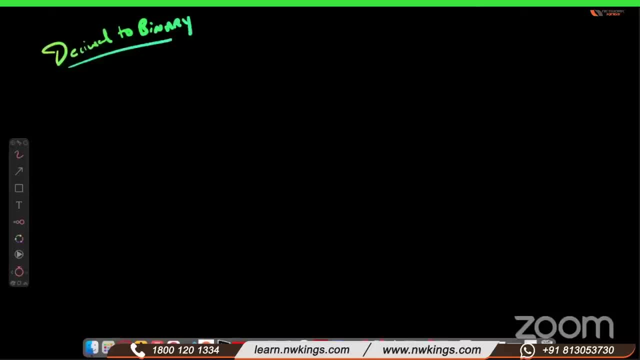 the laddar stepwword: okay, just complete these three days workshop. you will be mastering, submitting, and when you come- soon, you come to the moment we, we will have a full agreement and once you are ready to go, and then you will be to our next workshop, which will be: you have three, no étant said regardingой, then you'll just 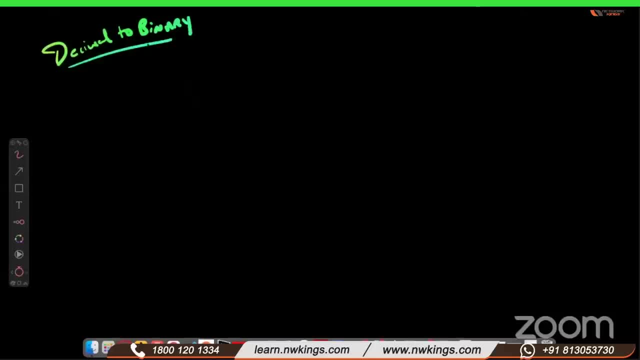 have three. no, NICKEN know booking up andeses and see you in the landing page. just come何, i'm sure. so decimal to binary, okay. so what is a decimal number and what is binary? so whenever you get, when you, whenever you see ip address like this, so this is a decimal. 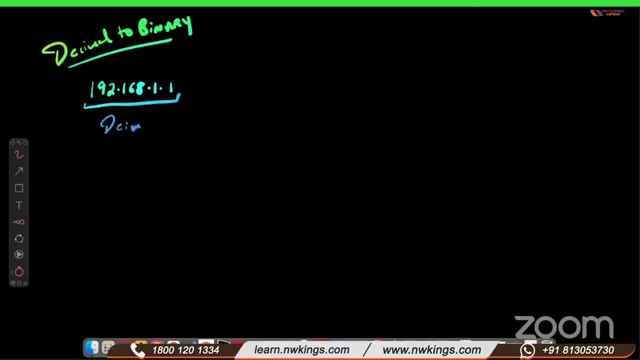 format. so this is a decimal, decimal format. and when you see any number like one zero, one one zero, one, one zero, something like this, so this is called binary number, so this is called binary number. so tell me, your computer understand decimal or binary? so obviously binary, binary, right good. so now we have to understand first how computer understand your 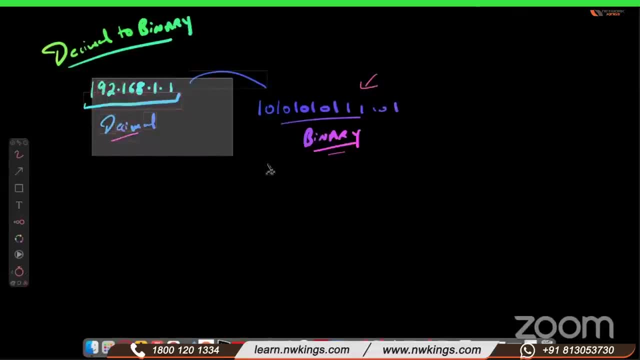 ip addresses. so to understand this. so everyone knows that from school days also that so you have two different digits, zero and one in binary, yes or no, so zero or one binary, so this is also called machine language or something like that, so it's like binary. so now, so these are two numbers, so this 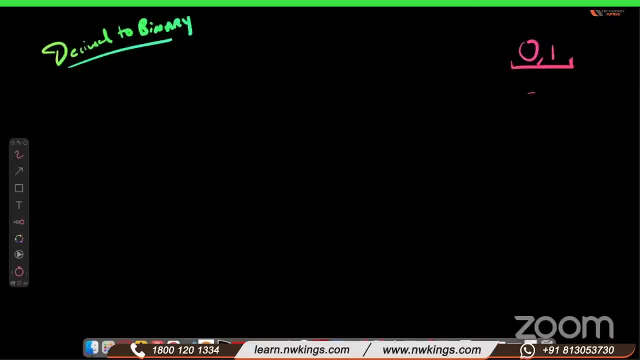 is why in ip address we we always use power or base of two. we always use base of two because these are two numbers. so this is why we always take two number. so now you can understand. so this is ip version four. it is divided into four parts. so ip version four is: how many bits? 32 bits? what is? 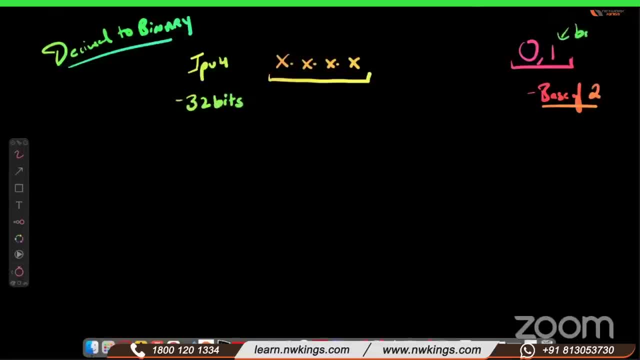 bits zero and one is known as bits, so it means your ip version four is a combination of how many bits- 32 zero and ones. okay, so now an ip address is divided into four parts. so ip version four: 32 bit, 32 bit, 32 bit. 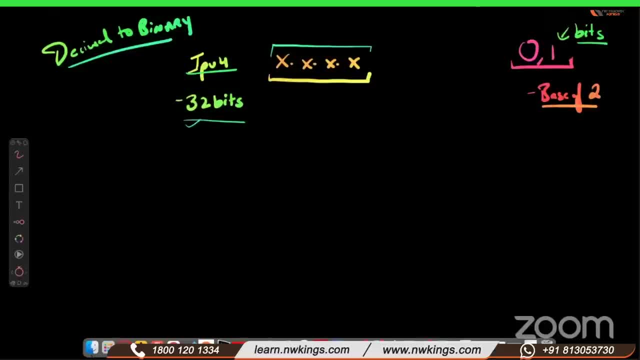 32 bits. it has four parts, which is called okay, because every block is of eight bit, eight bits. you can say that eight bits, eight bits and if you calculate eight into four you get 32. okay, so now two away. So first of all, you should know why we are learning, because we should know how to get the binary. 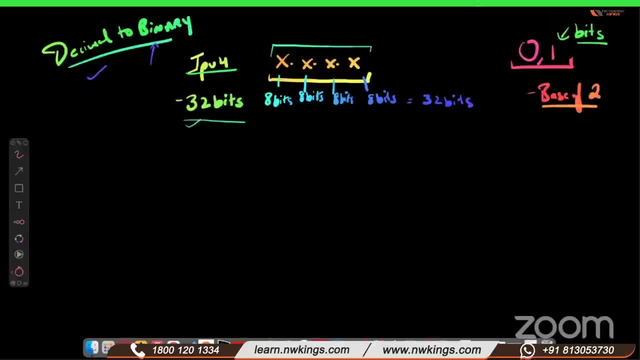 Then we will be able to understand how Ina divided the number So 8 bits. So how we represent 8 bits. So we represent 8 bits with the power of 2, because your 0 and 1 is 2.. 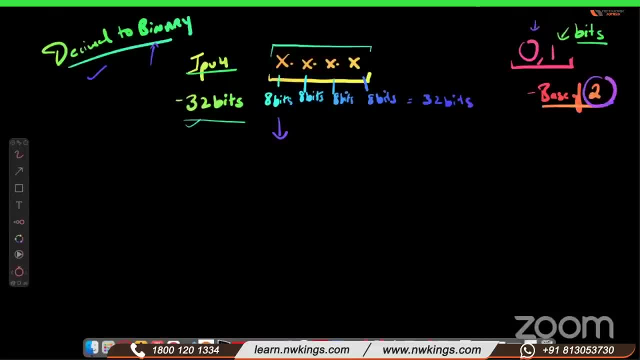 So we always use power of 2.. So how to represent 8 bits? So 2 to the power of 0,, 2 to the power of 1,, 2 to the power of 2,, 2 to the power of 3,, 2 to the power of 4,, 5,, 6 and 7.. 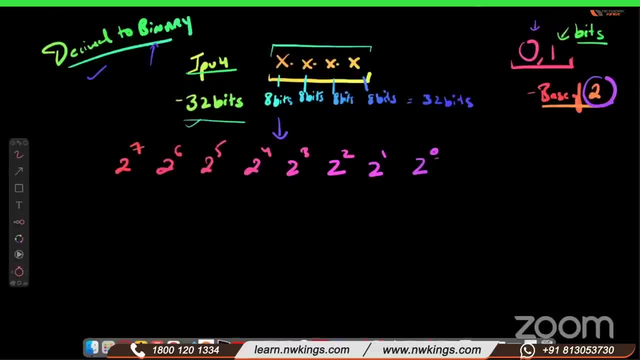 We will not write 2 to the power of 8.. Why? Because we started with 2 to the power of 0.. Right, And if you check the table, 2 to the power of 0 is 1, 2,. 2 to the power of 2, just double the value 8.. 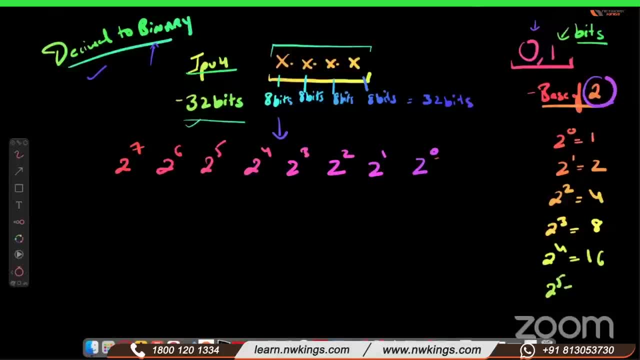 2 to the power of 4 is 16,. 2 to the power of 5 is 32.. 2 to the power of 6 is 64, and 2 to the power of 7 is 128.. And 2 to the power of 8 is 255.. 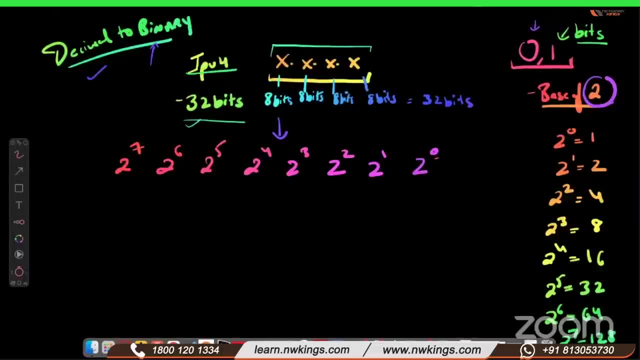 Okay, 2 to the power of 8 is 255.. So you can write these values here like it is 128.. You can write on top also 128,, 64,, 32,, 8,, 4,, sorry, 16.. 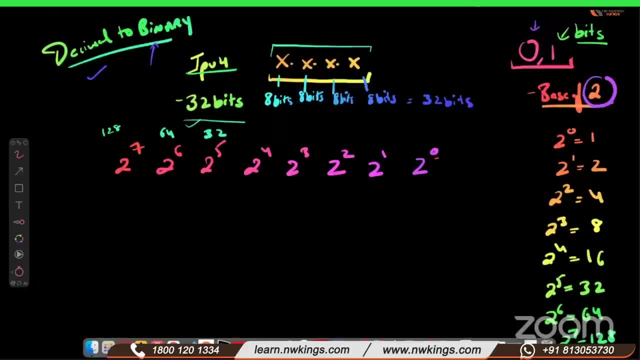 It is left 16,, 8,, 4,, 2,, 1.. Okay, So, please remember 2 to the power of any number. power of 0 is called 1.. Okay, So now how to calculate the number. 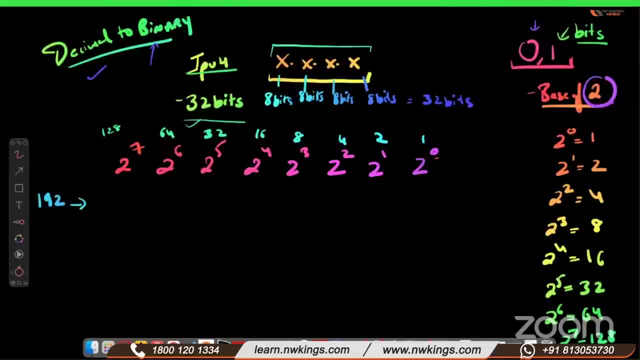 Suppose you want to get the binary number of 192. So how to get the binary of 192? So how to make the binary of 192?? So you can just count: 128 plus 64 is 192.. So you just have to on the bit which is called 1.. 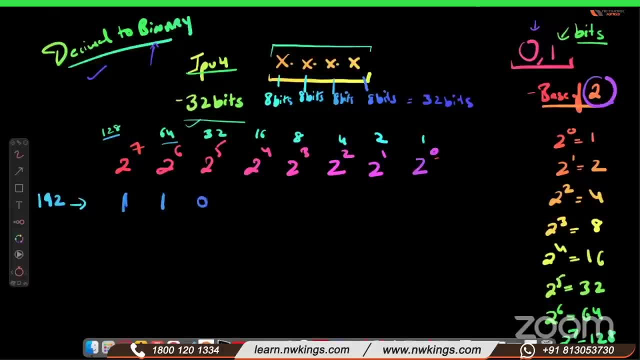 So you just have to on the bit On means 1 and rest values will be 0.. And this will be binary means. your computer understand 192 in this format. Okay, In this format. And after that, if I calculate for, suppose, 192, after that let us calculate for 168.. 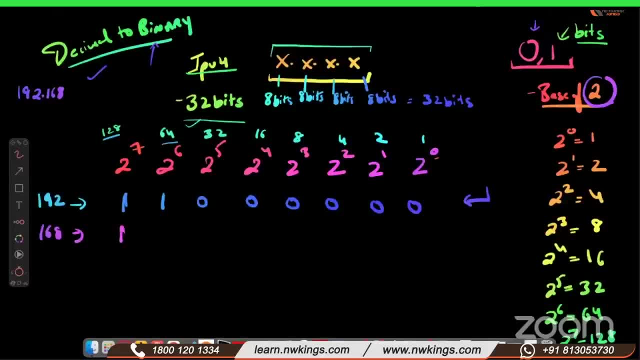 So 168 would be 128 plus 32 is 162.. 160 plus 8,, 168 and rest value 0.. Okay, So guys tell me what will be the value for 10.. And then after that, please write in the chat what will be the binary value of 10.. 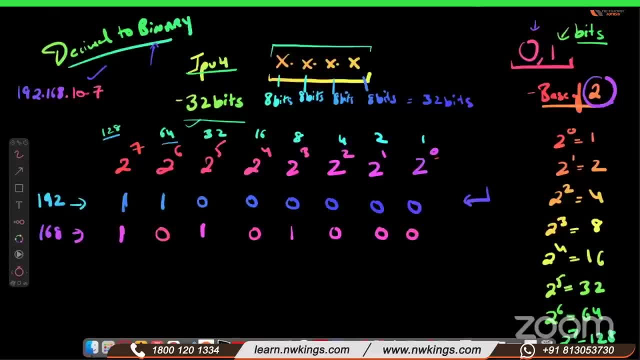 And after that give me binary value of 7.. Suppose this is IP address. So the binary value for 192 is this: 168. this, Tell me the binary value for 10 and then for 7.. Just do it, You have 2 minutes. 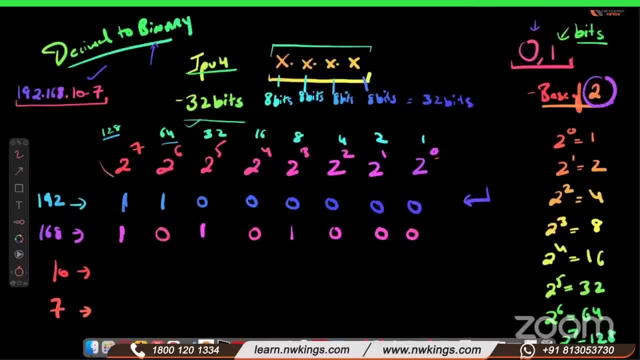 Okay, Okay, Yes, So we are going to plus 8 plus 2. 8. Just see the number here: 8, 2.. 8 and 2 is 10 and rest value 0.. Very simple. 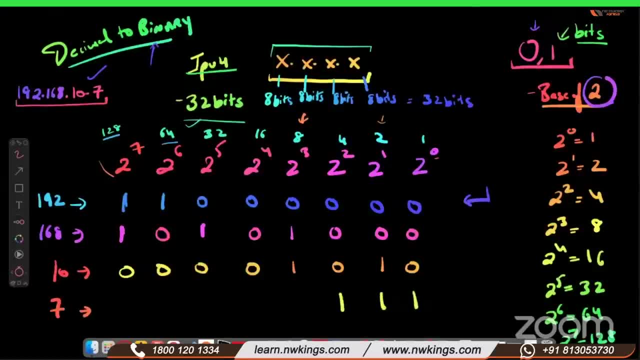 What about 7?? 4 plus 2 plus 1 is 7. Rest values: And that is 3 plus 5. par. That has been the finish of 42 points so far. Zero, Zero. I put 0.. 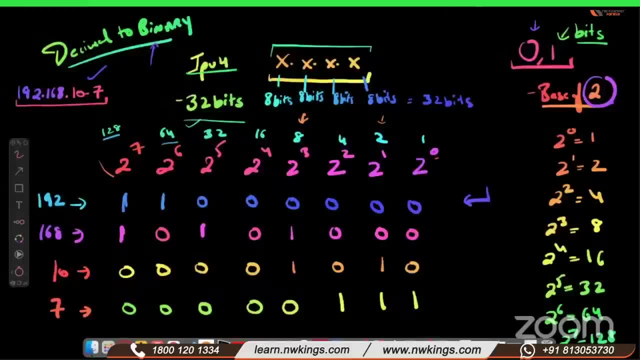 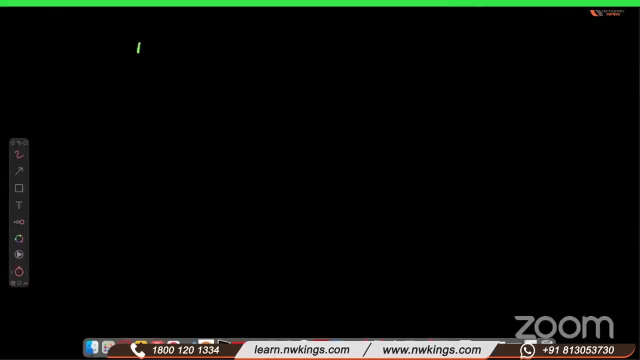 Clear. Yes, Sir, Okay, good, Okay. so this is a decimal to binary. Now the good story: Let's understand how aina divided to this number. In every live session we just write hi, sir. So how Aina divided the number. 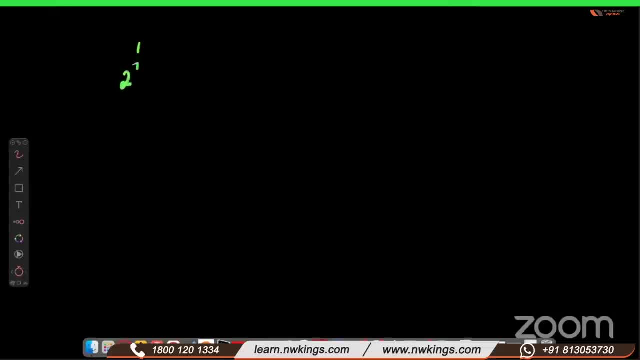 So you can just write down the gain values. 2 to the power of 7 is. So you can write down the number again. So just take into consideration one octet, So you have four octet. So each, every octet is like this: 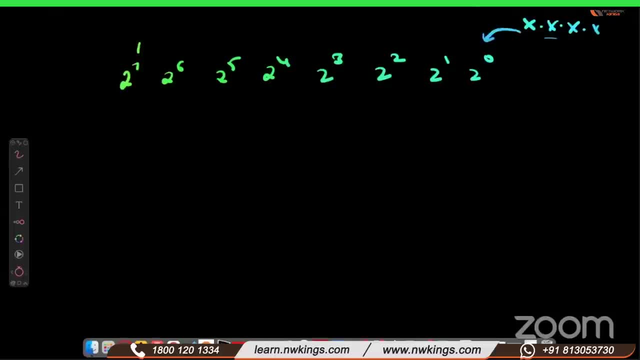 Not just one octet. So this happens in all four. All four octets are like this: This is the calculation. So all four octets have similar calculation. So now you can see 2 to the power of 7.. 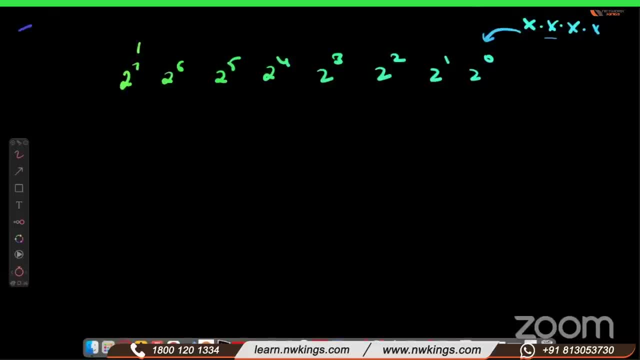 How Aina divided the number system, which is called IP address range. So I have delivered some batches first. So IP address range. How Aina divided the IP address range, So 2 to the power of 7 is obviously 128. 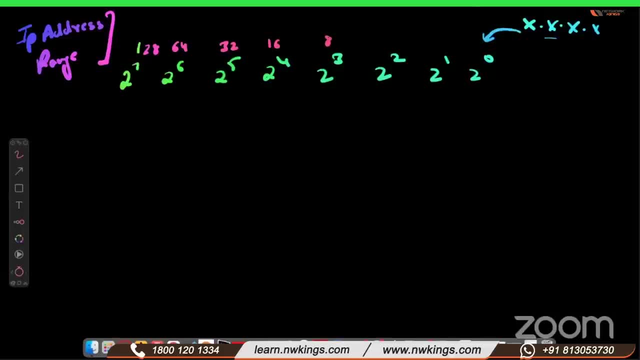 You can write down 64,, 32,, 16,, 8,, 4,, 2,, 1.. Right, So this is the value. So in the first octet, in the first part, you take all 0.. 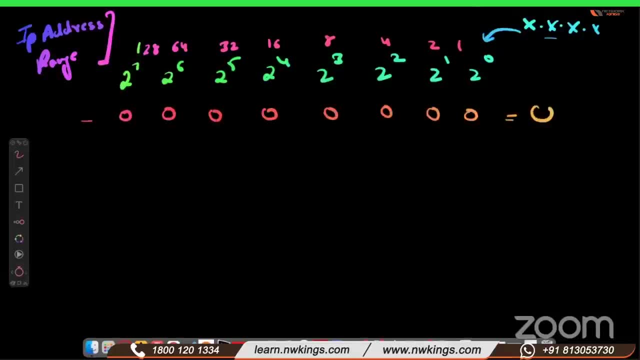 And tell me what will be the value? Obviously 0.. In the second time you have to take 1 here And on 1, you can see there is 128.. So rest value is 0. So see what is above 1.. 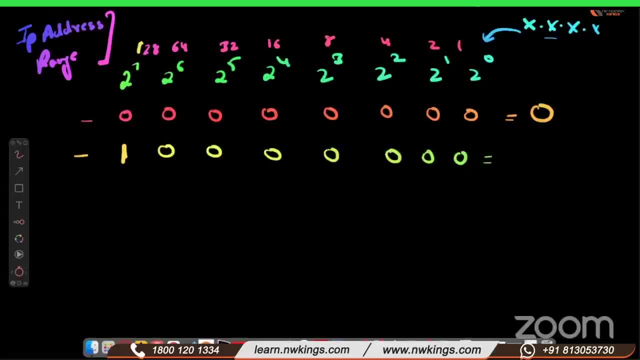 So you can see there is 128.. If you take this 1 only, So the binary of this, this value, the decimal value for this is 128.. And if you take 2 ones, what will be the value? 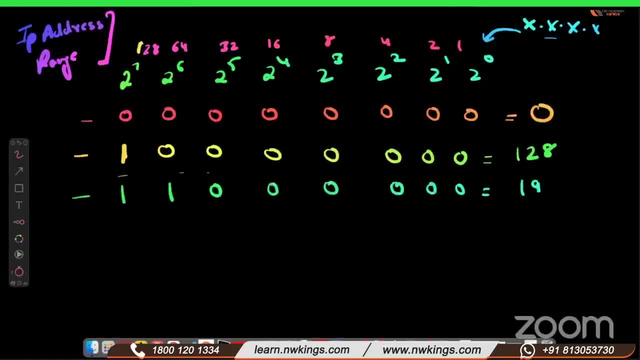 Just plus 128, plus 64.. Okay, Just plus 3 ones, You will be getting 224.. Okay, And then you take 4.. And then Aina thought: let's, it's enough. I think we should not go, because the maximum we can go up to 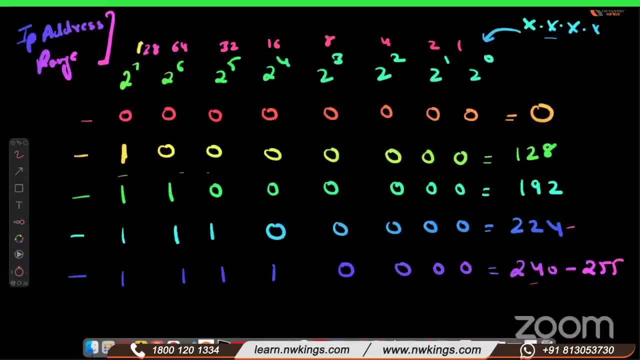 255.. And before 240, we get 239.. Right Before 224, we get 223.. 192, 191.. And before 128, we got 127.. So this is A, class B, class C, class D, class E class. 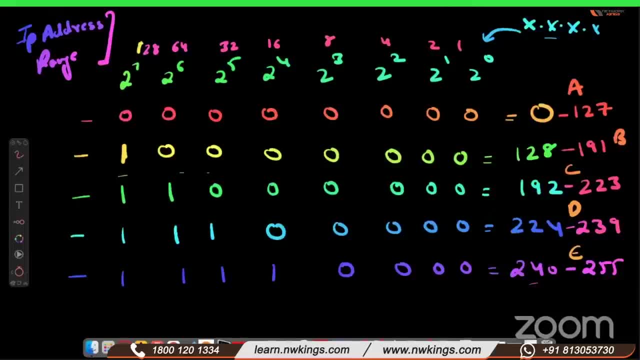 Tell me who was beating me now. Great, Great sir, Great Okay, Got it now. So this is how Aina divided the classes and this is how, actually, we got the ranges. Okay, Cool, Did you understand? Yes, sir. 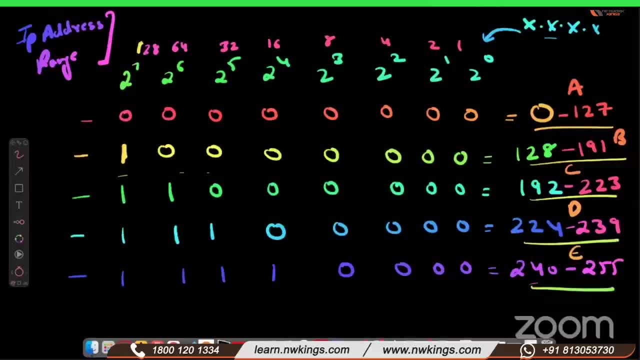 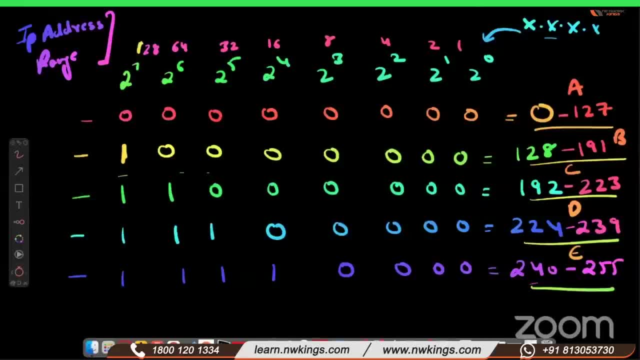 Now you know how IP Address has evolved. Okay, Tell me in quiz time, Like: what is the first step to get the IP Address? Who starts the IP Address? Aina, Aina, IETF, Internet Engineering Task Force, Then Aina. 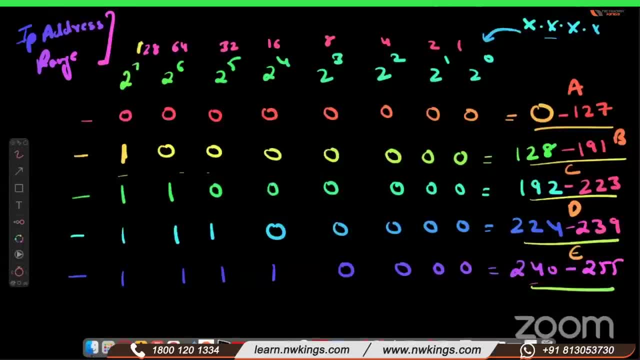 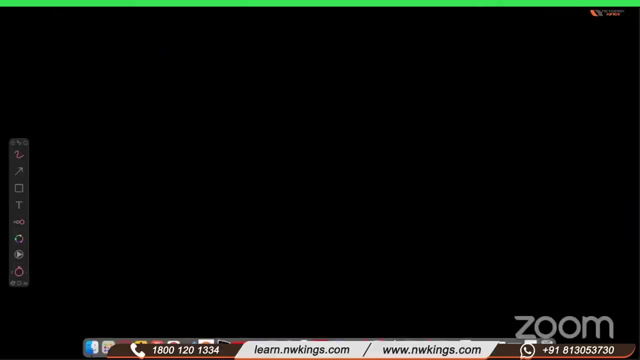 Then RIR Right. Then you get IP. you go Wow. then you get in companies or any network, then user gets right. so i'll share that ppt with you, don't worry, you can just check on that, okay. so now let's go to another thing. now, if we talk about 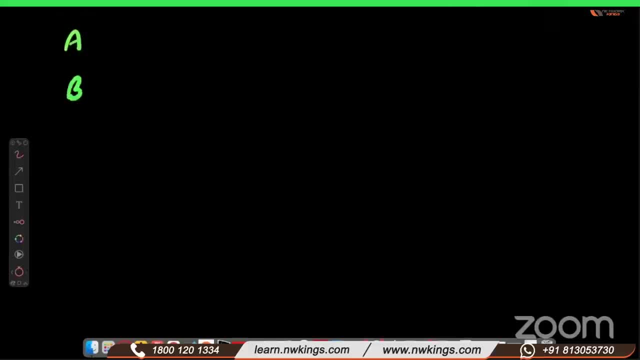 a class, b class, c class- okay, this is mostly we use. we don't use d and e class because, because your computer does not support d and e, d class is used for multicasting, like routers using some uh like, if you have done ccna or not, i don't know, but if a router wants to share their 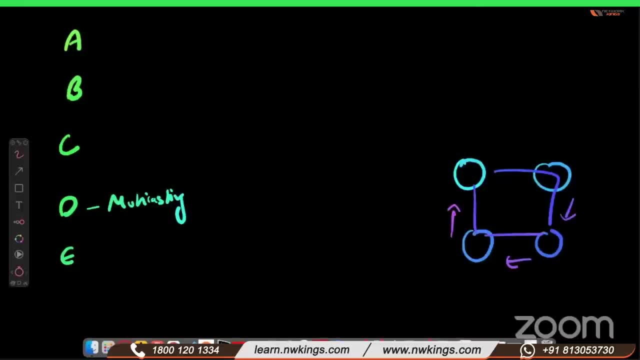 information with each other, mostly routers. uses multicasting, like there is a protocol called rip. it uses two to four: zero, zero, zero, zero, nine something. okay. eigrp uses two to four: zero, zero, zero, nine something. okay. eigrp uses two to four: zero, zero, zero, nine something. 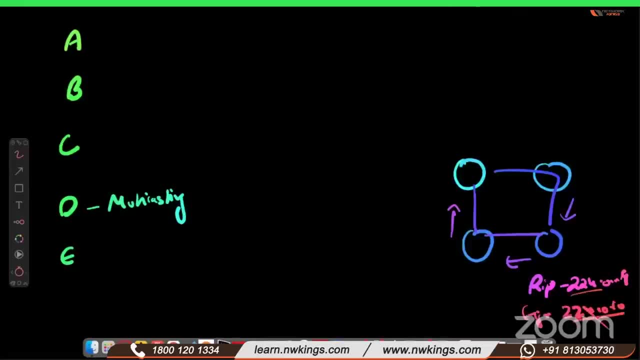 four zero zero zero ten. so what is this? this is the ip address of some protocols which are which you learn in ccna or ccnp, so that routers can share information with each other. so this is called multicasting. so your computer don't understand this language, so this is called multicasting. and e is used for some in most of the books you will. 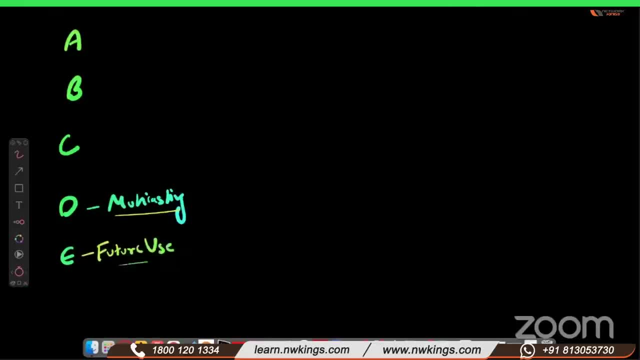 see future use, but from last 20 years all books are saying future. so what future they are talking about? actually there is no future use, it is actually wasted. why? because not even a single computer or operating system like windows machines. if you try to give any ip address above 223, windows is going to give you warning that you can't. 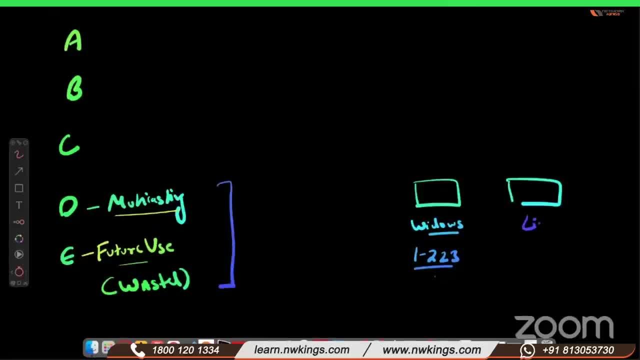 use d and e in windows also, in linux also, you can't use a, d and e. you can't use in android phones, you can't use in iphones, mostly, like all hundred percent of the time. you can't use d and e for 100 devices like you can't use d and e. now tell me, even if we have a, 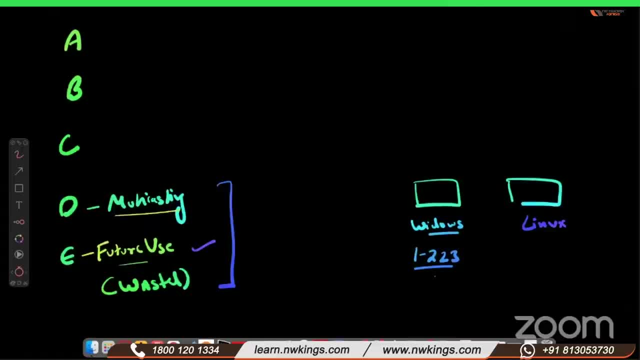 e-class how we are going to implement, because not even the old machines, not even the new machines can't understand e-class. hello yay, don't sleep. so Yes, guys, Yes sir, It has been wasted because no operating system supports it. So from where will we do it? 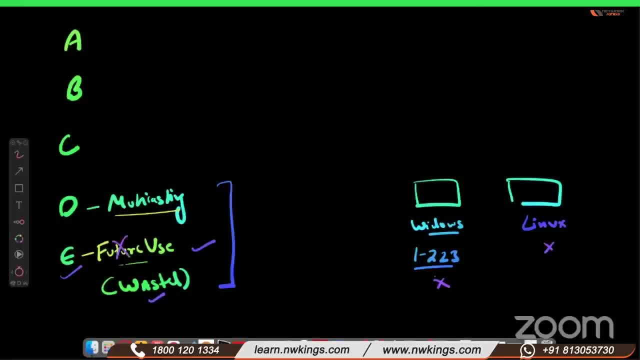 Its future has gone. There is no future, Obviously right? Yes, Yeah, that makes sense. Okay, So this is why we can't use E class and D obviously is reserved for routing and all. So we can only use: 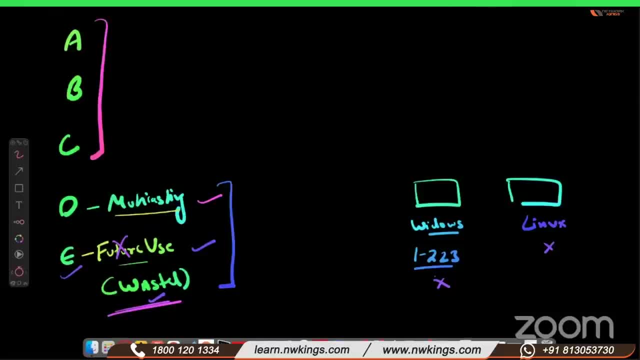 A, B and C. Okay, So let's understand A B C, Why we have A B C. So in all IP address, in IP address version 4, even in version 6, you have 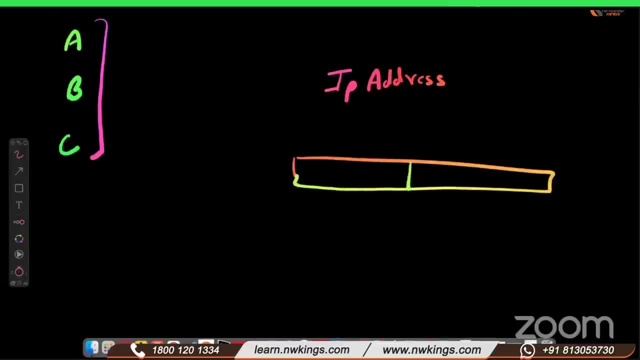 two components or two parts. Every IP address divided into two parts. One is called network and one is called host. So if two machines wants to speak with or want to communicate with each other, your network portion should match. then only they will able to. 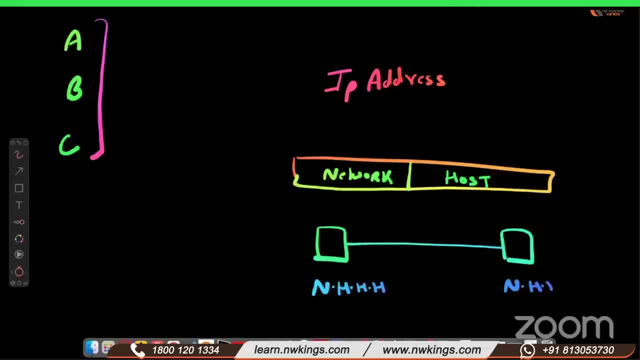 share the information. If your network is not matching, it means the computer won't able to communicate. So for example, like your class A has one octet network and rest part is host. So what does it mean? So if you? 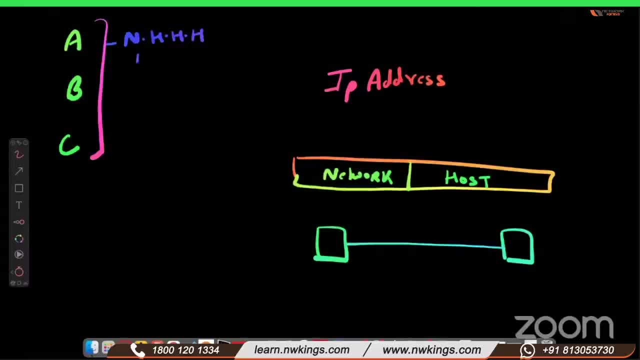 use a class A which is like the range is like 1 to 126, 0 and 127 is reserved. So if we give IP address like 1.1.1.1 and if you give IP 1.5.7.8,. 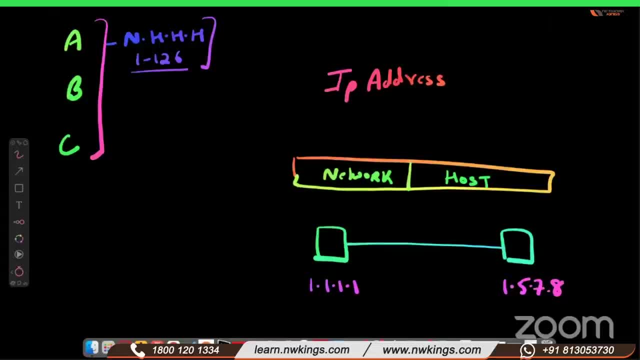 so tell me if they will be able to communicate with each other. Yes, sir, Yes, because class A only checks the first portion. This is network and you can see both. the network is matching Yes or no, The same digit, both. 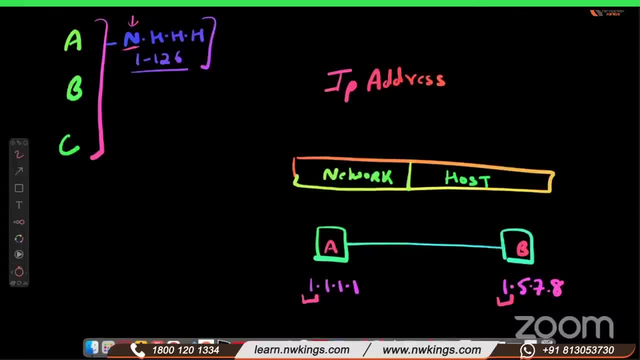 the end: Yes sir, Yes or no. Yes sir, Both the sides are matching right, So it means it is in the same network. But now you understand right. Because you are human, you can understand my language. 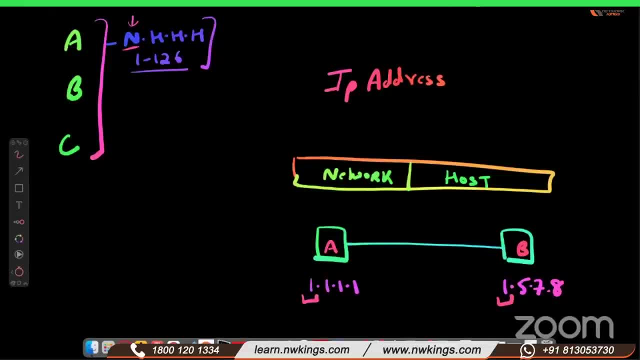 You are able to understand my Hindi English whatever I am saying, Right? But how computer will able to understand that? this is my network? So we call: we use a subnet mask. So there is a number called subnet mask so that we 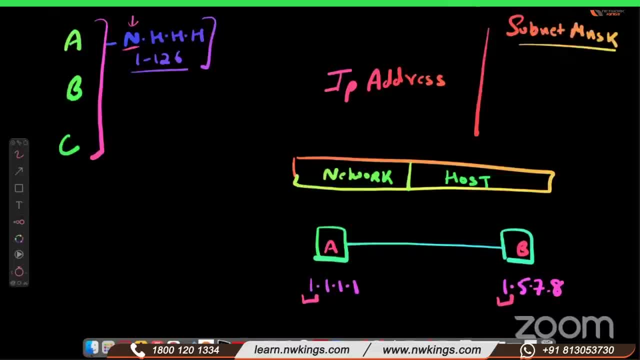 can inform our computer that. what is your network part? Okay, So if you write 2, 255.0.0.0, 255.0.0.0, 255.0.0.0, So what does it mean? 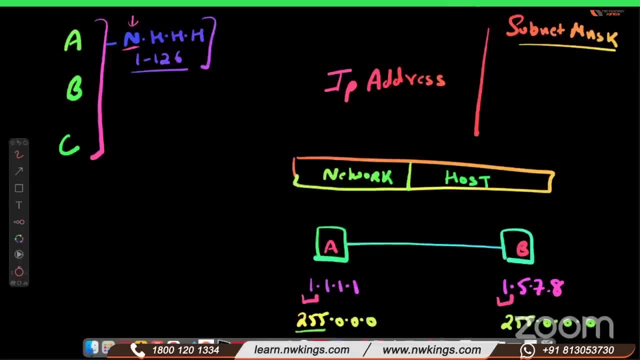 So it means just 255 means like first 8 bits, is it? you have to match. So means the first octet of the beginning. So first octet 255 means you have to match the first octet You have to match. 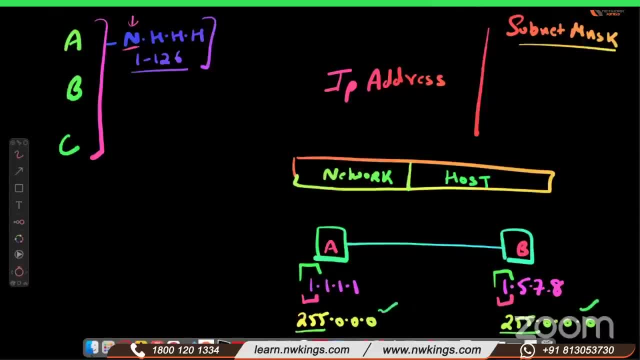 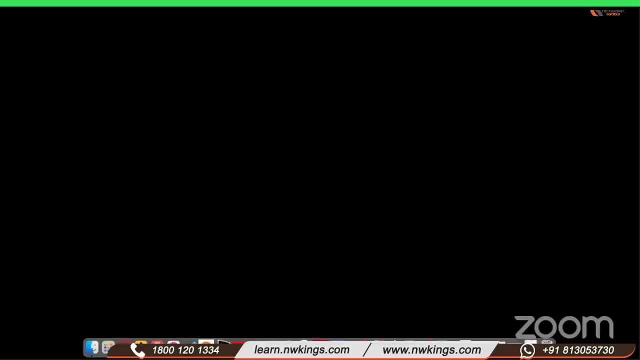 the first octet. This is how you give IP address to a computer. Okay, So let's understand how to give IP address to a computer. Let me share. just hold on, It's very simple. I am sure most of you are advanced learners, but still. 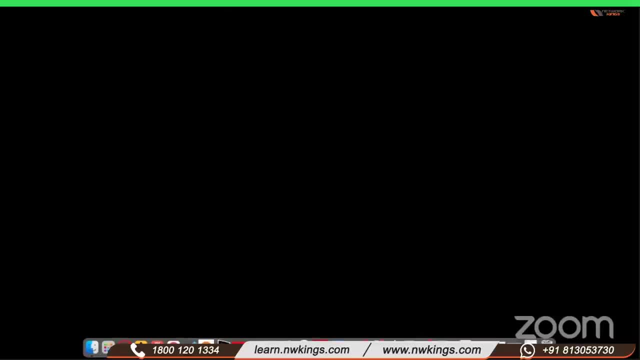 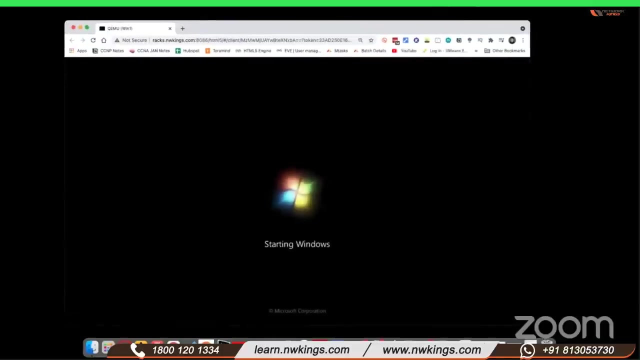 I don't want to, I Okay, So just hold on. Okay, So I just started a Windows machine here, So it's very basic how to assign IP. Okay, So in Macbook also you can assign in GoToSystem. 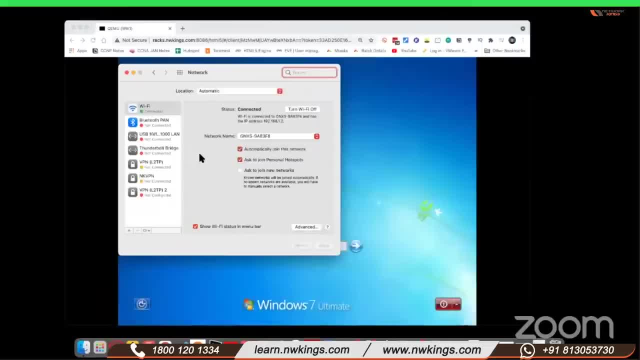 and there is a network and you can see on the advanced part and it go to TCP IP and here you can give the IP address, You can use the manually IP and you can assign all your IP, whatever IP you have. So you can see. 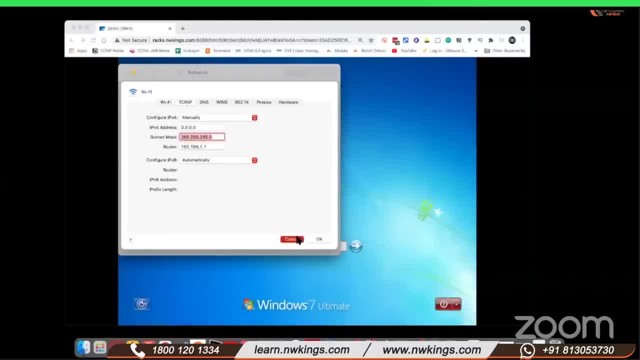 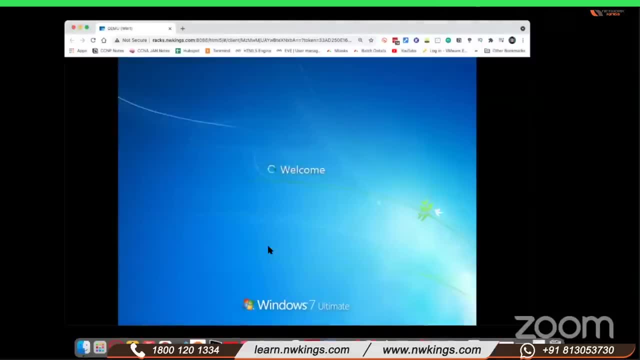 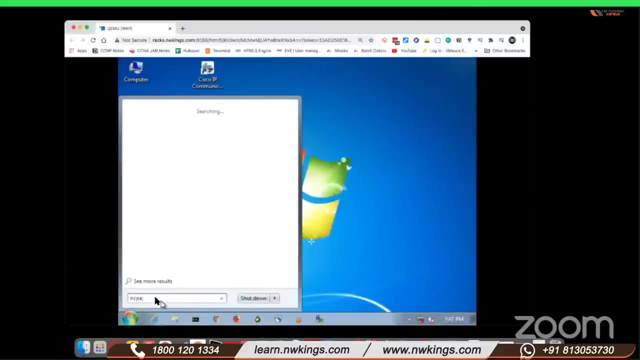 there is a subnet mask here. So this actually tells what is your network part. So this tells you the network part. So let's see the Windows, because most of you are using Windows. So there is a shortcut: directly go to ncpacpl. 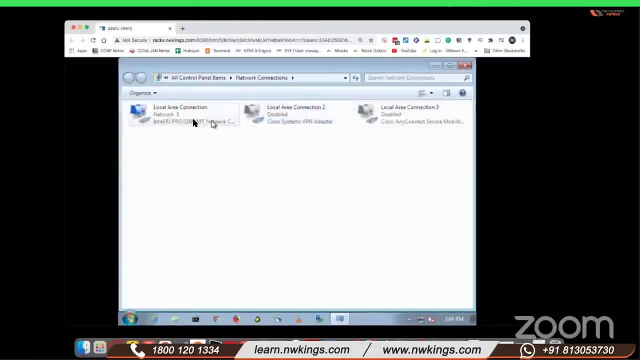 Okay, So you can go to ncpacpl or you can go to control plane. control plane, sorry, control panel. So control plane is like we have in routers, So control panel network connection. So this is the my ethernet adapter. 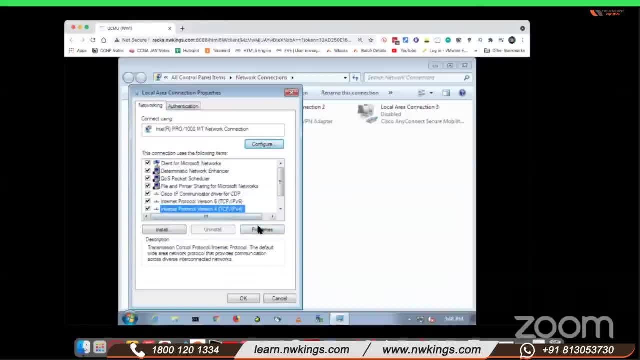 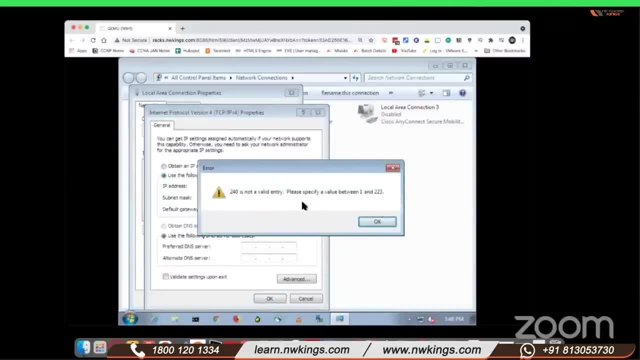 properties. Click on IP version 4, Go to properties and you can see So whenever you try to give any IP like 240.. So you can see the system is giving you a warning that you can only assign IP from 12223.. 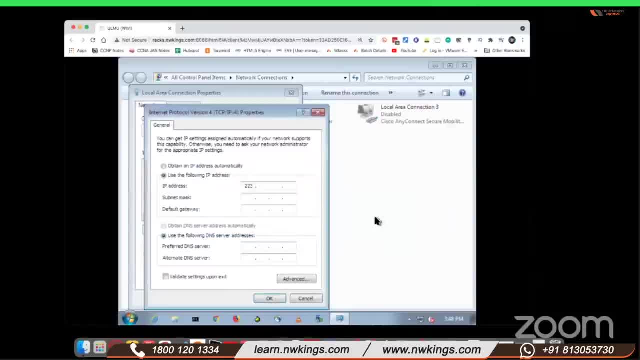 It means you can only use A, B and C. Okay, So suppose if I am going to give 1.1.1.1 and if you click here, automatically, system is taking 255.0.0.0. So this is called by default. 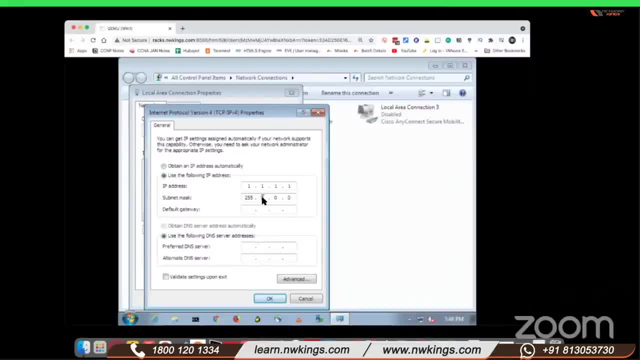 subnet mask. So somewhere might be you have seen 255 here also, or maybe like this: Even this is class A, might be. you guys have seen different subnet mask, or maybe like 128.. So what is this? This is what we call subnetting. 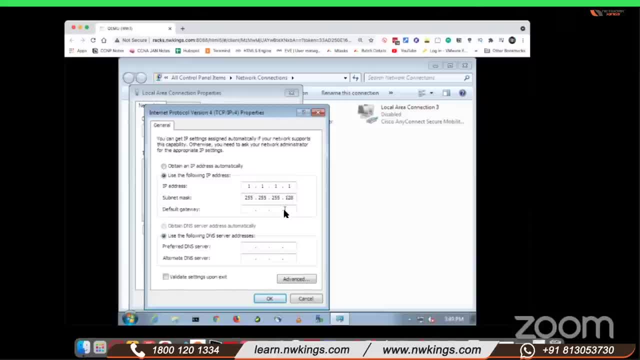 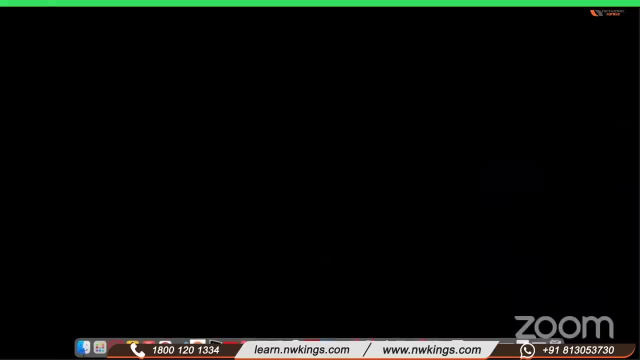 which we are going to learn, and this is why we have conducted this workshop. Okay, So what do we need to know now? So what is this subnet mask? I will explain that subnet mask, but you can also understand this. First of all, we need to understand. 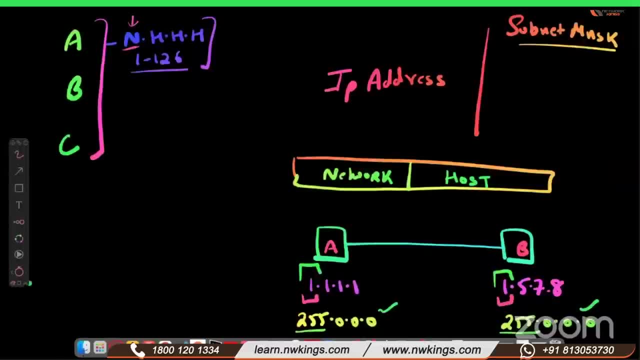 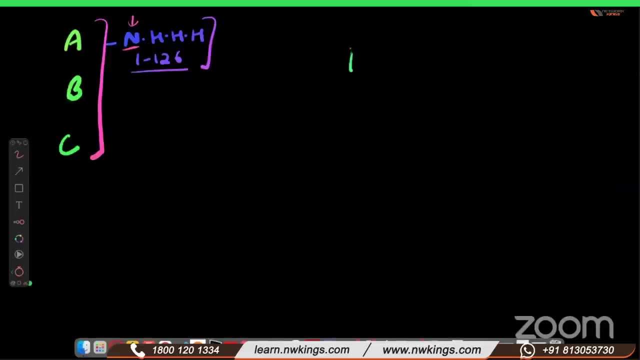 like: what is the difference between A, B and C? Okay So let's take one example of class A. Okay So if you have two computers or two servers or any device? Okay So let's take example of class A. If you 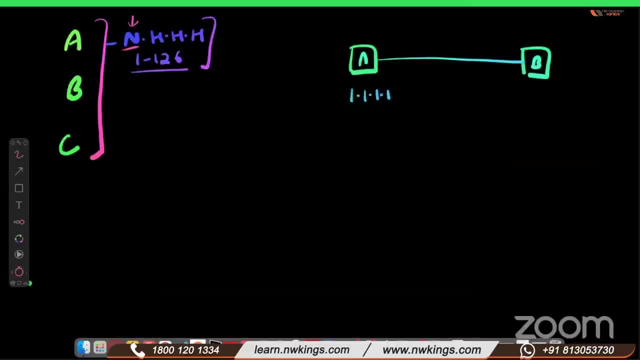 have IP. I have already given example 1.1.1.1 and you have 1.100.1.. any IP but computer only checks the first part and it means they will be able to communicate with each other if they use class A. 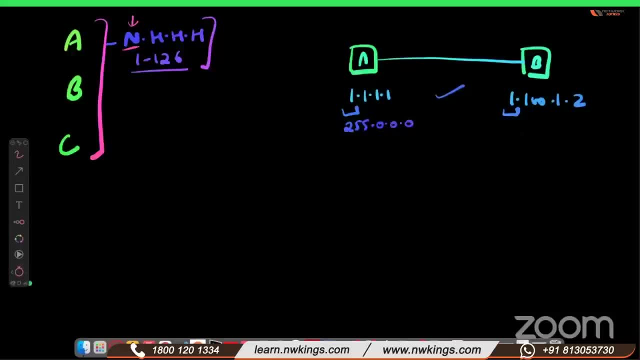 with this subnet mask. Right, Okay, Tell me the same IP address. but if I am going to use 2 times 255, it means you have to match two subnets, So will they able to communicate in this case? Check karo, kya do part match? 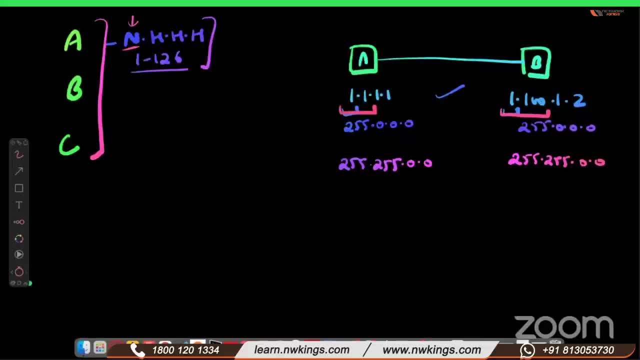 ho rahe hai. So two parts are matching. No, sir, It means they will not able to communicate if we will be putting this subnet mask. So this is called. so this by default. this is called by default. So in networking, we call this. 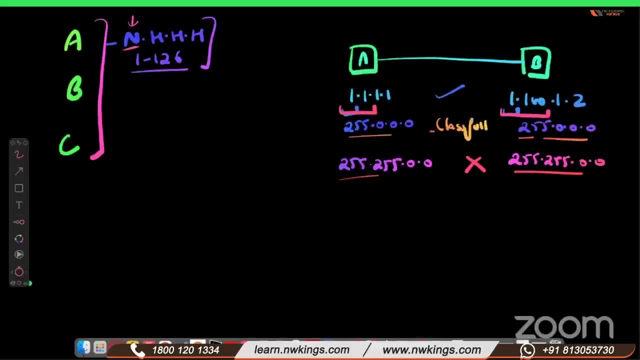 class full. This is called class full because this is by default Okay, And whenever you change the subnet mask- because this is class A- by default is 25500.. But if you use some different one, which is not default, this is called classless. 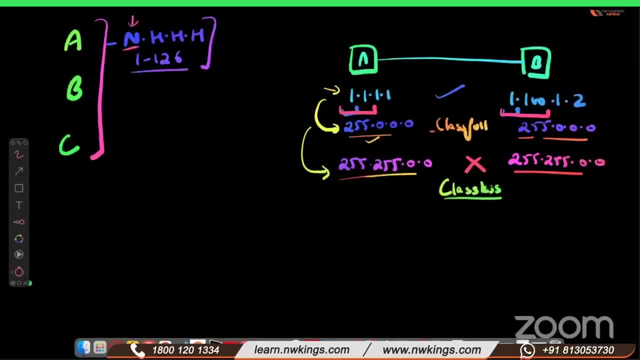 What is this Class? Classless? Yeah, Got it. Yes sir, Yes sir, Clear everyone? Any question? No, sir, Okay, So let's talk about B class now. If you have two another computers, but here we are going to assign one. 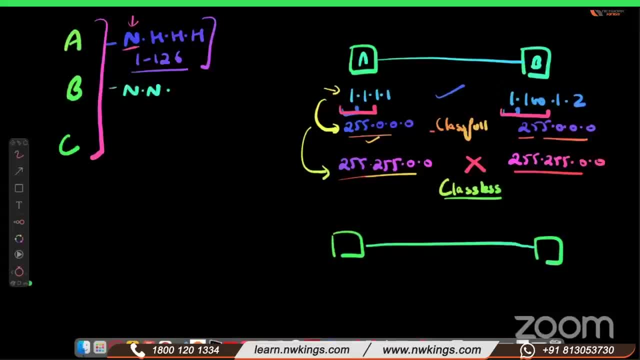 B class IP where we have two network part and two host part. Remember we have two network part, So range is 128 to 191.. So any IP address start from this range. Suppose you have 150 IP and you have 150.1.2.3.. 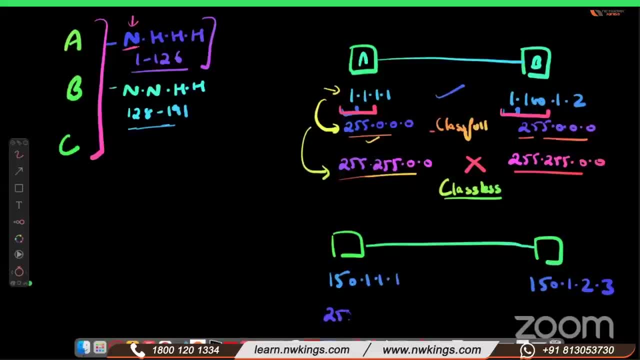 So tell me, with, by default, a subnet mask, by default subnet mask is 255.0, because you have one network part, So you have two network part. so by default, subnet mask will be 2 times 255.. And C will be 3N. 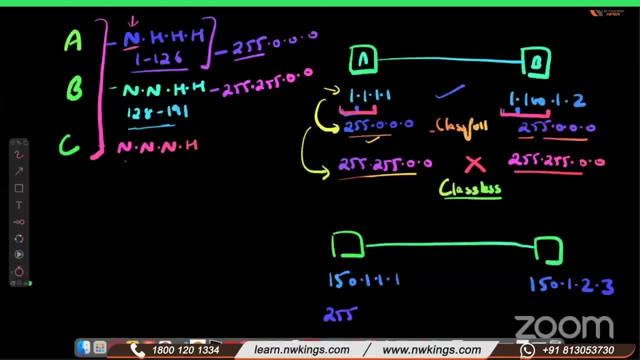 and 1H, Sorry, Okay. So 3N means 3255.. So this is by default subnet mask. Okay. So, remember guys, A class IP, A class IP address, by default is this, but when you go in your production networks, or maybe you go, 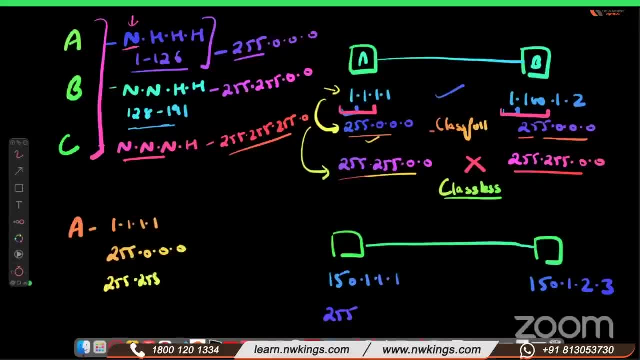 for any company, maybe have this subnet mask. Okay, So this is not wrong, This is also correct, but they have divided their network into some different parts. So this is not B class. So I have seen people ask me or student ask me. 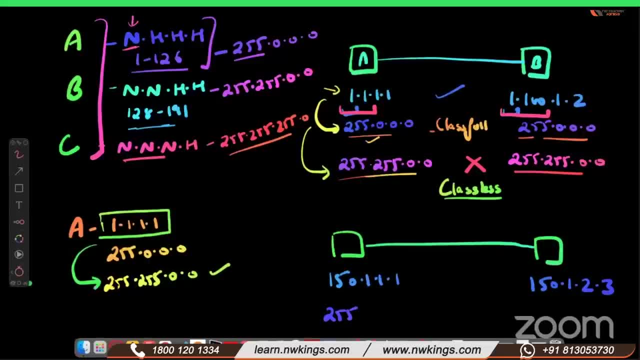 this question, Sir, this is class A, Why you have given this B class subnet mask. So remember, guys, this is not B. B has not registered this. Okay, So this is not B class, So this is default of B, but this: 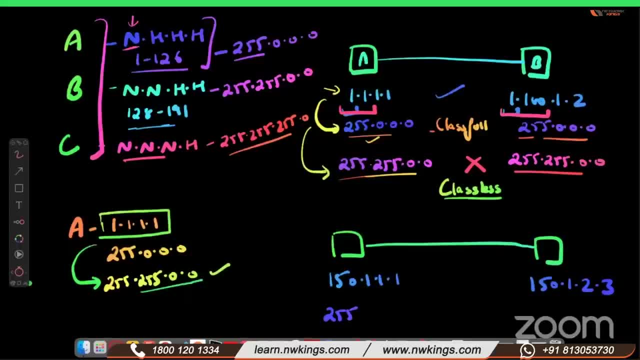 does not belong to B. All classes we check with the first IP address. We check all classes with the number, with, not subnet mask. Okay, Don't do this mistake. We always check the number to check. this is class B. this is class B. 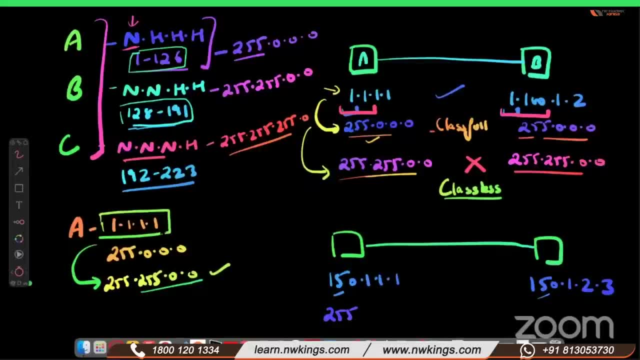 But whenever you see subnet mask, it can be of class A, it can be of This, can be of anyone. Okay, When we will study subnetting, even you might have 3 times 255, and remember this is not class C, This is class C default. 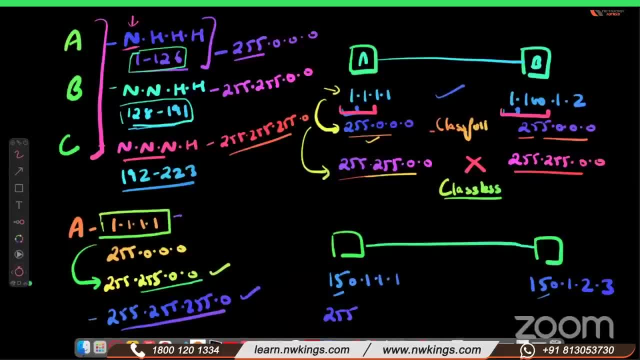 but when you give this IP address to class A IP, so it does not make this IP address class C, It is still class A. We have given subnet mask to class A separately. Okay, But I understand that we are making a mistake here. 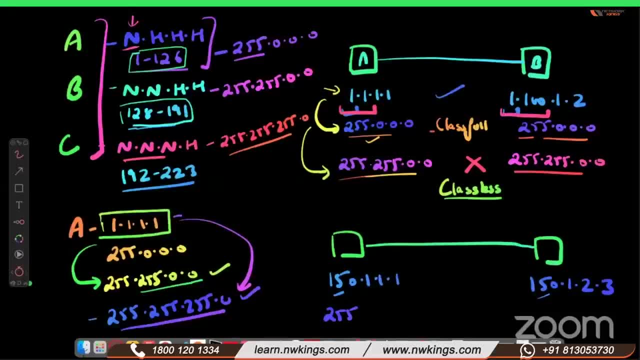 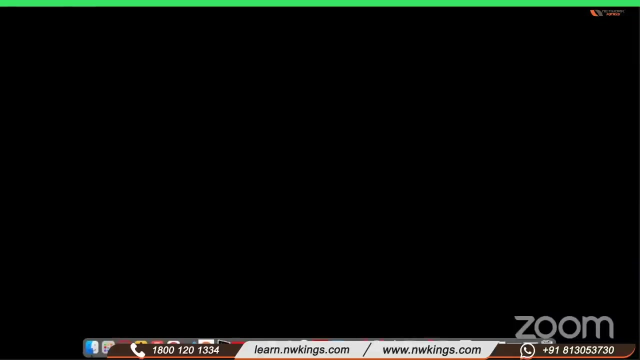 that's why I am saying this again and again. Okay, Hello everyone. Yes, sir, Will someone repeat for me What did I say? Yes, Yes, anyone Here? anyone why? how you are going to face interviews man? Yes, sir, Tell me. 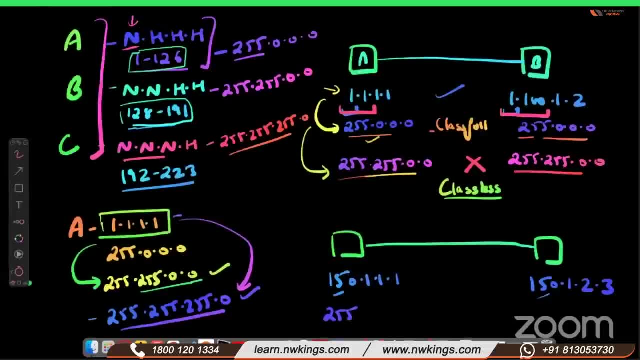 ematics, Tell me what I explained. There is a class in 3 types of ip address we are using. so that is a, b and c. so ip address will be defined on the net data network. yes, network. so we check ip address only by network, their network portions: yes, right. 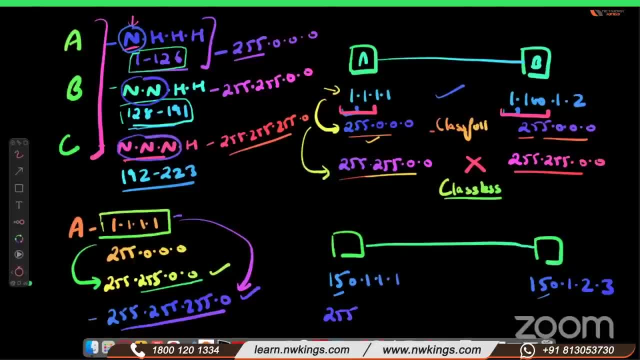 what we check from network portion, that they are able to communicate or not. yes, okay, now if i put two five five, two five five dot zero dot zero, this is by default. so definitely they are going to communicate with each other, yes or no? right, because you have two. 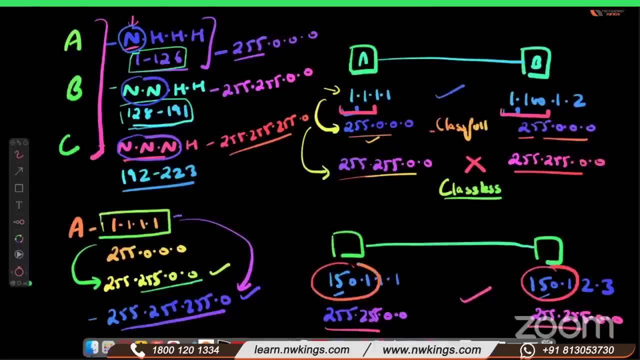 two five five, two, two five five and both 150.1. same in both the cases. right, so it means they will communicate. but if you put different subnet mask, then accordingly they are going to communicate. okay. so let's take example of a last computer class, what we call c class. 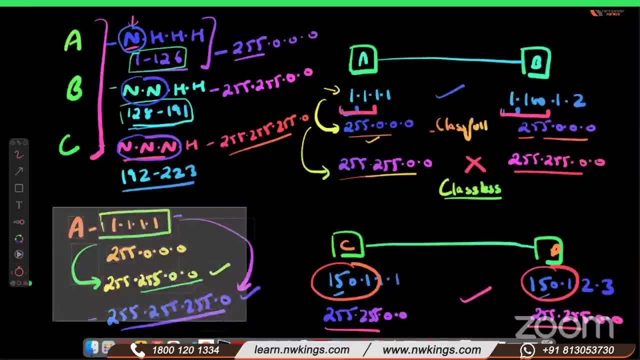 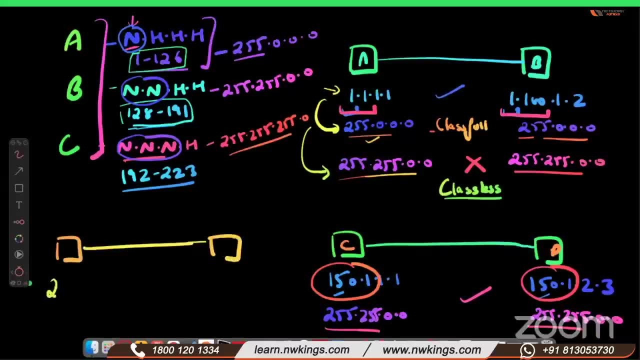 so i shall remove this. okay, so let's talk about c now. if you have two machines and one ip address is 200.1.1.1 and 200.1.1.3, so tell me if they are able to communicate. yes, i have not given the subnet, so without subnet mask you can't say: 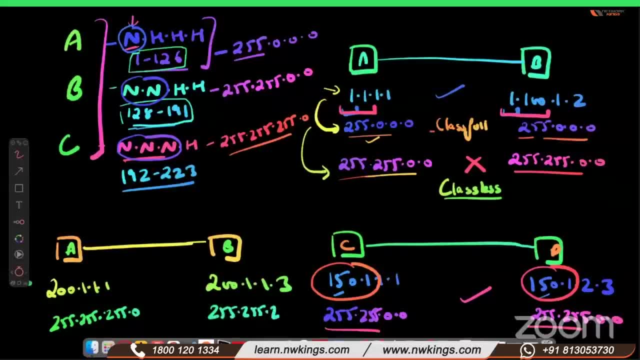 yes, okay. so three times two, five, five. now you can check. this is by default, so i am going to check my first three digits because i have three, two, five, five. so your subnet mask represent network bits. what i said. your subnet mask represents network bits. subnet mask. 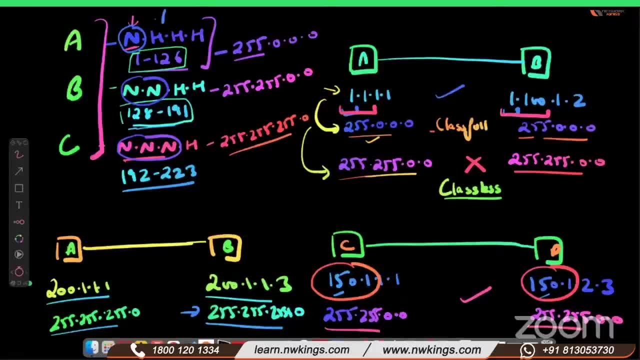 network bits, because this is normal language we can understand. okay, it has one. but how computers understand like this ip belongs to which network. so just count the 255 ip address belong to this network, and here also three type 255, so you can see network. is this? now you can check and compare. 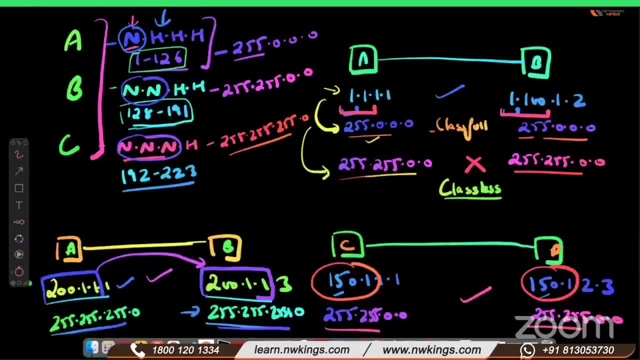 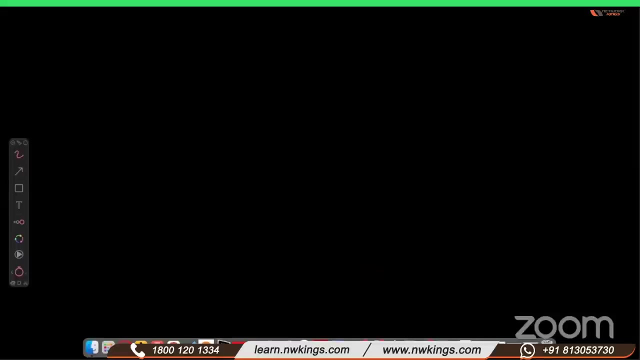 yes, our network is matching. it means we will be able to communicate okay, so. so let's discuss about why we divide our network right. so this is normal ip address and a class, b class, c class, so you should understand. network part was n and host was very three parts. 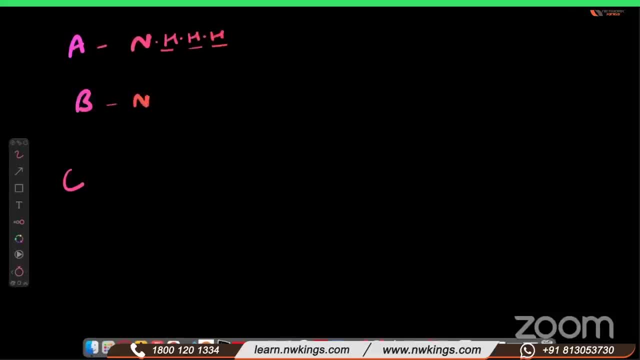 so every octet is how many bits? okay, so you have eight plus eight plus eight. it means to the power of 24, right? so you know when you give ip address with class a how many ips you get: one, six, triple, seven, two, one, six. so it's a very big number, 16 million ips you can assign from class a. it means 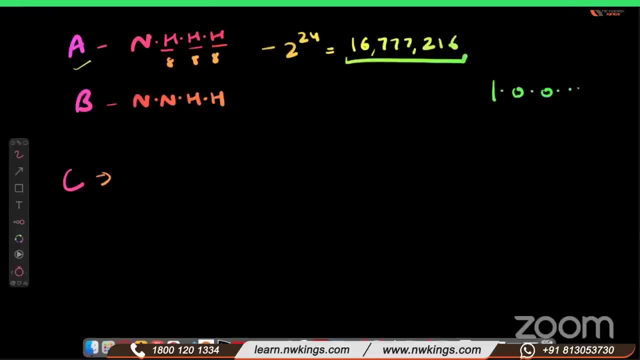 if your ip address start from one dot, zero, dot, zero. this is the starting ip address. so, like your timer starts with zero, zero, zero, zero. right, so it's like one zero, zero, zero, because this is class. a network is same and network will remain same at the end. but this host would be. maximum value is will be 255. 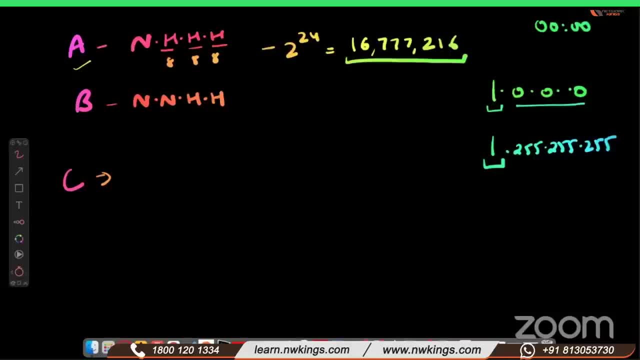 so your maximum value is 255. why? because you remember the table, right? yeah, then a table, yes, yes. so if you calculate all the values like 128, 64, 32, 16, 8, 4, 2, 1, right, yes? so if you get so, you get 255, and if you make all values 0, you get 0. so this is why. 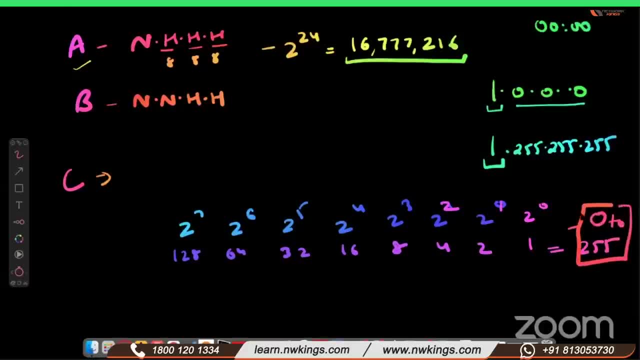 all groups are from 0 to 255. so 0 to 255, remember now understand. so 0 say 25. this is the minimum, this is the maximum and all. so this is the range. so how many computers or how many ips you can assign this much? 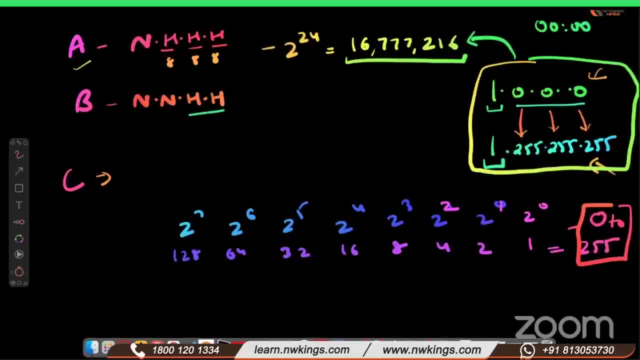 got it. so now if you check b class, you have 8 plus 8, 16, 2. the power of 16 is 65 536 ips. so if your company is around 50, 60 000 or maybe that much team members, you can use class b, but if you are, 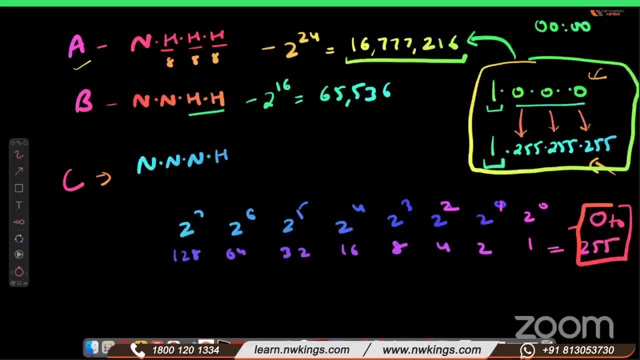 a home user, you don't need a very big number. so to the power of 8 is 256. so now your ip addresses belong according to users. okay, suppose i have 500 users, so i'm going to use b class or maybe a class, but i can't use c class because it only gives me 256 address. 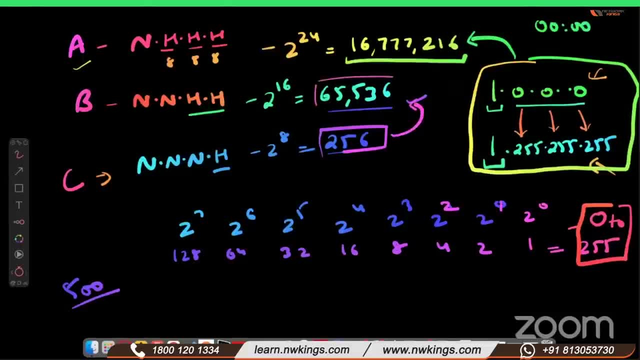 you have to jump on 65 000 maybe if, like, if you have done your college, so mostly have might be. you guys have seen 172 in colleges, campus mostly. but when you join any big companies they mostly use a 10 series, something like that. okay, totally depends company to company, clear, yes, everyone. 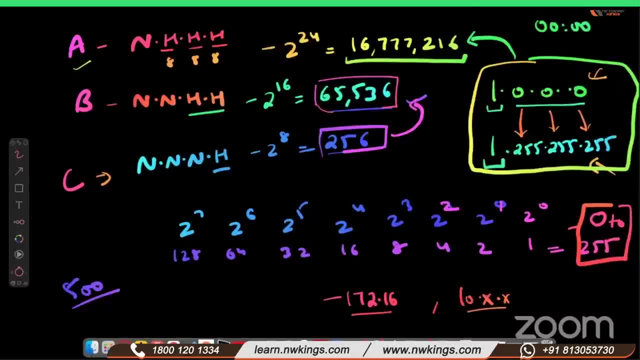 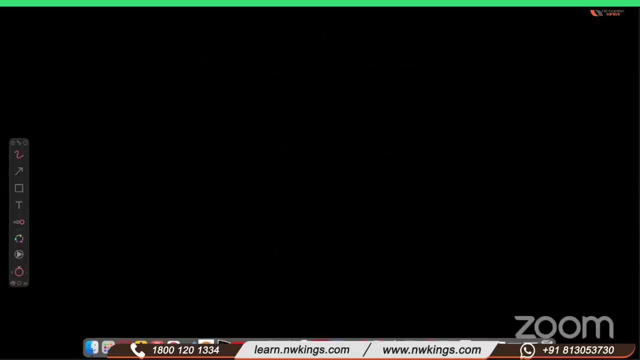 yes, sir, yes, yeah, yeah, okay, good, any doubt? okay, good, okay, this is basics. okay, so some scenarios. i'm going to tell you okay, so, uh, even though it's not a router class, but still i'm telling you: see, there is a company. okay, so generally we use a router. so why we use a router? so that your computers will be. 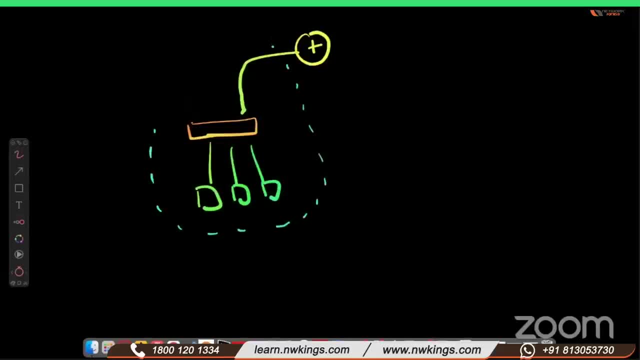 suppose this area is your branch office in delhi or delhi. okay, so 192, 168 dot 1.0, 24.. so what is 24? we generally use a class a has one network part, so we call him slash eight has two network parts, so what we are going to say? slash 16. yes, so c has three network part. 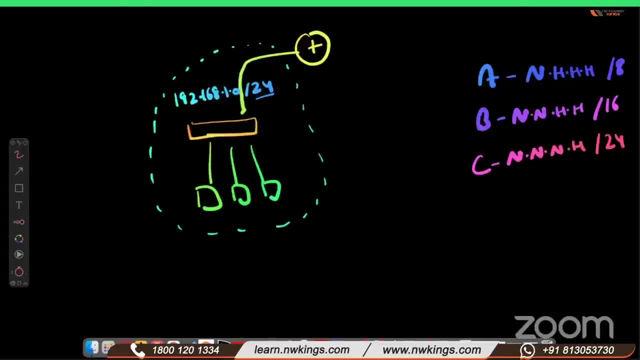 thank you, so we call 24. so this is also called c idr- classless inter domain routing. okay, so this is just a fancy name. you can call this slash value. that's it. so you can call this c idr also. okay. so now, if this is slash 24, obviously this is. 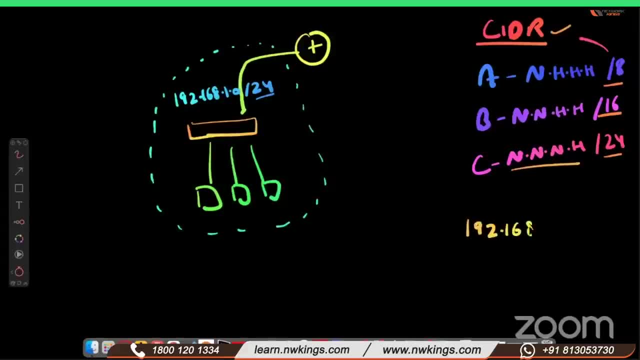 class c. so if ip address- tell me if ip address start from 1.0, so your network will not be changed, yes or no, the network change. right, so the ip will go from 0 to 254, 5 right, so the total ip address you get is 256. right, so you have another office, maybe somewhere. 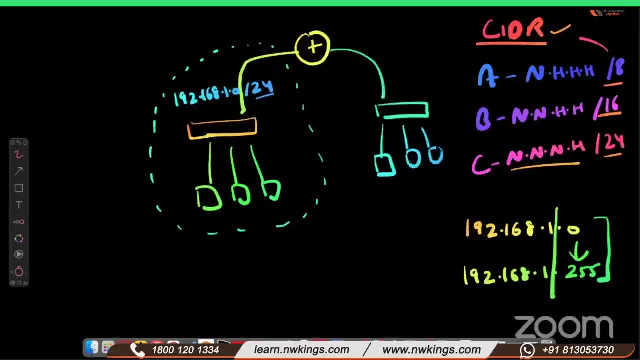 in a different location, so might be this side. you are using some 150 because it's a very big office. it has many user or maybe thousands of user. on here you are using slash 16.. okay, so it means this is a different network. this is also different network. so we use router device. we use router so that you will be able. 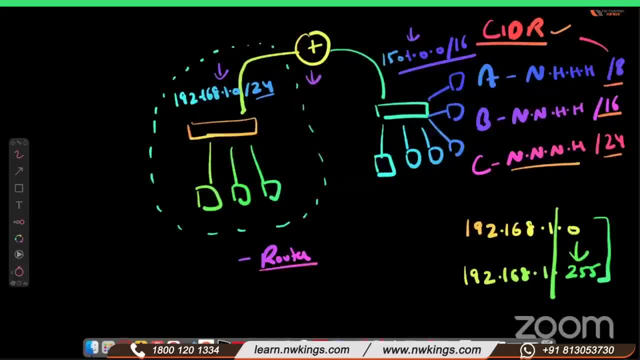 to communicate with the different network. so why we made router, why internet has a lot of big, big routers? because router is a device which is used to connect, to connect two or more different network. okay, so, guys, now you understand why internet big routing, internet table, like why? 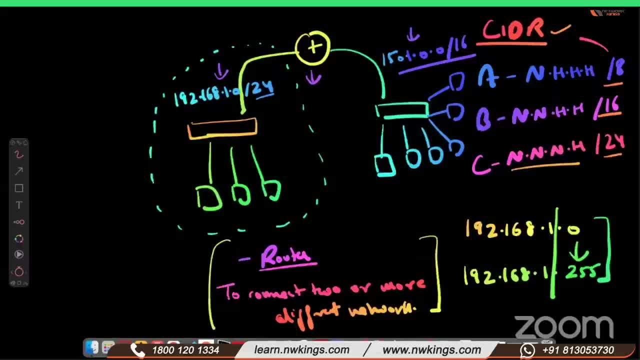 we have routers everywhere. when you get internet connection at your home, when you get internet at your office, when you get anywhere. you need router device. mostly that is a big problem because it has Zip Code which has 2 important rules. you need a USB port. this is the secret. 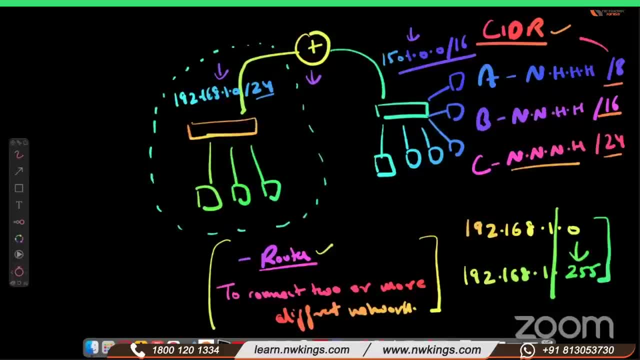 that is another great feature. so what kind of use of router take it to internet connect? the internet cannot be connected into cell hole. now you have a network hi. internet is different why? because you are having different wel and internet is different network. all networks are different and network is known as Internet. 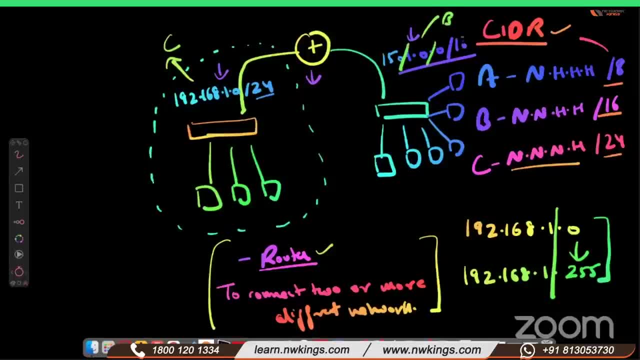 does everyone understand? Yes, sir, Yes, Sir. So router is required. So 192 168 5.0. Now you can compare 192 168 1.0.. So I told you to match three networks. So if you match three network with another IP, 192 168 5.0. 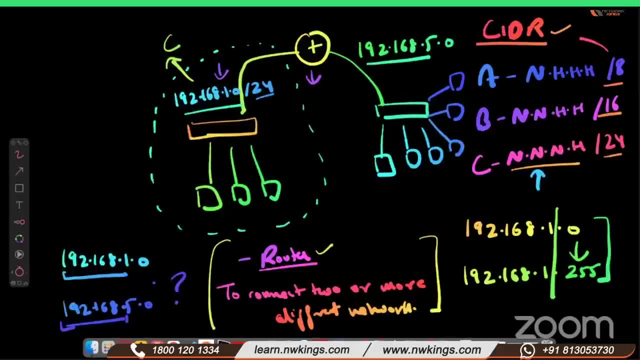 So we can able to match. No, sir, No, When we will not able to match, it means we need a device which is called router. Got it? Network engineers learn routing, router routing, Okay, whatever we do on router. So every network engineer should learn about routing and router. 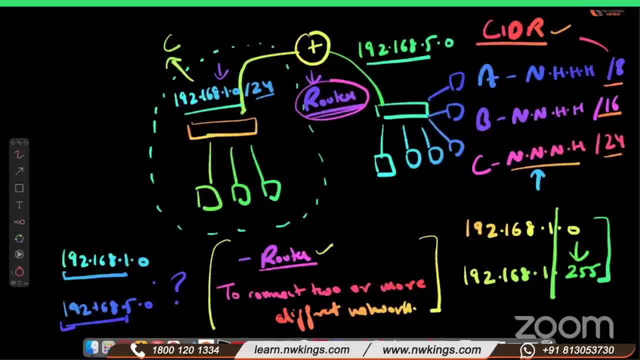 Configurations, because most companies hire network engineers so that they can able to configure router. Okay, clear, Yes, Okay, Sir. yeah, I have a question. one said they here ABC difference classes. Okay, they are network parties, first one and another host three, Okay, sir. I have a question one, sir, They here ABC difference classes. Okay, their network parties, first one and another host three, Okay. 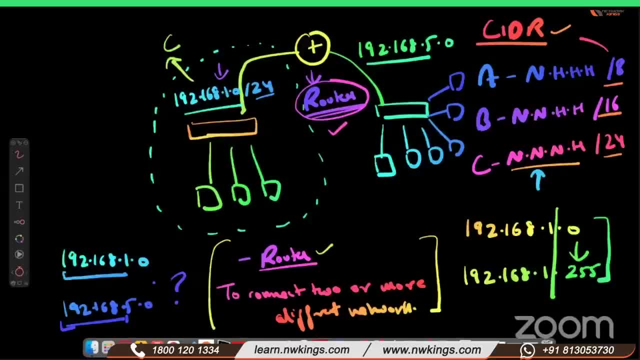 So then, host mean the computers are mainly nodes, and network means what? Network means that you belong to my network or not. That is like a particular area. This is my network router is going to share all the network information to all of the routers. It's like your home address. 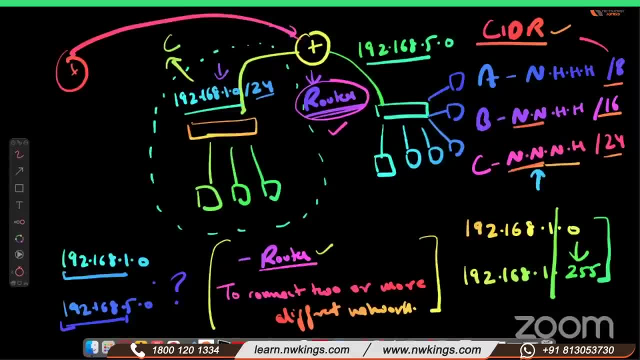 Your network portion is like your home address, Okay. or maybe you can say that it's like your street address and host is your home address, Okay. so if I kit or network is my street address or something, what do you mean? uh, home address or network means. i'm just giving example. don't say this. 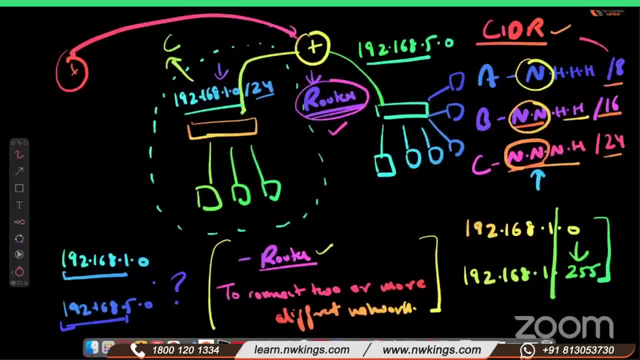 interview: no, no, sir. okay, so just understand, network means your city address or like your home address. so example, take example: okay, so network is like your home address and host is your name. suppose if anybody wants to send a courier to you, i can't send courier to santanu. 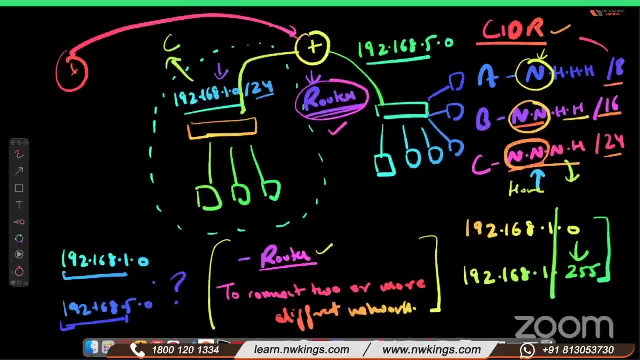 i have to put your home address, yes or no? yes, sir, right, so when the router, when this router share information with another router or share information with internet, so this router is not going to share all 50 computers, thousand computer information the router is going to share. 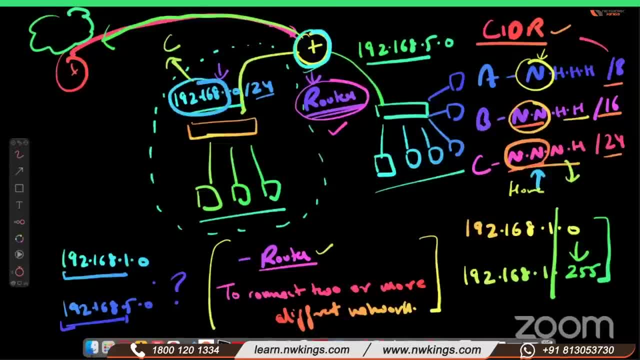 only the network part to another router got it. yes, okay, suppose your ip is your computer. ip is 192 168.1.1. tell me what is your network id. this is your network, yes or no? yes, sir, so your router is going to share this information. 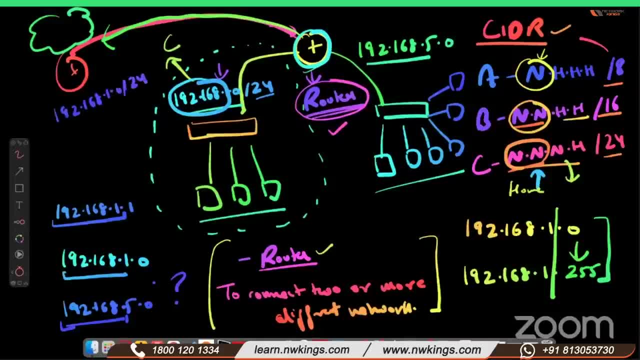 to another router like this. so router is not going to store 1.1, 1.2, 1.3, because these are your, like all family numbers, family members name. we are going to only put the home address in our routing table. i told you right. so we have a global internet table, global routing. 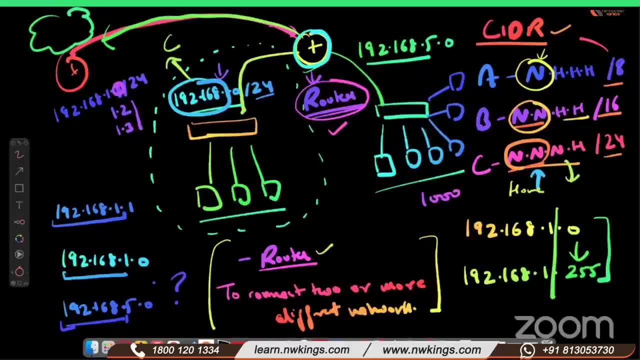 table social computer information. if we are going to put a thousand billion of ip addresses assigned to you or to all users in this world, so if all routers are going to put all the ip addresses, then it is going to have a problem, right? so just understand in this way that we like billions of 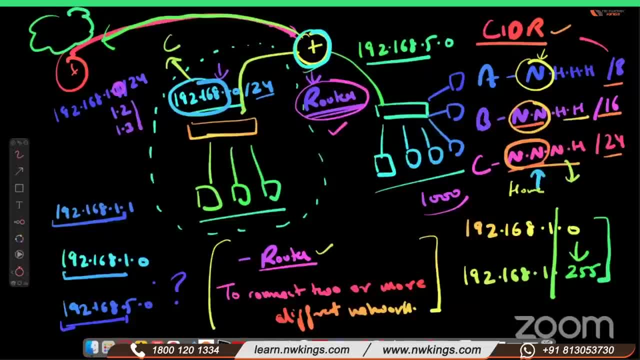 population. when your courier guy come to you, they can't, they don't come to you, they actually come to your network. they actually come to your home or office address. right, because it is easy, so understand. network address tells like all routers: router share the direction. that okay. 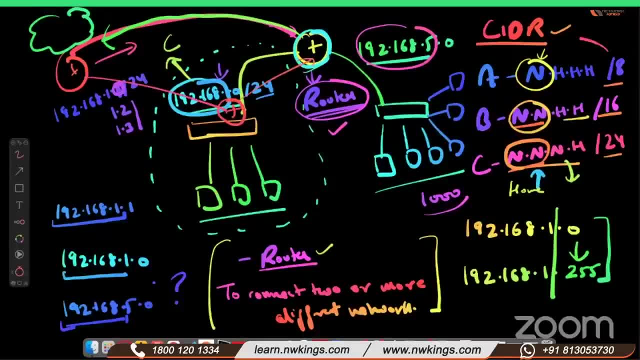 go from this side. go from this side and router checks: okay, home address is there, so it delivers to your switch and switch is not going to go from this side to that side. okay, and you can. will broadcast who is 192.168.1.1 and your computer say: I am 192.168.1.1. this is how. 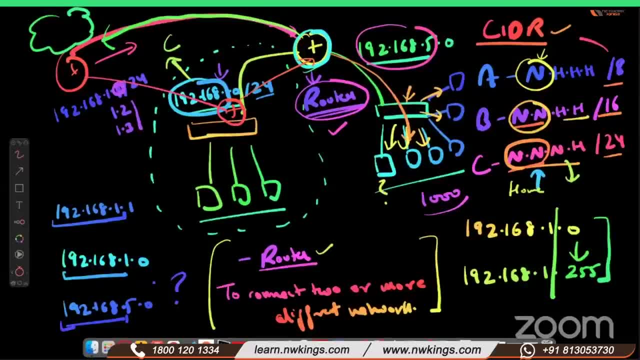 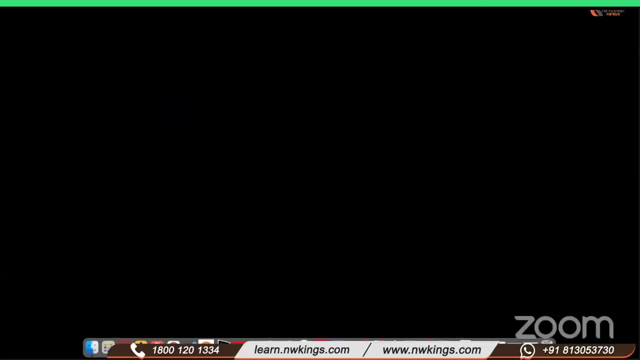 it works Okay. so let's come back to our sync. So now you understand: whenever you give any IP, Whenever you assign any IP like 192.168.1.1, like 192.168.1.2, so all these IP addresses. 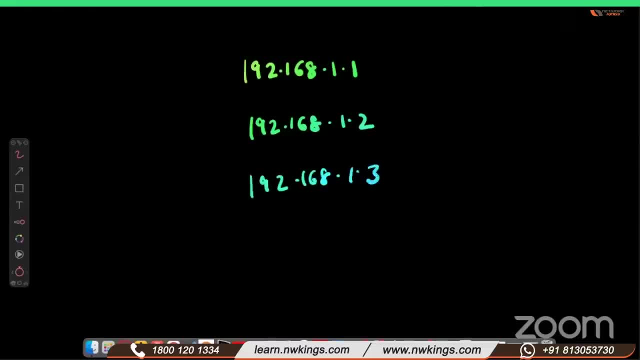 have their home address, or called house of IPs, which is just remove the host IP and you get your network ID right and put 0 here. that is network ID of all users, yes or no? Yes, sir, Yes sir, Got it Very simple. 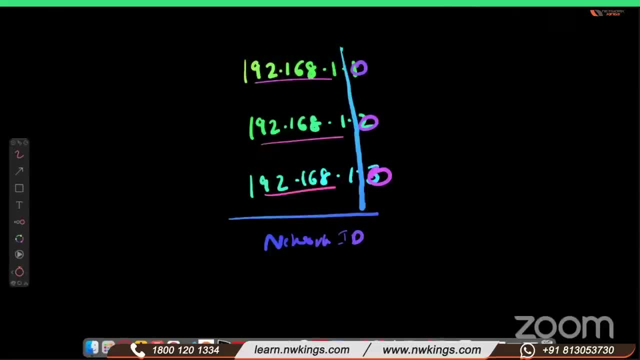 So when router is going to share information to any other router or maybe to internet, so all router- you know this is like- all routers- share their network ID with each other. So all routers are sharing their network parts, not their host IDs. Got it? Yes, sir. 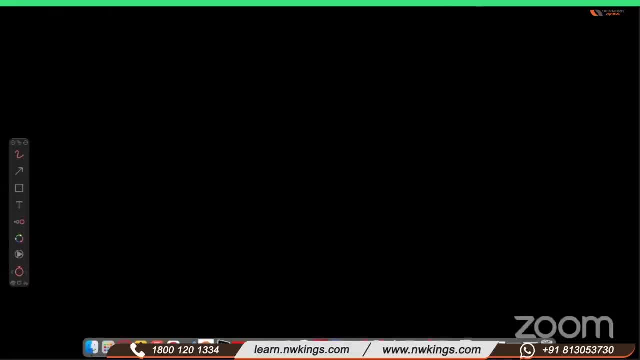 Now it's clear, sir. So this is why network ID is important. I hope now you may got it why we use network IDs: because all routers only share network IDs with each other. Okay, Yes, sir, Clear. So let's understand what is subnet mask more. 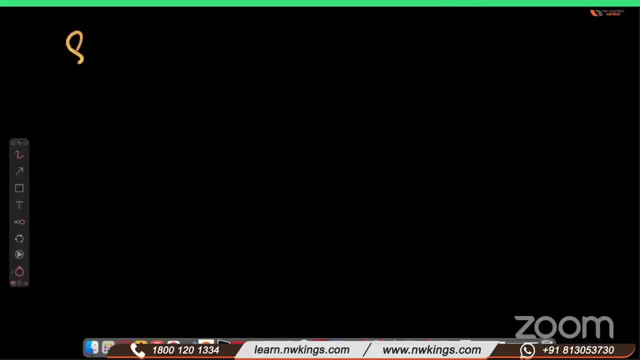 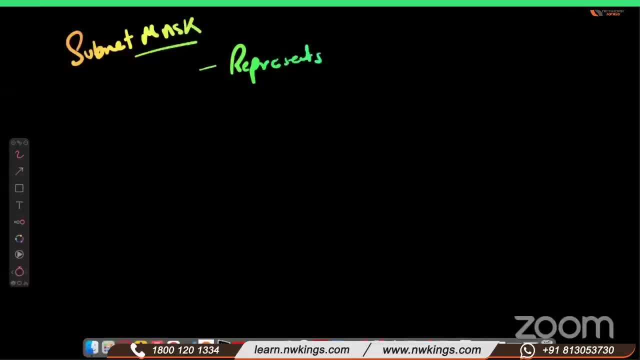 OK, Subnet mask is subnetfer, which represents network bits. So from both of them the subnet mask represents network bits. is it so Any? I can see only 2.. 2. Two begins Nothing, Nothing. Two begins, OK. yes, sir. 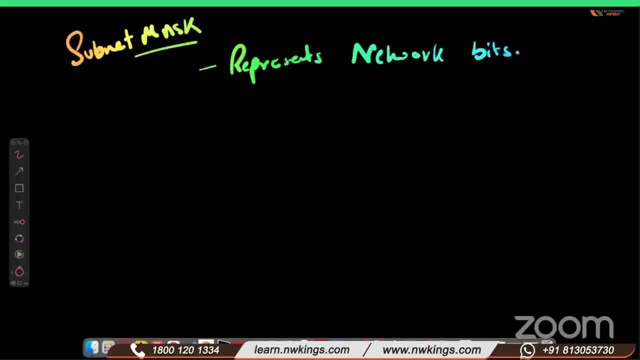 Two begins. That's all. Yes, sir, That's it open. OK, So this is only a your own ambassadors language, but to me this is faster and faster. I have running the same Boolean module, but for okay. Now let's discuss this. 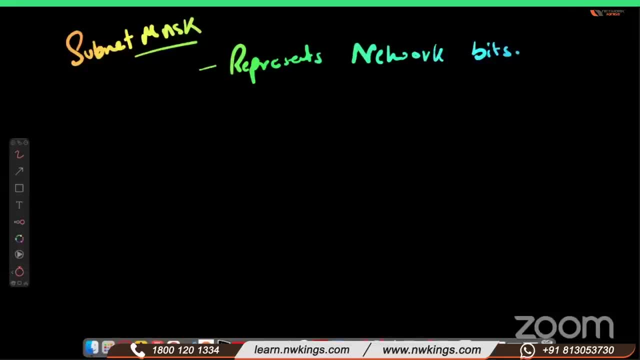 Second, to number 3.. The third example: What is number 3?? If assignment is something not oggi, we need code. How do I set number 3 inHN Zimmer? So I will explain you something okay. So slash 8 was 255.0.0.. 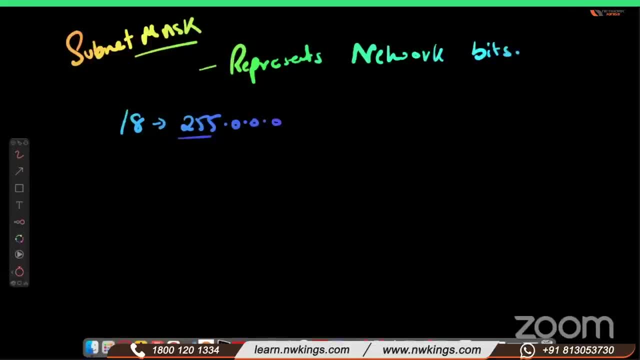 How? How we got 255?? Because if you calculate the to the power of errors- I have told you this 2-3 times before. So if you plus all the values, what you get, You get 255, right. 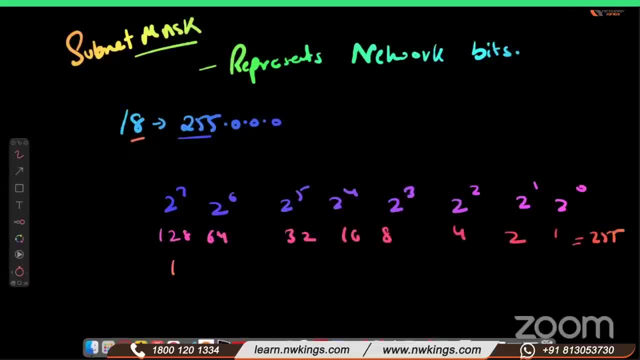 So this means 8.. 8 means 8 bits: 1,, 2,, 3,, 4,, 5,, 6,, 7, 8.. So 8 means 255.. But what will be the value for slash 9?? 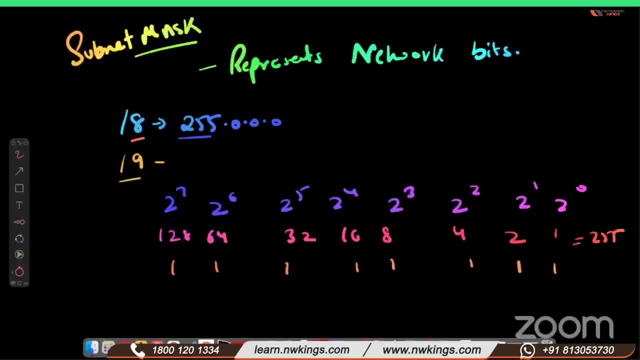 So obviously, how to calculate for 9?. What is the subnet mask of slash 9?? So slash 8, slash 9 means how many native bits. So what is slash 9?? So it means when two computers communicate with each other, right. 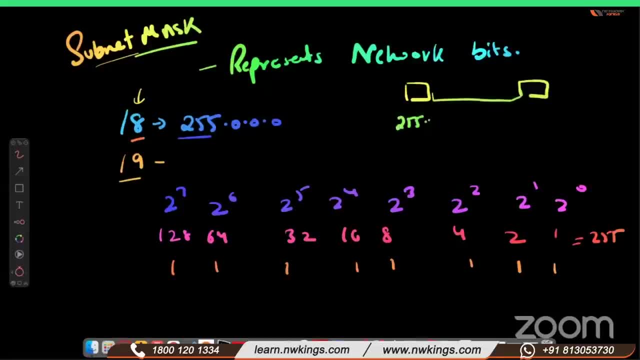 if you give any IP, but if you give 255.0, something, slash 8.. So first let us get the subnet mask for slash 9.. So what will be the slash 9?? So obviously 9,. how we make 9?. 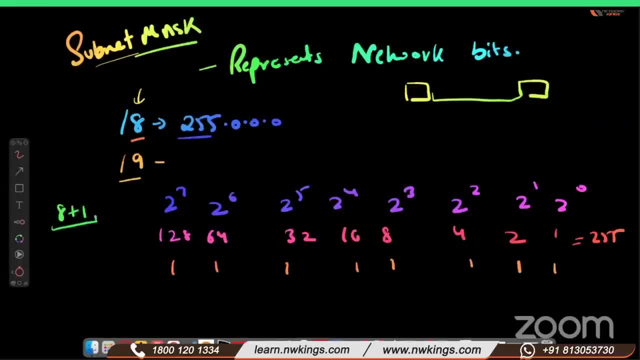 8 plus 1, yes or no? 8 plus 1 is 9.. So 8 means 8 means 255. and on another subnet, on another octet, on another octet, you just have to take 1.. 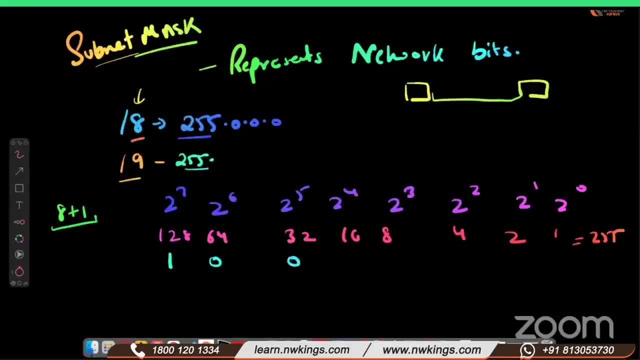 Okay, 8 plus 1 is 9, and just calculate the value. So you will be getting 128.. So 255,, 128.0.0, very simple, right. And if I give any value for slash 10, let us suppose. 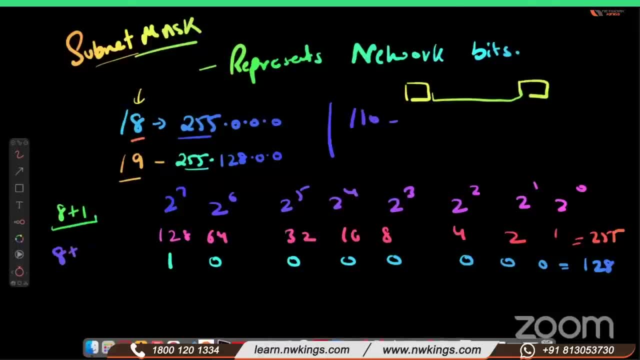 so to get 10, what will we do? 8 plus 2,, 8 plus 2, so it means 8 means 255, but 2 values, 2 means 1, 1.. So you calculate, you get what. 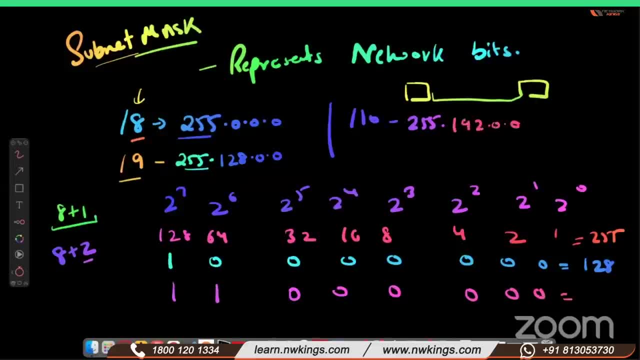 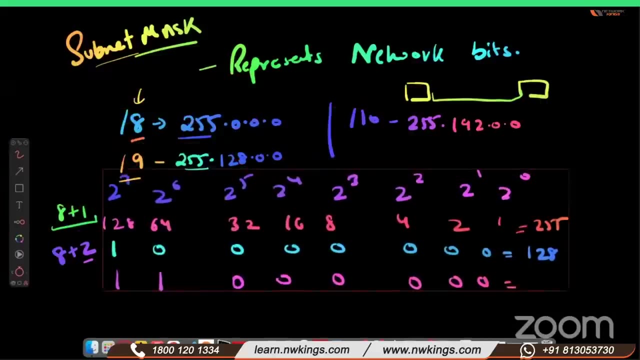 192.0.0.. So let us not calculate because it is a little complex formula. but I wanted you to explain how we calculate, So I will tell you the shortcut. You do not have to learn or write this. So there is a shortcut. okay, so let us understand the shortcut. 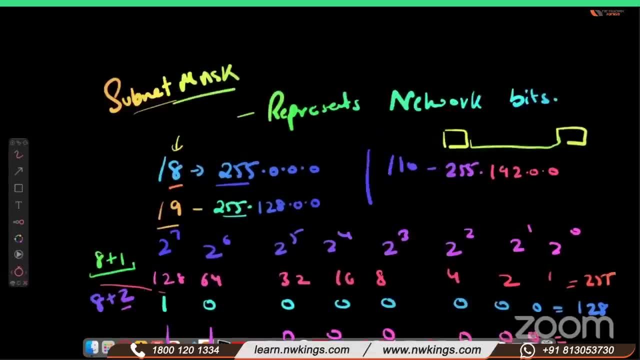 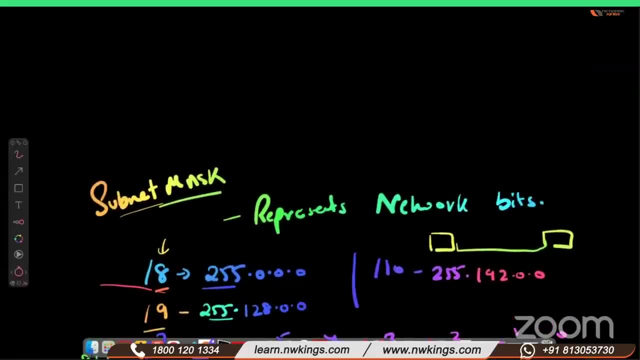 Oh man, Okay. Okay. so, guys, shortcut is: for 1 bit, always add 128.. For 1 bit, always add 128.. 128. If you add 2 bits extra, you get 192, 3 bits. if you plus first 3 numbers 2 to 4,, 4,, 240,. 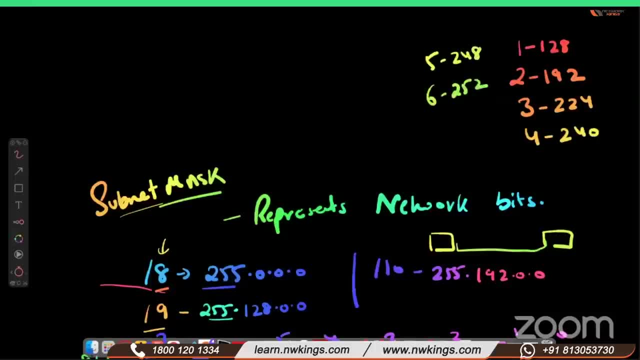 please note down this. it is going to help you. okay, just I am adding the values first: value 128, 128 plus 64, 192, 128, 64, 32 is 2, 2 to 4, so this is the value you will. 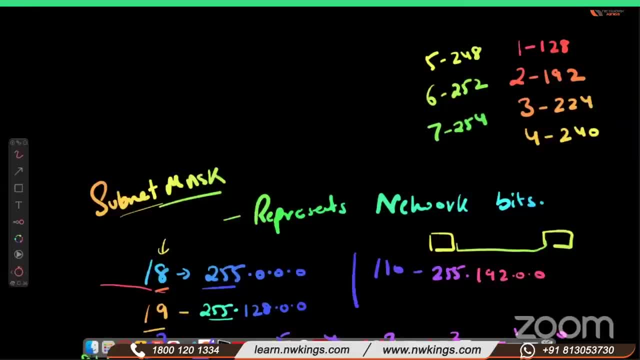 be getting right. So now you calculate it very simple. Suppose slash 12,, so 12,. how we make 12, 8 plus 4, 8 plus 4, right? 8 plus 4,, so 8. 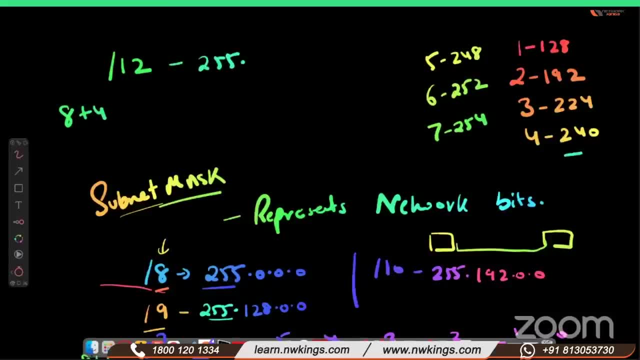 means 255 and 4 means 240.0.0, very simple. slash 15,. tell me for 15,. 8 plus 7 is 15,. 8 means 255 and 7 means 254.0.0, very simple. 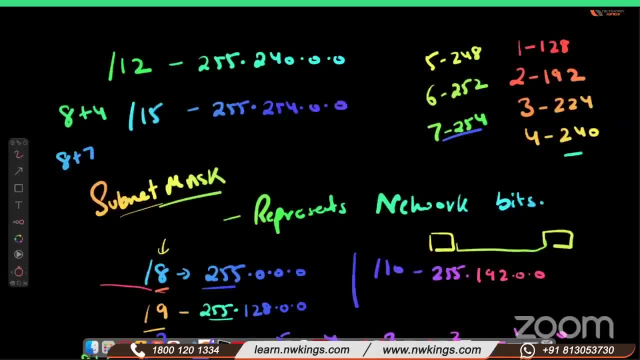 Yes, Ajit, you are correct, they are in same network If we give slash 20,, so 20 means I will tell you: now do 8,, 20,, 8 plus 8,, 16,, 8 plus. 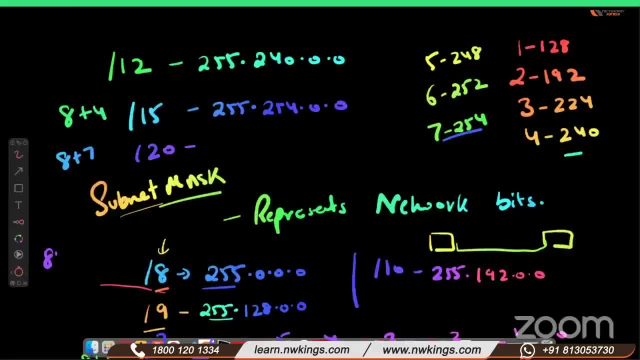 8, 16,, 8 plus 8, 16,, 16 plus 4.. So it means 2. Whenever you see 8, 16,, 8 plus 8,, 16,, 8 plus 8,, 16,, 16 plus 4.. 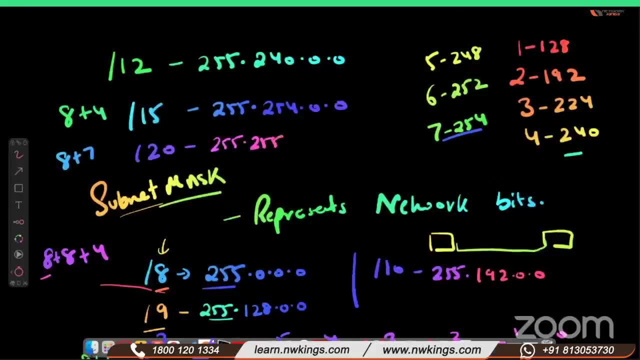 So it means 2.. Whenever you see 8,, it means 255,, 255 and 4 means 240.0,. very simple, Let us calculate for 18, so 255,, 255,, 16,, 16 plus 2, 190,, 2.0,. yes, Nainjyoti samajhaya. 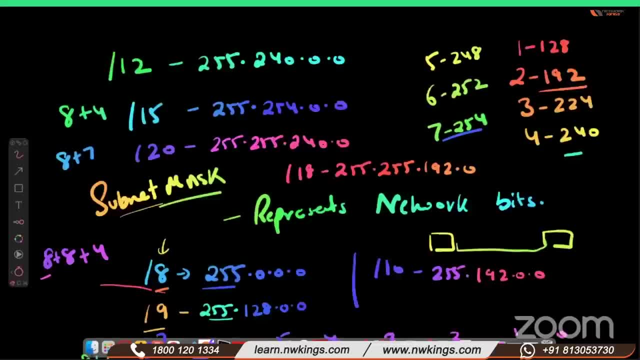 sabhi ko. yes, guys, this is very important and you have to learn this formula if you do not know how to calculate. Even I have not done it. Even I have not done it Till now, I have not done it. 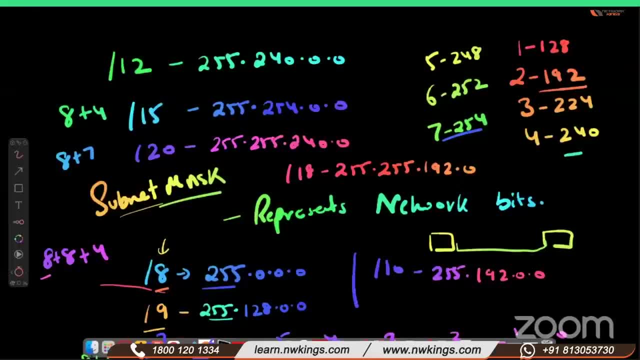 But just now, even I have not done it, Just now, I have given you the information how to calculate. Yes sir, Yes, sir, Yes, Nainjyoti, clear. Yes sir, Yes, sir, Yes, sir. 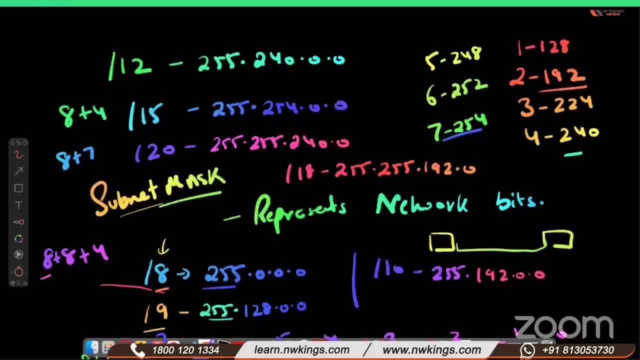 Sir, a question, sir, Sir, which means we have to increase the network ID from the default value. sir, it will open subnetting. yes, sir, Yes, I will tell you why it is subnetting, but understand how can we remove subnet Mask? 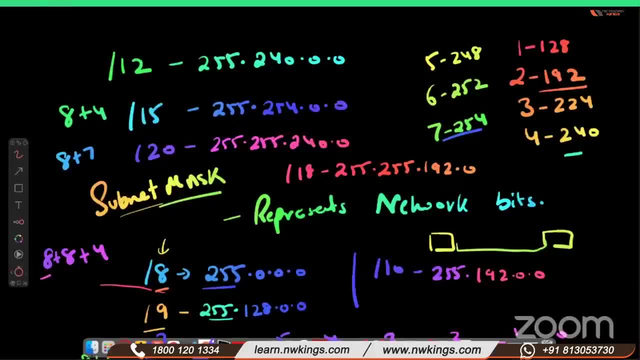 Sir, add slash 8 to the slash value. sir. Sir, add slash 8 to the slash value. Sir, add slash 8 to the subnet Mask. Sir, add slash 8 to the subnet Mask seven. no, no, no, no, we should not use. you can't go less than eight. 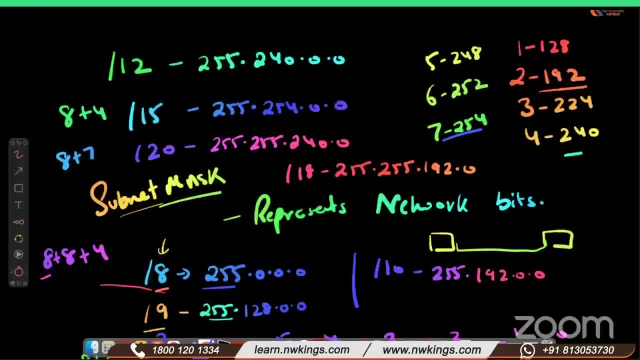 because the first number actually represents your network, right? so you can't go less than eight. yes, sir, yes, sir, so let's go further, okay. so, guys, this is highly important. please take screenshot, or even the class is getting recorded for you, don't worry, but this is very important. just write this. 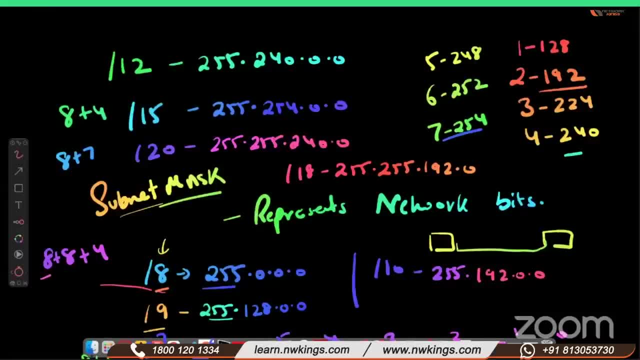 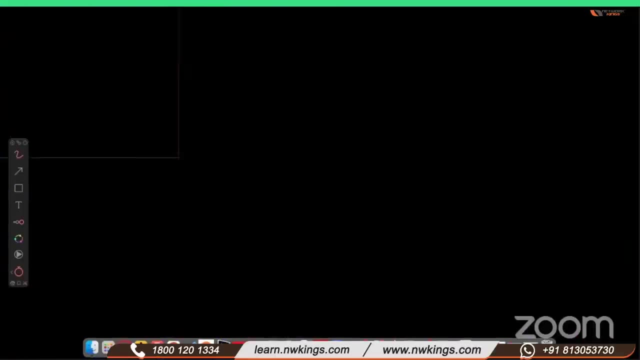 so why? i'm telling you? because this is the first step to learn submitting. you should know slash 15 is called two five four, two five four dot zero, like this. okay, so let's do more practice. suddenly, submitting is all about practice, right, but you need better strategy. 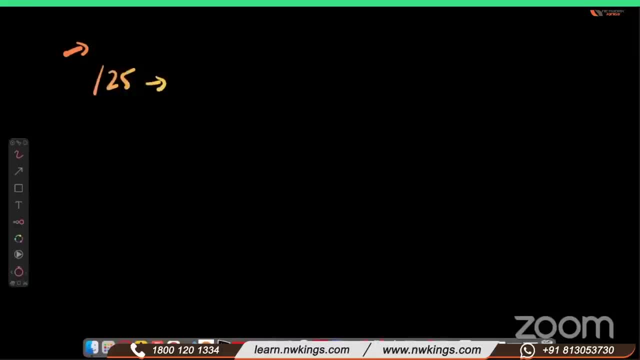 so if i give you slash 25, just divide into parts: 8 plus 8 plus 8, 24 plus 1.. tell me your answer: 2, 5 5. 2 5 5. 2 5 5 1. 28. yes, 128, 27. 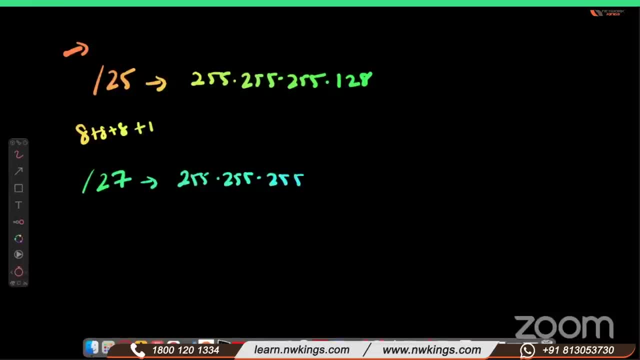 2, 5, 5, 2, 5, 5, 2, 5, 5, 24, 24 plus 3.. got it? yes, 8 plus 8 plus 8 plus 3.. slash 30, where we use last 30, just for your information. 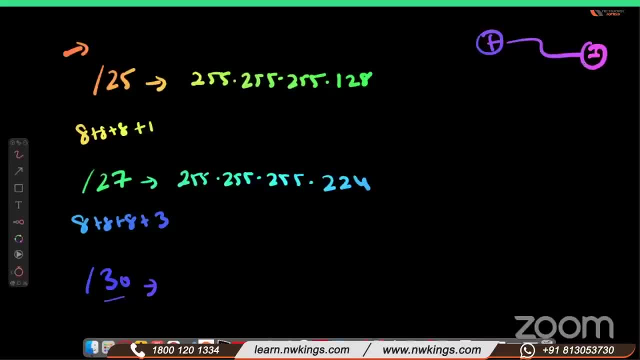 i'm kind of lost. yes, yes, tell me how. how are you getting 224 for that last octet? because there was a shortcut, like: for one bit you get 128, for two you get 192. so how i calculated this? so every octet, four octets. you have right. 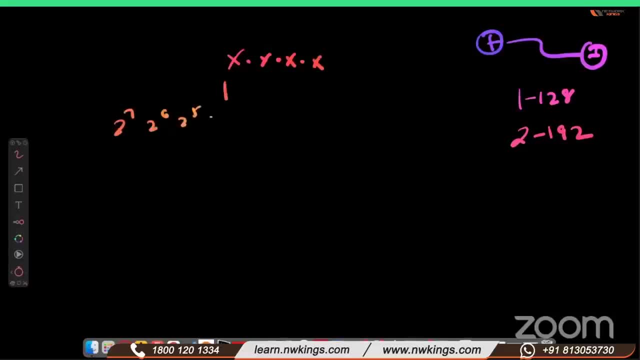 so every octet you have to the powers: yes, correct, yes, yeah. so if we talk about slash eight, so it means you have eight ones. this is, and if you plus all the values, their corresponding values, if you plus all the values, you get what? 255, right. 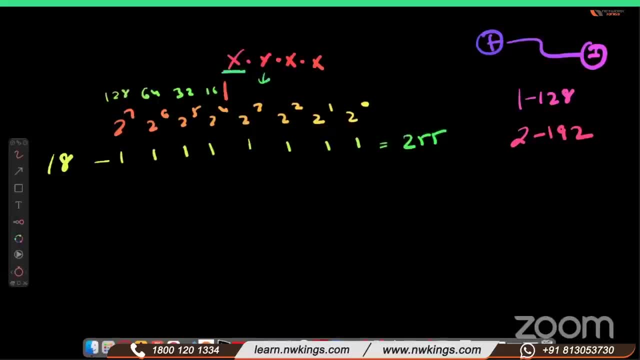 so in the second octet, because this octet is completed, eight bits is completed. but when you have nine you have to jump on the another octet, because eight is completed. now, in another octet you have same values, but you will take only one here: eight, eight plus one, nine. and if you calculate 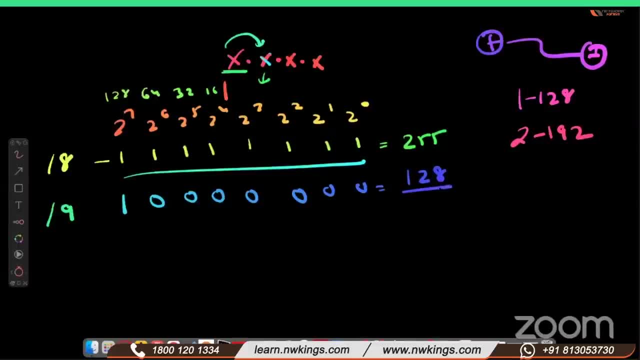 what you get: 128, yes, yes. so this is why i have written: one is equal to 128.. now another: if you take 10 for 10, what do you have to take? you have to take two bits more, right? yes, so for two bits. if you plus this two-bit 128, 64 is yeah, 192, yeah. so now three bits. if you take three bits, 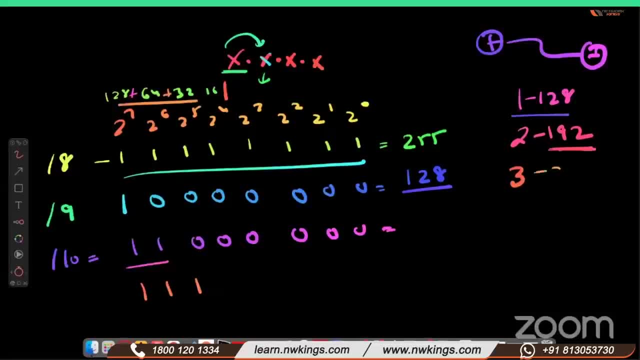 if you plus 128, 64, 32.. 3432, you get 224 players. what we're trying to draw and the type of character because we plus, we add when we say we want 11. this is my slash value. i want to write a subnet mask. how i'm going? 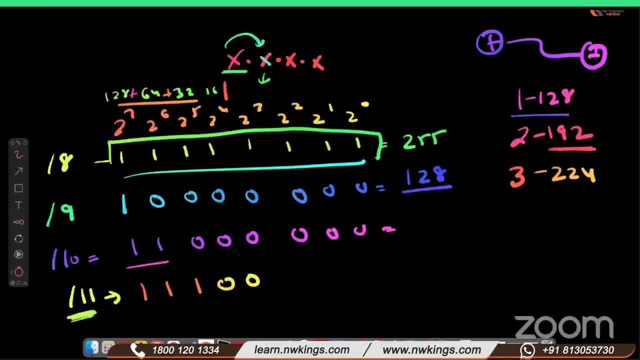 to write first. this is my eight bits, right? this is it. i'm going to write extra three here and if you plus, if you plus the first eight, you get 255, and for remaining three, you get 224, 128, 64, 32. you want more clarity, or it's clear? 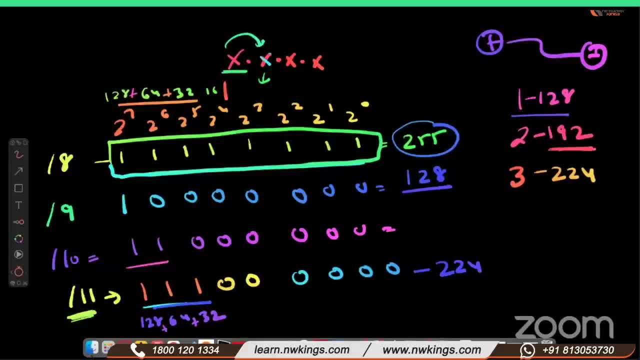 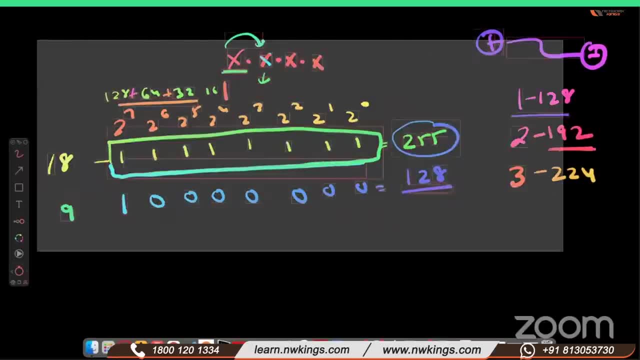 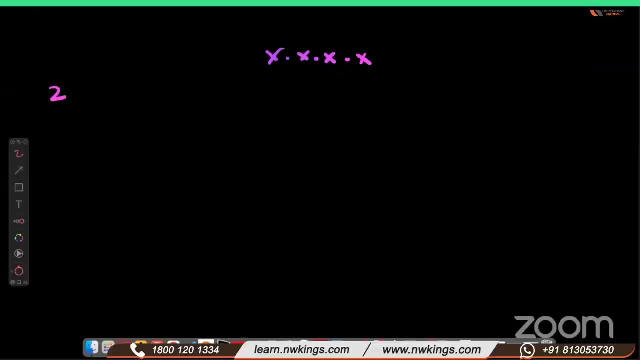 um, i think i need more clarity. okay, so just calculate. okay, so the another way to understand this. so i have to write all four octets. this is the last option i have, so please focus two. so all four octets will be written like this, to the power of seven. 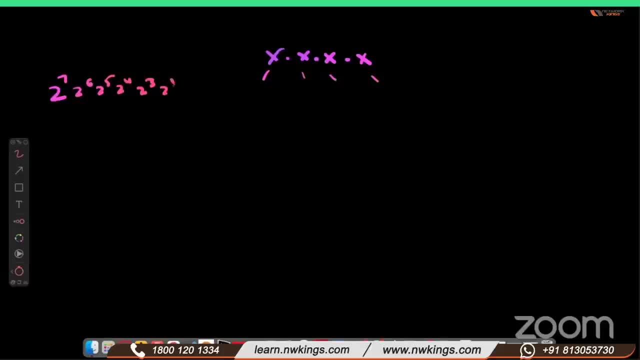 no matter what. two clear. first octet written. second, one same: black athletes in the game hockey and, uh, i guess okay. second is clear. third octet: same, i think you know, because eight bits is represented like this only. i hope that makes sense. but why can i play hockey, right? yeah, the power two, yeah, so all octets are like this. 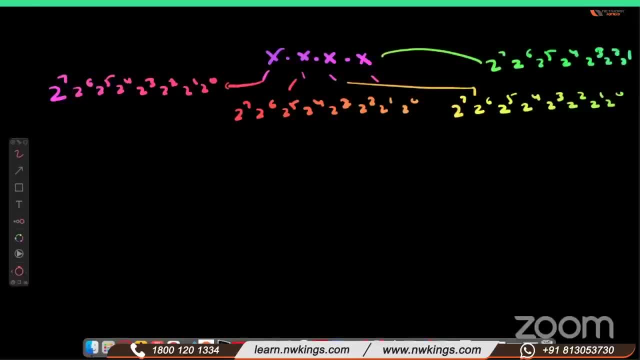 clear. yes, okay. so if i talk about slash eight, it means you need to write one one eight times and rest all octets will be just the hockey player: zero, right, yes, yes. and if i talk about slash ten, ten means ten bits, this eight means eight bits. and if i talk about ten slash ten, what does ten means? 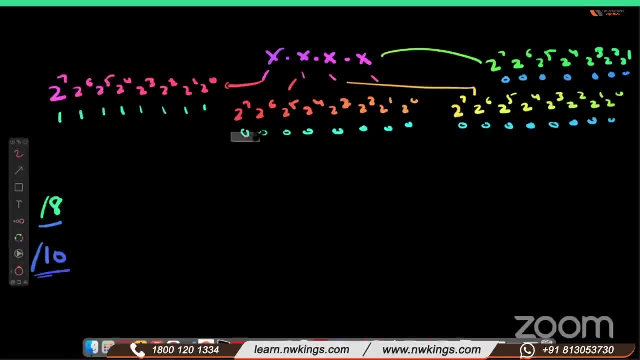 eight and you have to take nine and ten from here, yes or no, from second octet file: yes, got it. so if you plus this value, what you get: 255, yes, and if you plus this value now, you will get 3 somersault length, 255. so what you are going to do if you do this? 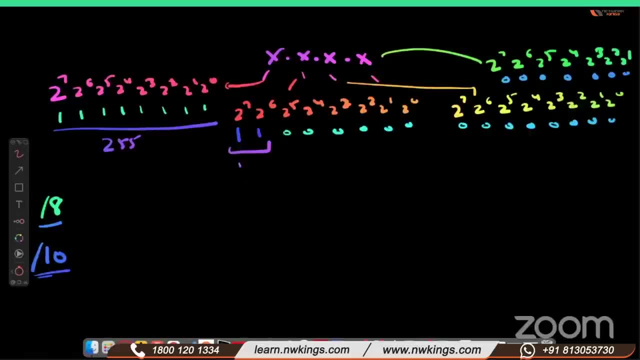 yes, keep reading the year before. so that's just a small thing. so that's the goal. so, whatever it may be, no more questions and bye, bye, bye, bye, bye, bye, bye. wszystk coordinates should be: value what you get, 192 way that you could feel part of the. 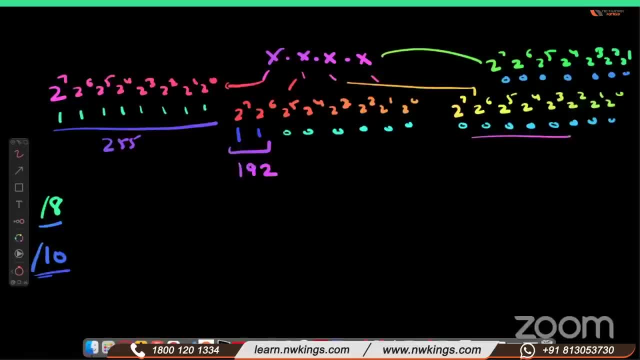 community by being engaged. third octet is 0. fourth octet is 0, so slash 10 is 255, 192.0.0. yeah, I think I see how that works. yeah, so now, if I talk about slash 11, 11 means 8 is already set. 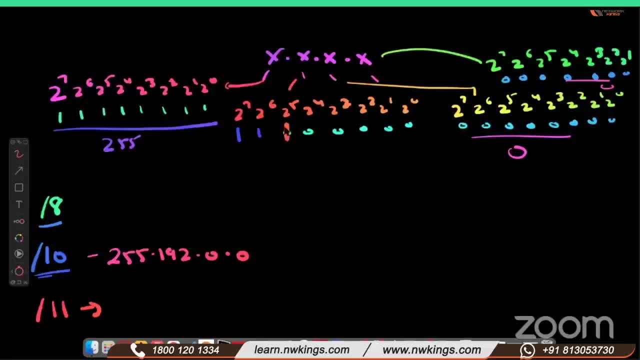 8 is already set. I need one extra. I want to borrow one more bit. so if you plus this, 8 is 255 always, and if you plus 3 you get 128, 64, 32, so that is 224. so you don't have to write a very big formula. this is: 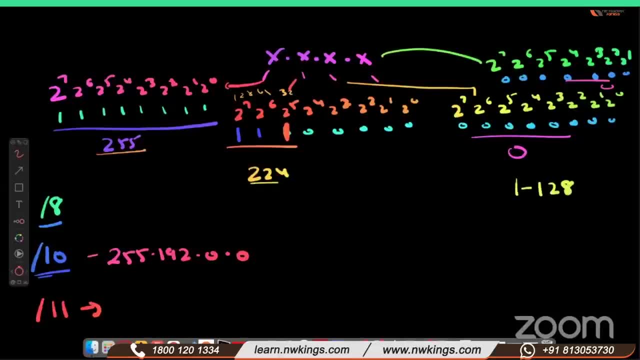 a shortcut: for 1 bit, we always get 128. for 2 bits, we always get 192. if we plus 3 bits, we always get 224. if we plus 4 bits, we get always 240. ok, if you plus 5 bits, we always get 248. 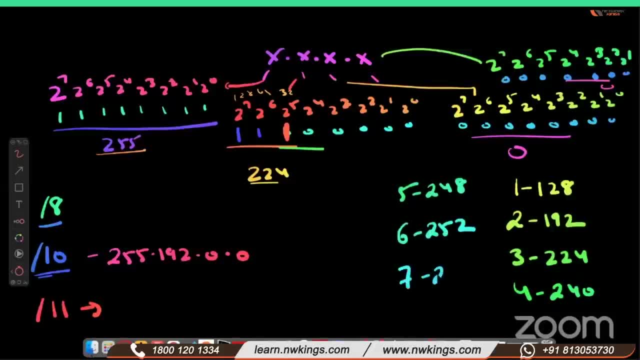 for 6 bits, we get 252. for 7 bits, we get 254. so this is what we get. if you plus 8, you already know the answer what: 255. yes, got it now. yes, ok. so guys, now you are like what we call that homework in schools. 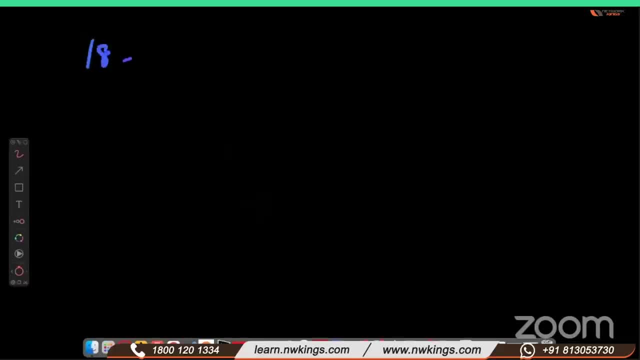 right, I want you to write all values from 8 to 30. ok, you can also get the chart also from google if it checks slash values or something like that. but please try to just write down from your end: slash, subnet mask. you can just type subnet mask. 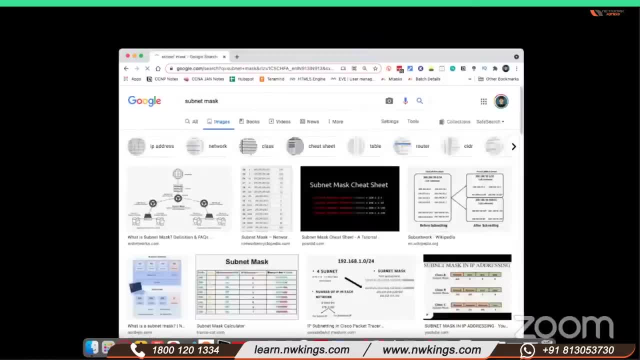 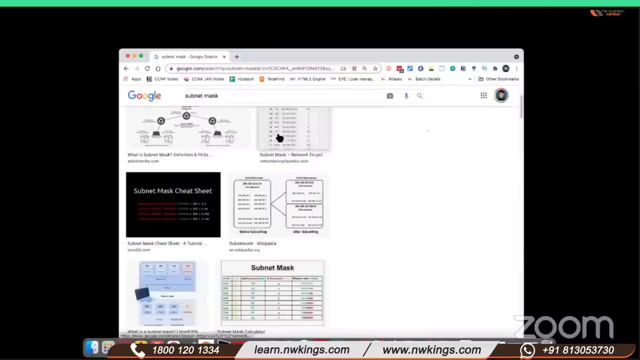 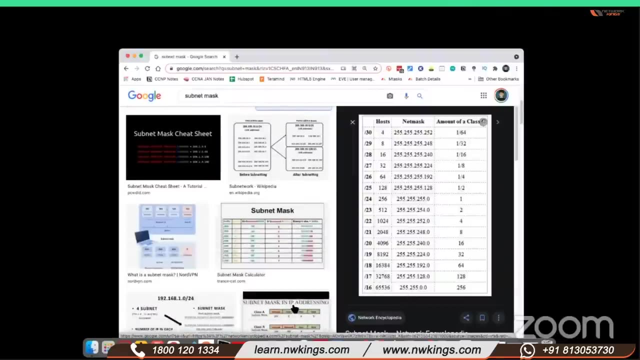 on google just type subnet mask and on the images like, so you can see there is a very big chart, right? so this is all values you can see. 16 is 2 times 255- okay, and 17 is 255 255: 16, 16 plus 1. 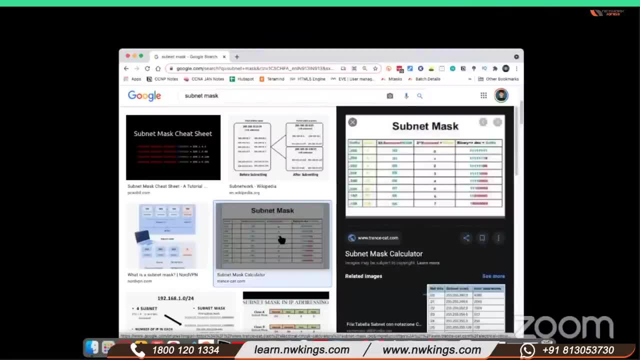 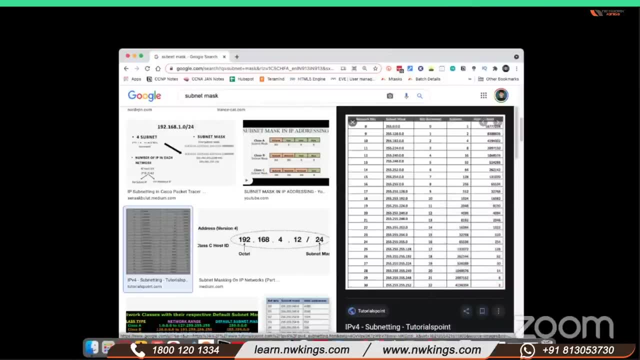 1 extra bit is added, 128. okay, so you can just check this one. so that is a simple one, okay. so, guys, i am going to share you some notes, what i have written on my screen and whatever is this image, i am going to share that with you. 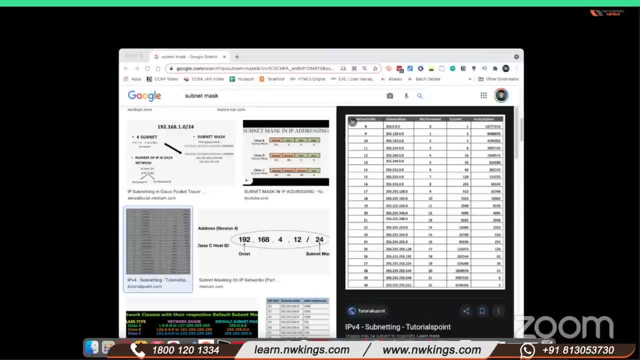 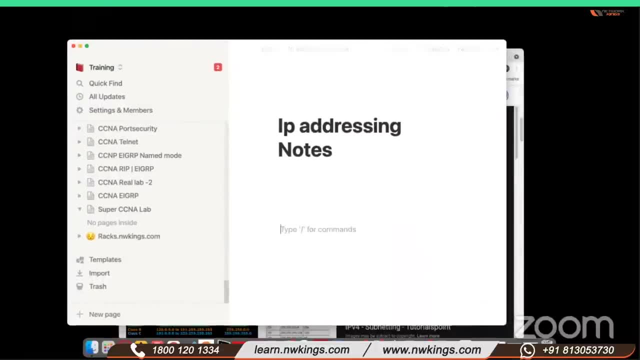 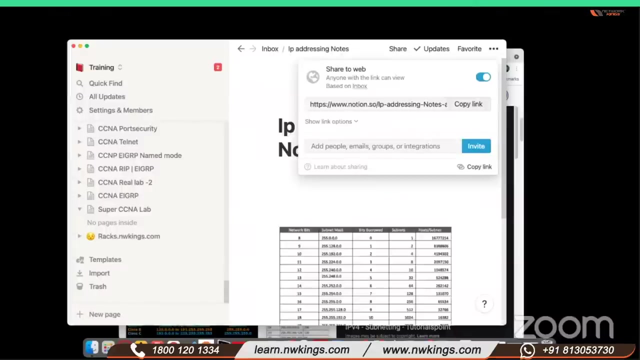 okay, so this is ip addressing, so this is uh, okay, so i'm going to add this note, so please bookmark this for few days. so this will be the same link you have to check the notes. okay, please bookmark this link and i'm going to upload this into your portal, okay, so? 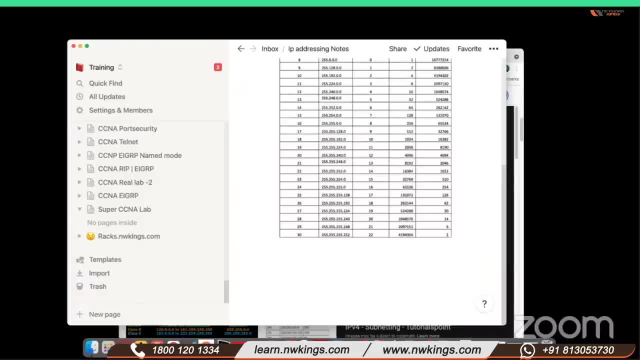 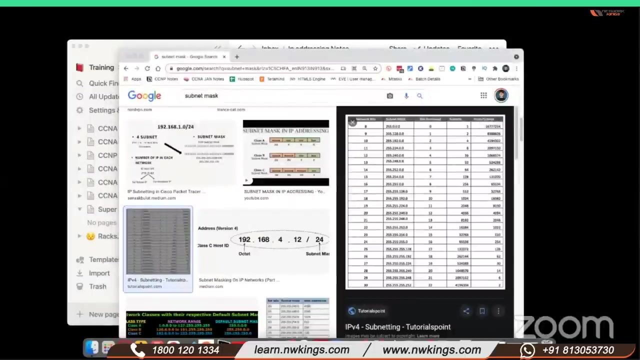 uh, just hold on, let me give you something iep addressing if i have. so one minute, okay. so it's okay. so give me one minute, give me one minute, give me one minute ip addressing, ip addressing: hello sir. yes, yes, so this is ipv4 and you will be getting that only, okay, sir. 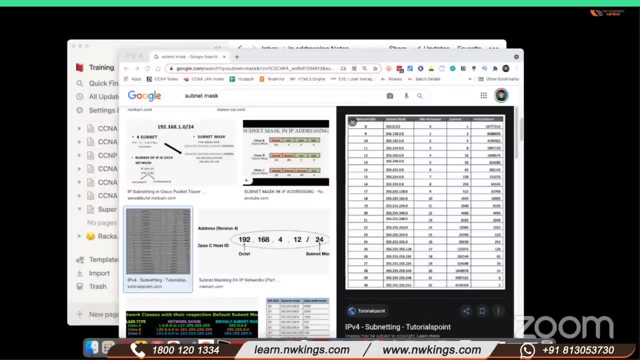 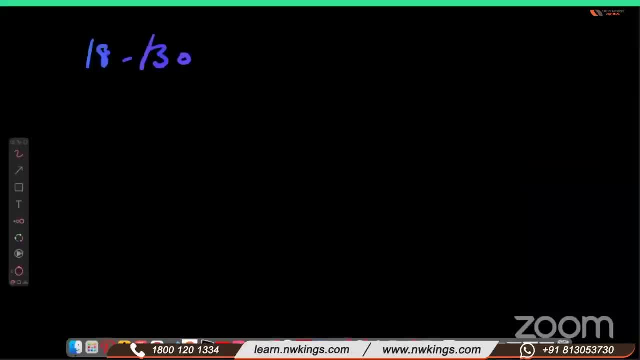 so just you have to remember why it's important, because i'm going to train you tomorrow. very simple, suppose, like if you you uh, so tell me when you use class c how much ip addresses you get. so when you use class c, 192 to 283. yes, so we had three network bit, one host. so one host means 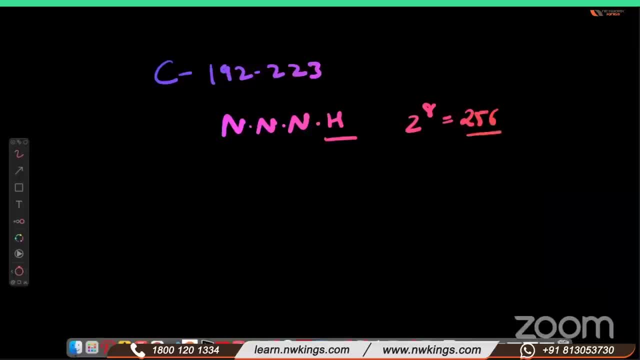 eight bit to the power of eight is how much ip you give from class c: 256, 56. but now you don't want to use 250 ip addresses, you want to save ip address. so we are going to learn something. so that is to reduce the. 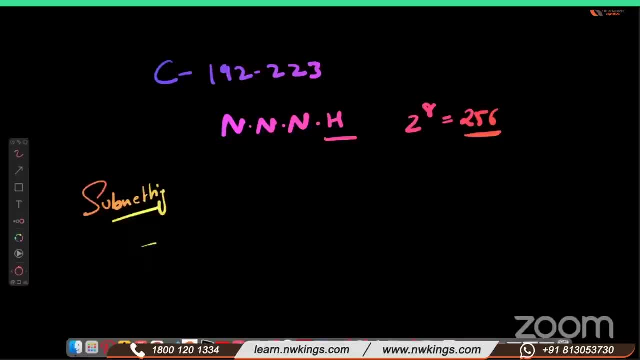 wastage, why we use submitting, why every company is using subnetting to reduce the wastage, to reduce the wastage of ip. okay, tell me, if you have 10 servers, if you have 10 servers in india and you do not want to use 250 ip addresses, then why you use subnetting? because 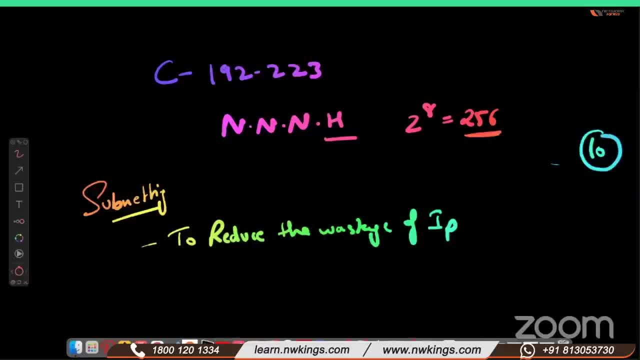 you want to save ip addresses. so we are going to learn. so that is to reduce the wastage. why? or maybe in any country? okay, suppose you have 10 servers, but do you guys are going to buy 256 ip? your requirement is only 10. are you going to buy 256 ip? no, no, sir, right. so that is not a good. 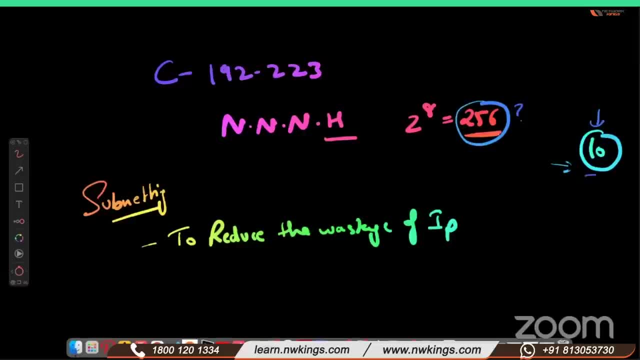 thing, so you will directly buy 10 ips or whatever you required. so the same pattern when we use subnetting, when we talk about public ips. okay, i'll explain public and private ip also tomorrow, but what you have to do now or today, so just whatever. i am telling you that please learn the. 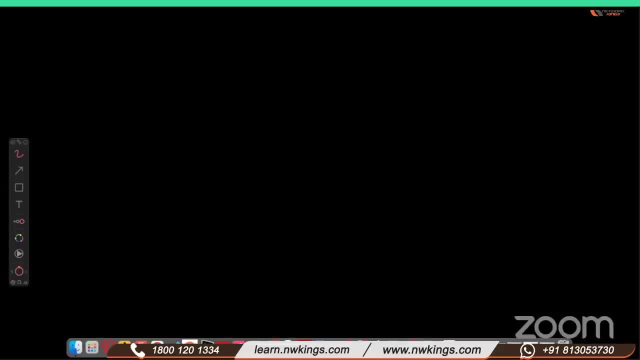 subnetting three things. first of all, whenever i write any ip- suppose 150.1.1.1, so you should quickly understand this is class b, you 129.1.1.1. tell me which class b. class b b great. so 200.1.1.1. which ip. 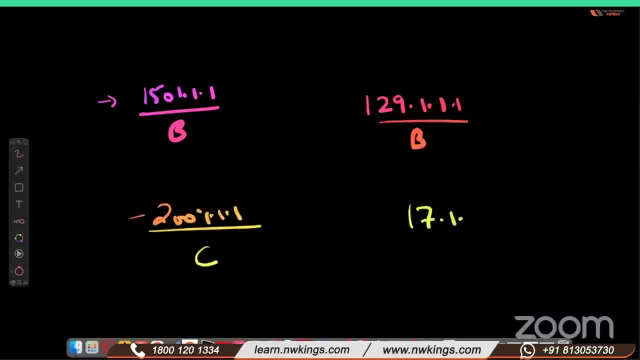 c: okay, 17.1.1.1. class a: class a: yes, so you are. so make sure that you practice that much. you will be able to identify the ip address and how you identify. just see the first part. okay, so just see the first part. only check the first part and you will be able to identify this belongs. 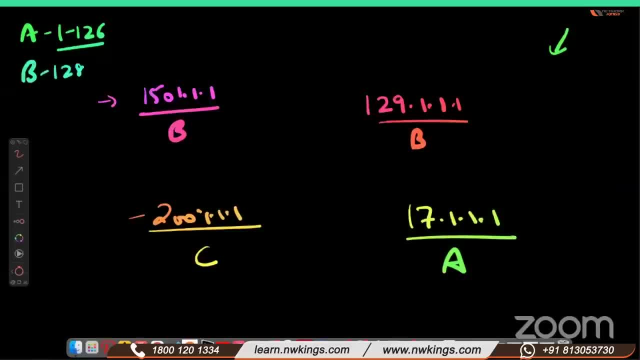 to a, b or c class. okay, got it. hello sir. yes, yes, sir, is there any range, specific range for public ip assign or is it can be any class. i'll explain tomorrow. okay, subnetting, subnetting, subnetting. i had a note which i couldn't find i wanted to share that i see i'm going to share some notes of. 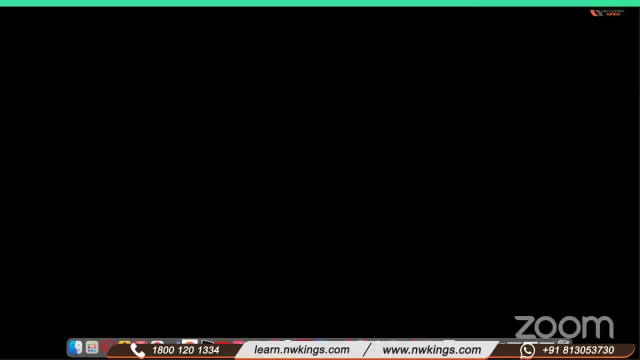 subnetting okay means it's just a practice material. let me check if i have- or maybe i have- some notes I'll share once I'll get, okay. I'll check my emails and I'll share with you, okay, or on your email ID. take it tomorrow the same time in the AT&T. thank you. 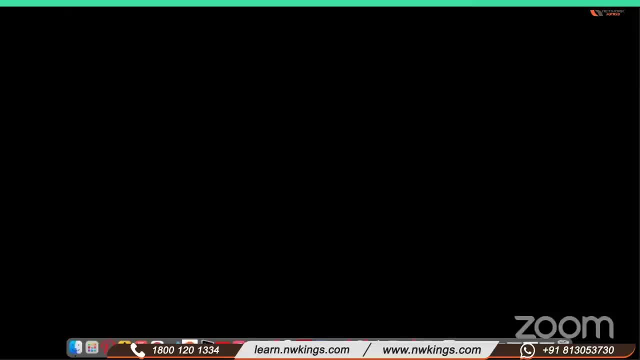 yeah, the session means you guys got to understand things, or not? yes, and this recording will be available on your portal where you have enrolled learnnwkingscom. okay, we will get any PPT for this. yeah, yeah, I'll be sharing all material, don't worry. 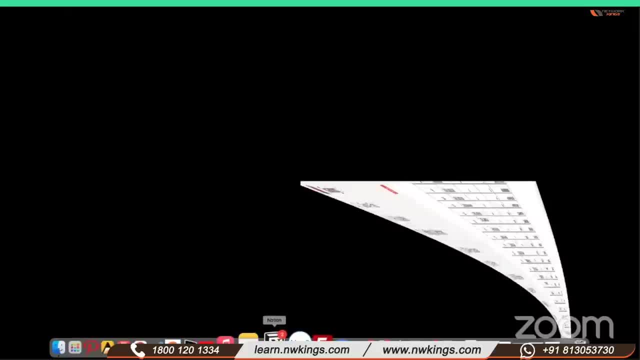 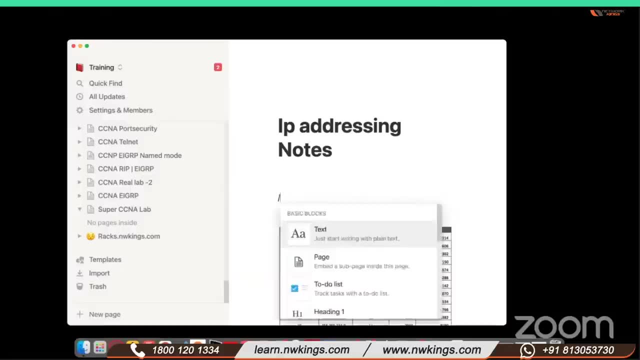 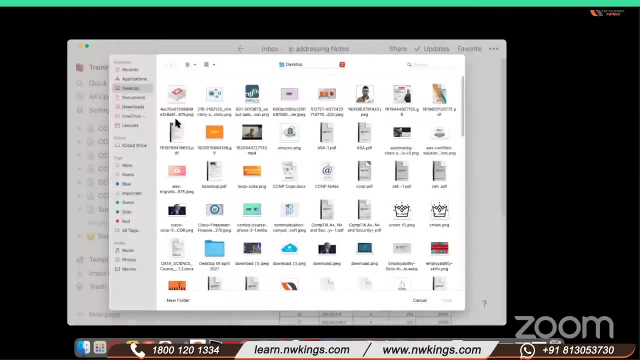 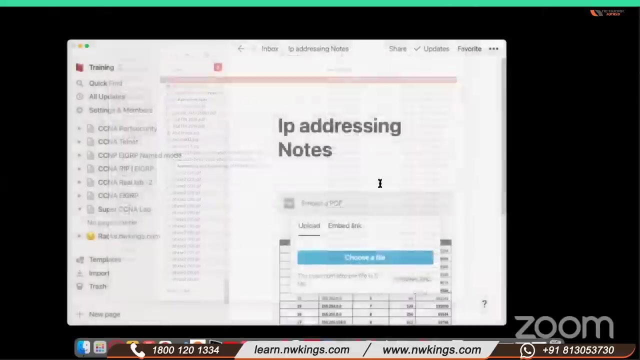 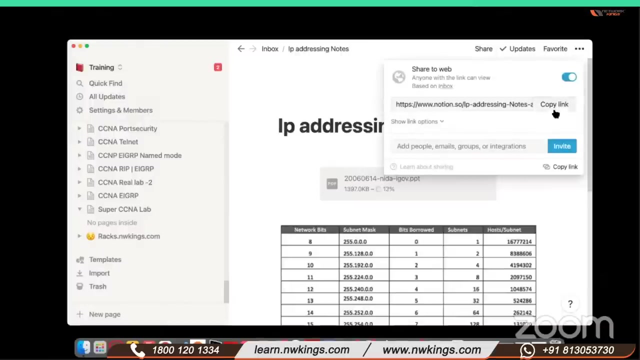 that PPT also and this notes I have already shared. I'm going to share that PPT here only if I can just hold on PDF. it's a PDF, so this PDF is something, something, something. so I have uploaded that. please open that link again. okay, so I have uploaded. 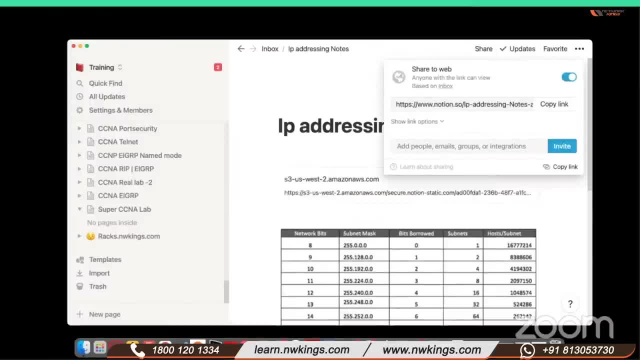 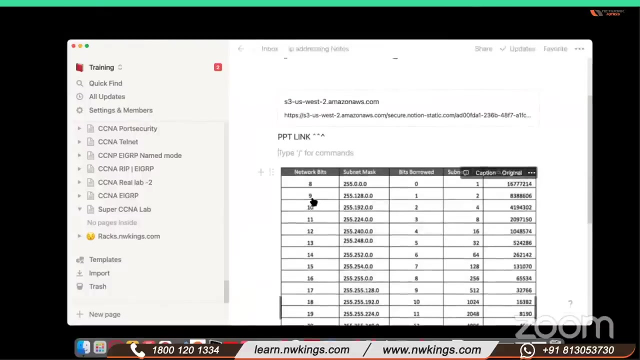 and you'll be getting soon here. okay, just click here and download this PPT. okay, so you can see all my lab and just I'm going to share a few things. where was that? The new video is on my website and I am going to share this video in comercialnet. so you can see if I sent it in your stream or not. so you can see what's going on there. I'll show it here and I'll see you in the live chat. Okay, so thanks for joining us and have a great rest of the day. 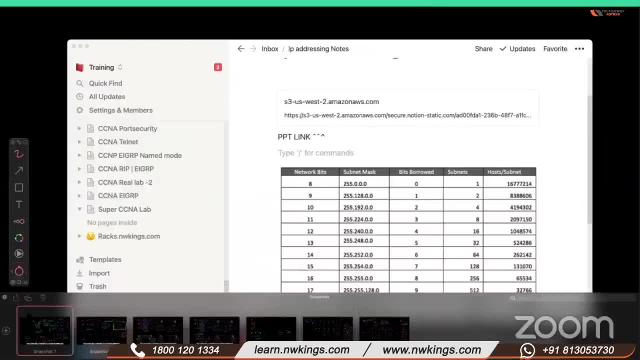 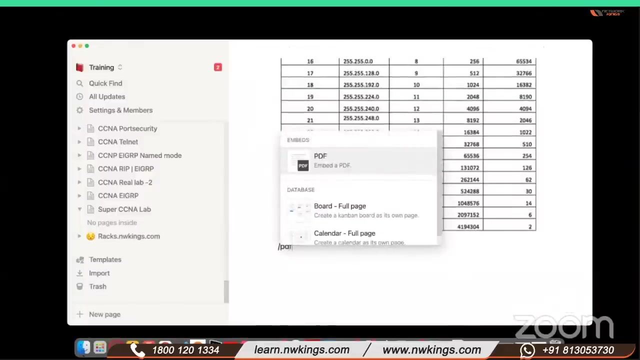 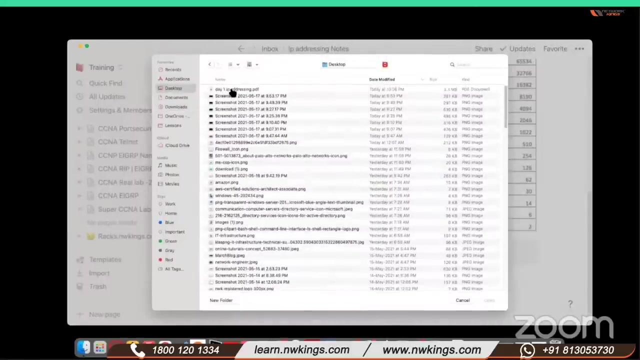 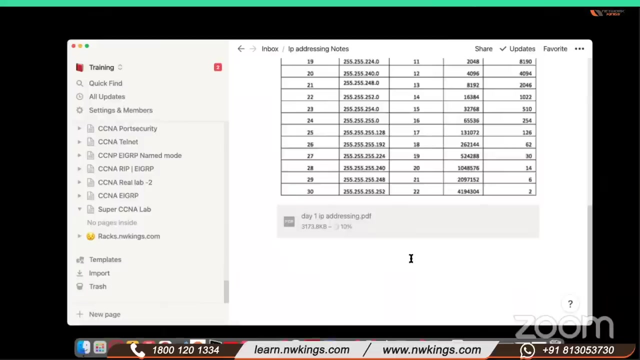 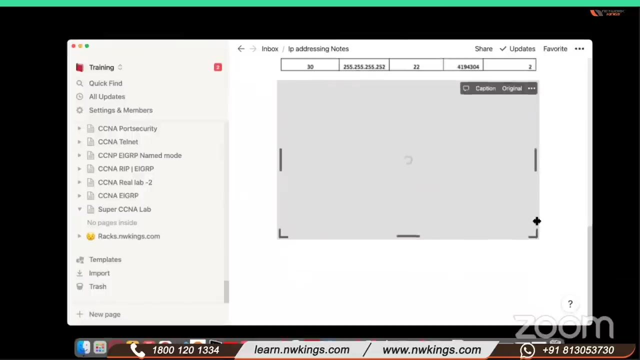 Bye, Bye. snapshots. day one: IP addressing. okay, so the notes will be shared with you, don't worry about that thing. that is our USP day one, day one. yes, so here you go. okay, so today I have written on my screen, right, so all the notes you will. 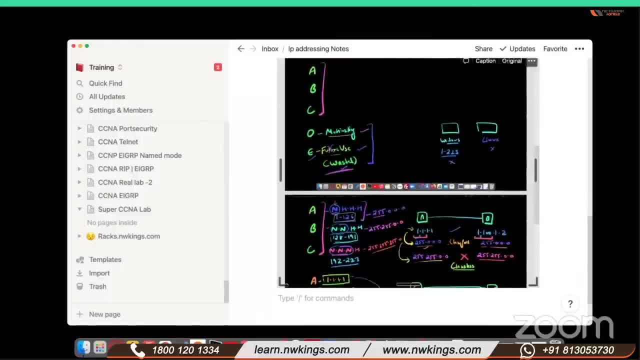 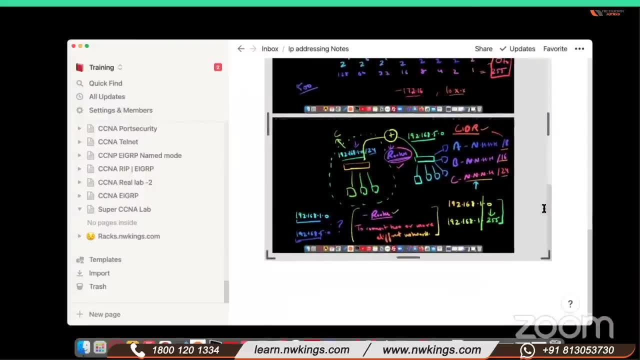 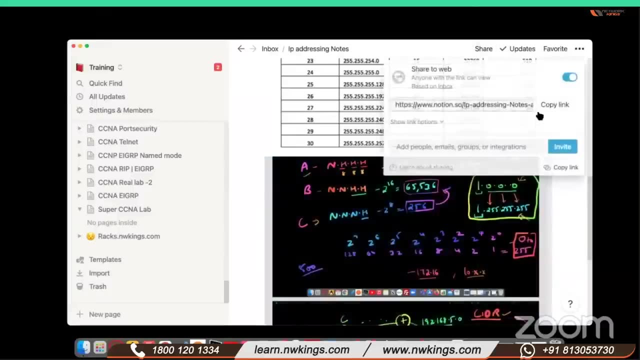 be able to see here. got it, yeah so. yeah, so you can also download if you want, just right-click or somewhere and you can also download this download, okay. so again, last time, again, I am sharing this link and I will try to capture. so just just learn: subnet mask today, okay, so make sure you understand tomorrow this. 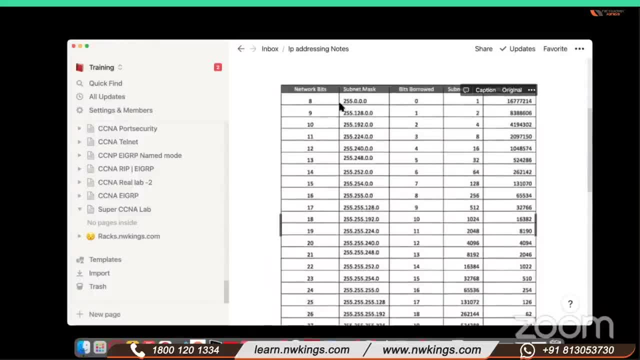 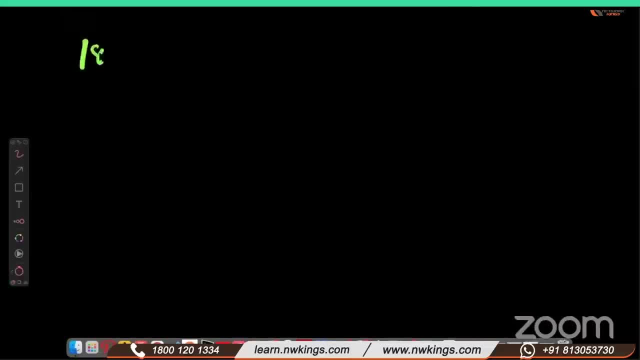 don't cram. okay, so do one thing, just right. just take notebook and write the filips like eight, nine, ten, eleven, twelve, like this, and try to do it yourself and do randomly also like 23,, 21 and 20, and match with your chart. okay, the chart I have shared. 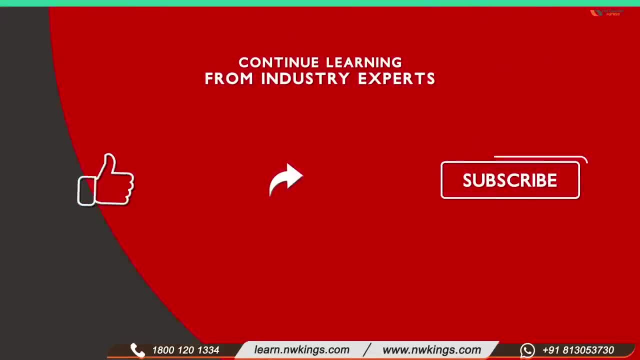 okay, Hi, You are watching the recording from one of our live session. hit like share and subscribe for new updates every Monday on Mustang habi: hi, you are watching the recording from one of our live session. hit like share and subscribe for more succs. 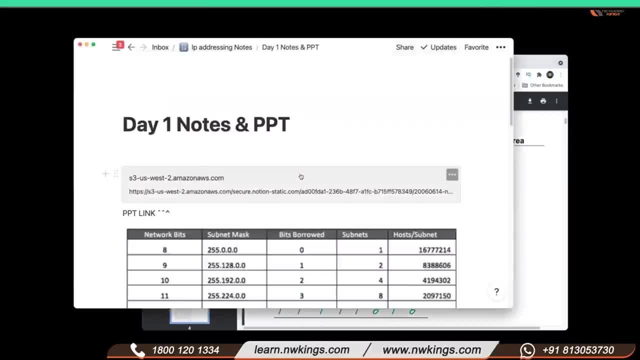 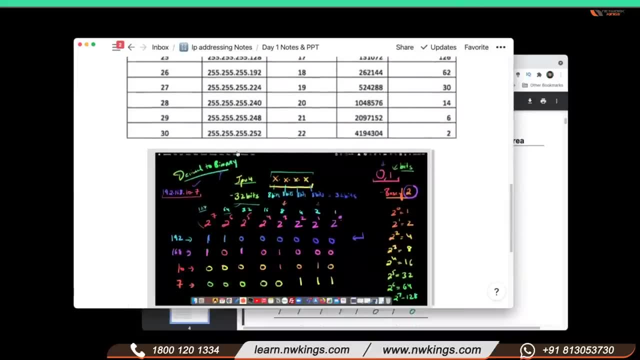 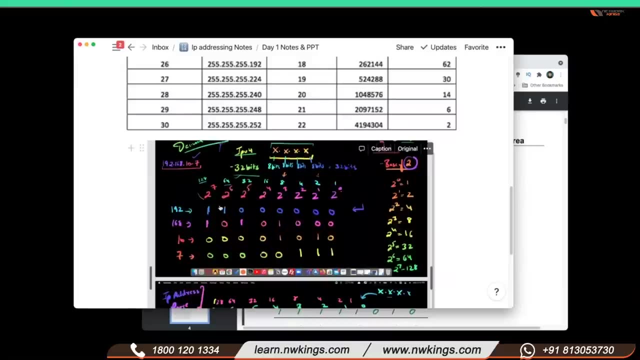 latin** fadsuuuuuuuu. more future updates. so yesterday, what we have discussed, like we discussed about the subnet mask, we discussed about i, a, n, a, aina, so we came to know that what is the decimal to binary conversion? ip version 4 has four octets and every octet is eight bits. so eight bits is represented in the 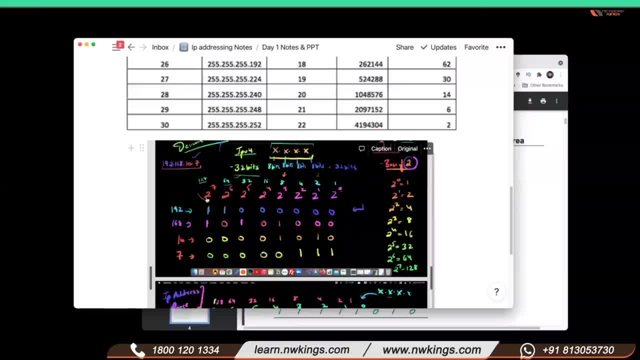 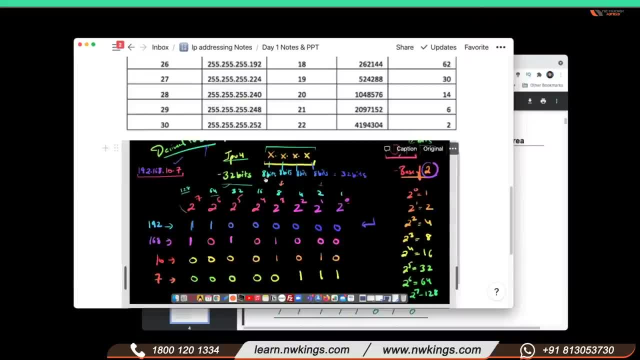 base of two, like to the power of zero to to the power of seven. this is how we represent eight bits. okay, but remember your ip address is of 32 bits, so every eight bits have this block. so this is why, if ip is 192, 168, 10.7, so the binary value for 192 is different, one for 168 different. 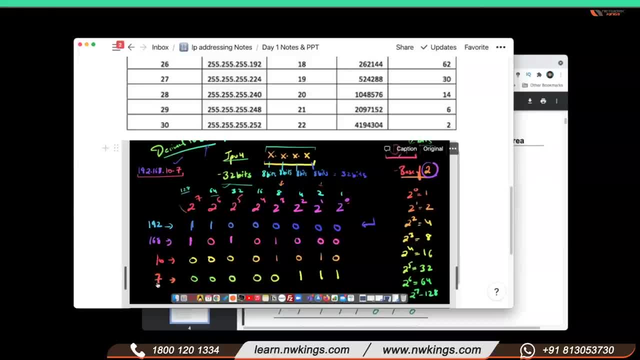 for 10 is different, for 7 is different. so it means when you type this 192, 168, 10.7, this whole zero, once computer understand all these numbers. so this is 38 bits. okay, but remember your ip address is of 32 bits, so every eight bits have this block. 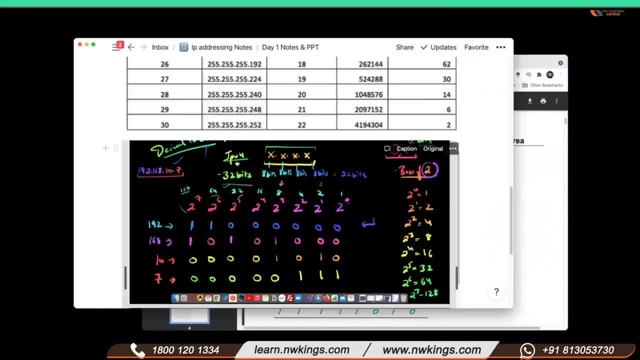 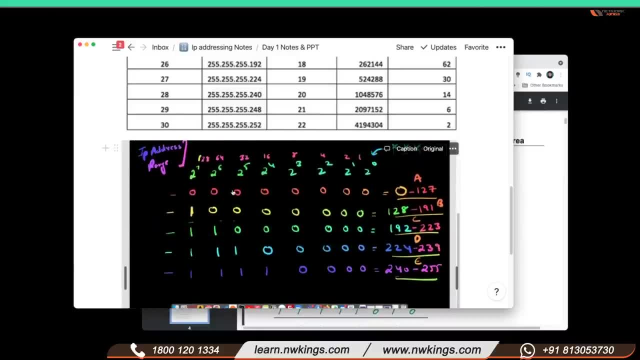 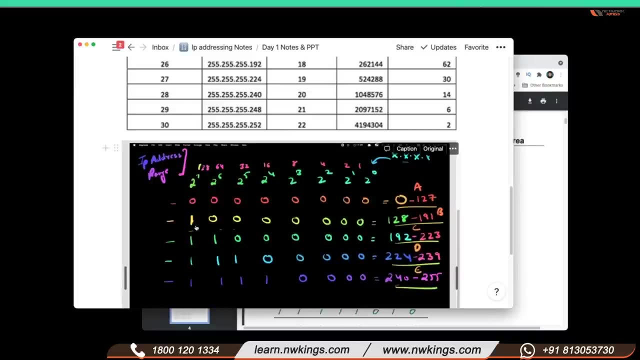 32 bit. so this is why we call ip version 4 32 bit, because it has 32, 0 and ones. okay, so this is what we discussed: how ip address range divided like: in the first block you will put zero. in the second block you will put one. in second block, in third, one you will have two, ones, three. 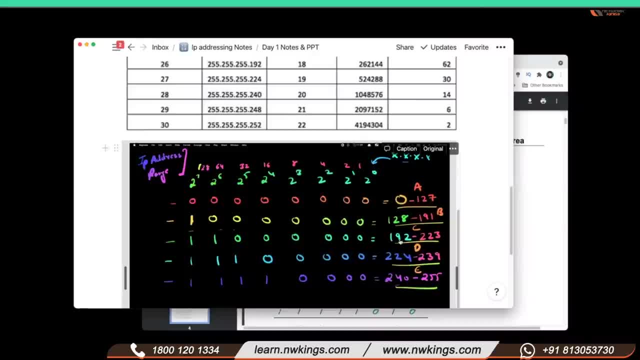 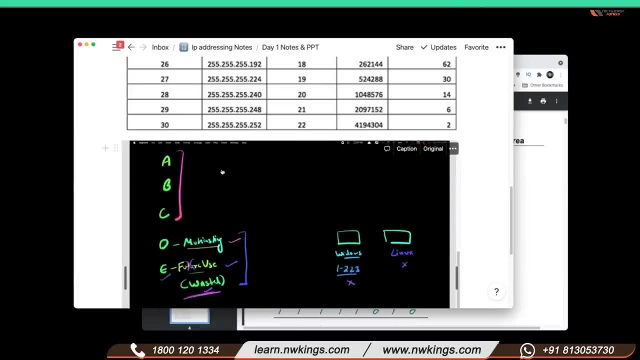 ones, four ones, and then we come to know 0, 128, 192, 224, 240, maximum it will go up to 255. and you, this is how you calculate the range, so you guys can practice the yesterday or previous session. so abc classes are used, okay, we can't give d and e classes. okay. and the main point, 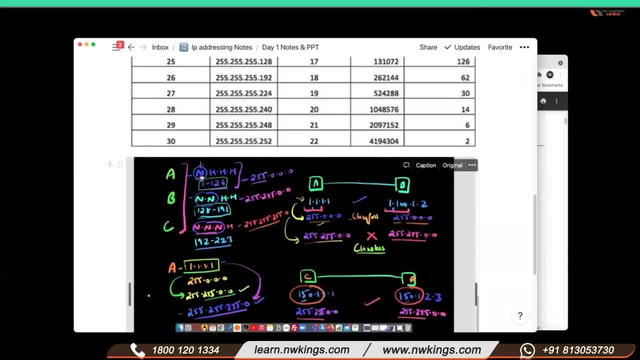 of yesterday class was that class a has a one network part. it means eight bits. so in whenever we give ip address, when we give a class ip, it only checks the first bit of the network part. so you can see here it does not check two network bits, it only tests one network bit and then the 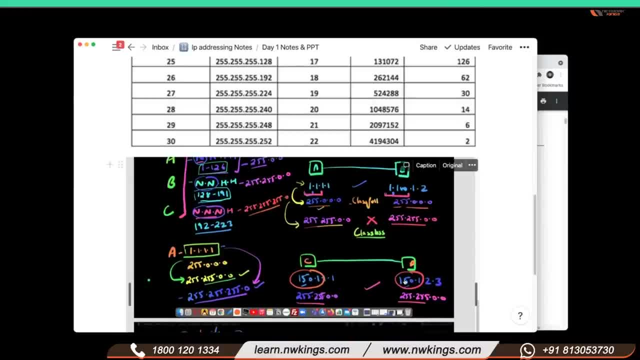 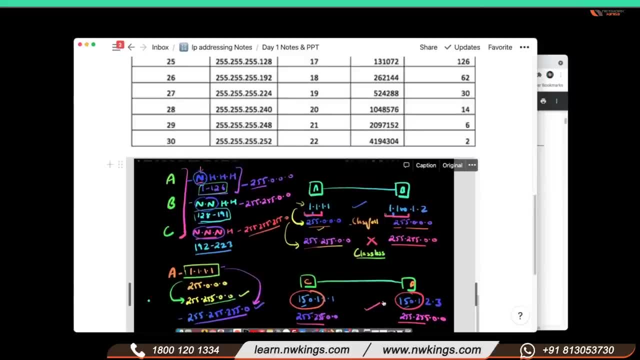 first part. b checks two network parts. you can see 150.1. so this has to match. okay. so class a, ken, there is a first portion match with our b class can there are two portion match with them. and in c class we match three network part and. but this is we know. but how computer. 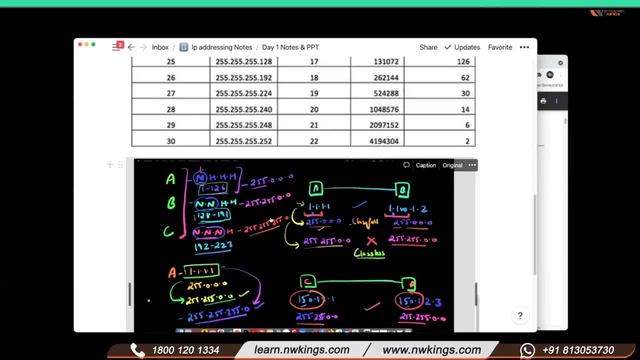 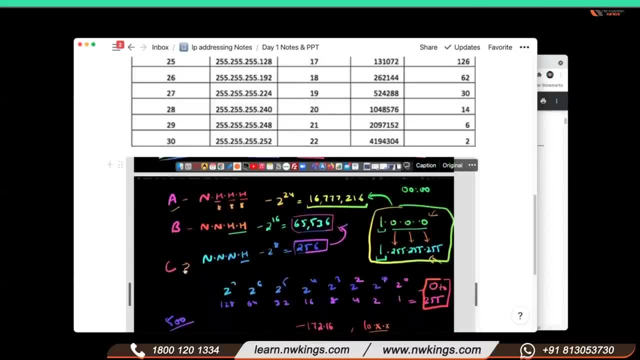 understand this network bits. we give subnet mask, then computer understand. okay, this is like my bit, so we are going to learn today also. and in c class we give ip maximum up to 256 addresses in class b, class b subnet. subnet means network, one portion of one. uh. subnet of class b gives 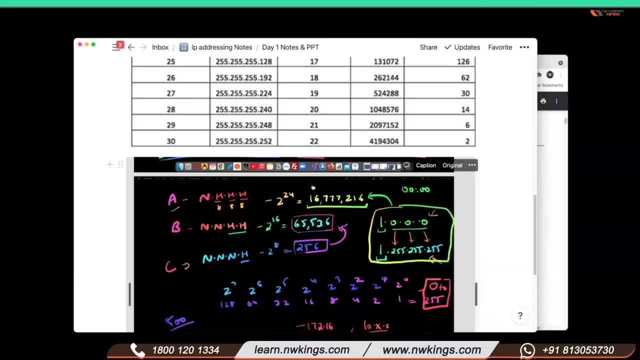 65 536 ips and class is very big, which gives 16 million ip addresses. so every ip addresses start with the network id one. so it will remain same. network will remain same, but host id will start from 0 to 255. so network id same, but host 0 say okay, 255, it will start from 0 and it will end on. 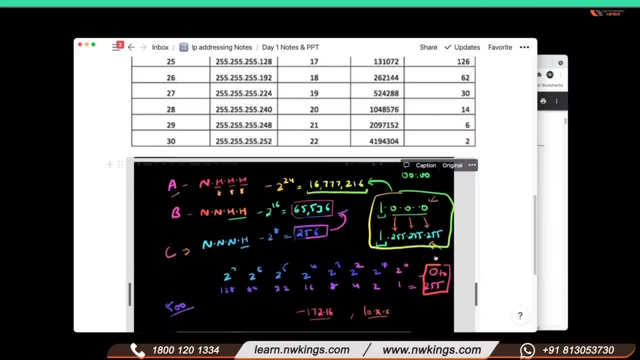 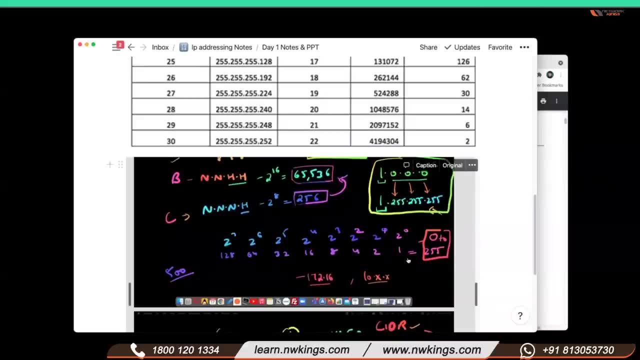 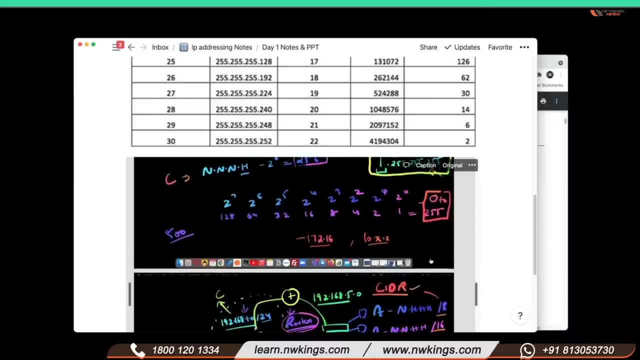 255. okay, so this is what we call range. okay, so maximum. if you calculate your values, if you put all zero, you get zero. if you plus all the values, you will get 255. so this is why every subnet is maximum. you can go up to 255. 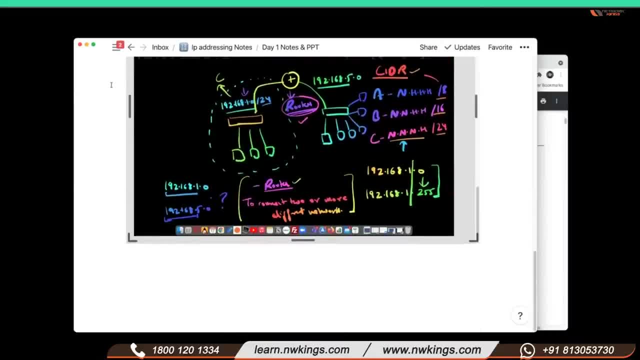 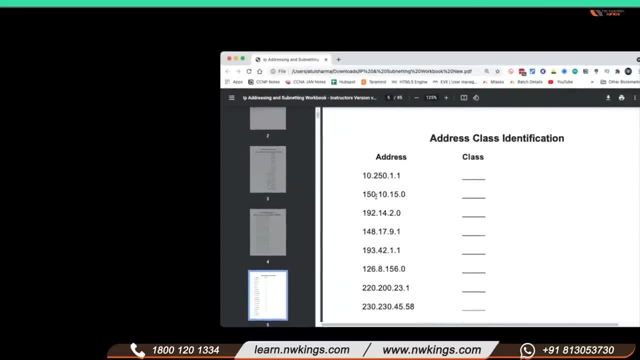 okay, so let's start further. okay, so this is the notes. you will be able to clear. this is so. let's do some practice. i'll share just two, three questions. okay, so tell me what class is this? so this is a. you have to type a. it's very simple, right, or you can take printout also, guys. 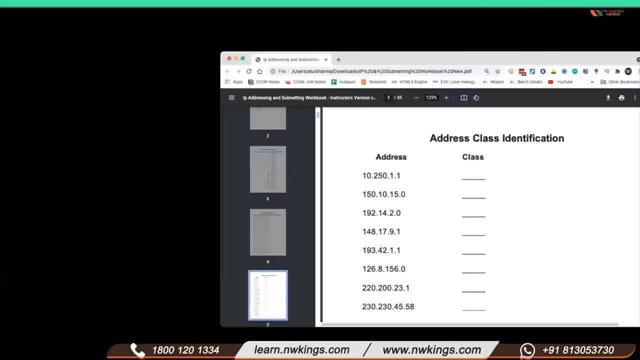 if you have a printer, if you don't love trees, definitely you can take printout also. okay, so this is class a, this is, uh, like b class, right, and this is like c class. so this is very simple, right? so after that what you have to do? so further you go on. so then you have to identify the 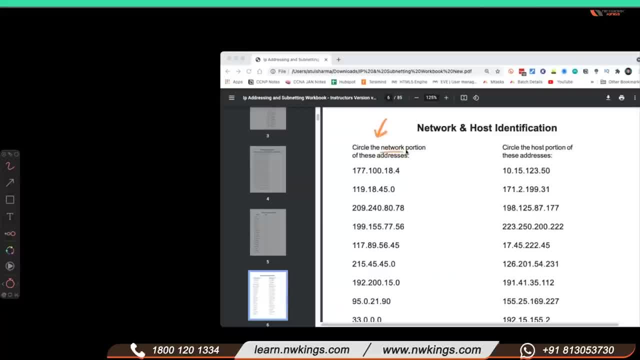 network and host part. on the left side you need to identify the network and host part. on the right side you need to identify the network part. on the right side you need to identify the host part. so this is class b, so the network portion you have to put in circle and host. 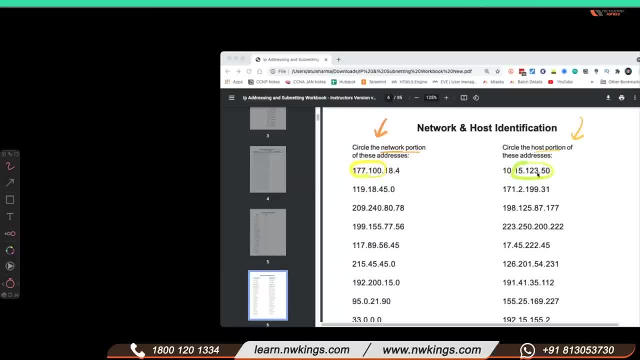 portion you have to circle. so this is class a, so host portion is this. so this is class a. network portion is this: this is class c. the network portion will be three. for class c again, network portion will be three, first three. so this is class a, so it will be 117 only, okay, so remember a. 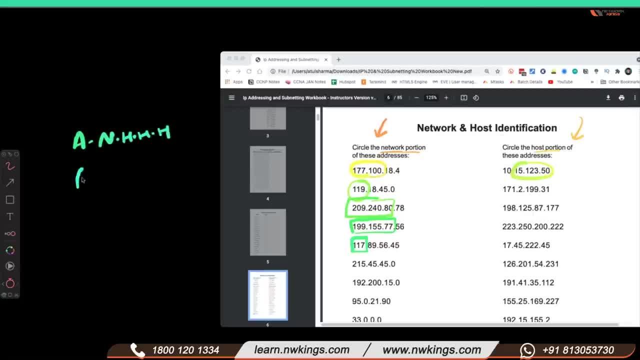 is network and all three host. b is two network and two host and three is three network part and one host. okay, part or octet, you can say that. so this is b, so this is b. so we have to identify the host, host here in the left side network portion. so this is c, so c, the host portion is only this. so you can see. 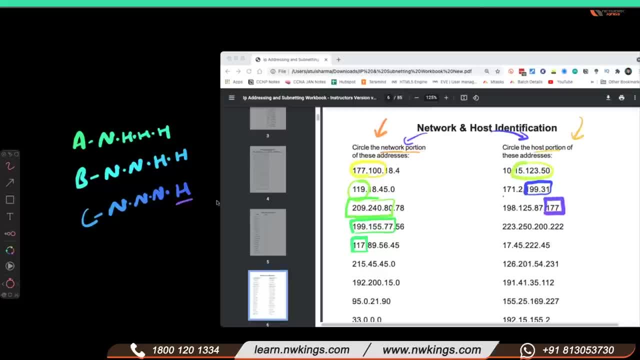 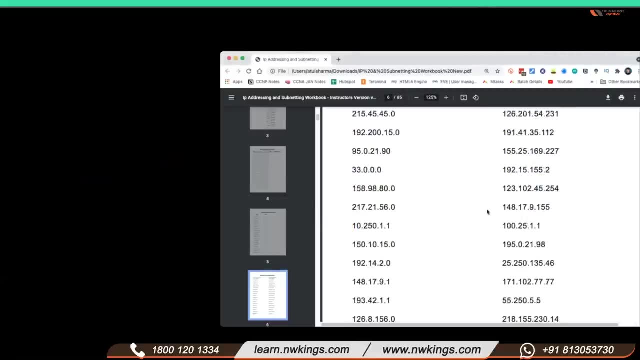 host of class is only one portion in the last. okay, very simple, right so? so, yes, everyone, you guys are able to do this, right? yes, sir, yes, sir, yes, sir, let's take it. okay. so now another part: that you need to identify: the network address. what is network address that router share network address with? 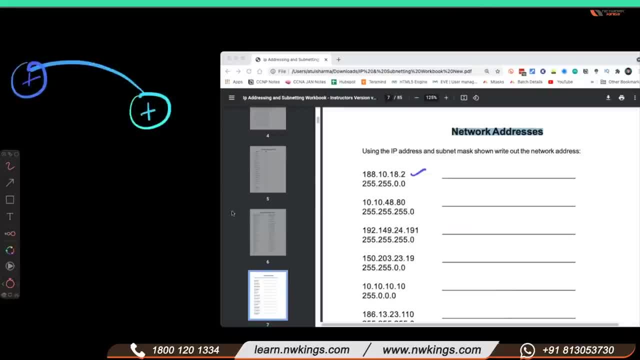 another router. okay, suppose you get this ip 188, 10, 18.2. so your subnet mask is 255, 255. so what will be the network address? just you need to write the first two portion: 188.10.0.0. remember? so when you put all host 0, that is called network address. 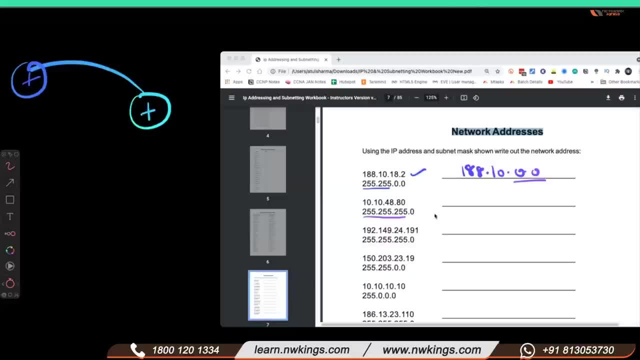 okay, so this has three, two, five, five. so what will be the network address now? 10.10.48.0. yes, okay, if we, if i change the subnet mask to 25500, so the network id will be 10.10.0.0. 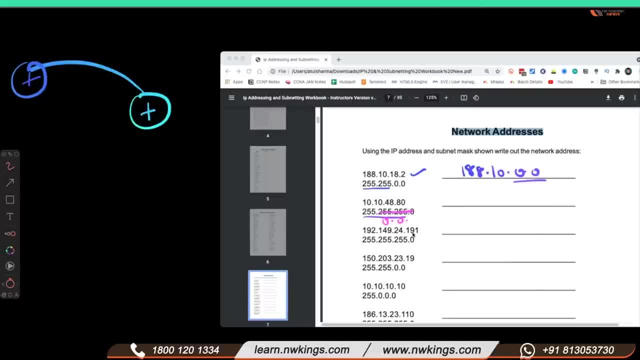 right. so it all. it all calculates with the power of subnet mask. so you can see we have 3255 just to three values: 10, 10, 48, rest value 0. very simple: 3255, it means 192, 149, 24.0, 2255, it means 150, 203.0.0. 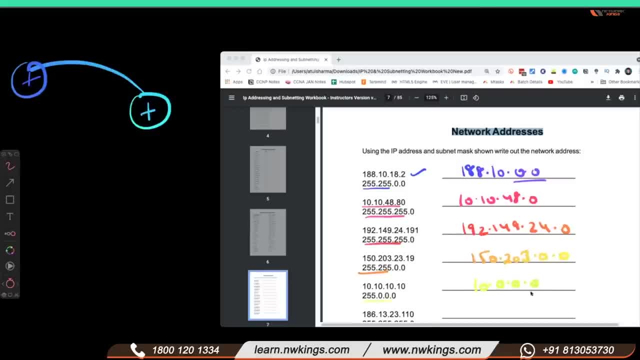 single 255 means 10.0.0.0. yes, everyone, any problem? yes, sir, if there is a another like number rather than 255, like 248 or something, or what i did, that i'll explain. you have to learn submitting, okay, you can't calculate in in this speed. 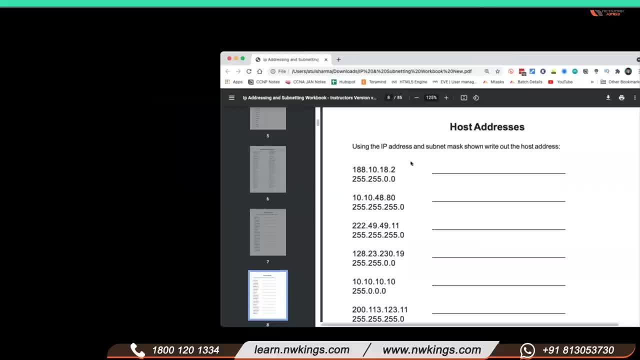 so you have to. so now you can see this is very simple, right? so you have to mention the host address. so just type the zero value. so tell me what is the host address: 18.. yes, only you have to mention the 18.2. so 3255 the hosted. it is only 80, right? 3255 means single. 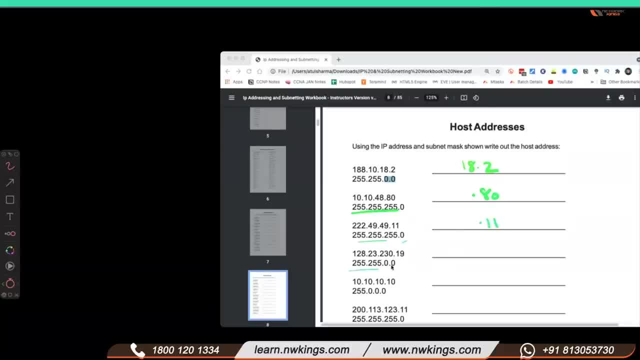 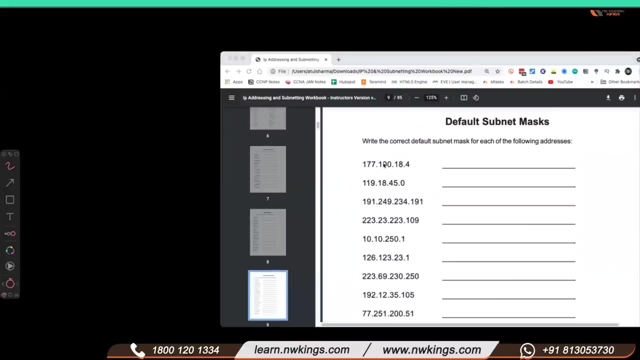 zero, it means 11 is my host address right? and so 2 230.19 is my host address clear, everyone? yes, sir, okay, good, okay, so this is by default the subnet a mask. okay, so these are. so this is which class b, so by default, the 3255, 30. this. why? because we have network part. 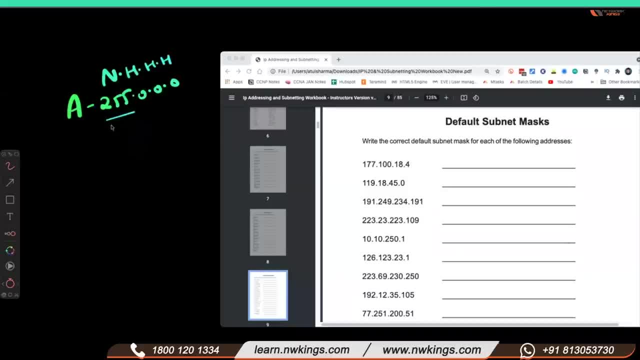 8 bits. for 8 bits we get 255. if you plus all 8 values, you get 255. for b you get 2 times 255. why? because at two network portion and two host portion. this is called slash 8. also slash 16. c is also known as 24, so it means eight eight, eight, three. 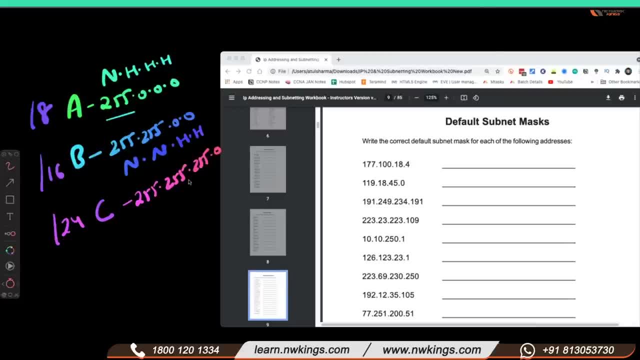 times two, five, five and zero. so this is my default subnet mask. now you can tell me which class is this? b, class b. so two, five, five, two, five, five, dot zero, dot zero. right, yes, so this is class a. so two, five, five, dot zero, dot zero, dot zero. so this is also two, five, five, dot, zero, zero. so if you want, 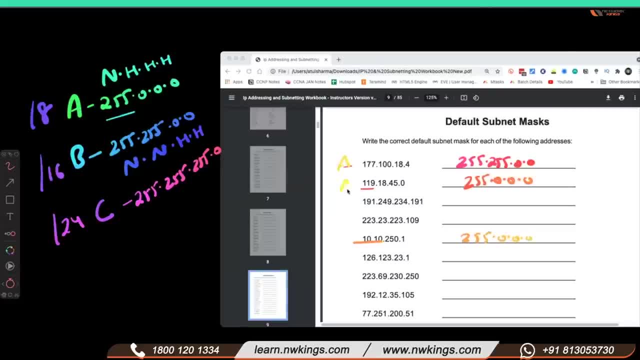 to speed up the process, just find the a class first, a, a, a, a and write the same value right. very simple. so you can check now which is, believe, b class. so, okay, there is no b class, so all are c. now three times two, five, five. yes, all clear. so this is yes. 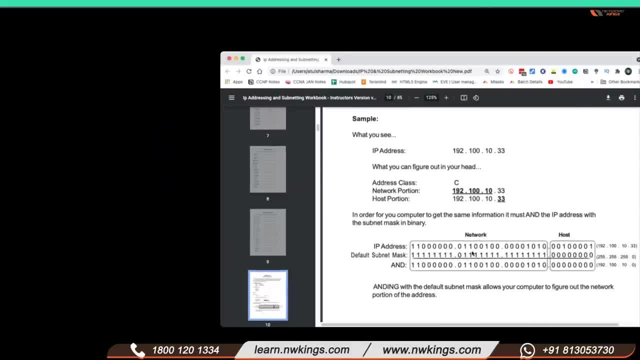 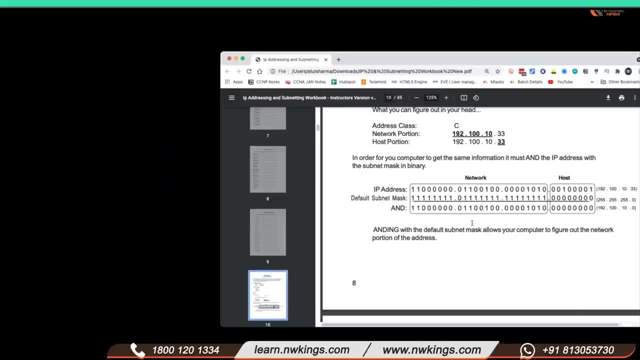 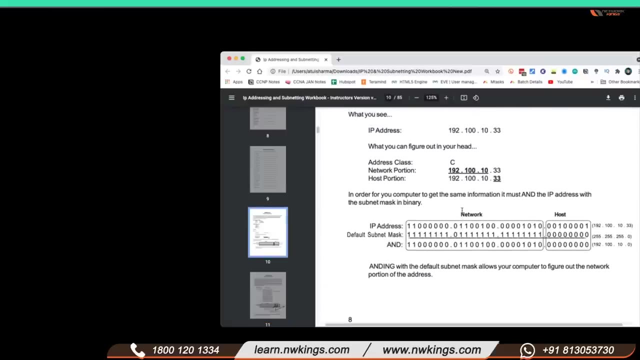 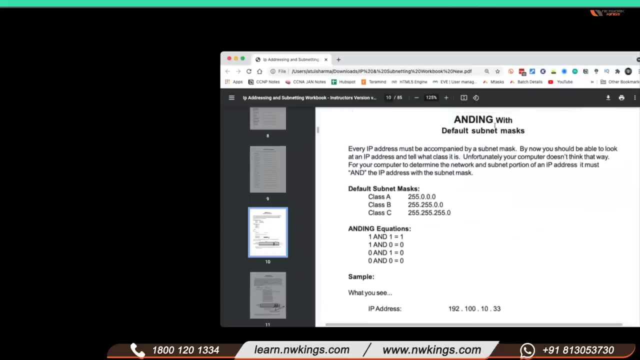 okay, so that is basically how it calculates the network bit. okay, so this is what we call ending process. okay, so what is ending process? so, guys, this is all related to ending what is ending. so it's like digital electronics. if you are an engineering student you must know about and gates, and gates. 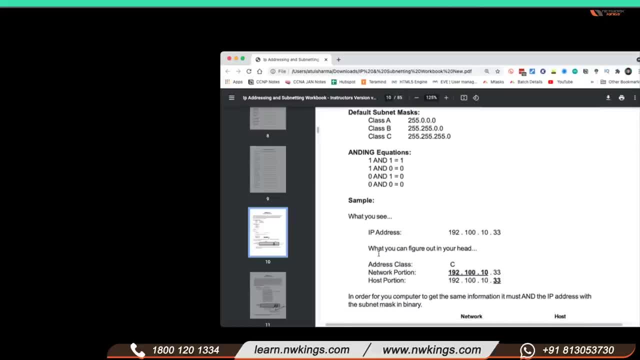 but even if you are not, and from engineering background. so just when computer process are digital values, so in when we use ending: okay, this is, this is behavior of computer whenever it gets one one, so it answer would be one. if one side is one, another is zero, the answer would be zero. so you can see one and one. 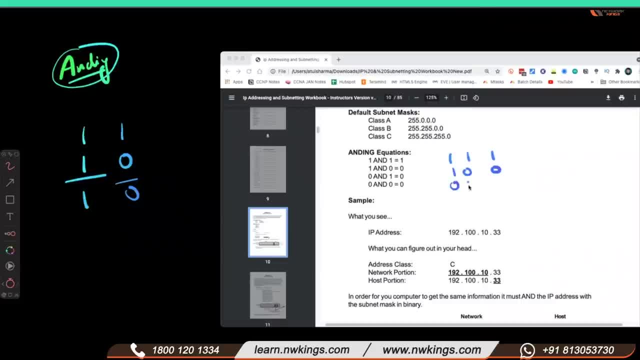 is one one zero is zero, zero. one is also zero, zero, zero is also zero. so only when both the sides are one, then only we are going to get one. so why? i'm telling you this? this is what we call ending pro option, okay, even though it's a submitting class. but i'm telling you, this is the first process. 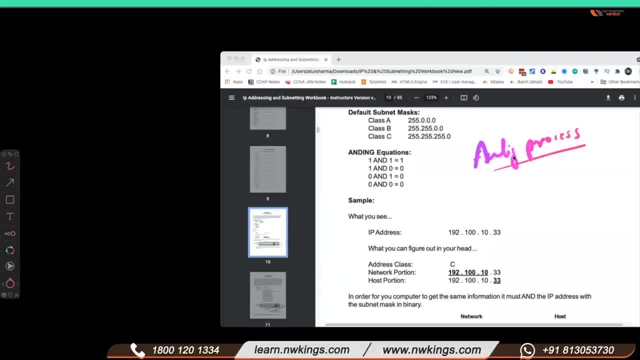 when computer try to, whenever you write, whenever two computers communicate with each other. so first computer ip, suppose 10.1.1.1, another computer is 10.1.1.2. okay, so computer is going to check what is my, what is my network id. okay, and then? those will be keys that i've mentioned once here. okay, all those keys are like two priority parts. okay, that's because there is no, that's people forward click. so that is the first queuing. i say on network details, several days. one second: okay, this is based on communicate with me, because it's like super if you can communicate with me. okay, and as well, in order to communicate with me, i suppose, okay, it may beтьis, but 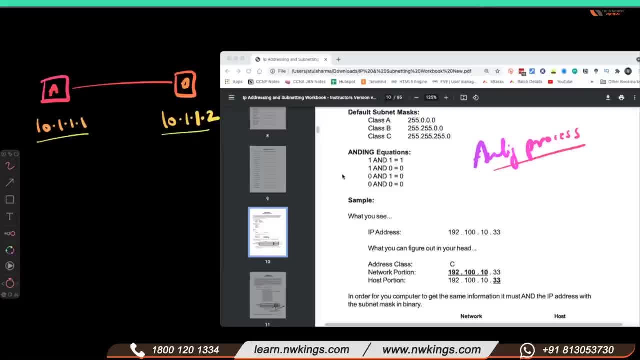 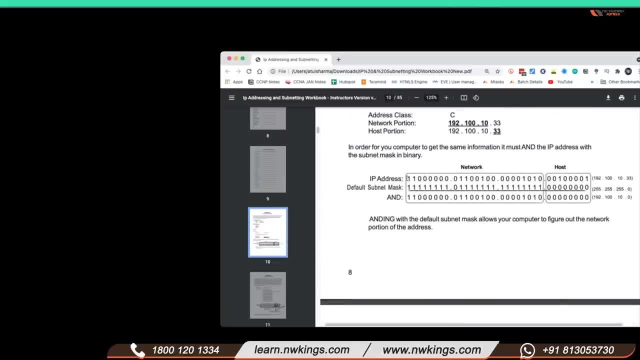 okay, and this also. so how technically it checks. this is what we call landing, so you can check also. so you are going to write, you are going to write the all binary value of your ip address and then you are going to write the subnet mask and then there is, and value comes out. then there. 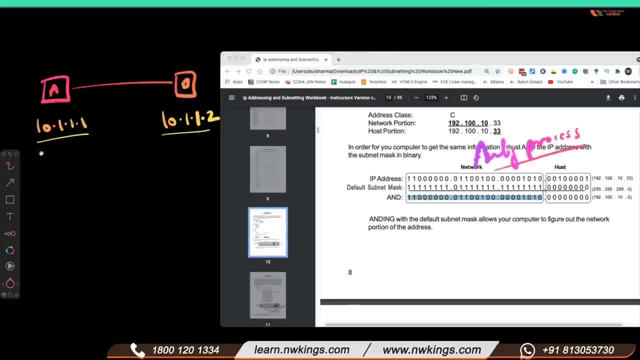 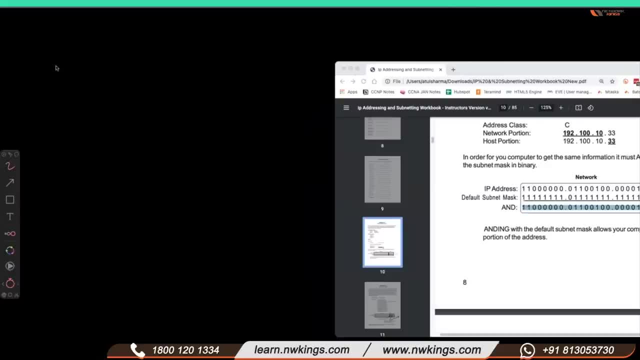 is and value comes out. so let's take an example, but a simple as we just. it's not that difficult, okay, so so suppose ip is 10.1.1.1. so what will be the binary value for this? it will be very big, like. 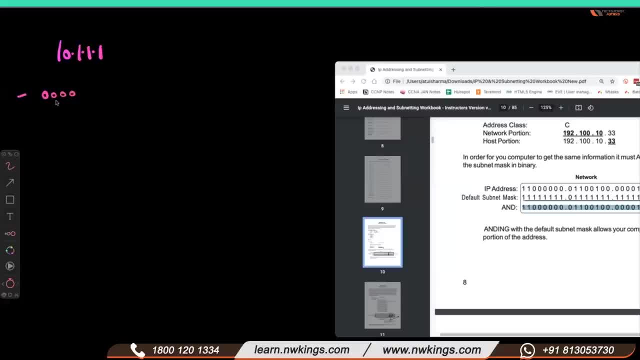 zero, zero, zero, zero, uh, 128, 64, 32, 16, 1, 0, 1, 0, right, 10 and all 0s are in the last. we will have one, the another, last, this binary for this is also okay and last is also clear. and suppose, if your subnet mask is by default 255.0.0.0. 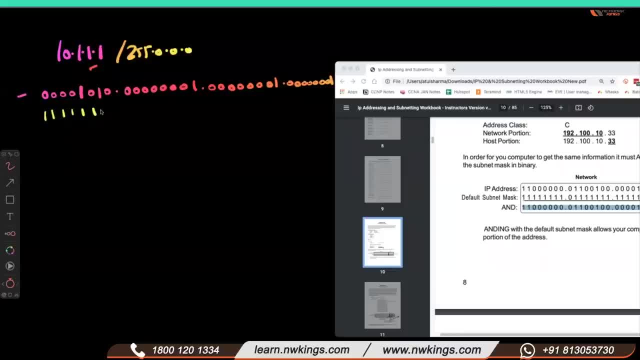 so what you are going to calculate: one, two, three, four, five, six, seven, eight, rest values: zero, right. so first you have to write the binary of your ip address, then you have to write the binary of your subnet mask and then, according to my formula, this ending: so 0: 0 means all zero right, only one means one. 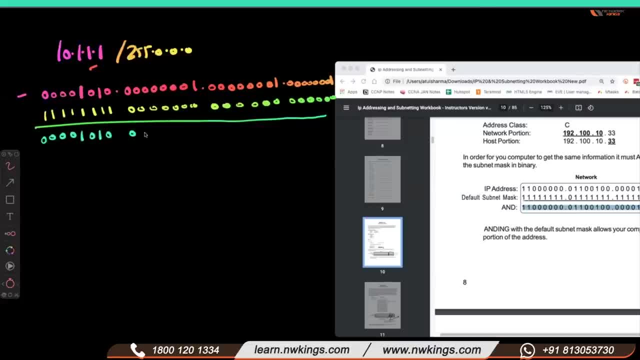 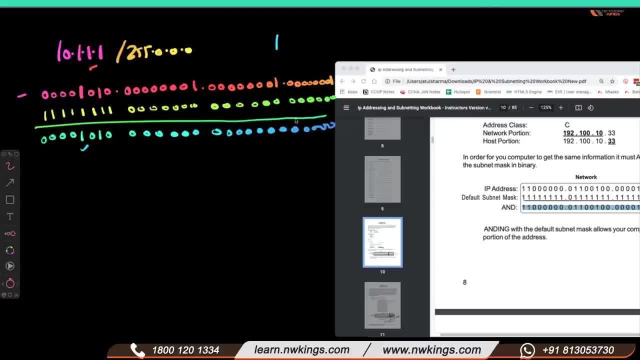 what? zero? yes or no? yes, sir, okay. so this is what we call ending process. okay, and now if you calculate, this is 10, this is zero. this is zero, this is zero. so this is how you also calculate your network id clear. this is how your computer identify. this is my network id. and if you calculate, 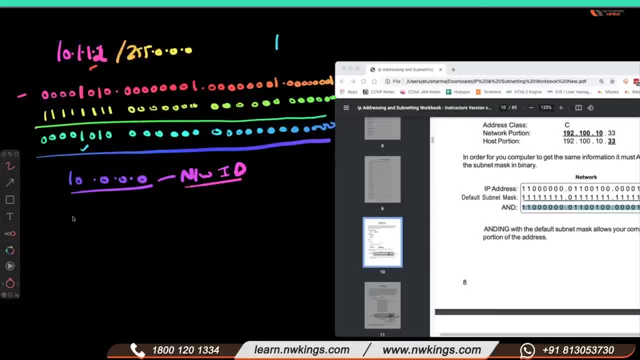 for another computer, 10.1.2. so the answer would be same, yes or no. if your ip is 10, 1, 1, 2, the answer would be same. it means both the computers have same network id. it means they will able to. they. 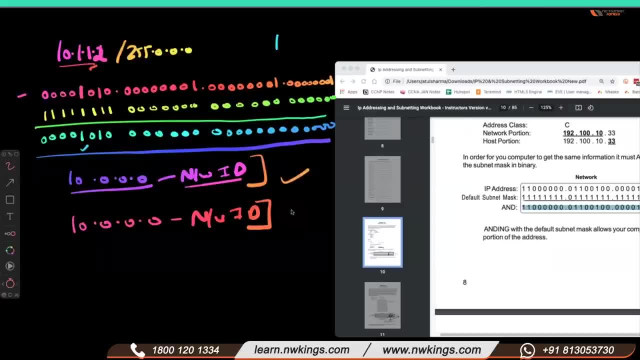 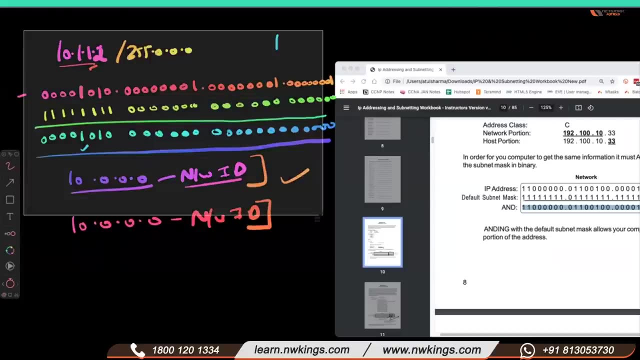 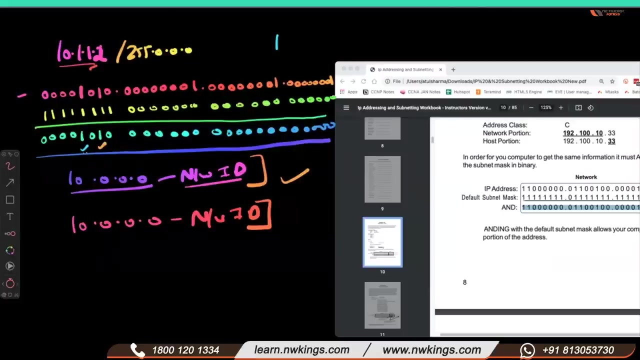 are going to definitely connect with each other without any router. yes, because same network does not need router. yes, clear, yes, sir. yeah, sir, last japan is a sub 1pana second line. your first say yeah, 8 plus 2, 10, over there, one network address at all. sub your one at 255 value. 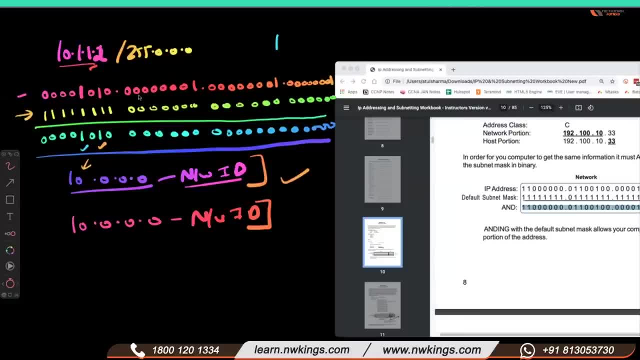 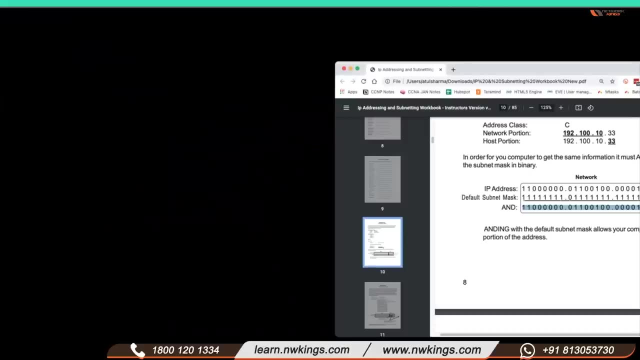 yes, yes, this is subnet mask. yes, this is okay. yeah, this is ip and this value you are getting from here, okay, so this is how, so you can read this book. i'm just telling you because i don't want to, uh, actually make the things complex, so it's very easy. if you read this, you will come to know this. 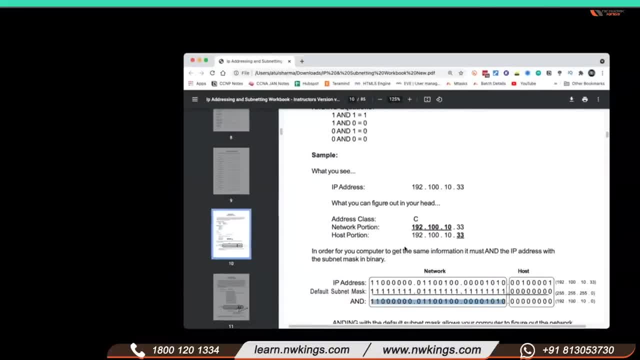 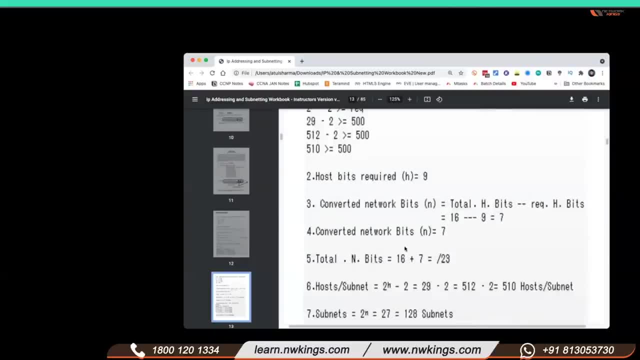 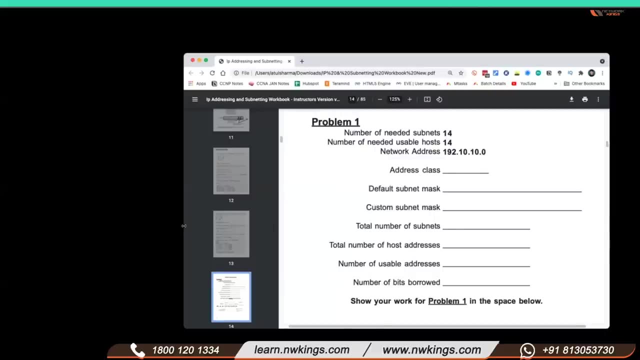 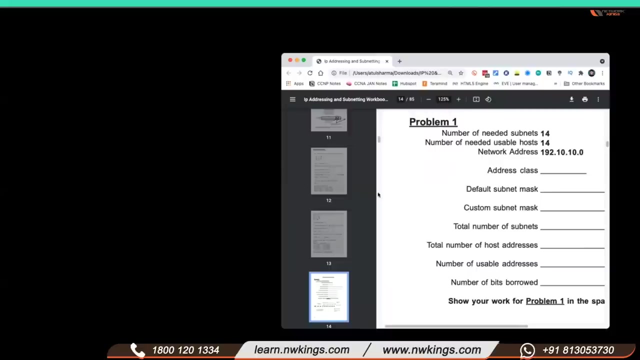 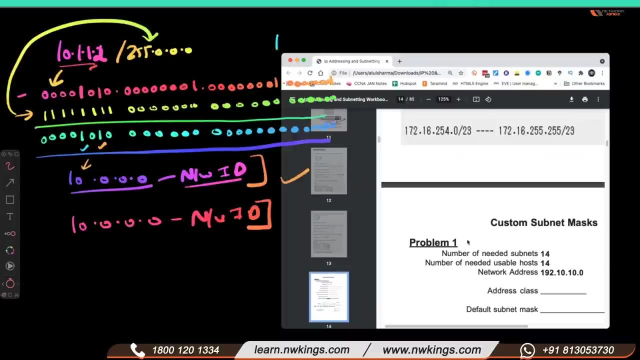 is a default subnet mask and this is the ending equation. if you calculate, this is how you identify the all your network ids. okay, sorry, it's three days workshop, okay, so guys. uh, now you can see there is a problem and we are going to solve this with our tricks. okay, so we? 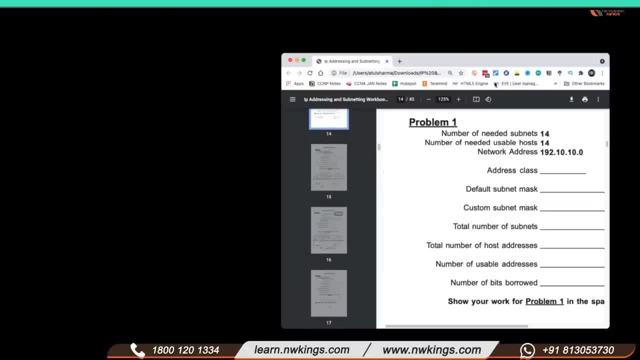 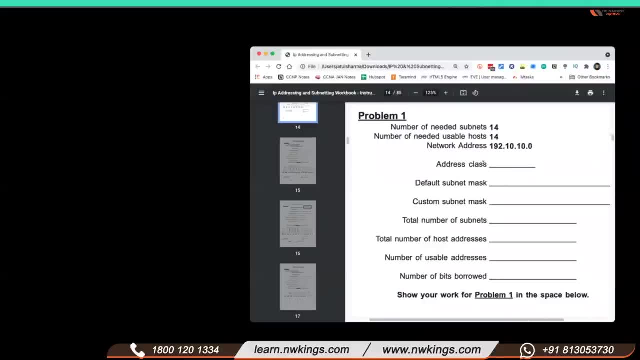 have to do a lot of questions, then only will be getting my trick and you have to understand that same trick. okay, don't worry. if you don't understand one problem, no worries, we are going to learn a lot of problems. i'll try to complete almost 40- 50 problems. 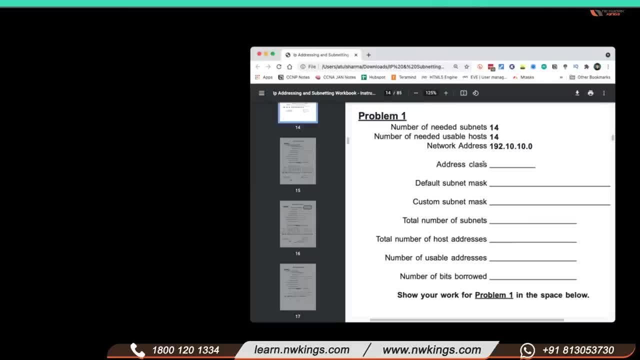 and which will make sense so that you will be able to complete all your submitting questions. okay, yeah, see, so this is a problem. one, okay, number of needed subnets: number of, so any company, even so, what is subnets? so subnets means you want how many networks. suppose there is a computer. 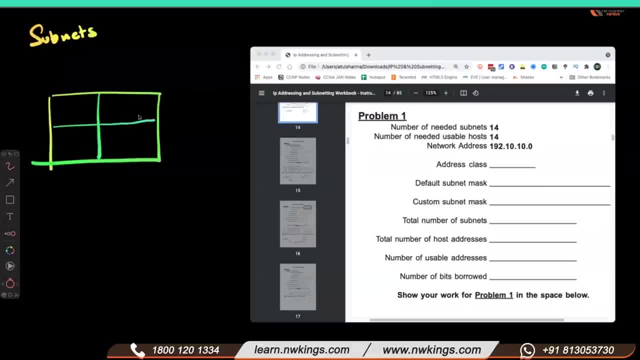 lab and in your, your manager is telling you that you have 192 ip. okay, this is class c, remember. so it has three n and one h. yes, clear, and h means eight to the power of eight is 256. so, in short, in short, when you calculate 190 to 168, 1.0, it will go up to 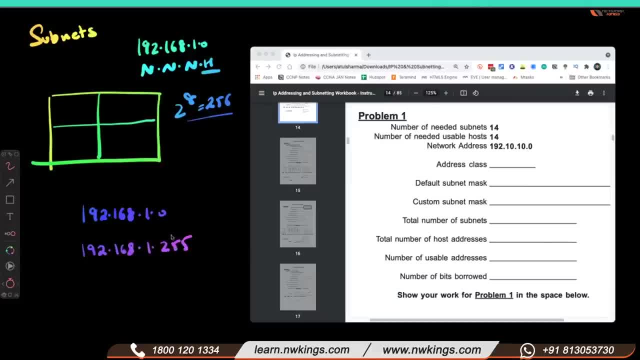 190 to 168.1.255. right, this is class c and host portion start from zero and it ends up to 255. you know this right. so now, if i'll talk about this, so this is my host portion, but if your manager or someone is asking, 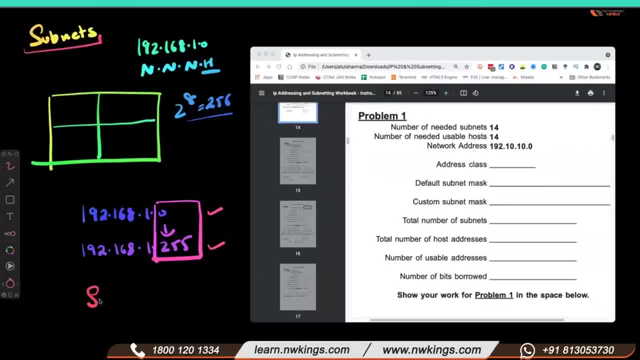 you to create subnet. subnet means sub network, subnet, subnets means sub networks like small portions, or, in short, subnetting means divide a big network into smaller part. what is subnetting? divide a big network into smaller part and divide a big network into smaller part and divide a. 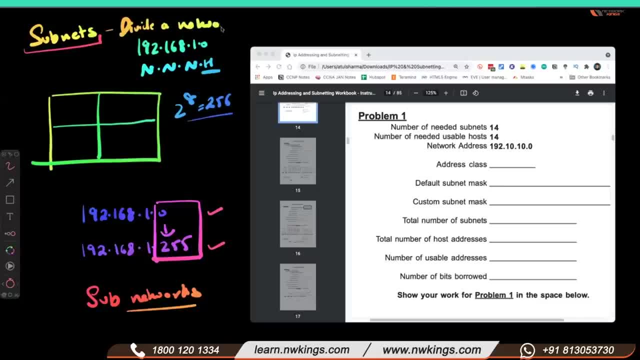 network into smaller parts, into smaller parts. so this is what we call subnetting and why we do subnetting: to reduce the wastage. to reduce the wastage. so if we have one block ip address, right, if you don't do subnetting, what will happen? you have to assign four blocks to all the computer. 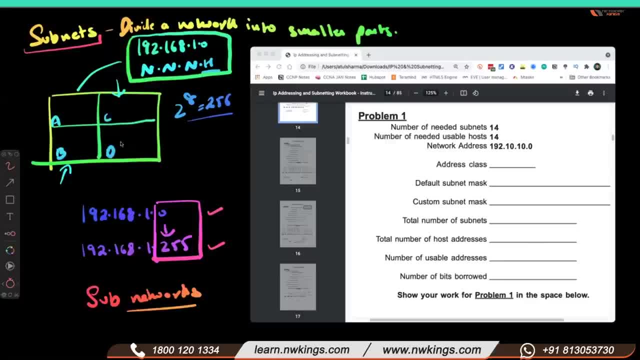 labs: computer lab a, b, c, d, for all computer labs you have to give different network, right? you can't use the same network everywhere, right? so definitely, and your requirement is that you should have different network. so requirement is different. i'll explain that later on, but as of now we want: 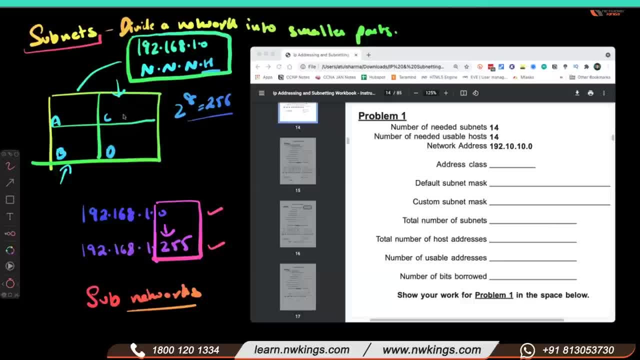 to make our like. we want to make four computer labs. so in short, we want four subnets. so if we want four different networks, this is what we call: four different networks, called four subnets. so you can see the question. now the problem one is asking to divide. 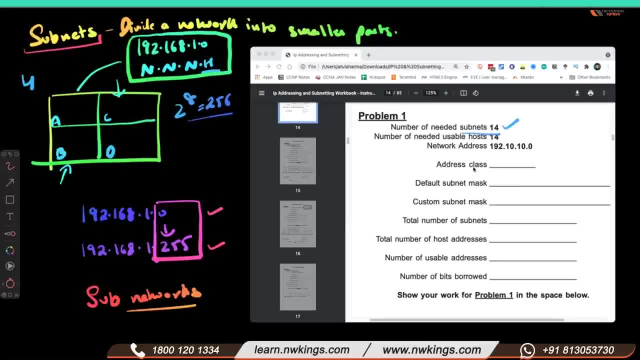 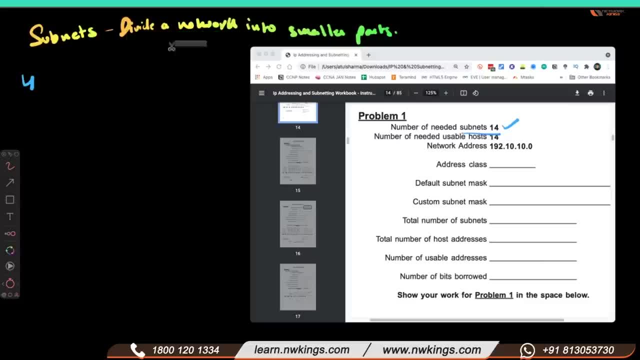 my network into how many parts? 14 parts, right. so it means, if we have any ip, so you can see this ip192. so we want minimum. this is minimum. okay, network address is 192, 10.10.0. so this is class c, so by default this is class c, so by default your network bits is 24. 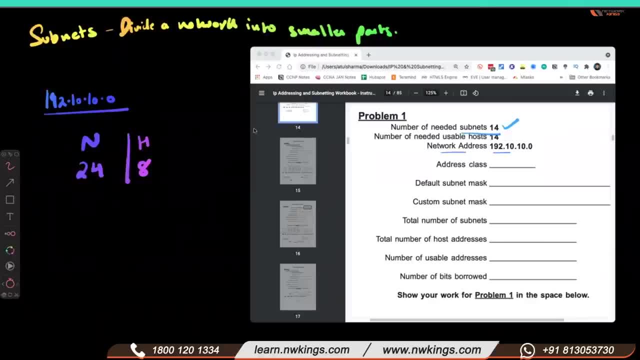 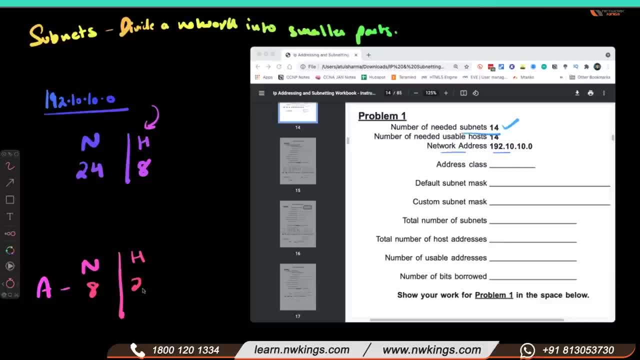 sorry, sorry. so network has 8. host is 24.. so in be bulb bits and 16 host bits. please note down this: we have 24 network Bits and 8 host bits. so this is by default. so you can note down please. whenever i am going to do question, you should. 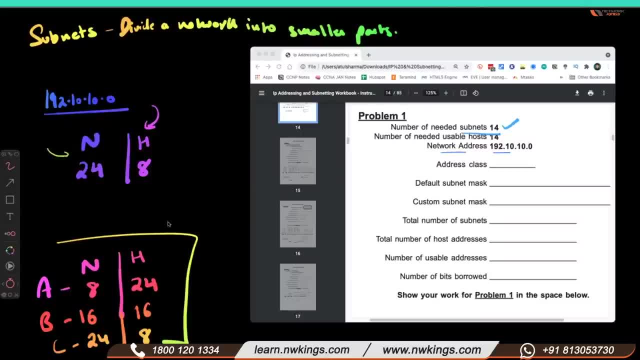 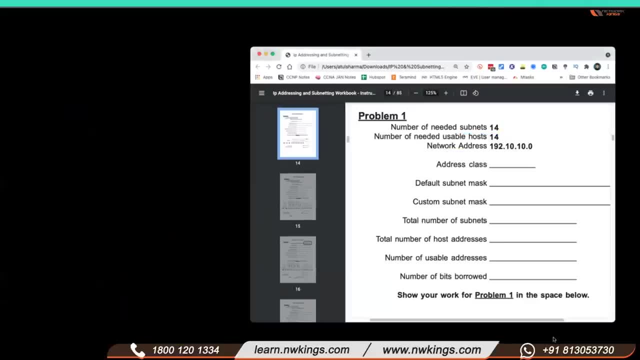 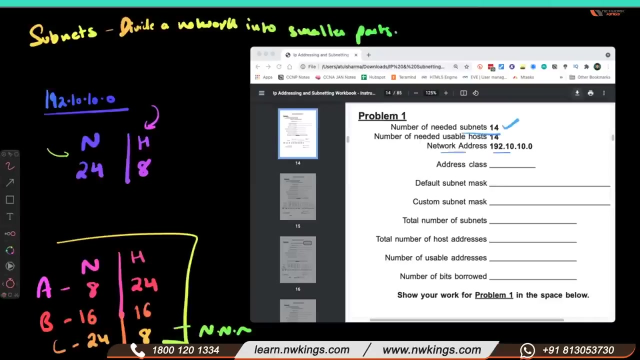 understand this, why i'm telling you network is 24 because class C has three native portions. just hold on, guys. okay, yeah, okay. so now let's please note down this, okay, so now let's understand the question. so the question is saying: we want 14 subnets, okay, so. 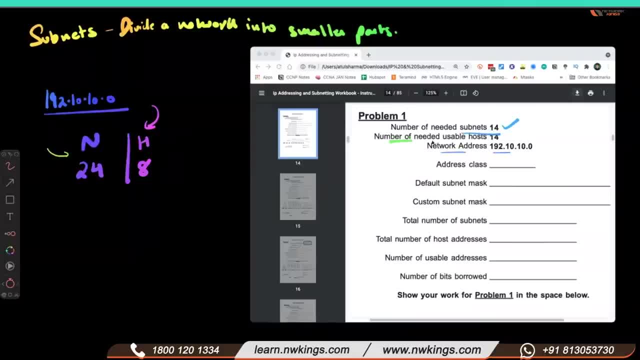 14 subnets and we want 14. every network will have 14 computers, so it means 14 networks. understand this? 14 computer labs we want, and every lab we need, 14 host. so each lab will need 14 host, right, and this is class c. so we need to answer these questions. what if default subnet mask? 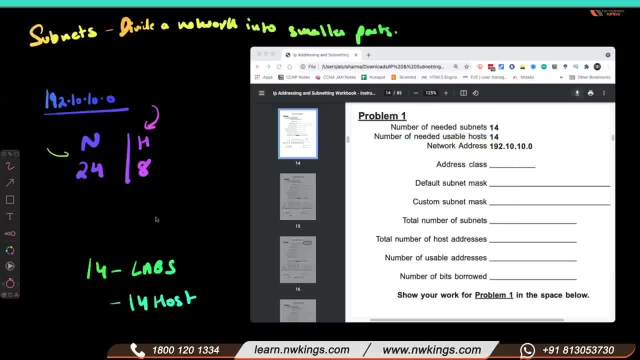 so this address class is very simple. so this address is class c, so this is c class by default. subnets mask is 255, 255, 255.0 right. custom subnet mask means how we are going to get this, so we are going to learn. okay, so let's not discuss the problem number one. let me explain some questions from my 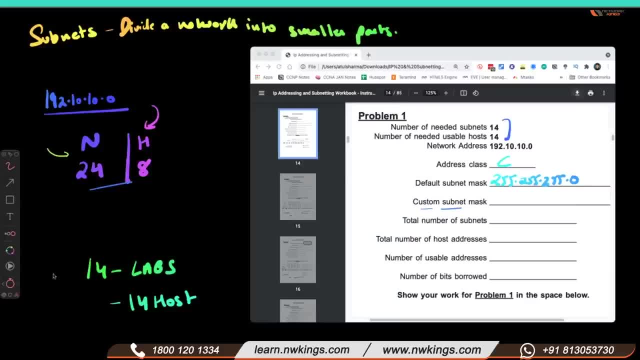 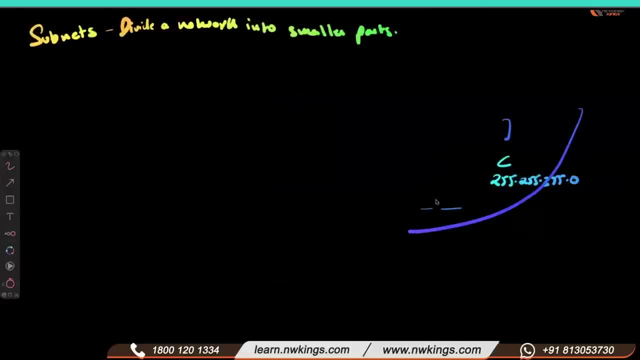 end. then we are going to check this problem one. okay, so let me explain you something which is very interesting. okay, so let's do the simple maths first. okay, so, guys, i have ip 192, 168, 1.0. okay, so this is ip block. okay, we have given to all our computers. this is so i want you to uh. 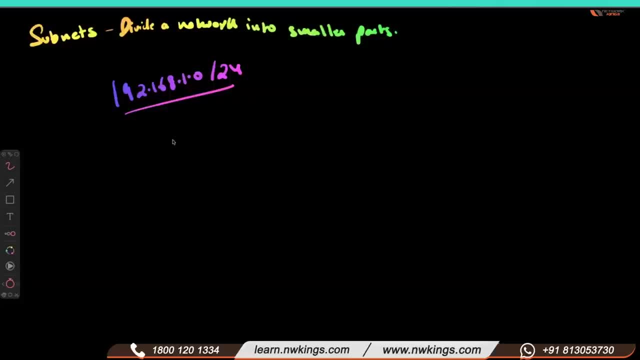 default, this class c gives how many ip addresses to the power of 8. is it around 256 ip? okay, but what is my requirement? i want set. i want to set up two computer labs. i want to set up two computer labs with this network. i want to divide this network into two parts and where i want a hundred. 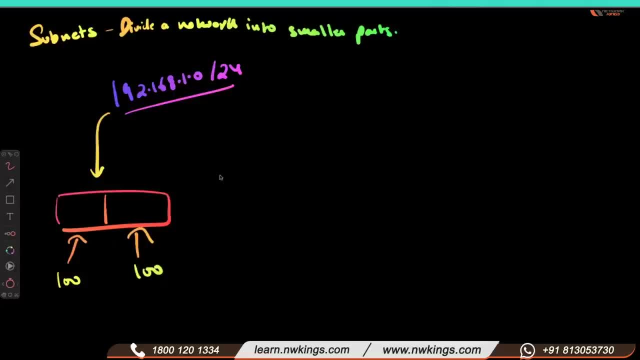 computers, each minimum hundred computers, okay, and you can see, uh, this class c gives 256 ip and it is easy to get hundred hundred computers, right? so you can note down. network bit says 24, host bit is eight. this is by default of class c, right? so please note down this table to the powers. 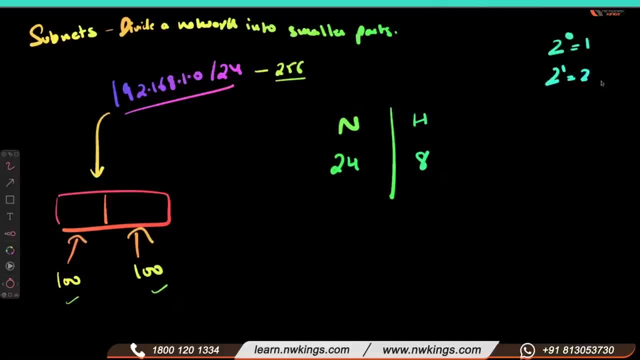 to the power of zero is one. to the power of one is two. to the power of two is four. to the power of three is eight. to the power of four is sixteen. to the power of five is thirty. two. to the power of six is sixty. four. to the power of seven is one. twenty eight. to the power of eight is two, fifty. 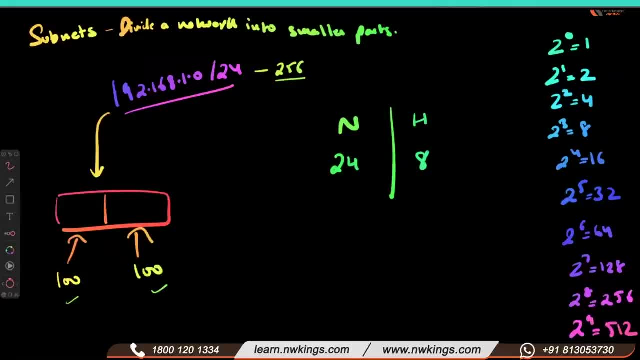 six to the power of nine is five, one. two to the power of ten is one, zero, two, four, and you can keep checking. just double the value. but for as of now you can understand this value. so you can. i told you class c is giving 256 ip because my host is: to the power of eight is 256, right? this is why. 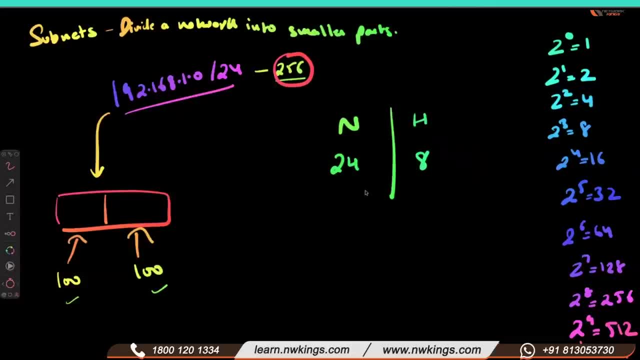 computer. class c gives 256 ip, but what is my requirement? check the requirement, guys. my requirement is only 100 computers, so eight, eight host bits. give how many ips? 256 ip, but how many? i want 100, but we can't take 100 exactly. suppose you want to eat some pizza? you have to. 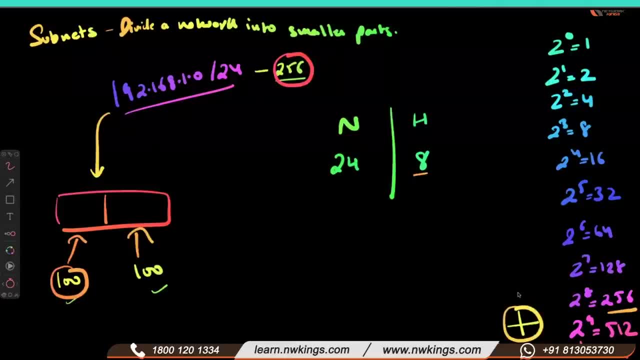 eat the portion you can't say. not that i want to have just one bite, please give me okay. you, either you have to divide the pizza or you can take small one, even if you take one bite or two bite, but still you have to pay the same way. even if you want 100 ips or 110 or 120, you have. 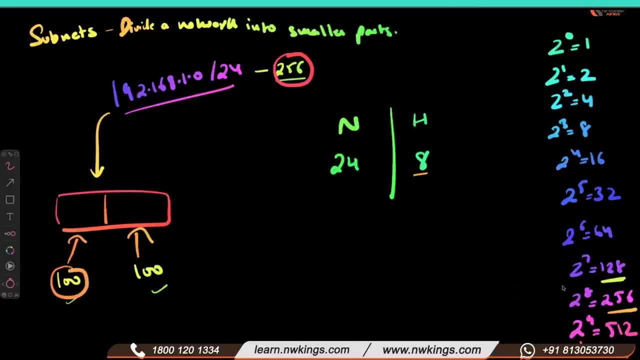 to use 128 portion. so, yes, definitely ips are getting wasted, but we will not. we can't eliminate the redu uh wastage. we can only reduce. then we can only minimize the wastage. we can't remove it. okay, it's like a simple one, like if you want to buy a plot of land or what we call plot or something, so you have. 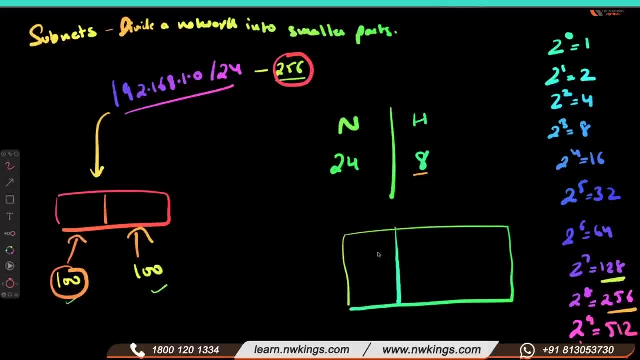 to buy some particular area, maybe like a 500 square feet area or maybe a 1000 sqf area, you can't say: i need only 250.. okay, okay, so the same way, what we call subnetting. so if you want to give 100 ips, you have to use that to the power of 7.. so, so what? we will say that i don't need 8. 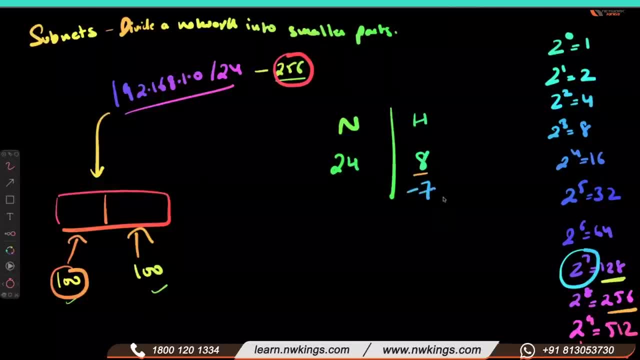 instead of 8 i'll take 7. only very simple, right? because i want 100 computers, 400 computers, host bit 7 is okay. i don't require 8, right? so 8 minus 7 is 1, so this 1 will be added to this side. 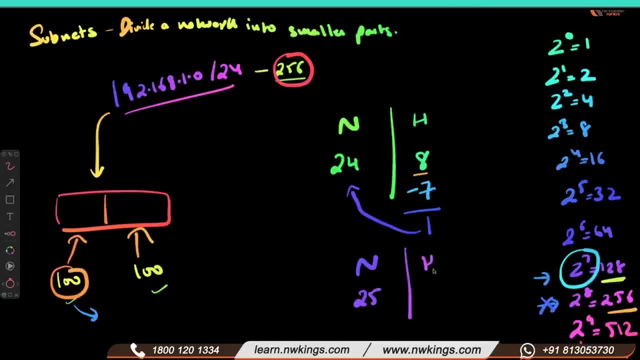 and network becomes 25 and host becomes 7.. right, very simple. yes, so now you can see this network. this is what we call network id and how to write the subnet mask. yesterday i have explained you that's subnet mask, for 255 is 8 plus 8 plus 8 plus 1. that makes 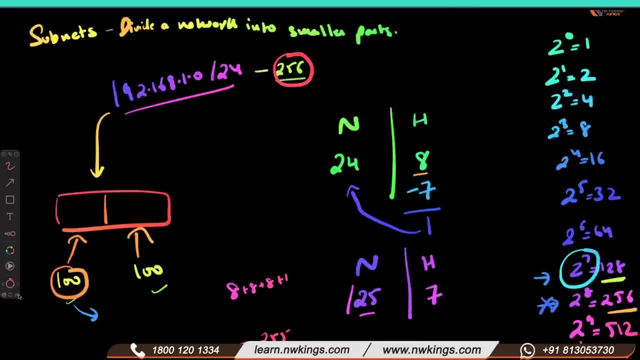 255. let me write in the clear space. the subnet mask is very important: 255, 255, 255, dot, 128. you can check. so again, i'm telling you, if you get one extra bit, you always i add 128 for two bits, you add 192 for. 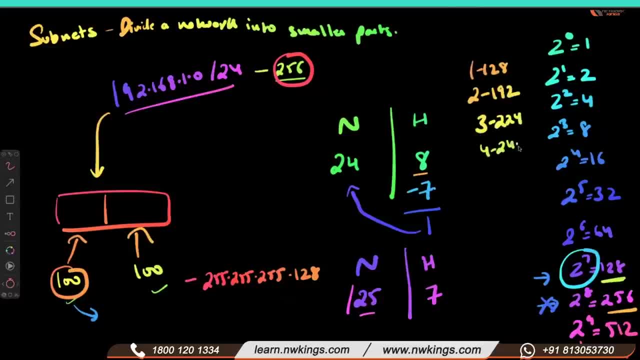 bits two to four. if you don't understand how it is getting, please watch yesterday or the earlier class. very simple, let me complete this. i'll take your questions, don't worry. okay, so this is my subnet mask now, right, so you can see. this is my value. i got 25 and i need to. 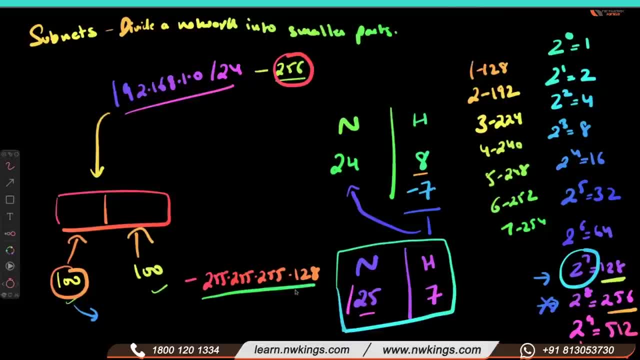 assign by default. my subnet mask was for this. by default is 24 my subnet mask. when we give ip without subnetting, we give this subnet mask. but when we divide the network into parts, we are going to give this subnet mask. but how we are going to assign the ips here and here in this block? 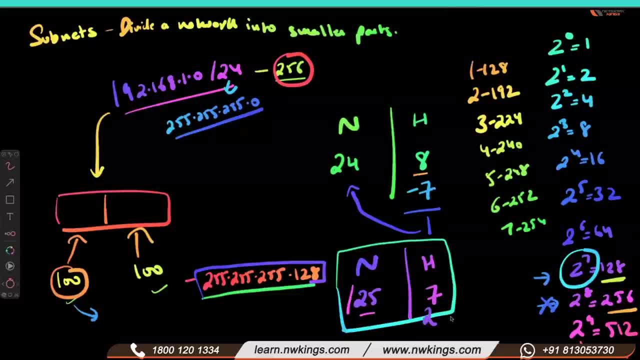 so you can see, the host part is now to the power of seven and this comes 128. right. so very simple, how to write the blocks or how to give ip to this. blocks so you can just make two blocks divide, okay. so 128, so you can every ip you can see start from. 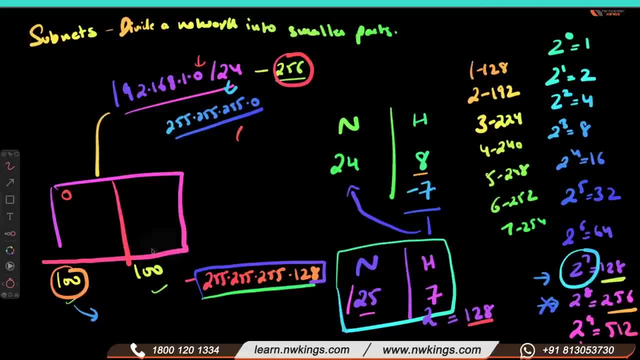 zero and it ends up till 255. right, all ips start from zero or khatam 255. so now you can see this. we got 128 right in the second block. and before 128, what is the value? 127. so this is my computer lab a and this is my computer lab, so how you are going to assign. 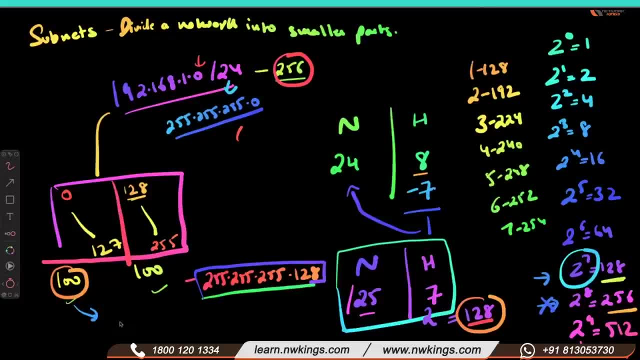 the ips here or in these computers. so you are going to give ip like 192, 168, 1.1 and 255, 255, 255, 128. if you give any ip on this side, on this computer lab b you are giving, any ip belongs to. 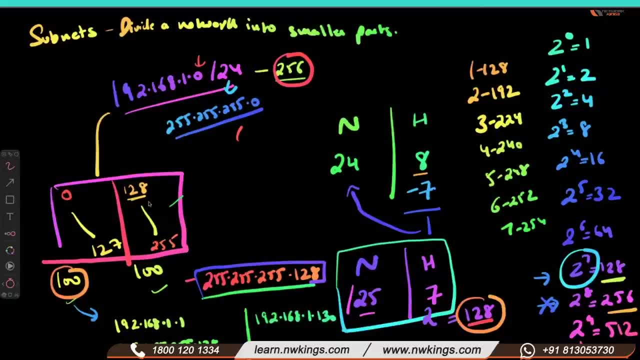 but remember, when there is this point and when you see theåt- the other one- you are giving any five- Monetee in the third ring. you are giving project promotion to this. so let's take this employee. the first condition here is one: not was gonna cancel the. 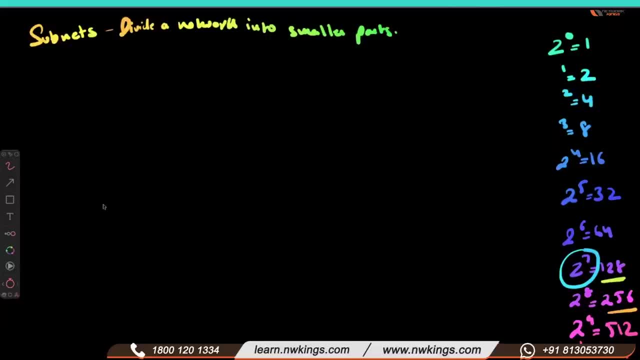 impulsivity, for example. so the client is going to look at what do i have here? a help: case 152, 168, 1.130. so 130 b lies between this group right exotesis under r. so 255, 255, 255, 128, very simple, yes, ok, so let's not waste time, let's try to. don't worry, i have taken the notes for you, so let's do another one. 192. every standing in a serverware file you will find those of electricity. 204. case 192, 60 285 gray Android by 5019. only puma internet Landscape code. full details. 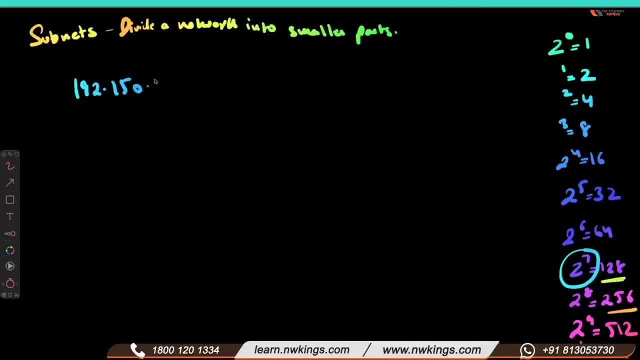 150. there is small difference in the ip, but this time i have ip 190 to 150, 10.0. this is by default, 24, so you can write down. network is 24. host is 8, so this is by default. now i want to divide my. 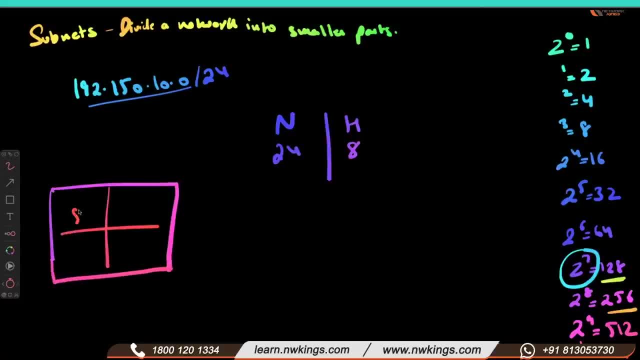 network like i want 50, 50 computers in each lab, almost 50. so you can calculate for 50 to the power of 6 is 64. so i want 6 host bits and this 2 will be added here the network becomes 26 and host. 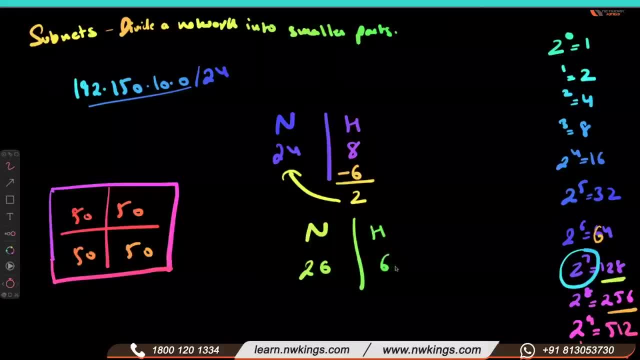 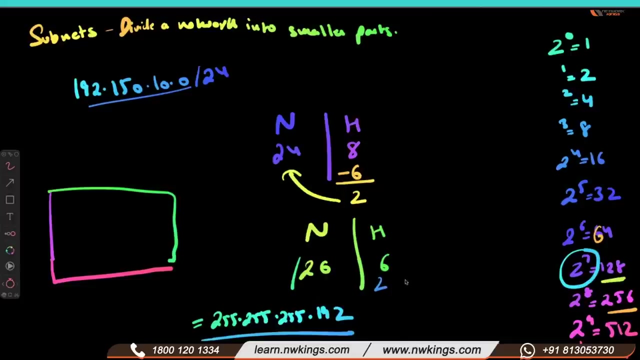 becomes 6. right, so very simple. it's the most easy subnetting ever. so. this is 26 and how you get subnet mask: 255, 255, 255, 192. this is my subnet mask. very simple and to the power of 6 is 64, so you can make blocks: 0 in the end, 255. 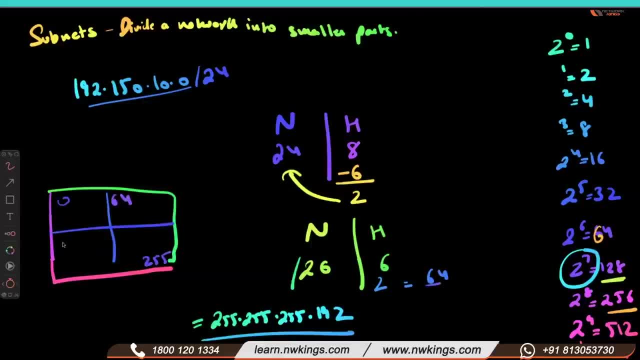 64, right in the another column, 64 plus 64, 128, 128, 64, 192, so before 192, 191, one before 128, 127, before 64: 63. so these are your four computer labs. yes, now you guys can ask me question. i have, don't worry, it's very simple, just you need to be. 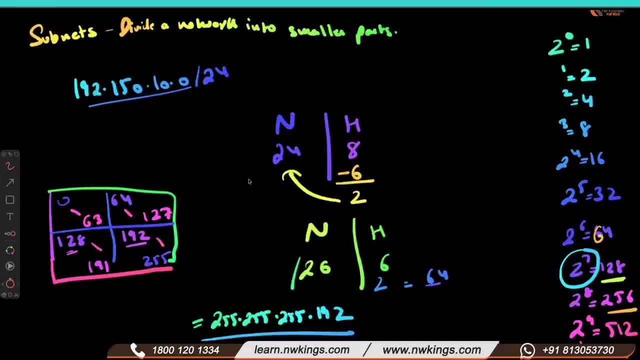 focused. yes, santosh, sir, i know it's uh flsm, but some of the guys don't know whether it is flsm or realism. so can you please explain realism? yeah, yeah, i'll explain other. any other question guys? okay, so i'll come to the technical word, santosh. okay, don't uh just see uh the technical aspects. it's. 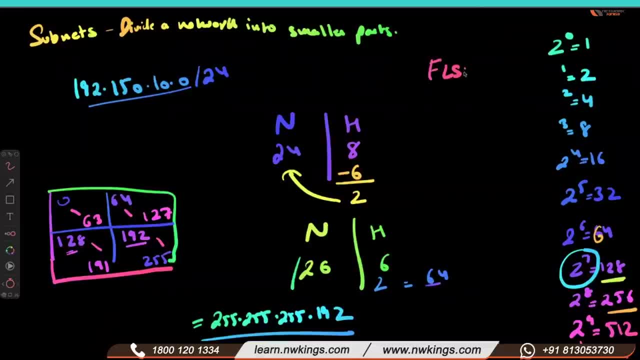 just a simple thing. uh, in technical language we call flsm fixed. don't worry about this. okay. so fixed length subnet mask fixed, so you can see all my computer labs have same identical computers, like all my computer labs have 50, 60, 100 same. so when we do this we call this flsm, but when we are 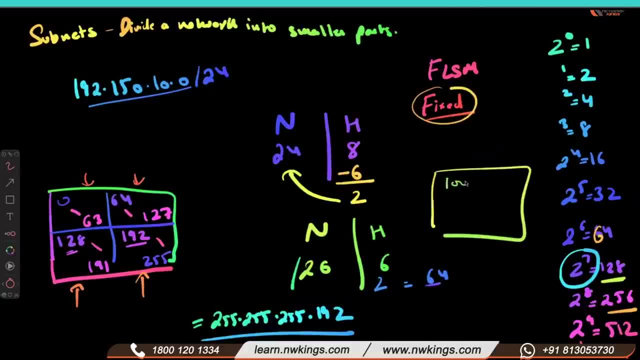 going to set up our computer lab like this: maybe we have 100 user in one lab, 15, another 20 in another, 10 in another. so this is called vlsm, that is, variable length subnet mask, variable length subnet mask, this lsm length subnet mask. so this is fixed. so i have given you two example, which is of 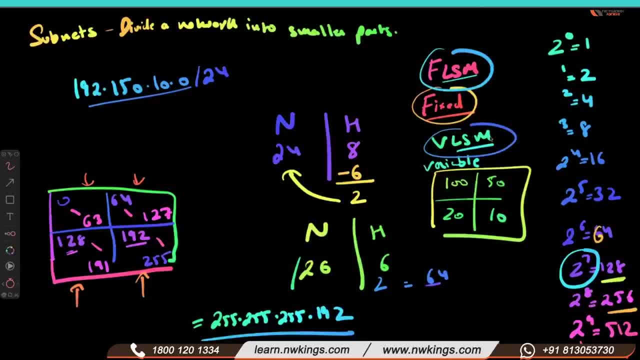 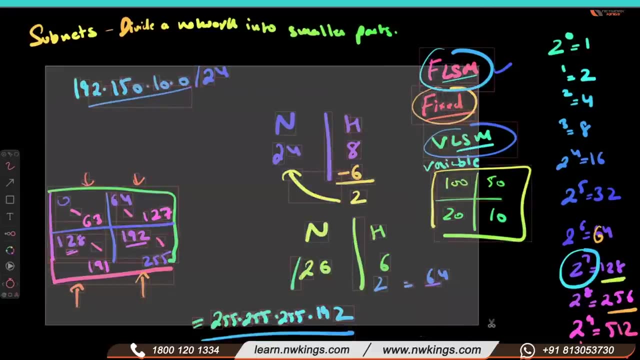 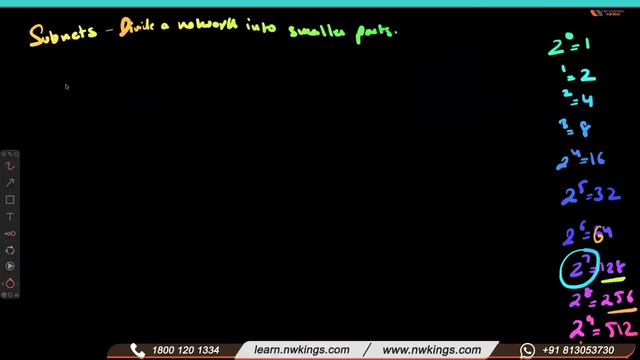 flsm. i'll explain vlsm. it's very simple. also, don't worry. okay, so, but you need to practice that flsm first. okay, master yourself into flsm, okay. so let's do another question. okay, this time i am going to use some another ip. let's do 200.1.1.1, but this network. 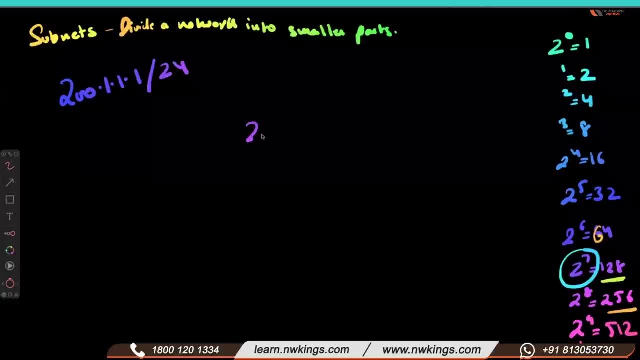 is like c class, obviously. so again you will say: network is 24, host is eight. but this time you want almost eight computer labs. okay, you want eight computer labs, something like that, eight computer labs and that also need, you need fix uh number. but this time i don't need, i don't have requirement of host. 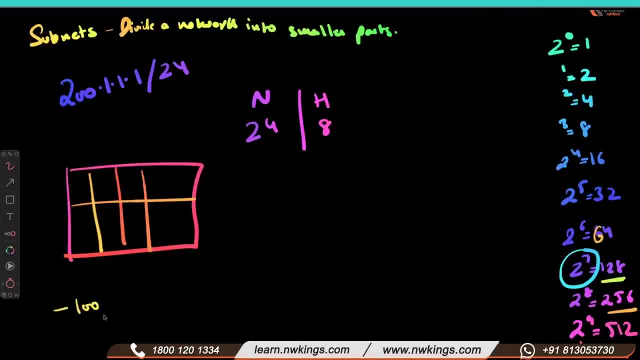 in last two question i have given you the number, that first question 100 computer, second question 50 computer. but i don't care about my computers, like how many computer per lab, but i need eight computer lab. so you can give any number, but i know my eight, i know eight computer labs. 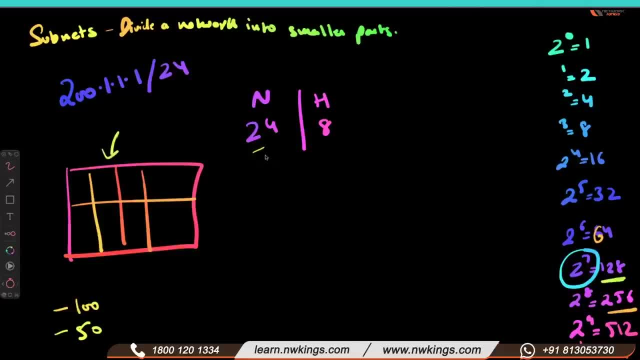 so it's just you need to check what i have to add here, okay? so if you just calculate according to subnet, not according to host, then you just play with this network part, and when you want a host, you play with this host bit. very simple. so if i want eight, 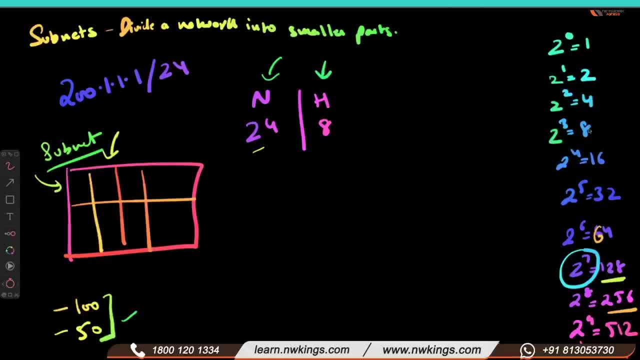 subnets. so tell me, for eight subnets, what is the power? what is the power? the third power? just you need to plus three. it means you nine minus three here, equal and a half super zero. let's see. and where is this? okay, cool, simple, started network is now 2007 and host becomes. 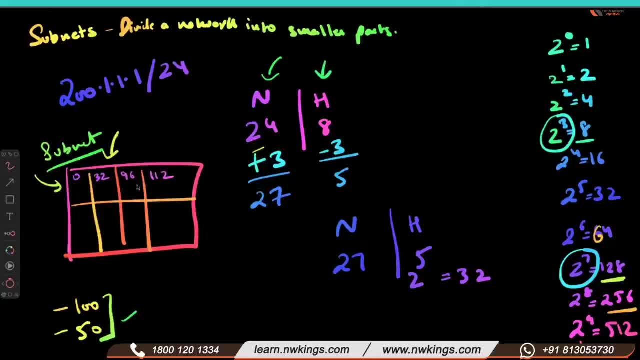 five and to the power of five is 32. so you start with zero, 32, 96, 112. just 32 is not 112, guys, it's 128, okay, and then after that i think you'll be getting 160, 192, 224. that's it, i think. 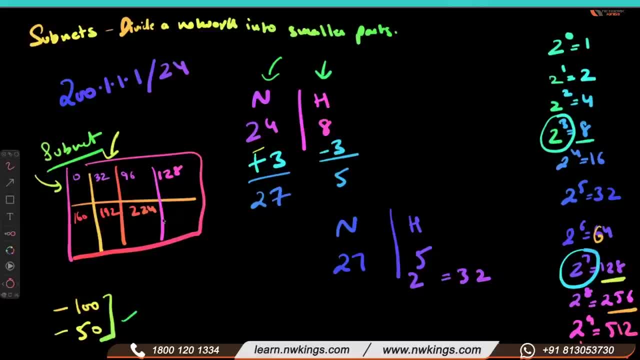 hello, yes, yes, sir, uh, zero 32. so it's very simple. just keep adding the 32 number, okay. so don't make it complex. just keep adding that 32 number. so it's very simple. just keep adding the 32 number. start with zero 32, 6496. keep adding this number and you don't have to figure out for all boxes. 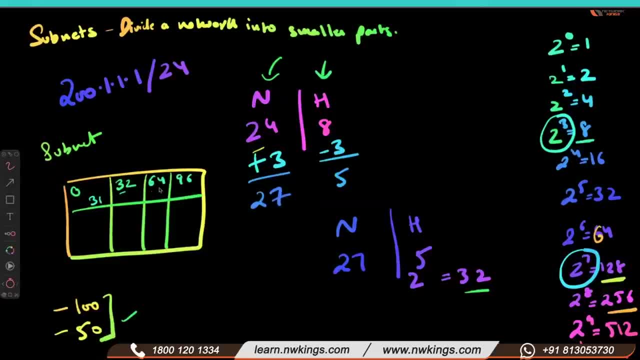 so 32 before 32, you get 31 before 64, 63. so this is the range. so when you are going to assign any ip on this computer lab, what will be the ip? 200.1.1.1.2 or something, any ip? 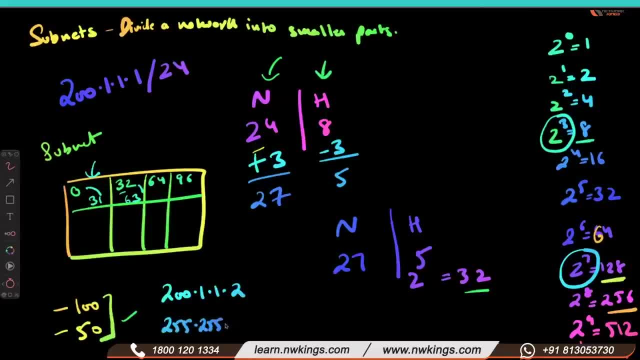 and the subnet mask will be 255, 255, 255. so two to four. two to four because 27 is 8, 8, 8, 3, 3,, 2, 2, 4 on three bits. 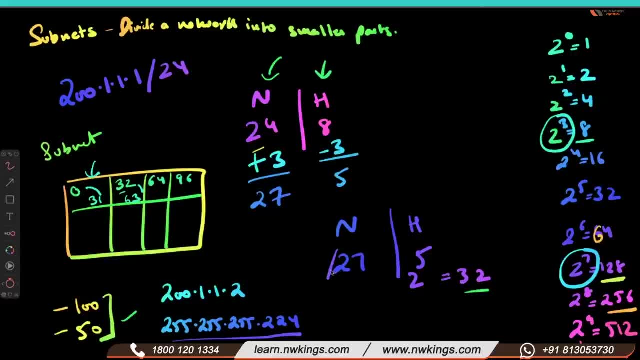 You have two to four, Hello, sir. Yes, Yes, It means there is no more than 32,. uh, you host in one network. There can be no more than one 32 user in one network. Yes, yes, yes. 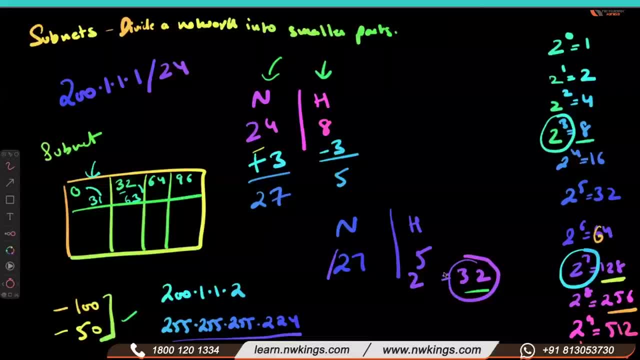 Related to this scenario. Yes, yes, correct, Easy enough. but yes, sir, it's the super. uh, I think I should change this seven eight workshop name to the super easy seven, 18 workshop. Right, Okay. 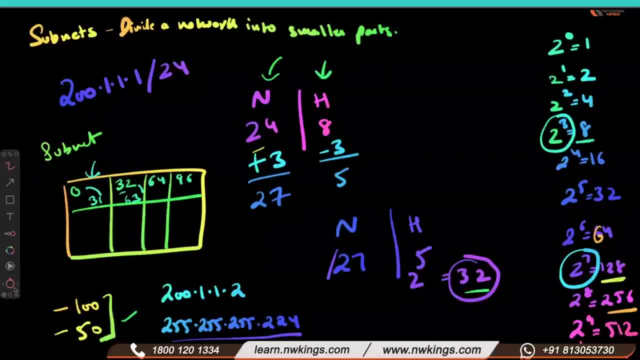 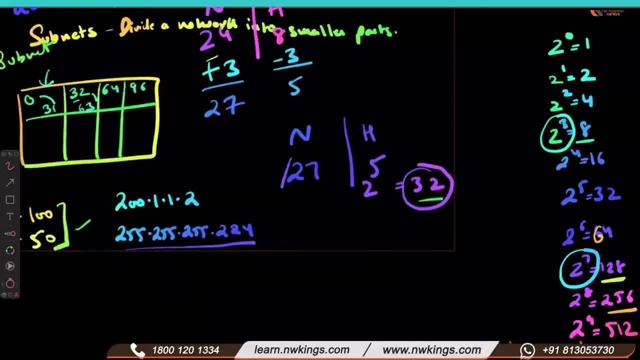 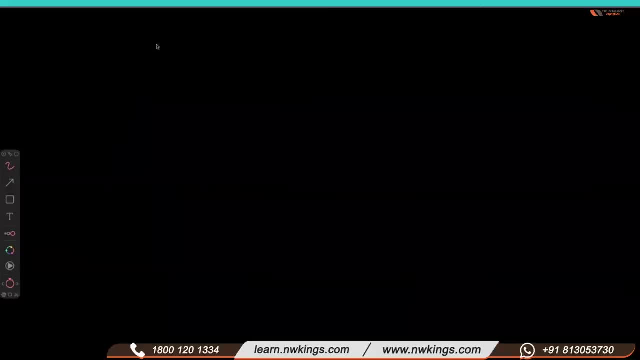 So now the trick part. So now you can solve any number. So now let's practice. Now you guys are going to Tell me hello, sir. Yes, Uh huh. uh, there's the DSCP. Decent, the DSCP is another thing and D is just a protocol. 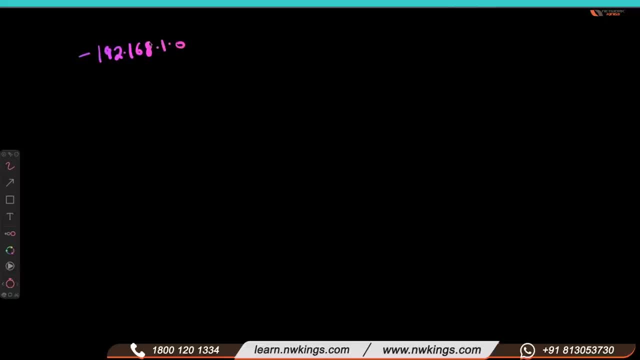 To assign the IP address is automatically, but you have to define the subnet. My, I'll come to that point. Okay, So that is not related. Okay, related to class, as of now. so you can just take example, guys, this is 192, 162, 1.0. but now you might. 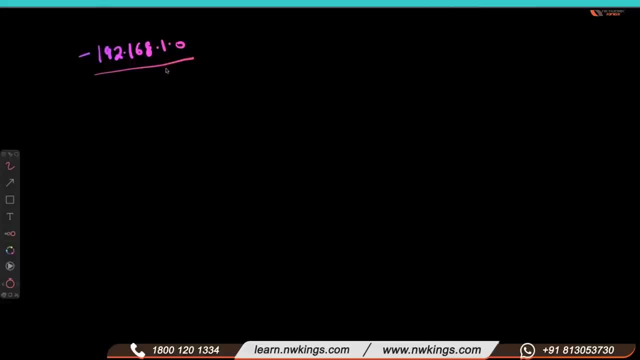 not, uh, like see this in any book also, because this is, I am going to explain you: subnet of subnet, or submitting of submitting. so already you have a network slash 25.. remember, when you divide your network into two parts, earlier we divided right. remember so when we divided our first question. 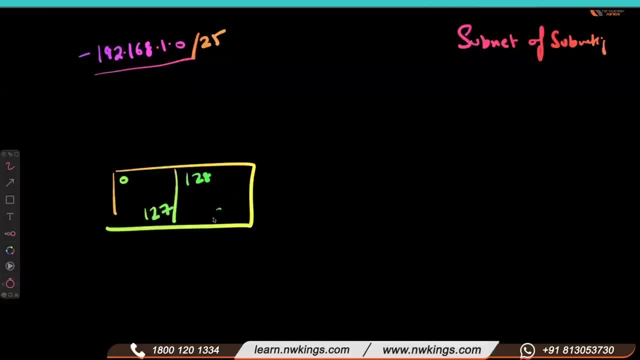 the 0 to 127, 128 to 255. that would. this was our answer, and we were using slash 25, yes or no? yes, sir. so now, now your requirement: you want to divide this network also in two parts. so now, very simple: network is 25 and host is. 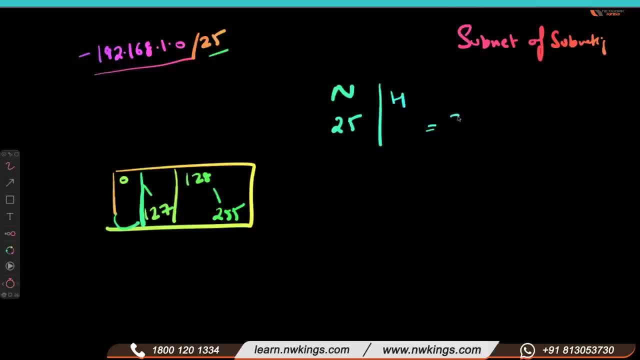 the, the, the remaining number. so IP address, is 32-bit. so you can calculate how much 32-25 host is seven. right? your IP is 32-bit, so your network is 25, the remaining bits is known as seven. so how to calculate? you can minus 32-bit IP from 25 bits. the remaining will be your host, right? yes, simple. 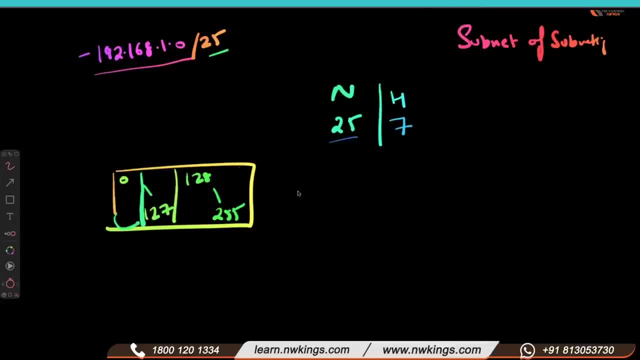 so now, this is your question. now you want to divide your network into two parts. so you know the powers guys to the power of zero is one. to the power of one is two. to the power of two is four. to the power of three is eight. to the power. 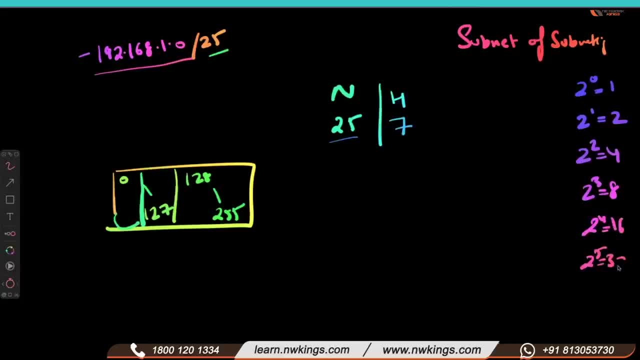 of four is sixteen to. the power of five is 32 to. the power of six is 64. you keep checking that so you can see how many networks we want now. one or two? obviously two. right, we want to divide this network into how many parts? yes, sir, okay, so if you want to divide this network also in two parts, then you can check for two how. 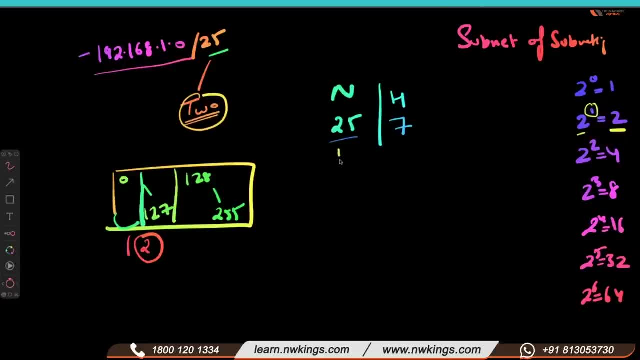 many bits. you want one, one bit, so you will add one bit here and minus one here, so you get 26 and the host becomes six. six right to the power of six is 60.. four, four, right, so you can write down this: zero. another block: 64, go up to 127 and before 64, 63, boom. 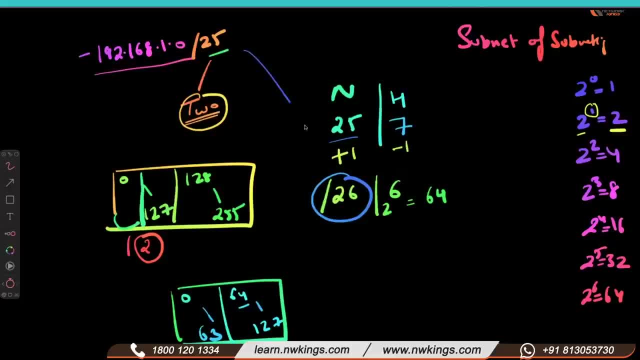 and your slash will be changed from 25 to 26 guys. super easy, just you need to understand what I'm telling you. there are many guys, even they are like ccna, ccnp- try to ask this question. okay, tell me, what is that like? if you divide this network into two parts, what will be the slash value? and you can just. 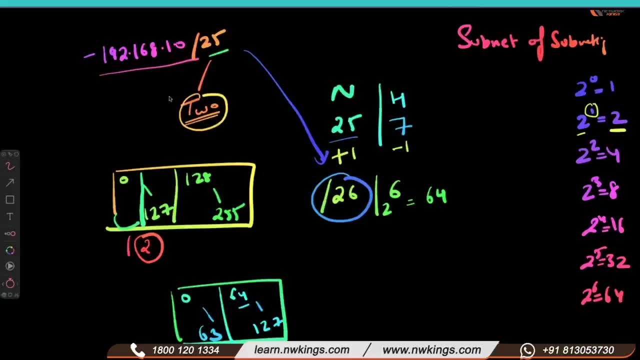 get this into fraction of seconds, right. yeah, sir, I have one question. uh, we, we can only divide the subnetting of subnetting in the power of the two means. in first, zero to 127, we have divided the network only two parts. if I want to this divide this networking three part, then then no, no, no, no, no, you can't, you have to. 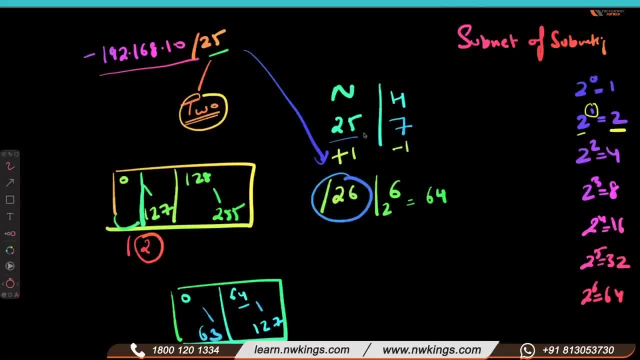 divide the network or everything within the power of two. if you want seven, you have to divide your network into eight. then only- or you can do one thing like for one subnet- you can take the bigger part. this is what we are going to learn in vlsm. okay, okay, but in flsm everything is equal, okay. 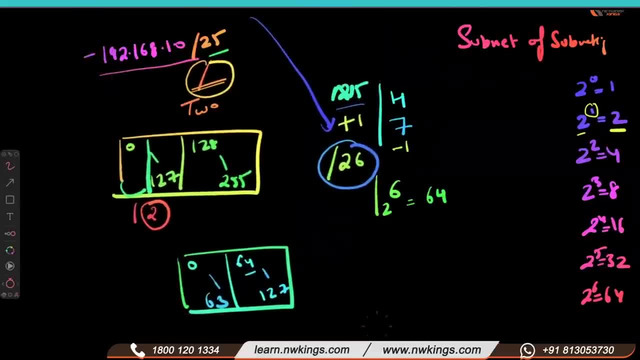 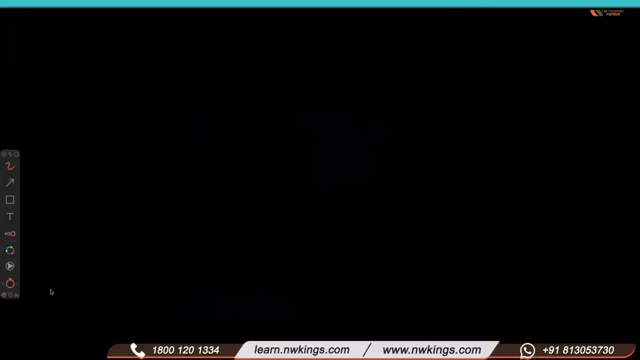 so, guys, all clear c class. yes, sir, yes, sir, yes, sir, I probably need to work on it. yeah, sure, so you need to work on what I need to work on: subnetting more to get this down pack. I've been looking at a lot of questions online. I'm studying for my network plus a ccna a study this more, so now you are understanding this. 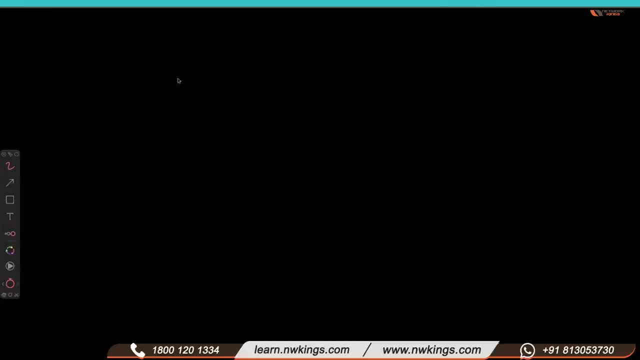 uh, not quite. I'm still a little confused, okay, okay, so keep doing the practice. this is the only way you can actually come out from this problem. even I was having the same issue. I literally like: uh, I never. I. I used to think: if I watch video, if I, uh, read books, I'll try to overcome. 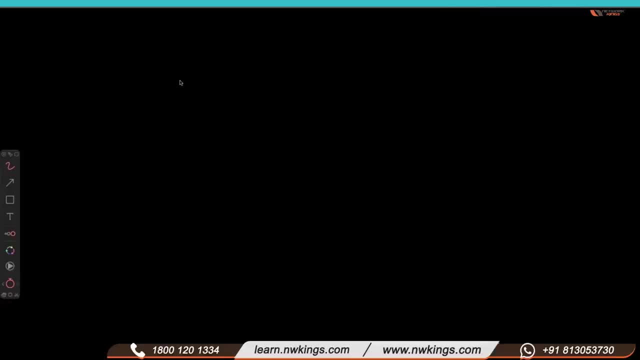 this problem and it took me around six months to actually understand submitting. trust me, even I have wasted a lot of time to just learn submitting because, uh, it is actually. might be my math was not good or something that, or maybe I didn't get any proper trainings from so what I did? 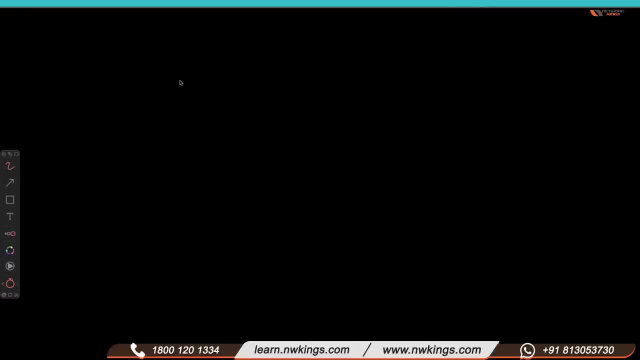 I just keep doing the questions daily, so this is the only thing you have to do, but the the examples and the tricks I'm telling you. it's very like I have practiced a lot, I have trained for like students from last 11 years, so I'm giving you the most easiest. 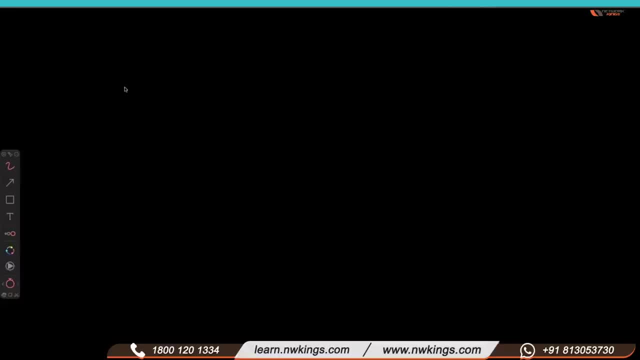 trick to solve the questions. okay, so now you can. so can you unmute yourself and try to do question with me? so I have a note. yes, yes, I'll try. I'll get back to you after this. okay, just hold on. so, Eglatrian, right, this is how I pronounce your name. uh, my real name is Nelson, but I'll see. 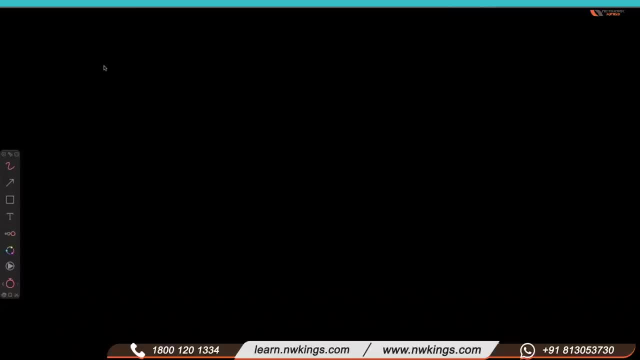 yeah, okay, okay now, so nothing. so what we have to do? so just take out the information, okay, so this is ip address, right? you already know this is ip right, so I feel address we are assigning so that every computer gets a unique ID, right. so now 192, 161.0. so 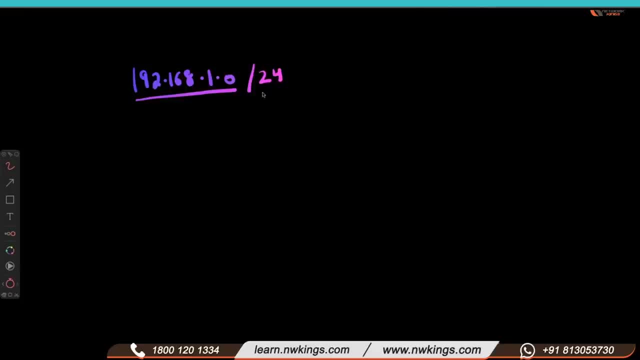 tell me what is this? 24- can you tell me what is this? that's the subnet mask. this is slash value. if you calculate this, this is subnet mask. oh, okay, the um. yeah, this, this is same. this is what we call slash value. but if you calculate this into, 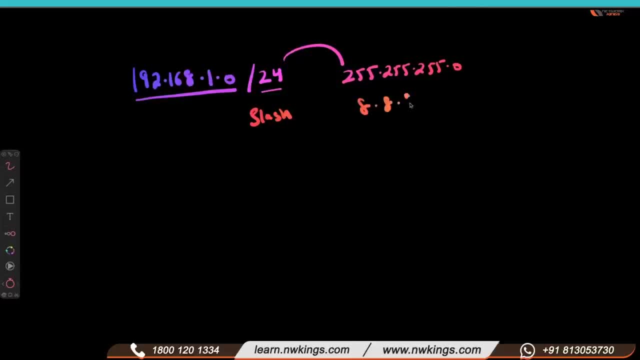 the decimal format by taking like 8 bits, 8 bits, 8 bits. so this is what we give subnet mask, which we assign to computers. okay, this is same thing. subnet mask, slash value- both represents your network part. okay, we can call this ip slash 24 or we can call this 3 times 255. also, that's the. 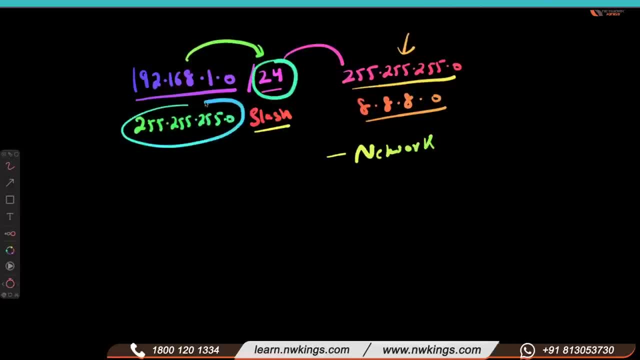 same thing. both are telling you the same thing: that this, this ip, has three networks. both the things are telling you exactly this: 24 means eight, eight. eight means this is your network, and two, five, five is also telling you the same thing: that you have network part three. 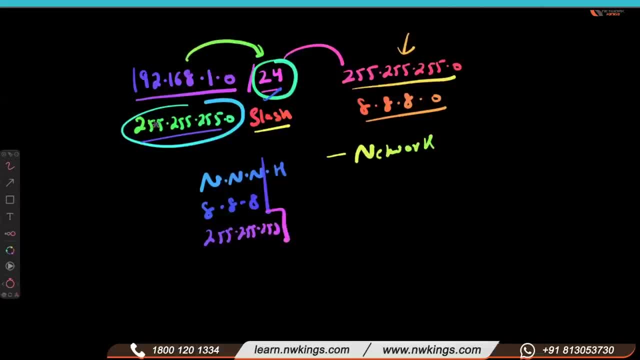 clear now. okay, yes, okay. now another question to you. so now you want to divide this network. okay, so you want to divide this network? why we are dividing? tell me because, because we have a lot of ip addresses, we want to get out there from where to where we have. 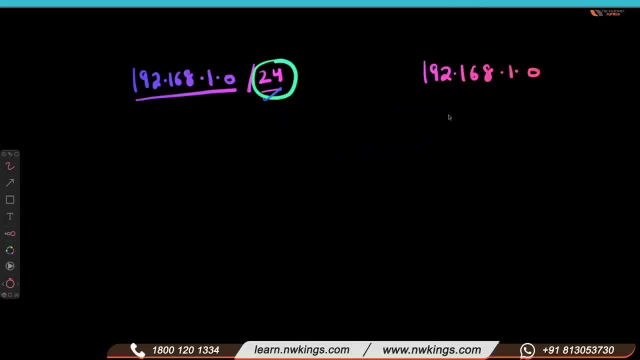 190 to 160, suppose this is the starting and, uh, obviously, this ip, the, this is network part. we can't change this. yes, correct, right, and it will go till what go to the maximum number will be. i mean 255. yes, correct, very good, okay, so 1.02, 1.255, clear. 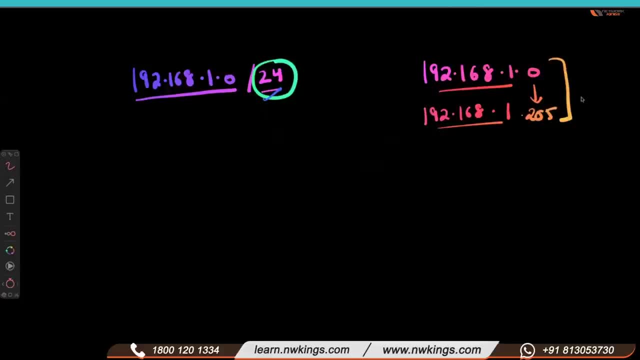 so now what we have to check that this ip is giving me almost 256 address, right, but i want maybe 100 on my ground floor and 100 on my first floor devices. okay, make sense, yes, okay, so now my network bits is by default. you can see if you see this or if you see this. also, if you check if you get any. 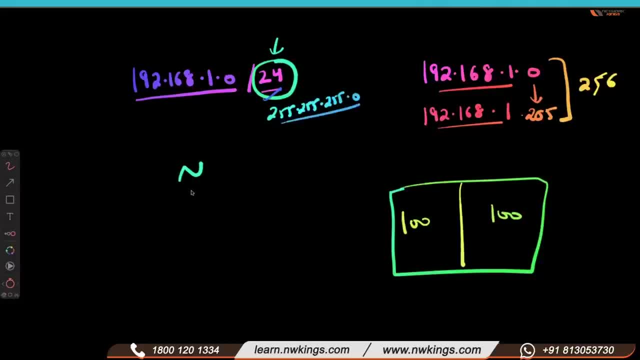 any of this. so your network bits will be. you can see both the values are representing network bits- is 24. yes, host is host by default host bits in class c, um eight. so if yes, so if you actually get problem to resolve this, it's a very simple formula: ip. 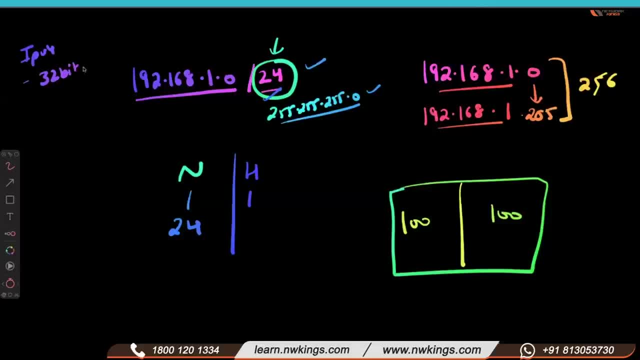 version 4 is of 32 bit, right, that's right. so 30 if you subtract, or minus 32 minus 20. it's a very simple formula. ip version 4 is of 32 bit, right, that's right. so 30 if you subtract, or. 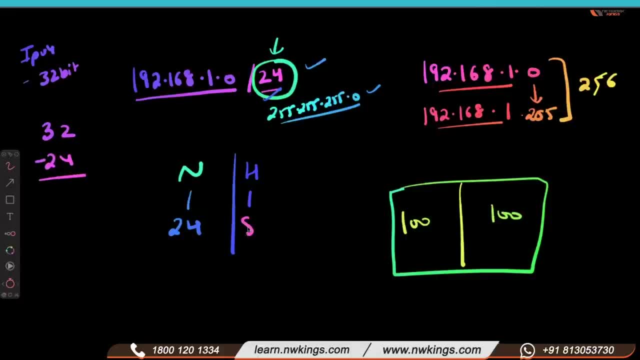 24, you get your host id. yes, clear now. okay, so now, if you check the table, to the power of 5 is 32, to the power of 6 is 64. to the power of 7 is 128, right to the power 8 is already. 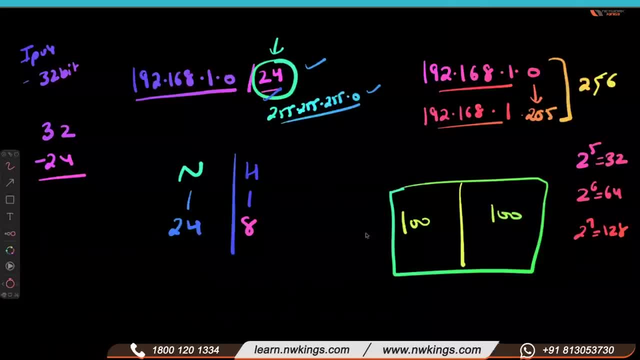 you know. so you can, yeah, yeah, yeah. so now tell me how many ip addresses we need in computer lab. 100, right? 100, yeah. so if i use 256, how much i'm wasting? 256 minus 100, i'm almost wasting my 156 ips, correct? that's correct. so we can't use 64 because it is less. so if you take 128 minus 100. 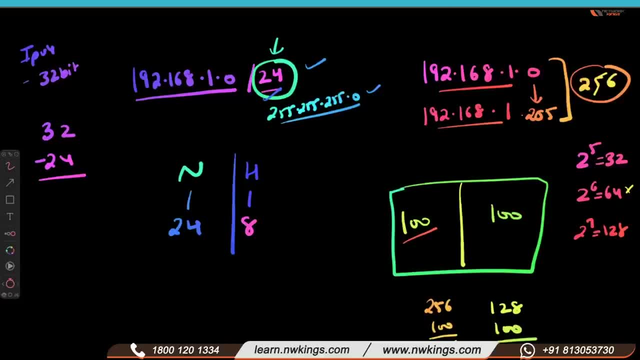 we are only wasting 28 approx, so it means this is the best for us, correct? that is correct. yeah, so this host is 8, but how many i want now, according to 100 computers, how many i need, how many host bits i need? you need seven, yes, so i'm going to say i need only seven. 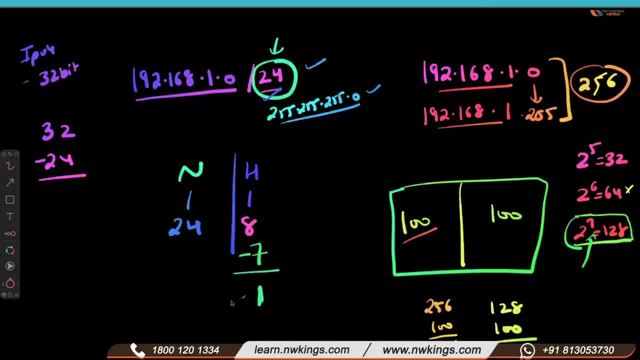 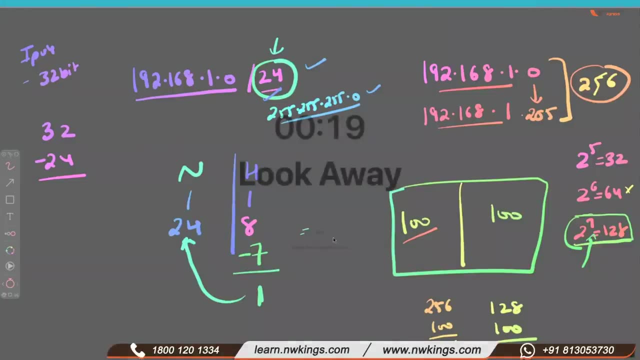 i don't need eight. so this will be converting into the nato part. i'm going. i don't need eight, i need only seven. so obviously your calculation 24 plus 8 is 32. so you have to make sure obviously ip version 4 is 32 bit you. 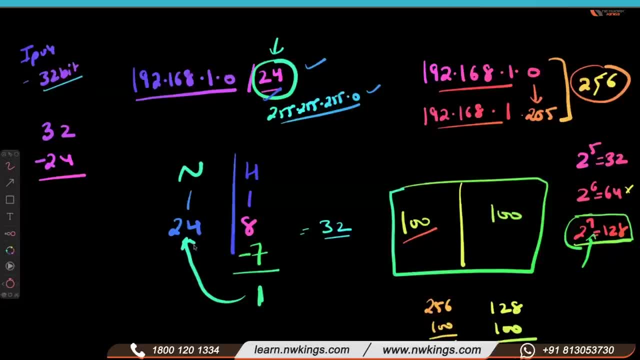 can't reduce this. it's normal. but you can just play that if you need less host bit. obviously that is going to add it into the network part, correct? yes, correct. so now the answer would be 25 network bits and host will be 7.. and how to assign this to the network for the network part. 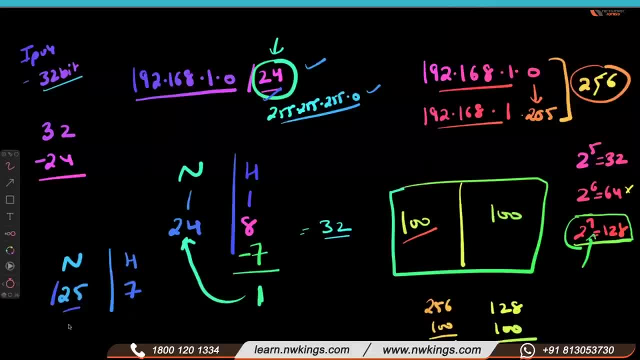 25 to computers. i have given you instructions yesterday. if you calculate the subnet mask of 25, that would be 255, 255, 255 and 128, correct, yes, correct. so this ip you have to assign in this computer lab. but how to get? what is the range? this is what we call range. how, like ip, start from where? 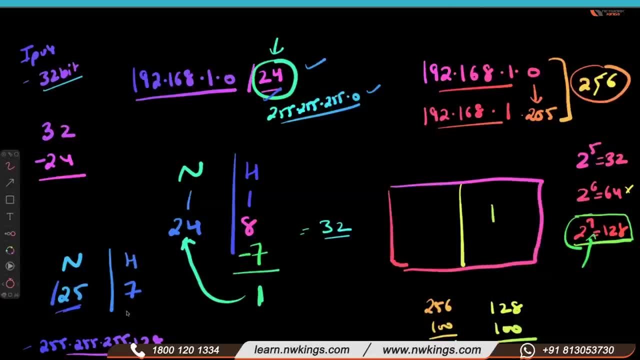 to where. so you can check to the power of seven you get is 128. right, that's right. you can just write 0 here. it ends 255 and whatever you get, please write in the second block 128 and before 128. what is the number which comes before 128 is 127.. 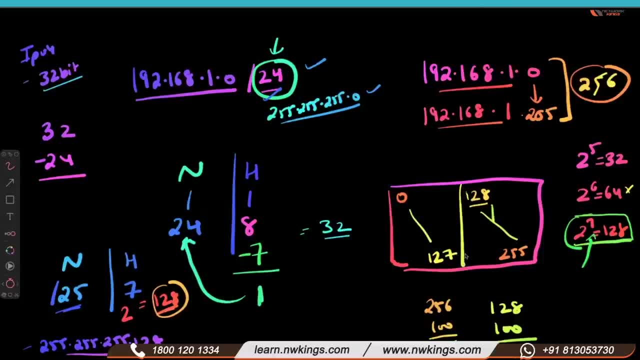 this will be your computer lab a. this will be your computer lab b. okay, so when you are going to assign ip addresses, whenever you assign all in computer lab a, you are going to assign ips from 1 to 126, because you can't use the first and last ip that is like called network id broadcast ip. 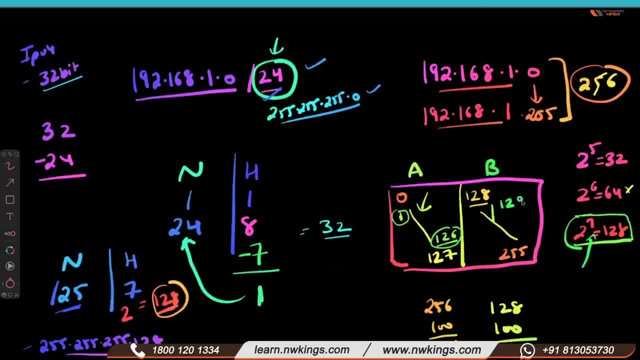 and in computer lab b you are going to assign ips from 129 to 254.. so this is submitting. you just divide your network into two parts. that's it clear. now getting some confidence, i'm getting a little bit of confidence. it's slowly but surely. 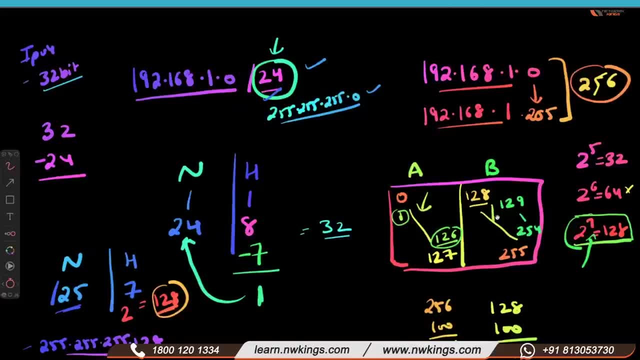 uh coming together. i've got to keep going over and over, over and over again. yes, yes, definitely. this is. i told you then on the first uh, when we interacted, that you have to practice the only way to overcome this. okay, okay, okay. so, guys, let's uh. 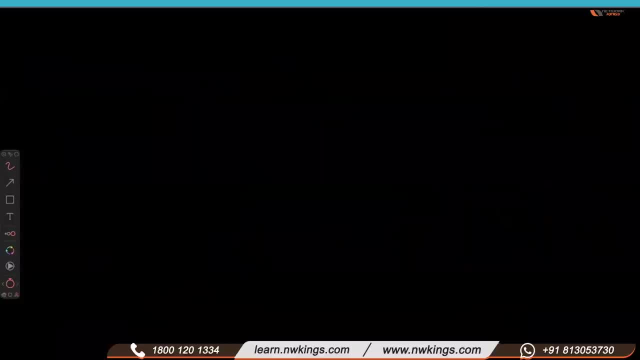 take five minutes break and come back in five minutes, okay, uh, shantanu, i'll take your question in five minutes. yes, shantanu, you were asking something. uh, shantanu, ah, yes, sir, sir, yeah, yeah, tell me, has subnet there now? yes, yes, everything will be in question, don't worry okay. 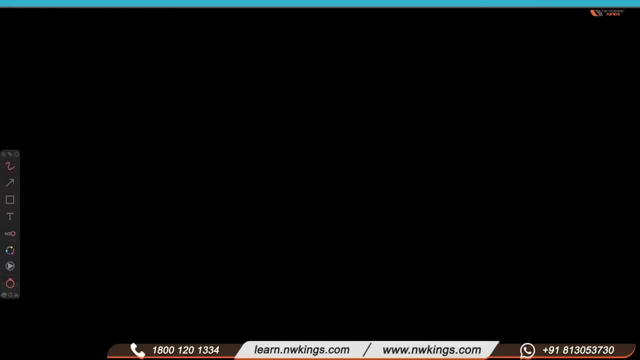 nike. yeah, let's explain i'll. i'll take the questions, don't worry. okay, just hold on. so we are going to use- uh, let me complete bna class and then we are going to learn directly questions which actually comes in exam and which will be completed in a particular way, or that i'll learn directly in the exam. 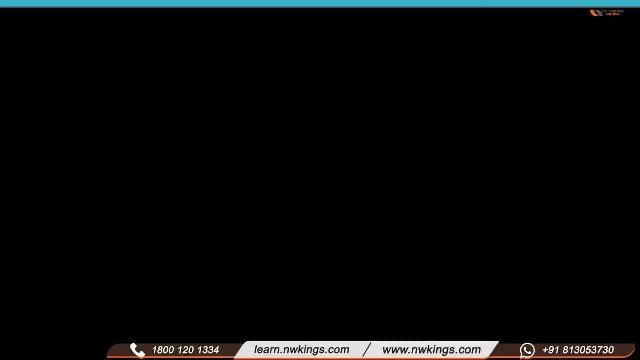 so then we are going to learn directly questions which actually comes in the exam and which will come in the exam and which actually uh help you to understand the real networks as well. okay, so don't worry. so guys, uh see in b and a class, so in when we learn the questions in b and a, 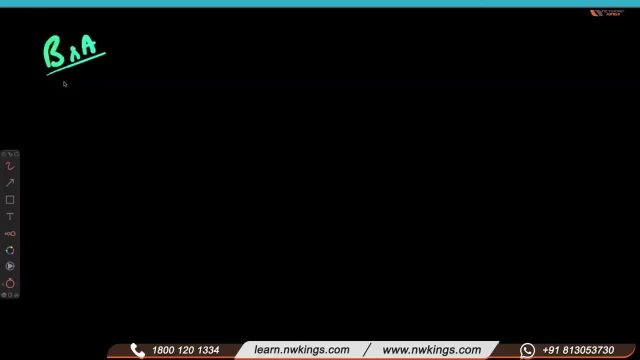 okay, just we need one extra step, which i am going to explain you, okay. so let's take example, uh, that you have ip 150.10, so this is b, so we can take two zeros, so this is network, this is host. so we can say that in b we have network 16. 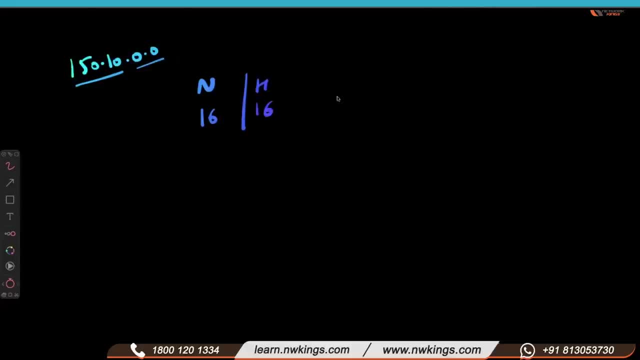 then host to 16, correct, right? suppose you want your network to divide. uh, means you want to give 500 computers in one computer lab. okay, you can't use c class in this case, because this for one lab. you need 500 user and only b and a can help you in this. 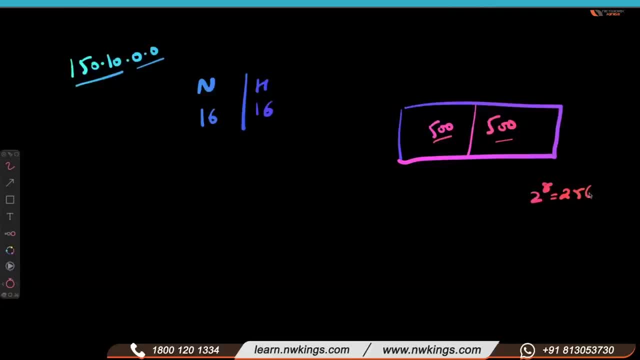 so you can check. also, to the power of 8 oz: 256. so to the power of nine is 512. to the power of 10 is 1, 0, 2, 4. to the power of 11 is 2048. so you can check, so you can tell me for 500 computers by default. 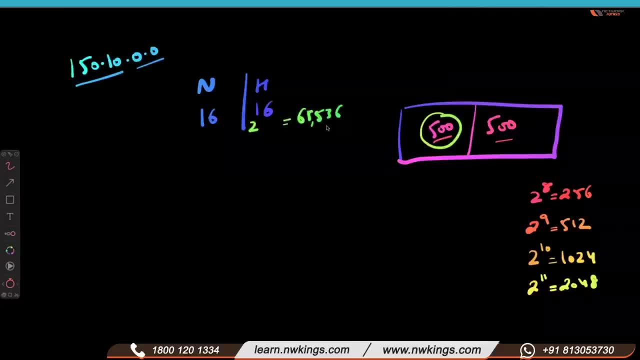 to the power of 16, we are getting 65,5, ear 536.. it's a very big number. if we give 500 computers and if we don't subnet so you can check how many, we are wasting. almost 60 000 ip addresses we are wasting right. so we need how many? 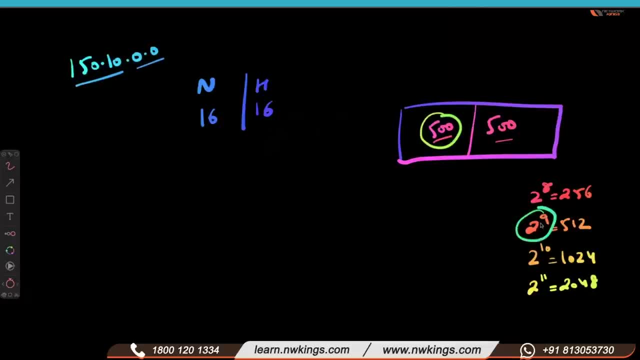 how many people? yes, because for 500 user my 9 bits is enough, right? so if you minus this, you get 7 and that 7 will be added here. so network becomes what? 23, and the host part becomes obviously 9, right, yes or no? very simple. 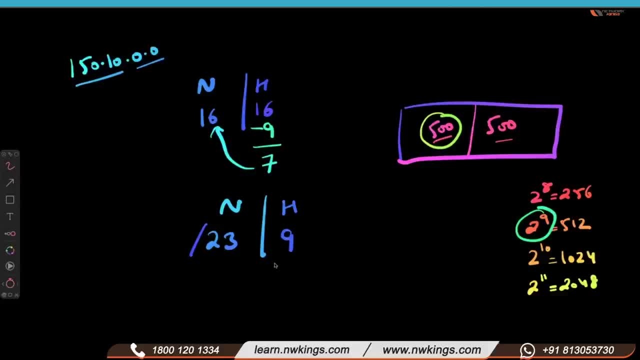 yes, sir, clear till here. yes, sir, okay, so now tell me the subnet mask. this is why i have really actually asked you, everyone, to learn the subnet mask. so what is subnet mask of? true in 23, 255, 255, 255 and, uh, eight, eight, eight, seven. this is how you make 23 for seven bits, you have 250. 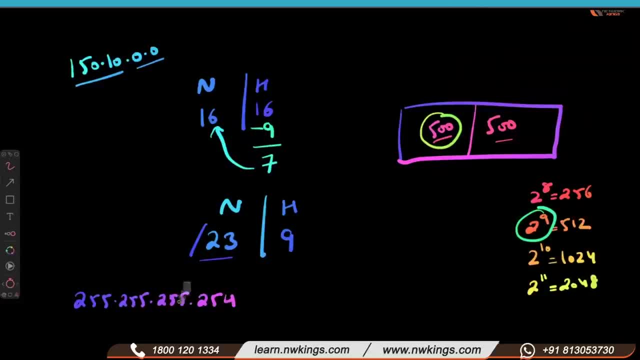 four, sorry. on the third octet you are take two, five, four, sorry, sorry. two fifty four dot zero, yes or no, clear, yeah? so now if i tell you that you have to write the range, it is going to be very complex for you, why. let me show you, if you divide network like you have to write the range, how you will write. 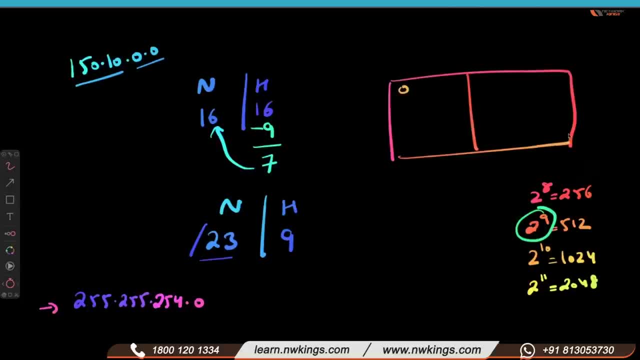 obviously you know zero, but you can't write two, five, five here because it's a very big class. okay, so we are just taking two boxes, so zero. but ip address doesn't start with 512, right? if you check to the bar of nine, five, one, two, right, ip is maximum till 255, so it means you have to. 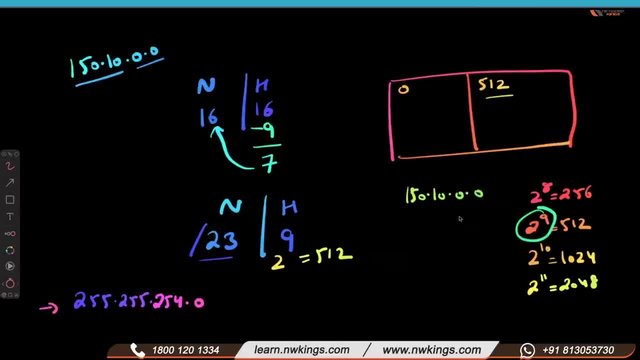 start with 150, 10.0.0, you will finish 255 and once it finish it becomes 1.0. like after 11, 59, what it becomes 12? right, right after 59 it becomes 12. the same way, after 10.255 you be, it becomes 1.0. 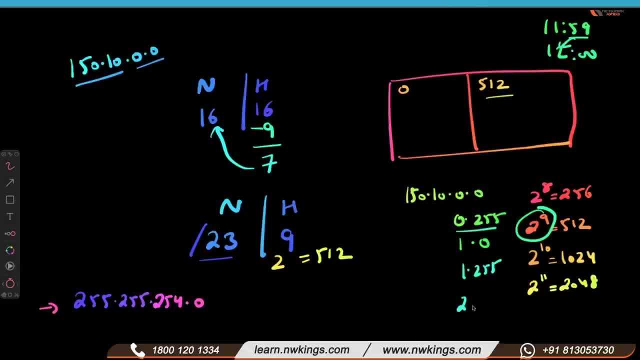 and 1.255, like this. after this it becomes 2.0, like this. so you have to calculate 0 to 255, 256, 1.0 to 1.255, 256, so 256 plus 256, 512. so do you think it's a very simple method. 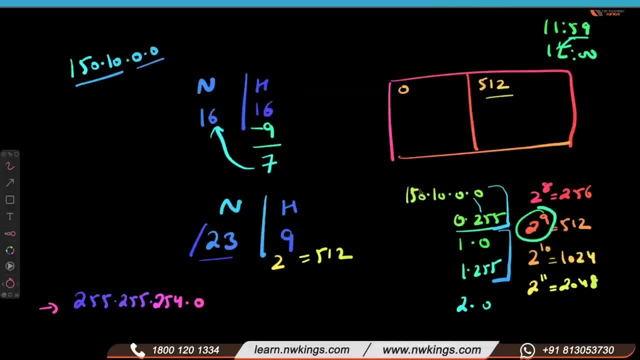 no right. if you have to calculate like this, 512 is very simple, but if, like in further questions, we will be getting 8000, something also, but suppose this is a number. you have 8192, can you calculate this one by one key, adding 256? it will take a lot of time, yes or no? 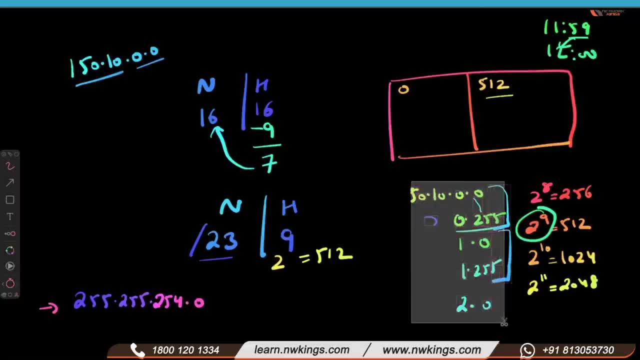 if you have a big number, then you have to do a lot of calculation. yes, so what is my shortcut for you that we are going to? you can see that we have network part and this is my host part, right, right, yes, so this is class b, so we will write the same. 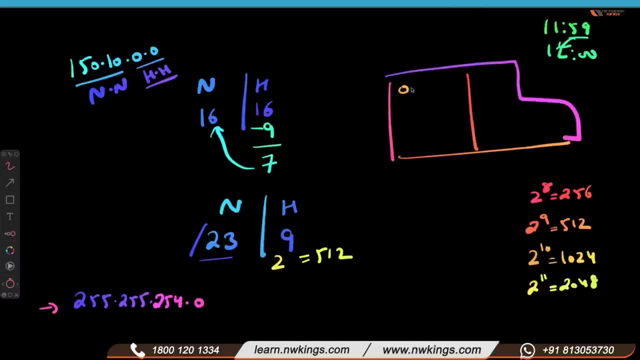 we are going to say it start from zero. not zero because we have class b, so it starts from 00. right, and how to calculate? so you can see: this is 2 times 255. but there is a shortcut to get the gap. this is the only extra step in class b and a gap. this you will not get in. 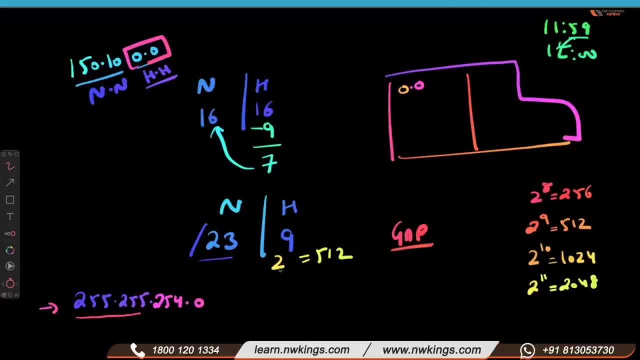 any book. this is my trick, so this is what i say: gap. so you subtract 256 in uh from the from two, five, six and you get two dot zero. This is what we call gap, And you write zero dot zero, two dot zero, right. 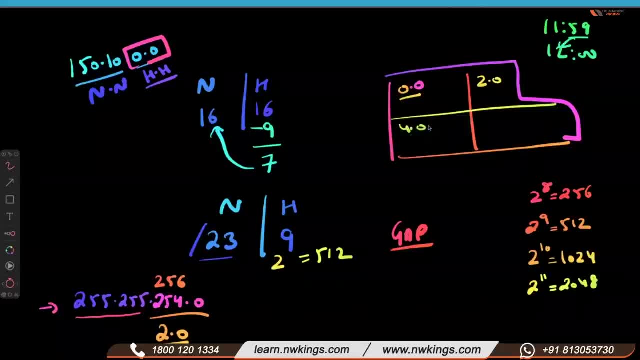 And in third block you can write two plus two, four dot zero. Ishmith Rohan Shambhu Nath. please turn off your mics. Okay, okay, sir. Four dot zero, four dot zero plus two dot zero, six dot zero. 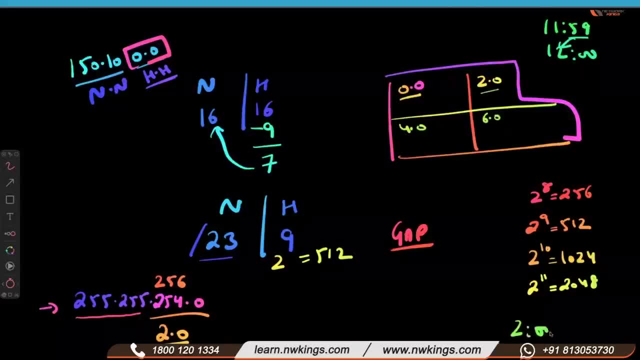 And tell me what comes after. Okay, tell me, according to time, What is the? when it becomes 2 am or 2 pm? what comes before? two 159.. Okay, but in IP two dot zero. 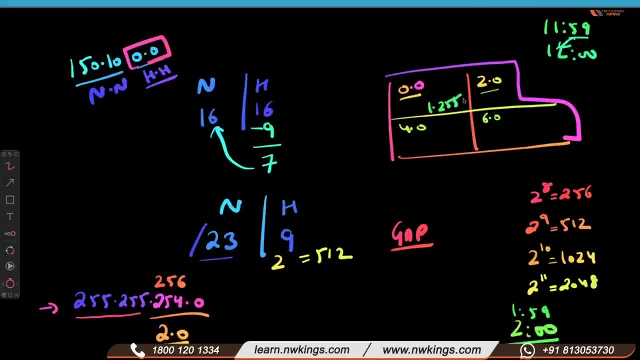 what comes before two dot zero, one dot Two, five, five Before four dot zero. what you get: Three dot two, five, five, right, Yes or no? Yes, Okay, don't worry, I'll do three, four more questions. 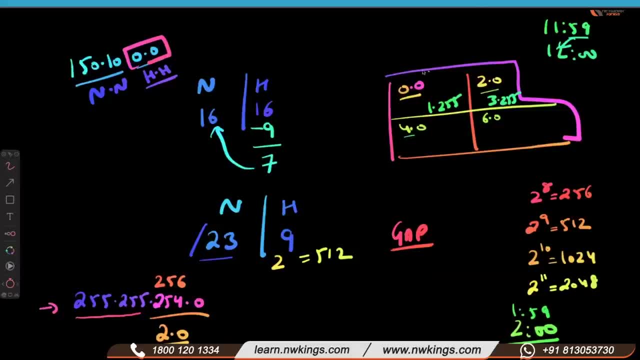 Don't worry, But you can understand. for 500 computers this is the block. So suppose you are giving IP zero dot zero, zero dot two, five, five. you have assigned IPs to 250 computers. after that you are going to assign IPs one dot zero. 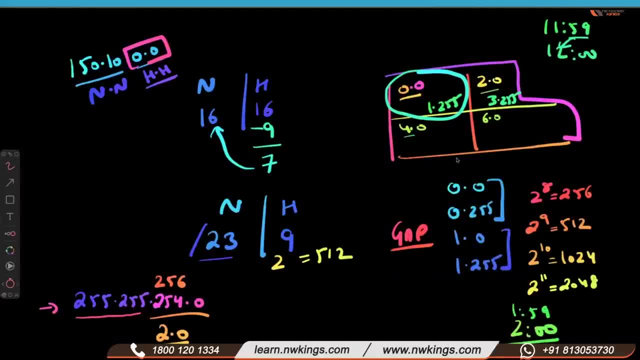 one dot one, one dot two. it will end up to two, five, five. This is the same. we got here, yes or no, But it was a complex method. but if you know it's not a complex method, but if you know. 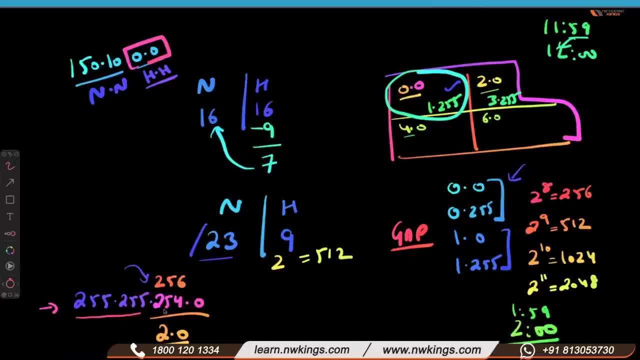 it's not a complex method, but if you know, you know two minus the value which is not getting completed. like you can see, two five five, two five five is completed, but this third octet is not completed. I'll subtract two dot zero is my gap. 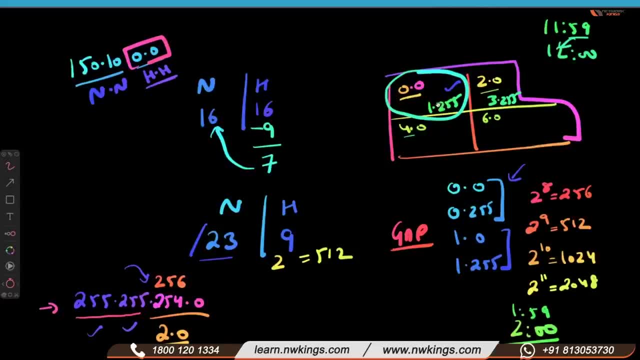 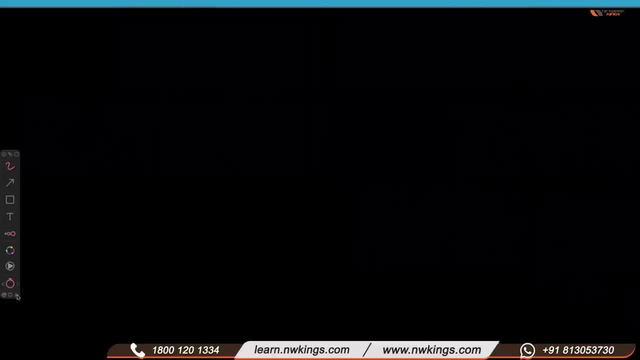 I'll start with zero, zero, and it will go up to two dot zero. Okay, let's not waste time. do another question, Because I know you guys are. if you check this too much, you will get confused, So let's do another one. one fifty: dot ten, dot zero, dot zero. 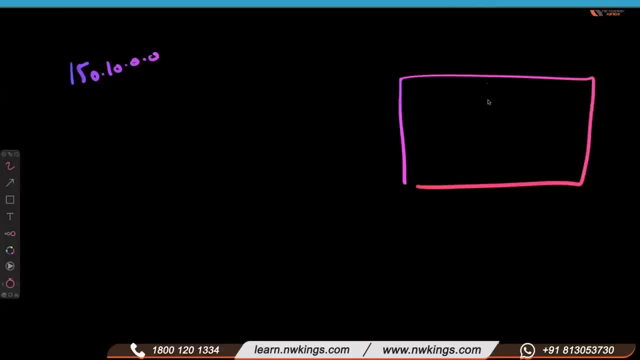 But this time I'll just add one more one. i want to give thousand computers in one in my delhi branch, and this branch maybe i have in london. i have two branch offices with one thousand users in delhi and one thousand users in london. 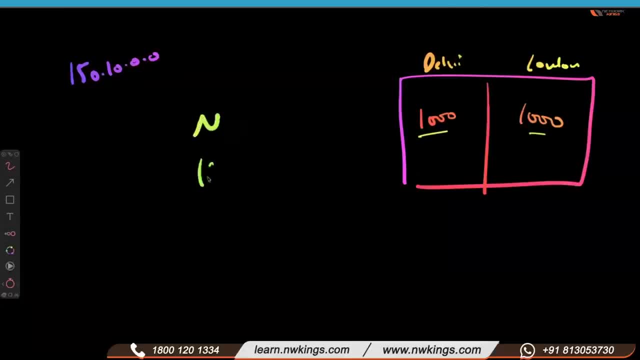 okay, so i want to divide. so network is 16, host is 16, right for to the power of nine is 512, to the power of 10. war is one zero, two, four. so is tell me which value would be good for you. one zero right. 10 is close right. yeah, so you will take minus 10 and that six bits will be adding here. 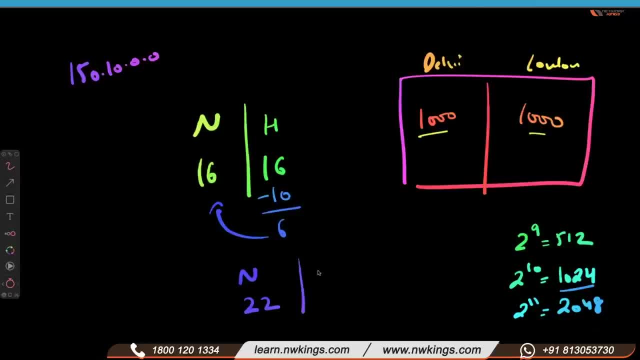 it becomes network 22 and the host part becomes 10. right, and what will be the subnet mask of 22? two five five, two, five five two fifty two dots. okay, if you are not understanding this, guys, please learn that formula. okay, i think most of you are getting confused there. i am. 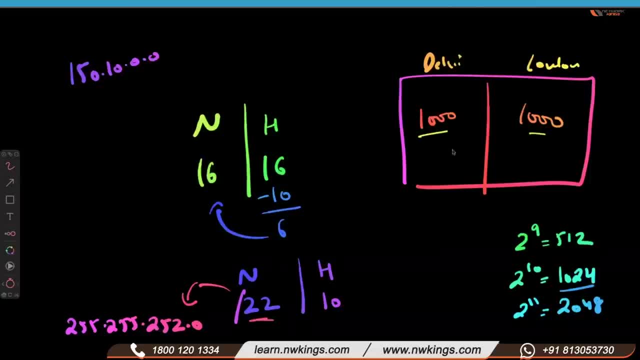 how i calculate this. but don't worry, you are going to calculate this with practice, guys. uh, okay, so tell me what i have to calculate: the gap 256 minus 252. what is the gap? four dot zero, yes. four dot zero, yes or no? yes, sir, you start with 0.0. next block is 4.0. 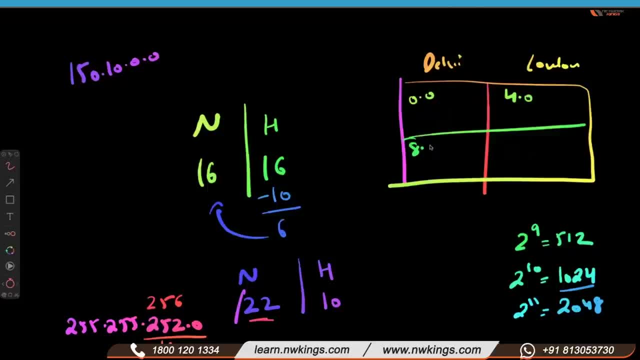 another next: 4.0 plus 4.0 is 8.0, 8.0 plus 4.12, 0.0. so before 4.0, what you get actually 3.255, 8.0, 7.255, 1, 12.0 is 11.255, guys, don't you think? 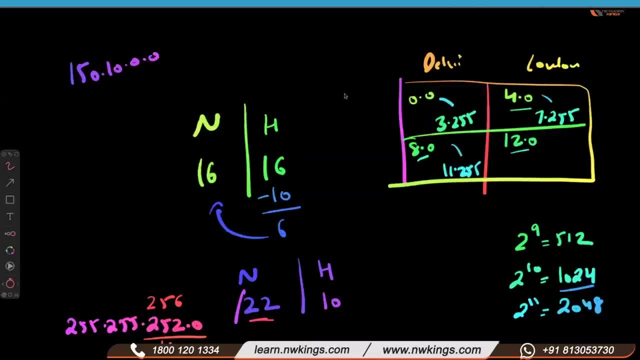 it's like very easy, you are actually calculating thousand computers within fraction of not even like it is not taking even at one minute. sorry, sir, sir, i'm repeating. this is second question. only don't worry, i'll come do two, three more questions. 150: 10.0 is my ip, with my slash value 16. this is my by default for class b. 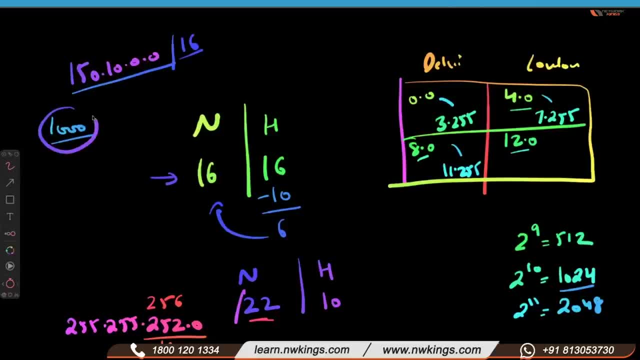 16- 16.. i want to give 1000 computers. so for 1000 computers i have calculated i need 10 host bits. so i have subtracted my subnet uh host bits from required. so this is my required. this is given. so required minus and i get six. so this will be added into the network. part 22 and 10: 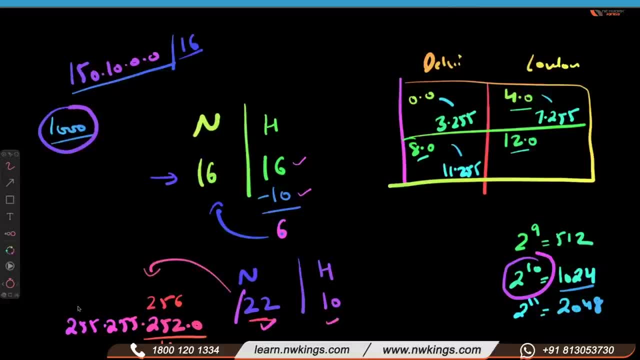 right, and if you calculate the subnet mask, so this will be my subnet mask. but to get the gap- this is my trick. okay, so i do what i do- 256- you minus it from the block which is not complete. this block is completed. this is completed. this is not completed. so i subtract 256. 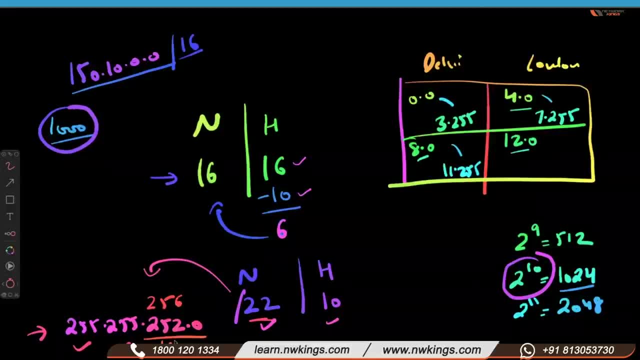 out of 250, 252 from 256 and i get 4.0 right. so my network part is this right: 150.10 will be outside always, because this is my network part. 0.0 is inside because that is my host part, right? so 0.0. 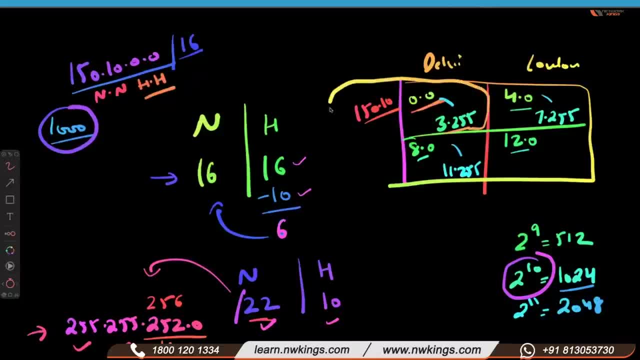 it will go up to 3.255. this is my delhi ip addresses and this 4.0 to 7.255- this is my london site ip addresses. this is my delhi ip addresses and this 4.0 to 7.255- this is my london site ip addresses. 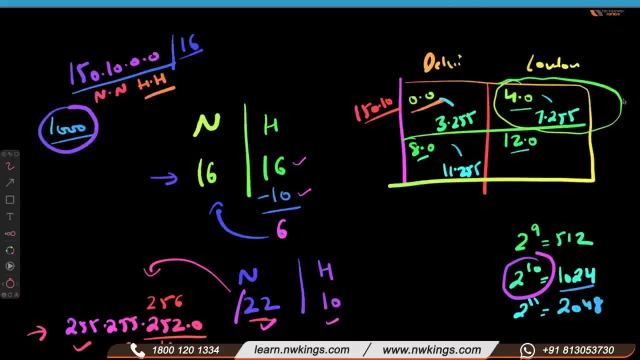 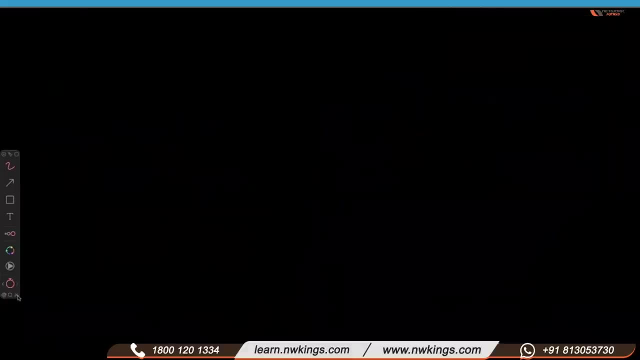 yes, clear. yes, sir, yeah, okay, so let's not waste time. for the same ip, for the same ip, let me have okay. so let's take a class also 10.0.0.0. so you remember, this is network and this is host. network is eight, host is 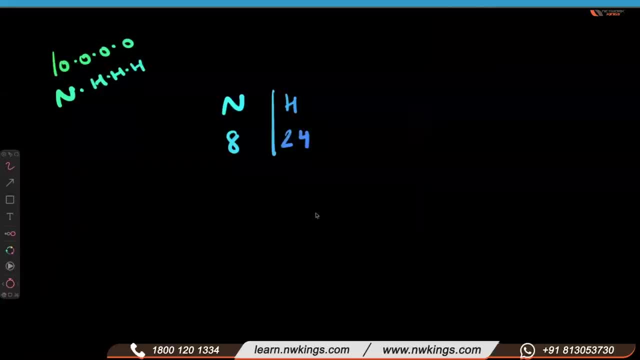 20.4, right. so now your requirement is like: uh, you have to build a location like for, uh, maybe for south africa. you need two thousand computers, two thousand computers at that location. okay, you can take four thousand, five thousand, ten thousand, what is? whatever is the requirement, right? 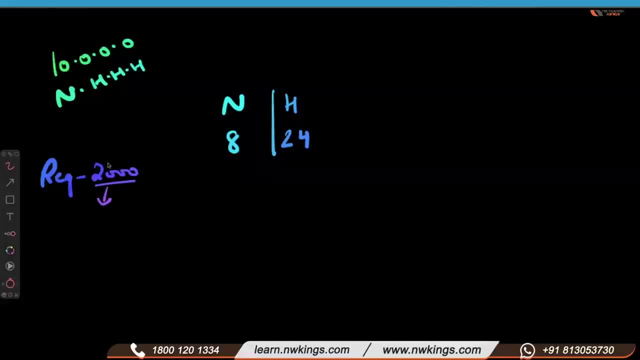 you can also further divide. also, don't worry, if you give two thousand to any country, my might be in that country. you have four locations. okay, suppose you are in india, so you have uh uh, 2000 computers is allocated for india users. you work for any mnc multinational company and you have four india sites. also, you can further. 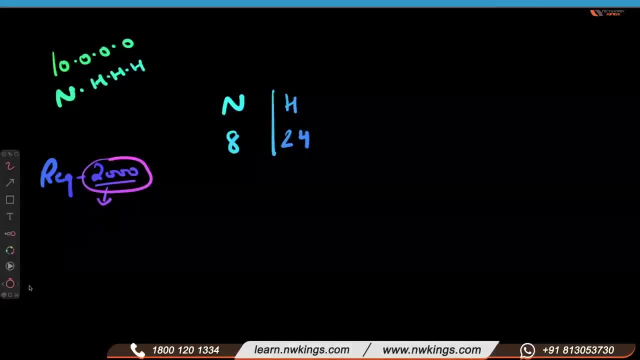 divide this also. okay. so, sir, for that we have to do some netting of submitting, yeah, good, okay, so we, for example- let's take example- i want to divide my network into 2000, so let's take a real example. okay, you guys want me to take a real example? yes, sir, yes, okay. so most of you know, 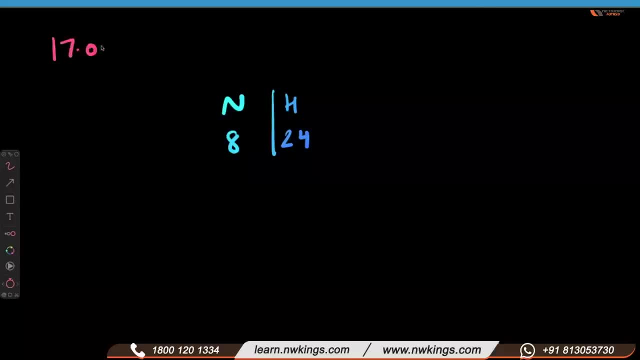 that i worked for apple and we use a subnet in apple that is 17.0.0. we have a public pool in apple. so, even like, all users get 17 ip. this is for all over the world in for apple. we have around 250 sites all over the world. we have offices in israel, we have offices in us, uk, everywhere- most. 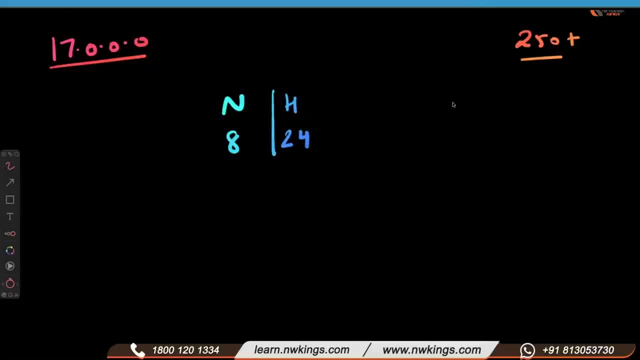 in india. we have offices in hyderabad. okay, we had sorry. okay, so we. and also in goodgown, also in bangalore, the apple maps. that apple maps development is going on in hyderabad for your information. okay, bangalore is taking care of all network part, so the data centers are allocated. 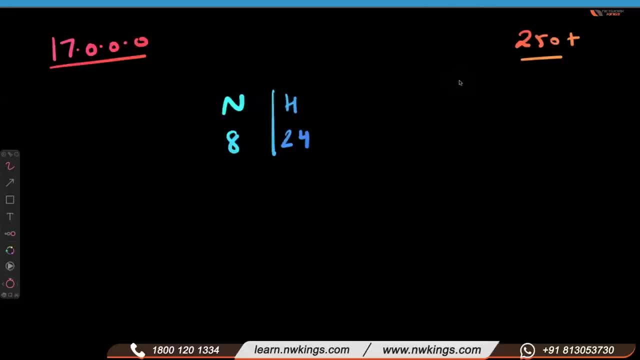 uh, apple data. and one is in usa also, okay, cupatino and all. so this is just i'm telling you from that real experience so that you will understand more. so i have a block, okay, so you can see the tim cook ceo of apple, so you can take that example also. so, or, steve jobs, uh, at uh, very, uh, like too many. 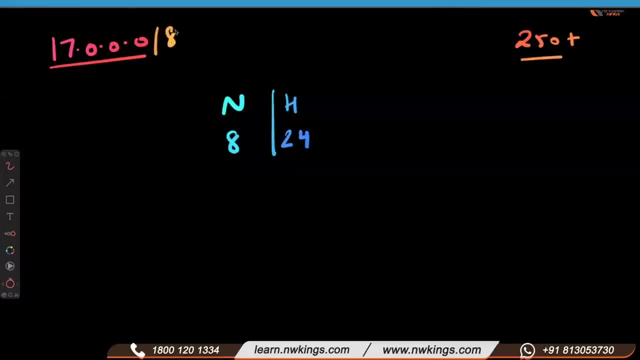 years back when apple started, they got a block, or obviously this block is 17 right, so this block is 16nm right, like total 17nm, for the messages is constituted by a little good network, so they could stomach like, for example, one and one or do the divide into twos existing. 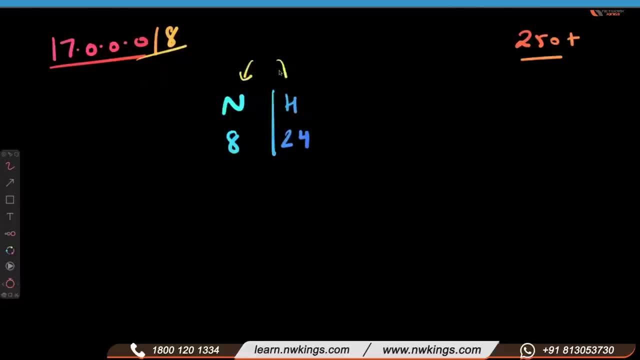 number of these. 16 is the median12 division of the network and about it by half of 16, three human length. so each one divided into 16ов. this is called one group of 1 is 2 to the power of 2 is 4, to the power of 5 is 32, suppose, to the power of 6 is 64. so i'm 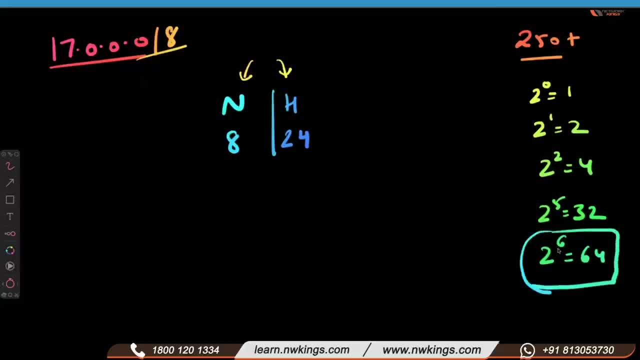 going to divide my network into six parts, right, or say sorry, 64 parts or maybe 64 countries. let's take example. okay, if you want, then you are going to add the six value here. right, if you want 64 countries, you want network in 64 countries or 64 locations, you are going to plus 6 here. 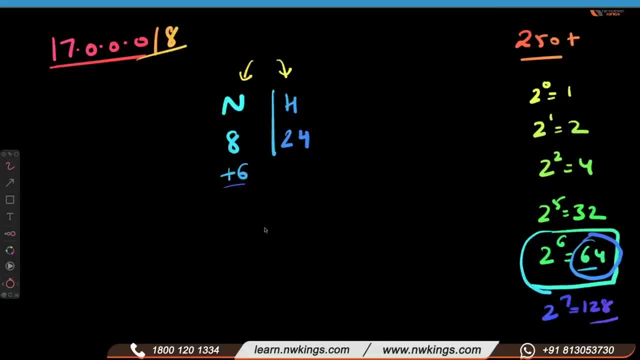 if you want to the 120 plus countries, you are going to plus 7 here. clear, okay. so it's totally your choice. but if you have, uh, if you do subnetting in this way, that for every location, every location, for every country, i'm going to assign 8 000 computers and for 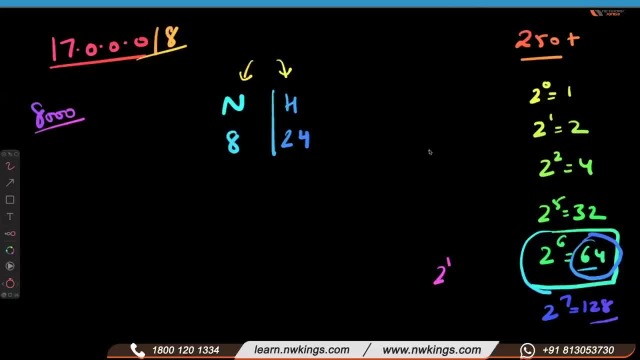 8 000. what is the value? to the power of 10 was 1024, to the power of 11 is 2048, to the power of 12: 4096 and to the power of 13 is 8192. yes or no? yes, yes, that is correct. yeah, so if i want 8 000, 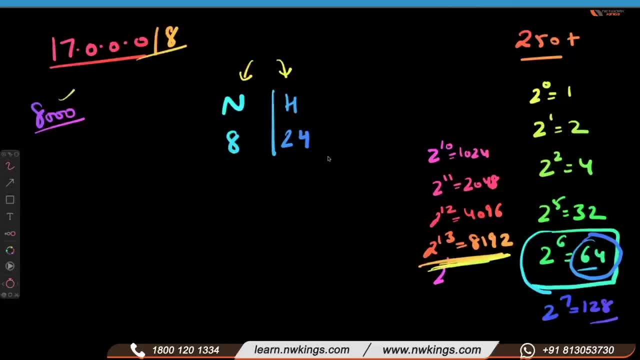 computers. you can also do the calculation with the host part also. so let's take, tell me what you want from network perspective or host perspective. both are okay, right. from network perspective, okay, no issues. so what i'll do? like, suppose i want to divide my network into one, 28 countries, okay, so 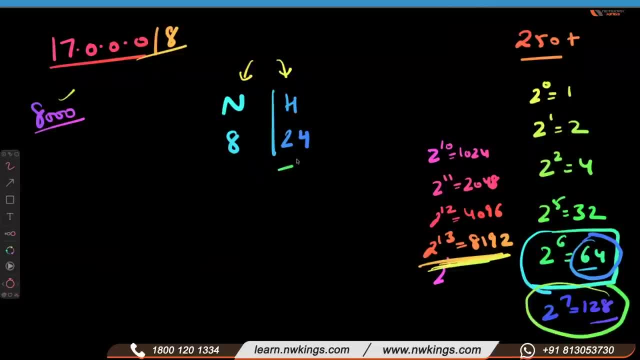 what you have to do. just for your information, for host, you are going to minus 13 here for 8 000 users. okay, so what you get here? 11, 11 plus 8 is 19.. yes, right, so you get. according to host, you get 19 host. 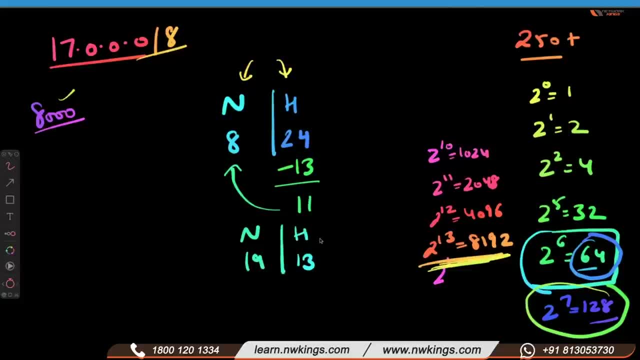 sorry, network and host is 13 and with this is according to host and if you calculate by, if you calculate by uh network, yes, yes, actually okay. so n is 824 for 128 countries. i'm going to plus 7 this side and minus 7 this side. 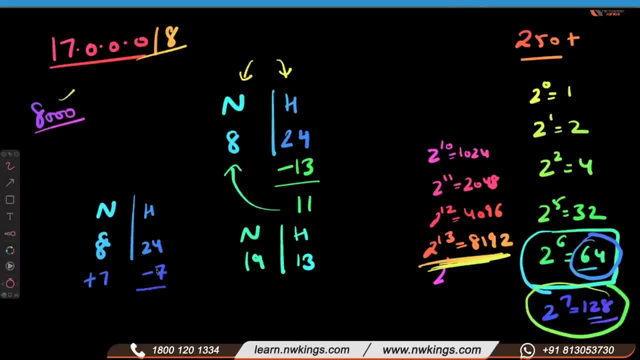 right, so i'm going to minus what i'm going to get here. 24 minus 7 is 17. yes, 8 plus 7 is 12. yeah, 8 plus 7 is 15. so this is according to my countries. okay, now it's totally up to you. now you guys can calculate according to this. 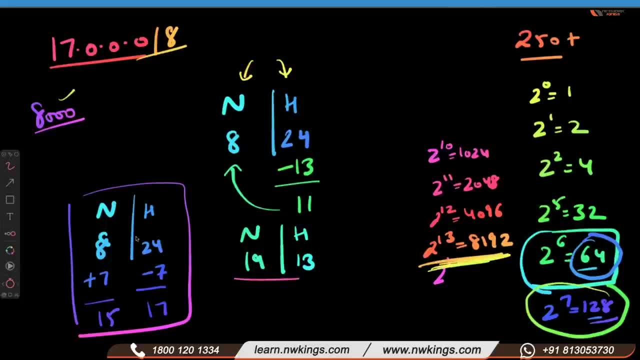 okay, so i'm telling you the both so you can see what i'm going to get for you. and slash 19 is 255, 255, 16, 16 plus 3 is 224, 224. okay, if you minus 256 minus dot 0, so you get 32.0, right, yes or no? yes, sir. 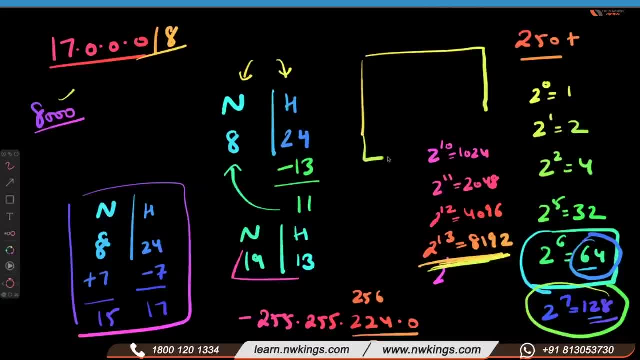 yes, yeah, so you are going to write a lot of blocks. obviously 2 is not enough, but still you can understand. so 17, so you can see we have 2255, which is completed. it means this is confirmed. you have first two octet network bits. so it means you are going to write 17.0 outside. 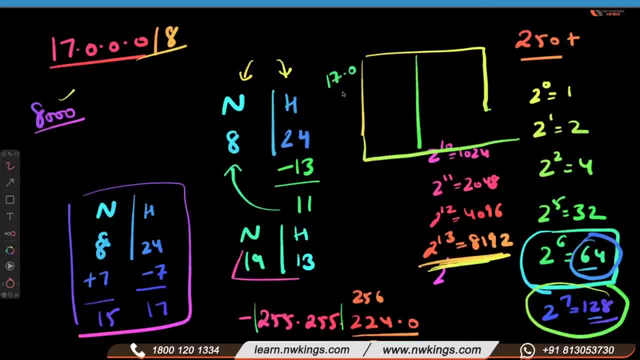 correct in starting. so you are going to write 0.0 in the second block. you are going to get what? or you can write, because this is class a. so what i recommend? you can write three zeros as well, don't worry. okay, but the calculation will remain same: 0.0.0. but your answer is: you can see 32.0, so you will be writing 0.0.32.0 because 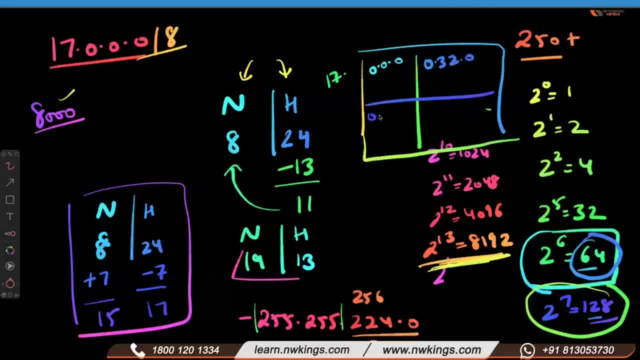 this is class a remember. so next block will be 0.64.0 and next is 0.96.0 and before 0.32.0. what you get? 32.0, 0.31.0, 255. very good, assigned to any country. 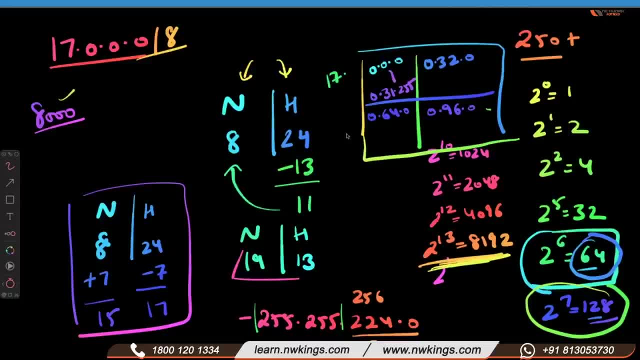 whatever. so this is according to 8000 user, so you can assign this to india and after that you 63.255. you can assign this to another country. then keep checking this. you are going to assign this whole subnet, starting from 17.0.0.0 to 17.0.31.255. 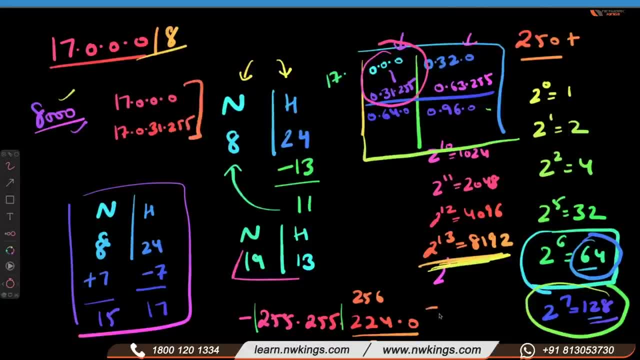 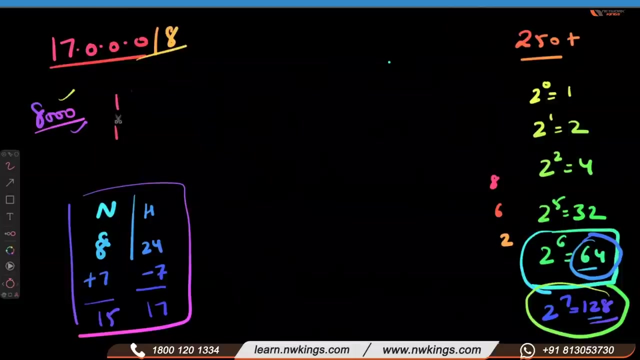 so you are going to use this one and the subnet mask for all the computers will be this one. if nobody had a grandes siete in india location, clear, yes, sir. so if i calculate it for fall, if i calculate this for E, this 128 countries, you can undersee that, that for 128 countries i have taken 77 sound. 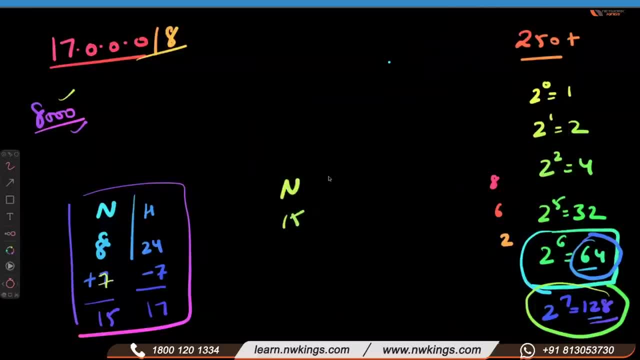 extra bits. so my network is 15 and my host is 17, right, so 15 for 15. i am going to have a subnet mass 255, uh 254 dot 0.0. like this: yes, correct, yes, so you are going to say 256 minus 254. that makes: 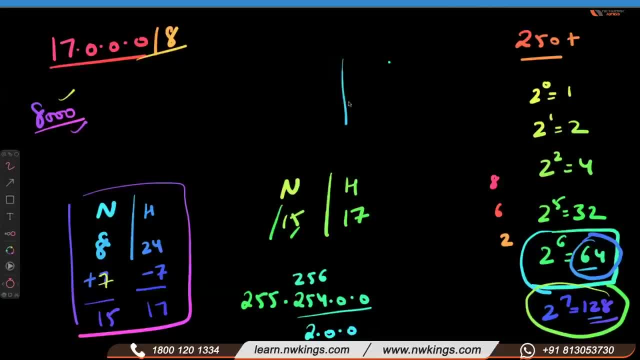 2.0.0.0. it means you are going to write the block 17 outside. 0.0.0 will be my first, and the second will be 2.0.0. right, and another one is 2 plus 0. 0 is 4.0.0, another is 6.0.0. so what comes before? 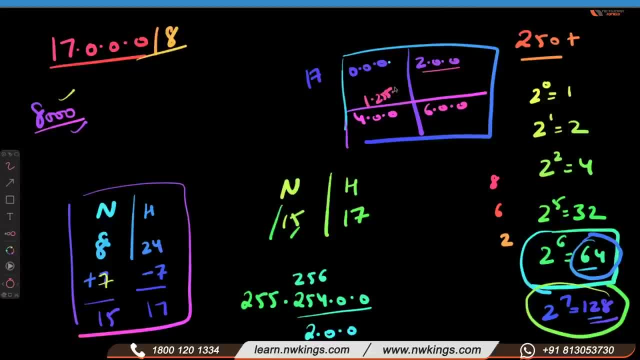 2.0, that i think. one dot, two, five, five, two, five, five, five, five, five. yes, very good, once you complete it two times- two, five, five- then only you come into this block: four dot zero, three, dot, two, five, five, two, five, five and six dot, zero, dot, five, dot, two, five, five. 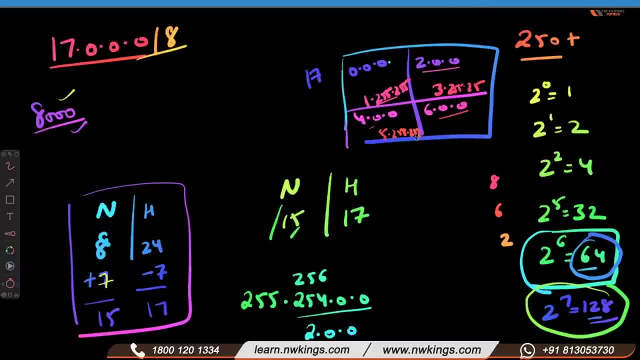 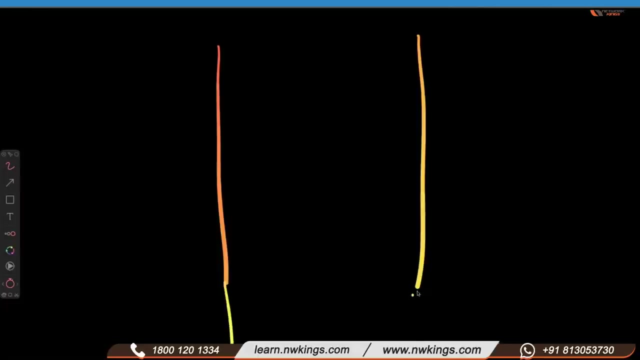 two, five, five, yes, everyone clear, yes, yes, yes, sir, so all all things. what we were doing is flsm, right, and now you guys have to practice, okay, so just take it, just do like in a very casual way, let's do last three questions for today. so let's take c, again b, let's do one a, okay, so give me any. 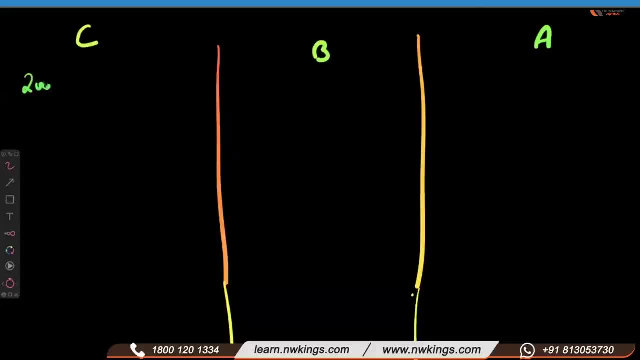 ip for class c: 200 is okay, yeah, okay. so tell me, this is my by default 24 and h is eight. so tell me, what do you want from this ip? you want to divide this into two parts, or you wanted to calculate: 400 user, 50 user, 32 user, what you want. 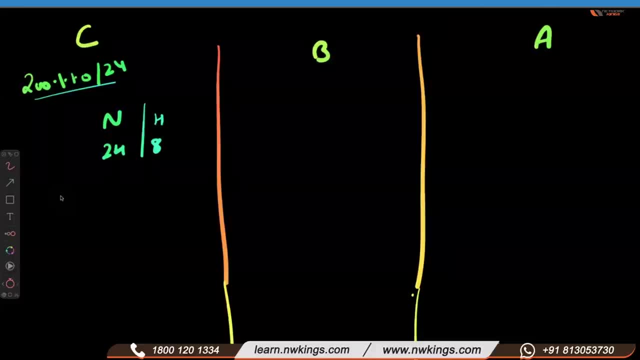 32 users. sir, 32 users, yes, okay, okay, for means approx 30, 32, 32 right, because for 32 also you have to take 64. so don't get confused for that. so let's take 30 user, okay, yes, okay. five, yes, two the power of five is 32.. two the power of six is 64 and two the power of four is. 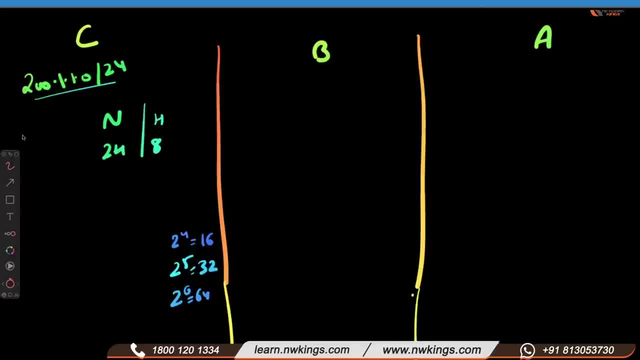 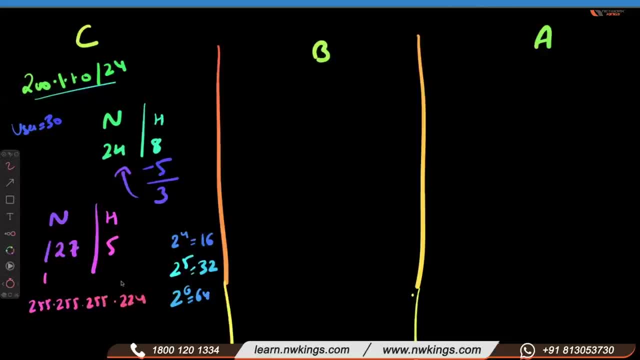 two to four. two to four. you can also subtract here also, so you get your. that's the same thing. you are going to get to the power of 532. if you minus this, you will also getting 32.. okay, either you check from this side or you can take the same formula like which you used for bna, just subtract. 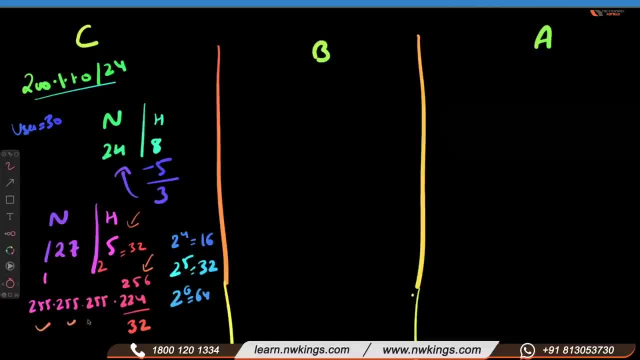 this, uh, from the gap which is not completed, and you get this one, 32 and you can write the range. okay, you can write the range boxes like zero or another box 32, so it will run up to 31. 0 to 31, clear, yes, sir. okay, let's take b class: 150 dot 10.0, dot 0, slash 16. so this is, by default, network 16 host. 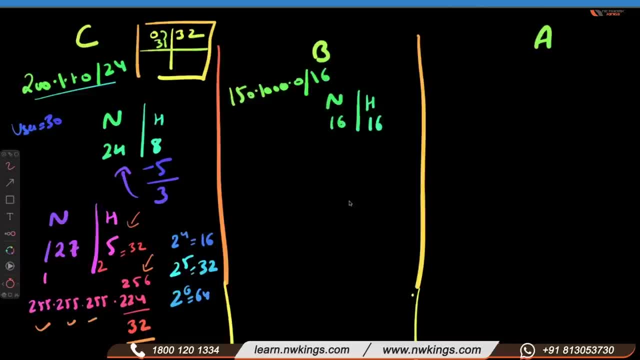 16. tell me what you want. let's divide the network into eight parts. what do you think? yes, sir, yes, sir, okay, so you can write the range boxes like zero. another box, 32, so it will run up to 31. zero to 31. okay, so to the power of a, one is a two. to the power of two is a four. to the power of three is. 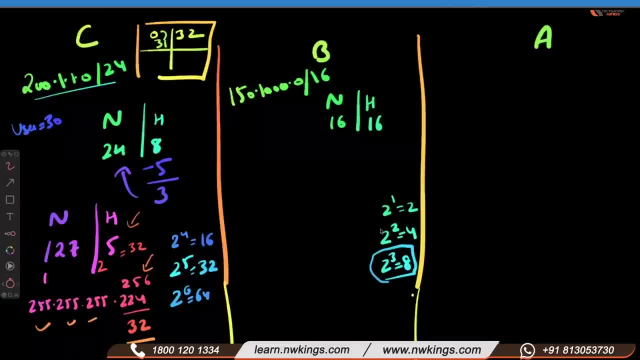 eight, how many networks? nine, eight, yeah. so you are going to plus nine, three, yes, and minus three, so 19, and you are going to get 13 this side, yes, yes. so for 19, what is the subnet mass? two, five, five, two, five, five, five, five. uh, sixteen, two, two, four, dot zero four. 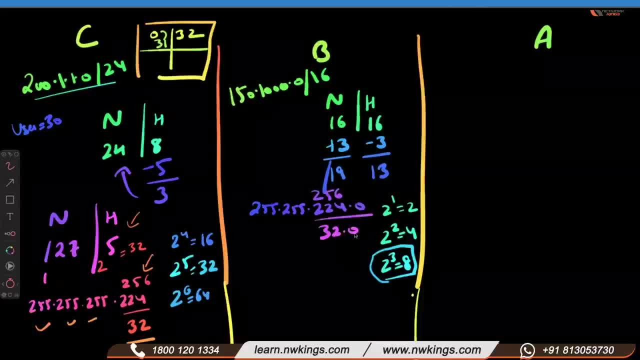 you minus 256, you get 32.0 right and you are going to write 0.0. next block will be 32 dot and before that what you get? 31.55 and keep adding because you need eight. now you are. your requirement was subnets. how many? you needed eight. eight network right for eight networks. you can make eight block. 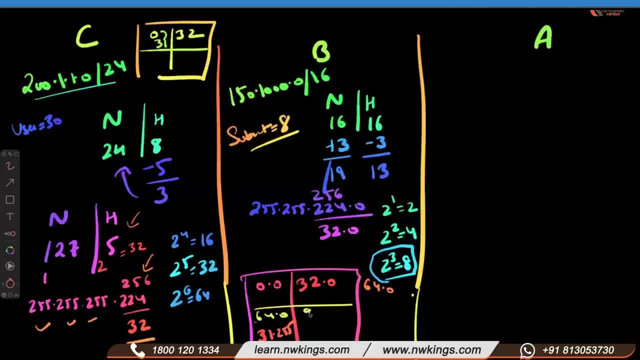 and keep checking this. okay, like 64.0, 96.0, make just keep adding 32 for eight networks. okay, 32.0, you get 31.255. clear, everyone. yes, sir, okay, a class. let's take a 17 block, which is my favorite. 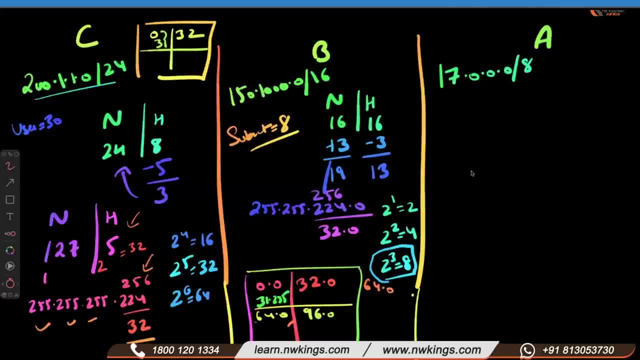 okay, so tell me what you want. already two questions in the chat. okay, so tell me what you want. already two questions in the chat. okay, so tell me what you want. already two questions in the chat. already two questions done. uh, we need 10 000. okay, let's uh, let's take example. 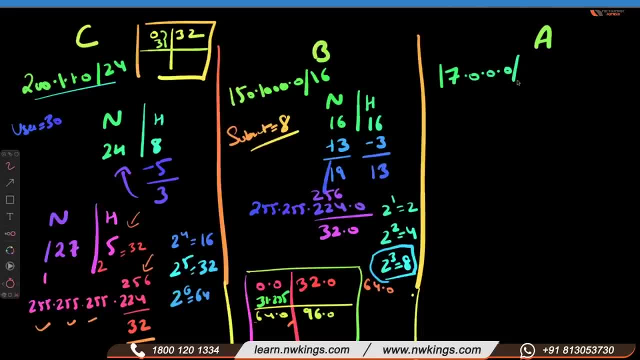 so what you got in? 8000 computers: slash, slash. what's our 8000 one for 8000 computers, are you sure? 32, 32, my host was 13,, so I was getting around 19,, am I right? so for like, let's do another. 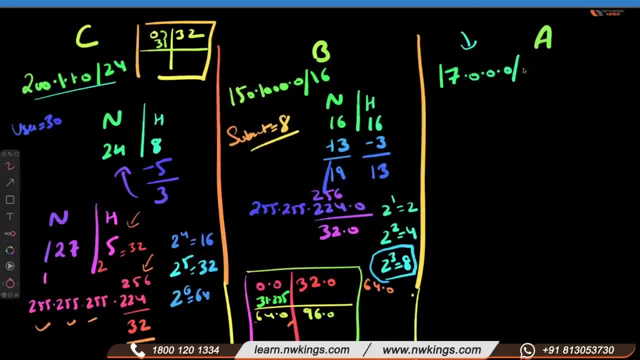 part. suppose India location got IP 1700019, right, right, yes, sir, yes, sir, okay, now you, for India location, we got 8000 computers almost, or 8000 host. so you want to divide this. network is 19 and host is 13,. right, so you want to divide this network into four. 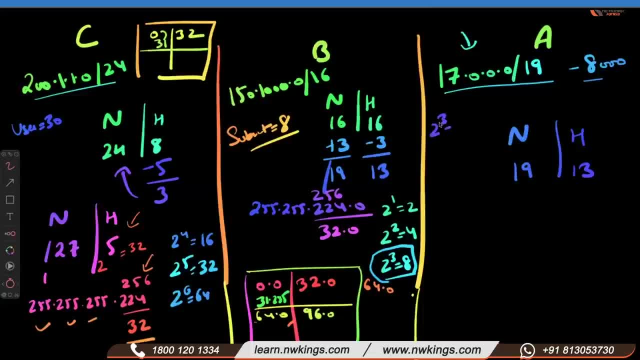 parts. so what you are going to say to the power of three is sorry, to the power of two is four, right, yes, so you need extra two here and minus two here. so 21 and you get 11.. For 21, you are going to get 255, 255, 16 plus 5, 248, 248.0, minus 256, you get what? 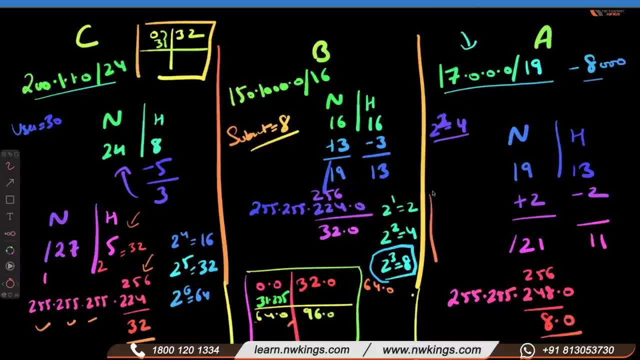 8.0,. right, and you can calculate your blocks according to this, that first IP will be 0.0,. second block will go up to 8.0.. Third block will go up to 16.0,, 24.0, and it will go up to 32, remember so R digits. 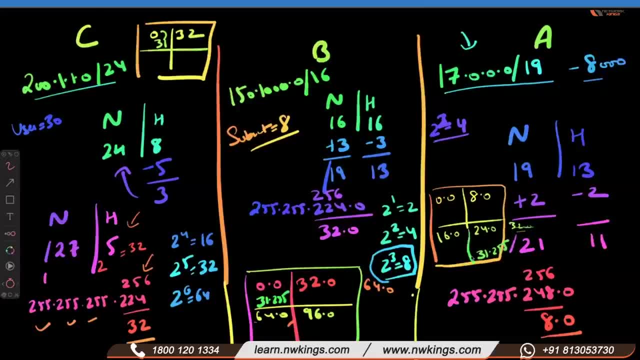 till 31.255 for India location. remember, yes, sir, 8.0,, that is 7.255,. yes, yes, 15.255 for 24,, 23.25,. oh, ma'am, okay, ABC. 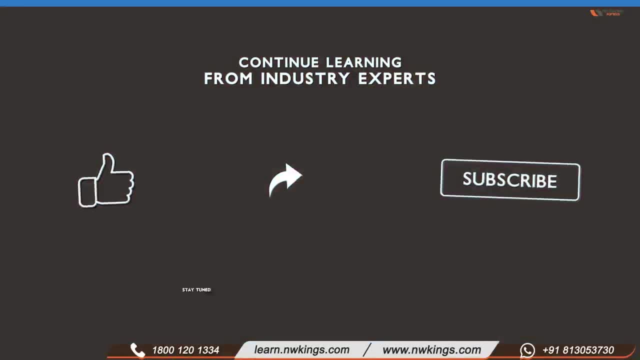 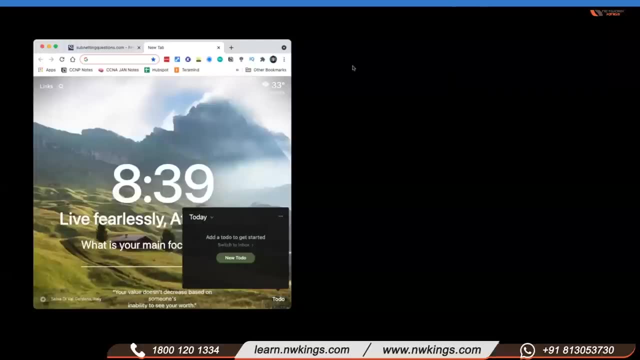 Hi, you are watching the recording from one of our live session. hit like share and subscribe for more future updates. So today we are going to cover VLSM VLSM questions. what is VLSM? variable length subnet? 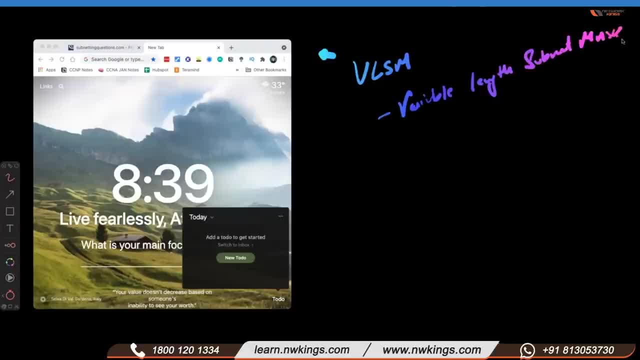 mask. okay, so this is our topic and after that we are going to do some questions on this website. This is a website called subnettingquestionscom. if you continuously attempt 10 questions and if all your 10 questions answers is correct, it means you are already expertise in subnetting. 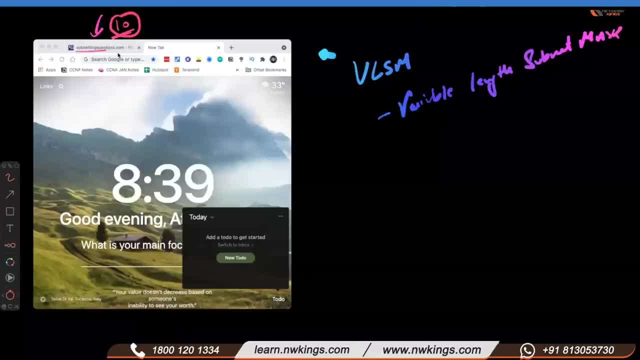 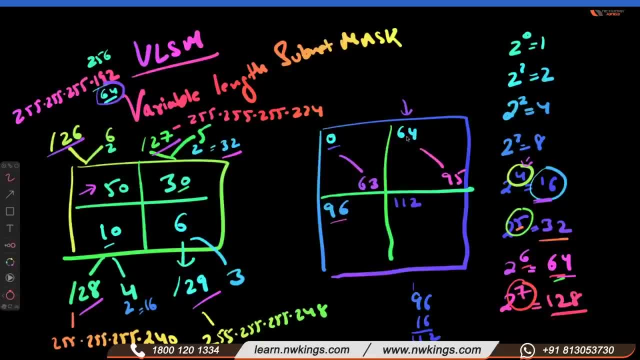 you will not be able to answer all your questions. okay, so this is your goal till the time. you will not be able to answer all your questions. okay, so this is your goal till the time. 255. this is for future use. you can use it for further calculations. but before 120 you have 119. 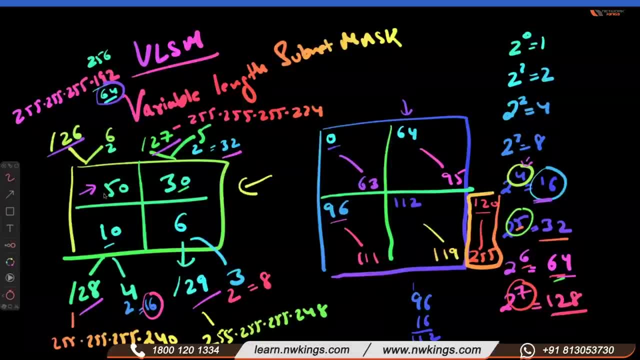 so it means you can assign your ips in these four computer labs. like for 0 to 63, my slash value, my subnet mask, will be this: 255, 255, 192. for computer b lab, i am going to assign this subnet mask. for computer third lab, i am going to assign this subnet mask. and computer 4, i am going to 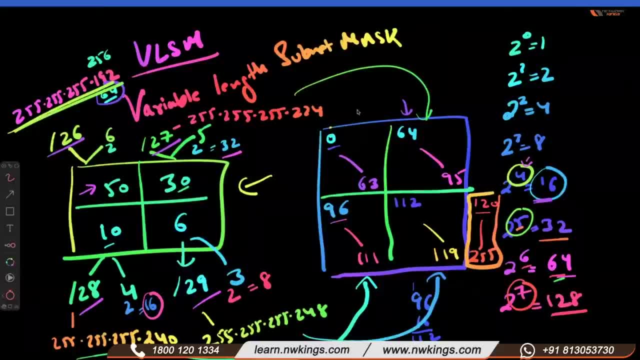 assign this subnet mask. so this is vlsm. so whenever you finish the first subnet, the second subnet will start from there only because 0 to 63 ips is assigned. right, so 0 to 63 ip assigned. you have assigned these 0 to 63 in computer lab a. then from 64 to 95 you have assigned in b. 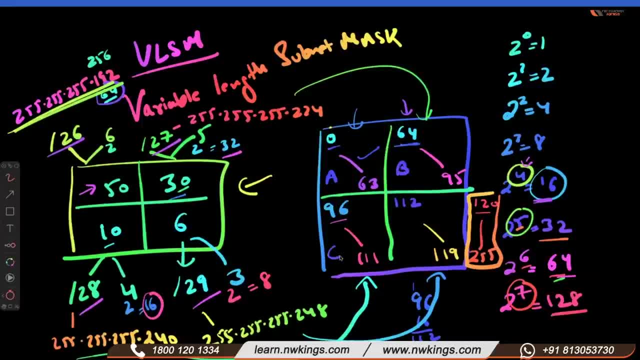 lab, then 96 to triple one you have assigned in c lab, and if d like, you have assigned 112 to 119, right? so this is what we call vlsm, this is what we call variable and subnet mask. all computer labs will have different, different subnet mask. 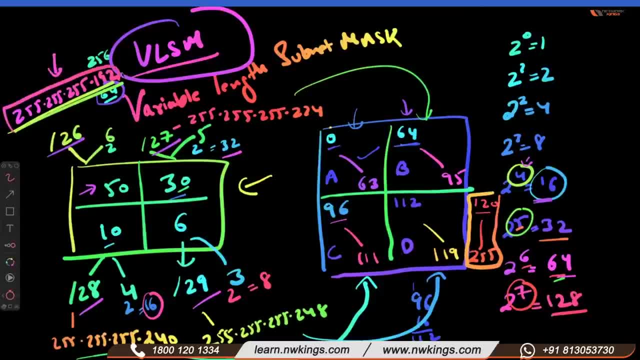 in computer lab a, we will have 255, 255, 255, 192. in computer b, we will have this. in c, we have this and d, we have this clear. yes, sir, sir, there is one question. yeah, sir, sir, uh, here is a. all the subnet masks are different. 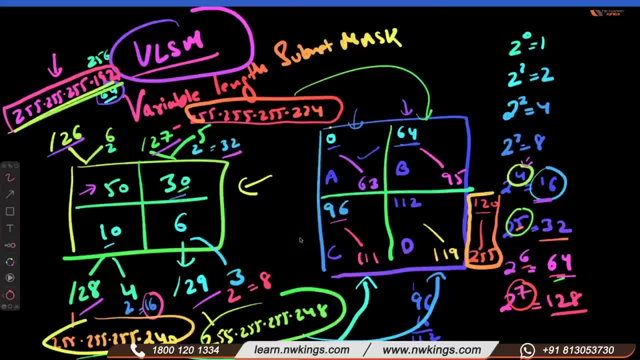 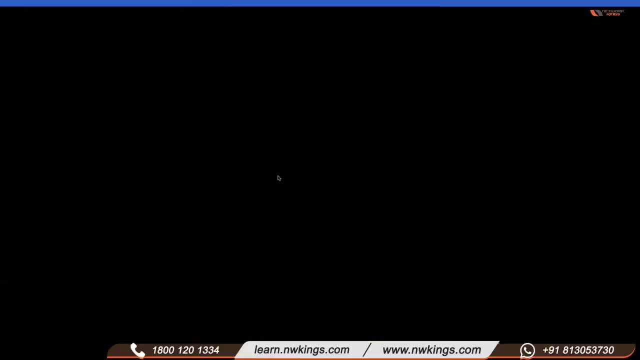 so without routing they all are in uh interconnect with or like a lab lab aip can be connected with lab bip also, or not? no, no, no, no, if you want. now they are in different subnet because when you do subnetting they all become in different subnet. so you need a router so that. 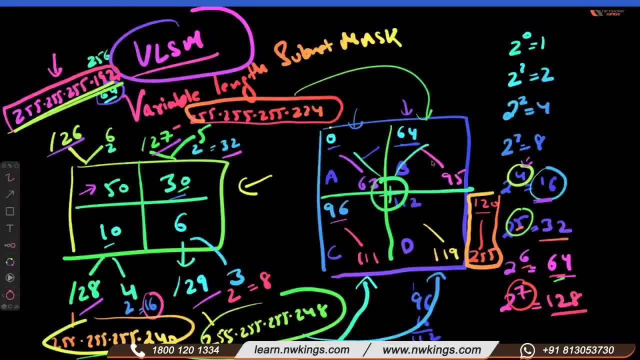 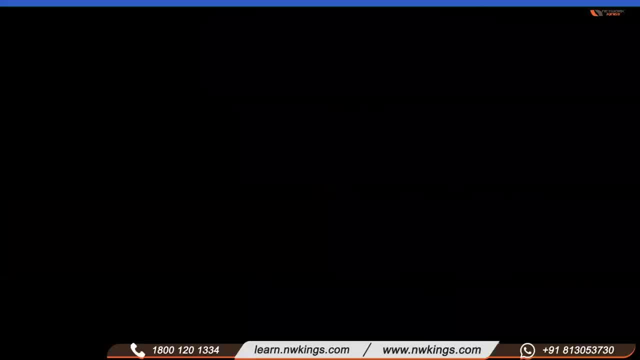 can communicate with each other, so you can have a router. you can create this same lab. so how many of you all know packet tracer? yes, i know. most of all of you know right. yeah, i know, yes, yes, i know okay, so i'll show you how to do this, okay. 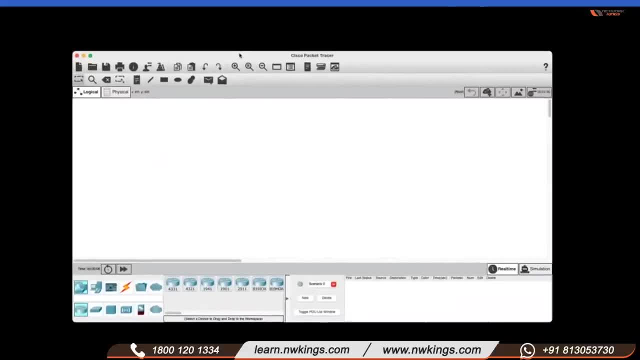 so this is packet tracer. you can use a gns3, even g, whatever is your choice. so now you can take four departments, like i have a told you, like four computer labs: 1, 2, 3, 4. okay, so you can take a router with four. 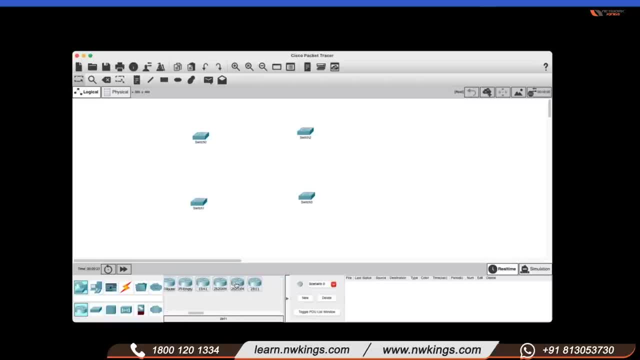 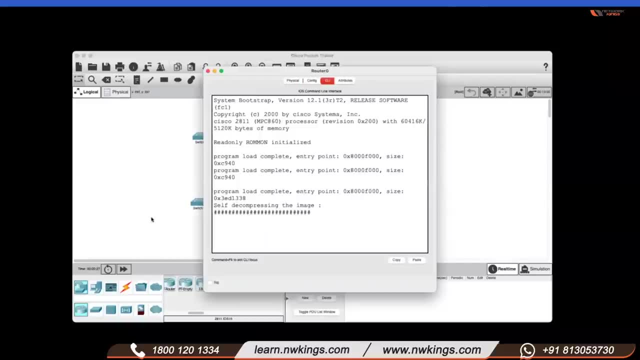 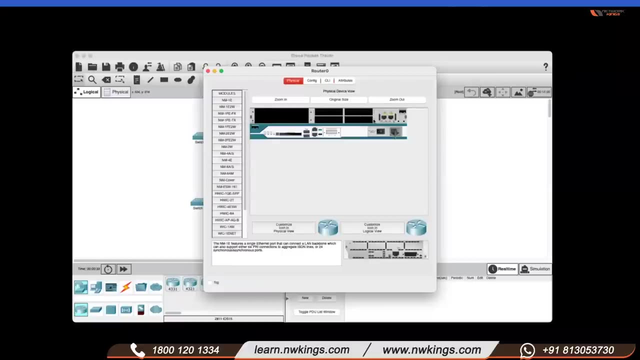 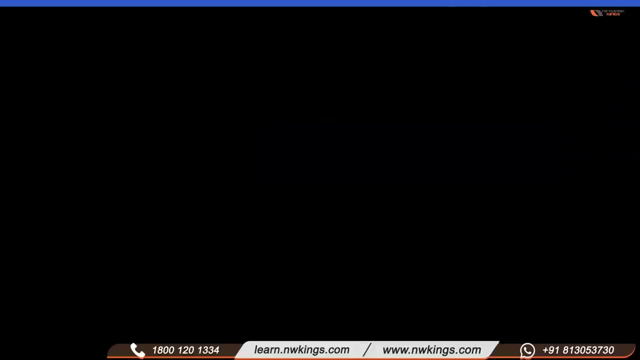 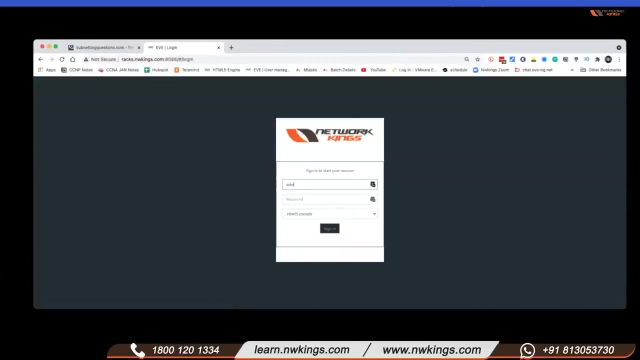 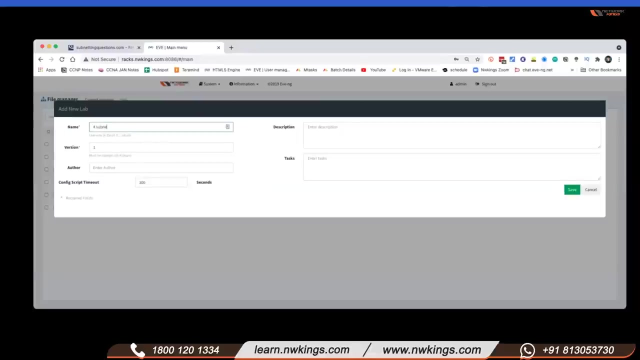 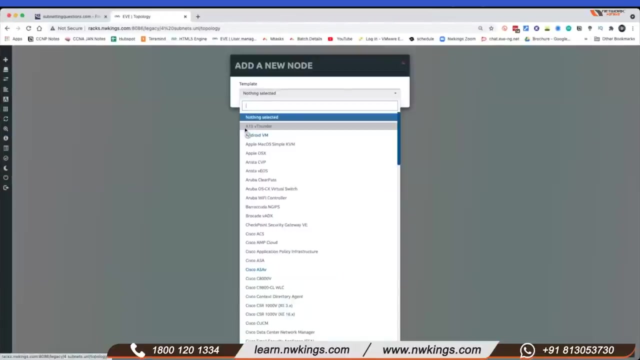 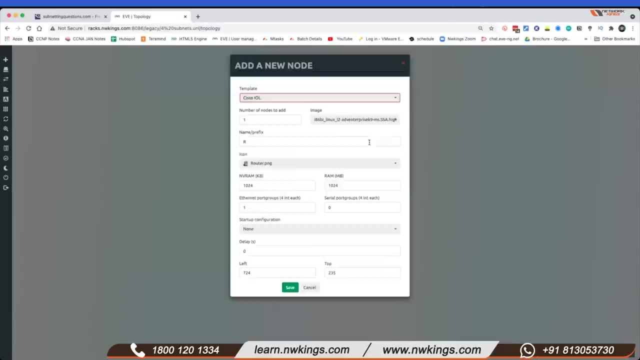 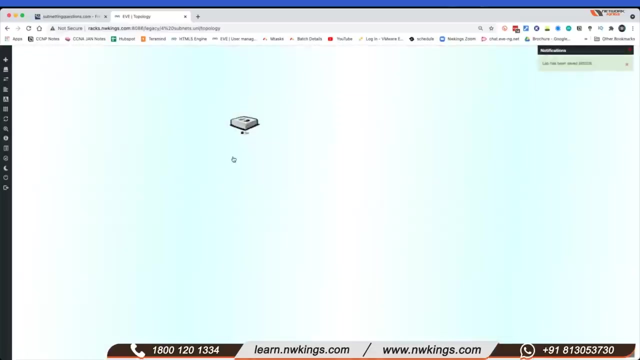 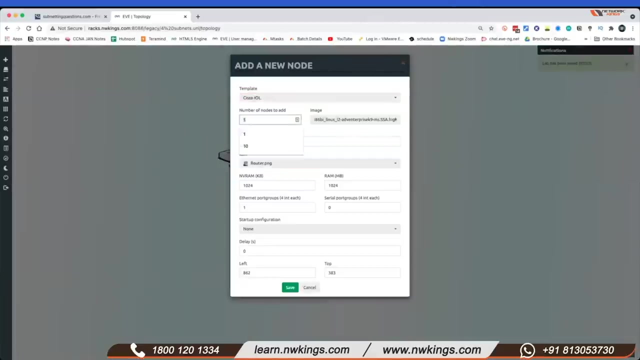 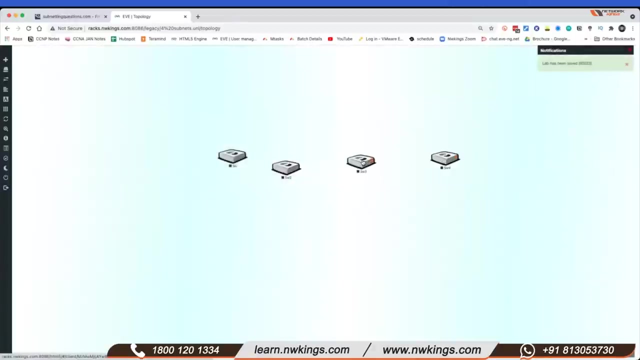 interfaces. so let me check if i can add a module so you can do. okay, so mac has a bug, think maybe because i can't add a slot. okay, leave it, so i'll show you in my racks. okay, so we take four switches, okay. okay, so four departments. okay, so you can assign whatever pcs you have. so i'm just. 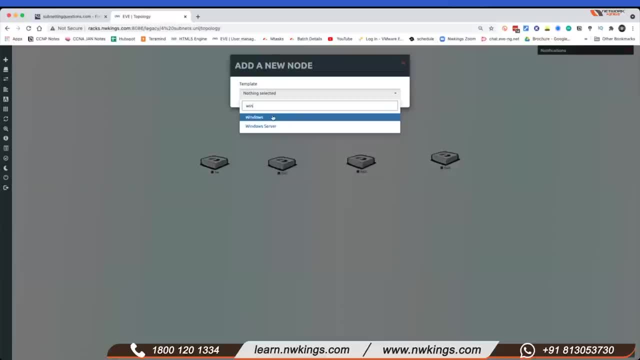 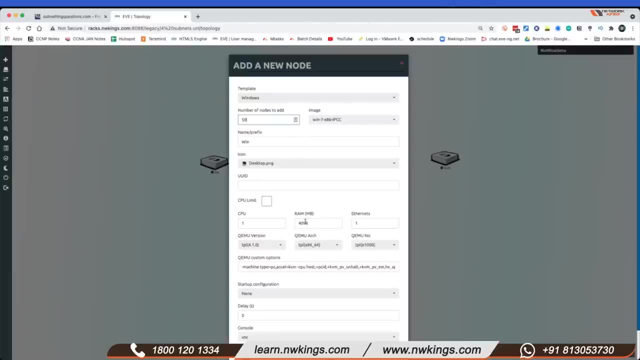 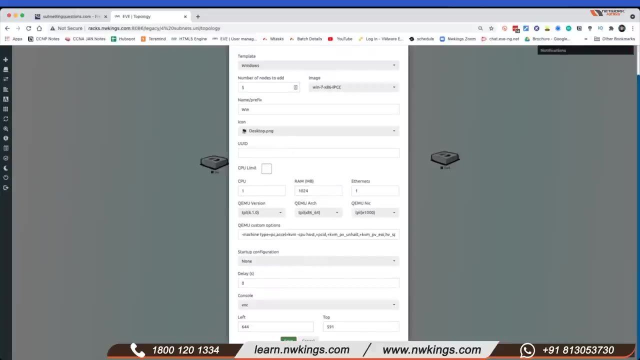 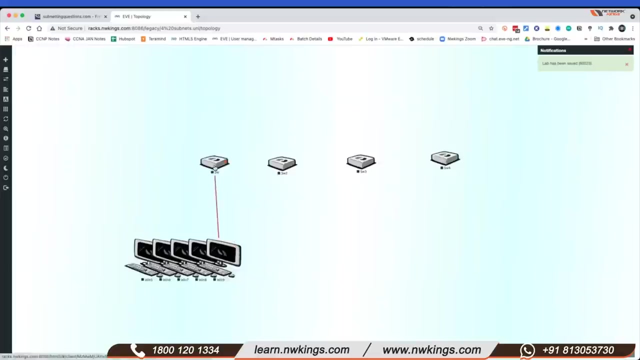 taking one figure like windows. okay, so i'm going to have almost how many 50 pcs, right? so it will be mess, so i'll write: i'll create five. okay, so consider these are 50 computers. okay so, but i'm just connecting one cable so that you will actually get understand. so what exactly? 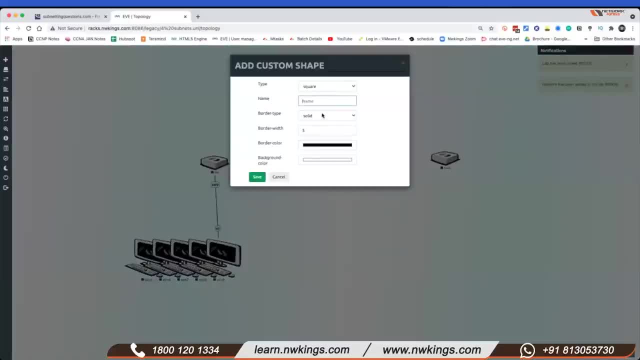 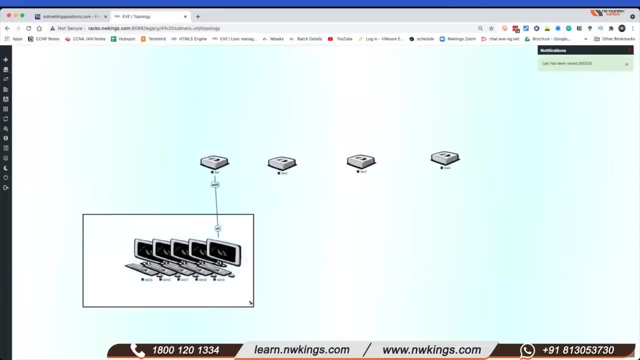 custom shape, let me add so. so 50, 50 pcs right 50 lab computer. so this is my 50 for 50 users, 50 users. okay. so now you can do this for further labs like this: 50 uses KEY sensor: okay. for main board senior citizens okay. and last two, two big pieces the left side of my PC also have more than 50 PCs right feet computer. so this is my 50 for 50 users, 50 users. okay. so now you can do this for further labs like this. okay, so now you can do this for further labs like this. 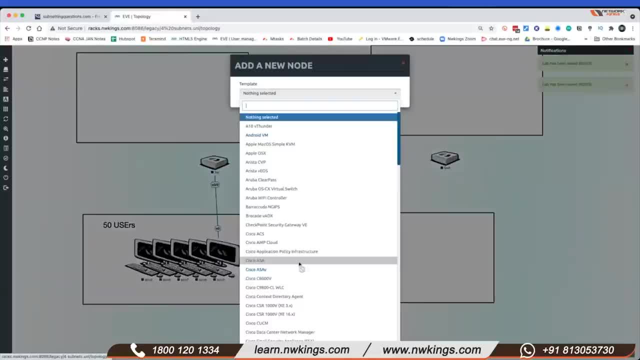 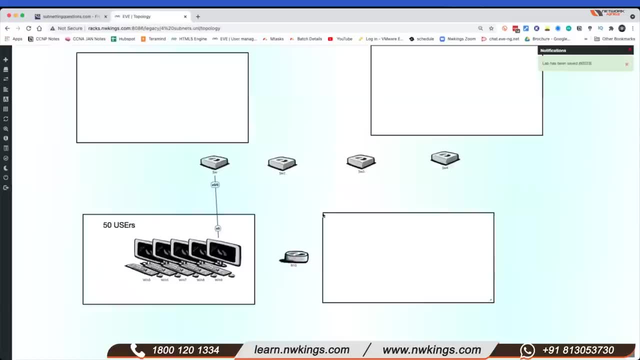 you know some summer differences, so it will be critical that you can do this anywhere and here you can do it wherever you want, without��서 to switch with another browser. Okay, so let me add a router. okay, so all the subnets or all the labs, like all the labs. 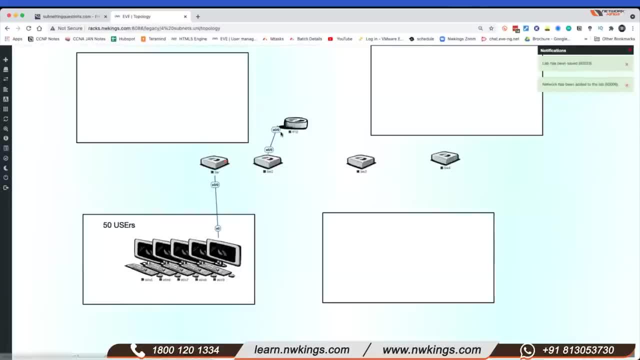 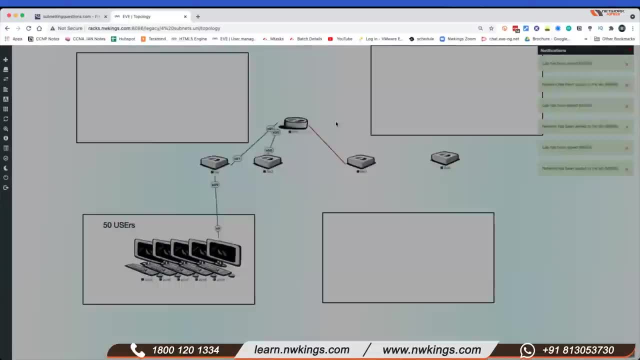 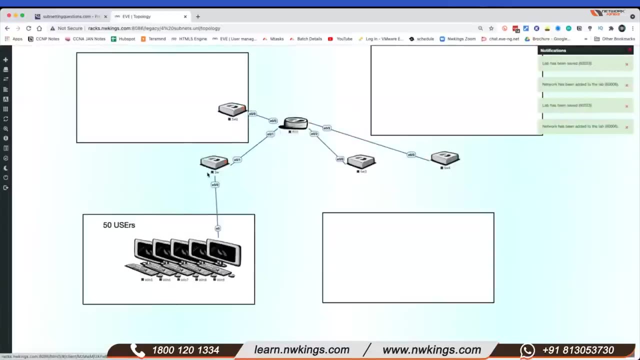 will be going to connected with router, okay. so, whatever is your requirement, you are going to do subnetting, okay. so this is for computer lab a, this is for b, whatever you want. so just for design, i am taking one pc so you can write down, but okay, so like 50 user. so third, so 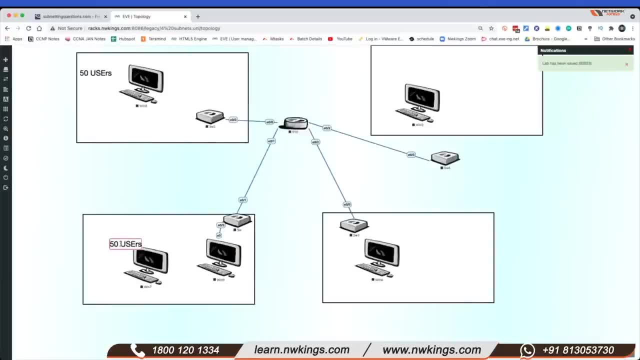 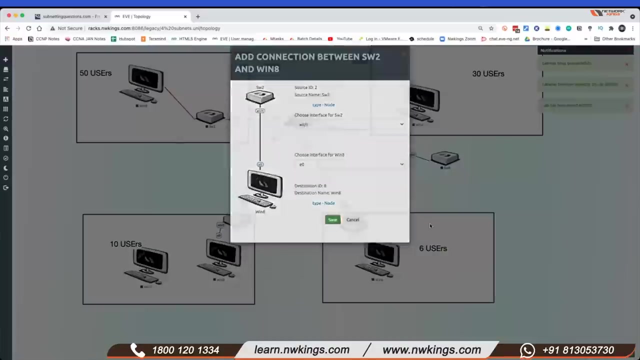 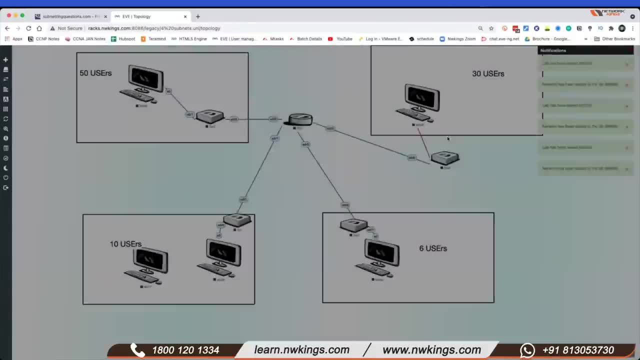 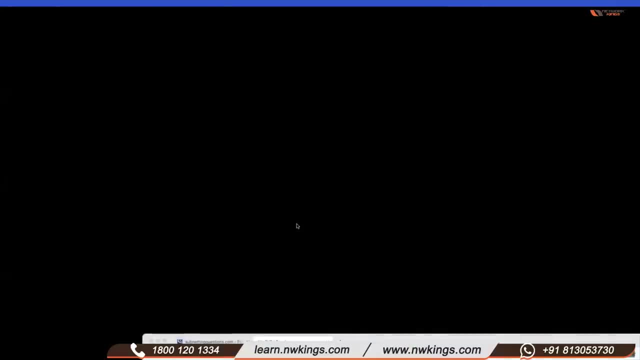 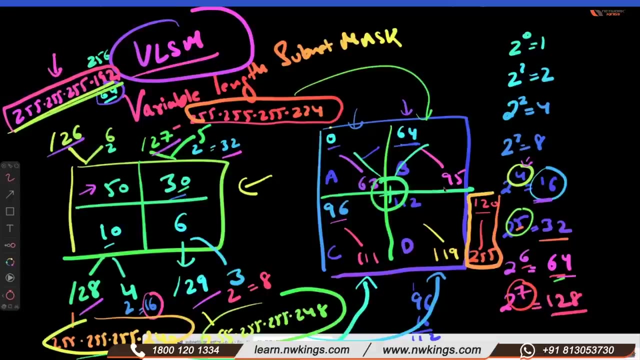 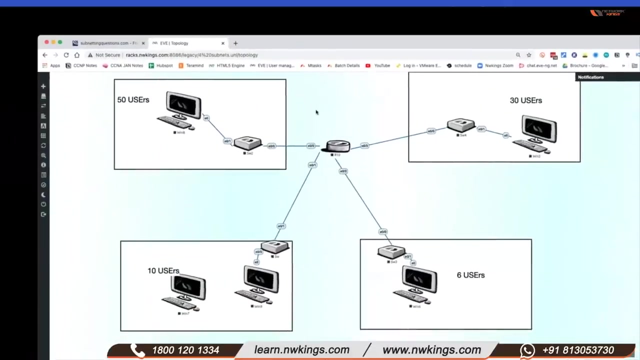 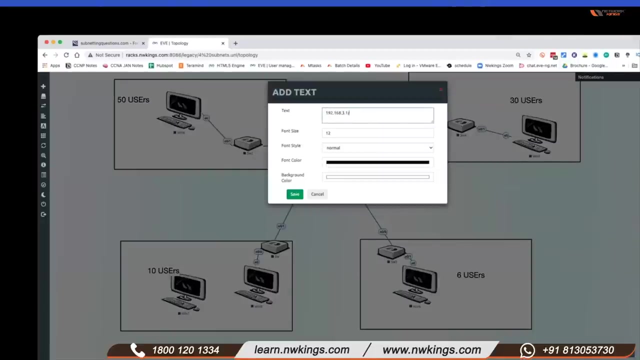 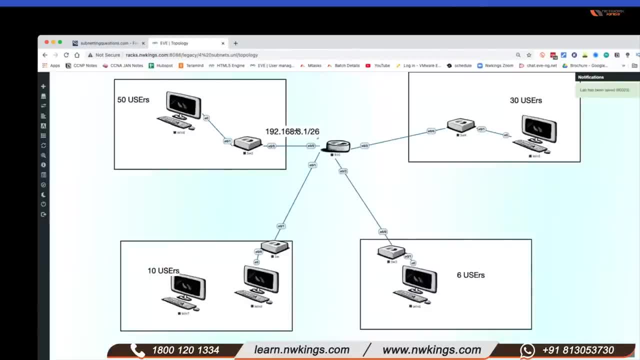 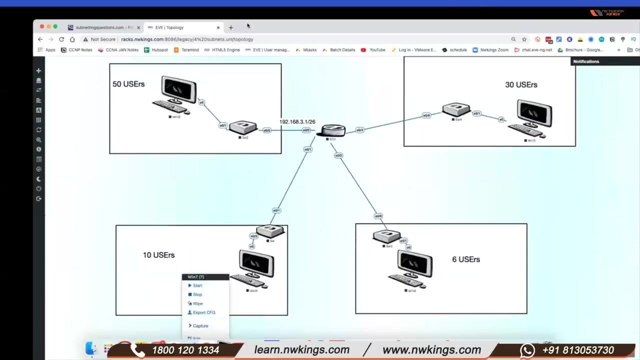 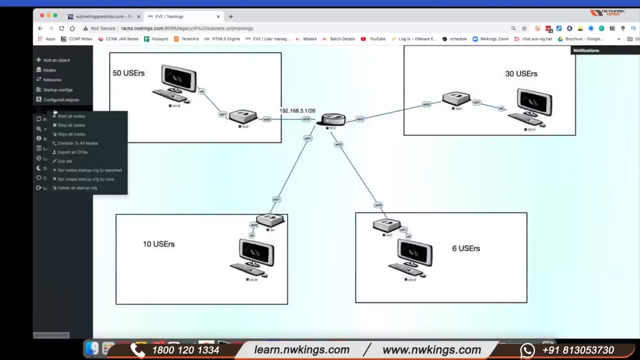 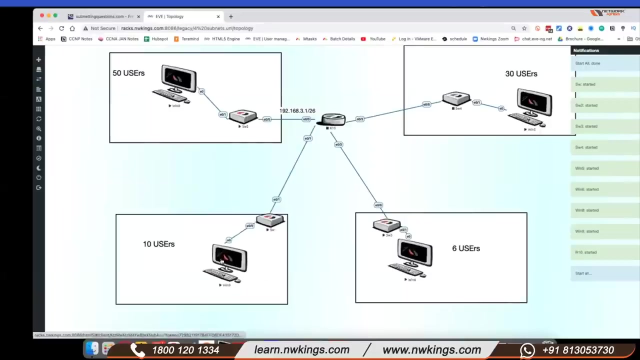 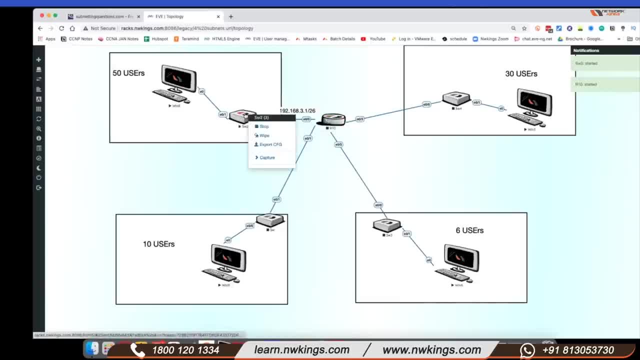 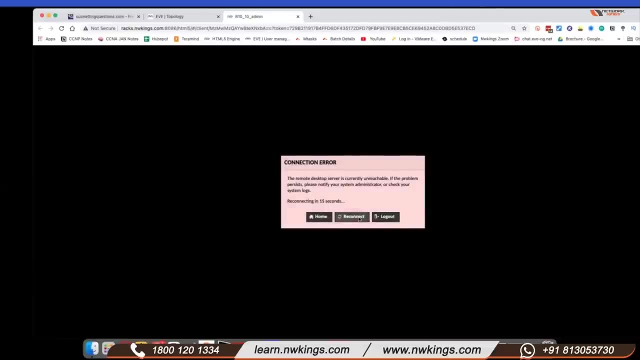 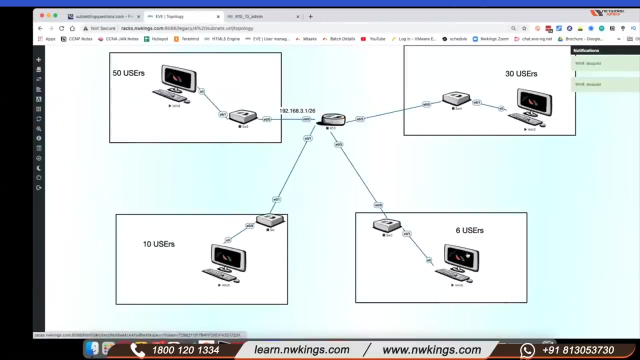 with anyK sun. ok, good thanks, no problem. ok, so this: how are you going to implement and whenever you actually connect the device, okmamacare, okmamacare, okmamacare. some issue is going on in this lab. i need to do the maintenance, okay, but once you do the 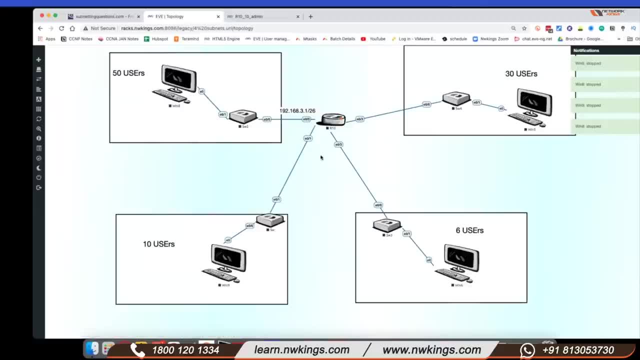 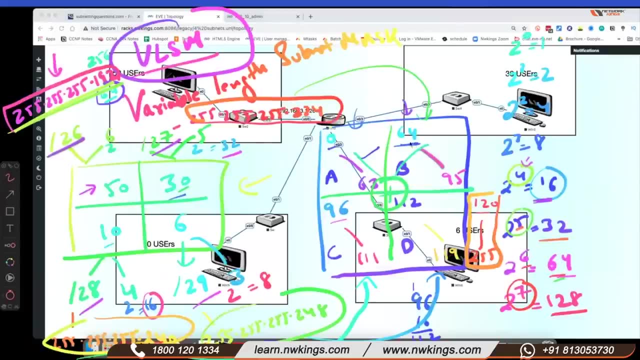 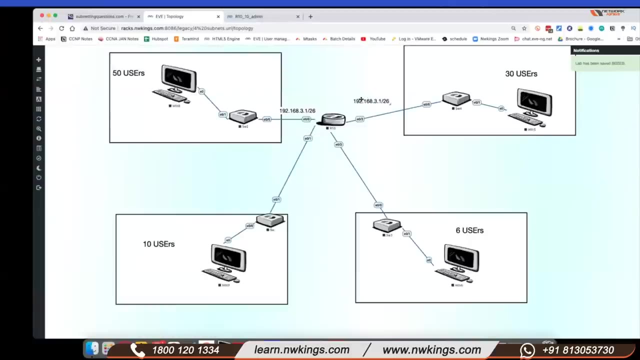 submitting. you just need to assign the ips on this particular interface. okay, so like 3.1, 26, the second subnet start from 64 ip. so you can't assign the first ip, so the second is subnet. you will give ip like 64 to 1- 1- 1. so let's assign 65 ip to this subnet. okay, third subnet: start from 96. 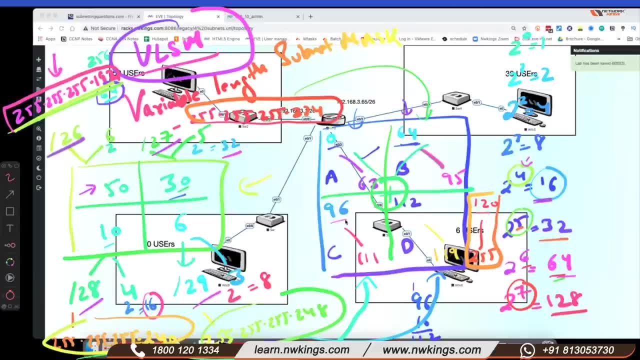 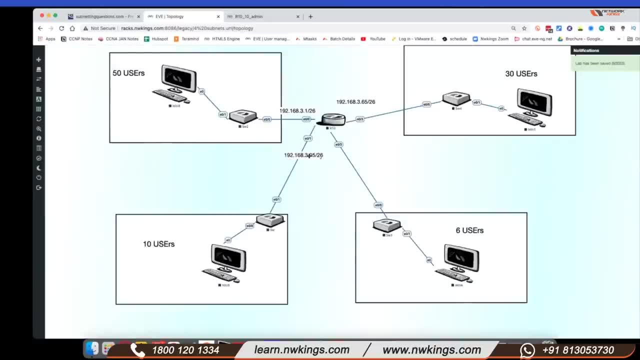 so we can give 97, or you can take a round figure 100 ip, also in c. so i'll take the first ip of each subnet, 97 on this subnet. okay, guys, any question? no, no, no, sir. okay, so this is what we call subnet 113. okay, but one mistake i am doing. tell me what is the mistake. 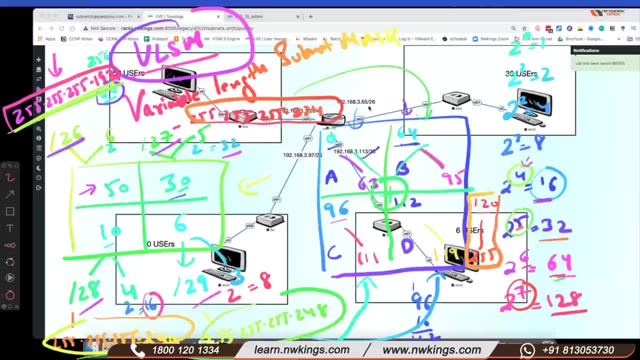 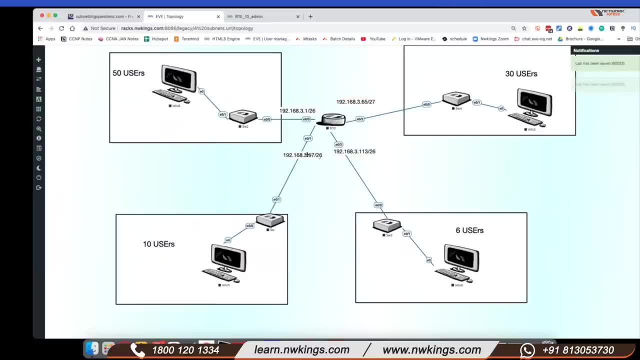 subnet mask: yes, so it's 26, but second one was 20- 7, and third one was 28- yes or no? yes, and last one was 20- 29. okay, you guys can take this screenshot. even i'll take if you want, okay, so this is how we are going to do. okay, let me check also, what is the issue? 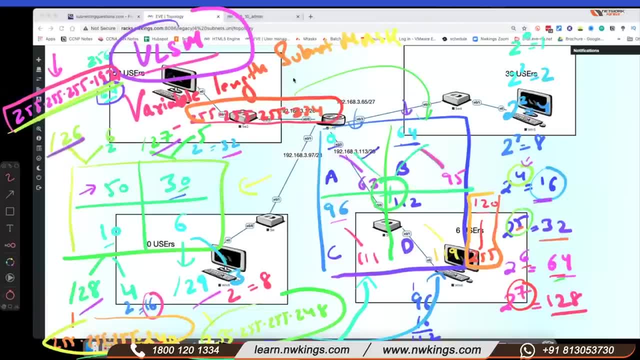 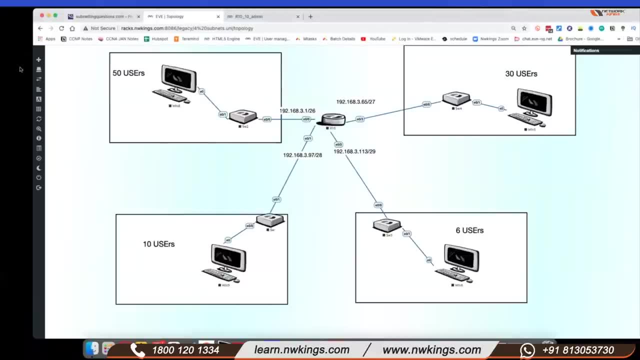 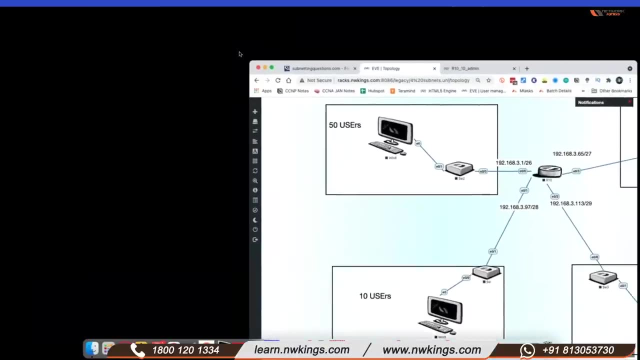 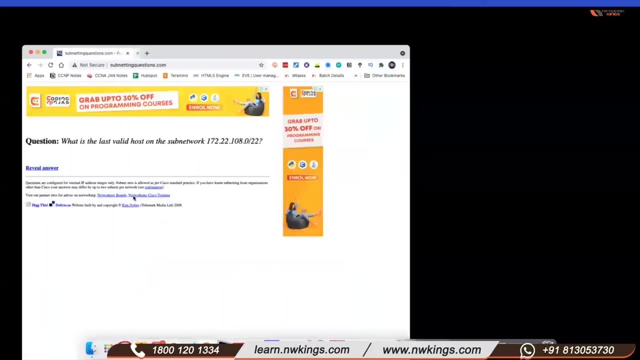 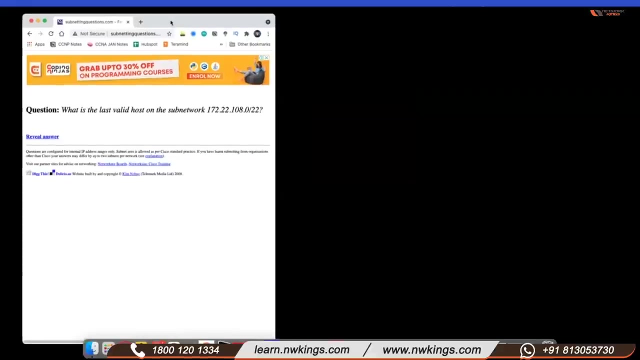 okay, guys, yes, sir, okay, okay. so our other focus should be on which website? 718 questions. so now, even if you're going for any attempt for any exam, you are going to get these type of questions also, but from interview perspective, i don't think somebody is going to ask you or these type of. 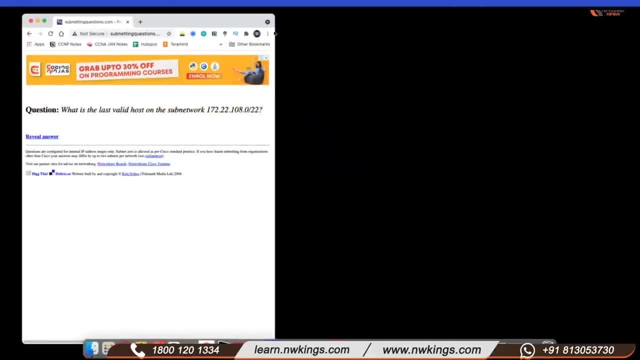 questions. so the type of interviewer questions might be. someone is going to ask that i have already covered. suppose you want to give any exam, so this is according to that. okay, so now? so, so this is the question, right, so you can write down this question and always remember. 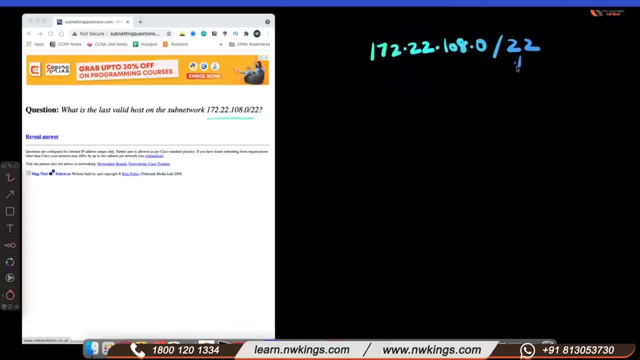 whenever you get the network part, you can just write down the subnet mask of that: 255, 255. tell me what is the subnet mask? 16 plus 6, 6, 248, 52, 252. yes, okay, so 252.0. so you can minus 256 minus 252. 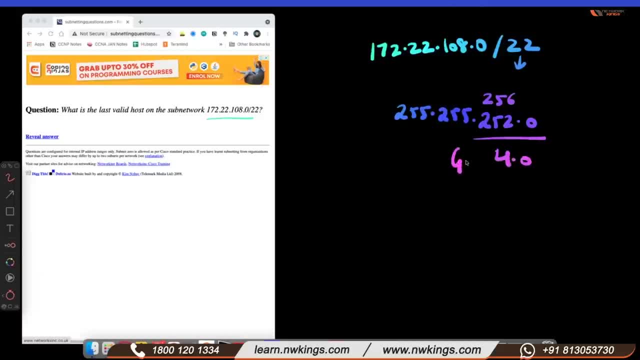 what you will get: zero, four dot zero, what we call this gap. yes or no? yes, sir, yes, right, so now you can see. my ip is third block is going on. which ip 108? so tell me if i start with 0.0 to 4.0. so i'll keep. 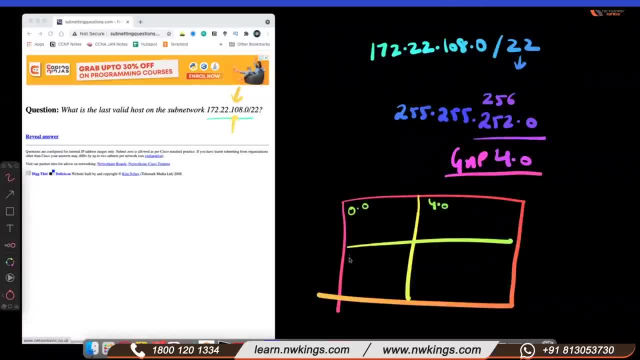 going on, so might be after few blocks i'll be having 100, then after that 104, 108 also, yes or no? yes, sir, right, if i'll keep adding 4.0. so this is a dividable by 4. so it means i'll be having 100, then 104, then 108, yes or no? yes, and 108.0 plus 4.0. 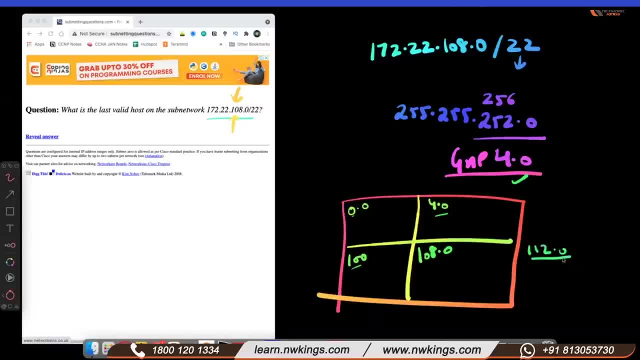 what you get: 112.0, right, yes, so before 112. what is the answer? triple 1.255, yes, yes or no? so this ip belongs to this network right now. this question is asking: last valid host means this is my broadcast ip and before that 254. yes, so answer would be triple 1.254. 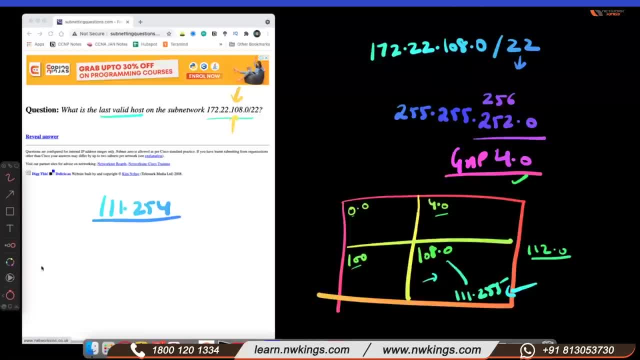 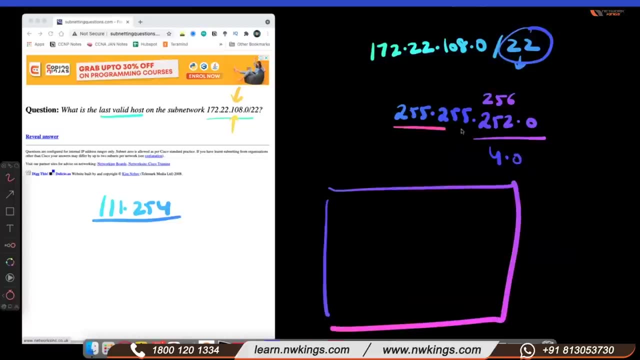 okay, let me calculate it for you again what i did. so i am going to just take out the subnet mask from slash 20 and i'm going to take out the subnet mask from slash 20 and i'm going to take out the subnet mask from slash 22. it is very easy: just get the gap 4.0 and i'll write my 255 is here, so it means my. 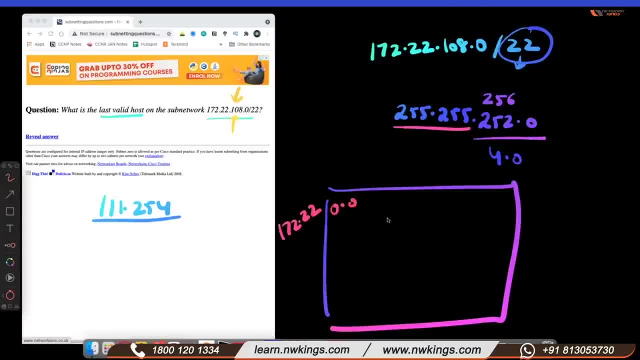 172, 22 will be outside, 0.0 will be inside right. so my gap is 4.0. so if i'll keep going to 4.0, 8.0, 40.0, so i'll come to one day for 100.0, 102.0, 104.0 and i'll come to 108.0. 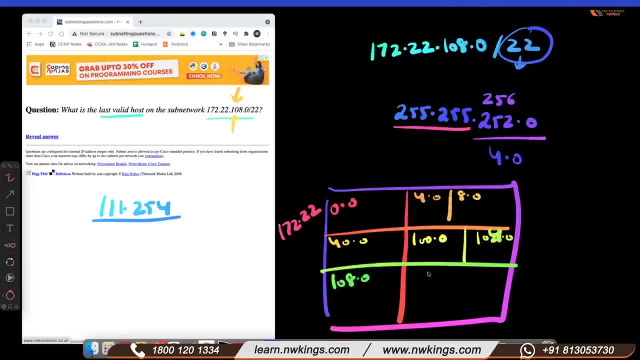 after few blocks and 108.0 and next is 112.0. so what is the question? what is the last valid host for this subnet? so this is my subnet, this is my before this ip i got my broadcast ip and before this ip. we call this last valid host. suppose if question is like first valid host, what would be? 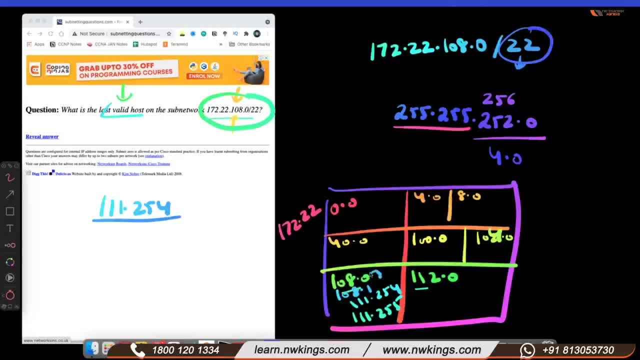 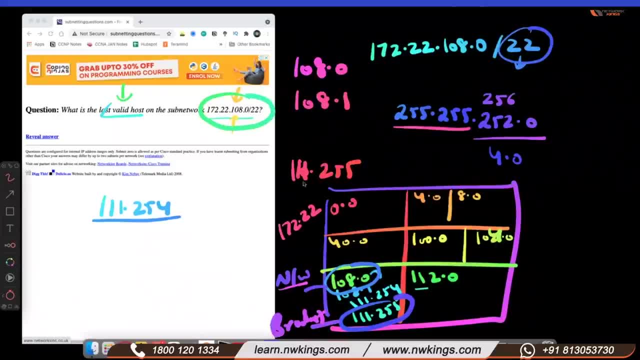 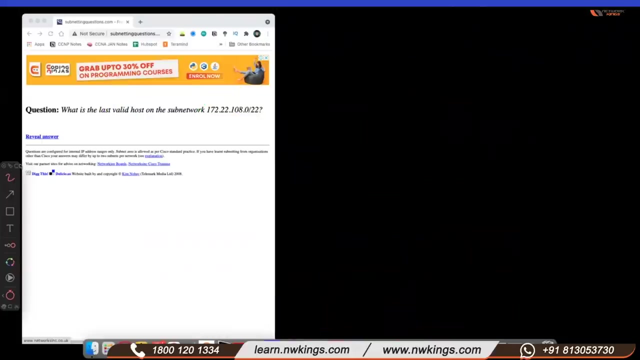 and this is your subnet mask. this is my subnet mask and before this ip, we call this last valid valid host, last host. this is first host and if some some questions are going to ask you range, valid host range and 108.12111254 is my valid host range. okay, don't worry, let's do another question and 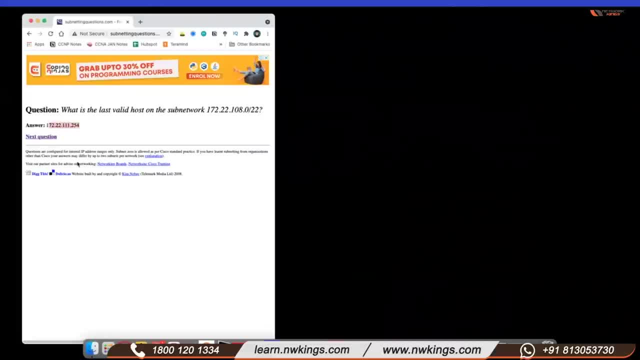 let's reveal the answer so you can see the answer is correct, yes or no? yes, right, let's go to another question. so now very simple question: 192.2, 192.2, 192, 168, 95, dot 128, slash, 27, right, yes, okay, so you can write down the value 255, 255, something. 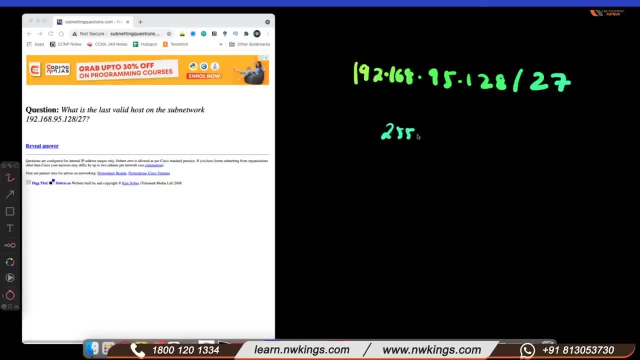 or you can just take out: uh, 255, 255, 255, 224, yes, right, 256 minus you will get 32. okay, so means only 3255, is there? it means your network id is 192, 168.95. start with 0, so we have to reach till. 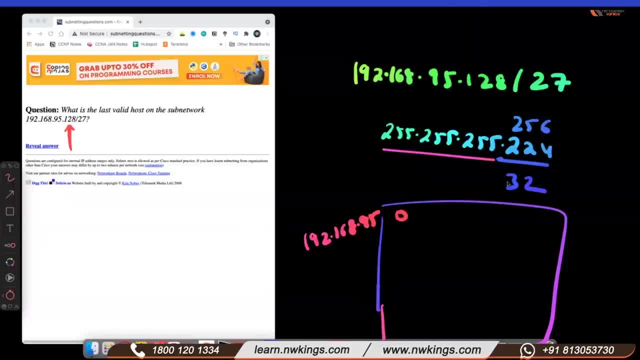 which ip 128. okay, so what is the gap? 32. so 32, you will go to 64, then go to 96, then 128, then you will go to 160. right, so before 160 you get 15.95, 255, yes, so what? i would be the last valid host before 150. and what is 954, 15, uh, 95, 159.55. 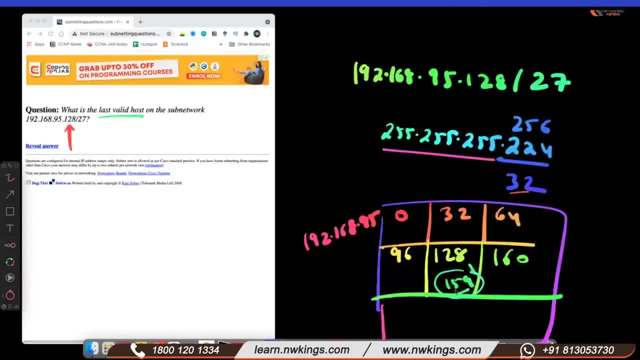 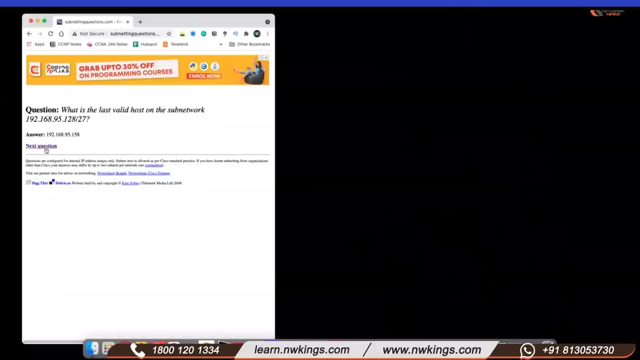 no, no, 158, 158. yeah, 159 is my broadcast ip, bro, 160 is my second block. yes, okay, okay, okay. so before is this 159 and before this, because last valid host is one ip before broadcast ip. so 158 would be answer yes or no. clear yes, yes, how much time we take only one. 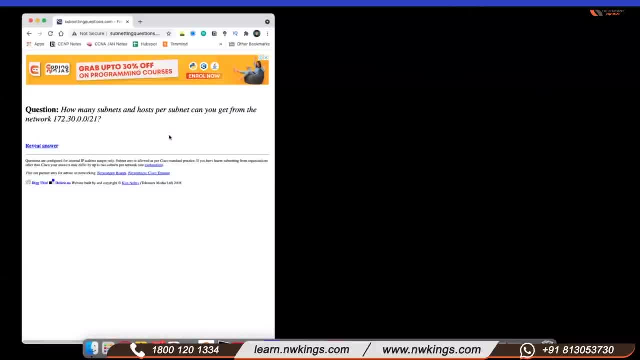 minute, right? so this is the question which is a little different. okay, so there are only two tricks, but to calculate that this is very simple, this is the most simple question. so this is class b, so you can write down network bits is 21 and remaining bit. 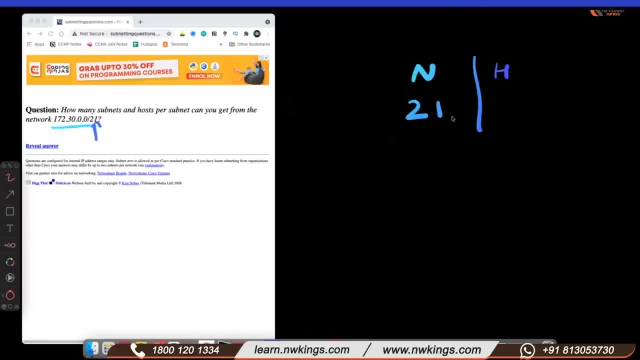 you can see, 21 is my network bit. remaining bits: 32 minus 21. 11, 11, 11 is my host. so now you can see: to the power of 11 is host. yes, so to the power of 11 comes 2048. so this is my host. but i'll subtract. 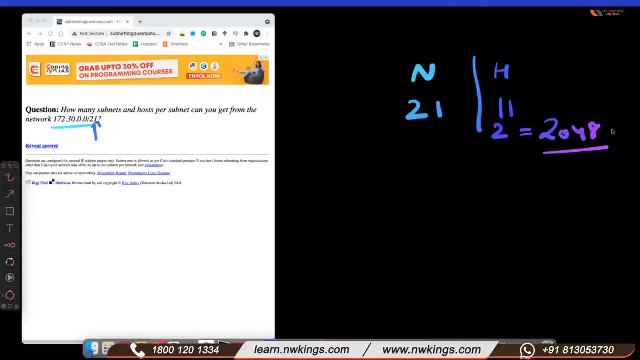 two. why? because, uh, i always network. one is network id, one is broadcast. so i'll take 2046 host. so i'll take 2046 host and tell me this ip belongs to which ip class b, b and b class by default value is 16, 16.. so how many extra bits added here? five, five to the power of five is. 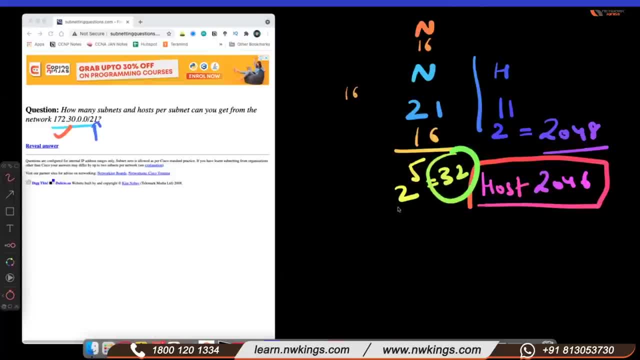 32.. so subnets will be 32. yes, okay, so in all the scenario the method will be same like this: yeah, but it is going to ask subnet and host, so you can see 32 subnet, 2046 host, even we don't take one. 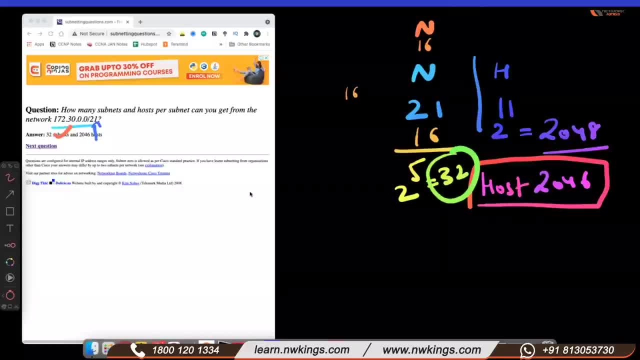 minute to solve this right. answer another question. uh, sometimes we are. there is a class cip or class aip and subnet. no worries, whatever is the whatever is your question right? so you are just going to identify what is the slice. let's do keep doing the questions. okay, you will get 10 also, don't worry. 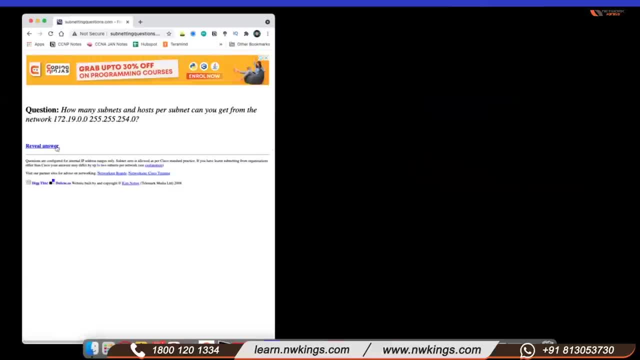 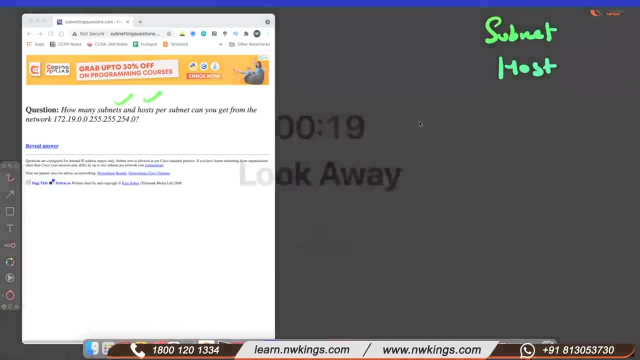 so this is c, let's ignore. let's take a or b. yeah, so this is which class. so remember, whenever subnet and host is asked, remember whenever subnet and host- so you have to write network and host part, the same, did what we did: network and host trick. okay, 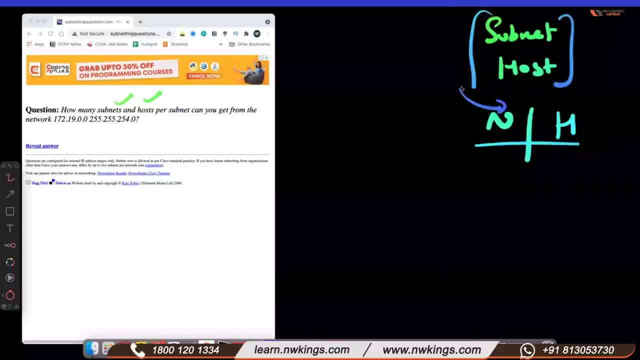 whenever subnet host is asked, you are going to do network and host part. but whenever host is asked or broadcast type is asked, last, uh, well, host is asked, okay. so whenever these type of question asked, you are going to minus the broadcast that, uh, subnet master. okay, so don't get confused. let 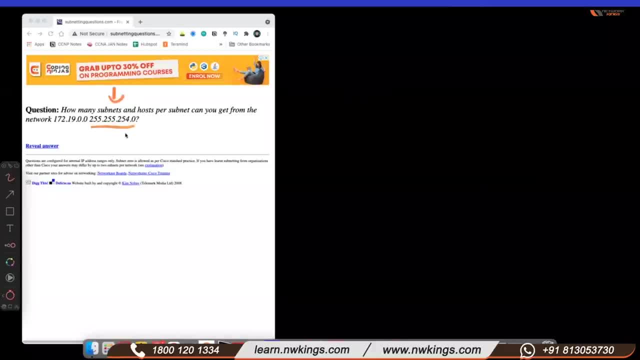 me do it for you so you can see subnet and host. now i want to make the slash value of this. this is opposite one. so tell me, if this is my subnet mask, what will be my slash value? 172, 19, 0.0. so this will be 8 plus 7, 15, yes or no? 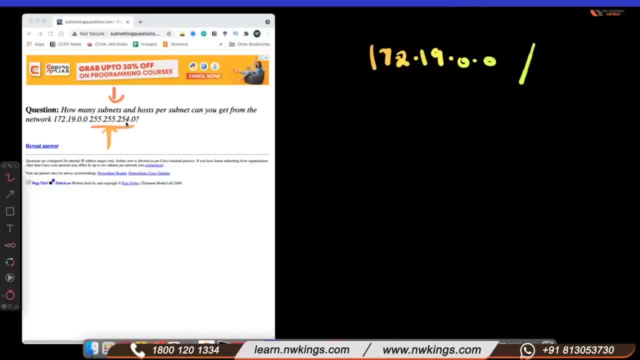 8, 8, 16, 16 plus 7. yes, correct, 23, right 23, 23, right. yes, so it means my network bits is 23 and the remaining 32 minus 23 is nine, nine, okay, so two. the power of nine is five one, two. 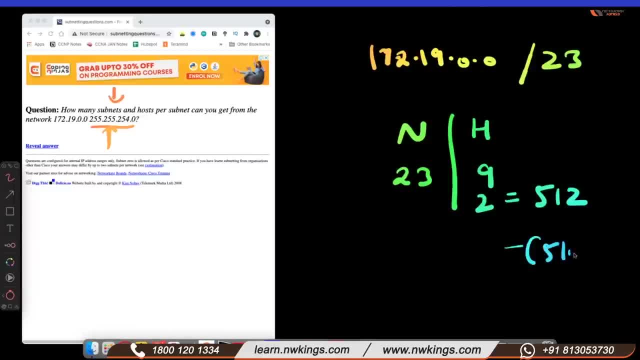 minus two is five one ten. yes, so five one ten. what host? host? okay, subnet says this is class b. so how many extra bits is added? let's say 16 minus 23. seven to the power of seven is 128.. so this is my subnet, this is my host. let's check boom. 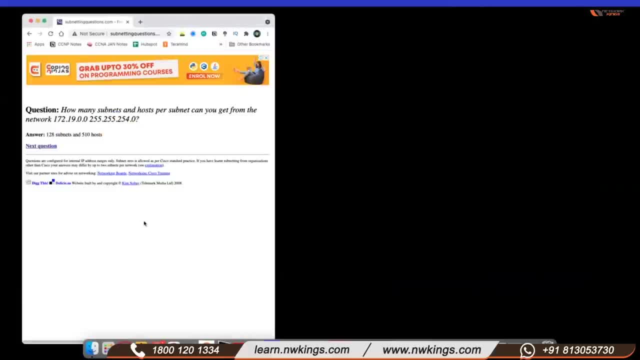 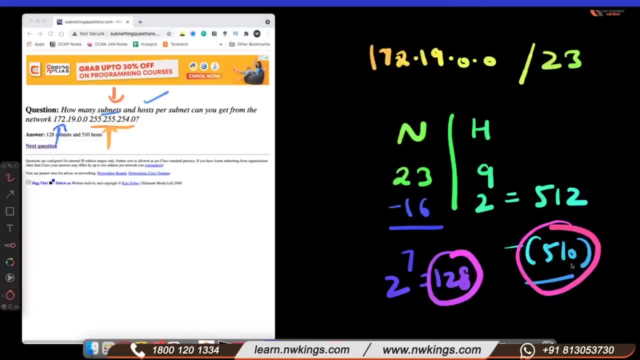 correct sir. hmm, sir, 510 means 510 is a valid host or total number of hosts: 5, 1, 10, 5. 510 is a valid host means you can assign 5- 10 ips, but you can't assign network bit and the last valid host broadcast ip. okay, 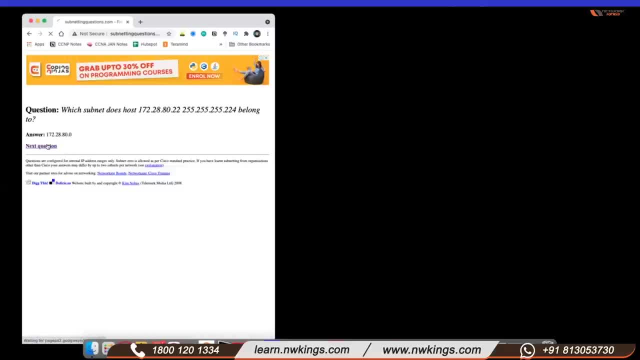 okay. so let's go further. this is very easy. let's do for a class. okay again, let's mix the question broadcast type. then we have to answer the broadcast ip. what is the trick? so whenever broadcast ip first valid, host all questions. you already just focus on subnet mask. 240 minus from 256, you get 16. right. you can write blocks 0, 16. 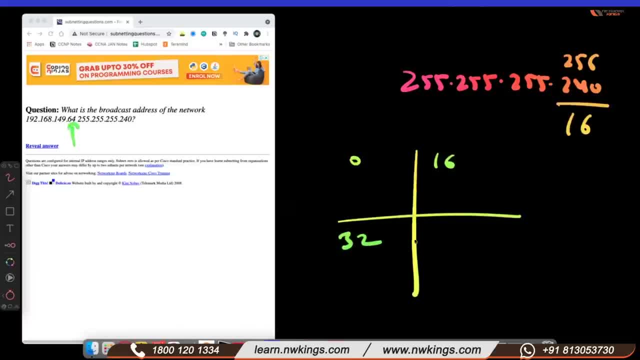 right, 32, until where we have to go till 64.. right, 48, and after that 64, yes, right, and after that what we have, 80.. okay, okay, yes, and before and broadcast ip will be 70: 79, yes, got it. yes, yes, sir. 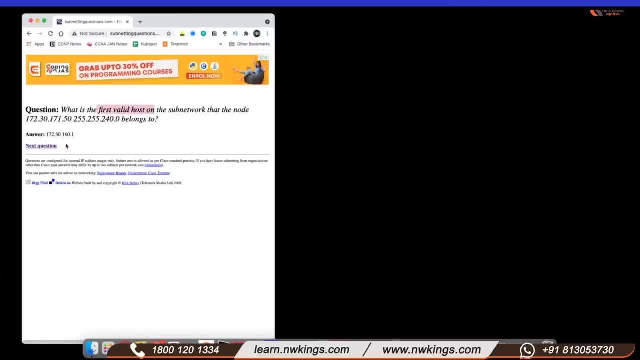 the again first valid host is the first ip after subnet. okay, so it's like 161. okay, so don't get confused when these type of big questions comes. it is nothing, just it is asking you something that this is the ip, 192, something you can note down: 192, 168, 216.0. so how many host? 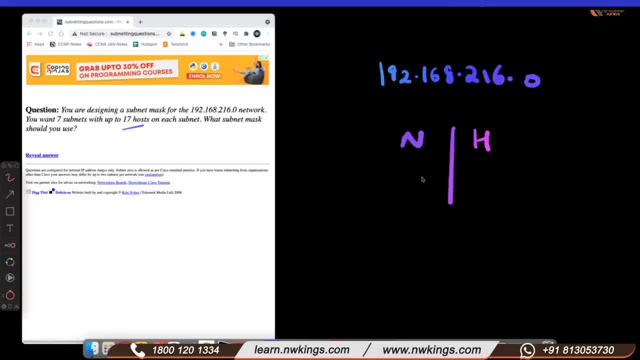 is required 17.. so you have to play a game where you only need 17 hosts. tell me what is the trick to the power of five is the power of five is 32.. 532 because to the power of 4 is 16. you can't take this group to the power of 5 is 32.. 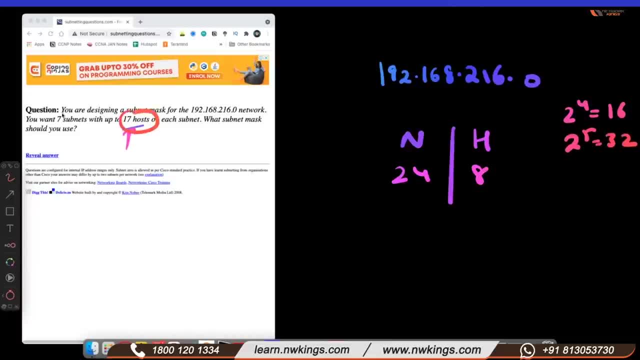 so i will focus on 32.. just take the host part, don't get, don't see the subnet automatically you will get the answer of subnet also. so just focus on subnet. and 8 minus 5 is 3, 3 will be added here. right, so you can see 27, but so when this ip 20 is 4, 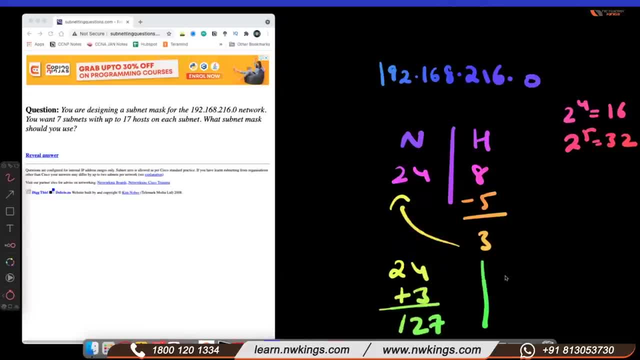 plus 3 is 27. okay, and here we have 5, right, so you can check. also, the 3 which is going this side to the power of 3 is 8, 8.. so i'm getting how many subnet more than 7, right? yes, so already. so the 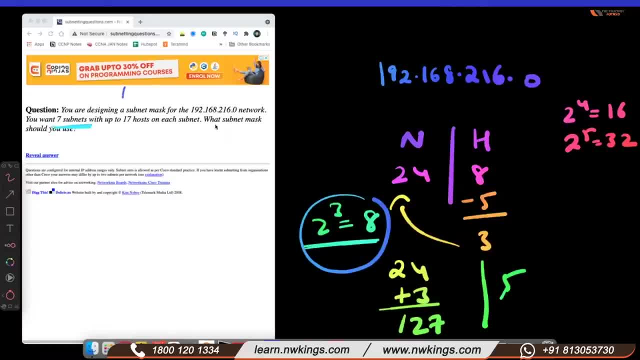 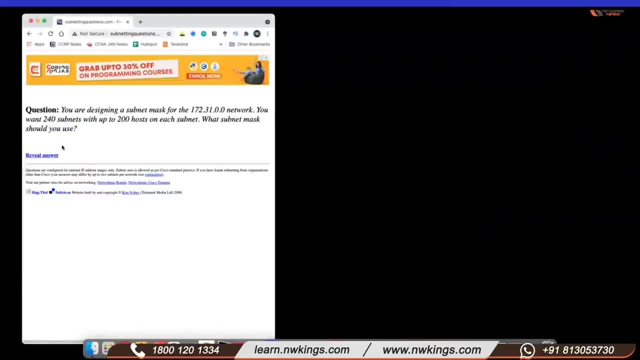 answer would be subnet mask you are designing. so it is asking: what subnet mask should you use? so tell me the subnet mask of 27.. two to four? yes, so the answer would be two to four. so let's do one another. so 172 ip 172, 31.0.0. so network bits is 16, host is 16 in class b. yes, so. 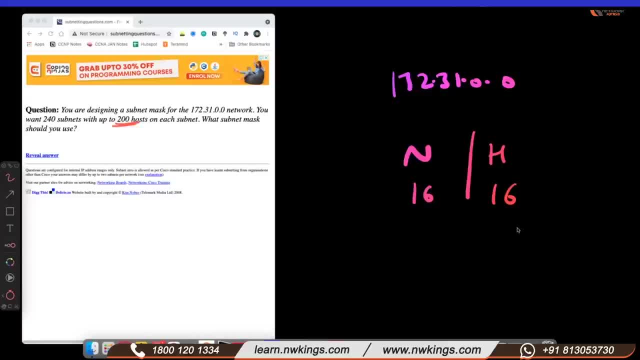 how many hosts? i need 200, so 200 k is 256.. yes, so i need only eight, so that eight will be added here, that becomes 24.. so don't get confused. the ip is c. okay, so this is by default of c, but it can be of b also. 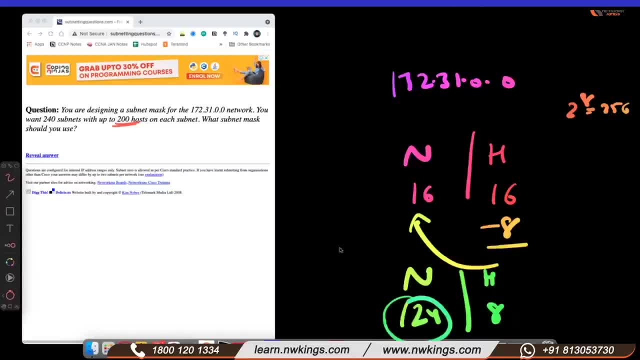 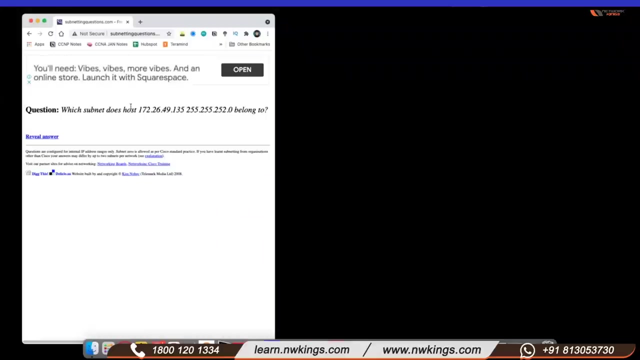 host is eight, right, so the subnet mask will be two, five five, two, five, five, two, five, five, zero. yes, right, yes, sir, hello, sir, repeat this. okay. so you're going bit fast, salian, because i want you to practice fast. don't worry if you don't understand one or 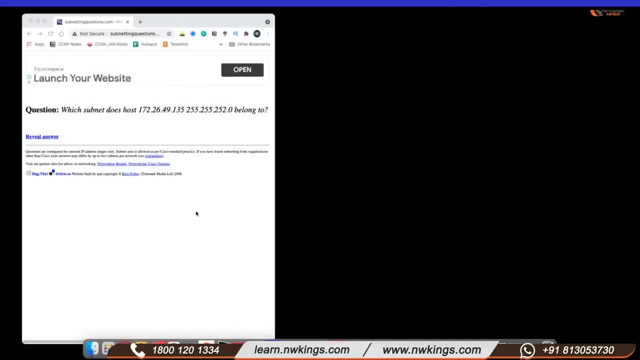 another question. keep checking the another one and class is getting recorded also. and don't worry, i'm not in a hurry to close the class, even i'll sit for 11.. but i'm just making you practice that you should do this questions very fast, okay? this is why i'm 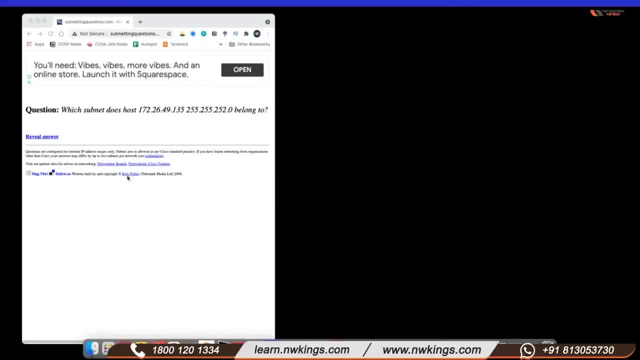 going fast, okay, okay, so you can check. okay, let's do in slow pace also. so which subnet does host? which is subnet means you have to calculate the 255, 255, 252.0. so i'm going to subtract, right, kalyan. so this comes. what is this what we call this? yes, sir. 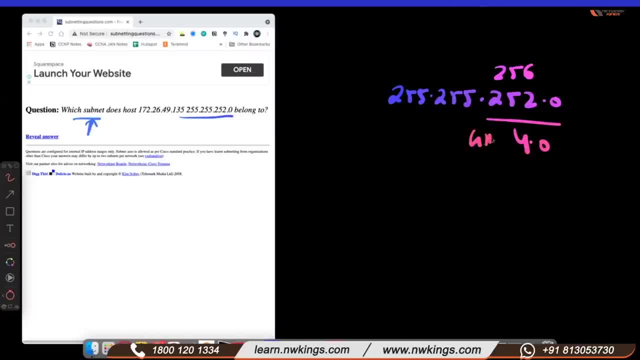 is call this gap. yeah, yeah, yep, i'll write 255. it means 0.0 will be inside 4.0. so till where we have to go till 49, 9. yeah, i am checking third block because only two, two, five, five is here, so change will happen in third block. okay, so 4.0, 4.0 will come a 40. 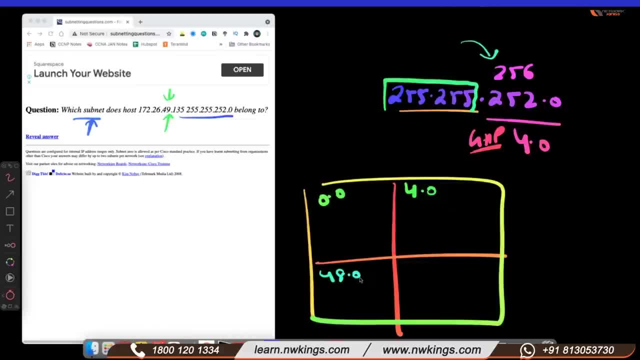 44, 48.0. yes, yes, you keep going. 48.0, 52.0, yes, so what comes before 52.0. 51.255. so this ip belongs to which subnet this block? yeah, so which subnet? so this? my network id is called subnet, so answer. 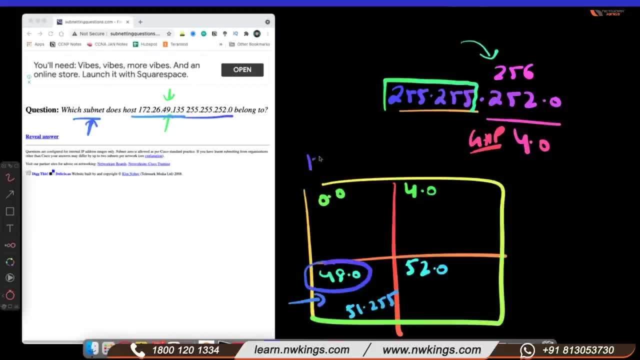 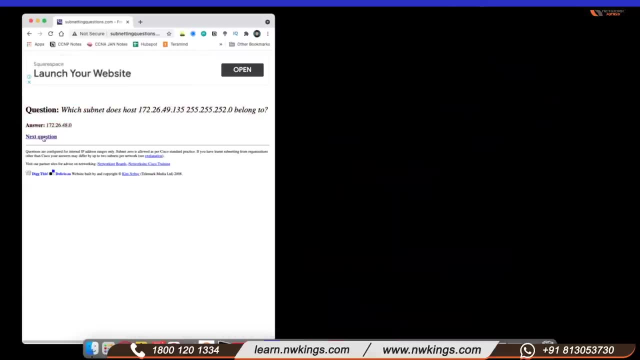 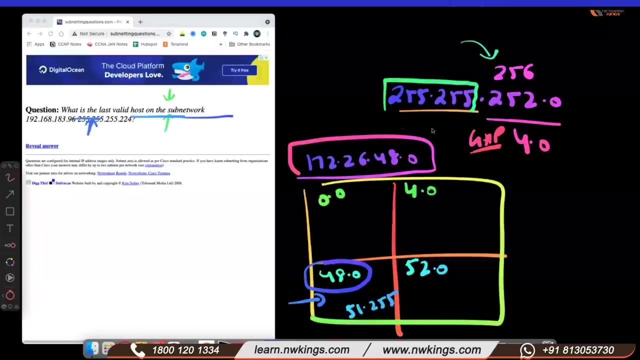 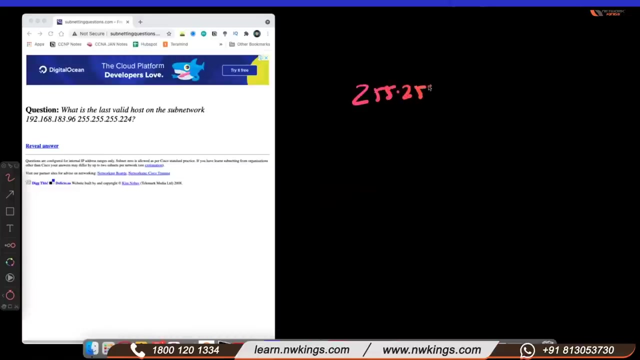 would be 172.26.48.0. clear, yes, so let's check clear. yeah, okay, let's do another one. so last valid host. okay, very simple. so what you have to do, you will write the subnet mask: 256 minus 2 to 4. what you will get: 30, 32.. so 3255. it means only single zero inside, right. 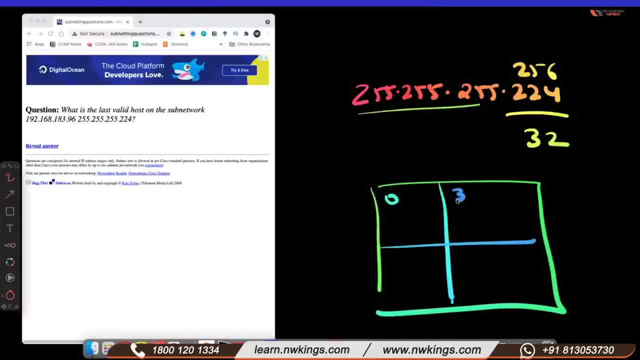 yes, 0, 32, okay, till where we have to check 96, right, because 3255 is there. change will happen in fourth block: 32, 6, 64, 96 and then 128, before 128, 127. so what is the question last? will it do tell me what last? 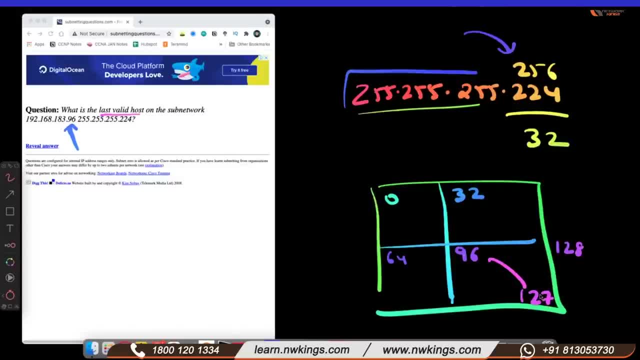 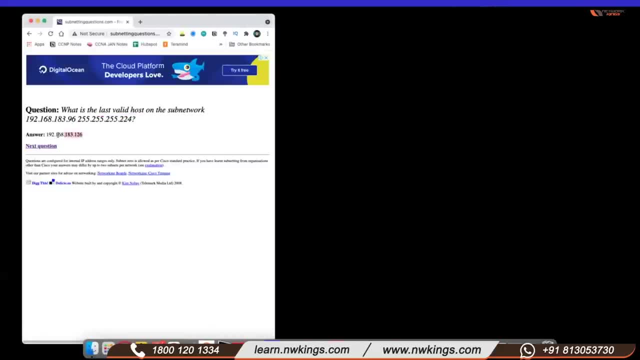 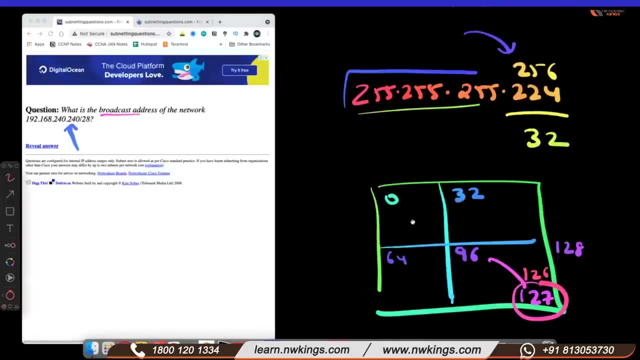 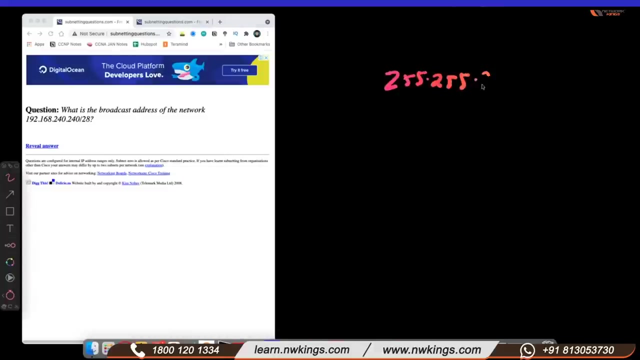 will it host kalyan 127? no, this is broadcast 126. okay, okay, got it. yes, sir, got it. let's go do another one. very simple, so just we need to figure out what subnet mask, 28 subnet mask, what will be the subnet mask? 255, 255, 255. 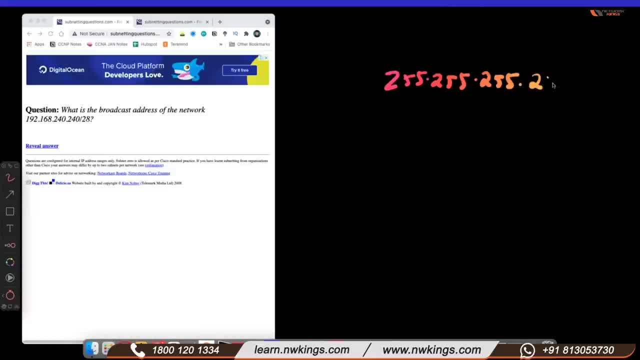 29. okay, sorry, 240. right, yes, sir, 256 minus 40, 16, 16.. three blocks outside, zero, single inside, guess 100 out. so till where we have to reach, it's little difficult, let's just jump directly: 16, 16. so 10th block will be 160.. yeah, okay, 160 plus 80, it means, uh, we will have 240 also, right. 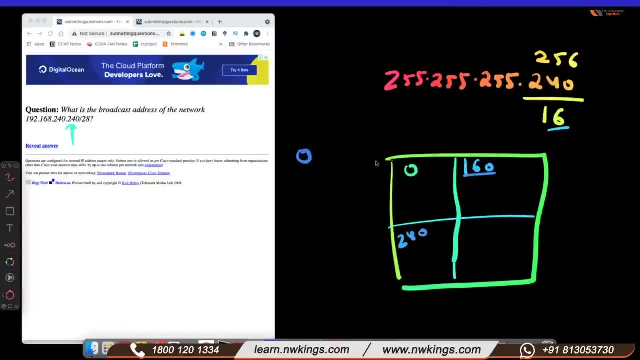 because if we can reach 0, obviously 16, 580, 16, 10, 160 and 16, 15 is a 240. now, when we get 20, 60 for our block code, we do exactly the same thing. guys that don't know if you understand what I'm telling you. guys, I give 50 and 90, 40, 20s, 60, 60, 60, 10, 60 and 16, 15, 80 is a 240. right, because if we can reach 0, obviously 605, 80, 16, 1, 60, 60 and 1615 is a 240. two. so that means 20, 60, which gives us less. I get 60 or 40, 60, 10, and then we raise protests which we will change to 8. emotion. you work out on direction of eating quiuqai, or right? so we so lucky to complete st G1. so that means, if this was only 16, isn't that participants, only receiver, we are. 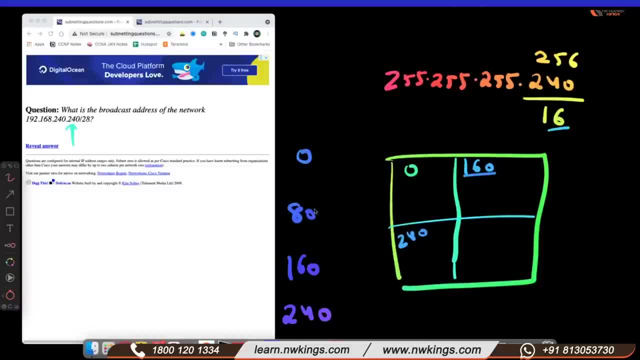 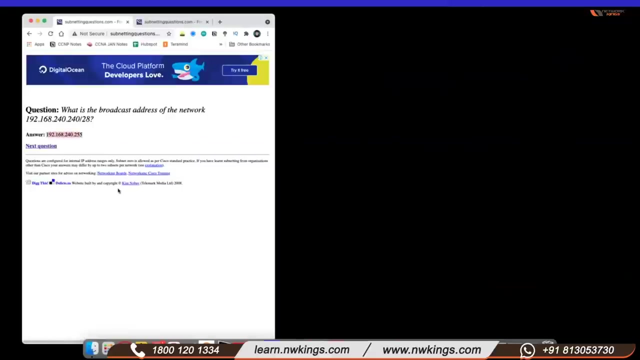 is it 240? yes, sir, right, just i added five bit, five extra 240.. so we have to reach 240 and 240 plus 16.. obviously it will go to 55. so it is asking broadcast ip: what will be the broadcast ip? 250, 255, yes, okay, got it. yes, okay. so these questions are actually important and again, i'm 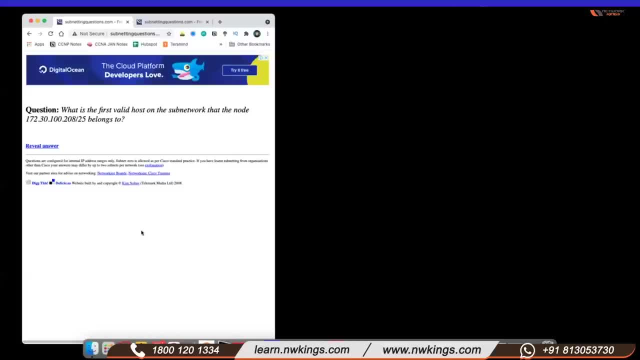 telling you exam, but it mean this session or this workshop i have taken so that you will understand the subnetting in and out, not just the submitting part. okay, like we, how we do submitting, how to do vlsm. so i hope you guys now got confidence. so what is the first valid host? again, very simple. 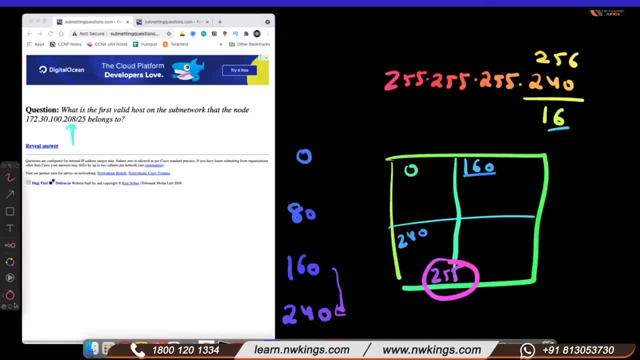 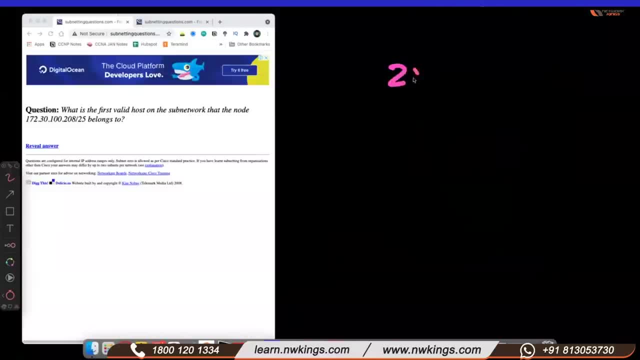 you are going to write the slash 25 subnet mask. what will be that? 128, yes, 255, 255, 255, 128. you will minus 255. what you will get? 120, okay, 156, minus, sorry, 256, 128, 128, right. so starting with zero, right, and we have to reach till 208. 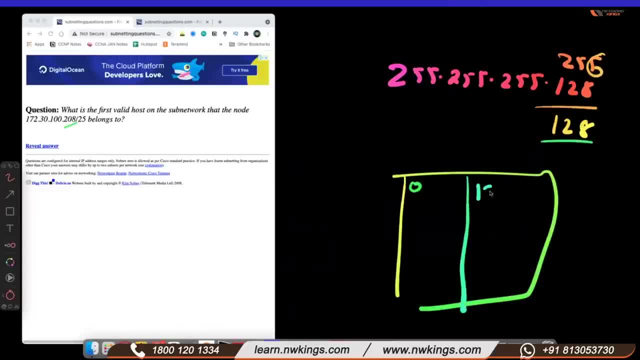 obviously the block is 128. only two blocks, right, yeah, so before 127. the ip208 will lies in this. so it is asking: first, valid host of this group. tell me what is that? this is my network id: 129, 129. the second ip is called first valid host and the answer would be 129. clear, yeah, yes, okay now. 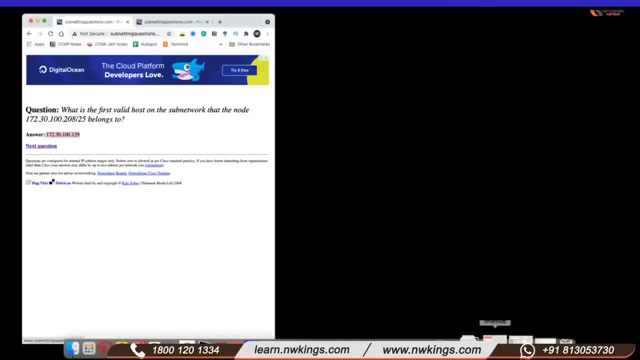 let's uh check who will be actually answering this question. okay, i'll take one by one name: sujit, tell me how to resolve this question. what is the first valid host on this network let me write, so tell me what is the first thing i'll do, sujit. 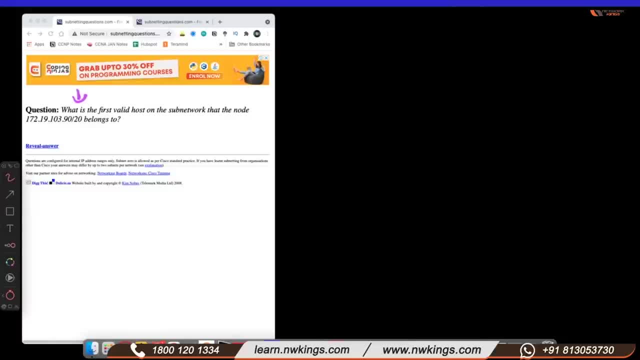 hello, are you there? see you guys, you have to participate. if you want to learn sujit, i don't know? kunal inside github, uh, it will save it. so how about? how about? we'll put stack, stack, stack, 256. i'll get 16.0, what we call this, yeah, yeah, and two, two, five, five. it means two things will. 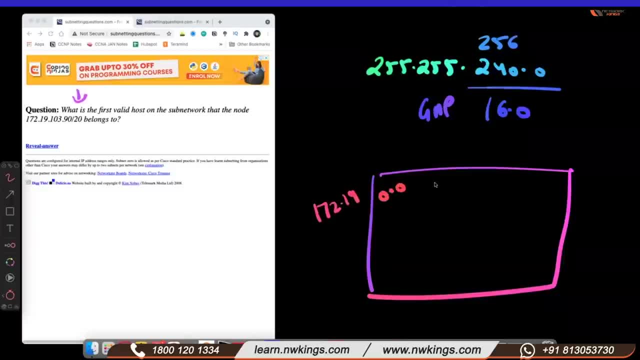 be outside, which is called network, and zero dot. zero will be out inside. right, because i got two groups. the change will happen in third block, right? yes, sir, so the ip. we have to check one zero three and the gap is 16. so i'll keep going and going, so i'll go till 96, 16 into 580, 103. yeah, so 96.0. 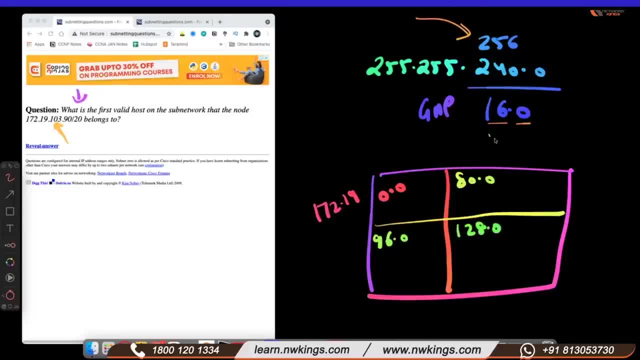 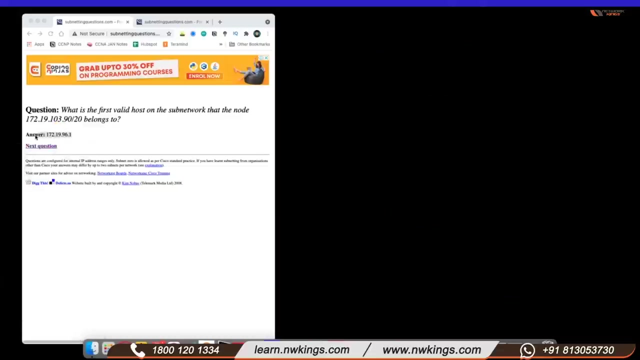 and i'll go till 128.0. so these will be my block with the 16 tables right. so 128 is 127.255. so the first valid host will be ip after this 97.. 96, oh sorry, 96.1, cool. 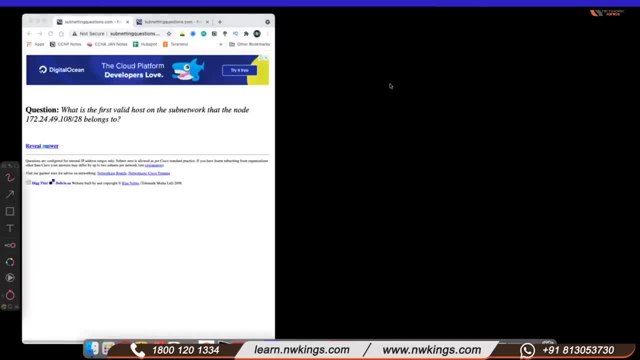 okay, tell me what to do. uh, so 28, remember 28, 28, so it's 8 plus 8 plus 8 plus 4.. so tell me how many? two, five, five. two, two, two, twenty four. so we will have three, two, five, five now, because it's twenty four. 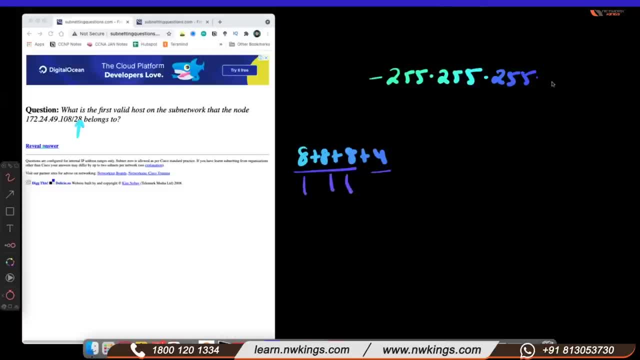 plus four. so three, two, five, five, twenty four, two, two, two, four, two, four, two, four, zero two. fifty six minus forty sixteen. so the change will happen in which block three blocks completed. the change will happen only on second. uh, last block, right, yes, sir, 49. so i'll write zero here until where we have to reach one zero eight and the yeah, sixteen, eighty. 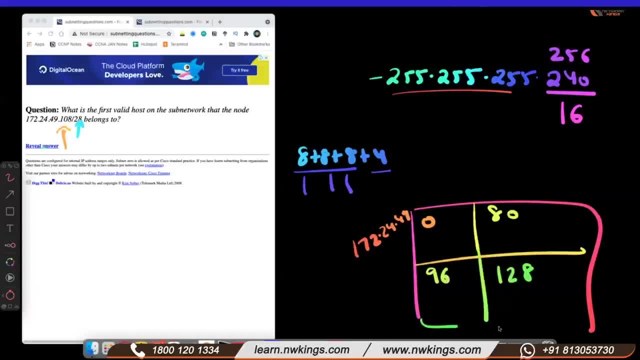 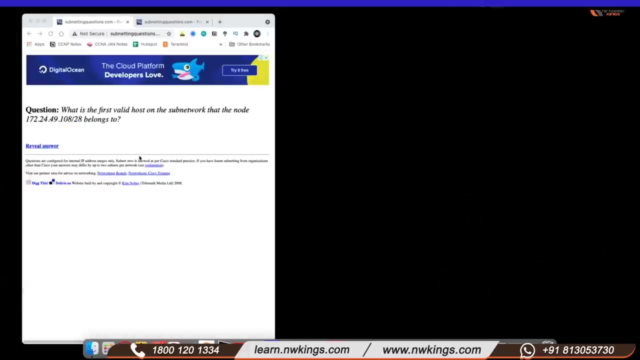 96.128 before 128, 127. what is the first valid host? 90, 7, yes, 97. this is not gap, ok, so this is not 96.1. so it's 97 after 96, 97. so the answer would be 97. 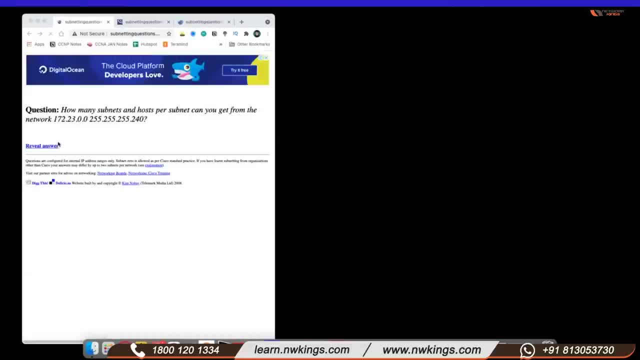 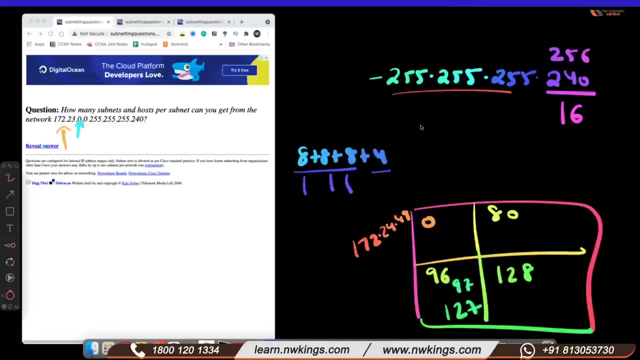 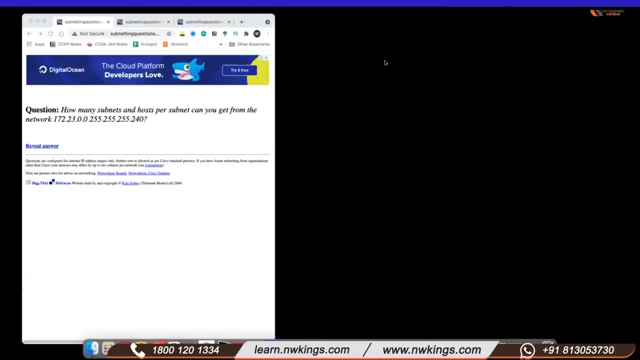 ok, please revise your subnet mask trick. how to get the subnet mask correctly? yes, dushyant, yes, sir, yeah, tell me how we are going to resolve this so you can note down: 888. so network bits will be. we have to whenever we get subnet and host. 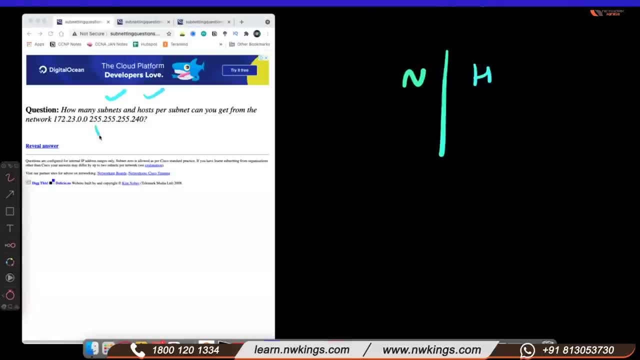 we have to write this right, ok, so 3255 means 2424 plus 28 and the remaining host 32 minus 28 is 4. so to the power of 4 is 16 minus 2. is how many host 14? ok, 14, and this is class. 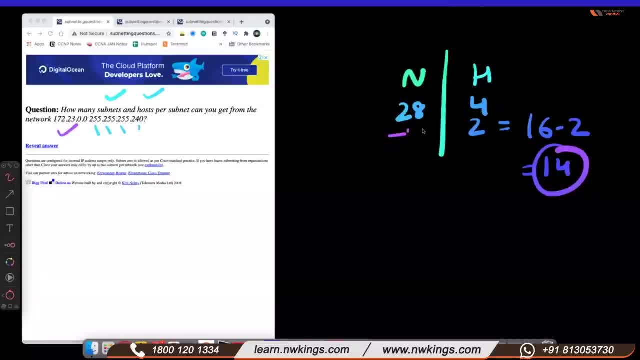 B. this is class B, so I am going to minus the 16. ok, I am going to get 12, right? yeah, so to the power of 12 is 4096. yeah, so 4096 subnet and each subnet will have 14 IPs, right, yes? 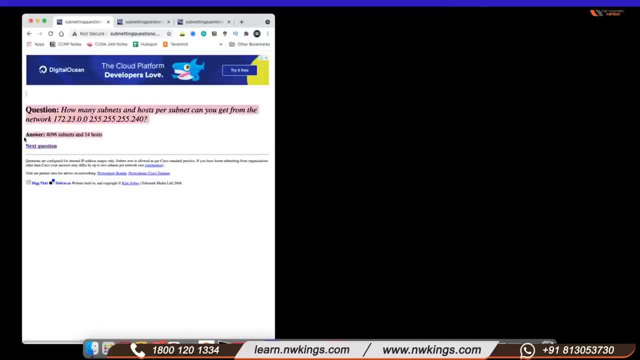 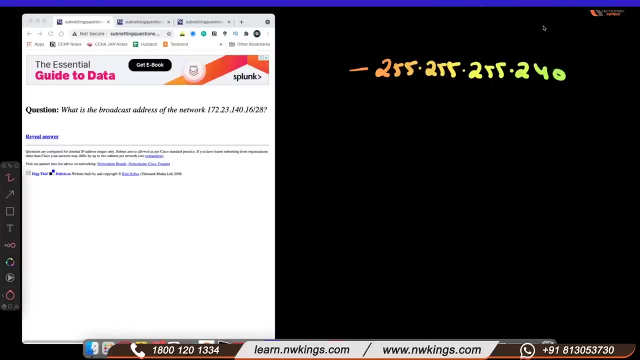 see. ok, so tell me the broadcast IPs. anil kumar reddy. yes, sir, broadcast address of network. so the trick is different. we need to calculate the subnet mask. yes, again, that same subnet mask is coming again and again. right, so again, 16. yeah, 0 to. 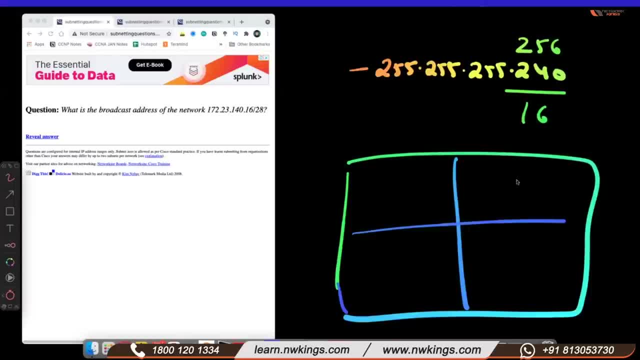 even if you don't remember the table of 16, once you are going to do some editing you will remember: yeah, 16, 32, so we have to go till where 16, right, so we don't have to go further. so before 64- sorry, before 32, 31 and before 16: 15. 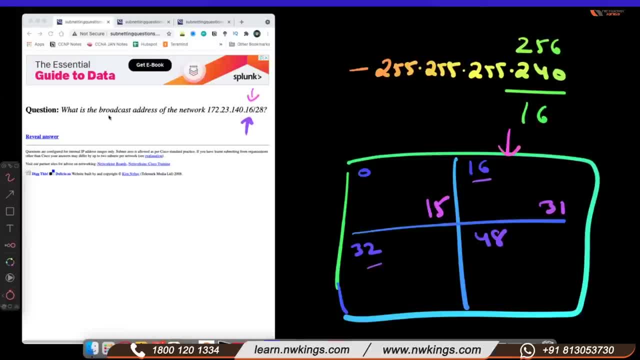 so 16 IP belong to this group and it is asking what last broadcaster to? so what is the IP? this is the last broadcast will be 31? yes, correct, remember this is my network ID. this is my broadcast. 17 will be first valid host. 30 will be last valid host. 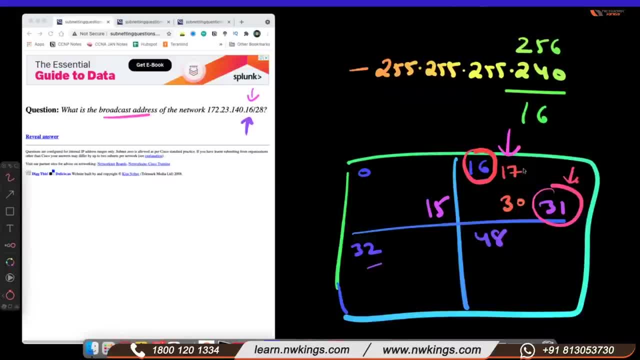 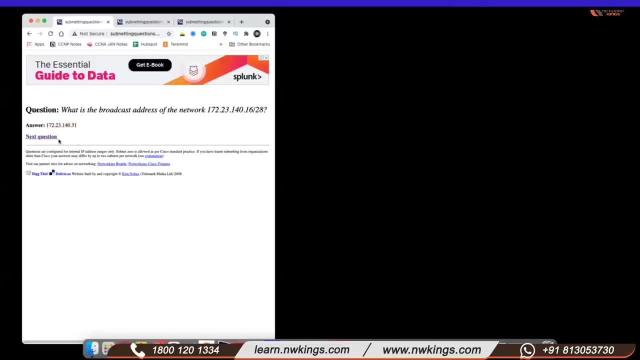 last, ok, and if some question is asking you range, range is 17 to 30. yeah, so let's check 31, correct, 31, correct, yeah, correct. so that question is again that different one: network and host part. so slash will is already given. network is 20. 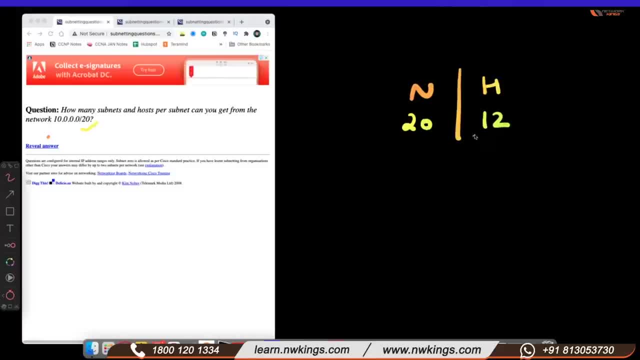 and the remaining host will be 12, so to the power of 12 is 4096 minus 2, 4094. ok, and network: this is class A minus 8 minus 8, and we are going to get 12- 4096, so 4096 subnet. 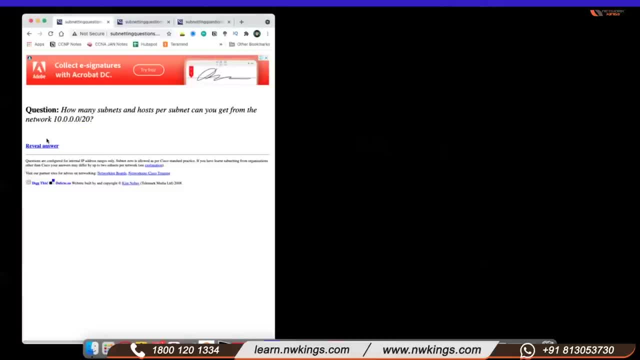 yes, how cool. someone took my photo. guys, tell me, are you feeling like you are actually learning subnetting now? you know the tricks. yes, yes, sir, yes, sir, yes, sir. those who are my student, they already know these tricks most of them, but the guys who are just came for subnetting. 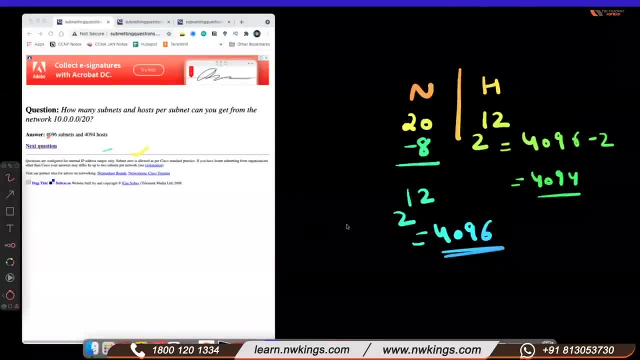 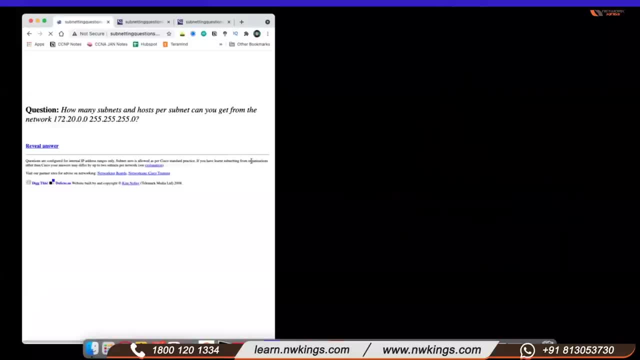 ok, so now you can see we are not able to. so every time we are getting random question and every time our answers are correct. so how many subnets? again, this is class C, B, B. see, we always do mistakes in small things. so this is B, so 255. this is slash 24, right, 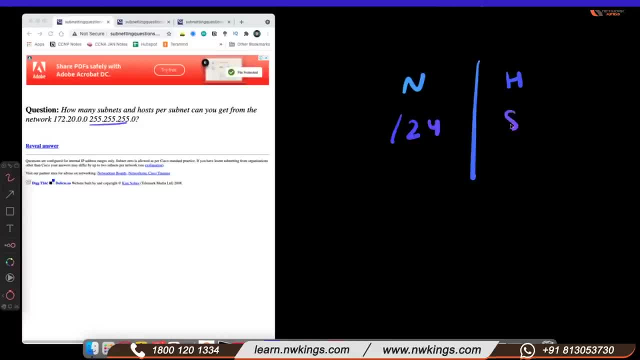 right, yes, sir, and host is 8. yes, so to the power of 8 is 256. minus 2 is 254, 254, host, 254, host, and this is class B, so I am going to minus 16 to the power of 8 is: 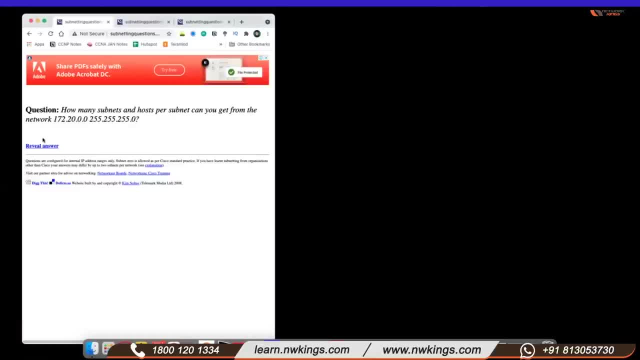 256, 256 subnets got it. yes, sir. so which subnet does host 172 belong? again the simple question: you have to calculate the 240.0 right? yes, whenever you see subnet first valid host broadcast just within a one minute, write the subnet mask and minus the. 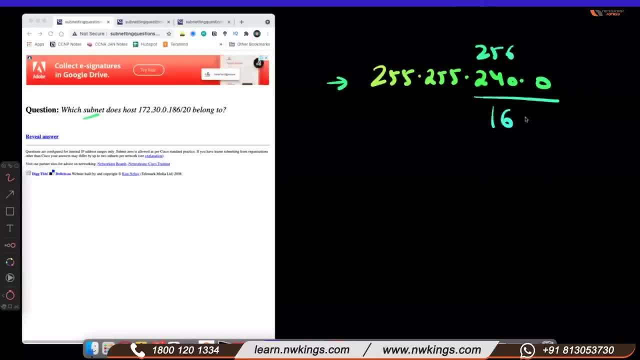 value which is not 255. you get what? 16.0 gap, right, yes or no? yes, yes, so ip start from 0.0 and it will be 16.0, and it will be 16.0, right, and it will keep going till. okay, we don't have to go further, it is 0.1. 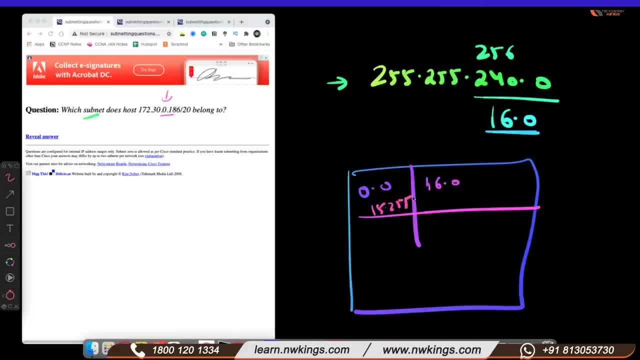 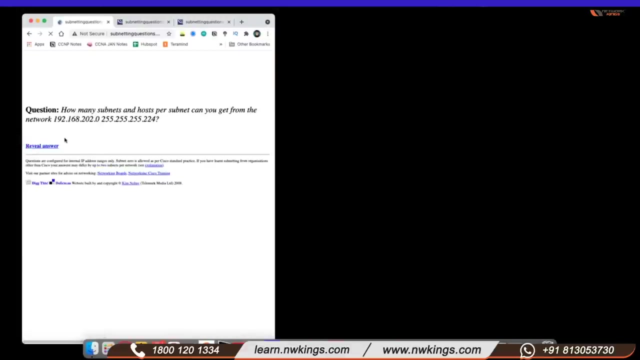 so 15.255. so subnet will 0. subnet is the first ip is known as subnet or network id. we call this network id and we call this the first subnet also. so the answer would be 0.0, right? 0.0, yeah, okay, how many subnets? 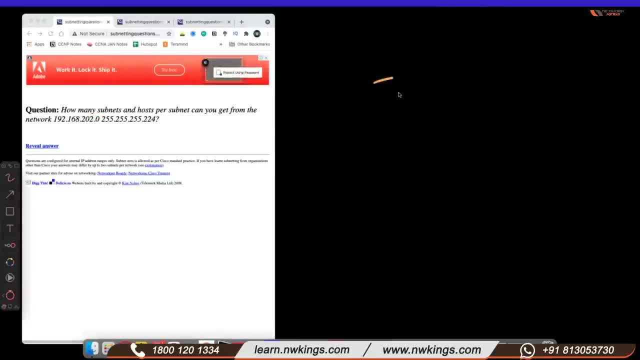 again. i'm feeling bored now because every time we are getting same question: 255, 24 plus 3, 27, the remaining 5 will be host, 30, 30 host. and which ipc 24 minus 3, 8 is subnet right, got it yes. 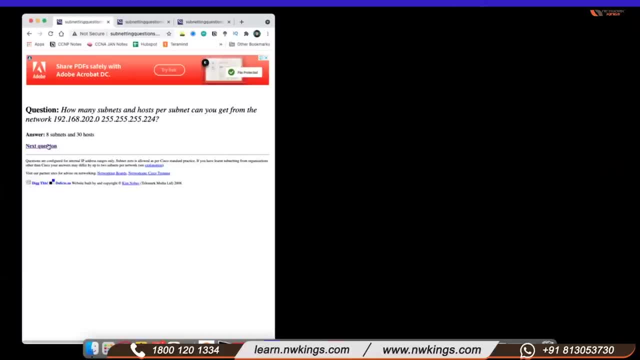 yes, sir. now you guys can see the speed is getting in, got increased and you are doing these questions in 10 seconds, right? yes, sir? so 255, 25, you can do this- 256 minus 254, 2.0, right, yes, sir? so start with 0.0 2.0. 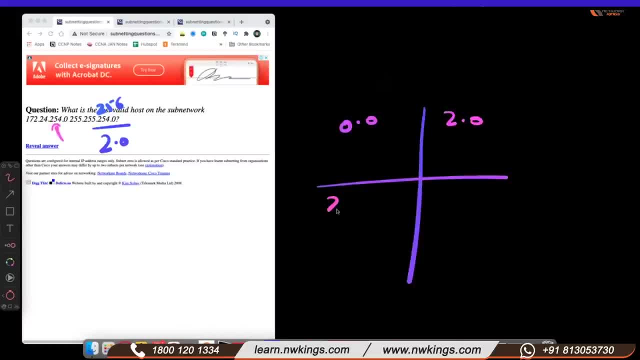 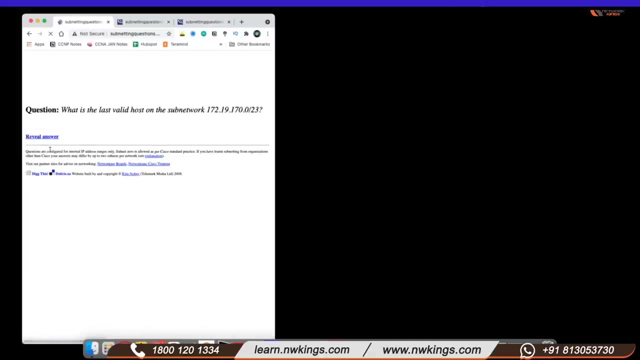 and till where we have to go: 254. obviously we will be going till 254 and maximum would be 255- 255. so it is asking the last ip. so tell me what is the last ip before this? 255, 254, yes, yes, right, yes, sir. 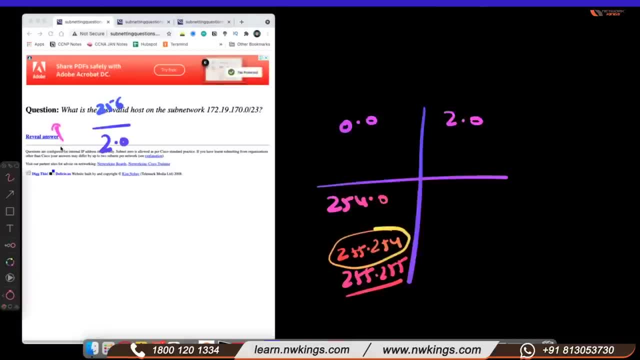 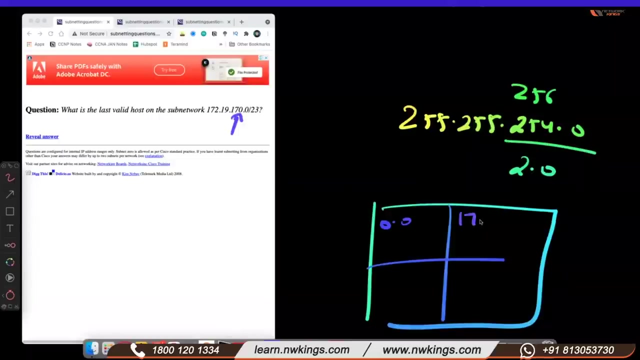 okay, so last valid host: 255, 255, 2, 16 plus 254.0, 256, so you will get the gap 2.0 right, right 0.0, and till where you have to go till 170. obviously that is divisible so that we can divide right 170.0, 172.0. 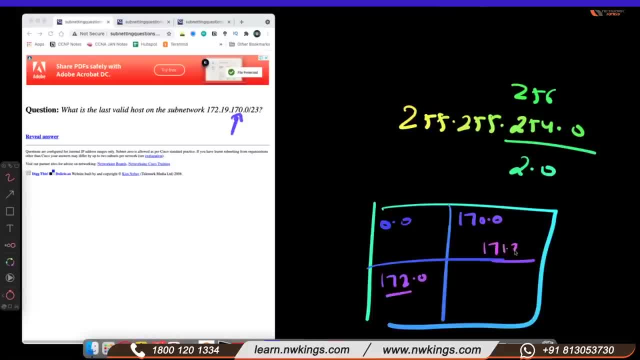 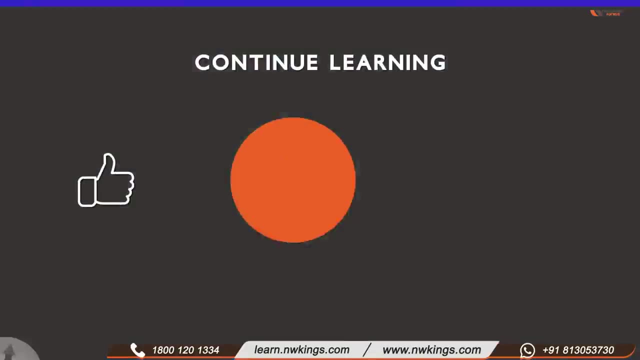 so before 170 to 170, 1.255 and the last valid host is 254, so 171 254 is your last valid host. okay, guys. yes, sir, hi, you are watching the recording from one of our live session. hit like share and subscribe for more future updates. 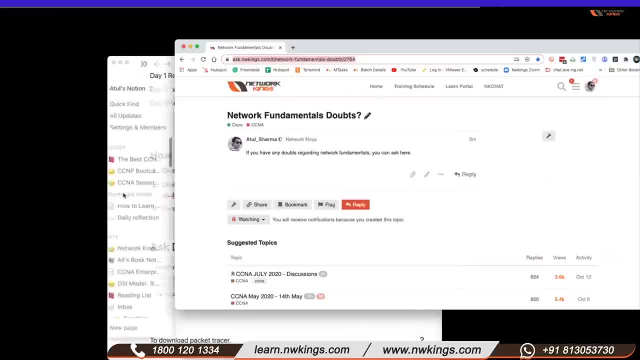 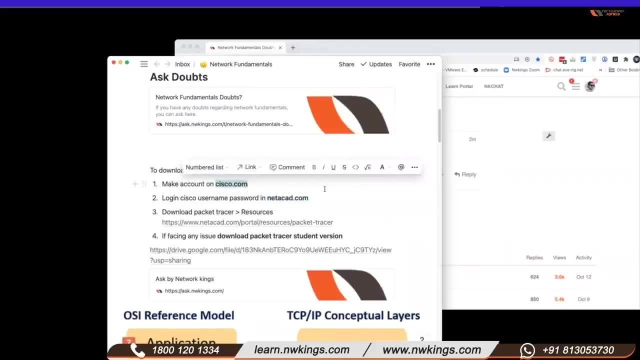 okay. so the second thing. now i am going to show you how to download packet tracer, which is a free software by sesco. so first you need to make a account on sesco, which is very simple: just go and make it so once you create your account. 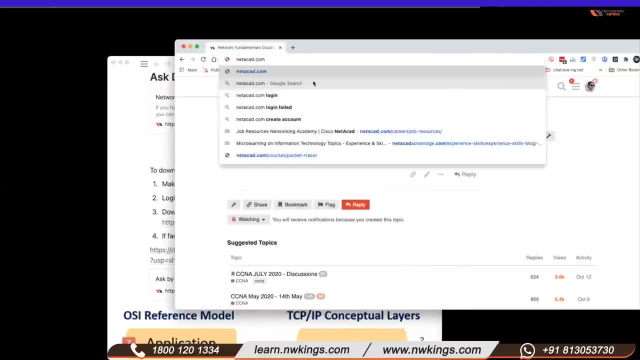 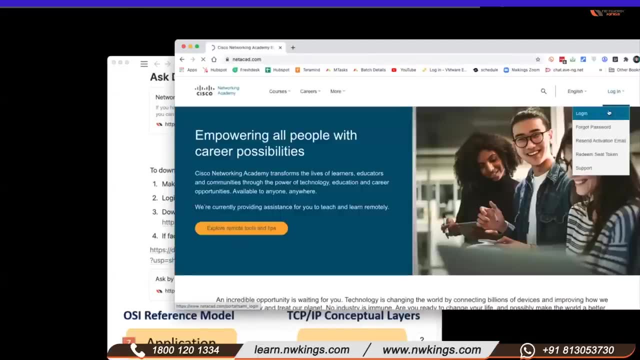 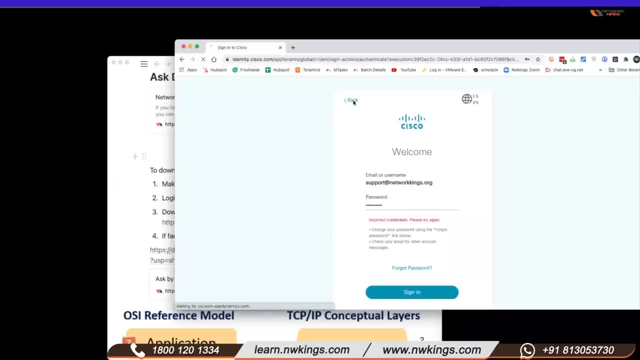 then go to another website that is netacad, that is network academy. okay, so in network academy you need to login with your sesco username password. so i have my email address network academy link. i told you that i have shared the whole notes with you, right, everything is mentioned on those notes. 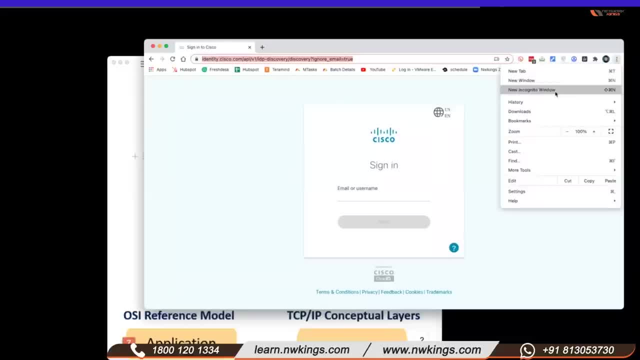 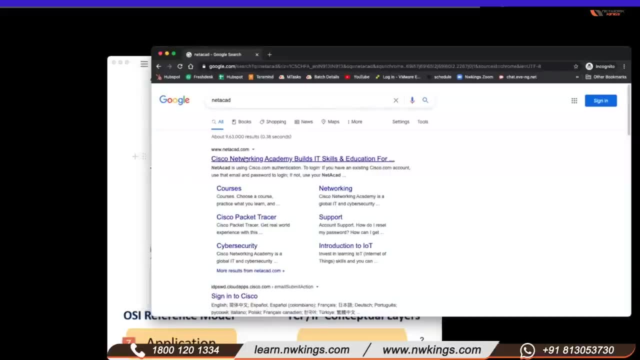 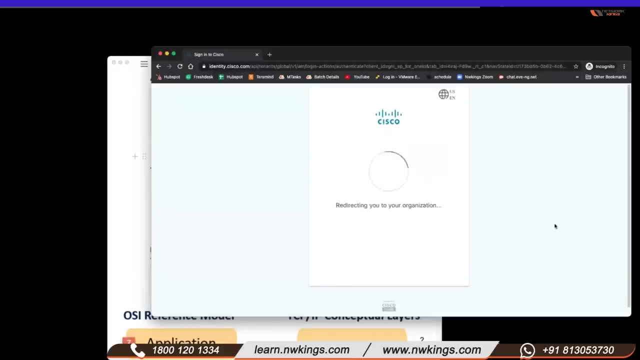 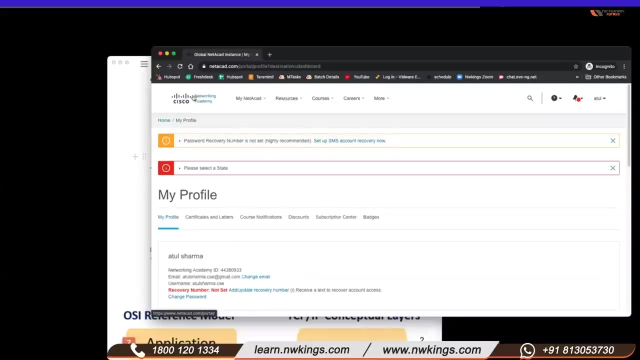 just check once again in your chat. just hold on. yeah, so go to netacademy. login with your sesco username password. okay, see now. yeah, so you can see once you login into this network academy. there is on the right side of the screen. there is on the resources section. 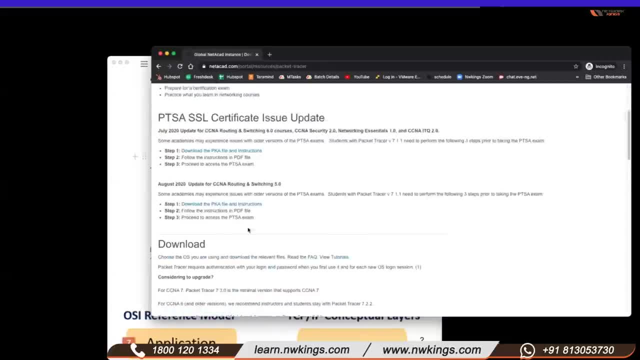 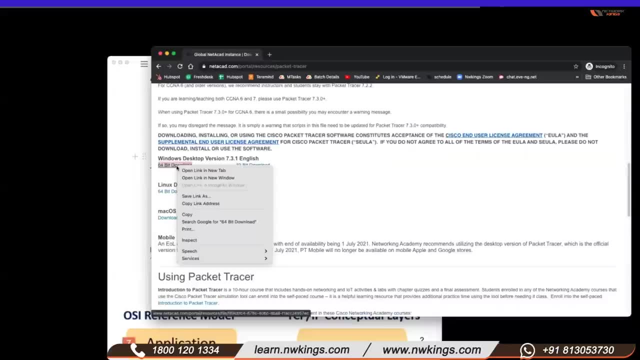 so you can see download packet tracer. okay, so once you download this so you can see here windows desktop version and linux or mac os. so even i can share the direct link of packet tracer and all from here also. but the problem with that this link is that you still need to create account. 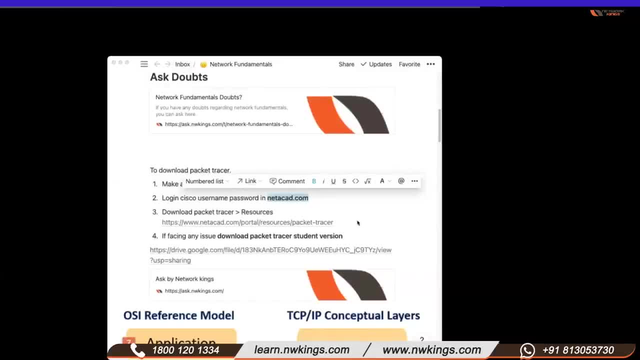 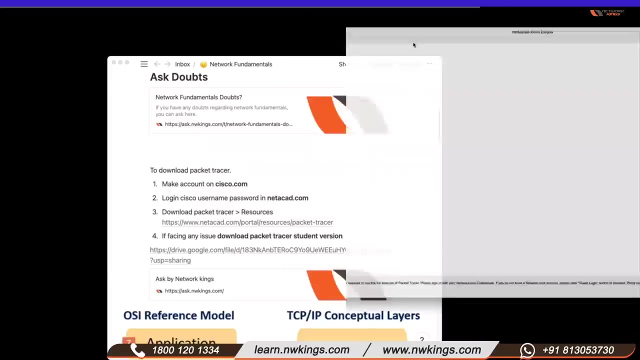 okay. so, even if i am going to add a direct link here, even i already shared this right, but you still you need to create the sesco account, because in packet tracer nowadays you can't login without entering your sesco id. okay, so i'll show you just a quick overview of this software also. 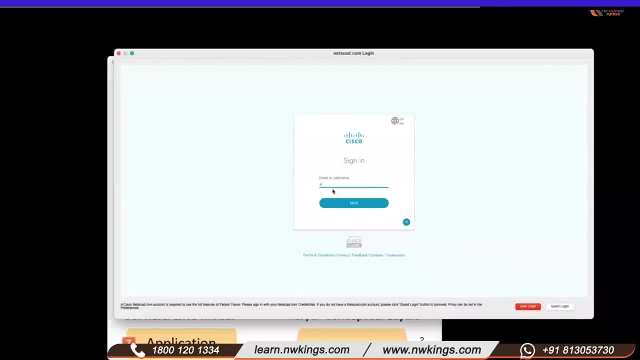 so it's asking me to login again. i have to type the same id which i was typing there, okay, and the same password which you created for sesco id, okay. this is a little annoying every time you have to login into the software, but it's okay. 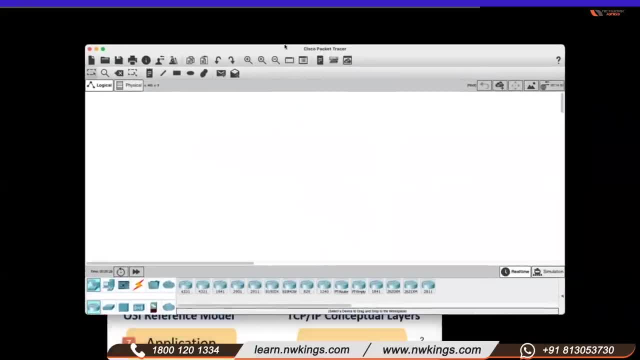 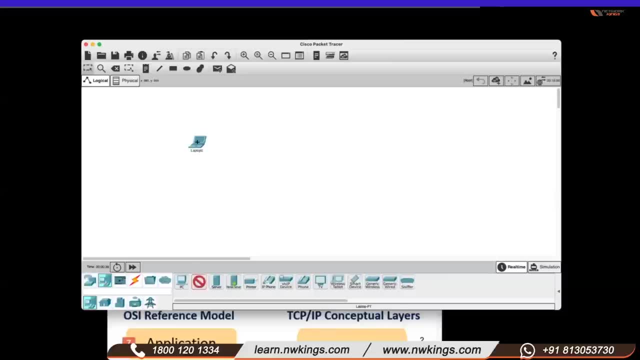 yeah, so my software is ready. so this is the software which is known as sesco packet tracer, and if you want to do the lab, you can just create or add a lot of devices, multiple devices, okay, and here you can create the switch. you can add a cable from here. 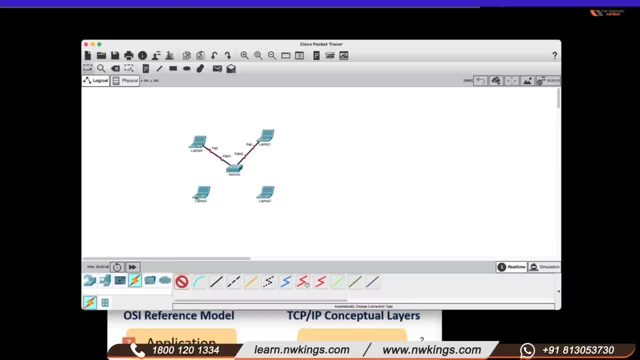 okay, so you can also do the same commands. you can type the commands of switch also just by clicking here: cli. so here is the console. so from your means you can install this software into your pc, okay, and start doing basic labs. okay. so this is overview of packet tracer. 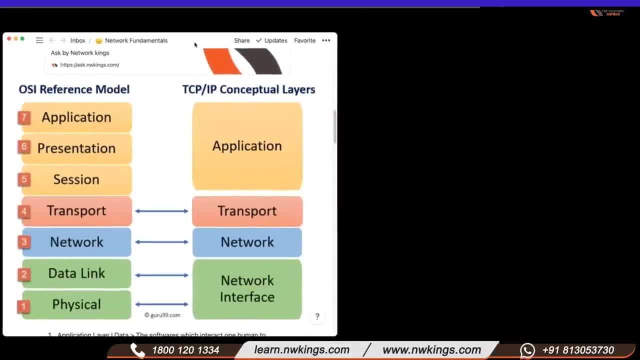 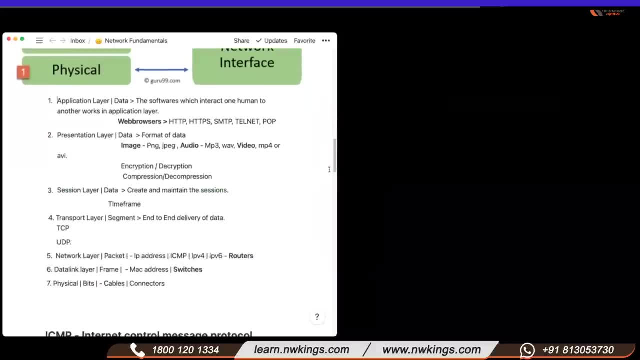 okay. so let's go further, guys, and let's quickly review the osi model which we discussed yesterday. so, in application, what happens? the softwares interact, one human to another, that all protocols like http, https, smtp, telnet, pop, all the applications works under application layer. 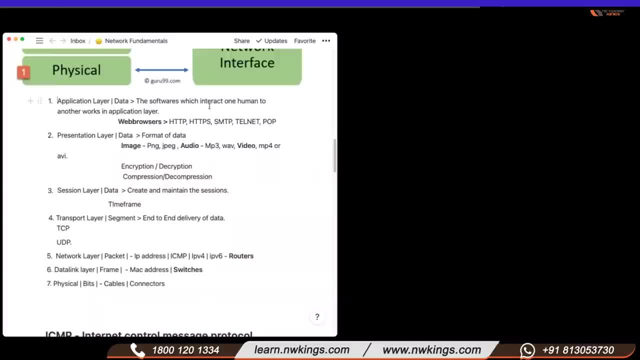 so, whenever any layer is actually deciding what is the format of the layer or the format of data, either the image is into png format, jpeg format, or audio in mp3 or wave videos in mp4 or avi. this layer is also responsible for encryption, decryption, compression, decompression. 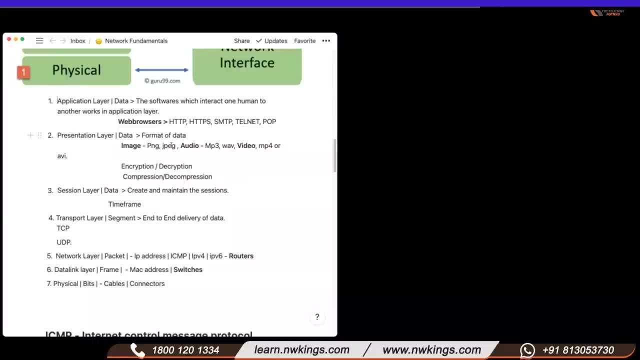 so all comes under presentation layer. so now we have another layer, that is session layer, which actually create and maintain the session within a time frame. so if you are opening any bank website, it takes around 10 minutes right to log out automatically because that is a time frame which is actually created with the session sockets or session programming. 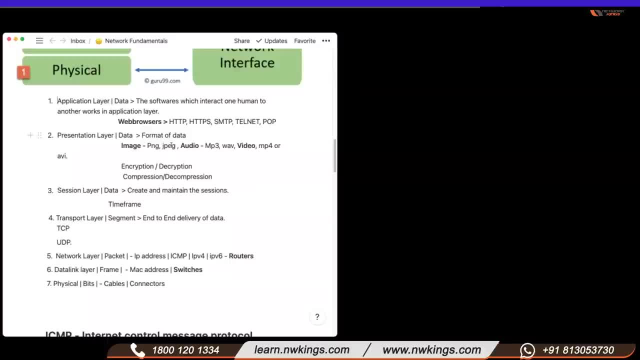 so this session layer- just you can remember this- it's responsible for creating and maintaining the sessions. okay, so in transport layer we have end-to-end delivery of data, where we get tcp and udp. so tcp is a protocol where we get acknowledgements, but in udp we don't get the acknowledgements. 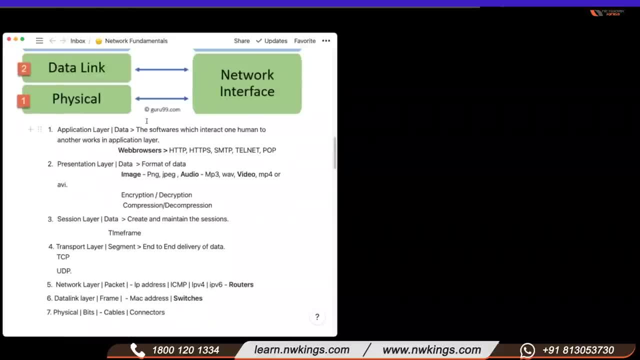 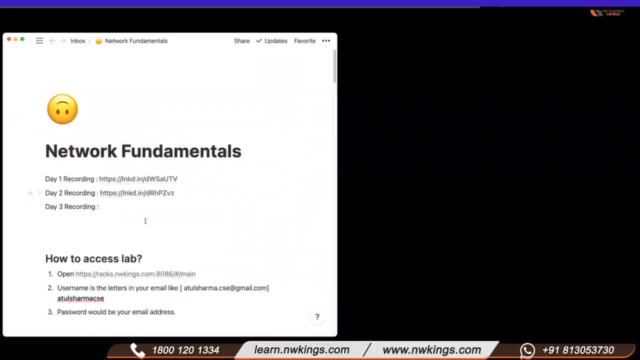 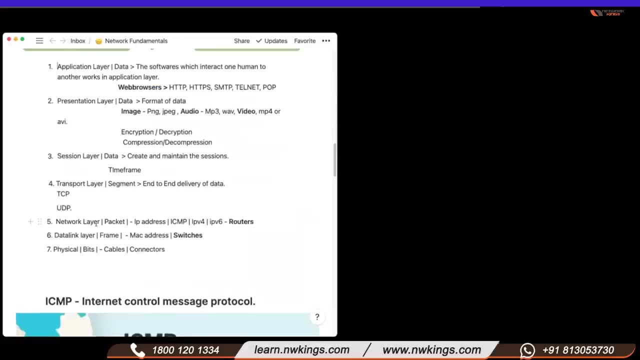 so just check the second day video, the link already shared here. if you are attending this session today, so you should watch these two videos which are yesterday and the day before yesterday video. so in network layer all the ip addressing and the ip address is added over here. 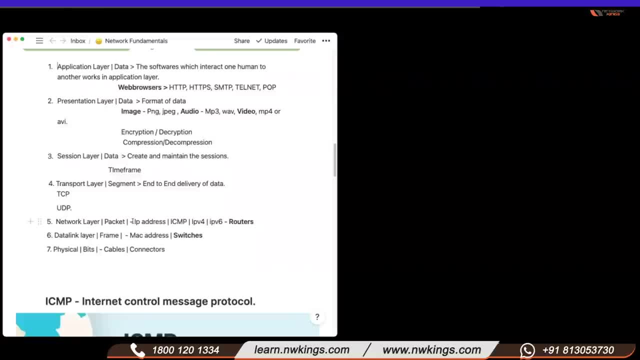 router works on this layer and the packet. in transport layer we have segments, but segments are now converting into packet. packet means the ip address of source and destination is added into the packet. so we have data link layer which actually may adds or mac address information in the packet. 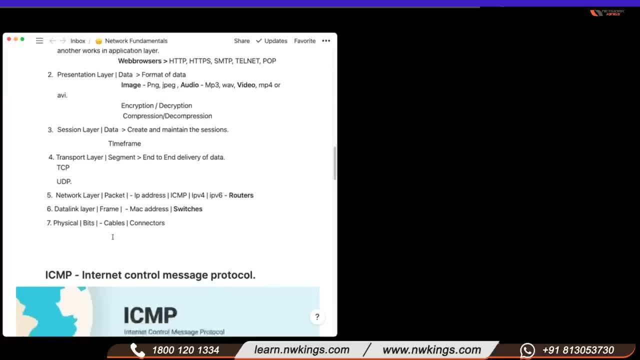 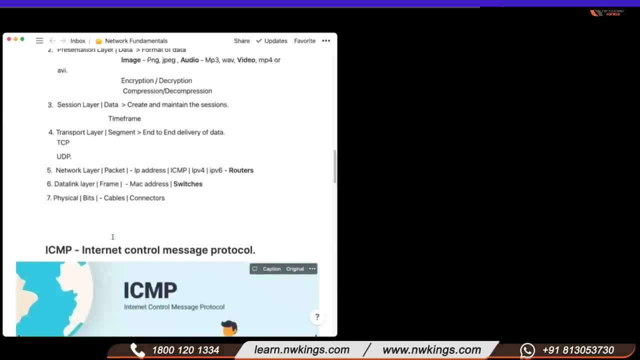 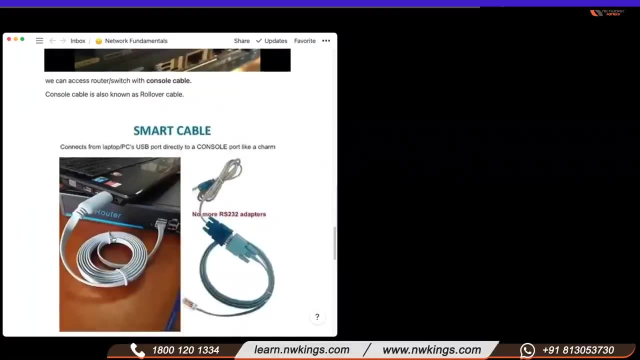 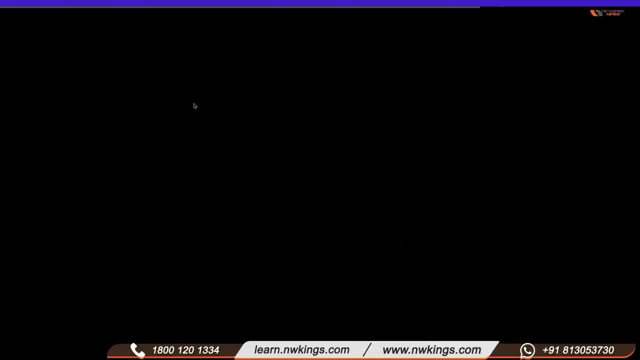 and that is known as frame, and switches works on this layer, and physical means your cable connections, all connectors comes under physical layer. so this is the overview of this osi model. okay, so, guys, today we are going to do subnetting, which is very important part. most of you were asking for it. 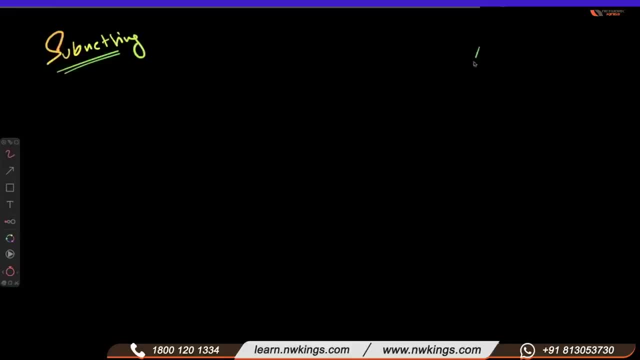 and if you still remember classes, that class a, 12126 b stands for 128 to 191, and i am not going to explain only subnetting, we are going to do small practical with the subnetting part also today. so 192 to 223, okay, so just you need to learn subnetting with abc. 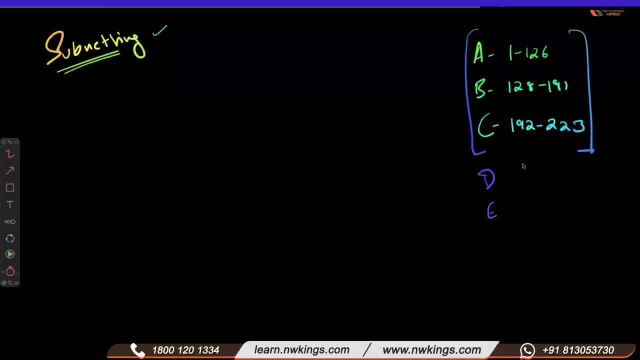 so d or e classes are actually not used with the host means you can't give d or e class to the computers because d is reserved for multicasting. so what is multicasting? you can just take one example: when all routers in a network wants to communicate with each other. 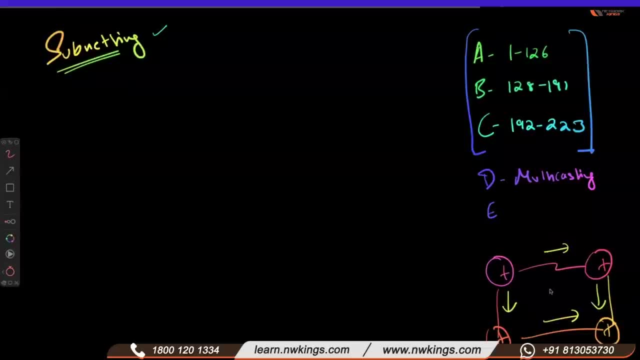 they are going to communicate or they are going to share information with routing protocols. so these routing protocols are working on multicasting, so you can just take that example. so multicasting means, from multicasting, they are sharing their information to each other. okay, multicasting is like reserved ips. 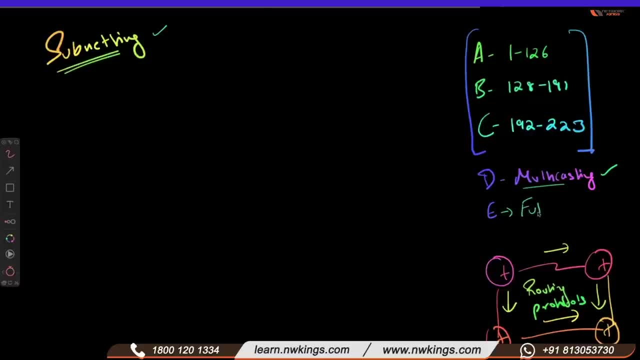 and e also. that is known as like future use or something, but it is now wastage. so why i am saying wastage? because they thought, like once we have shortage of ip address, abc, we are going to use class e in future, but no system like, not windows, not even linux. 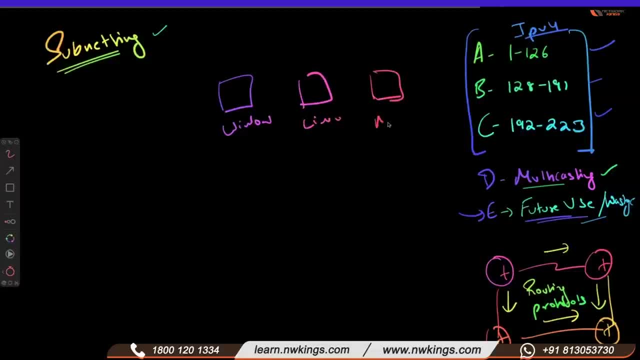 not even apple or mac os. not any single operating system support e class because initially it was meant to be used in future use. but we can't use that ips now because no software in the industry supports class e. so ideally you can say that it was reserved for future use. 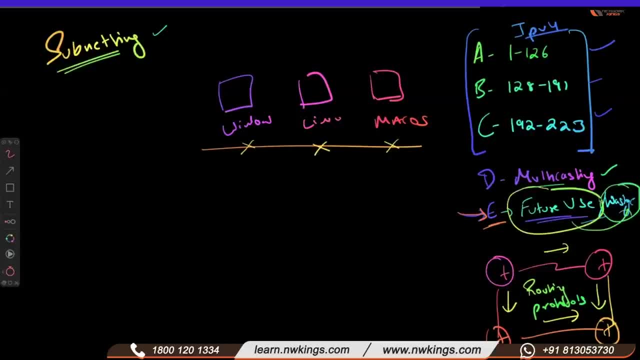 but now it is now a wastage. okay, we can't use this clear. just say yes in the chat and please keep interacting in the chat. yes, no, something, so that it will give me boost also, else i will feel bored right to train, because when i usually take my live classes, 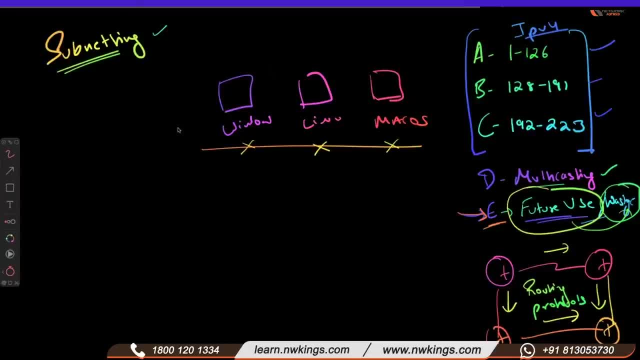 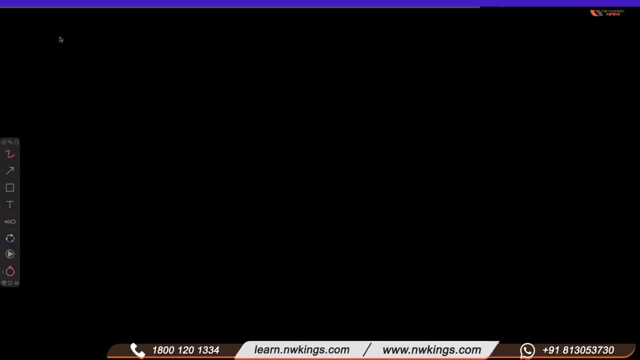 i actually ask students to raise the hand and they can speak with me, but yes, this is a public session, so it's always better to have discussion on the chat, okay, so let's understand what is subnetting. so what is subnetting? see class a b. class a b c. 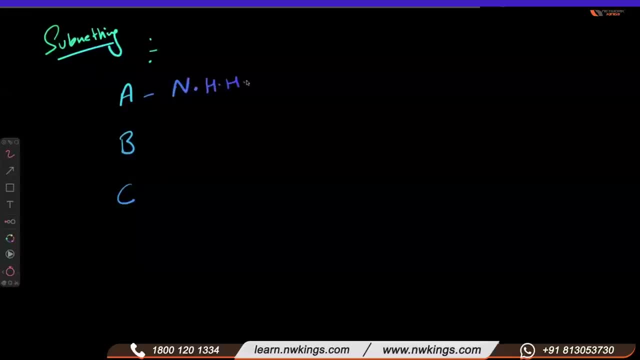 so in class a we have first part is network. it means if any computer is connected to another computer and ip address is 1.1.1, another ip is 1.1.5. so for the we need to check the first part right and how computer checks the first part. 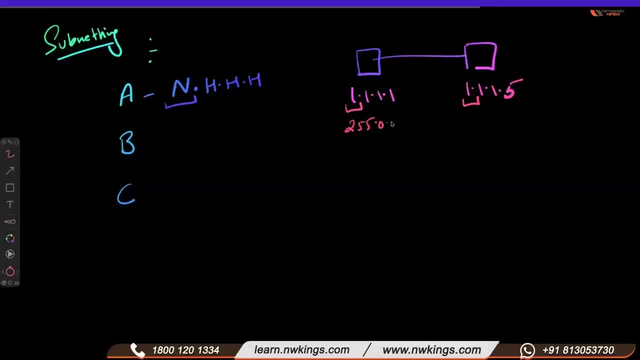 because we give one thing that is known as subnet mask. so whenever you give ip, there is one extra information is added automatically. that is known as subnet mask. so what is this subnet mask? it actually represents network bits. so it represents network bits. okay, so subnet mask represents: 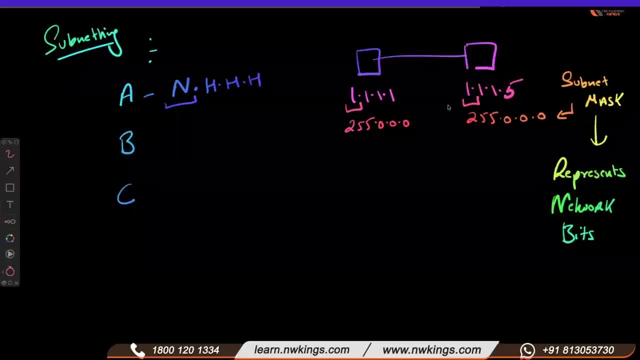 definitely okay. so this 255. it is representing that i need to match how many part. only the first part. so class a is known as 255.0.0.0 also. so that is the by default subnet mask of class a. it is representing that only the first part is network. 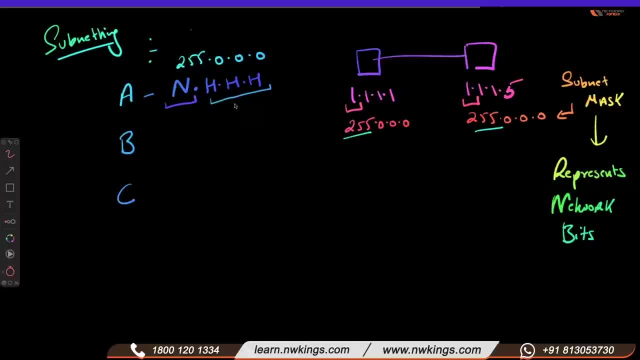 and rest. all part is host. all part host means in class a we can assign a lot many ip addresses. so in b class we have two network part. so how computer understand? so when we give any ip like 172.16.1.1 and another computer is 172.16.2.3. 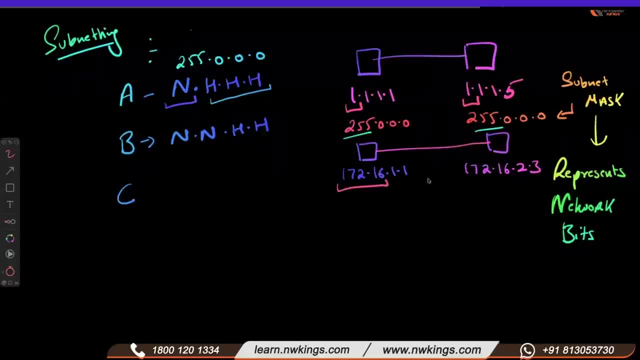 so they are going to communicate with each other because their first two portion are matching right. they are in same network how? because when we assign the computer automatically takes 2 times 255, this happens automatically. you can try it out. so 2 times 255, it means the by default subnet mask is 255.0.0. 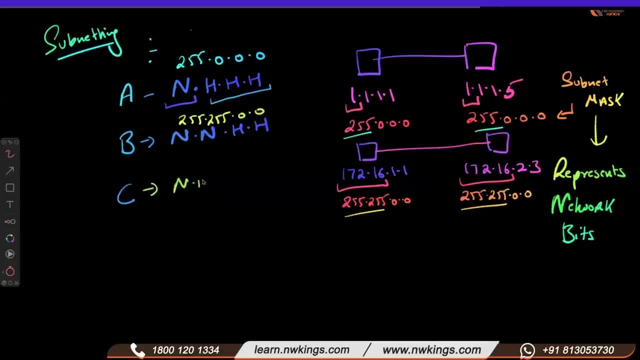 in c. so then we have around three network part and one host part. it means we have 3255. so how many parts we need to match. so when we assign: give any ip address to computer of class c, suppose 200.1.1.1. 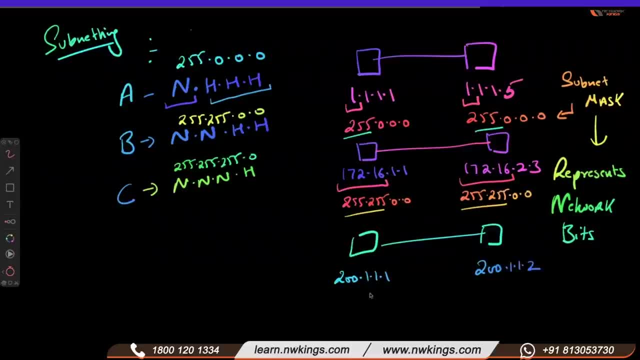 and 200.1.1.2. so, like the first three parts, if both, if both machines parts are matching up to three network, up to three octets. so it octet means one group is known as octet also because it is 8 bits. 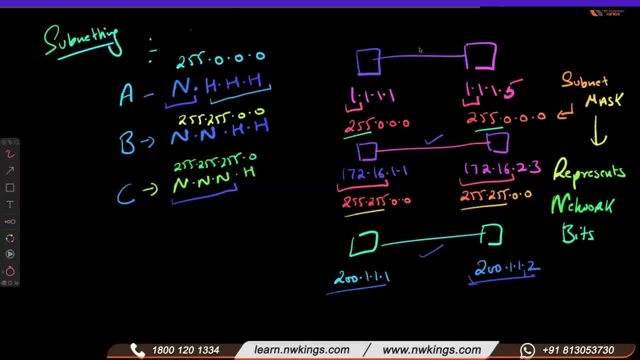 so three parts are matching. they are also able to communicate, so this means 3255.0. yeah, yeah, i will explain. so the ips i have. so i will explain private and public ip later on. so just you need to understand this first. ok, so just type yes, if you understand. 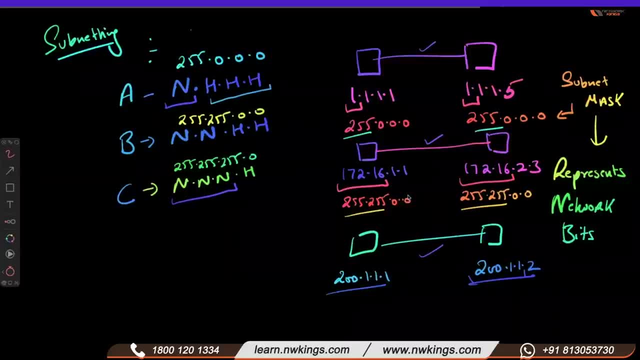 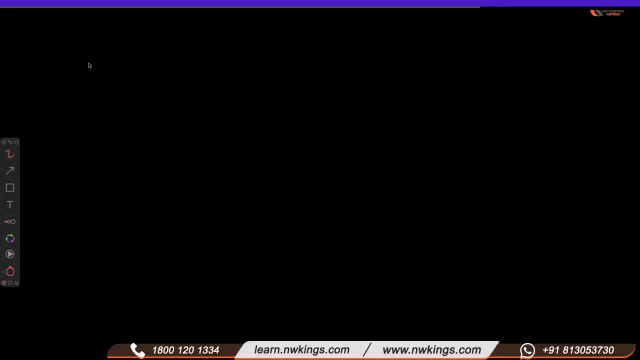 and then we can go on ok, ok, ok. so now he is submitting: divide a large group, divide a big network or divide a network into smaller parts. so why we want we are going to divide the network into smaller networks. i am going to explain you. so, first of all, class a: it has network part, one octet network part, but rest three host. so it means 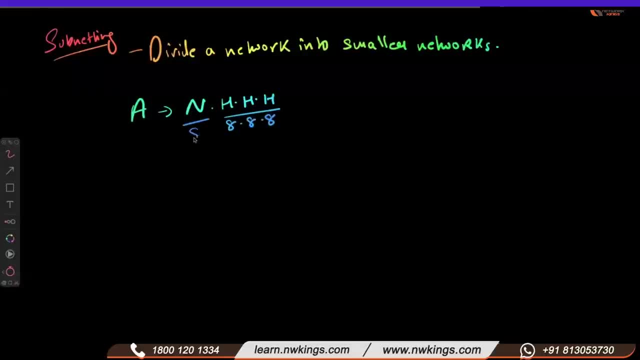 eight bit, eight bit, eight bit right it. this is also it. so eight means it has a 24 host bits, 24 host bits right eight, eight, eight. so to the power of 24. so how many computers like one class, a ip range class, a subnet, gives one six, triple, seven. 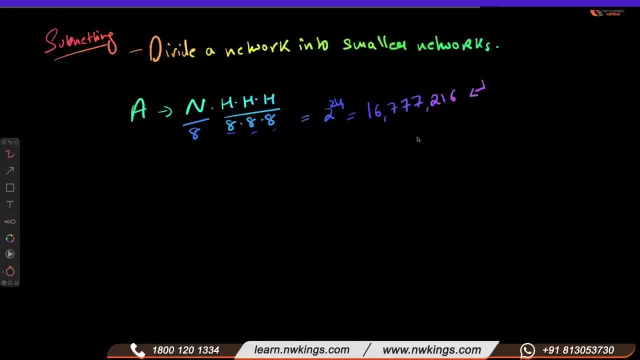 two, one, six. that is the number to the power of 24.. so if you start giving ip from one dot zero, dot, zero, dot one, it will go up to one, two, five, five, two, five, five, two, five, four. almost. so you can start with zero and go up to two, five, five, but the first 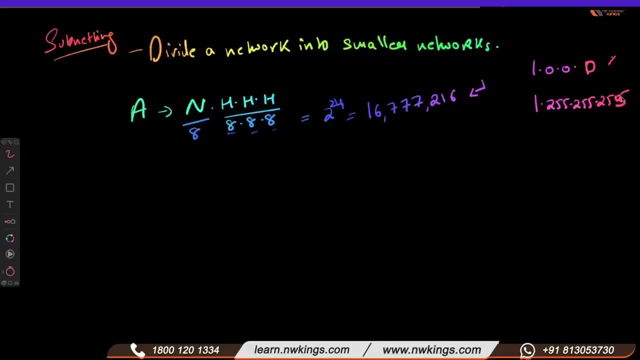 ip, and the last type we don't use because of network id and broadcast id that i'll explain later on. so you can just count these numbers. you can't even count these numbers manually, so it's a very big number actually. you can't even count these numbers manually, so it's a very big number. 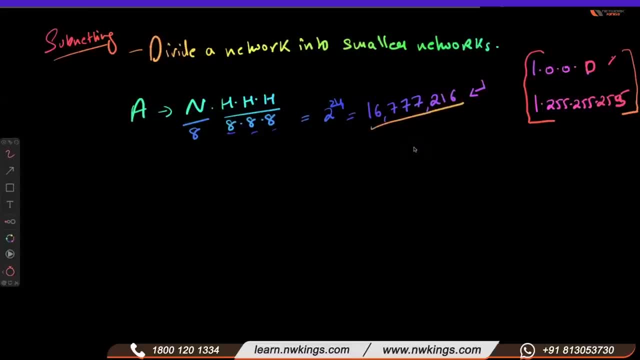 actually so that ips is one, six, triple seven, two, one, six, the one subnet. it means one network of class a gives that much ip, so another. if i'm saying two dot zero, dot zero, dot zero, so that is a separate one number. so that is here, we have that number also, and here also we have that number. 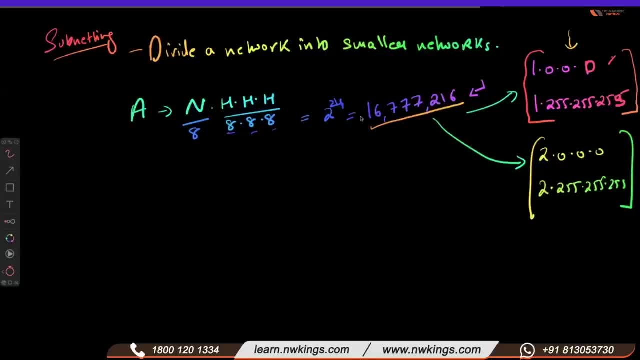 so means these are two complete different groups. each groups give that ips. okay, so in class b subnet, any subnet of class b, that gives how much ip addresses, that gives to the power of 16, that is 65 536. in class c we have three network part and one host. 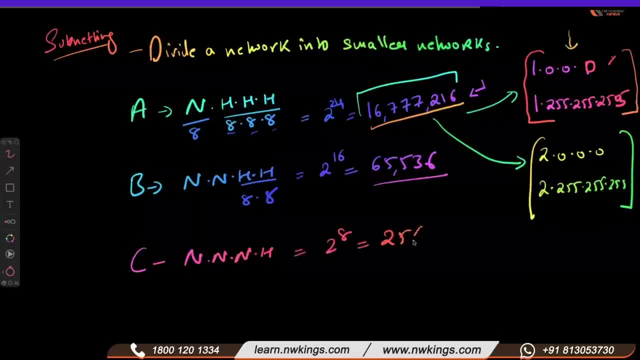 part so to the power of eight is 256.. so c class networks gives 256 addresses, b class gives 65, 500, 36 and a class gives one, six, triple seven, two, one, six. yeah, network bits always remain same. this i am talking about host. now i've already explained. 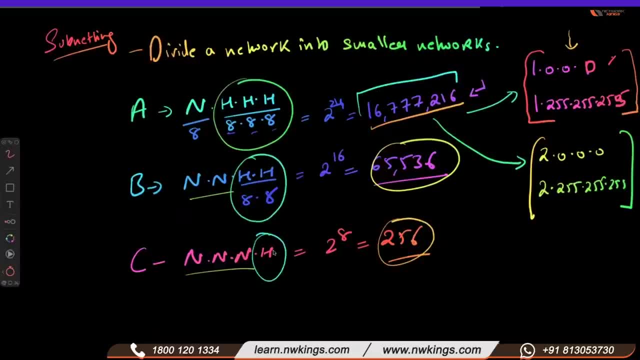 in the last slide, or what we call last, where i was drawing. so so that i'm discussing now host part for non- balloons or any kind of to 거칠앵. these are to operation rate. okay, so we have for an ol and for and for juice and for. 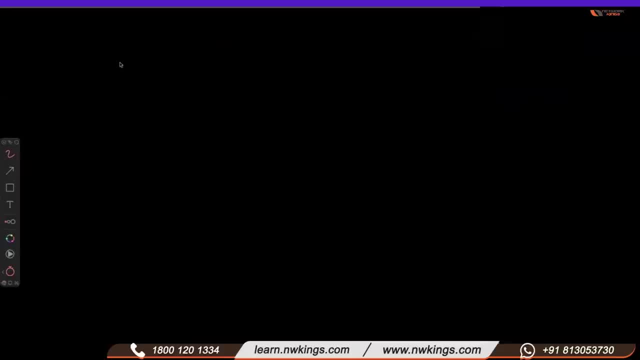 and also for. so i gave all these terms. i gave classes as p and twice k and once p times. it is twenty-three engine units. so this is common in it that i give to and from this î and one-term ku won't be exactly u? n at the beginning of class one. the big idea is to prove that this is normal. 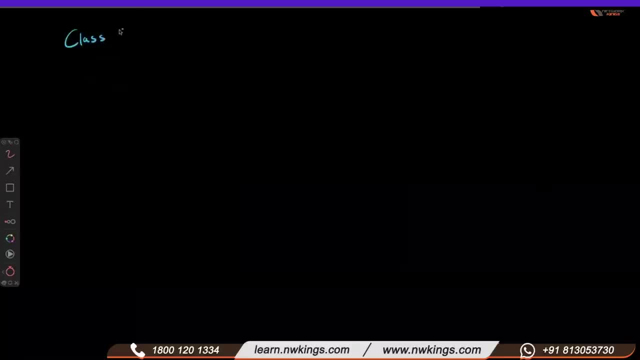 method. and last thing i will point out first, which is that if you have several different classes, so i will think first let's use the t- donné and not the other. i am not, Katie, what was our? so? class c gives 256 address, so it means 192, 168.1 if the ip network bits are like this. 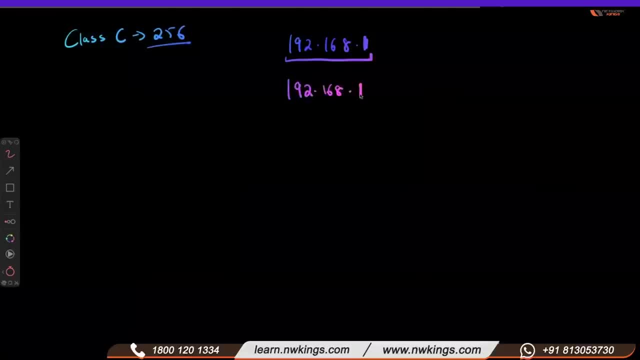 so this will keep. this will remain same. right because of network, bits remain same. so it starts from 0, it will go up to 255. so 0 to 255. if you count this number you will get 256 address. okay, so if this class c ip is giving 256 address, and if i want to divide this into 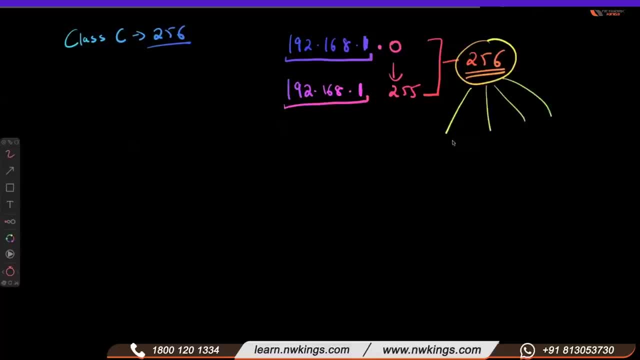 four parts, or two parts, or like i want to divide this network into four parts. so i'm going to divide this network into four parts. and i'm going to divide this network into four parts so that we can give ip addresses to these networks. maybe i'm creating computer labs. 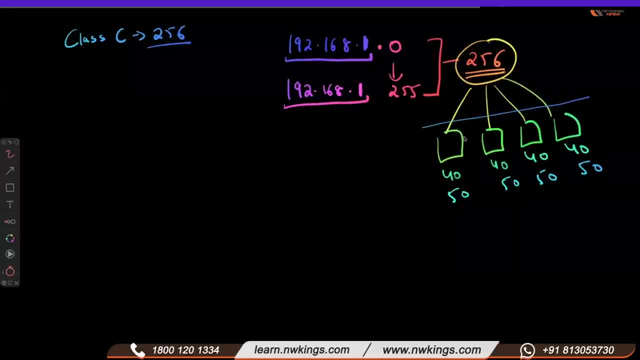 in my college, or maybe i'm creating some odc's in my college, or maybe i'm creating some odc's in my college, or maybe i'm creating some odc's in my office. so i want to give 50 computers group in all networks. so if my requirement is 50, 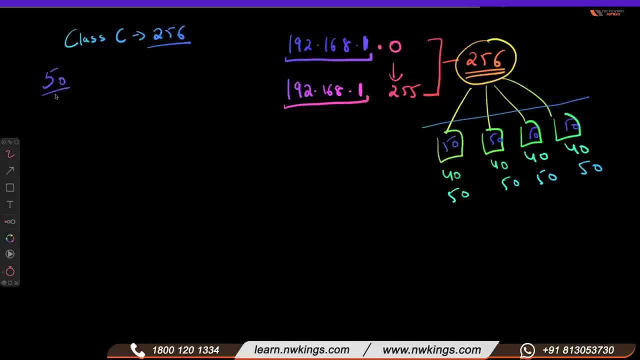 suppose i want to give ip addresses to 50 computers, but class c is giving me 256. so if i am going to use 256 ips in 50 computers, how much i am going to waste? i am going to waste stage of 206 ips, right? so 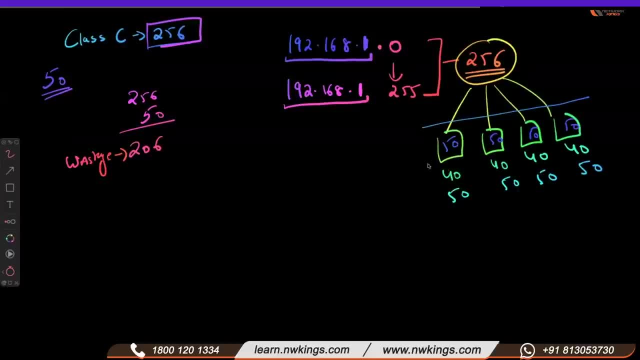 so so that is happening. if i, if i want to create four computer labs, uh, either have to use multiple networks, and we should not have multiple networks. why tell me most of you know 190 to 168. if you don't know this, this network is free. you can see, say that. 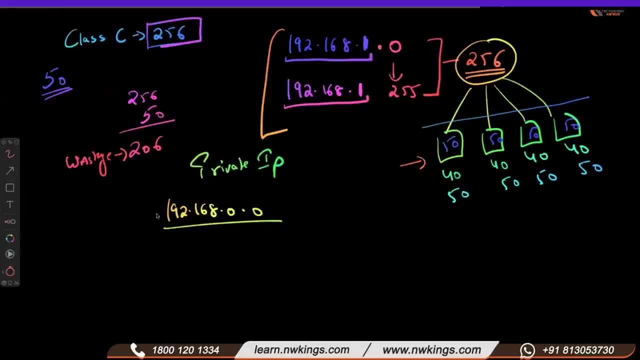 it's a private ip and private ip is free, but why we are doing subnetting in private ip. can anybody, can anybody explain me? or you can explain me? how can i provide subnetabilty here? if i can provide, let me show this and i can add also: you, can i canhlp get some more worldwide network? i can add. 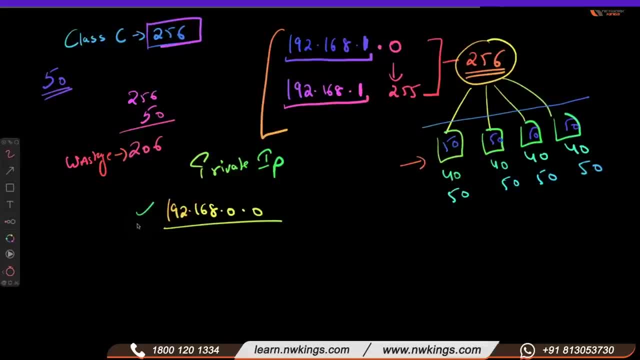 can anybody ever seen me? or you step change bus as well. if not, i can apply. be that is that this carte. can anybody ever seen me? or you can play something. that is what stuff? that is why, hi, please explain me in the chat. Kunal 192 168 series is private IP series. This is the reason. So in what? 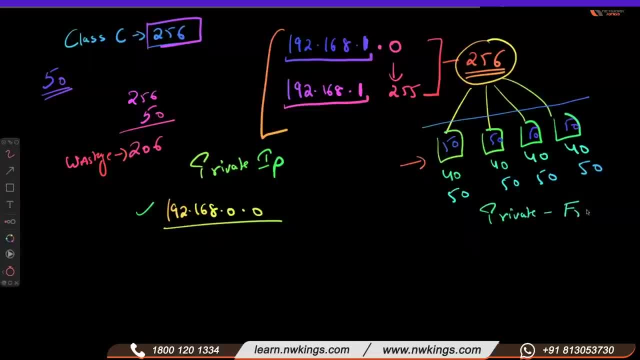 is private IP. These are complete free IPs You can assign or you can use it for anywhere. So in class A, 10 IP is private. Any IP start with 10 IP that is private and free. So 172, 16.02.02, 172, 31.255.. Means any IP start from 172, 16 to 172, 31.. All are private IPs And 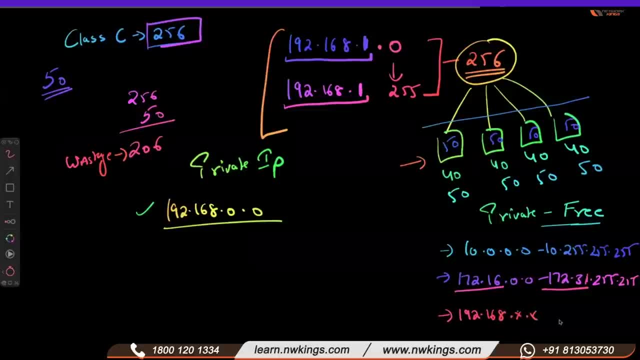 in class C we have 192- 168. So any IP start with 192- 168.. So any IP start with 192, it's private IP. So I'm asking if IP addresses are so free, because in class C you are getting almost every network. You can use 1.0,, 2.0,. 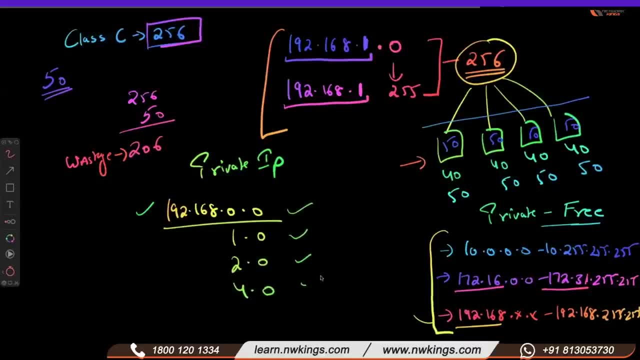 4.0. So you can use all four networks in these computer labs Because these are free, right. So why we are doing subnetting? then Anyone from industry Here? Ok, let me put everything on private IP and I will give. if private IP is free, is I'm. 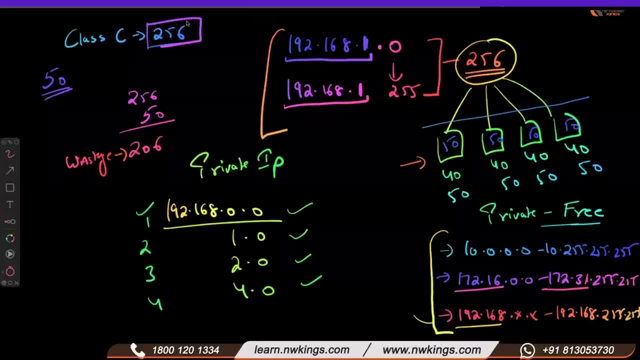 going to use privately. First of all, private IP. Think for two, three minutes Why we are doing subnetting. If Private IPs are free ips, you need to buy all ips, right? so you want to use any ip address, you need to register it. but private ips are like free. you can use it for free and how you will. you can't access internet with private ips. if you want to access internet you want, you have to use isp or internet connection, because internet connection actually gives you public ip. so when your internet, so you can do. 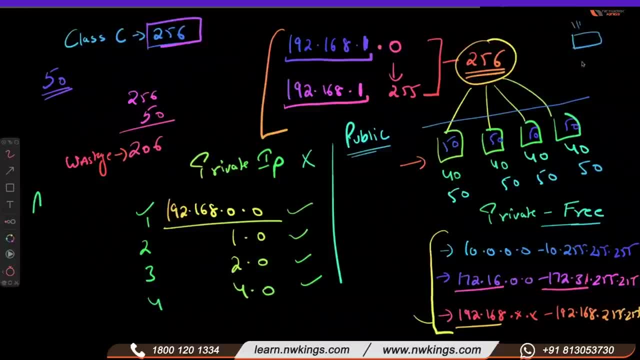 one thing if you have wi-fi router or wi-fi device at home. so what you can do, you can connect all your computers, you can check if all are pinging together or not. and what you can do, you can disconnect the internet cable from your router and still check if they can communicate with each. 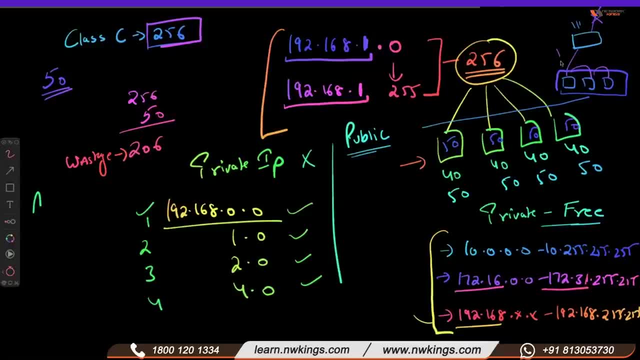 other or not, so they will communicate with each other. so that is my private network, okay, so public means routable to internet. private ip is not routable to internet. so my question was why we are dividing the, why we are submitting when we can use free ips. so i'll explain. 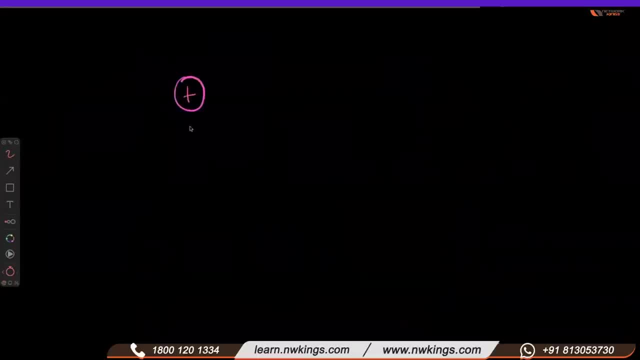 so when you will have a router in your office, okay, and maybe you have four networks, four networks or maybe you have different, different networks, right? so if this router has different networks, then you can use free ips. so if you have a different network, 192 168 1.0, 192 168, maybe 2.0, so it may be 192 168 3.0. 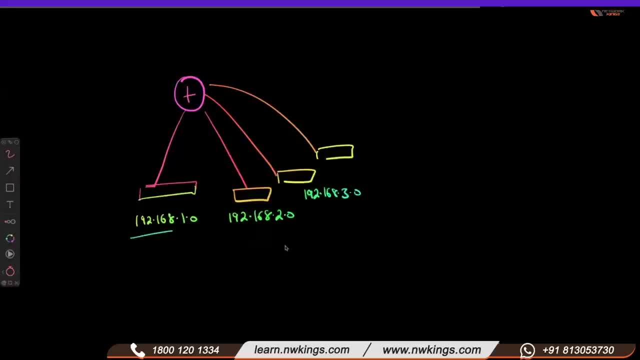 okay. so if you have 192 series, that's okay, but maybe you have another 192, 168, uh, 99.0, something like that. so, uh, why it's better to always do subnetting, because when this router is going to share that information to this router. 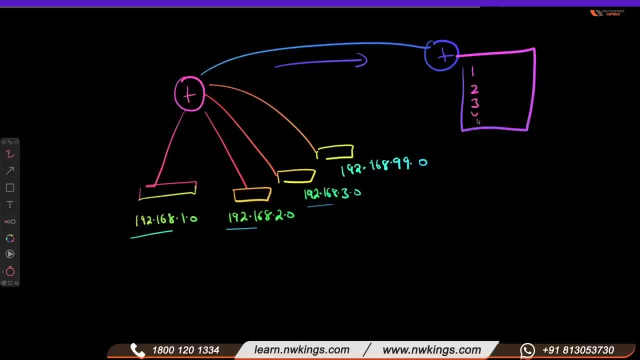 so router will have all four networks. so instead of sending four, four in our networks information, uh, it's better to have one network only because it is going to take less amount of space in the routing table. so what we are going to do, we are going summarize means. instead of sending all the routes, i'm going to send something so that. 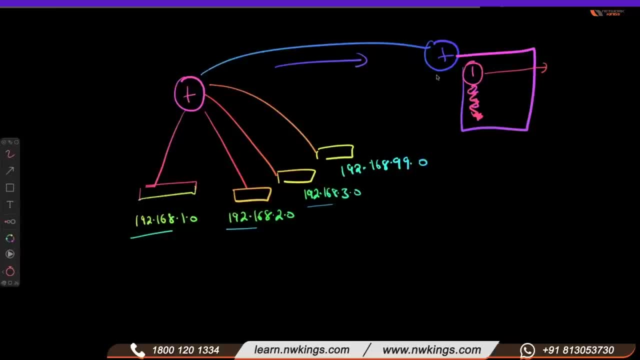 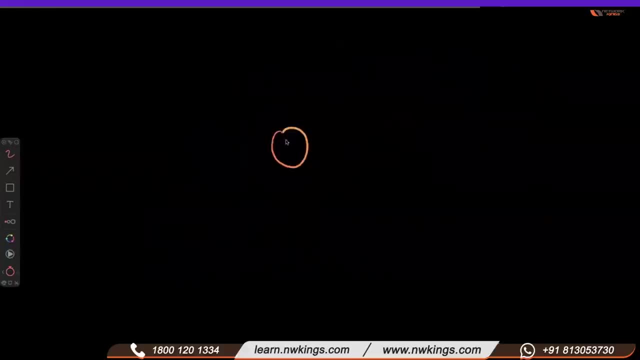 this router will get only one or two routes and and can access anyone. so one another example: if you have very big site, you have thousands of or maybe hundreds of routers. all your company routers are connected with maybe big routers like that- okay, so all these client offices. or maybe if you have your own branches, so all branch offices are. 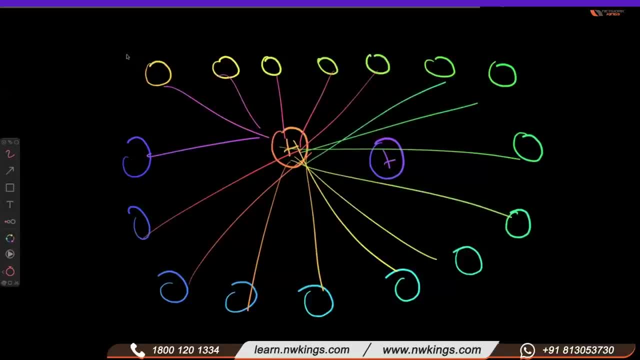 like this. so all branch offices are going to send the information to you and this router. okay, this router is going to have a lot of routes. so if you are sending four, four networks or maybe eight, eight networks from everywhere, what will happen? it will have a very big routing table. 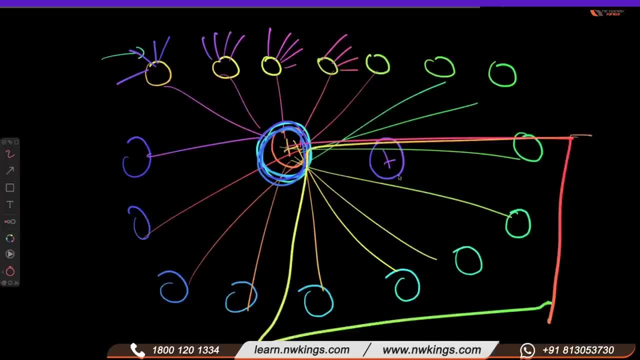 right, it will have a very big routing table with a lot of entries. so if your routing table is very big, so it means there is a load on our router ram, like when we install a lot of softwares, what will happen in our computers so they get slow down, or 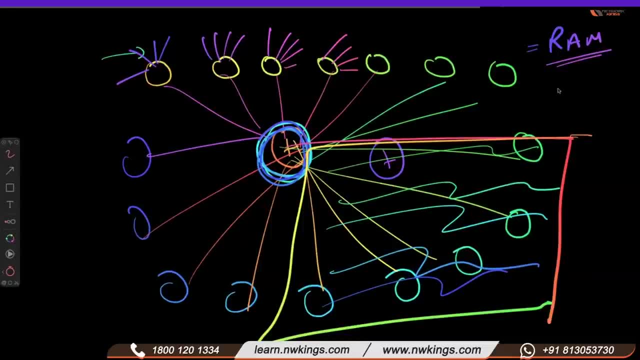 maybe they keep on restarting or blue screen comes right. so if you have a very, if you have a lot of many routes, what will happen? so your main routers can have a lot many routes and can lead to either you need to buy a very premium hardware or very big router to manage these routes. 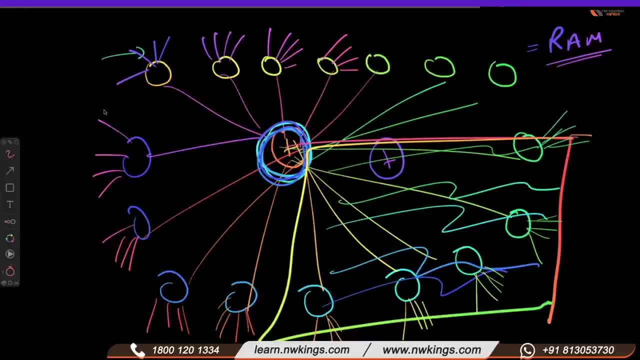 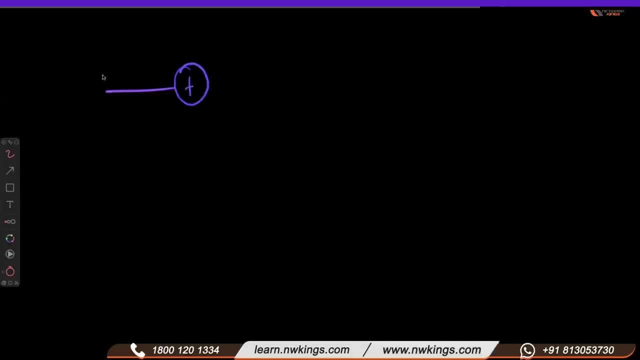 or you need to short these ones. instead of sending four, four, eight, eight routes, i'm going to send only one route. so this is the purpose of subnetting. so means if router is sending 192, 168, 1.0 from here to another router, so router will have only one. 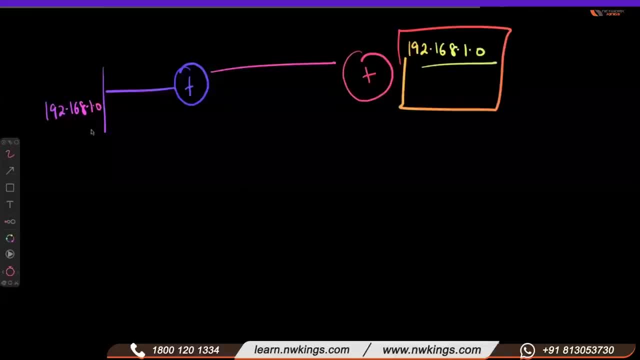 route 192, 168, 1.0 in the table. but here i am going to divide this network into four parts and i am going to create four computer labs. now understand why we use subnetting to subnet network. to divide subnet and network network. yeah, to summarize means, instead of see, if first learn how to divide a network. 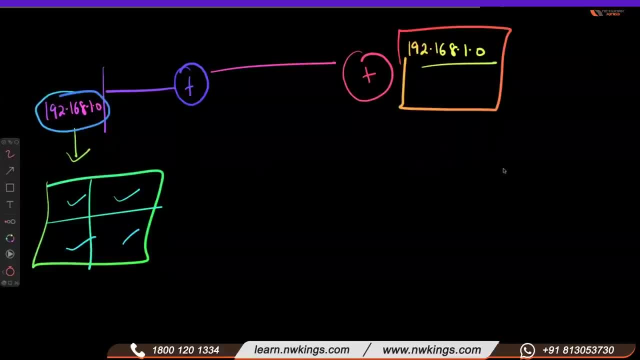 so why, before submitting, i am showing you why we do submitting. subnetting. okay, so that, instead of sending four routes. so tell me which is better: sending all four routes or just sending one particular single route to the another router? one is better or four is better? you must be thinking: four is better, maybe. no, it actually consumes a lot of ram. 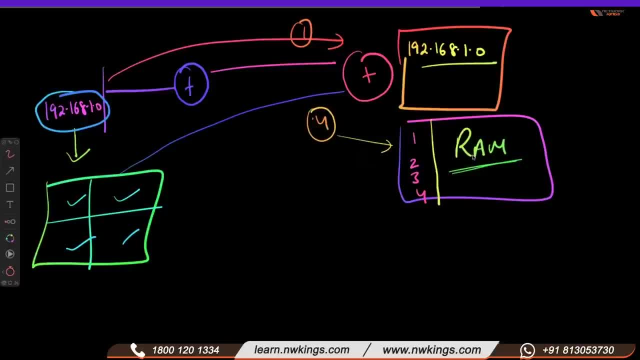 one is always better, right? so just don't imagine this with two routers. just imagine if we have 100 plus routers or maybe thousand routers in our company whole. suppose if i'm working for apple, samsung, like these brands. they have offices almost in every country, right, and subnetting is all not only in private. subnetting happens in public networks also. 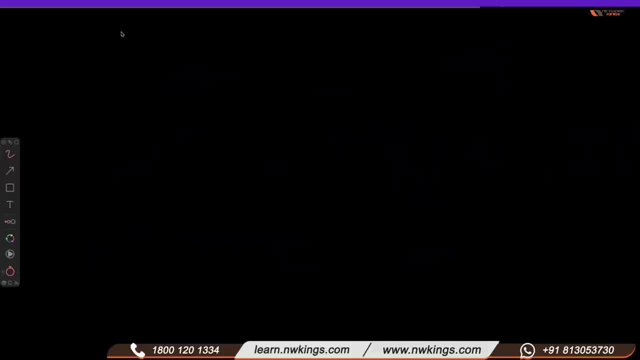 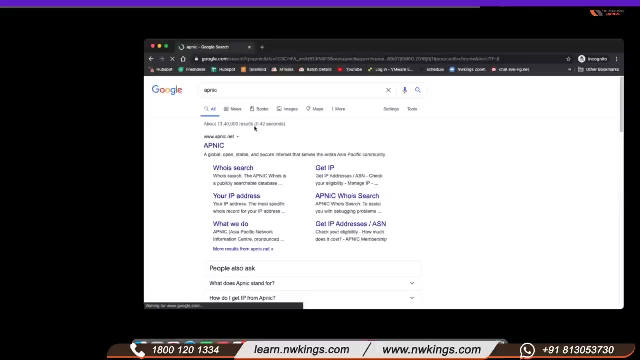 what exactly suppose you got a ip address? i told you you get ip address from aina rir. that is apnic. so you will go to apnic website and buy a ip address. okay, so let me show you apnic. okay, so let's see if apnic gives me two ip addresses and why you need to have public ip, tell me. 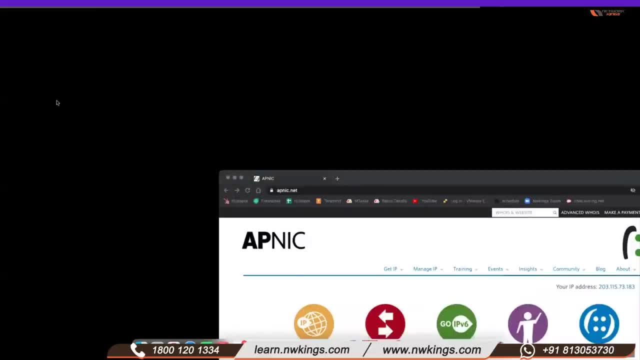 i'll give you one real example. see, i have a server where we have installed the labs like racksnwkingscom, and you guys can access this website right. so this is a url, but on this url has some ip like 203 181, 25 like that, and you can access this website right. so this is a url, but on this url has some ip like 203 181, 25 like that. 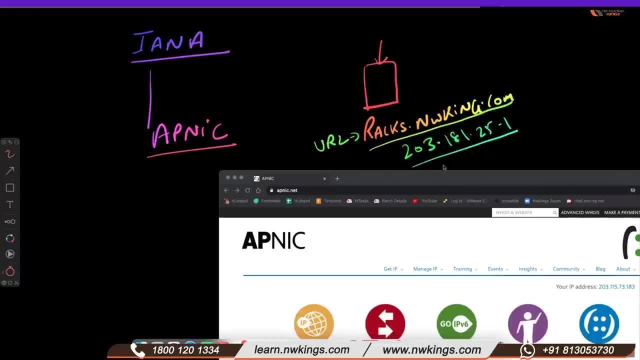 okay, so this ip is my public ip and this ip i got it from where? from my isp. okay, so i just bought one single ip or maybe two ips. that is known as static ip. so this is my static ip and static ip i have entered into my dns so that if anybody goes to rackscom so it will redirect to. 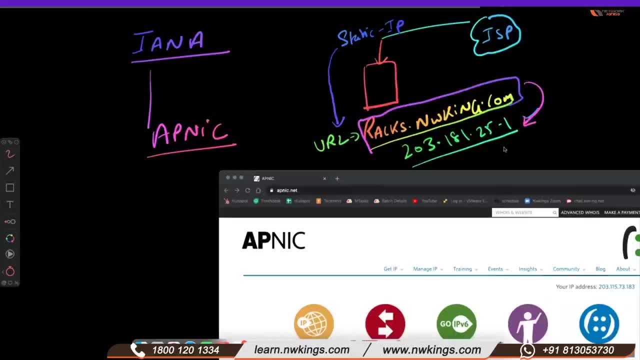 this. okay, that is a dns entry i need to create in my website. okay, fine. so static ip is to access anything from internet, so static ip is a public ip, so this ip is public ip. so why everyone needs public ip? so that you can access the servers, you can access the websites, so you need public ips. 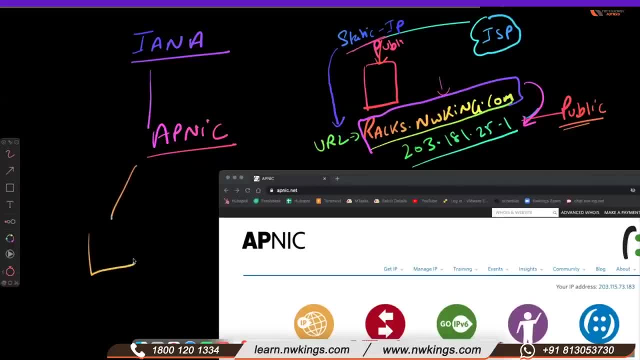 and if i'm, if any big company is going to buy ip, suppose you work for apple. okay, so they have a lot of servers like itunes, from where you can stream the music, uh, like apple cloud, where you can store your images and all, or maybe something else also right, like apple tv and all. there are a lot of. 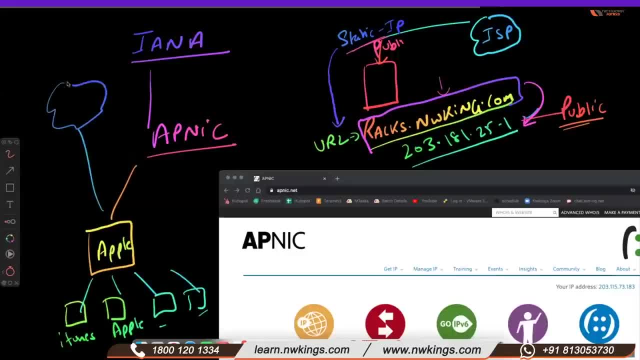 apple servers so that the users can access this from internet. so apple have public ips, right, so they have a network, public pool 17 network, right, so they are going to assign these ips to the server- you can say that- so that these users can access, put, take their selfies and upload to the apple cloud or something. 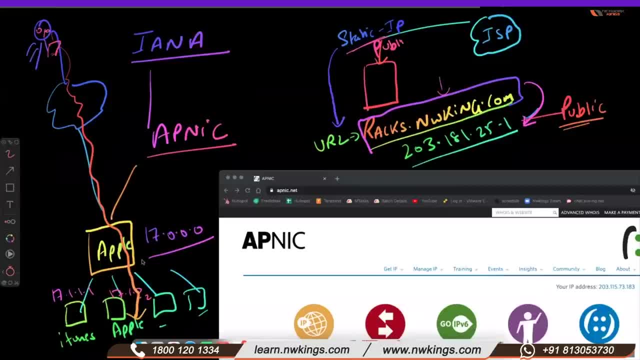 so just take an example, okay, or maybe you can take an example of facebook. so just take an example of facebook. so everyone needs public ip to access something. even this appnicnet, this, this website, is also having one public ip. but if any company wants to buy ip address from a big organization like appnic, you can't buy a single. 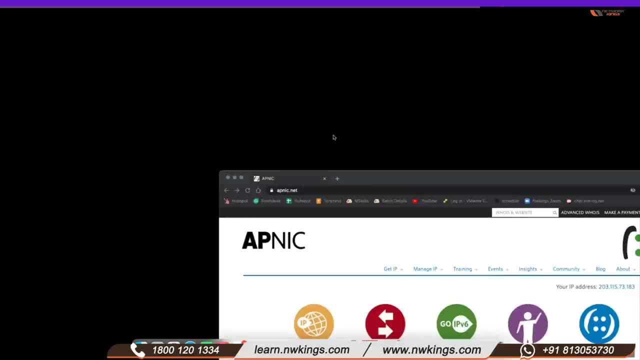 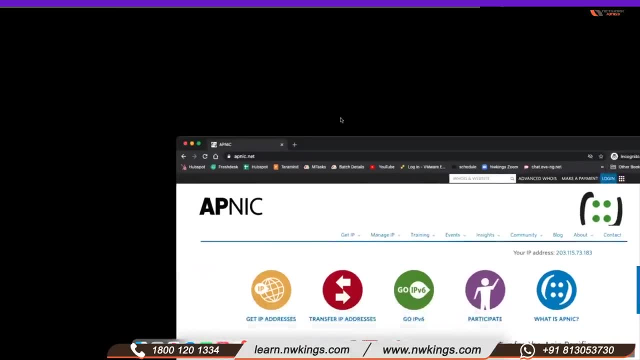 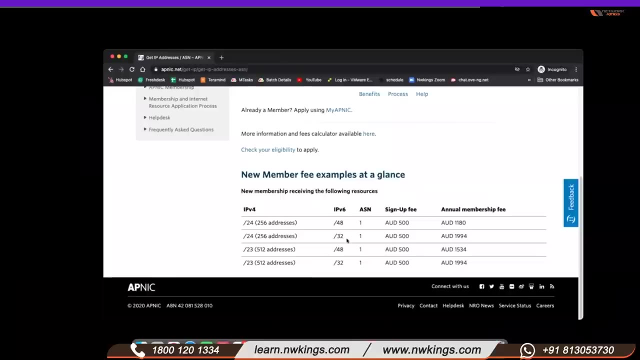 ip. if you want single one- ip2 ip, you can directly contact your isp. but if you want a very big uh, if you have a very big company, you can directly contact your isp. if you want a very big uh, if you have a very big company and you want to get ip, so just click on get ip address. it will show you you can buy minimum 256. 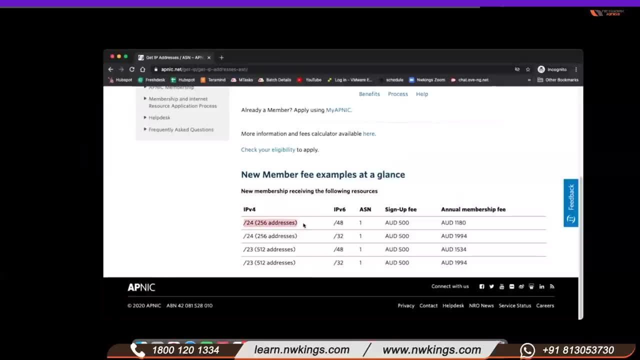 address from apnic. you can't go less than that. if you want 50 ips, you still. you are going to contact your isp. if you need more than 256 address, you can directly buy from apnic. that is asia pacific network information center. okay, got it now. so now, if you have 256 address and you have 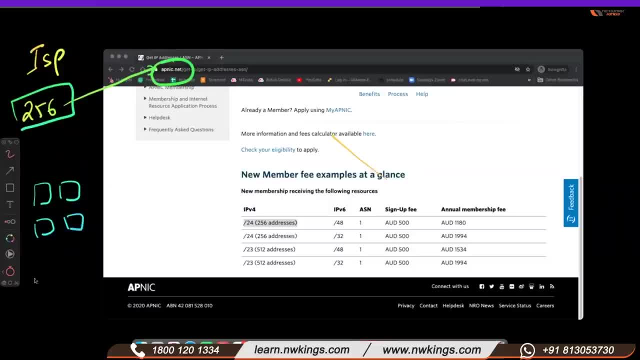 a lot of servers. maybe you have four servers in delhi, you have four servers in mumbai, you have four servers in hyderabad. so what you are going to do, tell me, subnating or not? right, you have to divide, right? you can't use one pool at one location, right? 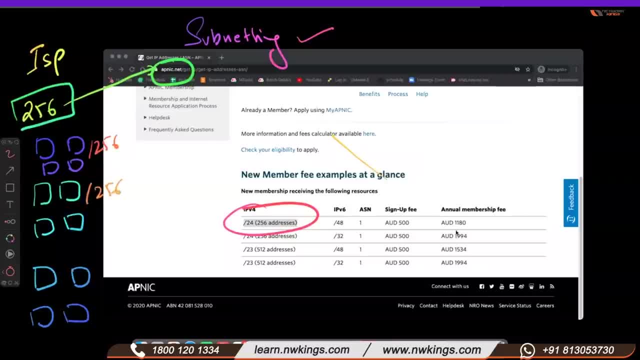 else you need to buy a lot of public ips and it will cost you australian dollars. annual membership fee 1994. you can multiply by 50, 60, whatever is the dollar in australia. so this is the annual membership fee and that is a separate sign up fee. 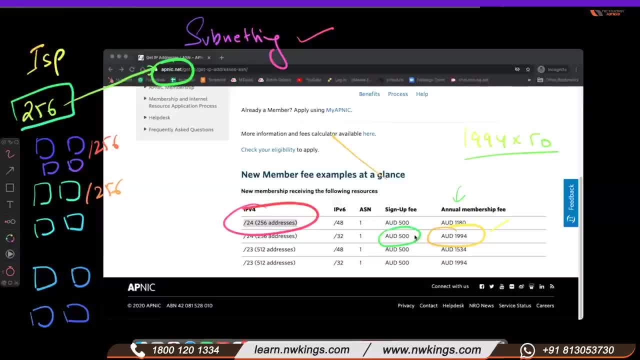 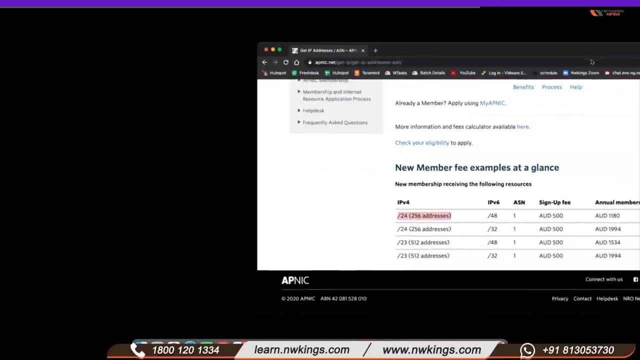 so i want to point out that with subnating, it's really not a free at all, not a free service. i am just thinking about those guys, those who have not attended still registered the session. these things are not in a book, man. okay, got it. so now you understand why we use subnetting, so tell me subnetting. 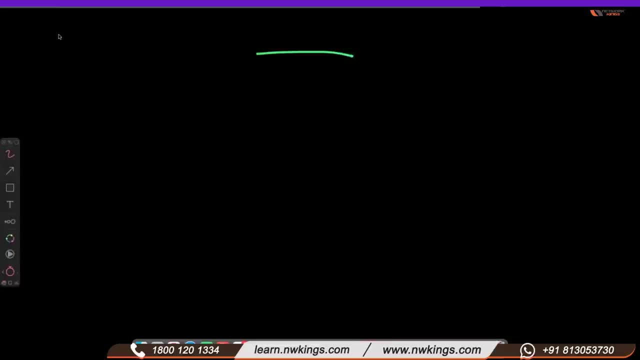 is important to learn or not. people ask me, sir, is this subnetting important? so i always say: see, everything is important. if you really love to understand, see, maybe in interviews, no, nobody is going to ask you. but if you really want to do wonders in this network field and if you really want to become a good engineer or maybe a network consultant, you. 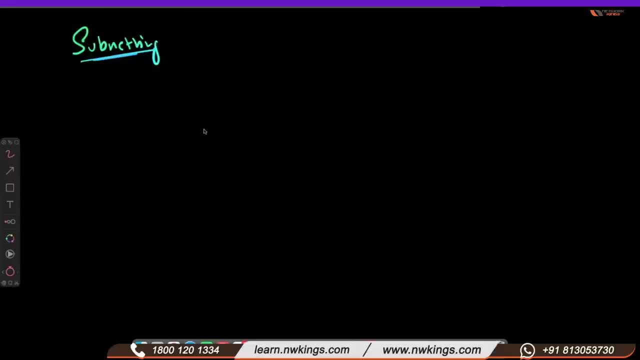 should know about these things. abhinav, this is not permanent time period. you can keep on paying them so that you will still maintain your membership. but, yes, ips will be with you till the time you are paying. okay, so let's do submitting. so we got a pool from where apnic. 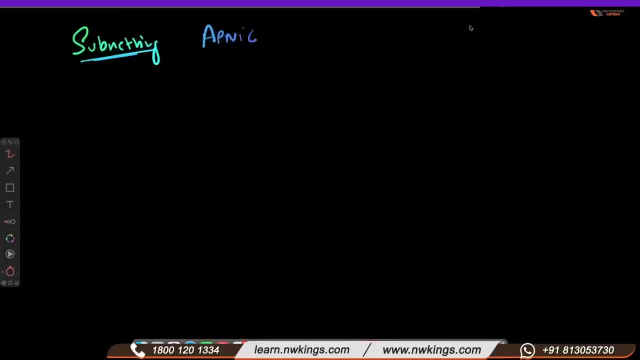 okay, okay, so let's create a data center today. so data center is what? when we have a lot of servers and we want that people can access these servers from outside world? any limitation on number of users for ip address- see public ip- is even one single ip. 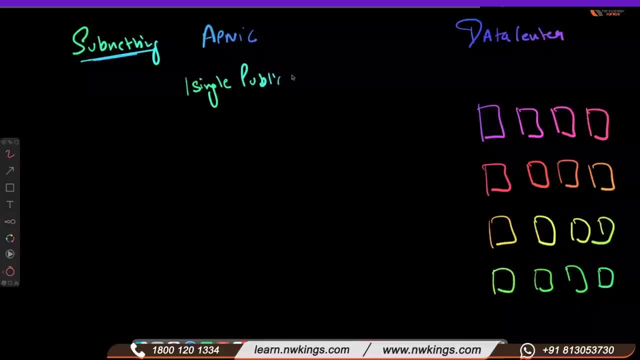 one single public ip is enough to access internet. just imagine, like if you, if you are still a student in a university of almost 10 000 students, so tell me how many ips they need to access the internet. they can still access the internet with one ip. how? because these? 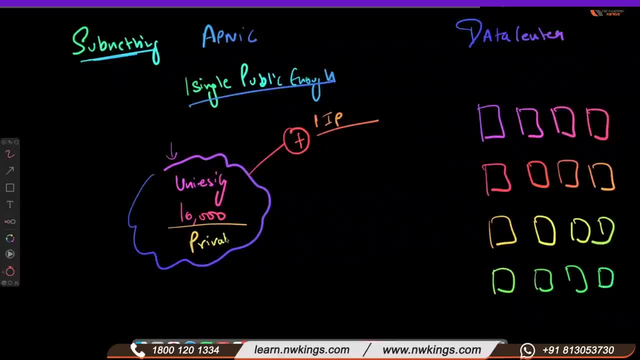 10 000 student who are in university of almost 10 000 student. they need to access the internet with computers, will get private ips, and all these private ips are going to convert into one single ip and with the help of a concept that is known as nat network address translation. 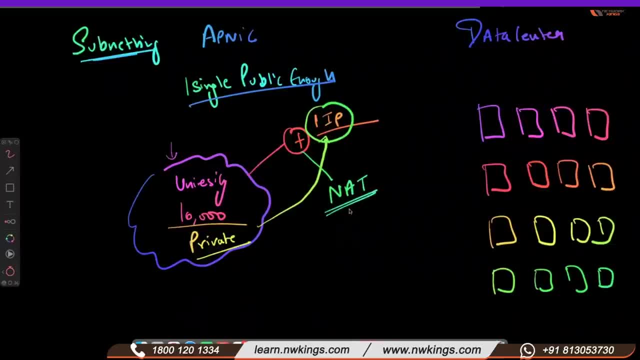 okay, but when we are saying we have bought a pool of 256 ips from apnic, what exactly it means? i am talking about a company where they have a lot of servers and from internet, people or anyone can access these servers, or maybe they are uploading the. 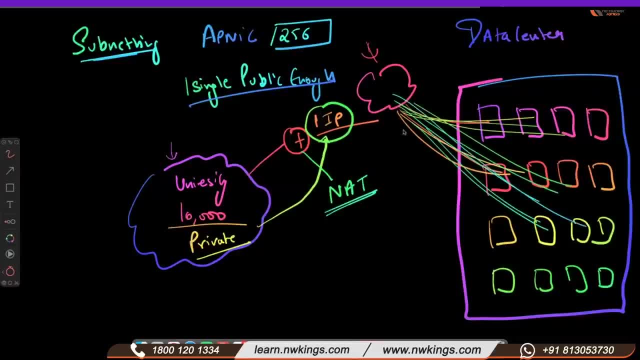 videos or maybe images, because in one like- just take an example- when anybody uploads the images in facebook, so tell me, all images are going in one server. or they have a data center with a lot of many servers. okay, so i am talking about a company where they have a lot of servers and from internet people. 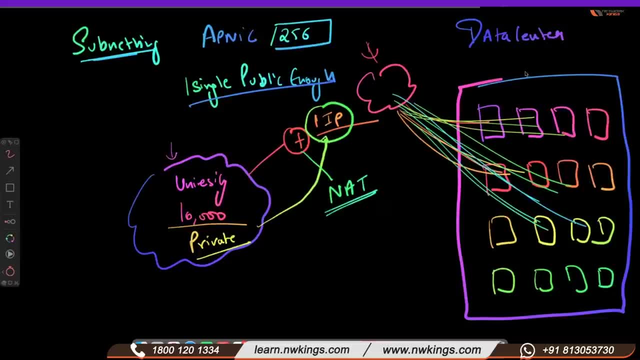 lot of servers, right, so they will have a lot of servers. so they need a lot public ips or they can use one single ip, see accessing internet. you can access the internet with one ip also, but if anybody wants to enter into your premises or you, they want to access your servers, then you need. 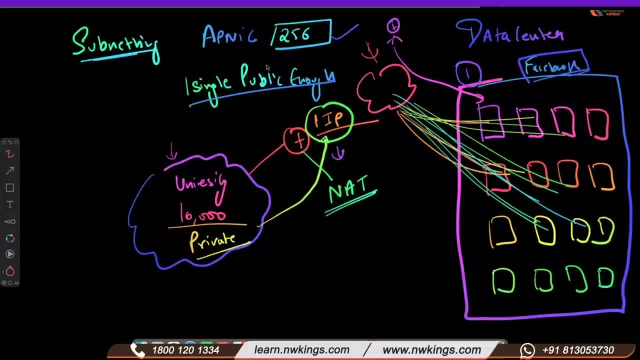 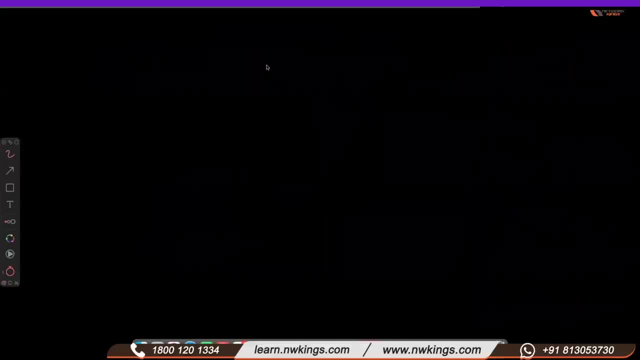 public pools: okay, got it where we need public ips. lot of public ips are needed when you are actually a big company. okay, so. so we got a public pool. let's take example 200.1.1.0 and this is a class c, so we always say slash 20.0. 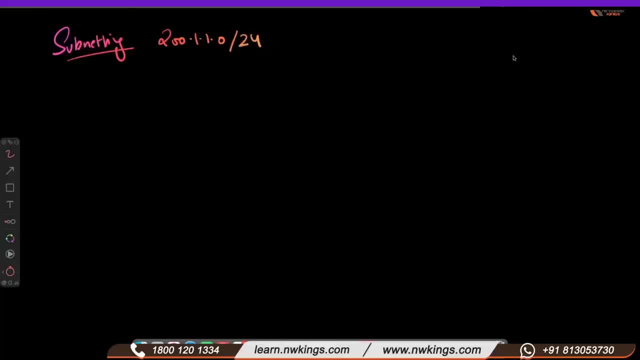 24. what is this 24? this is known as slash value. you can say that in a class we have how many network part one, so this is known as eight slash eight because it represents eight network bits. in b we have two n, so this is the reason we say this- 16, and in c we have three network part and this 888 is 24, so this: 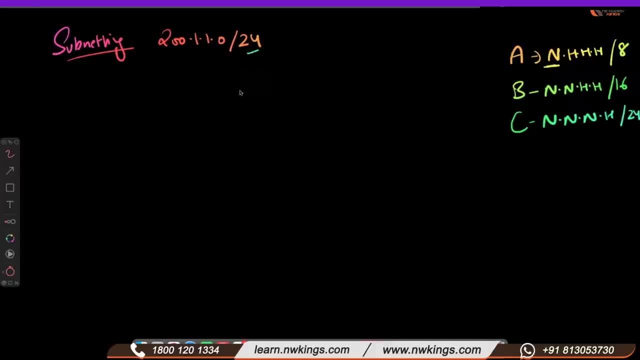 is the reason i have written here 24.. now i want to divide this network into four parts for my daily: mumbai, cheney and kolkata. location numero 32: 32, 32, 32, 3, 3, three, 3, 3, 4. 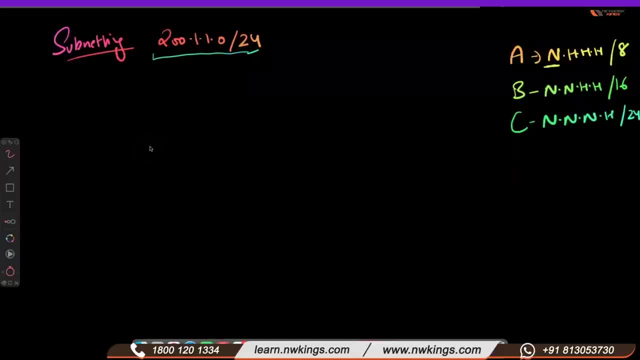 5, 7, this network into four so that i can use to my four locations: dilly, mumbai, chennai, kolkata, maybe, okay, yeah, rahul, correct. so how i'm going to divide this network. so it's very simple. so your ip addresses of how many bits- 32 bits, right. so what i'm going to write here in my. i have network bits. 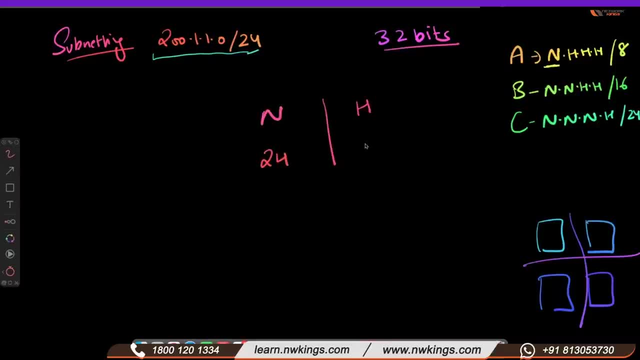 and then i have host bits. so i have total 24 network bits and host bits eight, right? so by default, how many ips we are getting to? the power of eight is 256 ips. i am getting right now with one. this network is giving me 256 ips. how i have calculated mine? 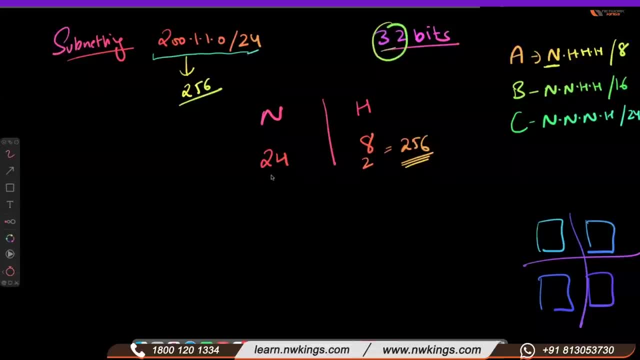 total ip address is of 32 bit. if class is 24, the remaining 8, 24 plus 8, is 32, right, yes or no? so the to the power of 8 is 256. so it means i am getting 256 address from one single. 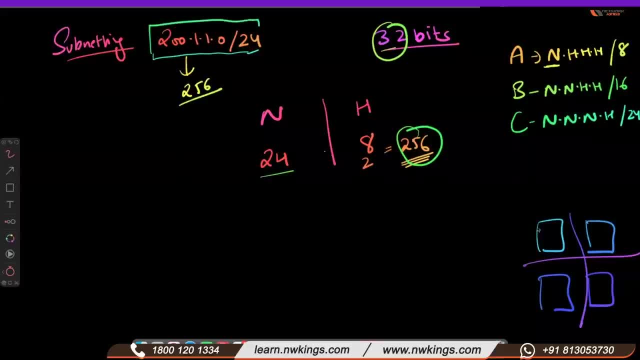 from this pool, but what exactly we are going to do? we want to give 50 to 60 ips, or maybe we want to divide this network into four parts so that we can give this one network. we can divide this into four parts so that we can give this to multiple locations. okay. 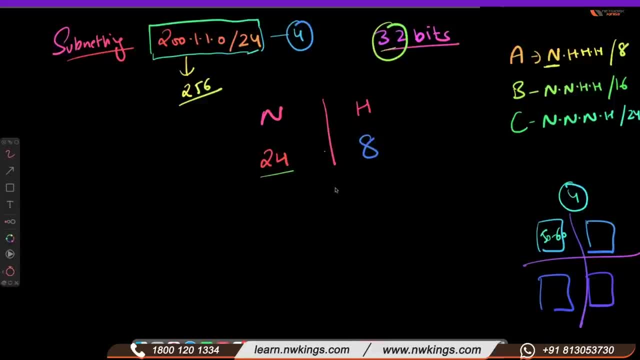 so i have eight host part. so tell me how many networks we want to divide into four parts. so i have eight host part. so tell me how many networks we want to create. so tell me how many networks we want to create, two or four? how many networks? 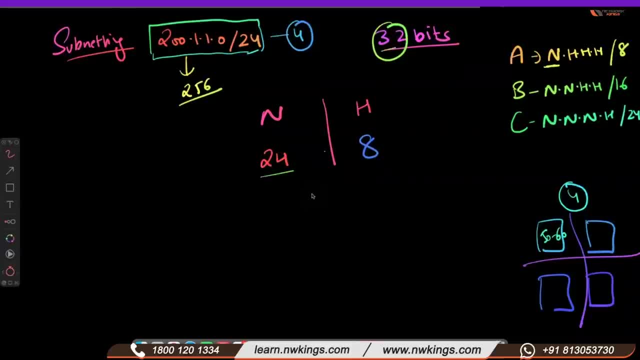 four right. darshan, you are in the class or not? yeah, so we want four networks means we want to divide this network into four locations. so tell me how we get four when we have to the power of two right. how when we get four when we have to the power of two right. 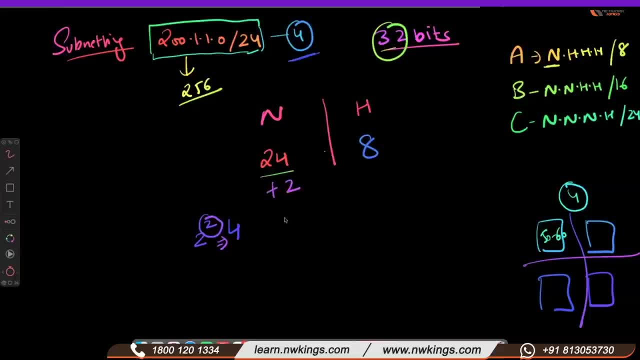 so it means we will add two here. it means we will have 26 here. okay, very simple. and from where we will get this two? when we will reduce two? here it means six host bits. so when we want to divide this network, we will add six host bits. so this is the third group. then we will use one host bit. 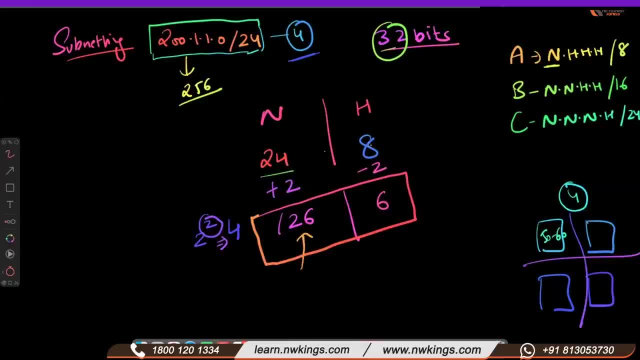 of this network into four parts. my network bits will be 26 now instead of 24 and i have reduced to here. why i have reduced this? because we need to balance it every time. i i need total 32 here, 26 plus 36, also 32.. i need to maintain this 32.. so you can shuffle the numbers from here and there. 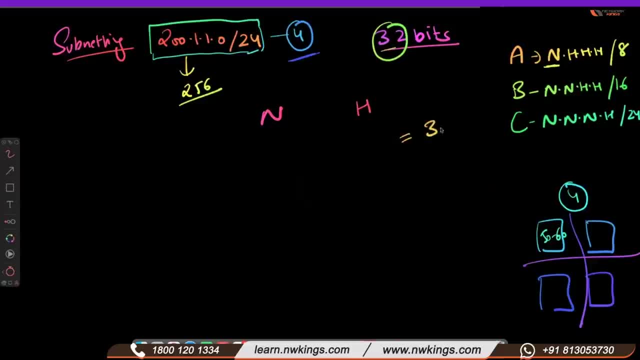 you can have one here and one there. so i will explain again how many networks we need to keep network bits we have by default in class C- tell me 24- and host bits 8. how many networks? we want 4 networks. so how I get 4 to the power of 2. so just check the power. so this is the power. so I 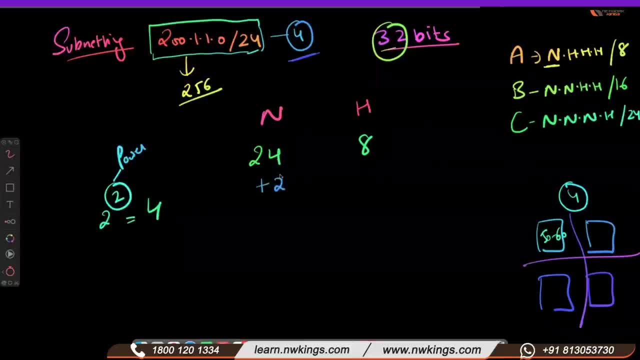 am going to add this 2 here. so because I want to increase my network bits. so that is 26 now and I need to reduce that 2 number from here because I need. I am going to change this host bits into network part, so this is the reason I am reducing 2 here. so I am getting 6 here. 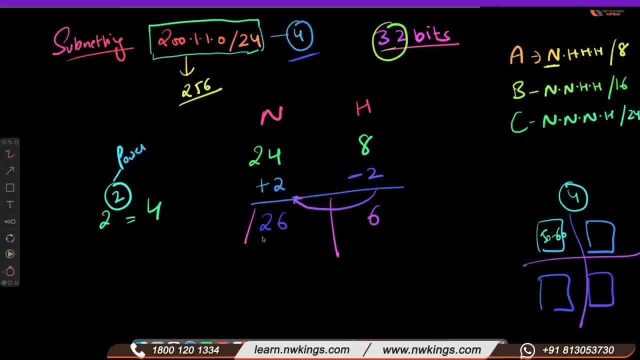 so it means I am going to have slash 26, and to the power of 6 is 64. so it means we will have around 64 IPs in every group. and what would be the network? the network would be slash 26. simple or not, right? let us take one another example. if I want to divide this network into 8 parts instead of 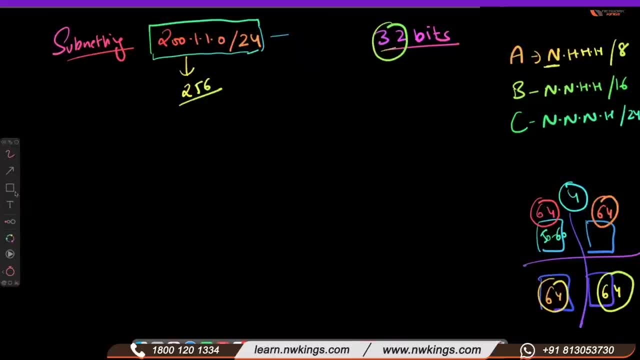 4 locations. right, let us take one another example. if I want to divide this network into 8 parts, instead of 4 locations, I have 8 locations instead of 4. we have 8 now. so, again, by default, 24. we have 8 here. so how we get. 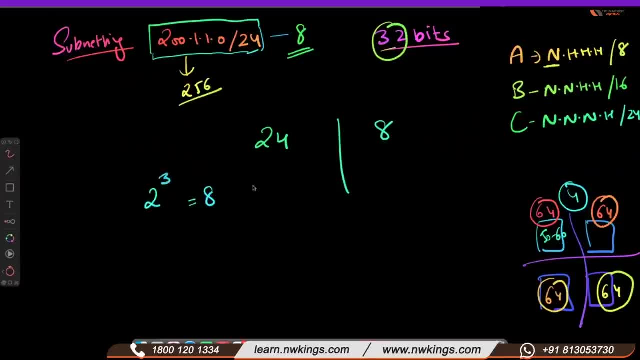 8 when we have to the power of 3. so I am going to add 3 here 27 and I am going to reduce 3. here that comes 5, so to the power of 5 is 32. so it means we will have 4- 8 groups. 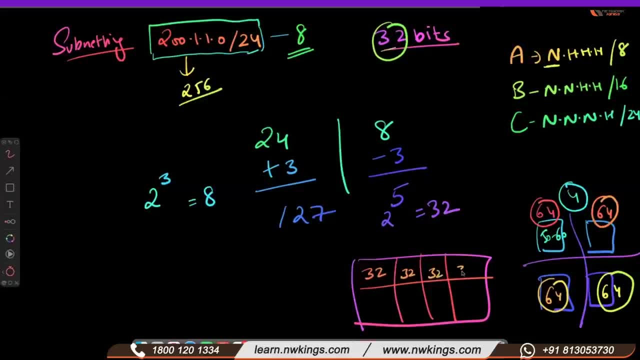 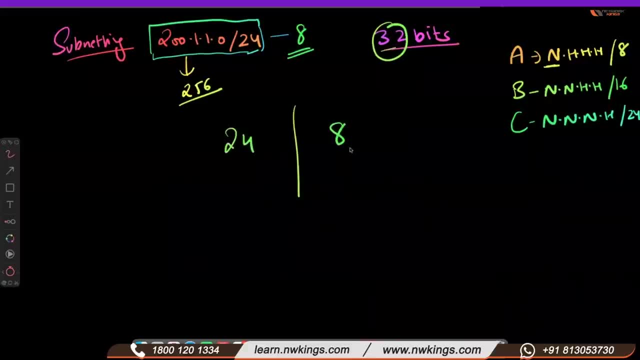 So again 24, I have 8 by default, so to get 4 my to the power of 2, so I am going to add 2 here 26 and I need to reduce here that is 6, right? so what is so when we are going to assign the IP, the first location suppose Delhi, so IP address would be 200.1.1.0. okay, so 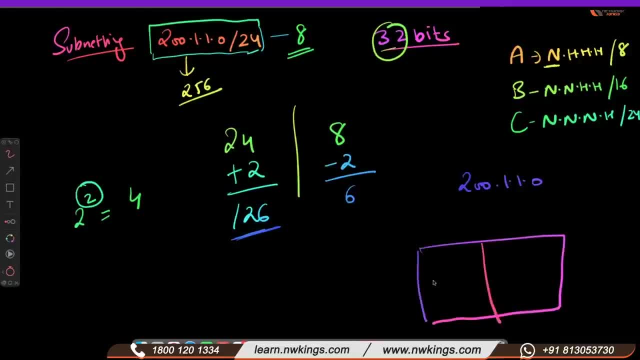 IP address would be 200.1.1.0. okay, so IP address would be 200.1.1.0. okay. so how you calculate your four locations there? how you calculate your four locations there, how you calculate your four locations? there is a simple maths. so IP address always. 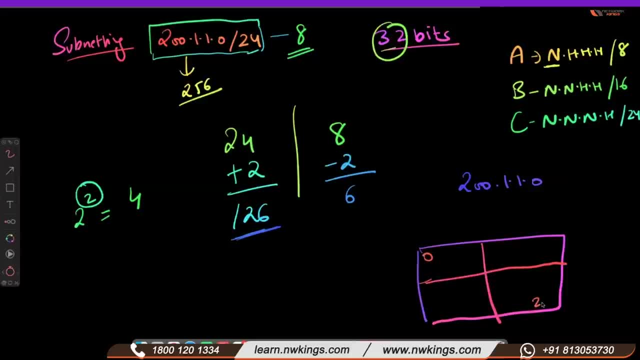 is a simple maths, so IP address always is a simple maths. so IP address always start with zero, okay, and it always ends start with zero, okay, and it always ends. start with zero, okay, and it always ends with 255 Deepak, if you have seven, with 255 Deepak, if you have seven. 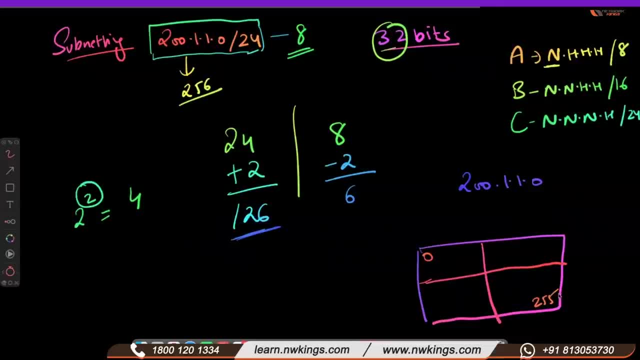 with 255 Deepak, if you have seven locations, obviously you need to divide locations. obviously you need to divide locations. obviously you need to divide the network into eight. you can't divide the network into eight. you can't divide the network into eight, you can't divide in seven or like that, so that also in the 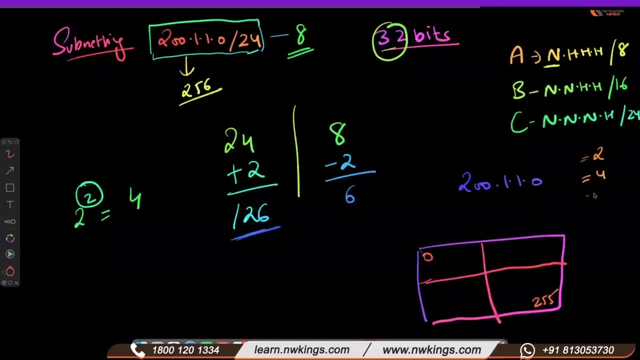 in seven or like that, so that also in the in seven, or like that, so that also in the increments of two either you can divide increments of two, either you can divide increments of two, either you can divide into two or maybe four or maybe eight, so into two or maybe four or maybe eight. so 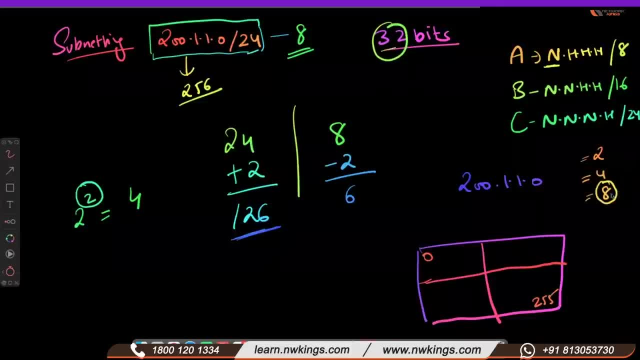 into two or maybe four or maybe eight. so if you have seven location, you can. if you have seven location, you can. if you have seven location, you can divide this into eight parts and you can divide this into eight parts. and you can divide this into eight parts and you can save one, a few IPs for future use. 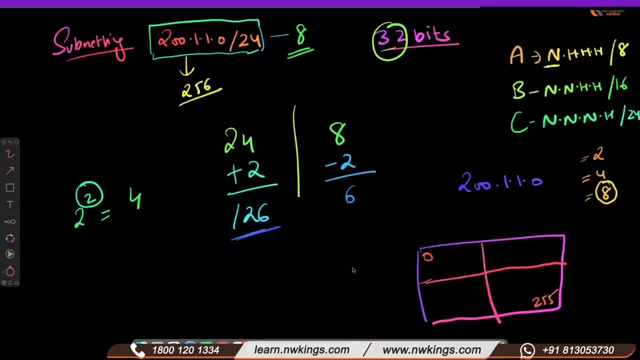 save one, a few IPs for future use. save one, a few IPs for future use. so it's like, yeah, so 26, so to the power. so it's like, yeah, so 26, so to the power. so it's like, yeah, so 26, so to the power of six is. 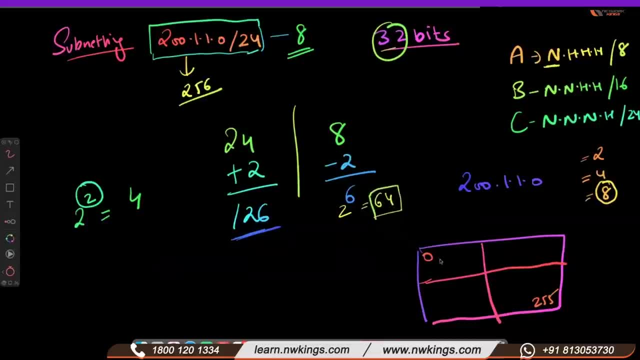 of six is of six is 64. so how i'm going to write this 64: 64. so how i'm going to write this 64, 64. so how i'm going to write this 64. so just add zeros within the starting 0. 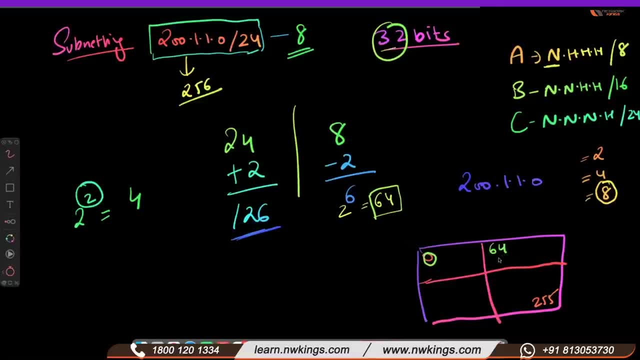 so just add zeros within the starting 0. so just add zeros within the starting 0 plus 64, 64 plus 64, 64, 64 plus 64, 64, 64, so again plus 64 plus 64, 128, so again plus 64 plus 64 128. 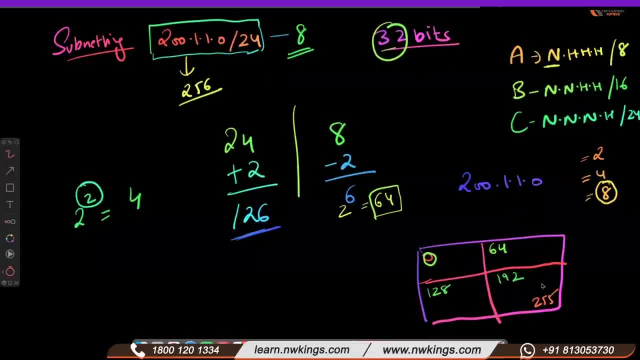 so again: plus 64 plus 64, 128, 128 plus 64, 192, 128 plus 64, 192, 128 plus 64, 192. so before 192 we get 191 before 128 we. so before 192 we get 191 before 128 we. 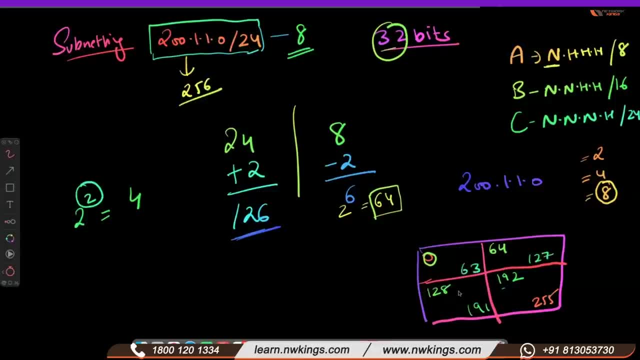 so before 192 we get 191, before 128 we have 127, and before 64 we get 63 have 127, and before 64 we get 63 have 127, and before 64 we get 63. so this is how. so this is how. 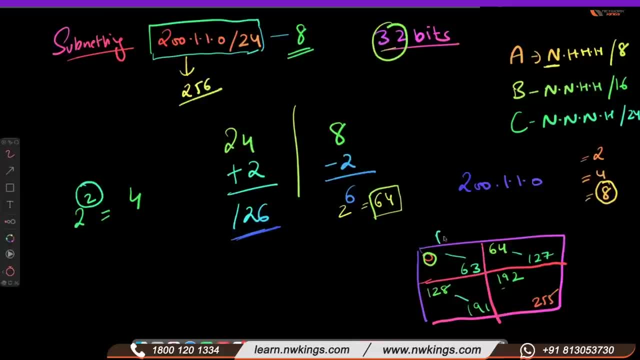 so this is how. so the ip address from 0 to 63, so the ip address from 0 to 63. so the ip address from 0 to 63 will be placed in delhi, will be placed in delhi, will be placed in delhi. so here we are going to assign in mumbai. so here we are going to assign in mumbai. so here we are going to assign in mumbai, here, this ip we are going to assign in here, this ip we are going to assign in here, this ip we are going to assign in chennai, chennai. 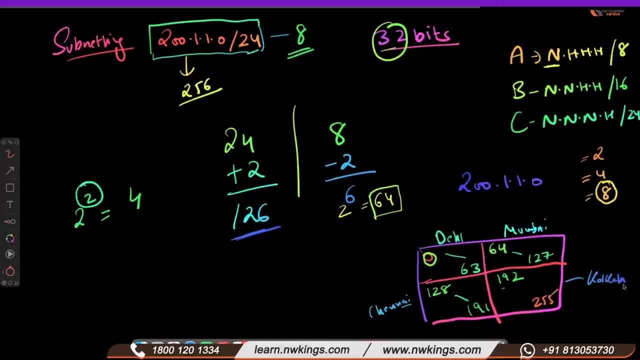 chennai. and here this network i am going to, and here this network i am going to, and here this network i am going to. assign in kolkata, assign in kolkata, assign in kolkata. got it very simple: now, now, now, yeah, so now how i am going to assign ip. 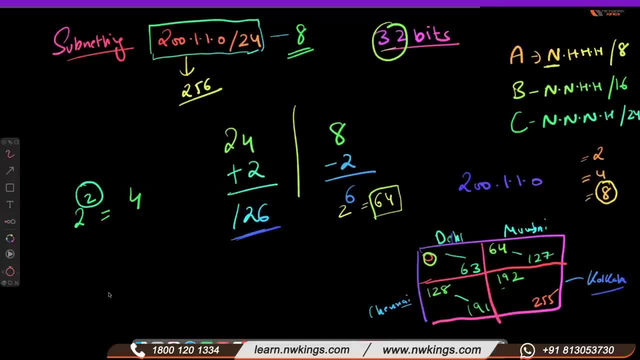 yeah, so now how i am going to assign ip. yeah, so now how i am going to assign ip: addresses in delhi, addresses in delhi, addresses in delhi. so when we are going to assign ip, so when we are going to assign ip, so when we are going to assign ip addresses in delhi office, or maybe the 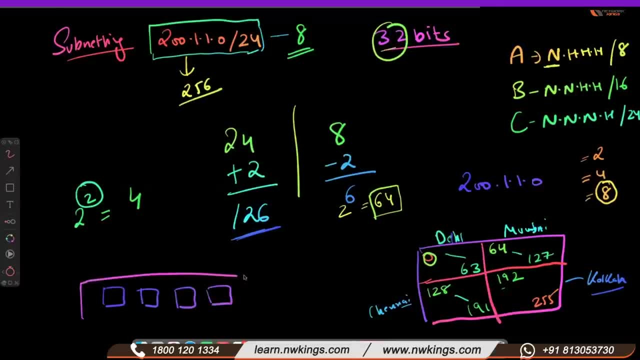 addresses in delhi office, or maybe the addresses in delhi office, or maybe the servers in delhi, servers in delhi, servers in delhi- what, what, what, how i am going to give the ip address in. how i am going to give the ip address in. 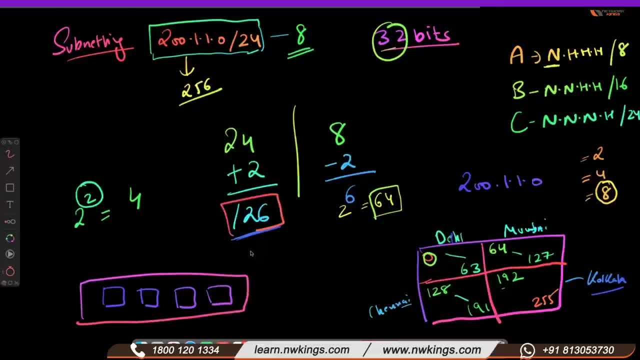 how i am going to give the ip address in computer, computer, computer. how we write this 26 in computer, how we write this 26 in computer, how we write this 26 in computer. because, because, because 24 is very easy, we can write two, five. 24 is very easy, we can write two, five. 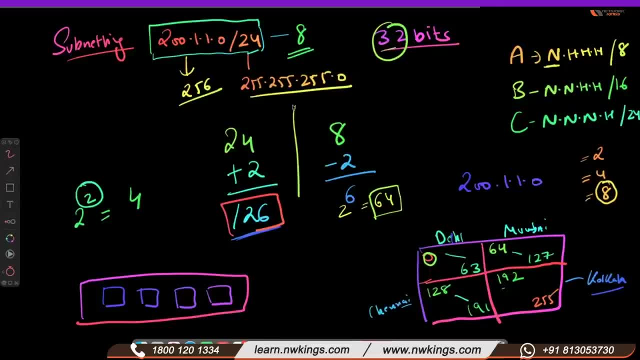 24 is very easy. we can write: two five five, two five five, two five five dot zero, five, two five five, two five five dot zero. so this is 24. but how i am going to write 26, i am going to show you. you have written down all this. can i move a bit? can i remove this? 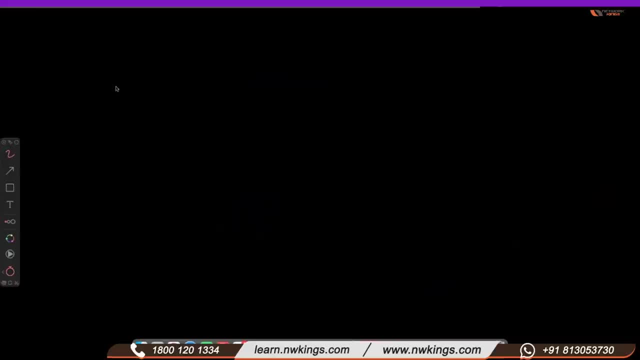 okay, yeah, see, understand subnet mask. so by default we get subnet mask 255.0.0.0. if, uh, your slash value is nine, how are you are going to add here? so again, that thing comes with the to the powers. so your one network will be represented with the powers. 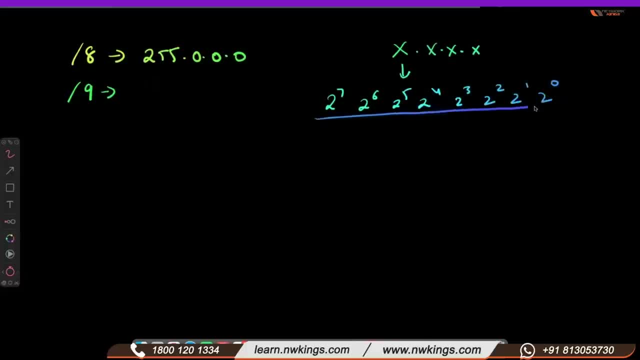 so you have, every block is like this: so this block also, this block also, this block also. so in the first block if you have eight, so it means one, two, three, four, five, six, seven, eight right. so this is first portion. and you get two, five, five right. so eight right, two, five, five. so when we have nine, so what we have, 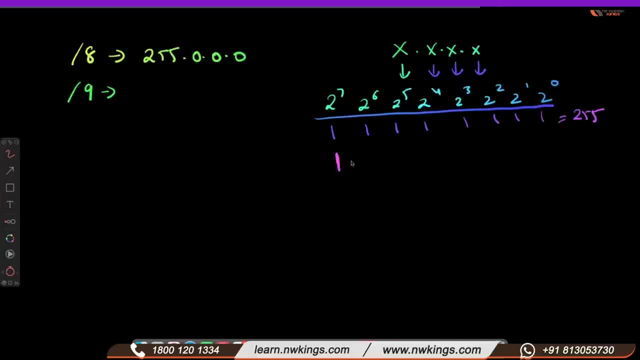 so in the first group we have eight plus nine, so again one. so rest all zeros, right? so two, five, five, and here above one we get to 128. so that means 128.. so it means we will have two, five, five, 128.0. so when we say 10, what will happen? so when we are going to solve for 10? so that means 8. 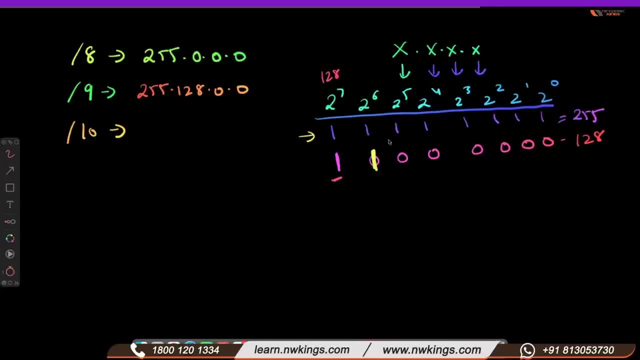 this covers eight, and here we need to add one here. so one. this is two five five, and just plus these two values on top of a 128 64, that comes 192.. so in here we are going to get 255, 192.0.0. 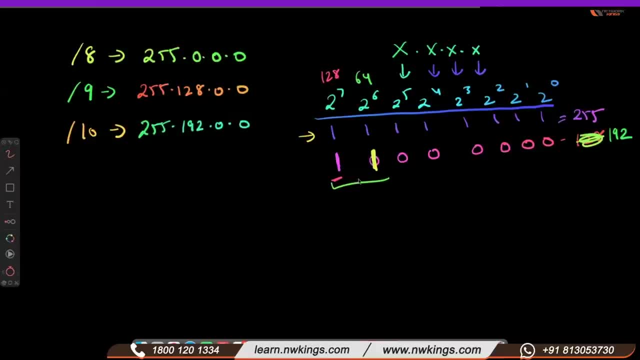 so i'll give a very simple formula. you don't have to calculate every time. so whenever anything, when we add one bit, you always add 128, when we get two, 192.. so when we have three network, three ones, we always get 224.. for four bits, we get 240. 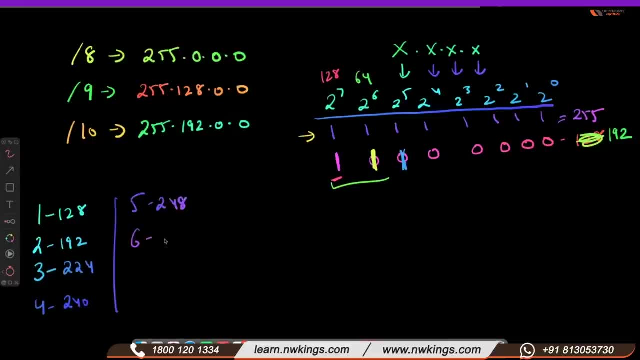 so for five bits we get 248.. for six bits, we get always 252.. for seven, we get 254.. and for eight, always, we get 255.. just write this and you will understand. subnet mask. now, if i'm calculating slash 14, what you will do: 8 plus 6 is 14, right, and you know always, 8 means 255 and 6 means 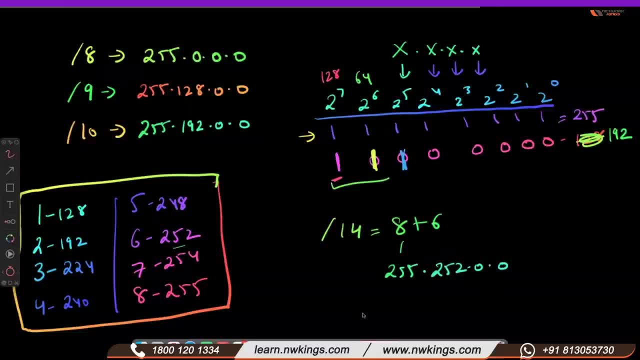 250, 2.0.0. let's slash 19. how you calculate? 19? 8 plus 8, 16, 16 plus 3, so 255. 255 and 3 means 224.0. just write this one. so what was the value we got in last question? slash 26, so 8 plus 8 plus 8, 24 plus 2, so that. 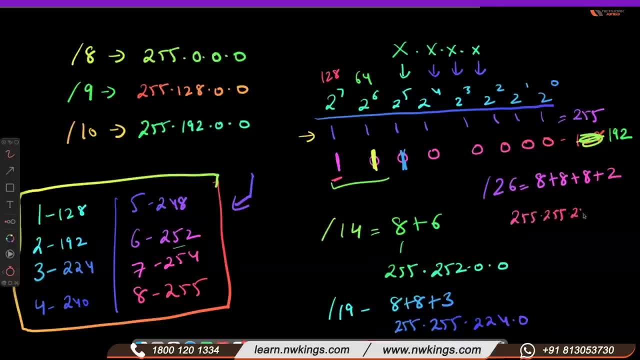 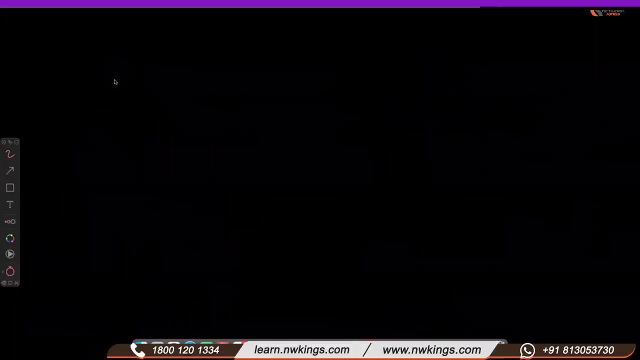 means 3255 and for 2 we get 192. so that means 3255 and for 2 we get 192. so in our last question, all computers in my daily location will have this subnet mask. okay, cool, hmm, so you can solve this for B also. A also like that, okay. 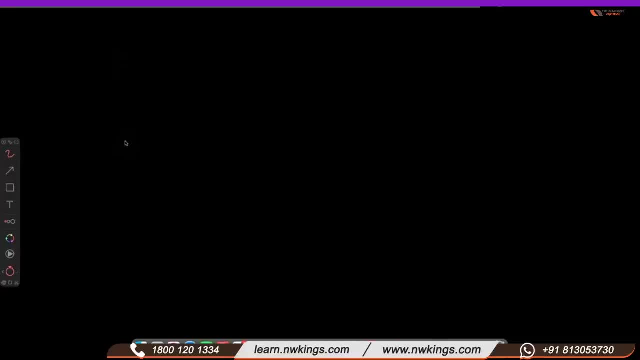 so, guys, let's take 5 minutes break, okay, and I'll come back. so, guys, let's take 5 minutes break, okay, and I'll come back. so guys, let's take 5 minutes break, okay, and I'll come back. okay, hi. so so, guys, we are going to do one practical now. 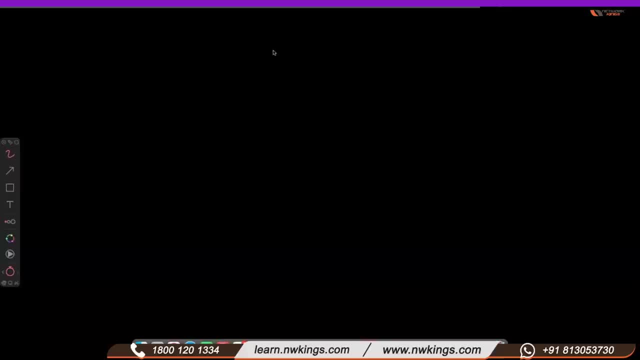 okay. so what i'm going to do, i'm going to connect to one router with one network. okay, maybe i have one or two pc here. okay, and here also i have another pc, okay. so if my computer ip address is 192.168.1.1 or maybe 1.11 and here i have 192.168.2.11, 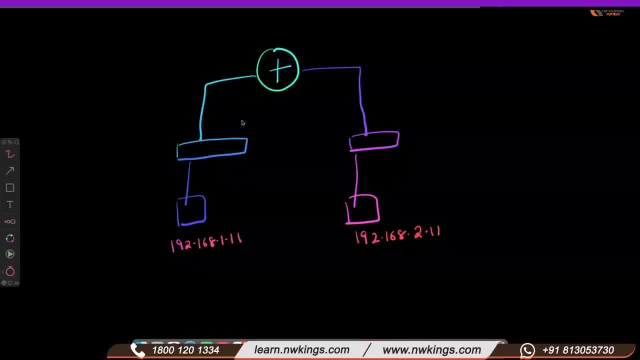 so tell me if they are able to communicate. if i have cable like that, okay, so i'm going to connect to one router with one network. okay, so i'm going to connect to one. just forget, we have router, so tell me if they are able to communicate. no right, so we need a device which actually connects. 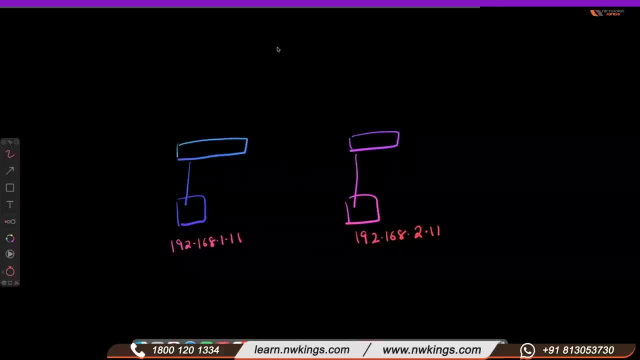 two different network and that device is known as router. so we are going to connect a cable with this router and when we add a cable in this device, so we need to give ip address here also, so we can give the same ip address where we have this network, 192.168.1.1. i am going to give here and here in another link. this is a. 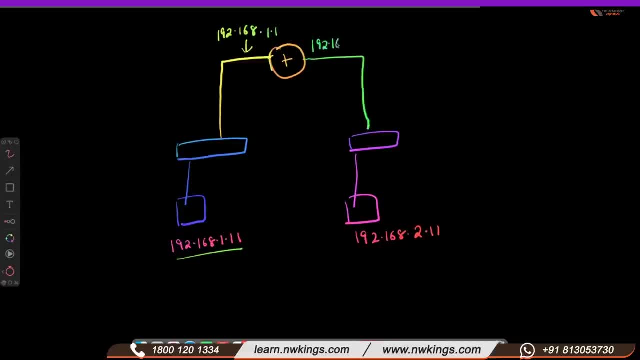 separate link in router. here i have to give 192.168.2.1, so it means a router will have two ip address. so this is the work of routers: to connect different networks. to connect different networks. we use this device okay, and computer will have subnet mask by default- 255, 255.0, and computer always have a default gateway. 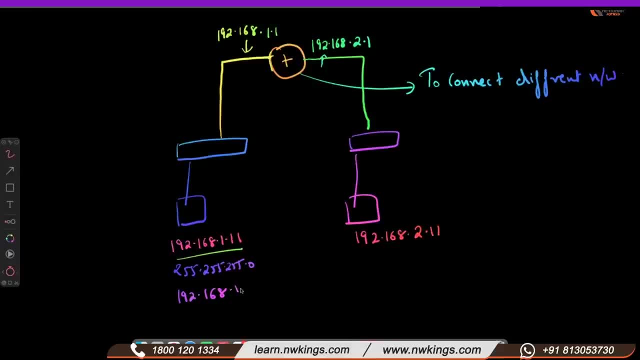 what is gateway? exit point of lan is known as gateway, so i'm going to assign 1.1. so that is my router ip, because if computer wants to go outside the network they are going to use, this is a gateway for that lan network. so this is going to be a gateway for that LAN network means when 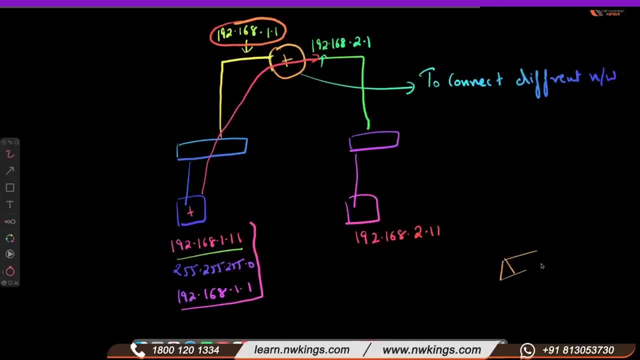 processes and like andThen. when you this is your home or something, right, so, suppose, and you want to go outside, so you always use the gate right so that paper your. so this is my gateway for you, this is my gateway. I see, So this is my gateway, so this is my gateway. or I don't want to go outside the game, right, so you always use the gate right so that you can exit and you can enter from this gate. so It's like that when a router episode is working as a gateway for you, so this is my, it is, this is my gateway for you, Because it connects two different networks. 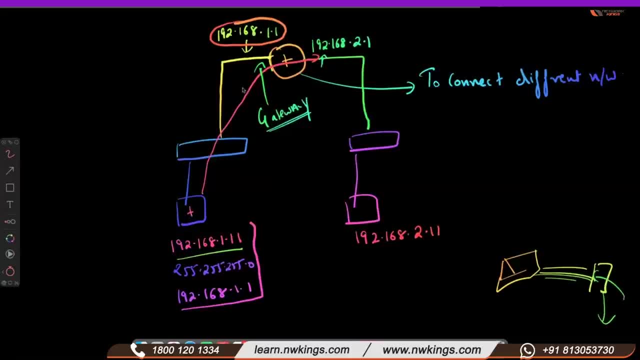 gateway connection. often it work. i am going to use the router ip as my gateway. okay, so somebody asked me like: so what is the difference between gateway and router? so router is a device, that is hardware, and router can have multiple gateways for each LAN. so this device will have this ip address as a gateway. 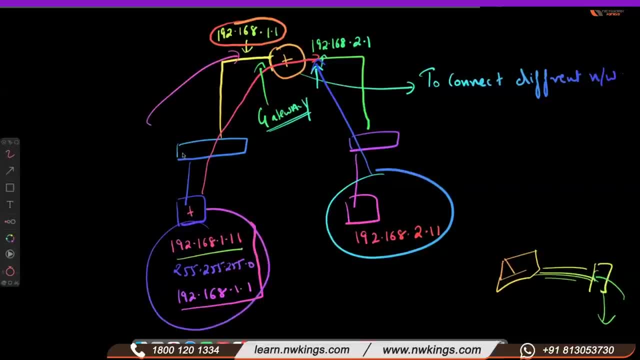 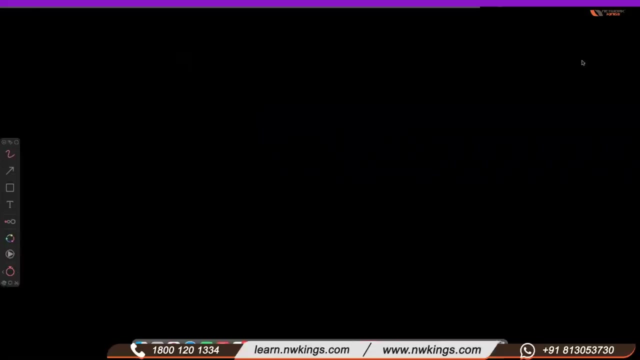 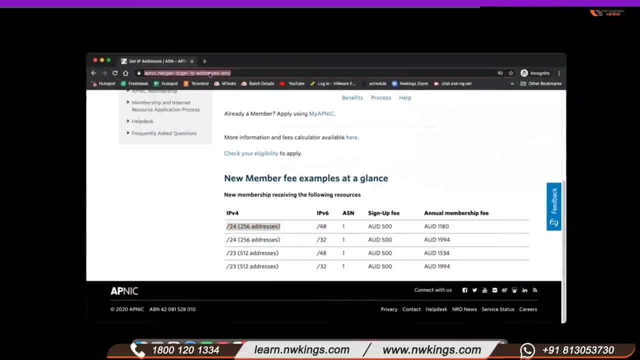 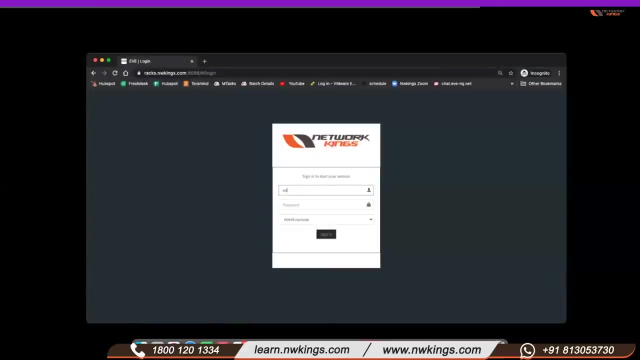 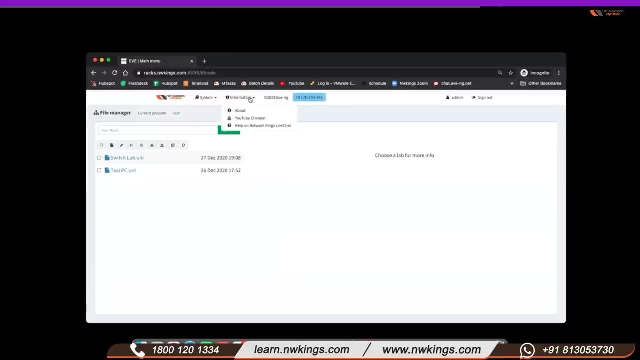 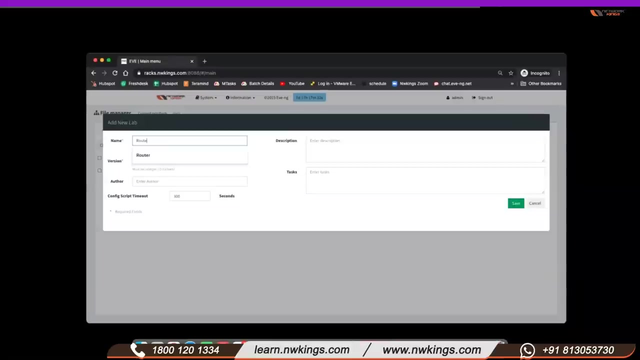 and for this computer, this ip address will work as a gateway, just exit point of the LAN. exit point of the LAN is known as gateway. okay, so let's go and create a lab. so i am going inside racks with 8086, so i am going to create a lab. 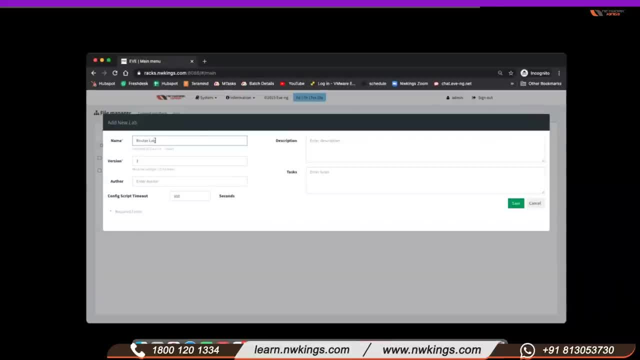 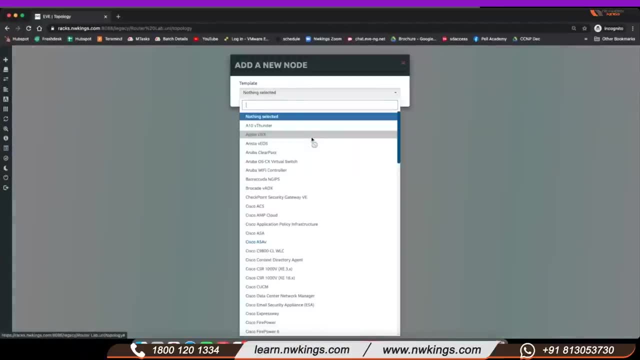 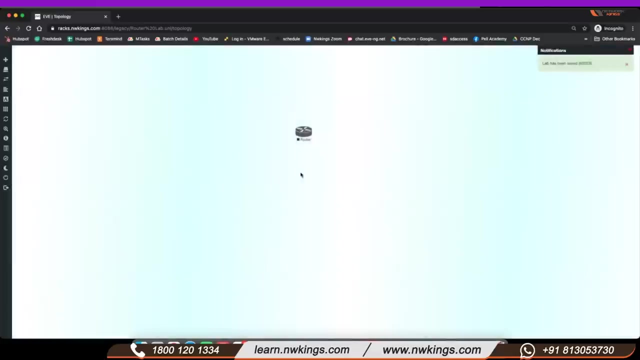 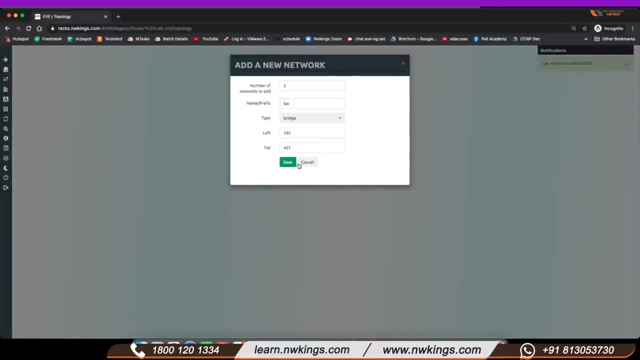 so i will name it router lab. okay, so here i am going to add a device. let's take this device, so this will work as: so i have router, so i have router, so i have two switches and i have two machines. so i also want to create some. 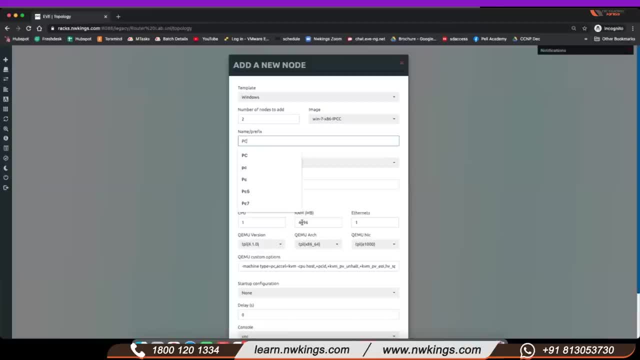 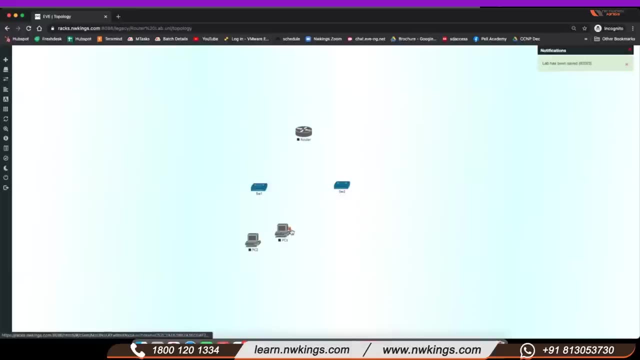 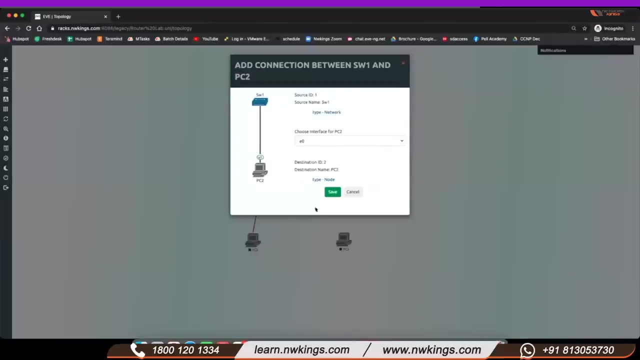 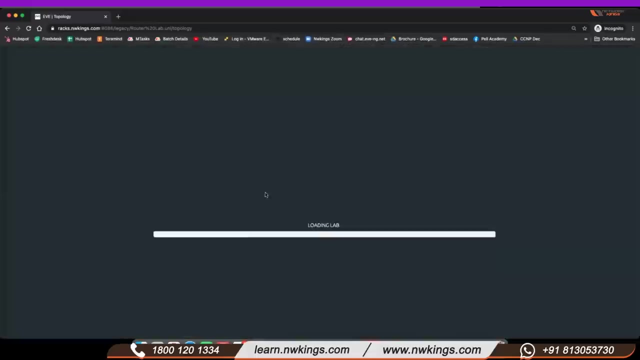 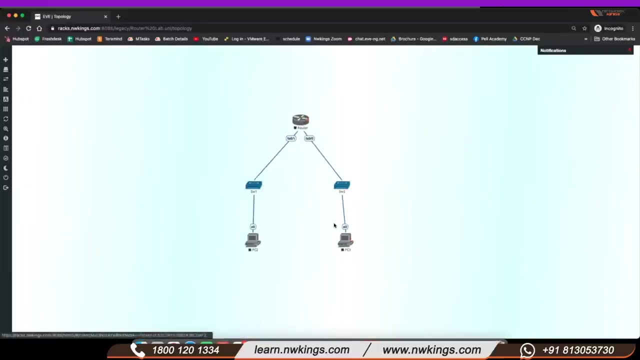 apk. so i want to create a total star. ok, so i'm going to create a COIN, So the same lab you can do in your lab access. So this is the lab. so I am going to start this router and before doing this, I am going 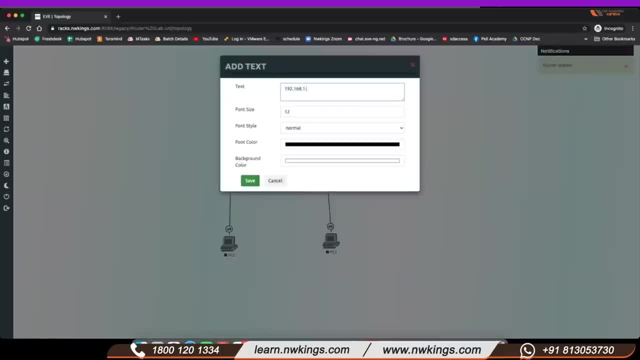 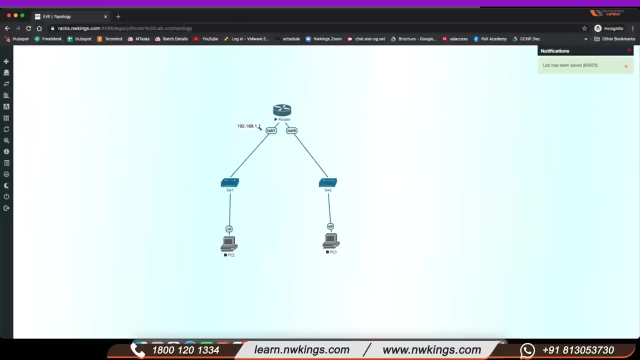 to type here the IP address. I am going to use 192.168.1.1,, here I am going to use 192.168.1.1 and at the below machine I am going to assign 192.168.1.11.. 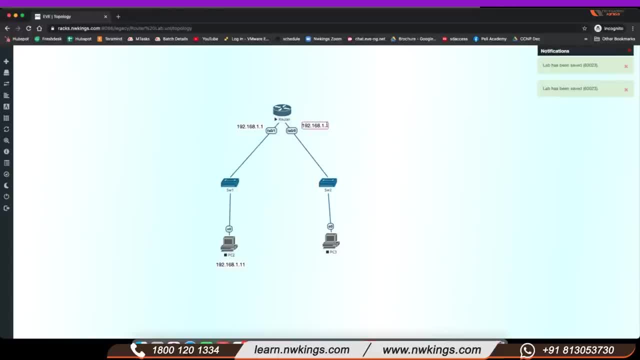 On the another side of router I am going to use 192.168.2.1, and here I am going to have another IP that is 192.168.2.2.. Ok, So from more action, start all devices. ok, so my all devices are up. ok, so I will open. 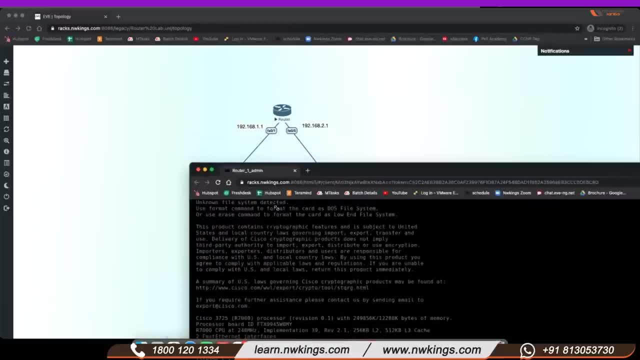 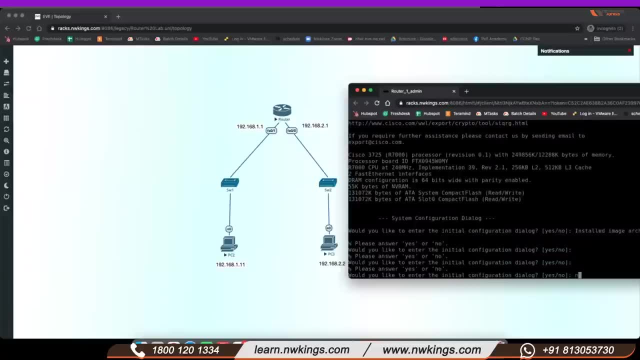 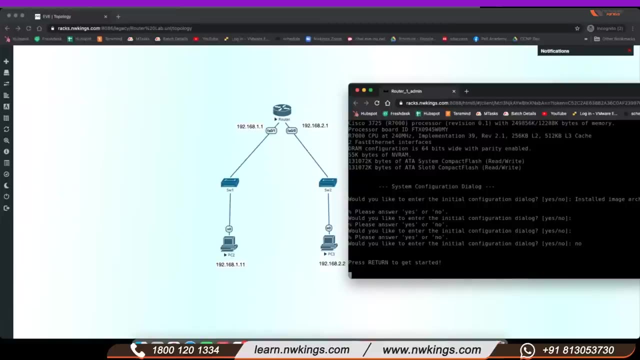 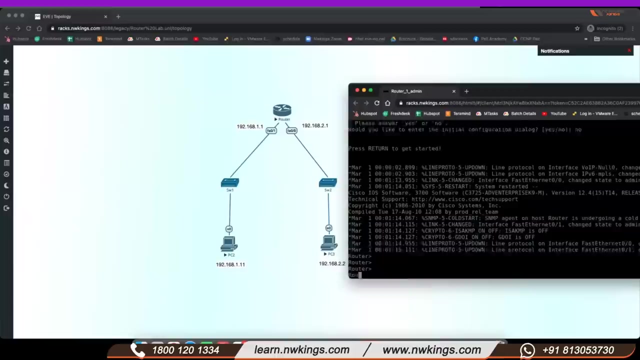 this router. ok, so this is my router. so I will always say no in the configuration. ok, so we will assign two IP address and you can see there FA01,. so what is this? I will show you. So once you login into your router, you are into by default which mode, user mode, and which. 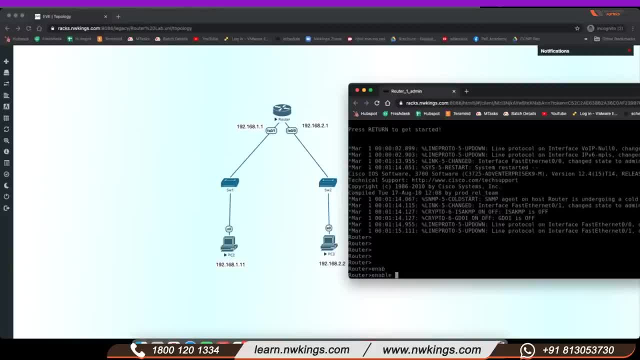 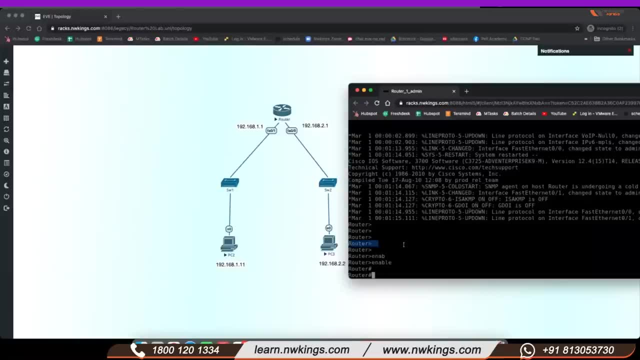 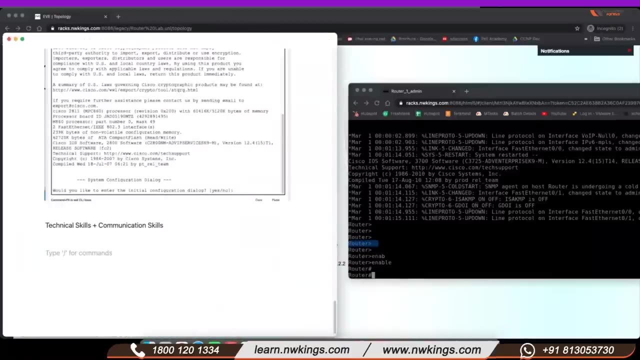 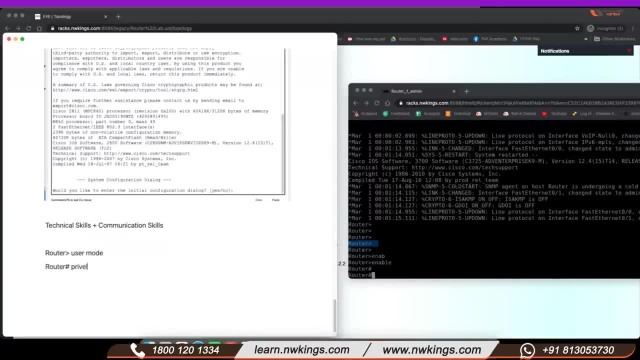 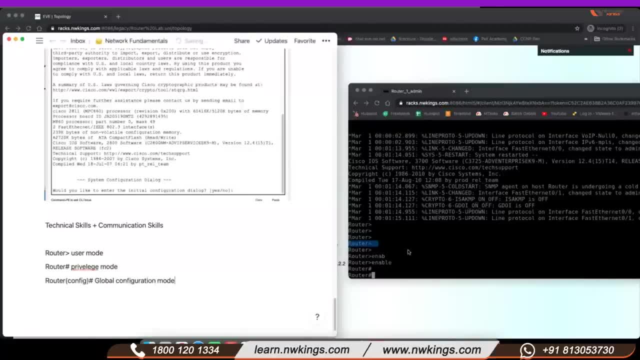 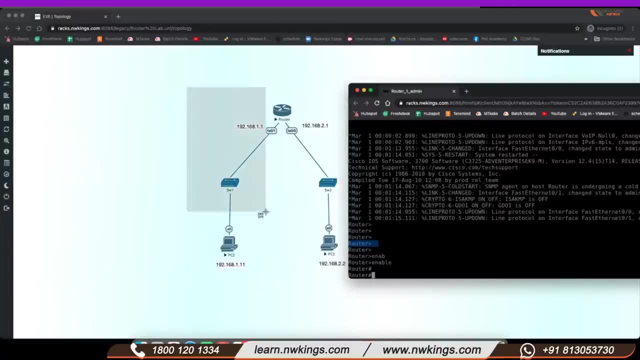 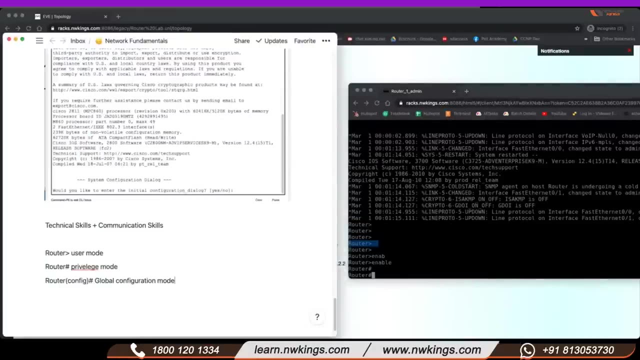 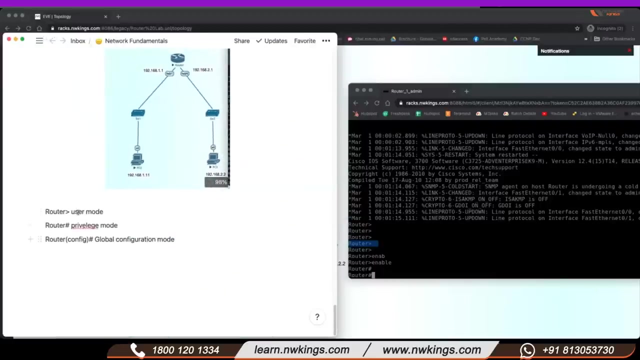 global configuration mode: Ok, Clear, Clear, Ok, Ok, Ok. So I am going to create a lab here so that you can do this. Okay, so what I am going to do? I am going to type the commands over here so that you can write the commands. 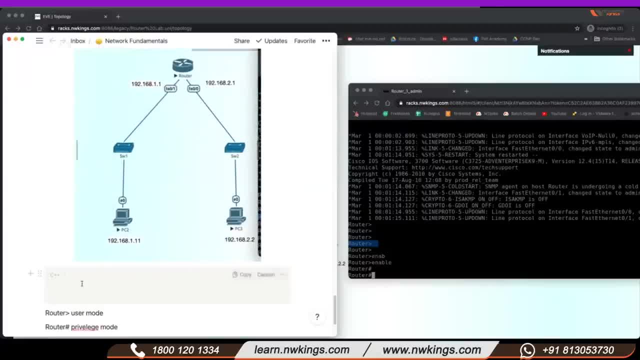 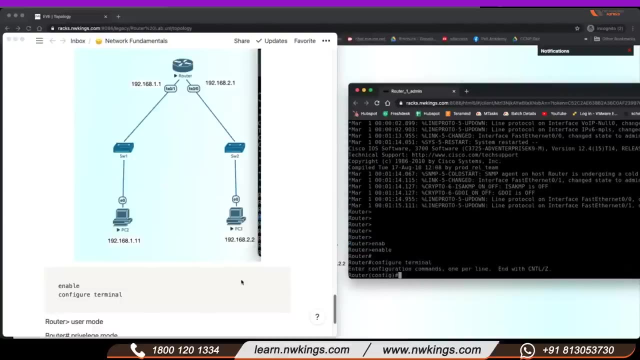 So first of all I need to enable the device, then I have to go configure terminal. So this is the command: to go into my global configuration mode: configure terminal. Okay, so now you are into global configuration mode. So after that, if I want to change the device name, so what is the command? 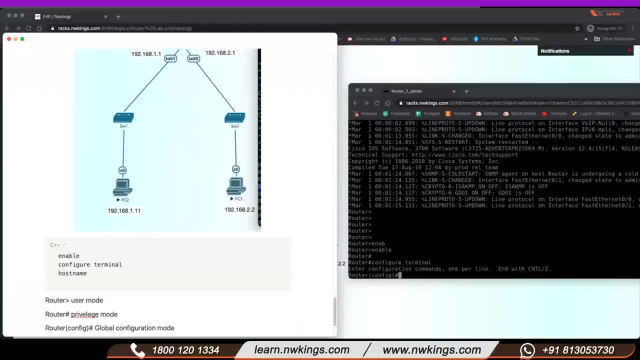 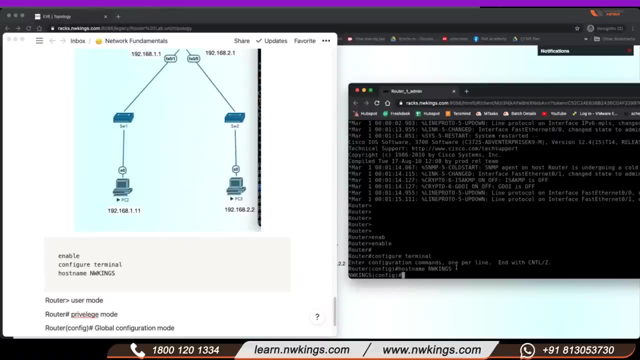 Host name. So my router name is router, So I can name it NWKings or something. So I will write host name NWKings So you can see. you do not have to commit anything directly. The things are changing here. 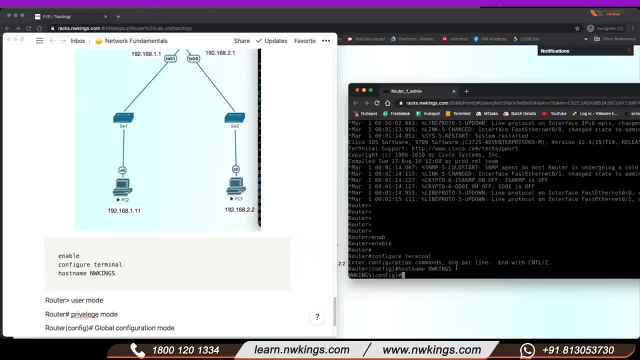 Okay, so in advanced routers or maybe if you work in Cisco ASR or Big Series or even in Juniper and all, So you need to save the things to enable the changes. But in Cisco normal devices, Whenever you do any change, it will not ask for to save the configuration to do the changes. 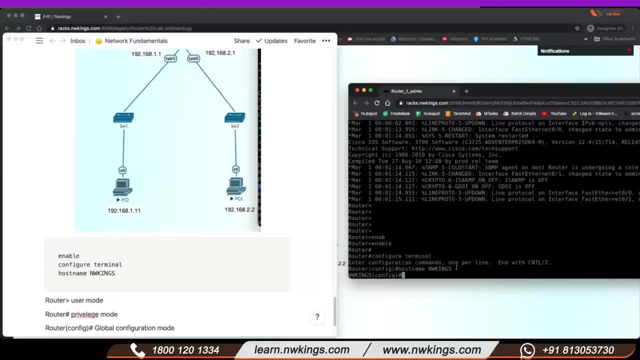 So whenever you type any command, it automatically changes Means. I have given a command host name: NWKings, and you can see the prompt here: NWKings, Right. So now I want to give IP address to this router. So this is the interface. 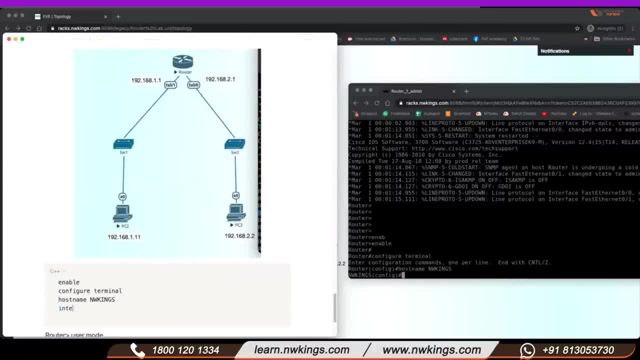 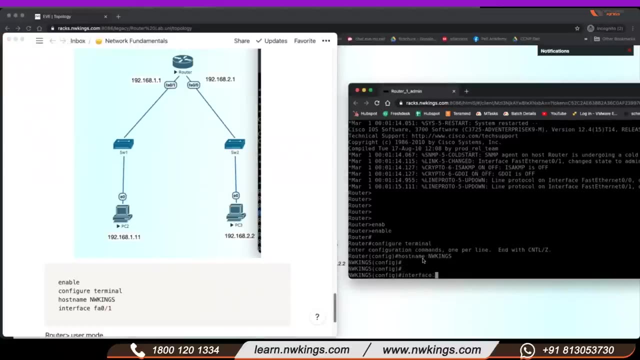 What is this? This is the interface. So I will type interface. Router ports are known as interface Interface FA0, slash 1.. So you can see FA01.. So I will type interface FA01.. Harishika, that is in Cisco. 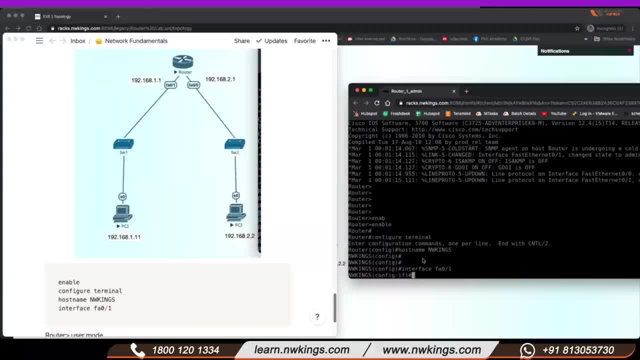 So it actually? it is like that only This is the reason we love Junos. Okay, So interface FA01.. IP address: 192.168.1.1 and with subnet mask. Just check here, guys. I am giving IP address and then subnet mask. 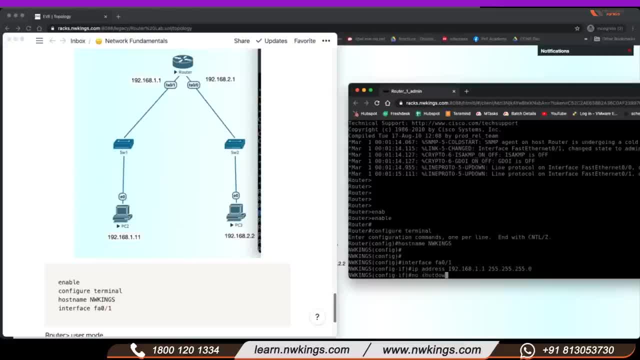 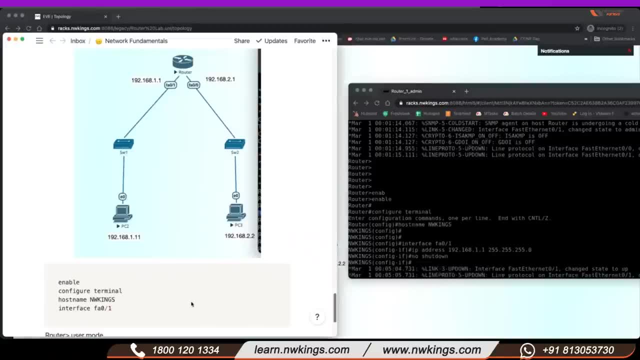 Just click enter and you need to give a command no shutdown here. So why we are giving this no shutdown command? So that we can enable. We are going, We are giving a command to enable this port. Okay, This is like enable, disable your port. 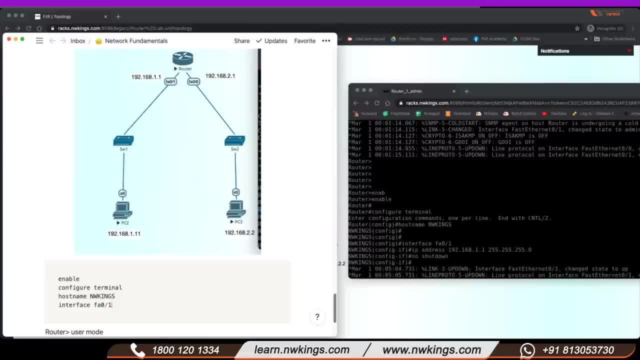 No shutdown is a command to enable the device port. So IP address: 192.168.1.1, 255.255.0, no shutdown. Okay, So tell me what would be the command for next giving IP address to another interface. 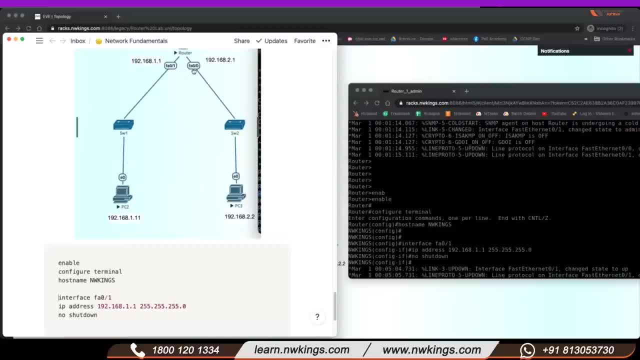 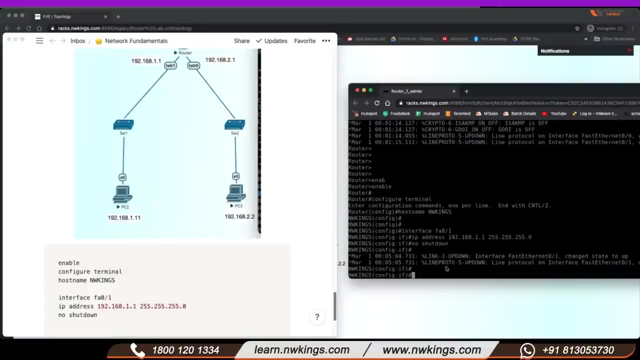 That is FA00.. Just type in the chat, It is FA00.. Yes, correct, I need to go inside again. Interface FA00.. Okay, IP address: 192.168.2.1, 255.255.0.. 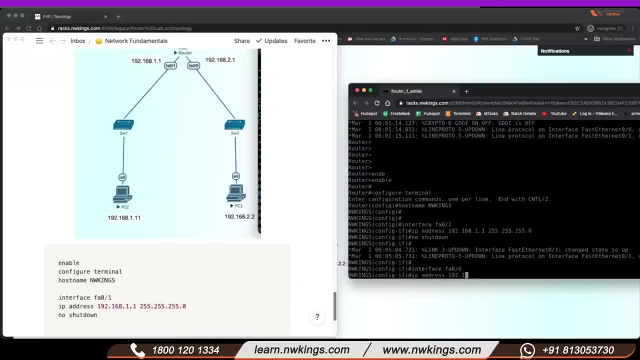 Okay, IP address: 192.168.1.1.2, 255.255.0.. Yes, correct, 168.2.1, three times 255 and again no shutdown, right, so the same way you are going to give the. 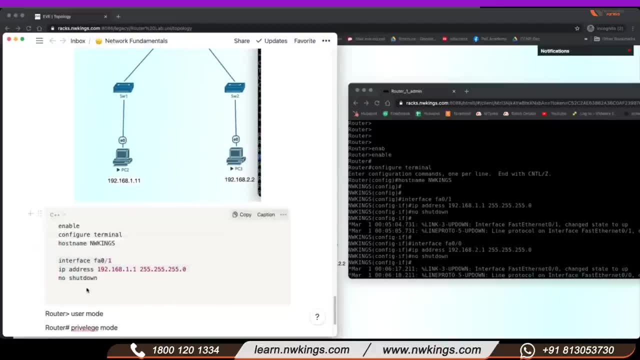 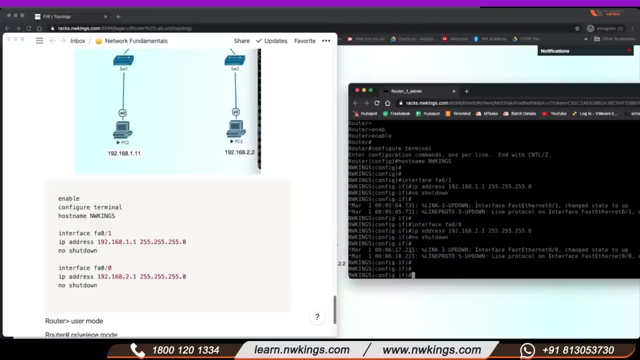 command interface fa00 and i'm going to type 192.168.2.1 and click on no shutdown and your ipad so you can see some messages here. you can see here change state to up. so it means the interfaces are up now. and how to check my interfaces are up or not you need to go back. 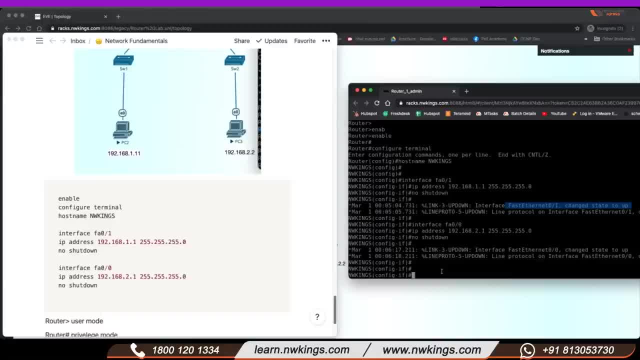 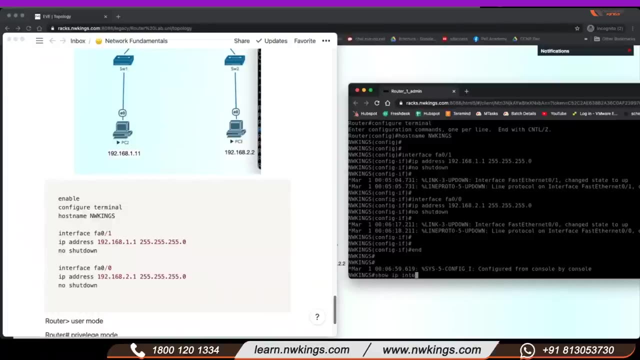 into privilege mode. so how to go back directly to privilege level? you can just type end, end or you can give exit two times. i'm giving end, so directly i'm into privilege mode. so now i'm going to type: show ip interface brief. this is the command to check if i have. 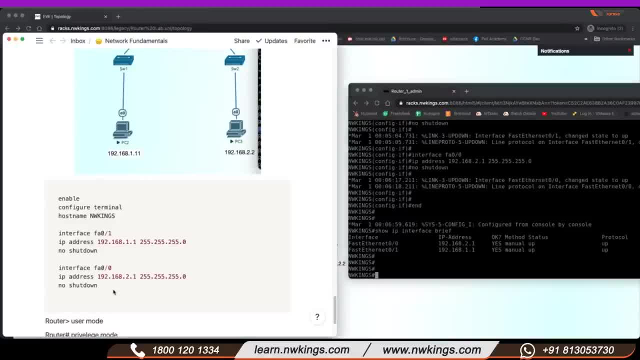 given the correct ip addresses or not. so tell me if i have given the correct ip addresses. okay, so router makes a table that is known as routing table. what is the command to check routing table? so i'm going to type: show ip interface brief. this is the command to check. 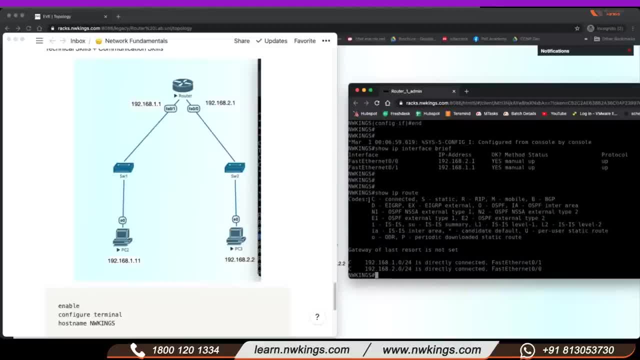 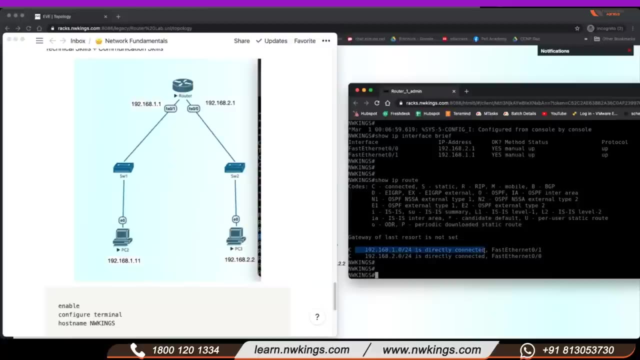 routing table: show ip route. so there you can see a lot of codes. that is for different, different protocols like eigrp, ospf, rip and all. but as of now we are not connecting multiple routers, we are working on one router and both the networks are connected to my router and it is showing you. 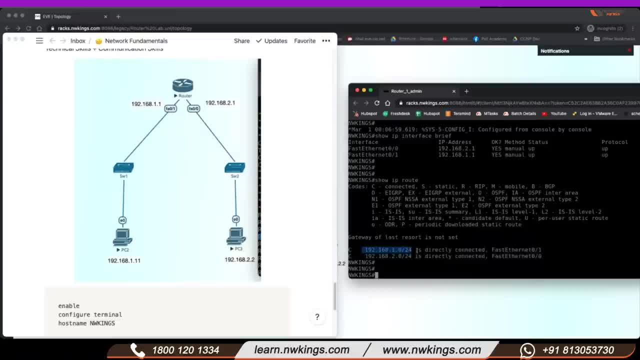 my 192.168.1.0, but i have given ip 192.168.1.1. but why this is showing me 192.168.1.0 is because i'm going to type 192.168.1.0 and it is showing me 192.168.1.0. and it is showing me 192.168.1.0 and 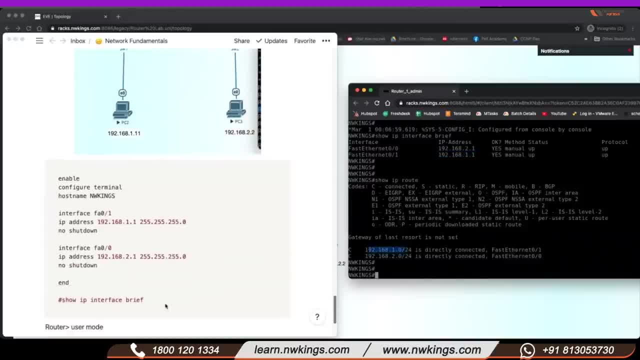 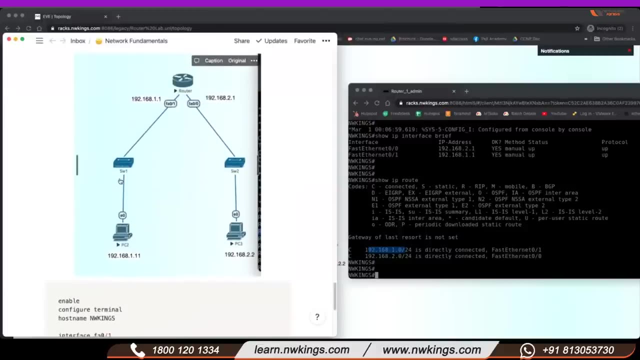 dot zero because router only saves network id. so what are network ids? so network id is like house of ips, like see, i have one computer, maybe you have 100 computers. so router would not save 100 computer ips in its routing table, it only only saves the house of ip address. or you can say that: network id. in networking terminology, network id means all ip belongs to this network. because when we will have another router, okay. when we will have another router here, yeah, when router is going to connect with another device further. so router is going to share not 100 computers ip address. instead of sharing, it is going to share only this network to this router. 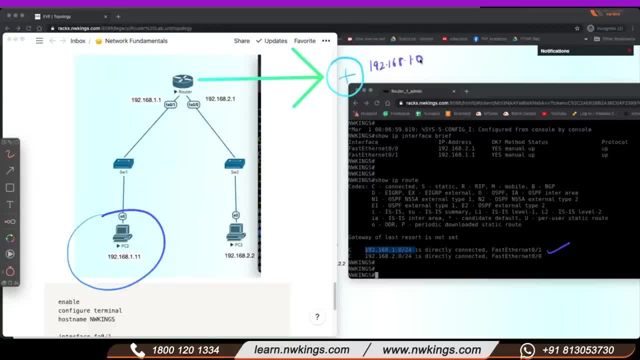 and router will have 192 168- 1.0 and we have another network. maybe you have one ip or maybe you have 100 ips or 100 computers here. so router is going to send 192 168 in 2.0. so instead of sending all host ip addresses, i am going to send my network ids, so these are known as 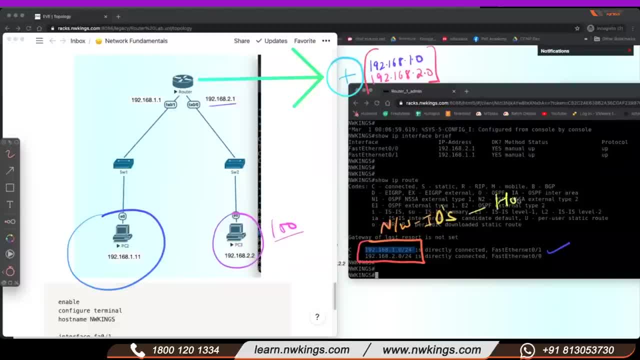 network ids. so that means house of ips. so that term you can't use it. this is just for your understanding. but in interviews or somewhere you can always say network ids, why we using default submitting? because this is the first network ip address. so network ids is a very, very practical of a router and i 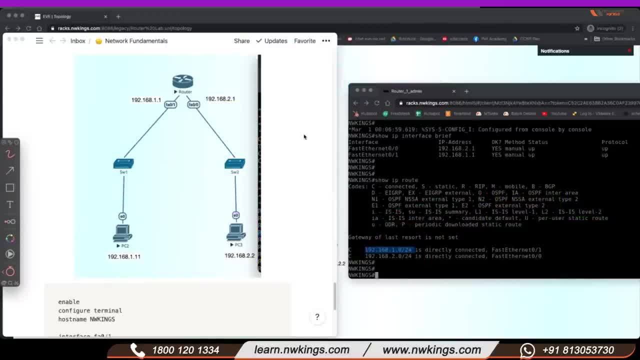 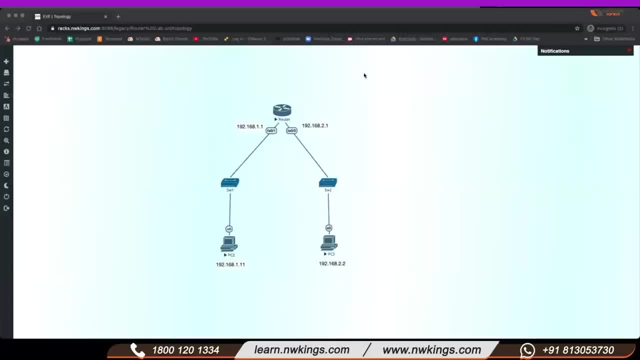 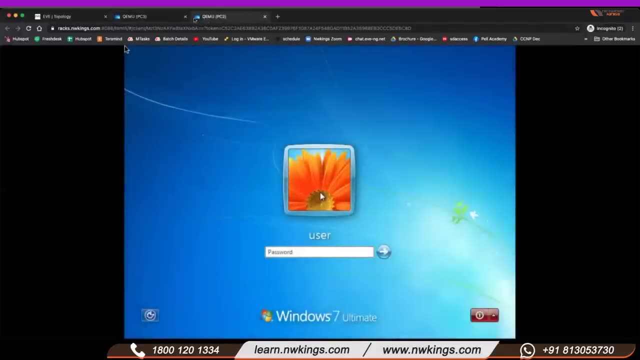 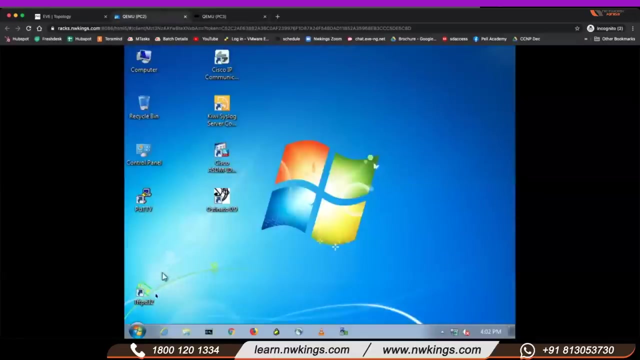 don't want a confusion, right, so that you will get confused. so let's go and give the ip addresses to computer, right? so very easy, just open the computers in your lab. so somebody was asking me what is the password. i have windows, test123, test123. but the first t is in uppercase. okay, test123. 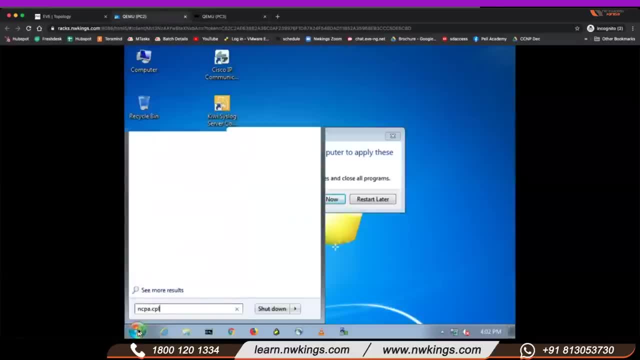 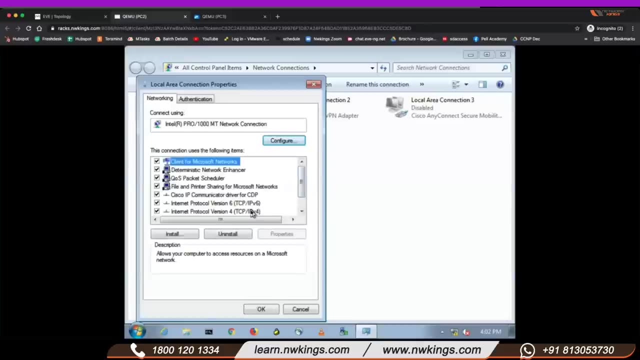 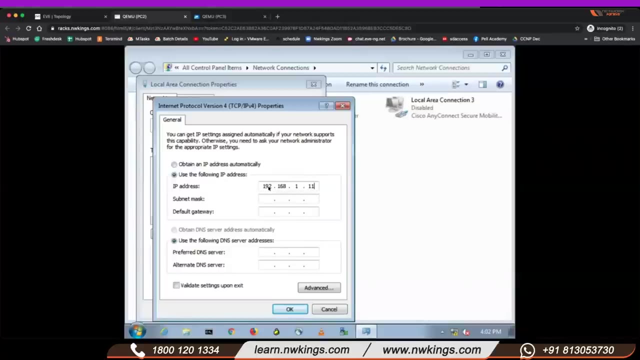 so in my first computer i need to go under ncpacpl and here i need to give in properties what would be the ip address 192.168.1.11, and my subnet mask is 255.255.255.0 and gateway would be router ip- 192.168.1.1. 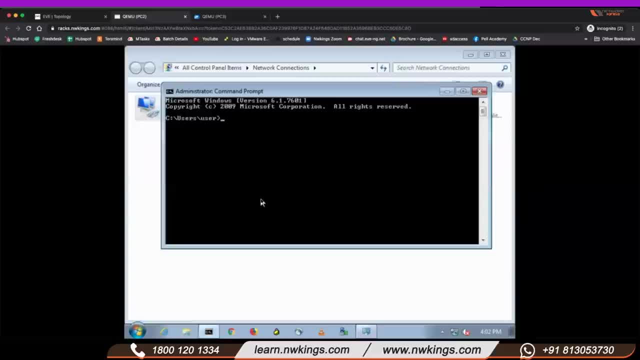 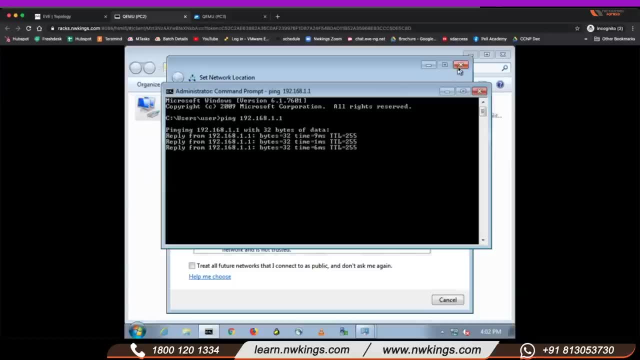 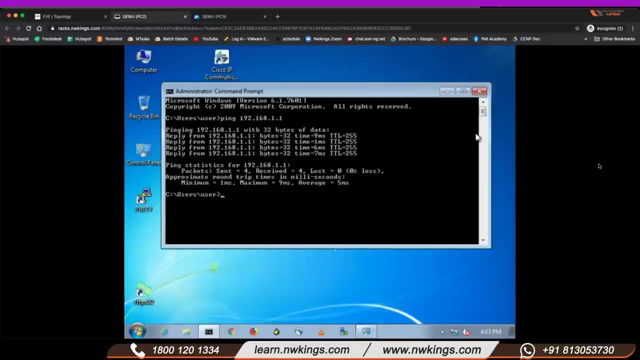 so once i assign this ip, what is the best thing? bus ping 192.168.1.1 so you can see a ping from router now. So you are pinging your gateway. This IP I have given to my gateway, So in. 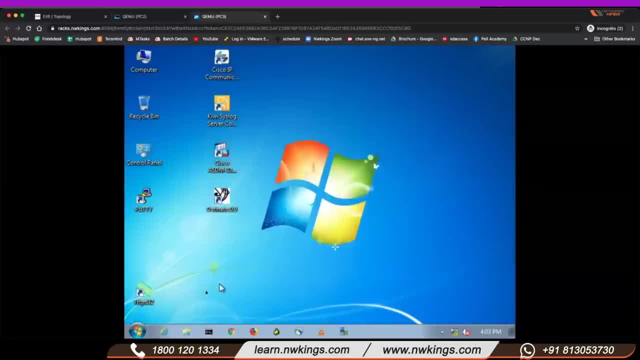 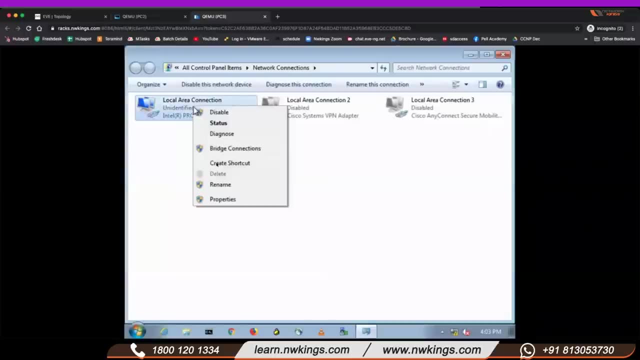 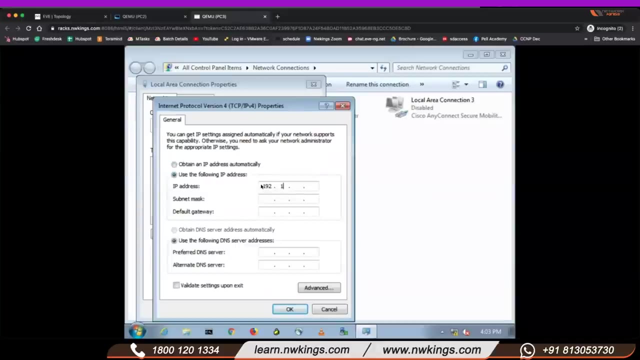 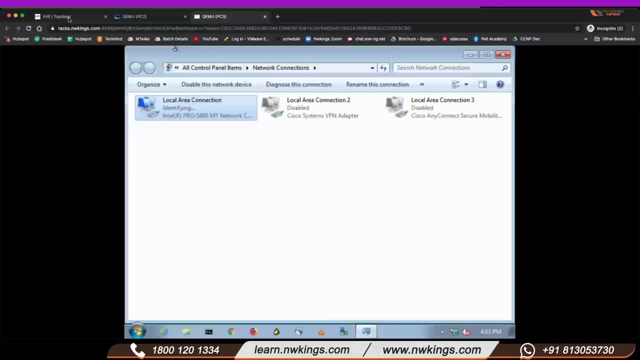 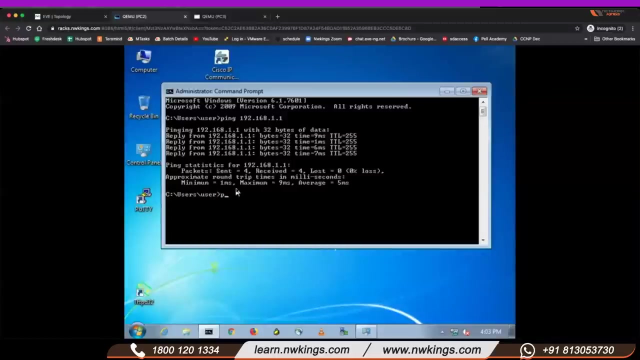 another PC, ncpacpl, inside my. so what would be the IP? 192.168.2.11, right, So IP address would be 192.168.2.1.. So let's test the connectivity from PC2 to PC3.. So what would be the IP address of PC2?. 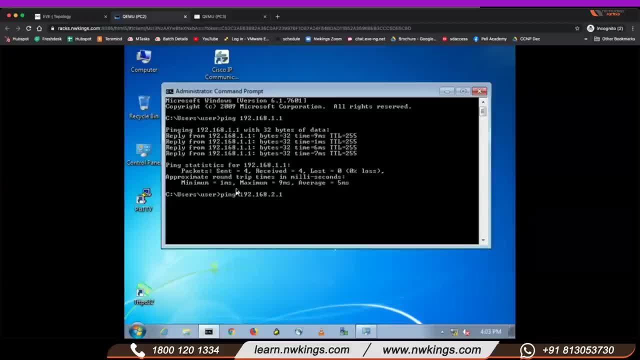 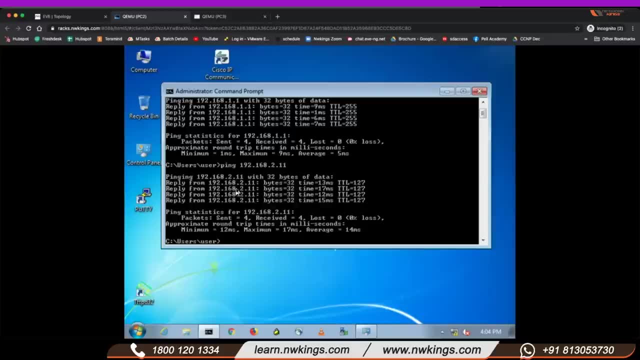 192.168.2.11,. right, So let's see. So here we go. You can see we have connected two different networks. guys, How much IP we can assign to router? It's better to always have IPs when you. have multiple IPs. So let's test the connectivity from PC2 to PC3.. So let's test the connectivity from PC2 to PC3.. So it depends on the router model. So we have very big routers where we can. 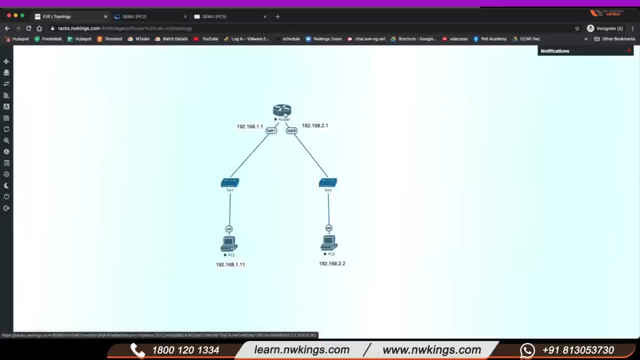 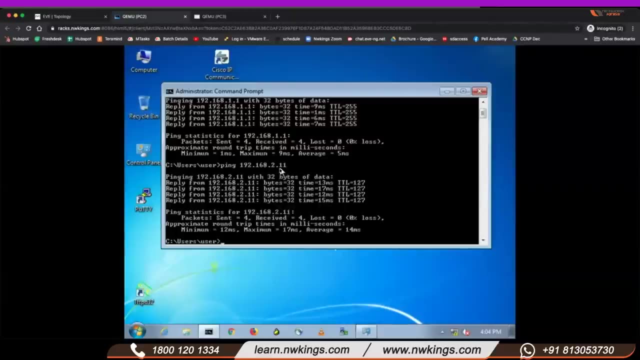 get around 100 plus ports also. So it depends. actually, The practical is successfully completed. We are able to communicate from PC2 to PC3.. So again, I have shown you that I am pinging to 2.11.. So, but my computer IP is 192.168.1.11.. 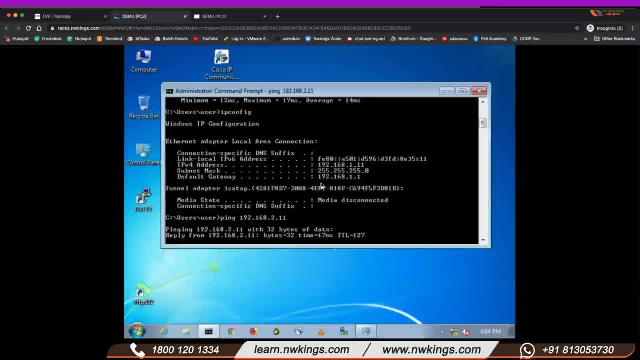 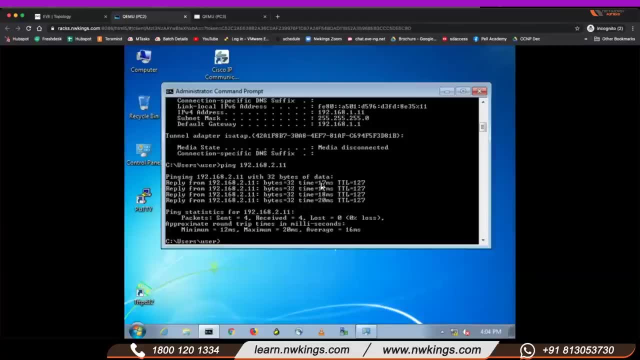 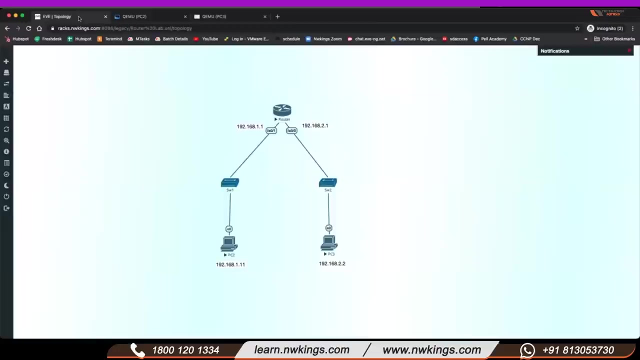 And you can ping 2.11.. Yes, I am able to ping this. Okay, Cool. How to check the? Okay, How to check the assigned PC IP from router? Okay, So I will explain tomorrow this ARP. Okay. 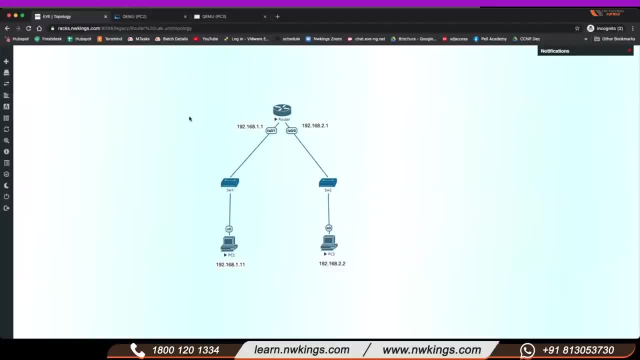 So tomorrow is very important. class to understand ARP. I am going to explain the packet flow. Okay, So tomorrow is very important, So, So I am going to explain ARP packet flow And we will see what is. We will configure DHCP on this device. 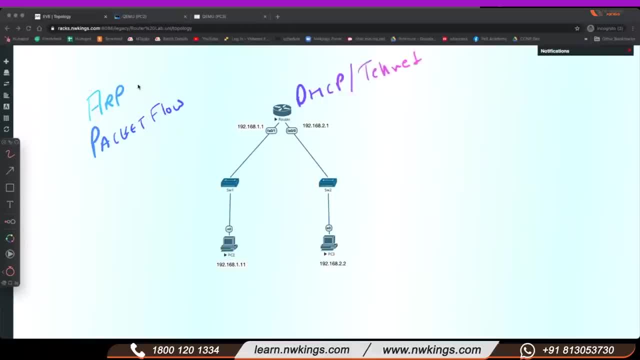 And we will also configure Telnet. So tomorrow topics will be ARP, packet flow, DHCP and Telnet. Okay, And guys, are you really loving these classes? Is this a good initiative from networking or from my side? What do you think? 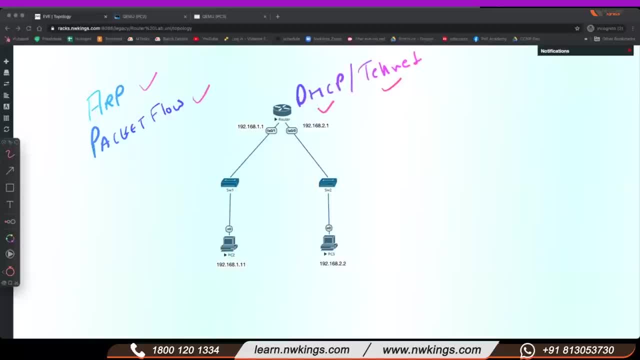 Because I am little worried that almost 350 plus candidates registered And only 70 to 60, or maybe sometimes some guys come, Yeah, So some are coming or going. I don't know what is happening. Maybe this is Okay. 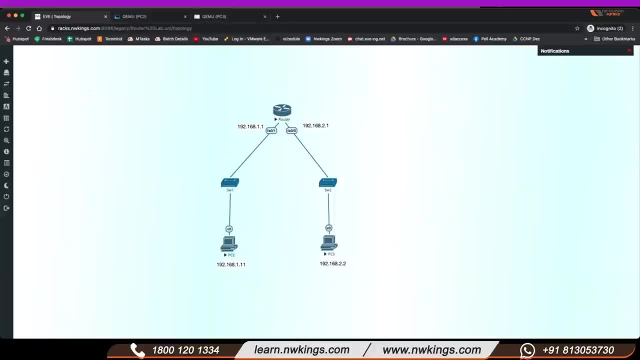 So because I thought if students won't come then it's better to have like three sessions. But you guys are giving me boost And I will have another session tomorrow And we will try to complete those five days as committed, Kunal. 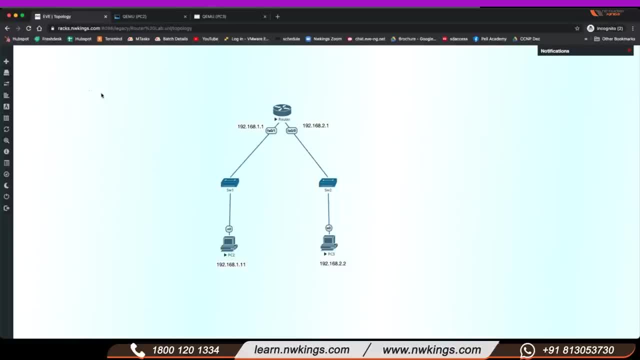 So what do Kunal is asking, sir? We can have 100 interfaces on router. Yes, it depends on the model number. This router may have around four ports Or maybe eight ports. Okay, So it depends on the model number. 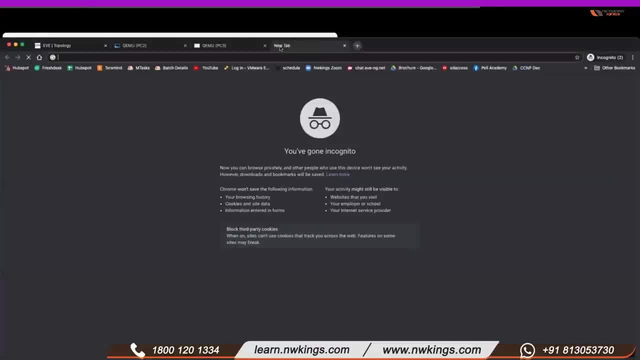 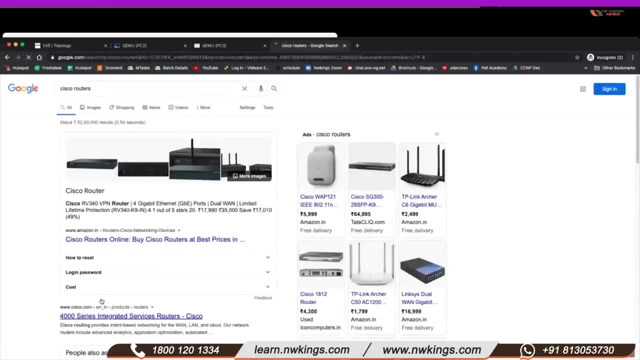 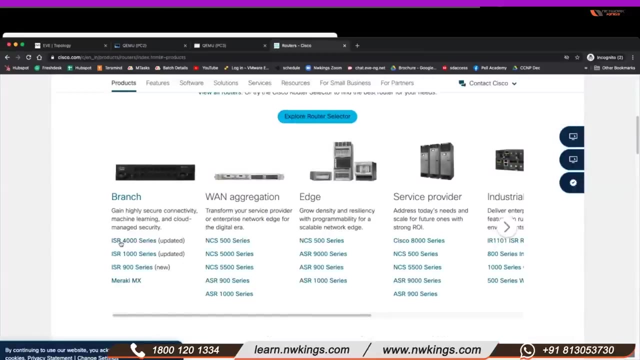 You can always check Cisco or Juniper or any company name. So let me show you Cisco routers. So just go and check the Ciscocom And there are multiple So you can see a branch routers. That is ISR 4000 series. 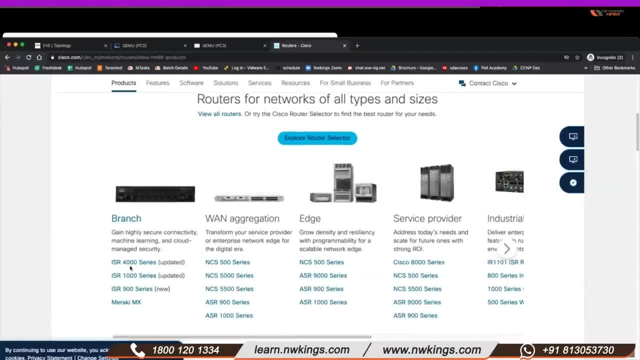 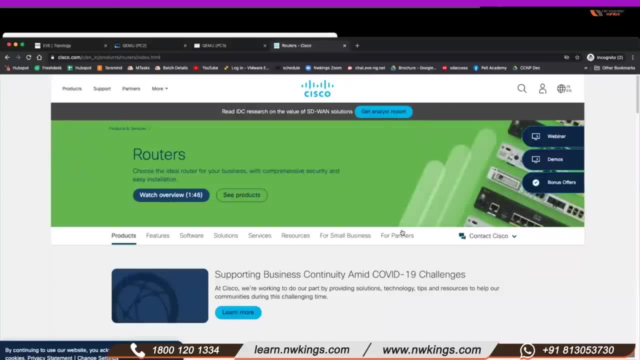 So if I go on ISR 4000 series, So you can see. So every device, Every device have a data sheets If you want to learn about the device information. Because if you complete CCNA, CCNP or anything, 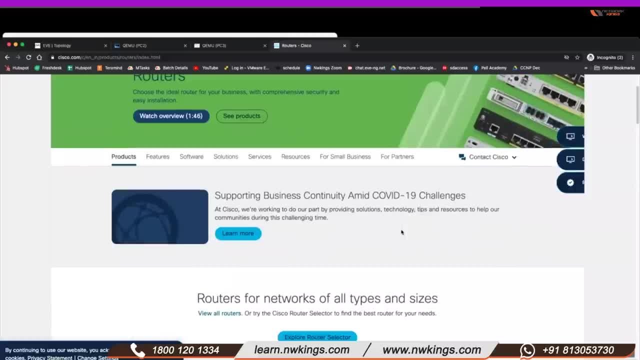 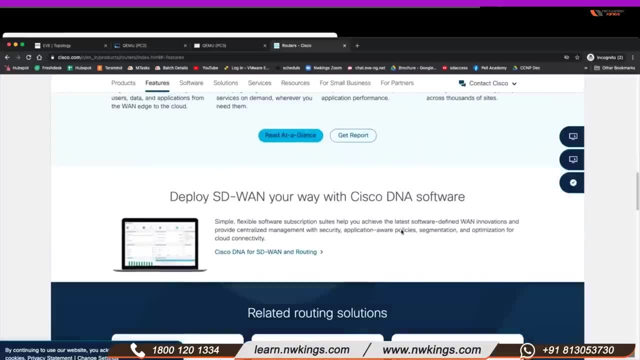 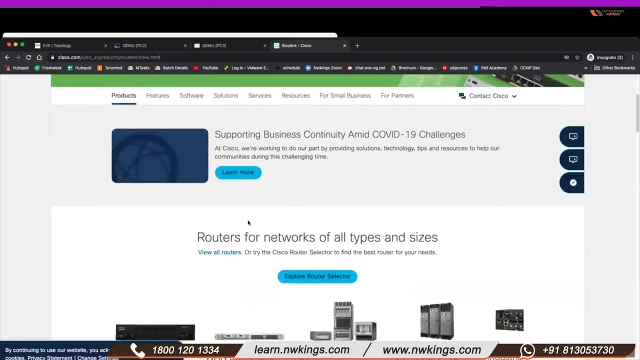 Or maybe JNCIA, JN, different certifications. Most of the interview, Most of the interviews you are going to attend, They might ask you on which devices you have worked on. So you should have a basic understanding about the devices And how to get those basic understanding. 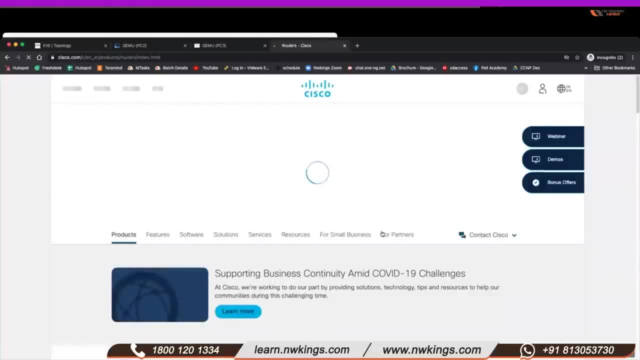 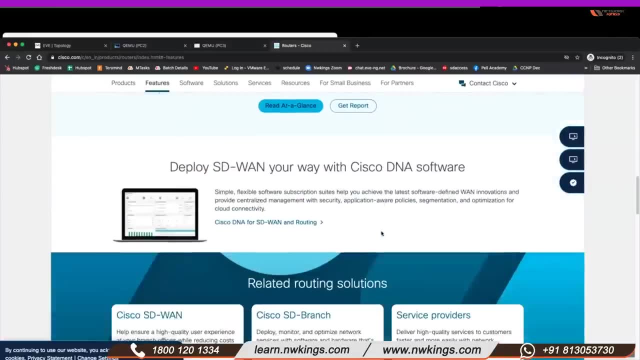 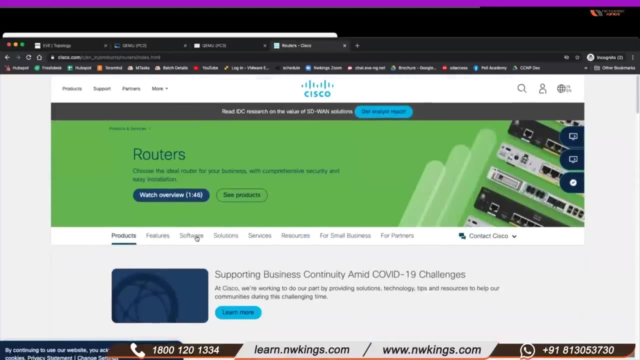 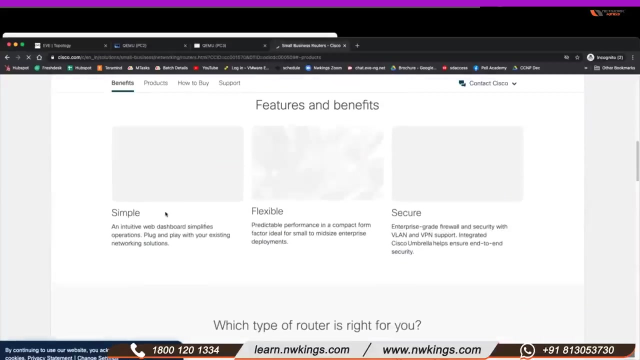 So just Keep on checking the data sheets. So how to check the data sheets? So on every device You can just search for the data sheets, Maybe inside this. Yeah, see products. Yeah, so you can see a lot of model numbers here. 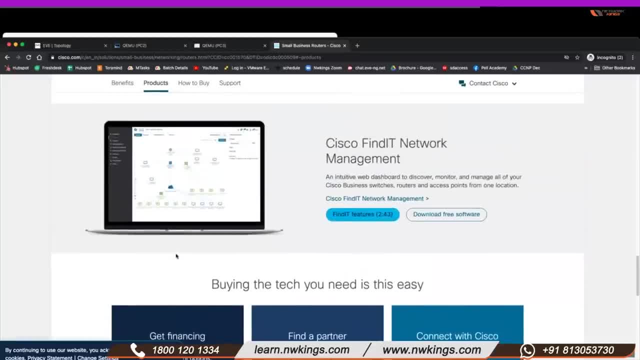 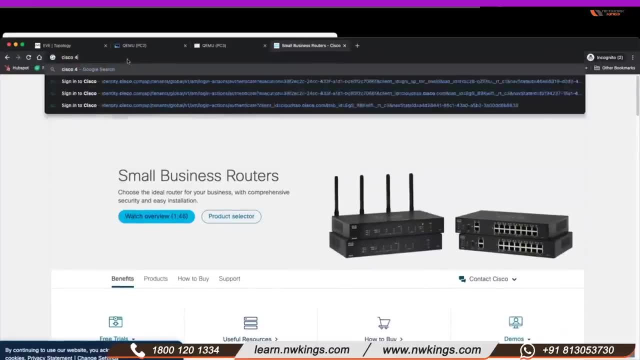 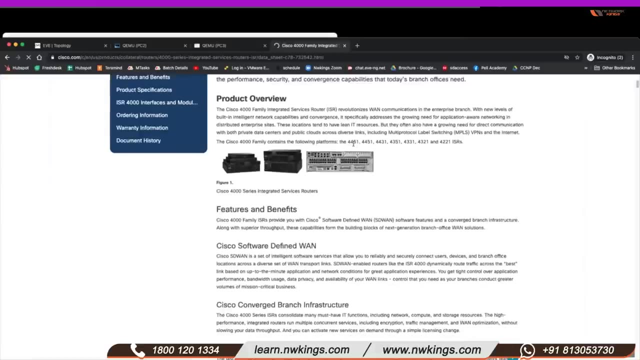 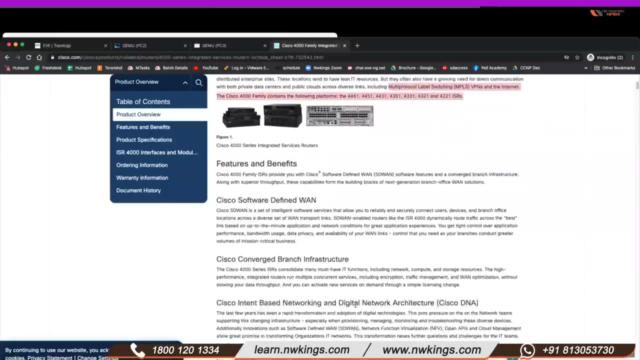 Okay, And they are doing so. you can check the model number like Cisco 4000 data sheet. Okay, so that is a data sheet and you can check Cisco 4000 series as that many model numbers and they can support these many technologies. 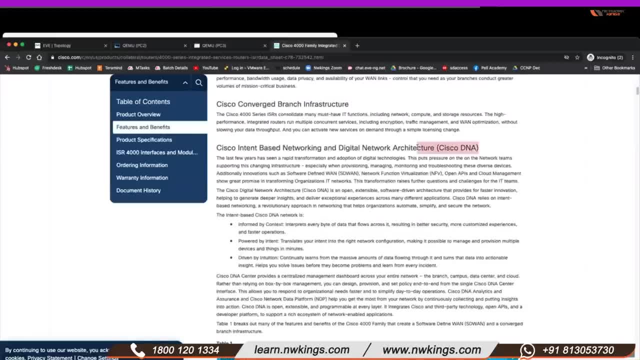 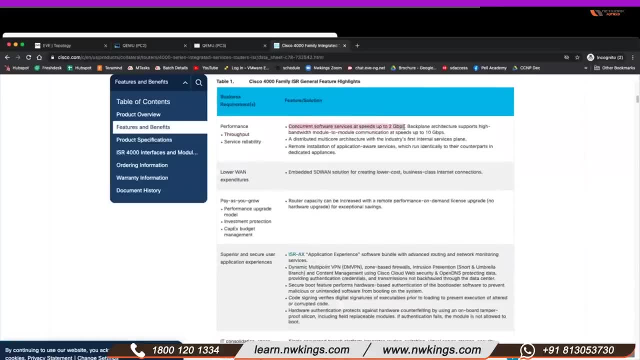 Okay, So they also support the Cisco latest technology, that is, Cisco DNA Digital network Architecture. and how much throughput means how much maximum speed you will get on these devices- up to 2 gbps And if you have, yeah, current software services at speed up to 2 gbps. 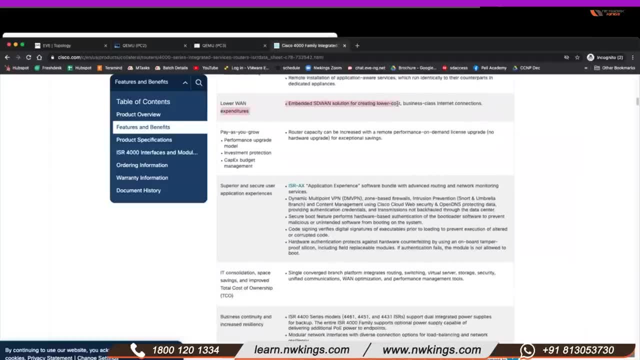 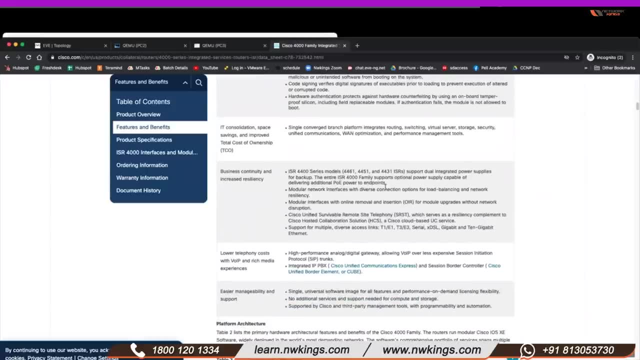 Okay, so it has integrated SD-WAN solution also. SD-WAN is a very new technology, recently introduced in last one or two years, getting very much popular and most of the companies are moving to SD-WAN. Now let's see. You can see the data that is coming out of the system. 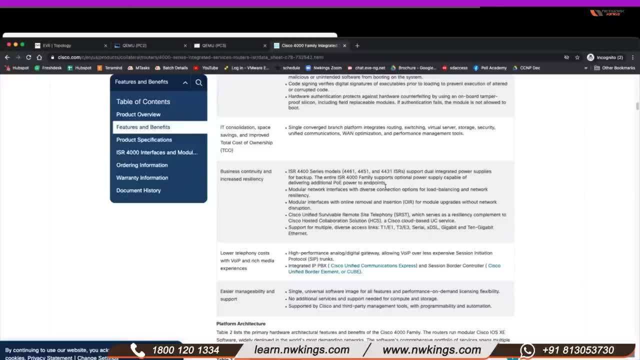 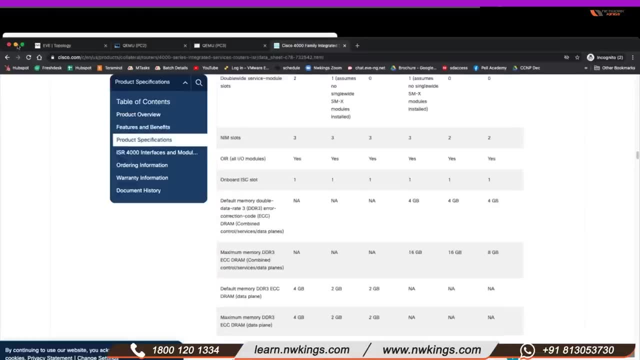 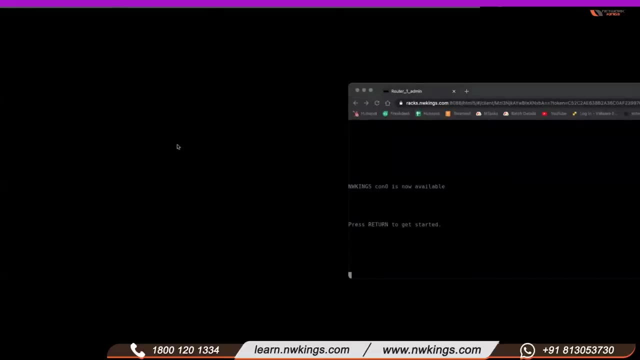 AWH technology, discrete network and this to know location. it's distinct. So let's talk about the data. See What is that? So let's discuss about the career path now. So what should you like, how we can start or how should you go and further. 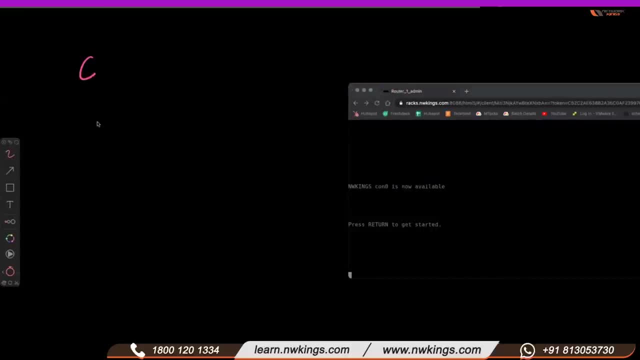 Yeah, So to become a good engineer. So the basic, the minimum things I'm talking, But some of it duncans I'm talking And some of it And some of it How I'm talking, telling you so you can start with ccna, okay, and or maybe you can start with the j and cia also. 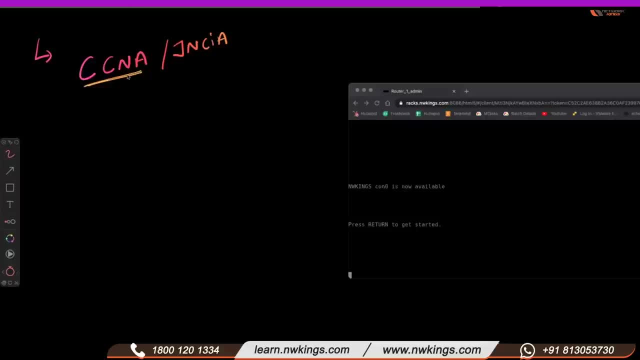 okay, but it's always go better to go with ccna because it has the sesco study or sesco books or sesco content is better. i would say even worked for both the organizations. so ccna you can start, you can learn juniper things after ccna, so it's better to go ccna first. so ccna, jnca is both. 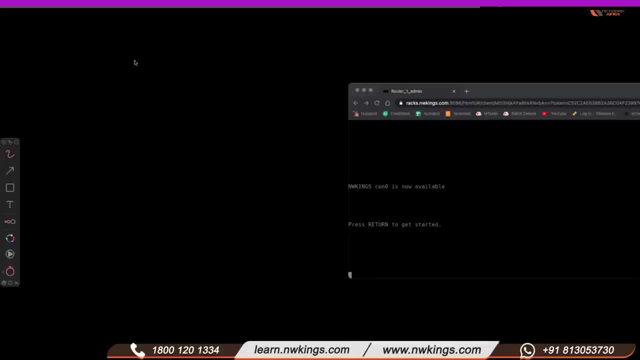 equivalent. okay, so i'll write here ccna only so you can start with ccna and further you can go for ccnp. so that will actually add on a lot of technologies like bgp. you will learn mpls, so you will advance, learn advanced things like dmv. 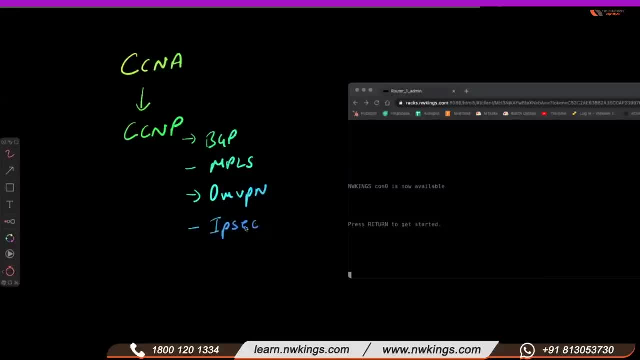 vpn, you will learn ipsec. so there are a lot of technologies here. you will understand in ccnp and after that, see every company i have seen on nokricom, i have seen on linkedin. every company needs firewall nowadays. so it's better to learn firewalls. 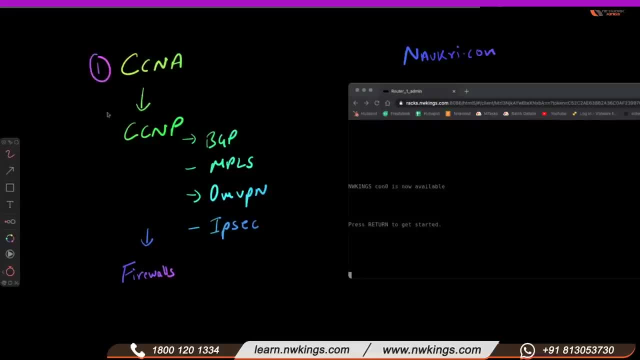 so i only recommend these three things to any engineer, because, because you will not restrict to yourself. so i'm giving you one example. uh, trust me, this is very important. so suppose i worked for cisco tac for almost three years, so i'm i'm very good in cisco. 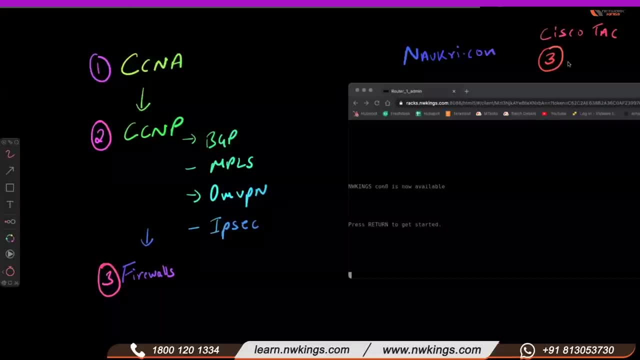 but outside cisco i don't know any, anything. so if i'm looking for a job, i can only go in a tac profile. i cannot go into enterprise, right? so it's better to always learn multiple technologies so that you will be ready. yeah, you will get only support jobs or attack jobs, so it's better to have 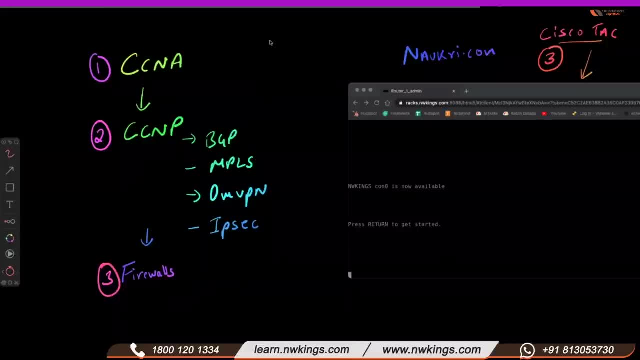 ccnp firewalls okay, and once you learn this, then go with the little bit programming stuff that is like python, you for network engine, you don't have to learn python which is actually making websites, you just need to learn python which is for network engineers, which firewalls, to learn. so there are many firewalls like paul alto. 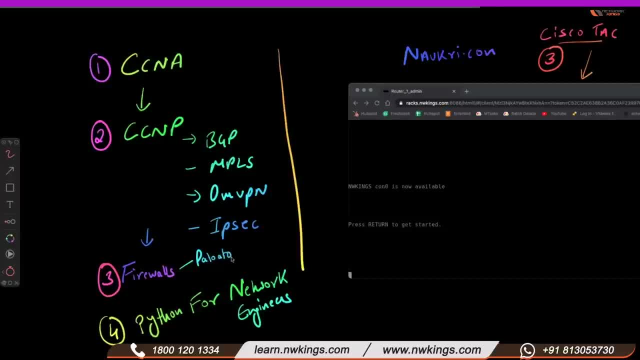 paul alto is very important nowadays because every company is using paul alto. i'm just giving example. so i used to work with apple and they have paul alto firewalls, so they have a lot of firewalls. and they have a lot of firewalls so they have juniper srx firewalls also, but they have replaced juniper to paul alto now. 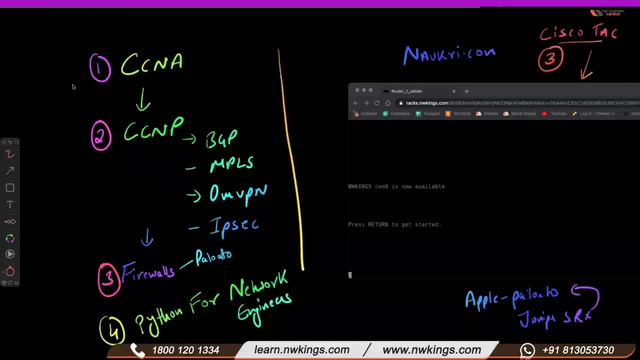 okay. so once you complete this, i think it will take maximum one year- and you will be having the same knowledge what 10 years experience guys have in industry. so if you have pix, firewall is obsolete, yeah. so if you have one year, two year, three year experience, trust me, if you learn these four things, you will be ready like you have 10 years. 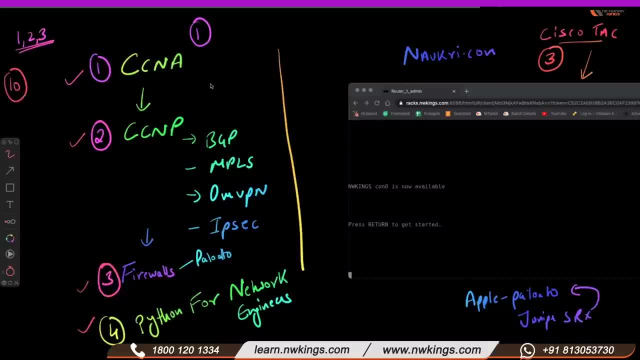 experience, because even 10 years experience guys have up to this type of knowledge. but you need to make sure that you will learn in a very good manner. you will not only do these courses just for the sake of completion. yeah, okay, so firewalls like paul alto checkpoint. 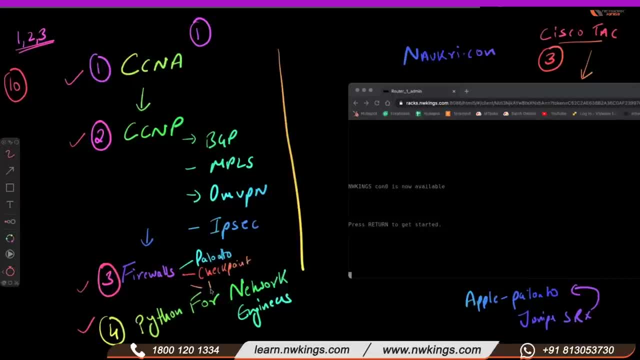 so and so, and so is one device called f5 load balancer. so like that you can go for this, and once you complete this, then you can go with the cloud technology. so i would recommend, fifth point, vmware vcp. that is for to understand the virtualization. so it's optional. this is optional if you want to learn. 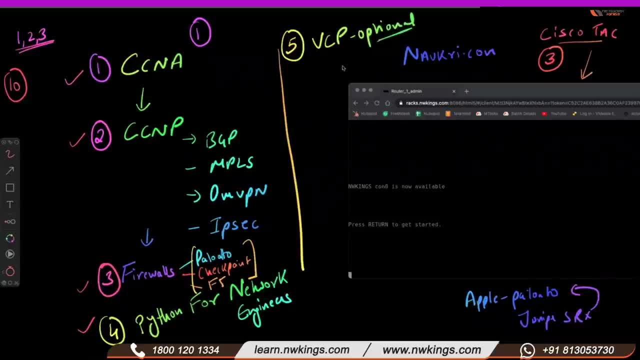 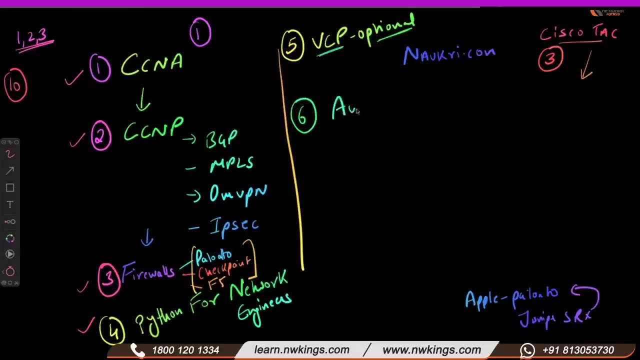 because if you learn this, you will understand virtualization and every. why i'm telling you this? because for one reason: because all cloud works on virtualization. so if you understand virtualization concepts very deep, then you go for aws or maybe azure. okay, so any cloud. and then seventh point: 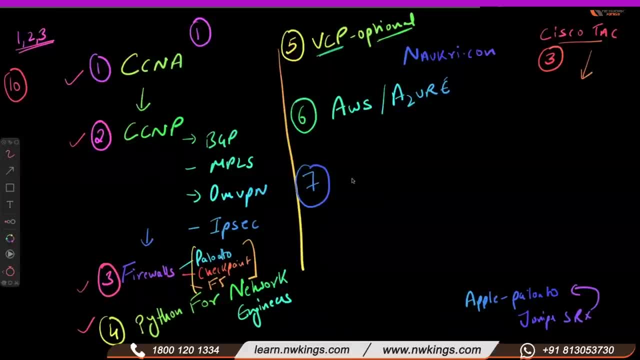 take, or you can note down my things. what i'm telling you, this is the future. so that is aws azure, cloud migration. cloud migration means companies are actually moving to cloud. you are going to configure in this course. you will configure router, you will configure firewalls, but you will be going to 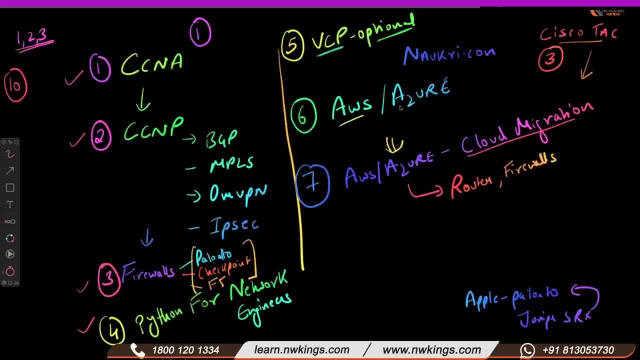 configure in cloud cloud. here you are learning what exactly is the cloud right, you will learn how aws works, how it azure works. but in aws says your cloud migration. you will configure routers, firewalls and a lot of other devices in a cloud. okay, so vcp is optional, sd-wan also optional. so if you want little more, 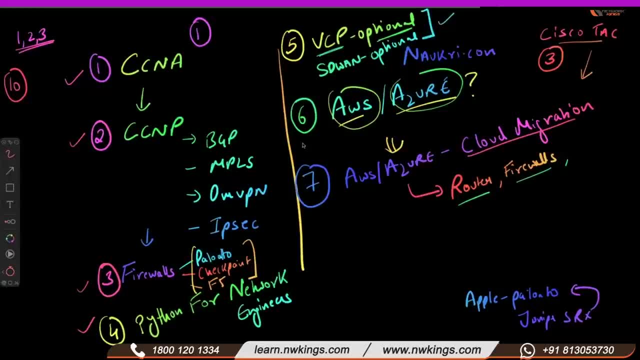 boost. you can go for when before, like that is sd, when you can learn here. or you can go for like this: uh, amr, vmware network, nsx is not required because vcp or something. if you learn this so automatically you can say that you are getting that type of knowledge. 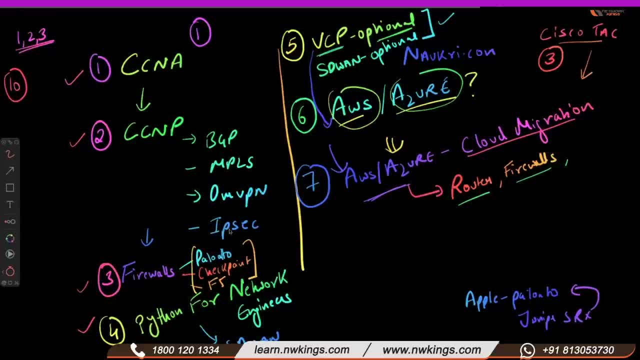 so this is see this: you are learning firewalls here, man, so directly you are going to network. security means you are in it. you will be a network ninja- okay, so you can be a network consultant for many companies. you can do freelancing also- okay. what does freelancing? 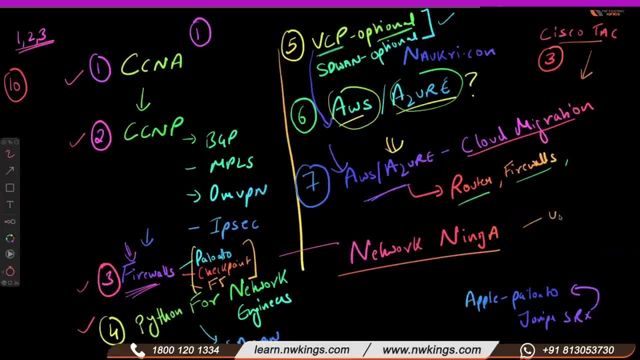 means means you can take projects from. lot of websites are there, like upwork, work and all so. but, yes, it's better to get freelancing projects, but never use your company laptops. okay, i have seen many guys got yeah, so if you want to learn azure, then there is no use of directly learning azure, so it's better. 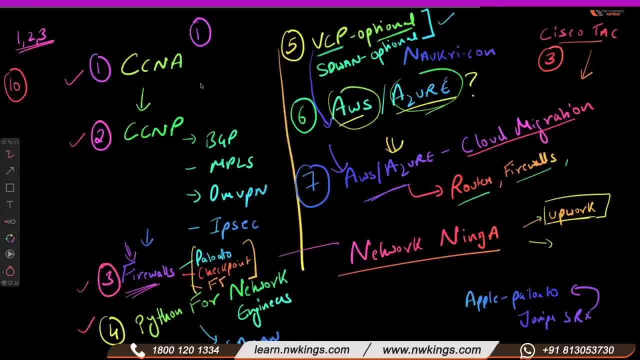 to always learn network fundamentals. and what is the best way to learn azure? because azure is, uh, microsoft oriented. so there is a course named as mcsa, so you can directly go with mcsa and azure also if you want to become a system engineer. so the x, this career guidance i'm giving. 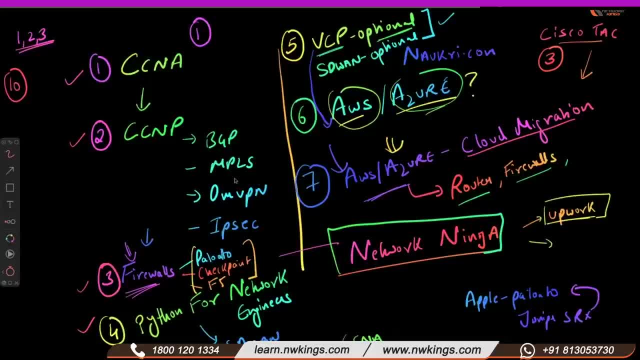 for network ninja, okay, and maybe after six months i will do some changes. but for next, at least for five, six years, this is the best thing. so you can start with. na see, if you don't have job right now, you are jobless. so we made a plan that 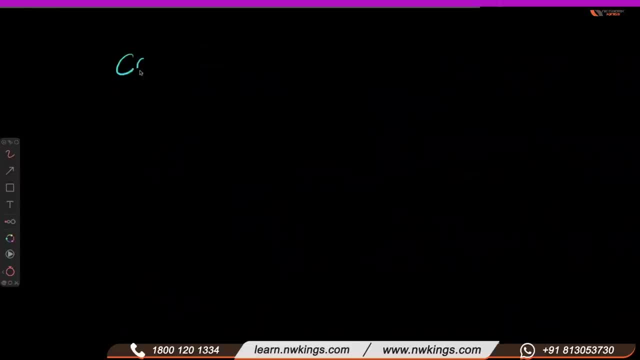 is known as ccna, mcsa, linux. so that is a very basic like uh, to become a network engineer, to become a system engineer, to become a linux administrator, so it's a combo. we call this phase one in network engineer. so it's a combo. we call this phase one in network engineer, so it's a. 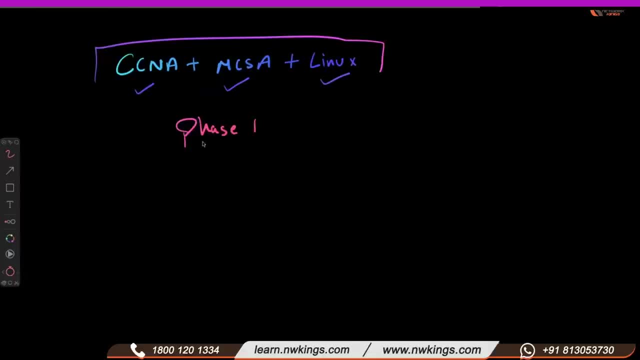 in networkings. so if you don't have job, directly go with this plan, because if you learn only ccna or you will do ccnp, actually you are going, you are learning a lot, many advanced courses, but if you don't have job it's better to learn the associate level courses so that you will at 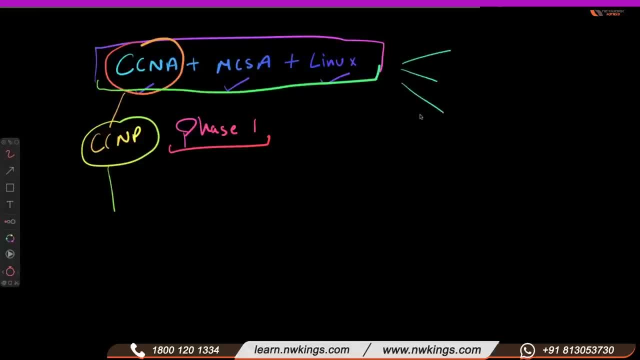 least find the correct job for yourself. okay, if you are a fresher. so by learning this ccn, mcs, linux, you can apply for network engineer, system engineer or linux engineer. so that is the best course in the market right now to get into it right now. yeah, so you can contact. 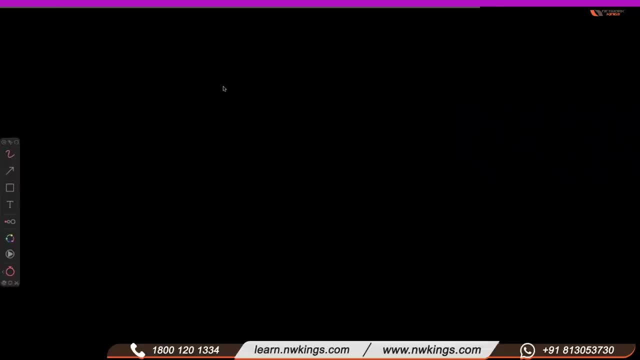 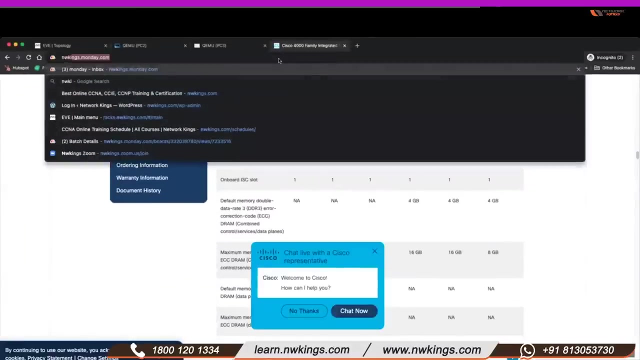 team or i'll share the link with you later on. linux takes approx 20 days. we cover these courses in 45 to 50 hours so you can check this website okay, so we have made our website with the career guidance also like go to nwkingscom, so here you can. 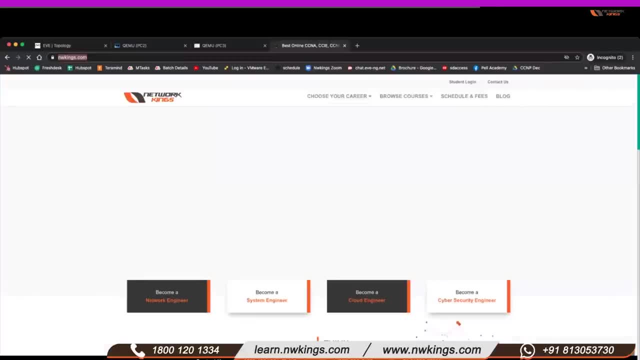 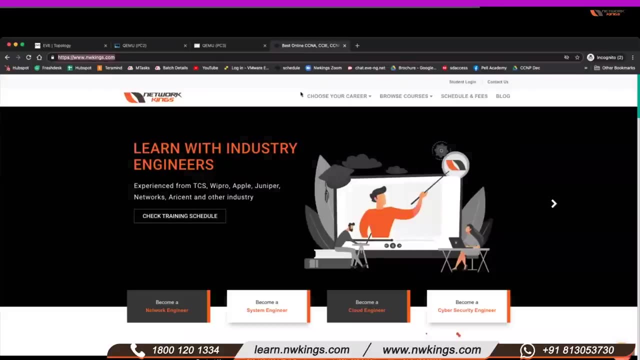 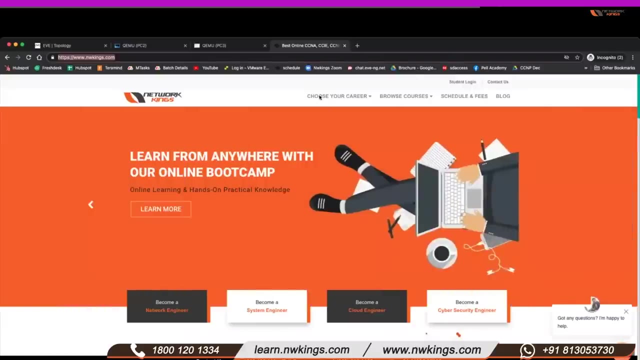 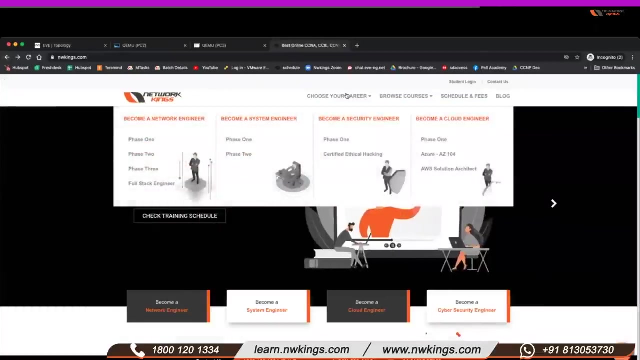 see all the career guidance by default. okay, so this we design for working professionals and for freshers also. okay, so choose your career. so we are actually training students on four different technologies or four profiles: network, system security and cloud. so if you want to become a cyber security engineer, so phase one is default. 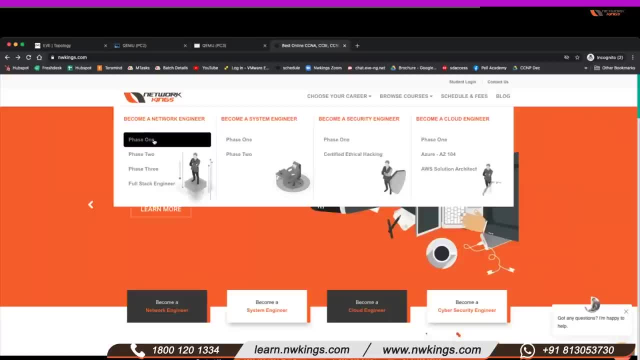 for all and then you can choose your career. so we are actually training students on four different technologies or four profiles: network, system, security and cloud. but if you are already working like but if you are already working like you, if you have two years, three years, four years experience, 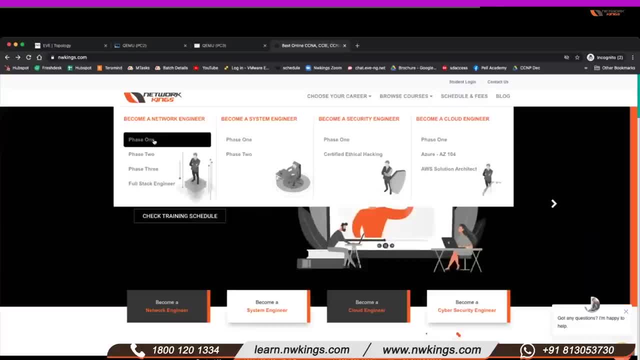 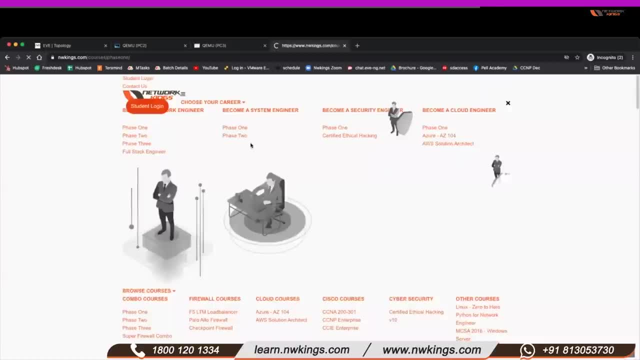 you if you are already working. like you, if you have two years, three years, four years experience, then you don't have to learn mcs linux. you can directly jump to ccna and ccnp. but if you don't have job, then go and start with phase one program, so which is a combo of ccna, mcs linux, so these 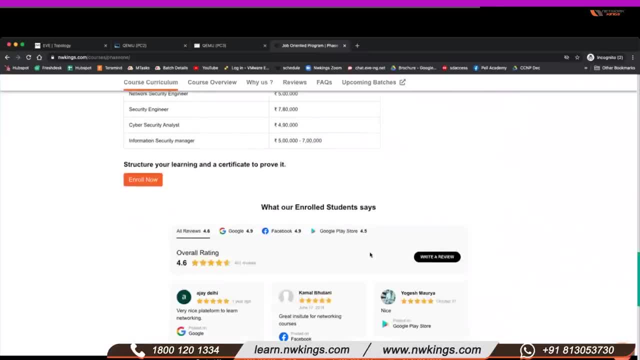 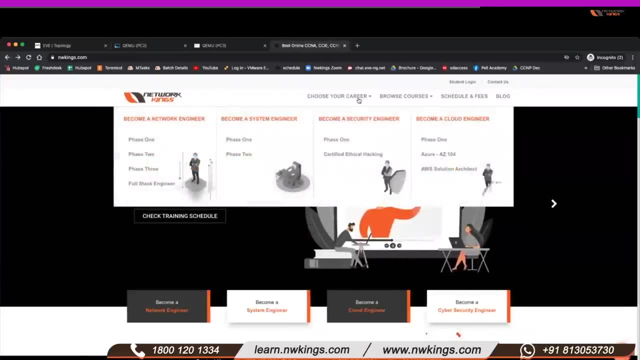 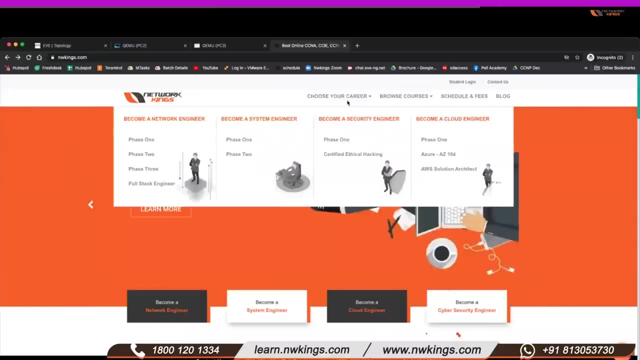 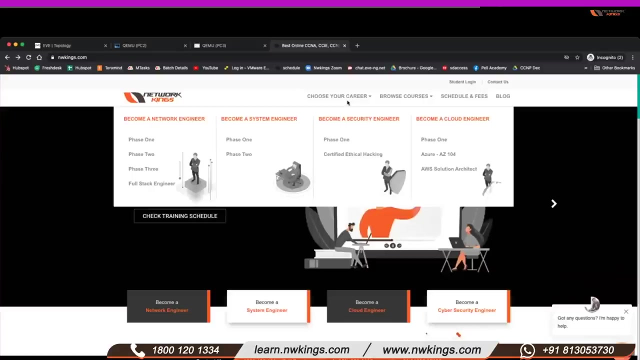 courses are actually designed by all like engineers. so we are a company which actually all our instructors are working professional. so, like the person who is taking mcsa or maybe the person who is taking linux, they are actually working as a linux administrator or maybe system engineer. okay, prety, i would recommend you to go with ccnp first, then learn paul alto pc nsc. 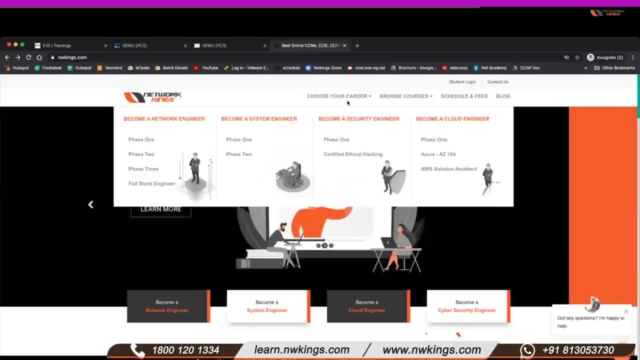 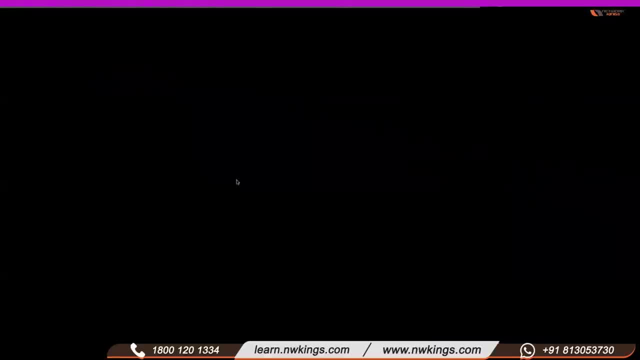 because, paul alto, because you are see, security is like add-on. suppose what i'm trying to say? you need to learn the basic first. it's like a pizza, right? so like, if you want to eat a pizza, you need to have a good base, right. then you can add all add-ons, like cheese or maybe olives. 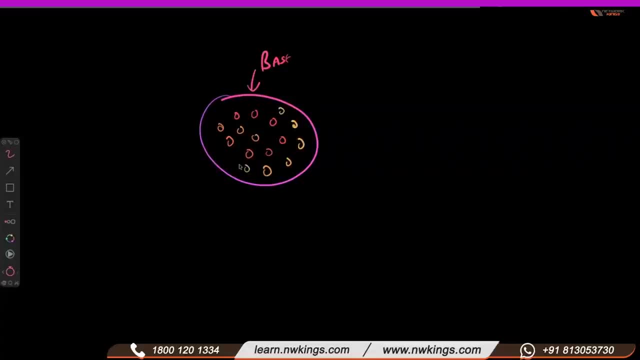 anything. so these olives or maybe mushrooms or anything, i'm getting hungry for this. okay, so these all are add-ons. so add-ons means, like you will learn. uh, like paul alto is add-on. okay, like checkpoint is add-on, but what is the base? so base is for a fresher, like basis to learn multiple things so that you will get. 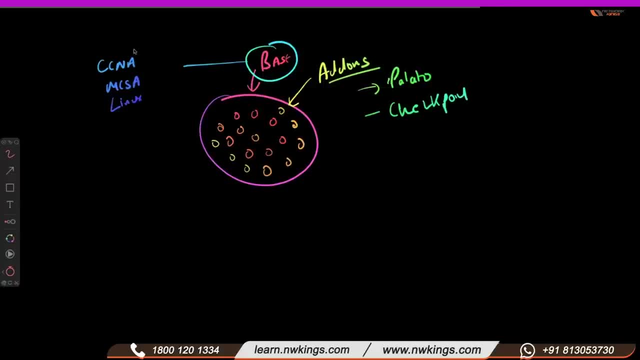 entry in job. so base could be like this, or base could be like ccn, a ccnp- okay. so either you can make a base from this- this is white bread, this is brown bread- so you can use any of the base. so once you get entry, you can keep adding the. 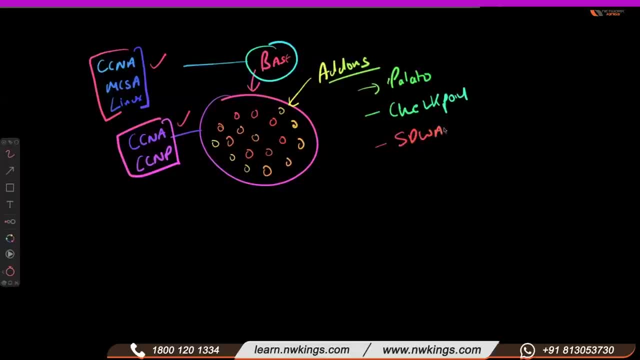 add-ons like paul alto, checkpoint, sd van or like any any further technologies like vmware, python. so all these are add-ons, but if you just use the base, you can make a base from this. or you can make this because if you just keep learning the add-ons, but if you don't have good base, then what you? 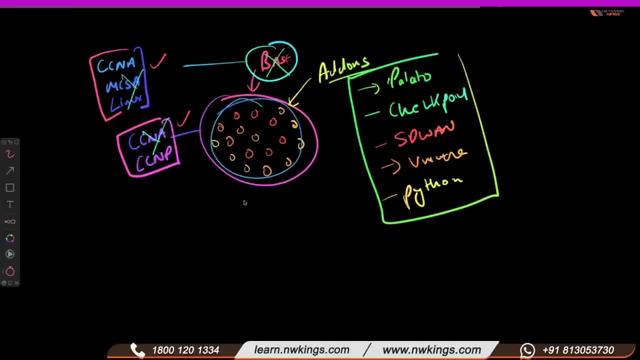 are eating. you are just eating the vegetables, man. you are not eating a pizza. i hope you are getting now and you are understanding the things. okay, yeah, bina, you can go with the ccnp. see, priti, don't stop learning pcnsc. you can start with npr and you can start with this ccnp. 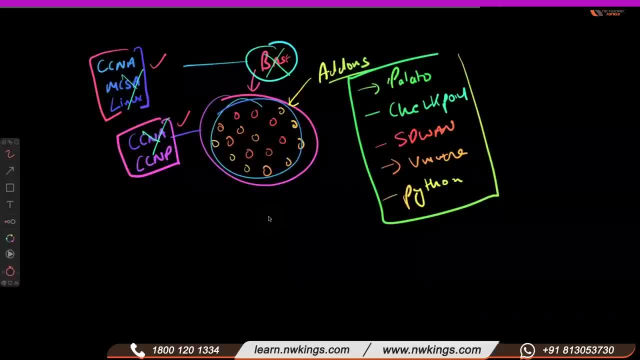 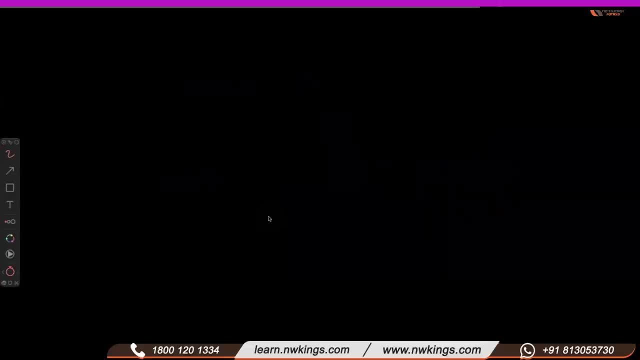 bgp, because it will help you to understand bgp mpls in detail. our certification is important in industry. and what is the global certification? yes, actually certification help you to boost your career. certification is like a booster. you have played a game called need for speed, right maybe, or you have seen it. so you are doing a car race, but 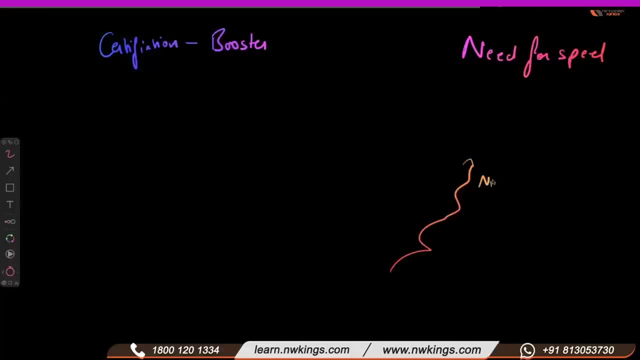 sometime you want to just enable the nitrogen to boost your career, right? so certifications are like that, it's like boosters. okay, so it's like boosters. so by learning new things daily, you are actually growing. right, you are growing. but if you have very good knowledge but still you are not growing, then 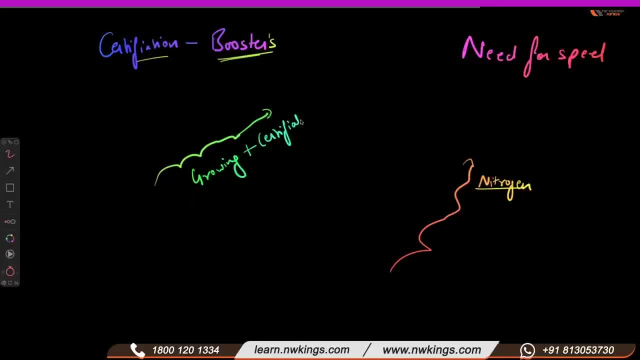 just add the booster boom then you will get more jump. okay, it means first focus on growing, means focus on growing how you get keep growing in the industry. you by learning new things, by learning. so certification is needed when actually you have enough knowledge. are you getting now when, when you have enough knowledge to boost? suppose 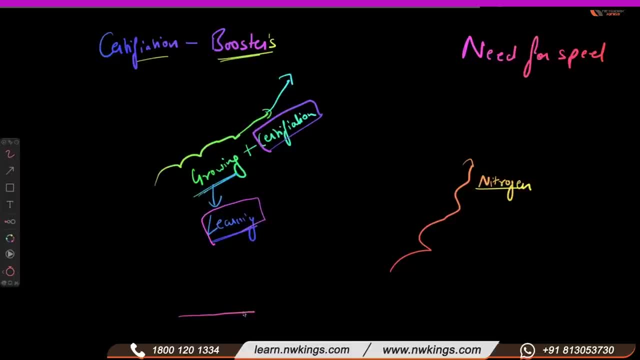 you don't have knowledge and you just get the certification done. you don't have knowledge, you get do the certification. you will be like this: completely plain. but if you have good knowledge, then you will be like this and booster is like that. okay, so means knowledge, but certification is very basic. you don't have to know anything about me together. so they are. 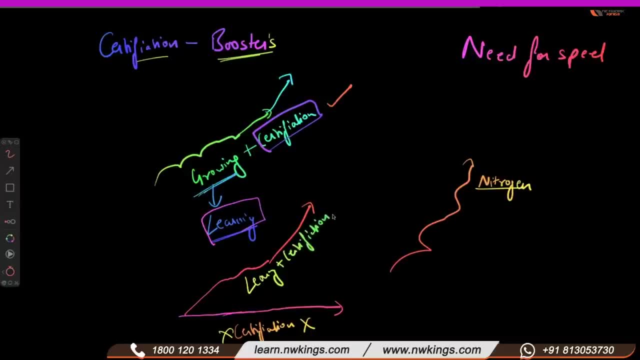 certain that you will know um. so you will be with just having um knowledge which has the key to, but there is no other motivation which you have, while you can't talk through the whole class without that, you must be Nerd. that's yourRadio, that's the threat to education and logic: 1.5 million episodes. 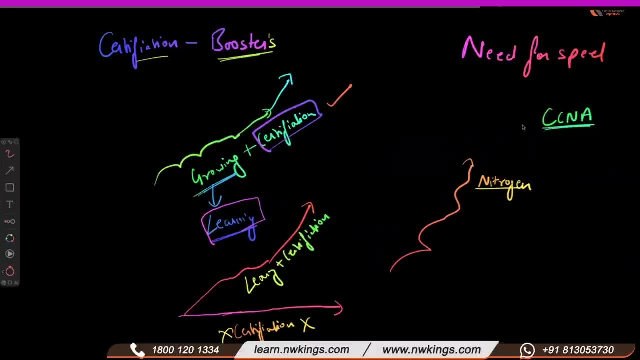 you will bekąan. you will be iosinh menском run more opinion on each of the cesarean online classes. k Mission and the newTrain Detective will be associated withries of social sciences. do ccna, so you can only apply the jobs related to ccna like network engineer and might be a chance. you will not find it in one month or two months. maybe it will take time, but, yes, within three to six months. or maybe it's your luck, maybe after a month also depends on your learning and how you give the interviews. so many guys do ccna and get the job okay. but if you really want to, if you are, 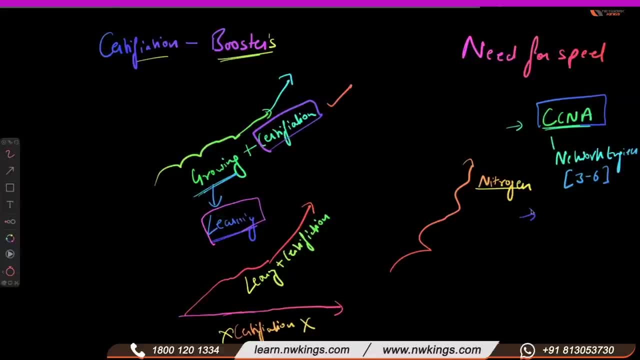 needy or you really want job as soon as possible, then again, i told you then you need to learn multiple technologies like ccna, mcsa will train you windows servers, linux will train you for linux commands, and all so for freshers. i recommend this because i 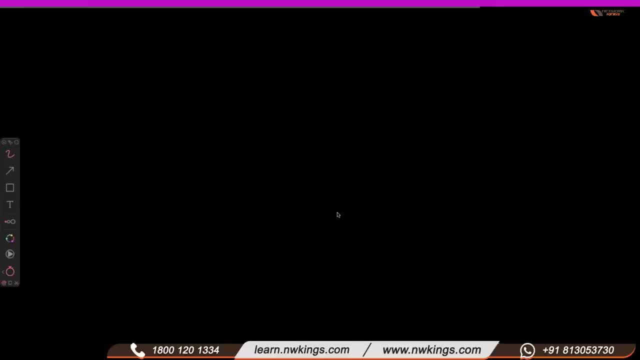 know from fresher point. so, fresher point of view, our main focus is to get a job first. so once we will have around three to five lakhs, or three to four, five, six lakhs package, or let's take three to five, okay, then it's good to go with the different things. hi, you are watching the recording. 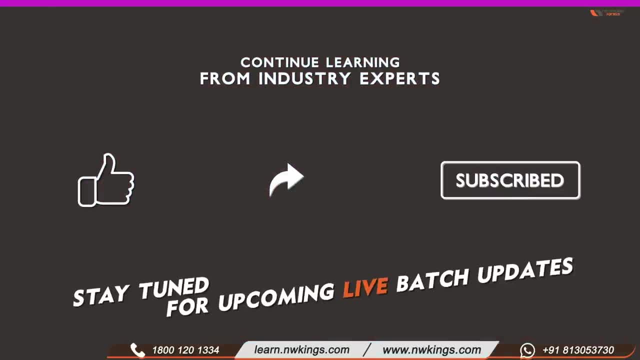 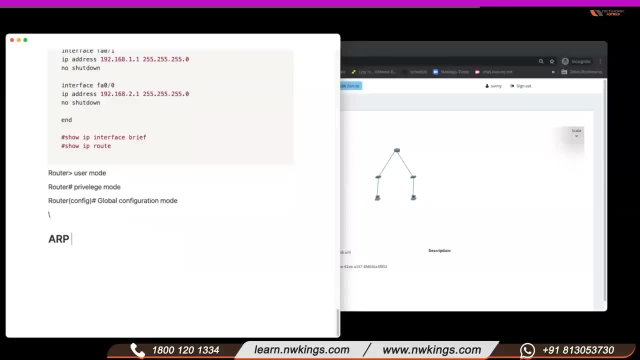 from one of our live session. hit like share and subscribe for more future updates. okay, so we will discuss now arp and after that i'm going to explain you about the packet flow. and third thing, we are going to discuss dhcp. and fourth thing, we are going to discuss telling it today. so are you guys ready? just say. 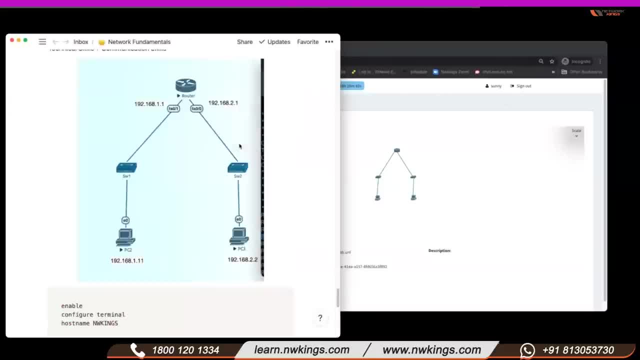 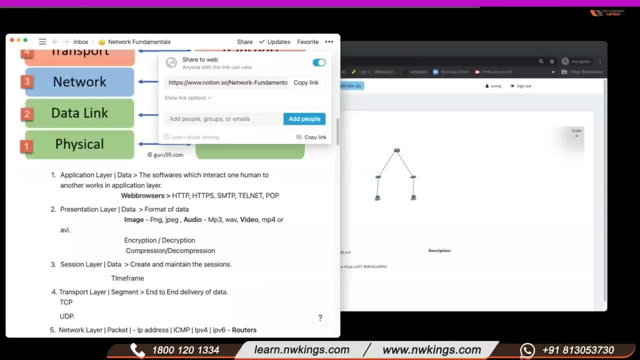 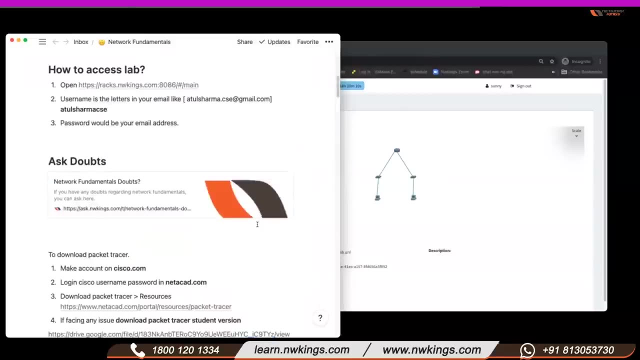 yes, in the chat. uh, how can access? uh, these are not pp das. these are my notes which we have created for you, so i'm going to share link in the. just check the link in the chat. i have shared the link. details are mentioned here also and you will be getting one email also if you want to join. 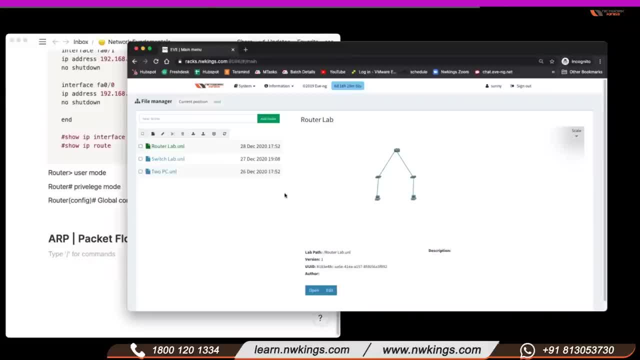 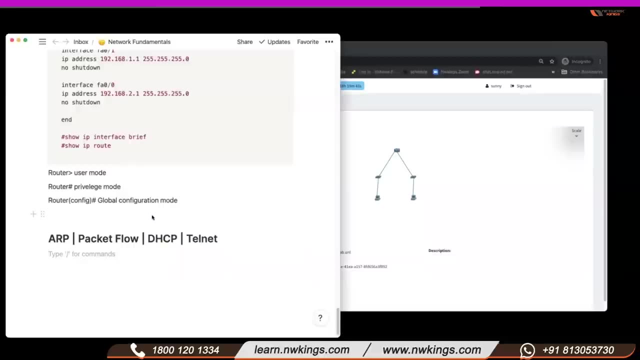 or like: if you want to join my ccna batch, which is starting from 11th, and i'm going to start one ccnp batch also that is from 9th jan, okay, that details i'll share in the email. okay, so keep checking your email. that comes might be with some discount. okay, so let's go ahead. 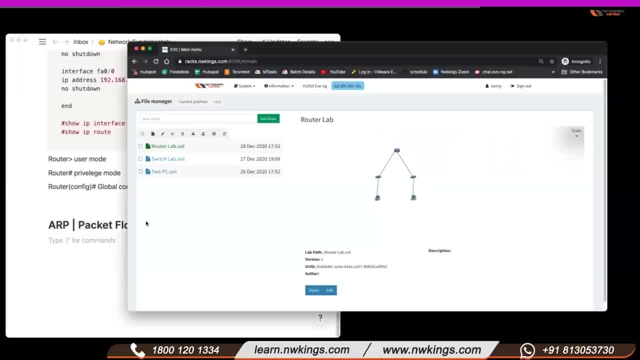 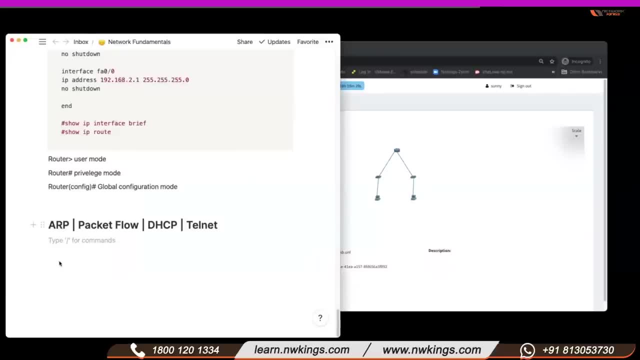 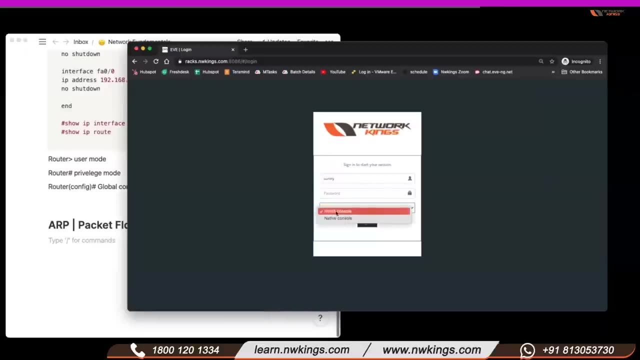 yeah, you need to always use html console. native console will not work, only use html console so when you log in, right. so there are two options: html console, native, you always you have to use html console native. we have blocked the ports, okay, so what is arp? what is arp? 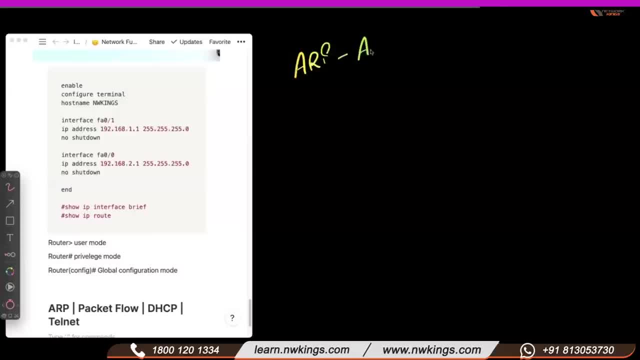 so arp stands for address resolution protocol. okay, so address resolution protocol. so i'll give you one example, like if i have one computer, a here and b on the another side, so like my computer will have one ip 1.1.1 and b will have 1.1.1.2 right. 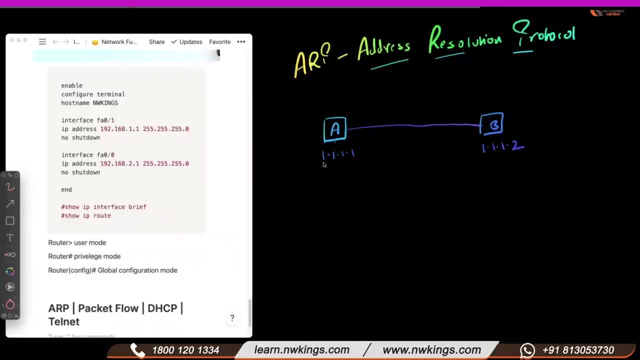 so if they are connected together, and in this computer you are going to type in the command prompt: ping 1.1.1.2. so why we are doing this? because we want to confirm if this device is connected to me or not. so ping actually means i'm going to send some messages. 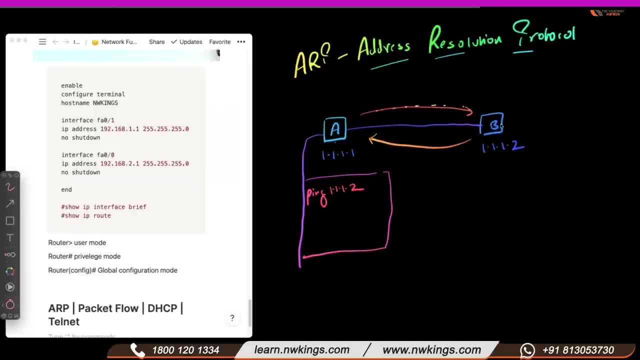 to this router, so the. so, uh, sorry, to this pc, so that c will lie back right. so i'll get replies. but what is arp? we'll say data to anybody. we need mac address of that device also, okay, so if i'm sending a data to 1.1.2, so i need a mac address of this device. by default, my com does address this computer will not. 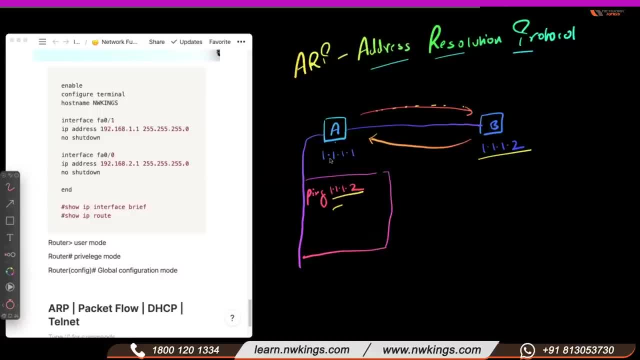 have my computer will not have. so every computer, like it's a windows or linux or something, they have arp table, arp table. so what you will see in our table you will see all mac address against with the ip. so suppose this ip uh is one two. so computer a is going to store the mac address with the. 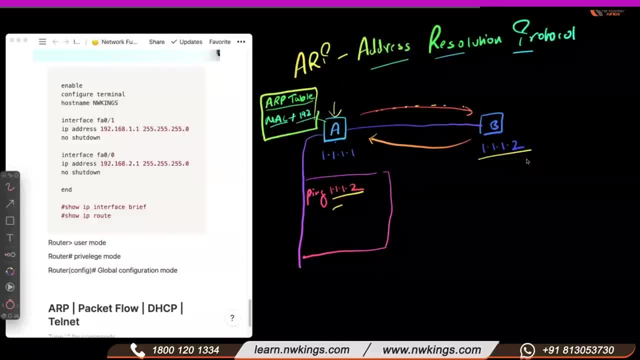 corresponding eb b. suppose this is mac address of b computer and this is for a computer, okay, so if i want to send a ping packet to is mac address of this device first. okay, i'll explain again. so computer a has ip 1.1.1 and computer a has a mac address. double a, double a. 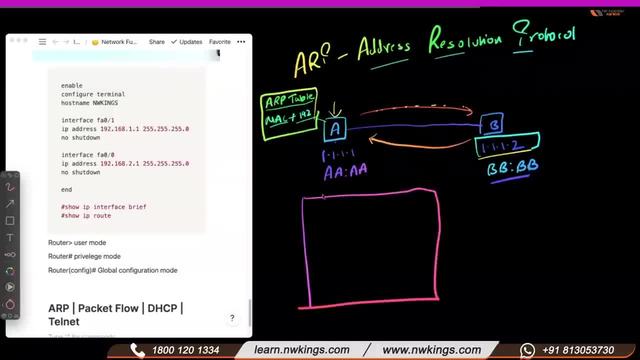 so computer a will have a table that is known as arp table, address resolution protocol table. so whenever we send data to anybody we need mac address for that device. so if my arp table have no arp entries- it means if i don't have any entries- what will happen? 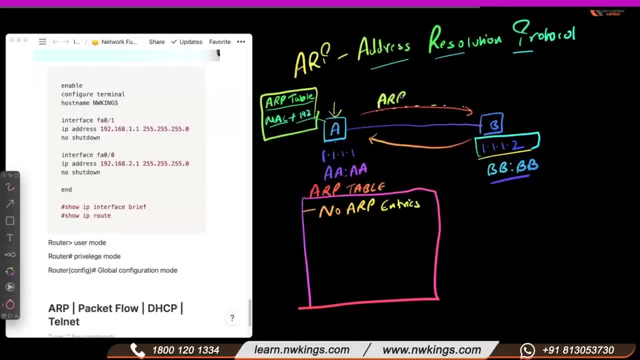 i'm going to shoot out a arp broadcast packet- arp broadcast packet and i i'm going to ask who is. so i'm going to ask who is 1.1.1.2? okay, so whenever you send a ping packet or anything to 1.1.2, so the ping, the ping packet, will be on. 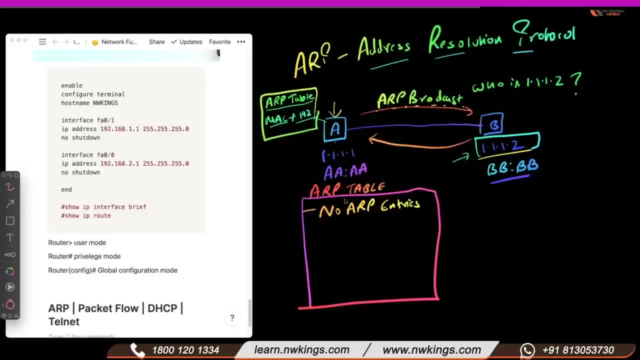 hold. i'm going to say just hold the packet. before i send data, let me check if i have mac address of that device. so if i i want to send any data to this device, what i'm going to do? first i'm going to check if i have the mac address of 1.1.2, but sadly i don't have mac address of 1.1.2. 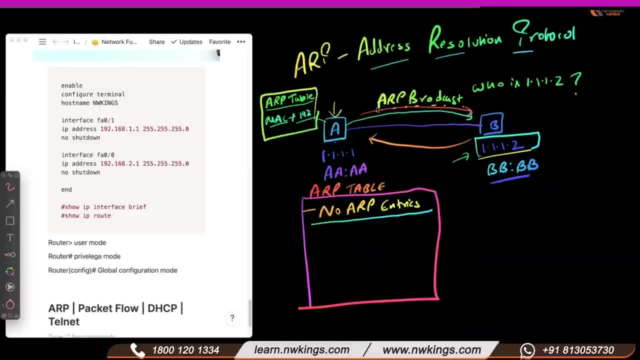 and if i don't have mac address, what i'm going to do? i'm going to send arp packet first before sending data to get the mac address. so i'm going to send a arp request. please give me your mac address and b will send. b is going to respond with his mac address and we are going to store that. 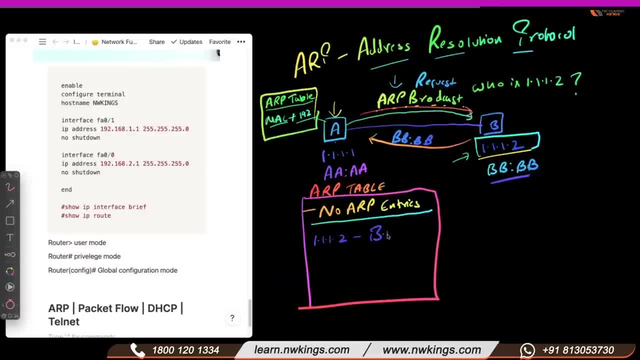 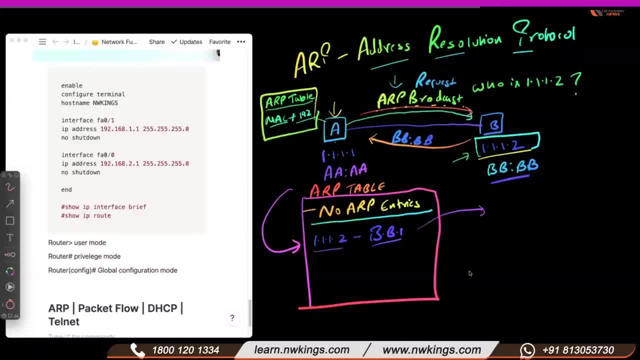 the machines don't send data to the device: clear yes or no, okay, great, okay. and this is the story of two computers. but when i'm going to connect with a router, suppose like this scenario- what will happen? if i want to go to the computer, go from 1.1.1 to 7.1.1.1, what will happen? 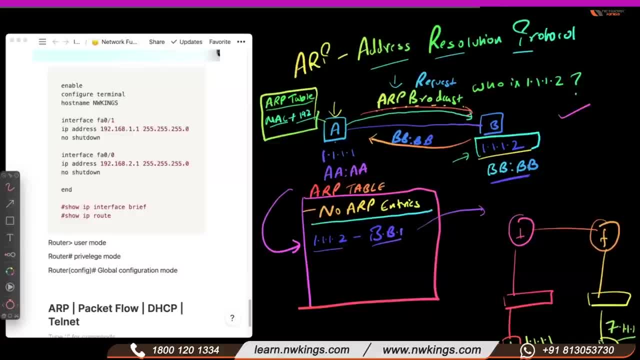 this computer does not have mac address of 7.1.1 right, so this computer will not have 7.1 mac. then i'm going to send information with the help of router to another network, because router is a device to connect with the different network and this network, and this network is in different. 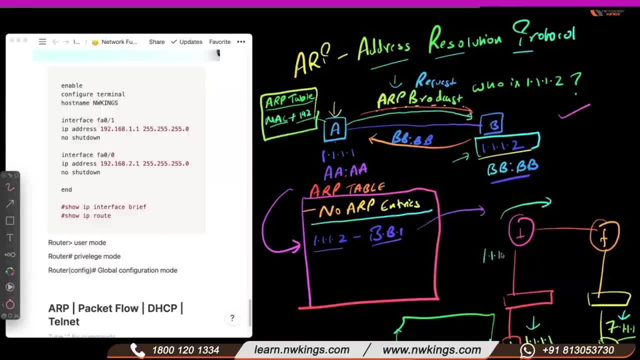 network. so i'm going to connect with this network and this network is in different network, so i'm. so i'm going to get the mac address of my gateway. what is the gateway? the router ip is known as gateway. so instead of getting the arp entry for different network device, so my computer will have 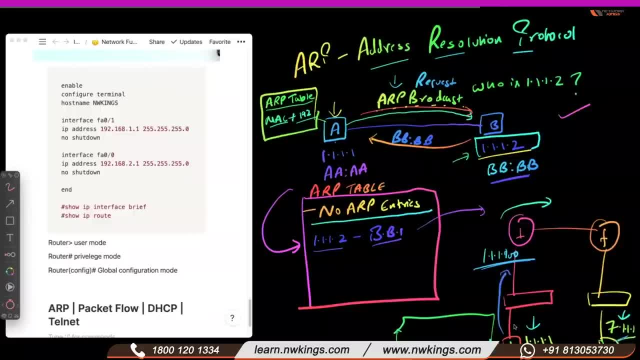 arp request, or my computer is going to send arp to my router to get the mac address of router. so instead of saving different network mac address, i'm going to save the mac entry for 1.1.100 and corresponding mac address, like, suppose a double c, like that, because i will only 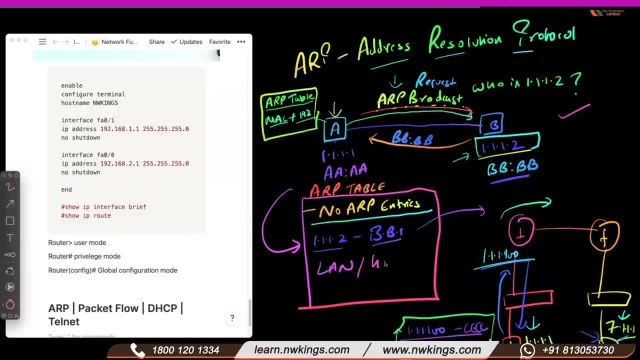 have my lan network ips or my gateways mac address in my arc table because, uh like, if you want to connect different network, you need a router. okay, and router does not forward the broadcast packet, and arp packet is a broadcast packet, so if you are going to send a r message, router is not going to forward to another. 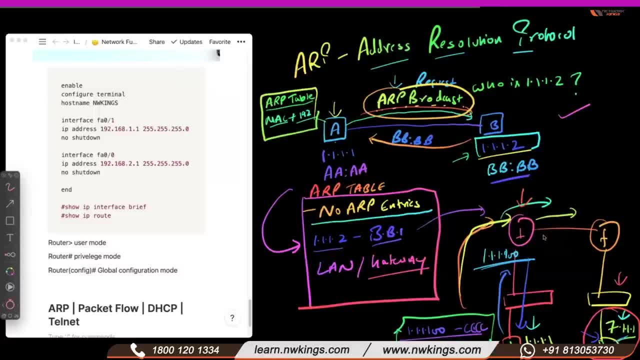 network because router stop broadcast. so if we can't send arp or broadcast packet to outside network, then router is going to respond with his mac address. so i i will only have mac address of my router. so this is a very good question, rajat. rajat is asking how computer will understand if the another device is in my network or different network. i'll explain. okay, that is known as ending process. 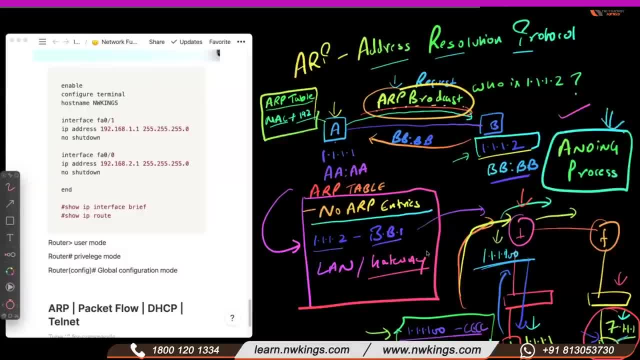 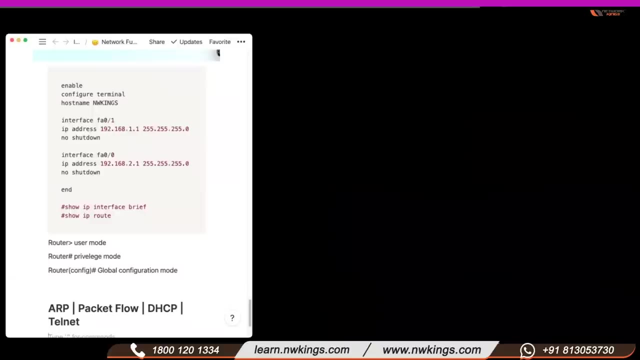 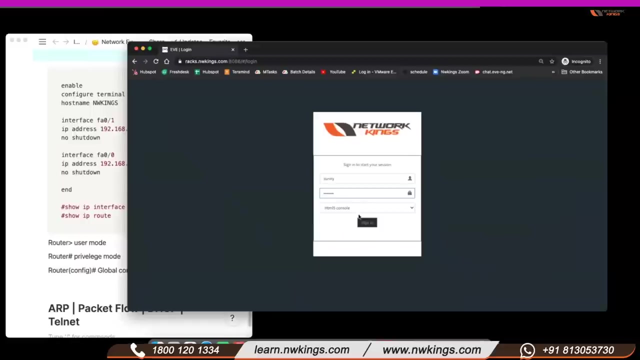 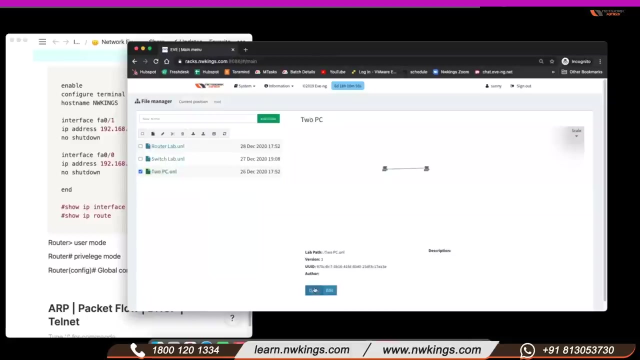 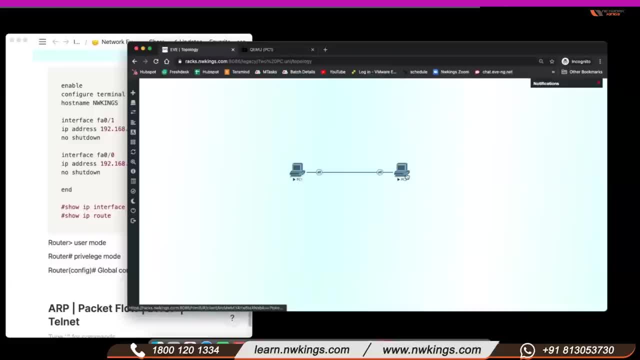 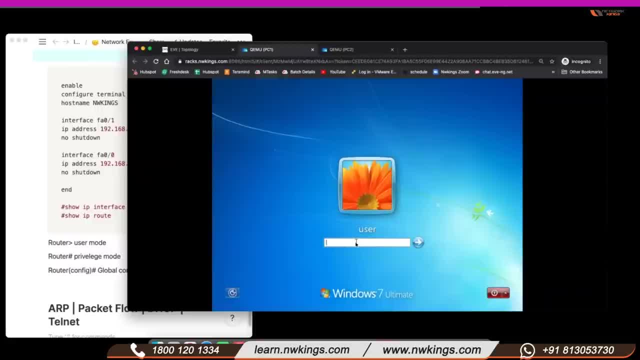 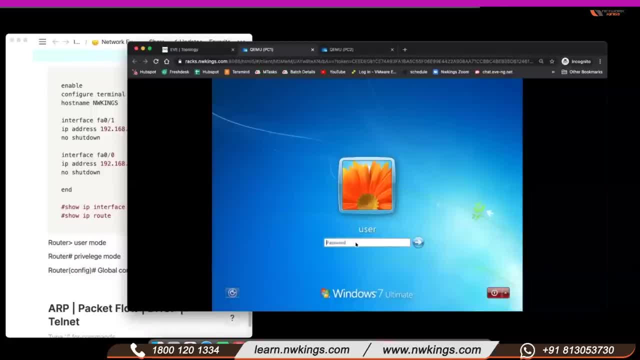 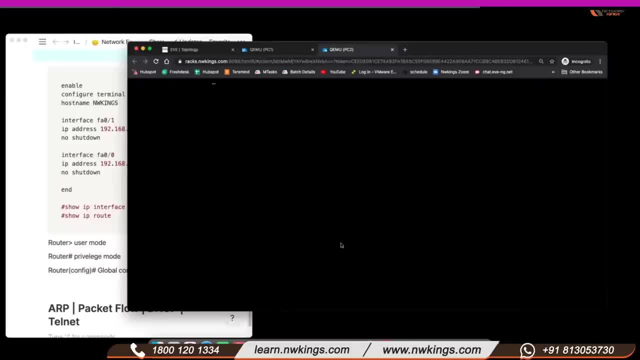 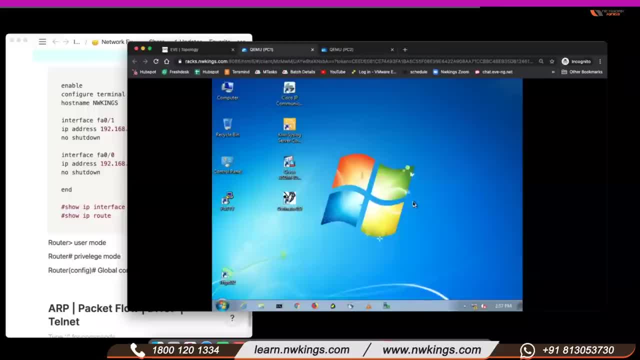 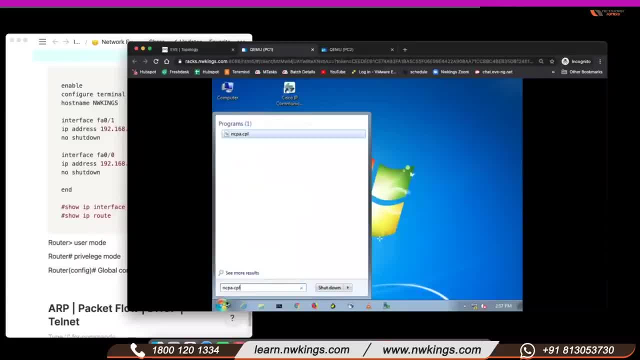 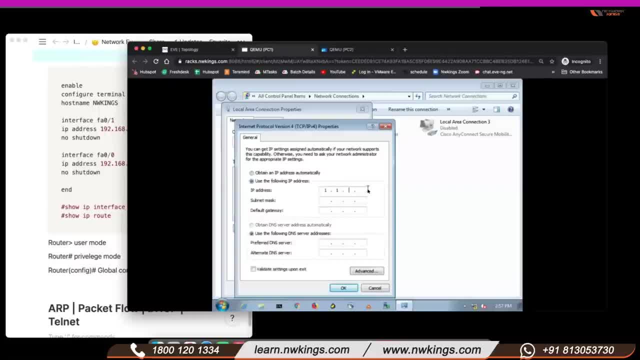 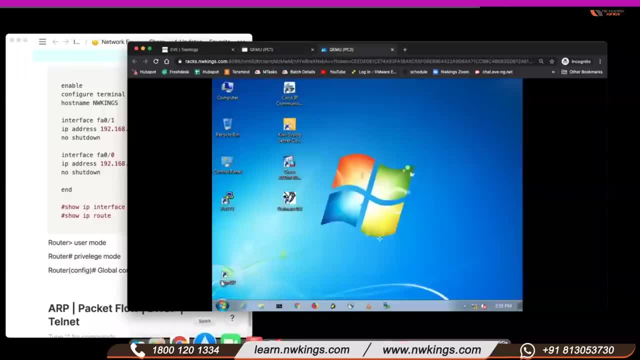 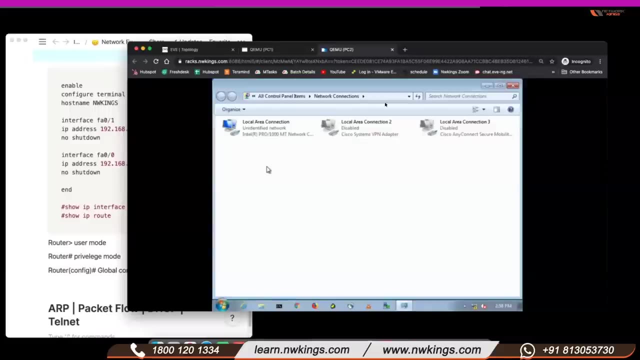 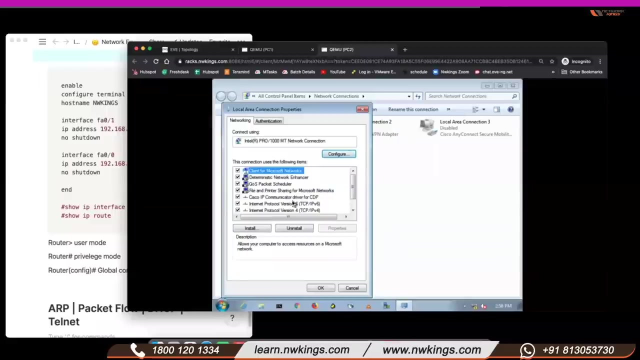 so my two machines are here. so my two machines are here. so my two machines are here, one one, one one. okay, so in another pc. see, from my last 11 years experience, trust me guys, there are many guys who actually come for interview, but it, it, it's not like that, they don't have very advanced knowledge. actually, the problem 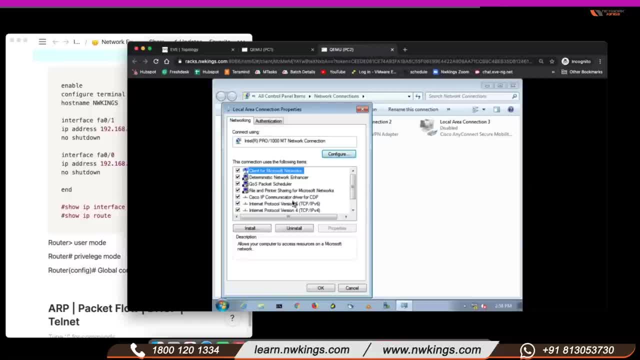 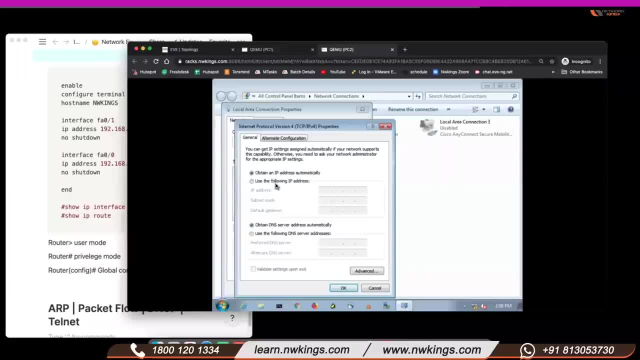 they are not getting selected in interviews because of their network fundamentals knowledge. they lack network basic knowledge. they don't know osi model, they don't know tcp3, hand shake and all. so to get a job you don't have to be expert. if you know the basic also, you can still try. 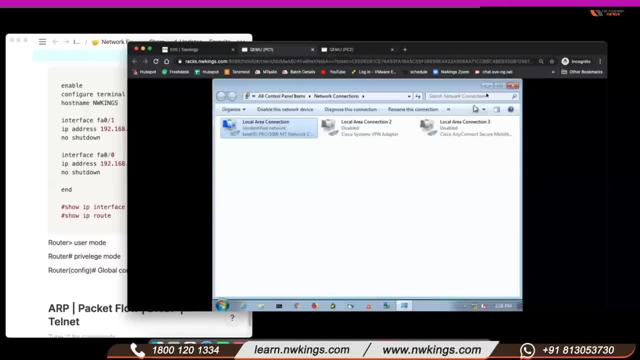 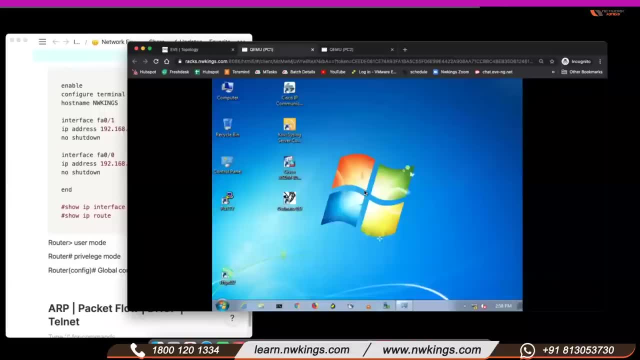 and get a job okay. so rather than becoming a network ninja, before learning expert courses, you should be very good in network basics, like one guy asked me with this question just now: rajat mittal, sir, how computer identifies if the network, if another device, is in my network or not? 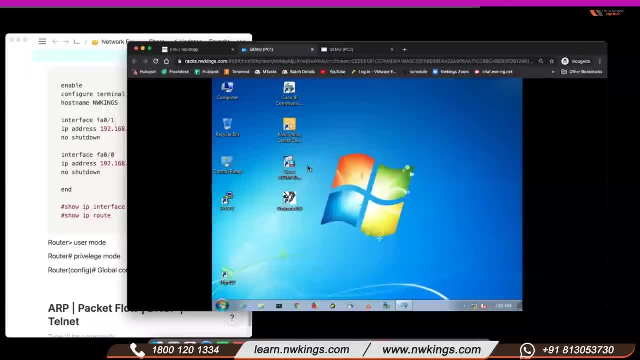 so if you don't know this, it means you will not crack very good interviews. actually, it's a process of ending, so i'm going to explain it today. cisco ios is developed on unix or linux. it's a linux based operating system. yeah, fundamentals never change. 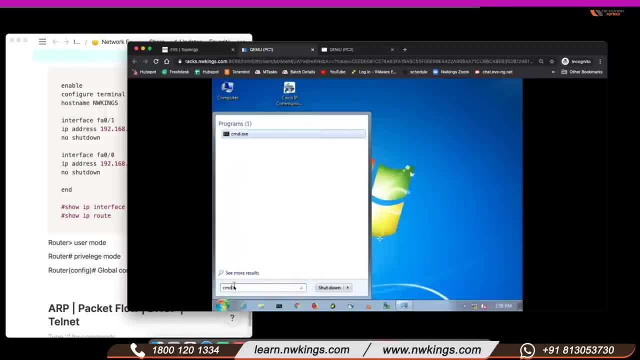 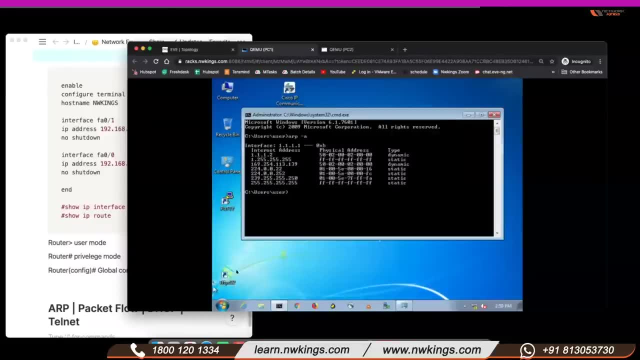 okay, so i have given the ip address. let's go on cmd and i'm going to type. first, let's see our table: arp, hyphen a. so i'm getting: uh, automatically, this, automatically, this computer is getting 1.1. let me delete this arp-d. okay, arp-d is to clear your. 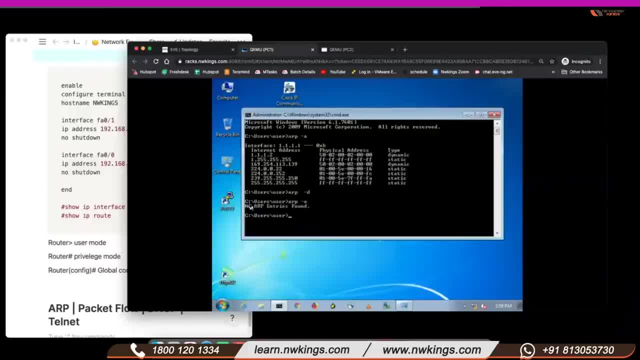 arp table. so arp-8 means my computer does not have any Mac address. so whenever I am going to send 1.1.2, any packet to 1.1.2, so what will happen? like whenever we send data, actually the network is very fast. you don't see any drops, right, because it's a LAN network. so actually my device sends. 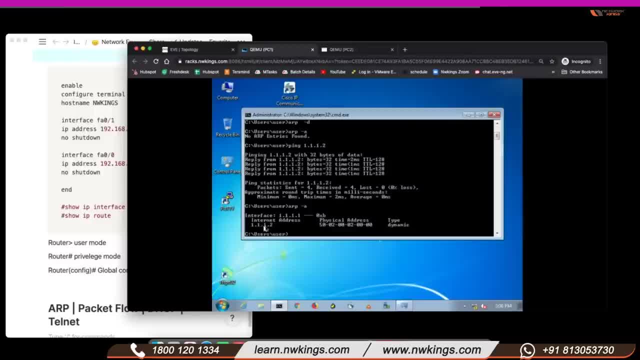 a ARP request first and get the MAC address of 1.1.2. you can see the MAC address is already in my ARP table before sending this ping packet or you whenever we send data, so the data will be on hold. computer is going to ARP first and ARP will get the MAC address of another device. then I'm 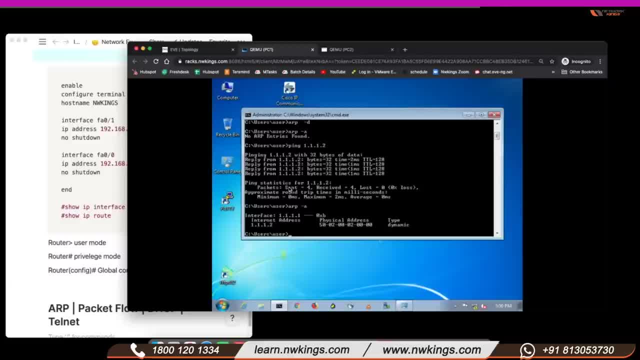 going to send data. okay, so means we need a MAC address of the same device where we are going to. if this computer is going to 1.1.2, I need a MAC address here. okay, so you can see. this entry is dynamic means the computer is generated, this MAC address or got. 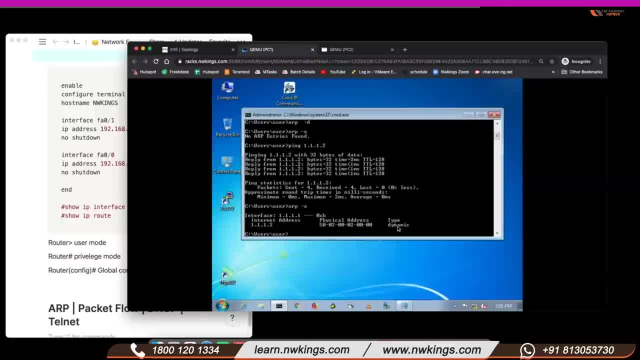 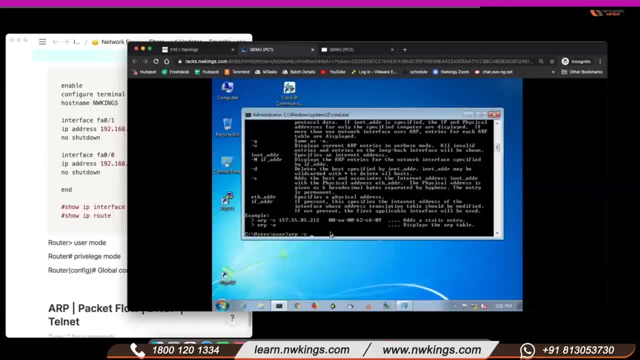 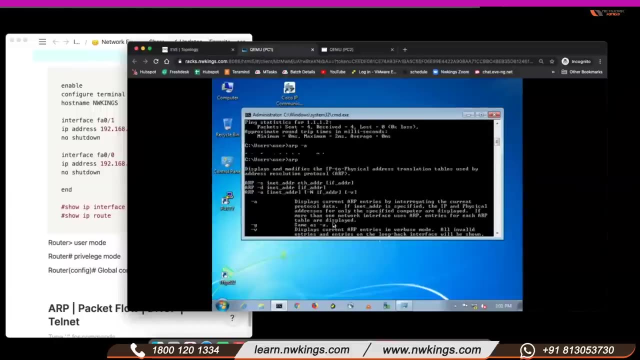 this MAC address automatically. this is not a manual entry, okay, but yes, you can do a ARP in Windows. you can do a static entry also, like ARP-S 1.1.1.2, and what would be the MAC address? let me take from here five: 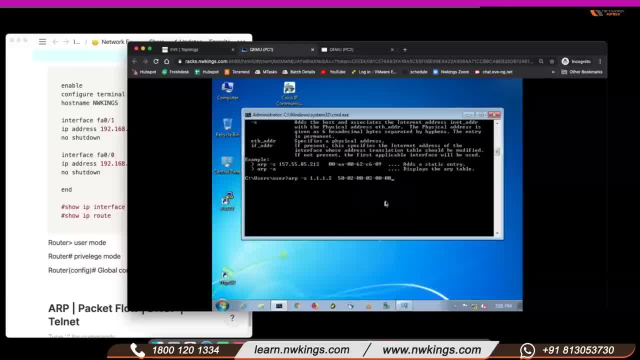 so, for example, I am going to going to message this one MAC address, so let me not flash this like a swag. now I can this MAC address send and if I did this, there means, like the ANV saved data- if this is plane value- to that monitor. I will send this message to unquote. 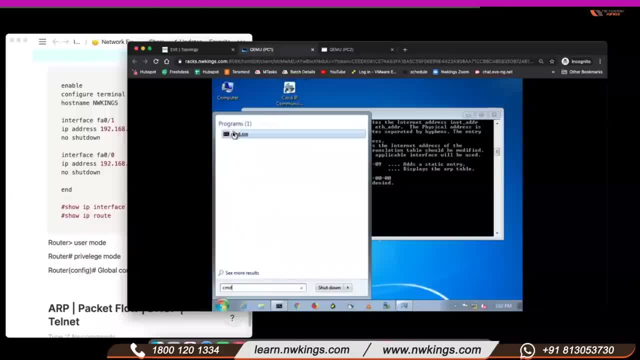 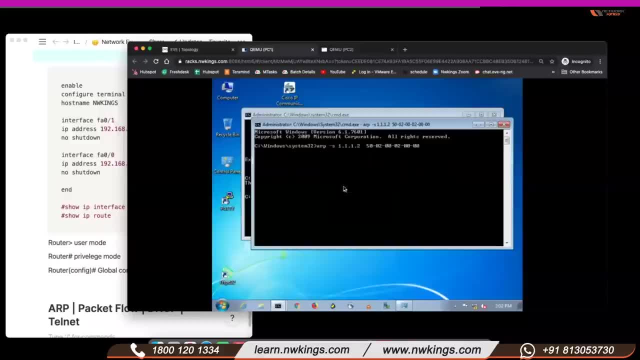 container. let me do this, so okay, so inside I can. this will send this message as point I will send, so I believe I should be able to attach this one to here and after sending it to this, your camera willち come here. Twitter paste: darp and tradition. field x is in it. 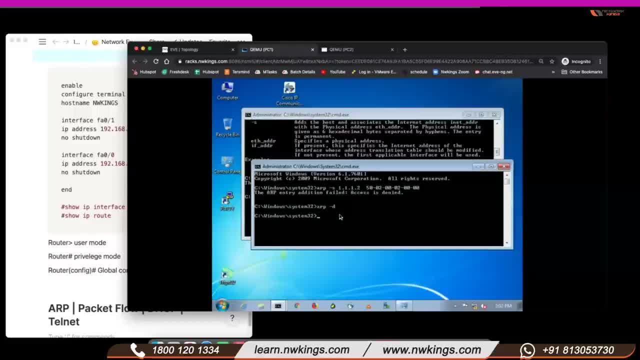 Maybe it's already there. This is the reason. Yeah, now it's taken right, So let's check now. arp-a. So you can see this is a static entry, So my computer will only listen this MAC address or only send the information to this MAC address. 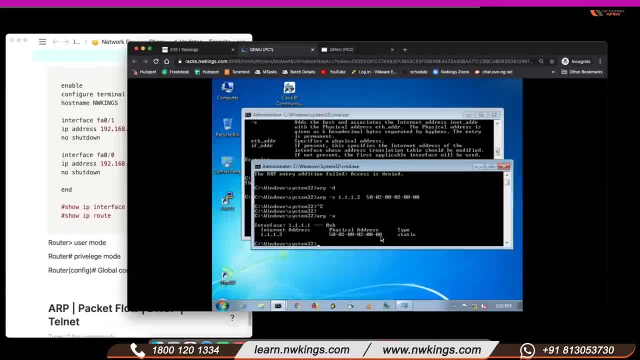 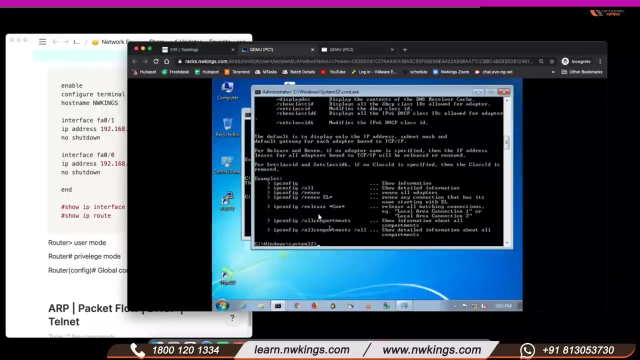 Okay, it's a good way if you don't want ARP broadcast. Okay, Yes, Got it. So in Windows there are a lot of commands, guys Like: if you learn this CLI, so it will help. So So in Windows you can give the command with like. 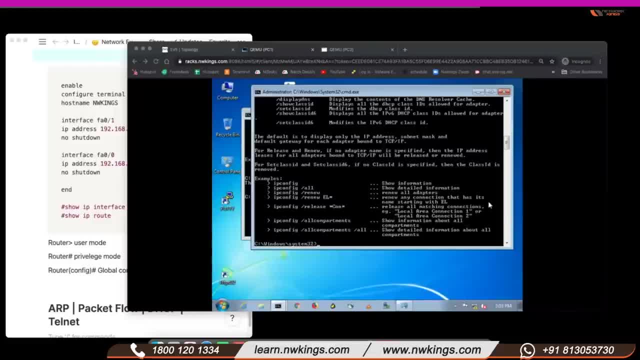 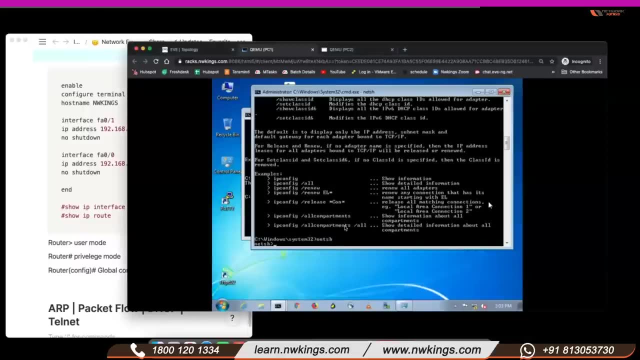 if you want to assign IP address, so you can give the name also. or you can assign the IP address from commands also. Like there is a command It's called n-netsh, so netsh. So you can see I'm an inside n-netsh and here I can give the IP address. 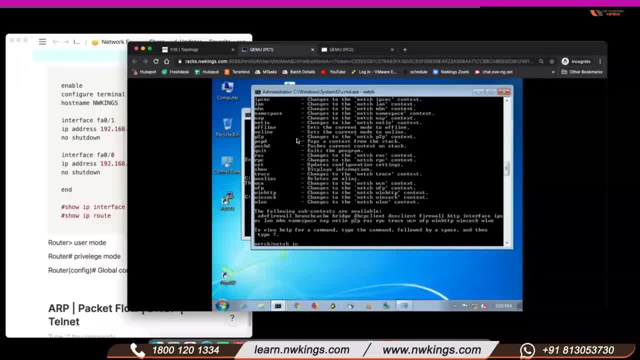 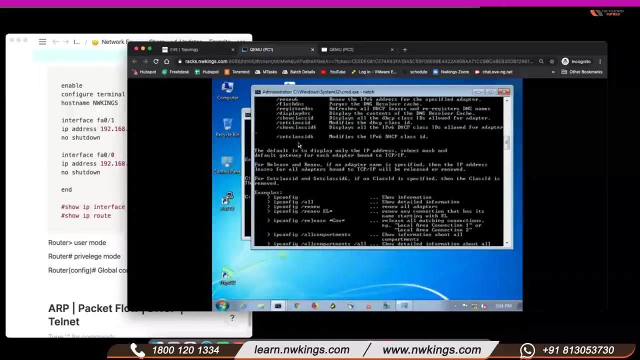 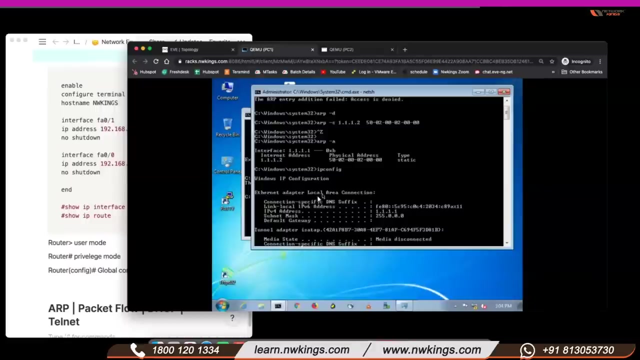 So netsh interface like that: IPv4.. Set address name. So my interface name is, I think. So what is the command? my net interface name is: I think this is the interface name. Yeah, So this is my interface name. 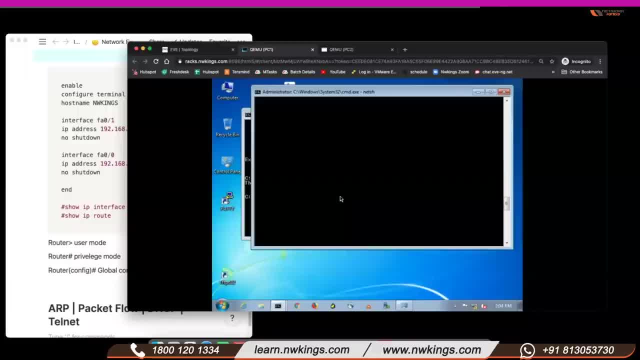 So this is how you give actually IP address. You can Google it And learn about the net as such. So I remember I used to give IP address with the command also. So right now. So this is just to have more knowledge, nothing else. 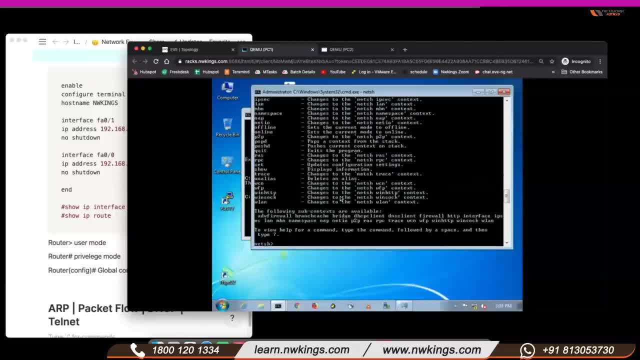 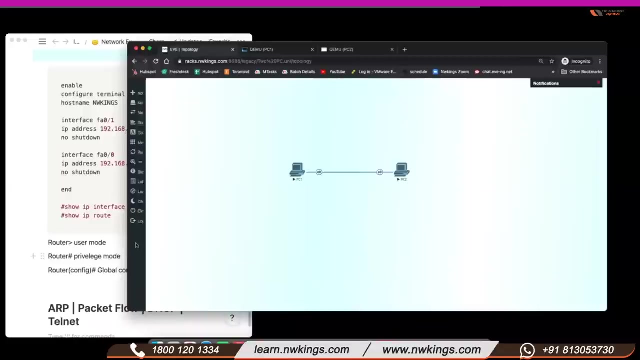 We know how to give IP address, So that is also enough. And if you want to give IP from here, you can also give IP from here also. Okay, So we have cleared the Okay. So this is all about ARP. You can check. 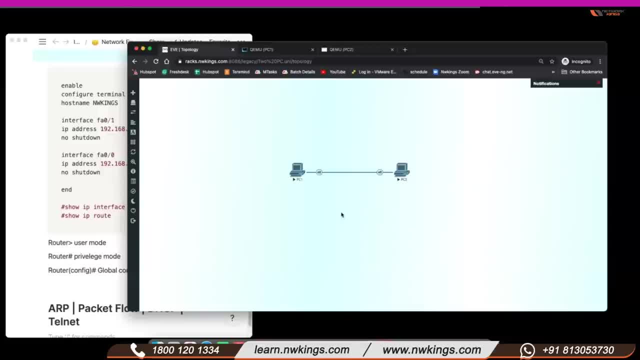 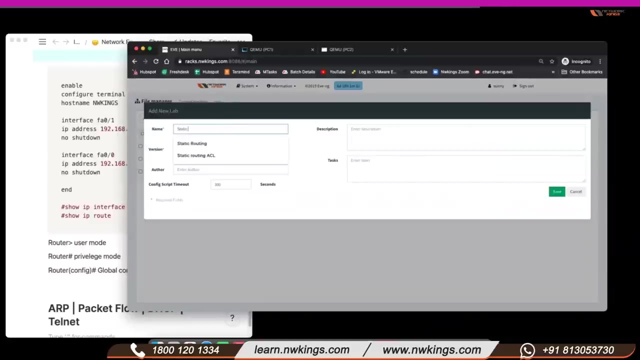 there. like you can just type net sh, hyphen help and it will show you what are the commands used for. okay, so so now we are going to do a lab again. so in this lab i am going to add four routers, so this lab will be known as static routing. okay, so i'm going to do a lab for static routing. 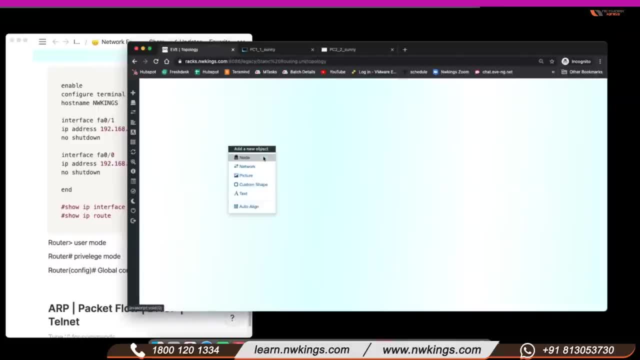 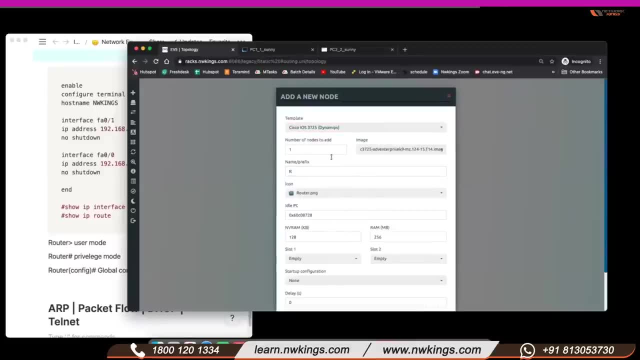 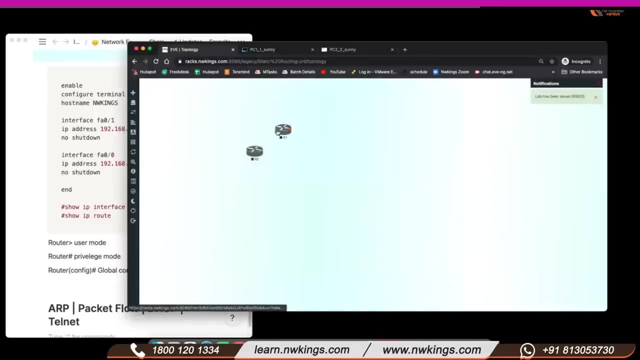 so in this, what we are going to do, we are going to take two routers. okay, so these are my two offices. okay, so you can just take an example of these are my two offices. okay, so i am going to take two routers. okay, so i am going to take two routers, okay. 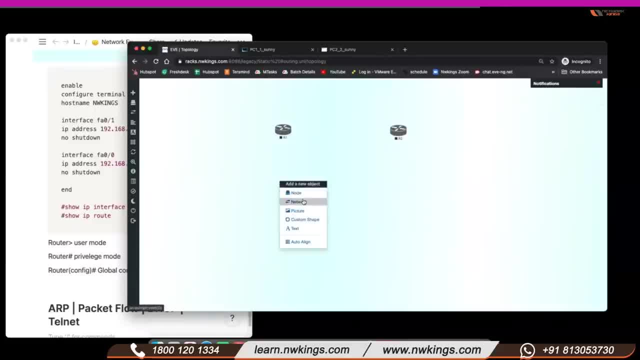 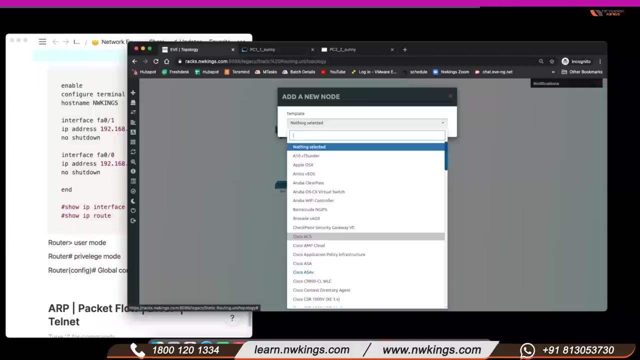 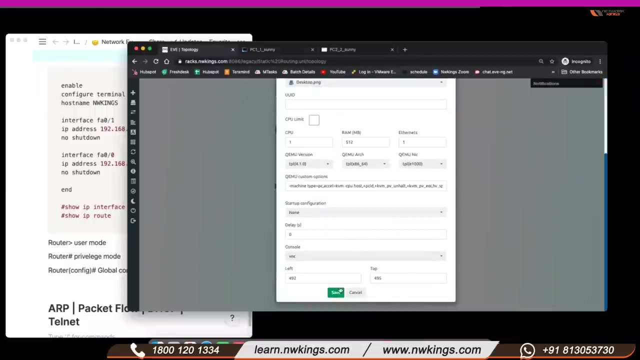 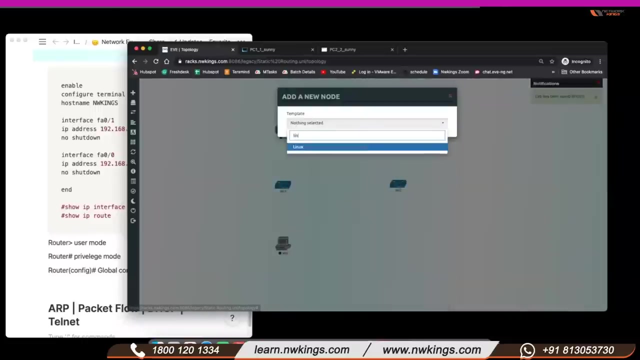 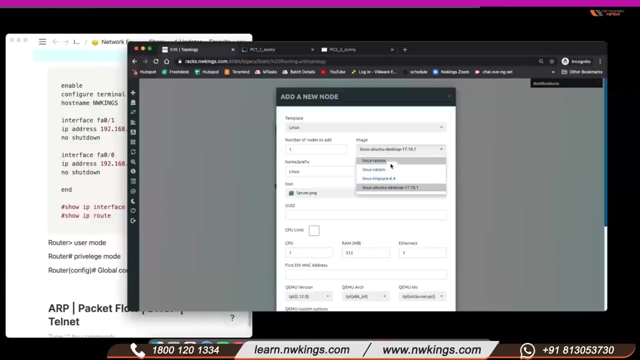 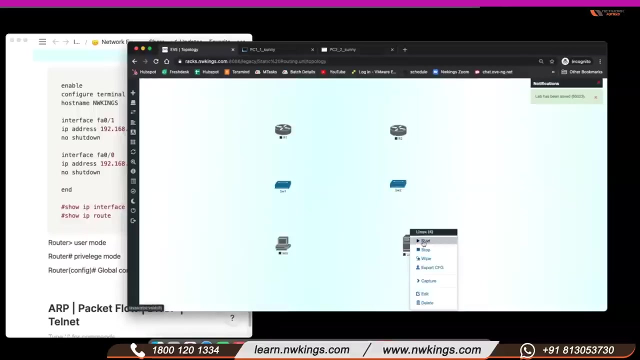 of branches or two offices, so i'm taking two switches here. so in the yesterday practical we have only, we had only one router, but here you can see i have two routers. okay, so let me add here one linux machine. let me check if this, this linux machine, works or not. 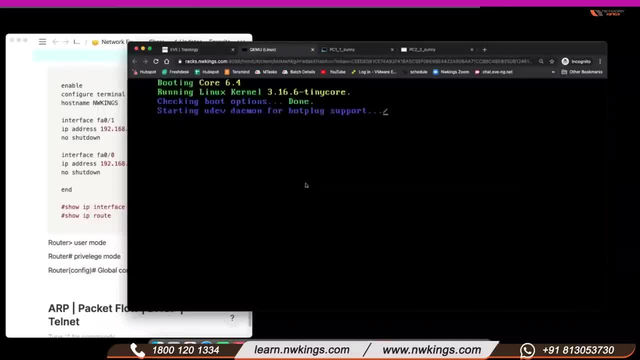 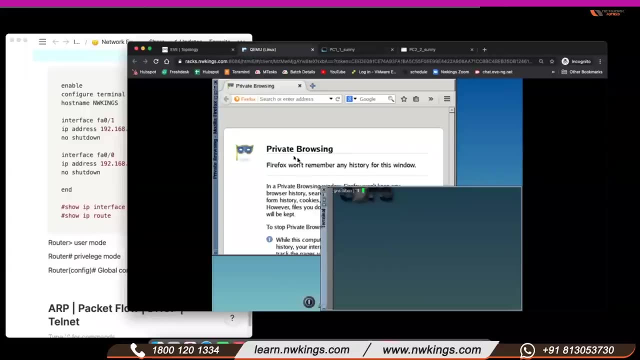 yeah, so this linux machine is working fine and we can give ip from here. or, yeah, so this ip is showing me. so we have not given any ip to this linux machine. so i'm adding one basic linux machine and i'm showing you here how to do this. yeah, and i'm adding to an side. 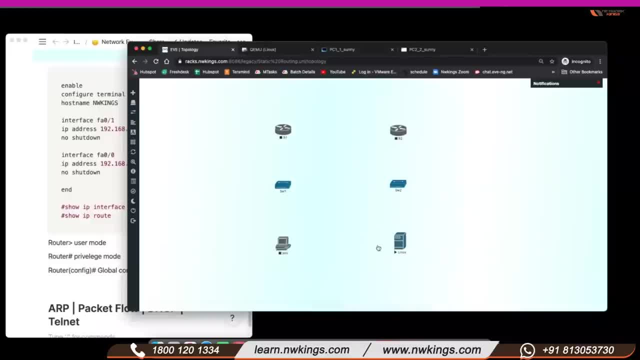 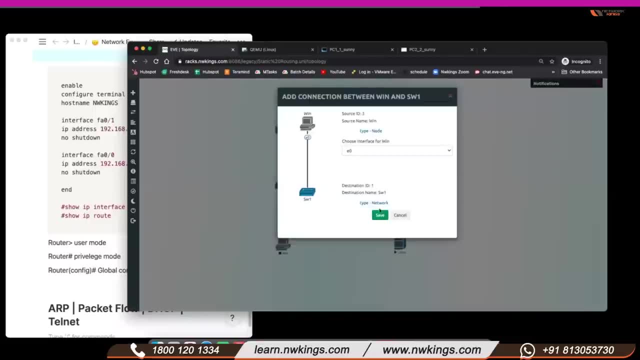 line. i'm showing you how to do that and i'm adding to one side line and i'm adding to that there's a machine over here so that you can run few commands for linux also. okay, see, we need to learn multiple technologies so real networks are mixed. we can't stick to only 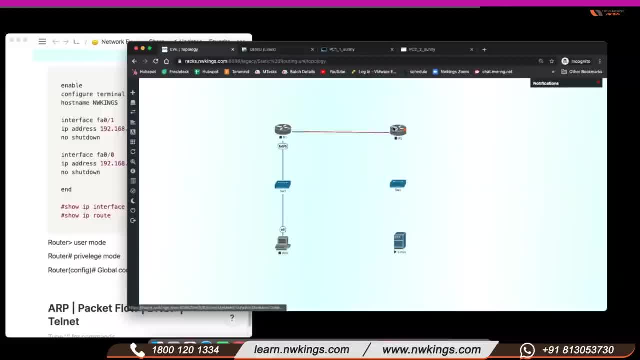 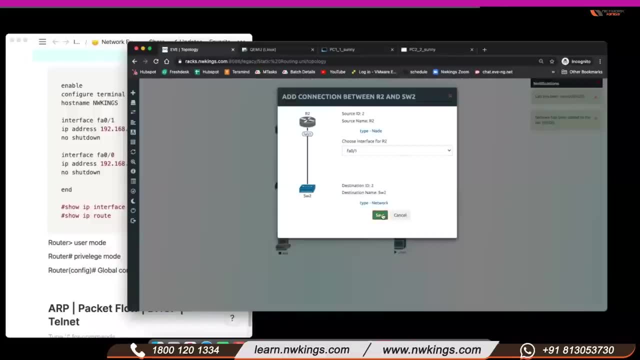 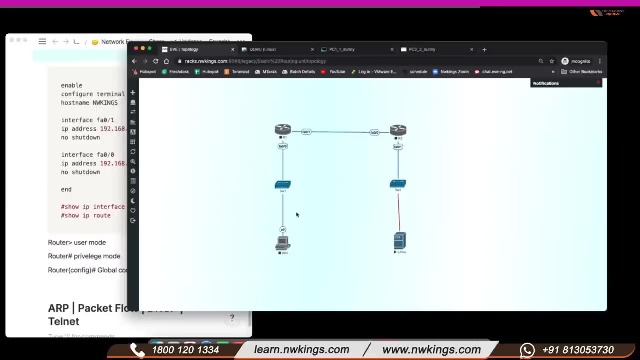 router and switches. we need to learn a few other things, and linux is very important for even network engineers. so when you will be with any good company, they actually get the logs on linux machines. so we need to find the logs with linux machines. so that is the use of linux, if you are asking me. 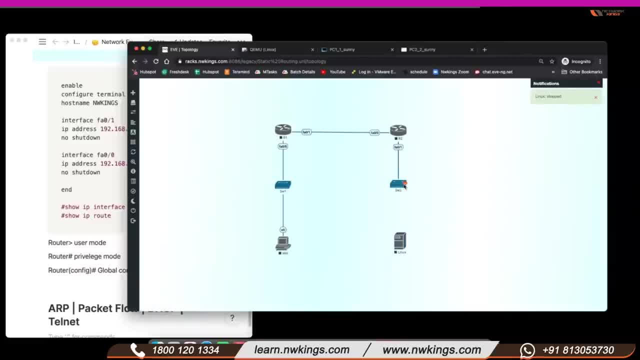 why we need linux or why we want to learn line linux or linux, whatever you want to say. okay, so this is my topology. look at this works good. yes, guys, it's visible, okay, okay, so what i am going to do? i am going to divide one network into two parts because we have learned 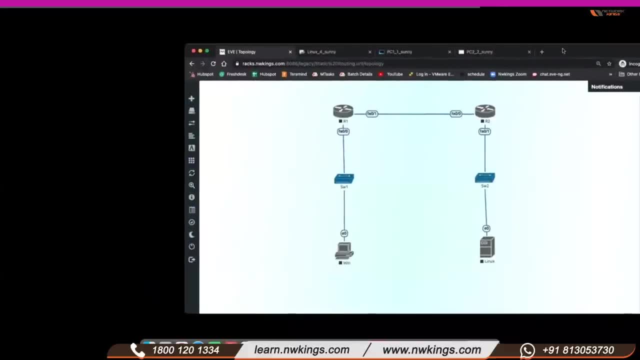 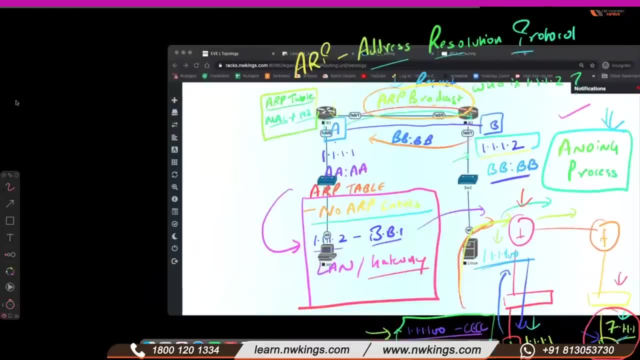 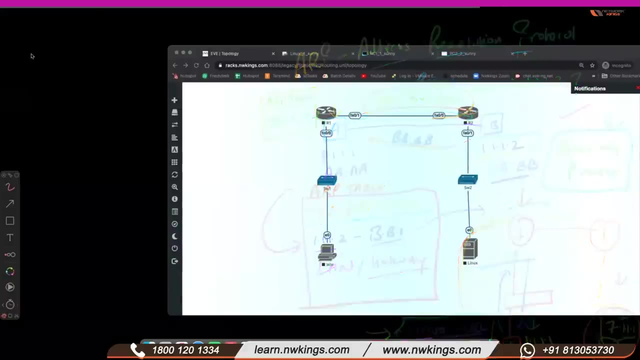 basic subnetting. so suppose we have a network that is 192, we have a network 192 168. okay, so we have a network 192 168, 1.0, slash 24, and i want to divide this network into two parts. so what i? what exactly i have to do? so i have total network bits and host bits, so total. 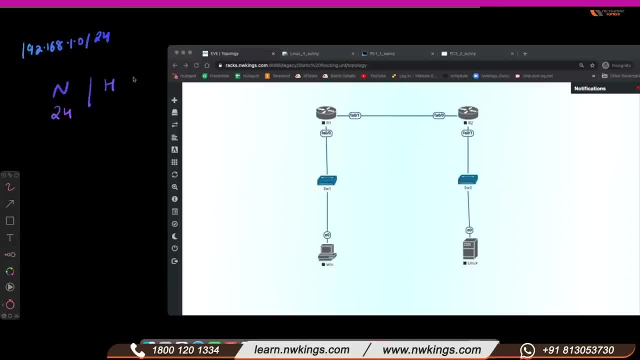 i have 24 and host is, and if you don't know this, just check my third day video. i have already shared the link. okay, so host is eight, right. so how many networks we want from this network? we want two networks. so if we want two networks, how we get two when we take to the power of one right? 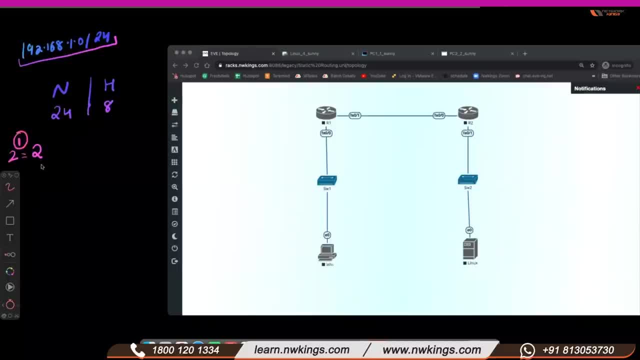 so just check the power. so we want to divide into two parts. so how we get two. when we say to the power of one, then it's two. right, if i want to divide this network into four parts, then i will have two the power of two. so we need to check the two. we always keep checking the power. so here i got the power. 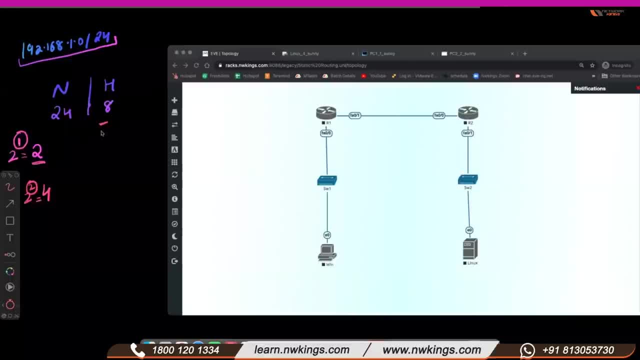 one. so what i'm going to do, i'm going to reduce one here and i'm going to plus one here. okay, because i need more networks. so this will be 25 and this will be seven. cool, so now this seven means to the power of seven is 128. so my network will divide 0128. it will go 255. 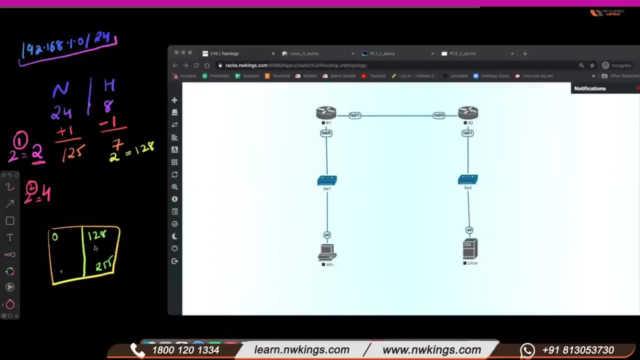 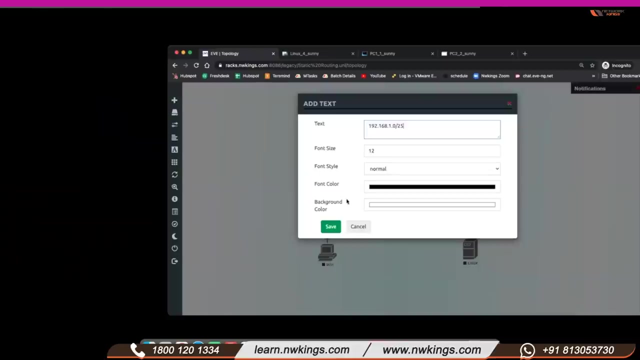 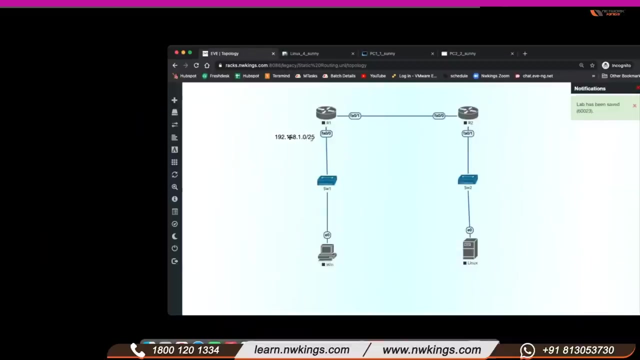 and before 128 we get 127. so these will be my two networks. super easy, yes or no? so okay, so i will have 192, 161.0, slash 25. okay, and don't worry, if you don't know this, you can keep checking the old. 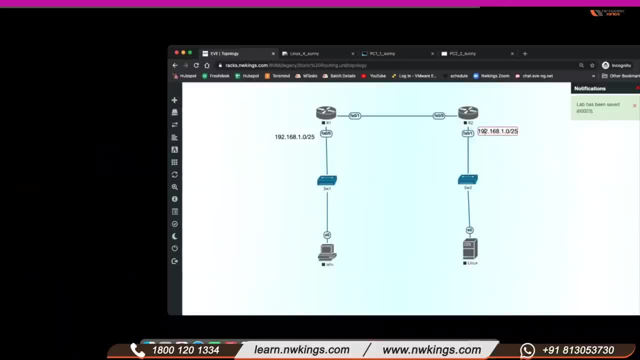 videos, and so here i'm going to give. see, we have two groups here, so zero we can't give, because this is the first ip, that this first type is known as network id. so i'm going to assign one. so i will write one here and from this block i will write either 129 or you can take a round figure here. 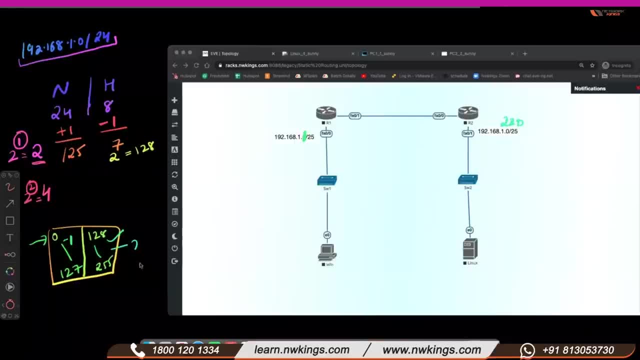 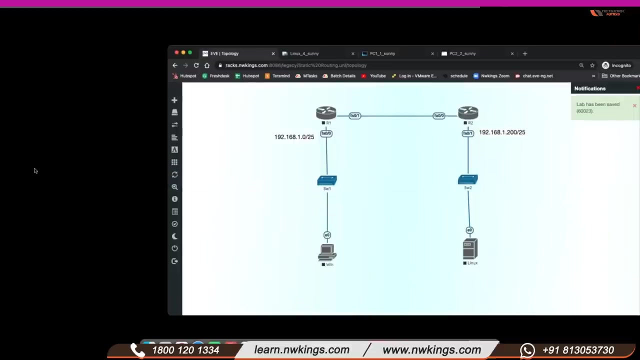 also like 200, because 200 ip is from this group and one ip address is from this group. okay, so, so i'm going to write here: 192, 161.200. okay, so these are two different networks. so why we have done subnetting? because we want to give. 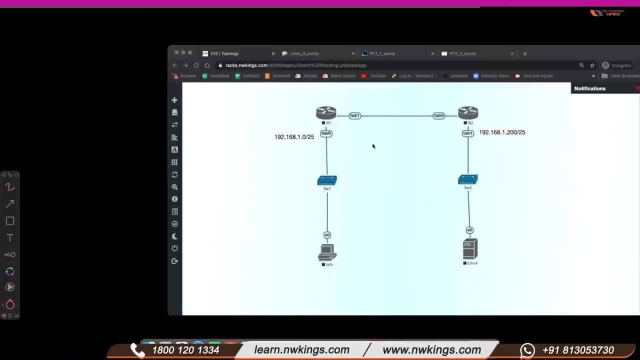 to our two locations. if we will not do subnetting, we have to use different network, okay, so between these two routers i need one another network, okay, so maybe i'll use. let's take basic one, so i'll not. so let's take another network. so i'm going to take here 200.1.1.1. 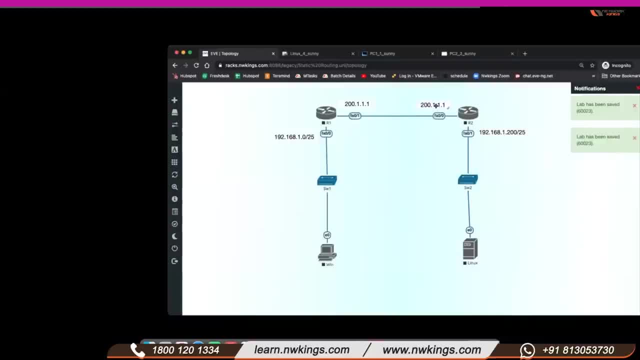 and here i'm going to take two hundred two. okay, so w ah ед can see my window machine. i'm going to assign here 192, 168, one dot ah, let's take one two, because here i'm going to give one two is 68, 1.1. 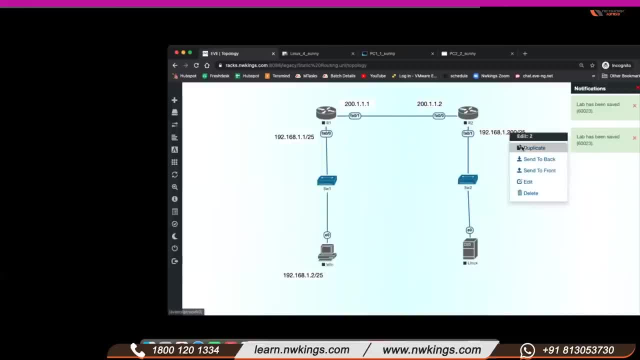 and below and below. here i i'm going to change a little bit atmosphere here, because now here i d to 192, 168, 1.20, and here i'm watching this videoяг going to use 201, okay, and this Linux machine I am using first time. maybe it's based on different IP. 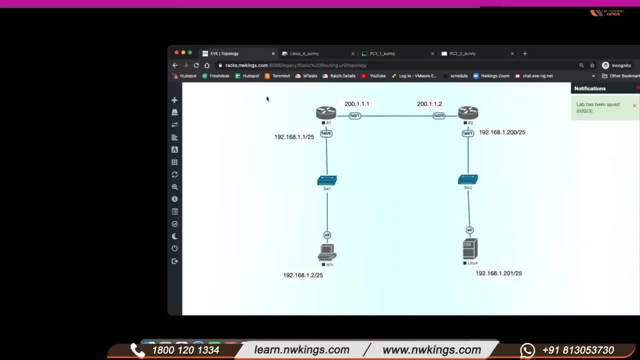 let's check how to give IP to this machine. okay, so let me turn on more action. start all nodes. so all of my devices are almost ready. okay, so are you ready with the left, or okay? okay, let's start. yeah, so let's count on thing why I'm not able to type. just hold on. 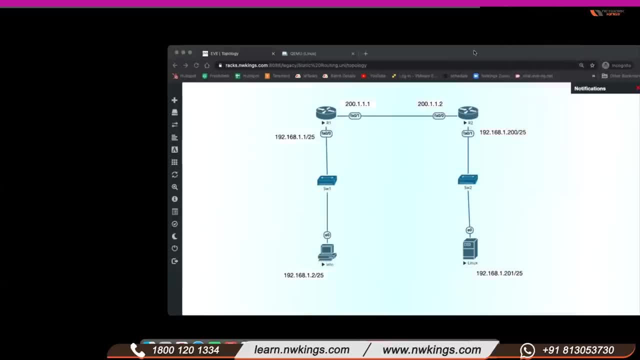 yeah, got it. so we have three networks. one is this, so one we have this network, another is this one, what? yeah, so one first network, second network and third network. so we have three networks, so first, second, third. so remember always, like when you connect routers, so router ports facing. 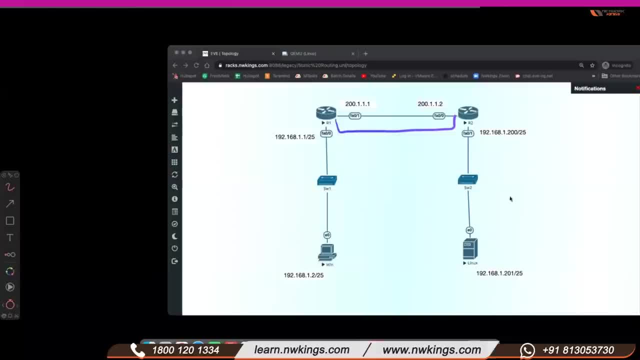 each other should be in same network. okay, so when we connect two computers with each other, they should be in same network. then only they speak, so it goes with the router. also, when we connect two facing each other should be in same network. okay, so here i am going to assign ip address. 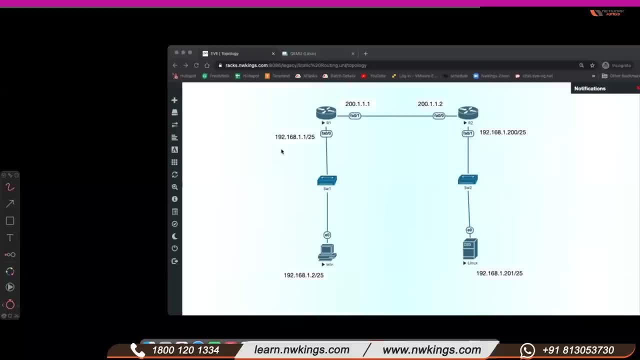 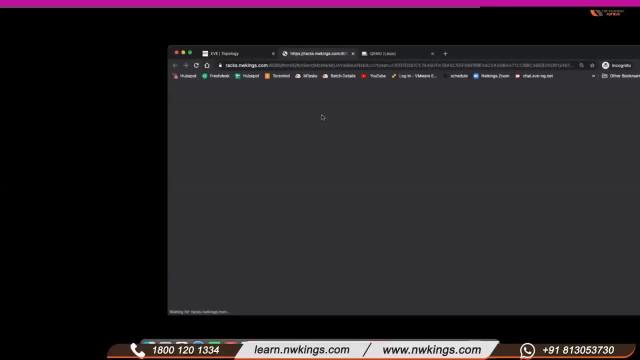 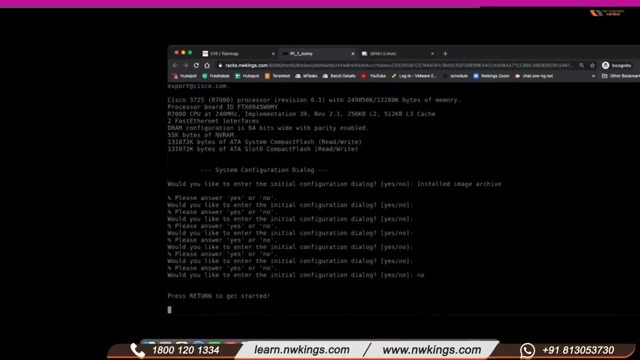 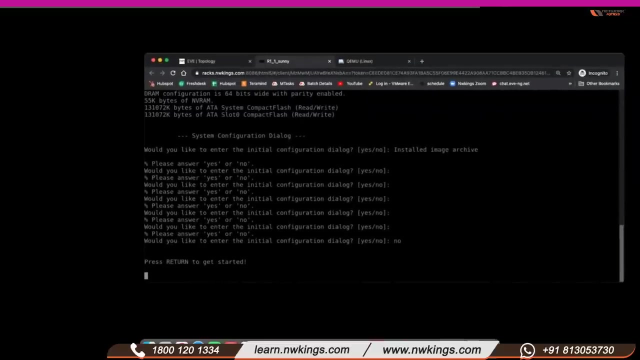 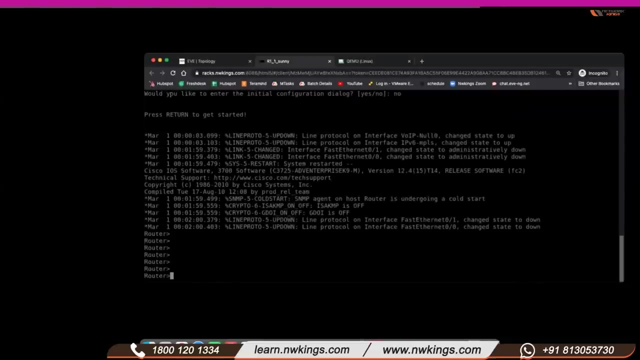 and then we are going to assign the ip address on windows computer. so let me start router one. so this is my router one. so remember always: we need to do no here. so now we are inside router. why we always say no here? because it is asking me if i want to do some automatic configuration or not. 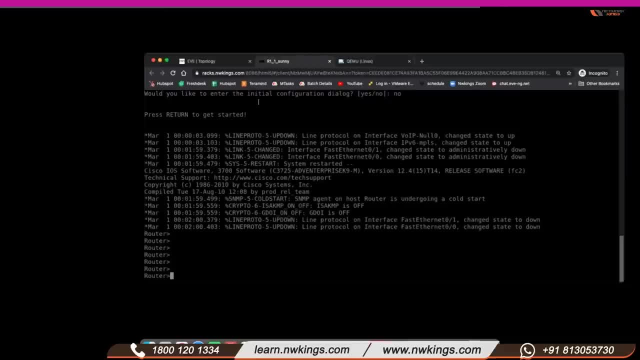 so just in a short uh like in, in a simple language, i can say that if you really want to become a network engineer, always say no. yes is for those guys who are like very beginner. okay, if you want router, will set up all the configuration for you. 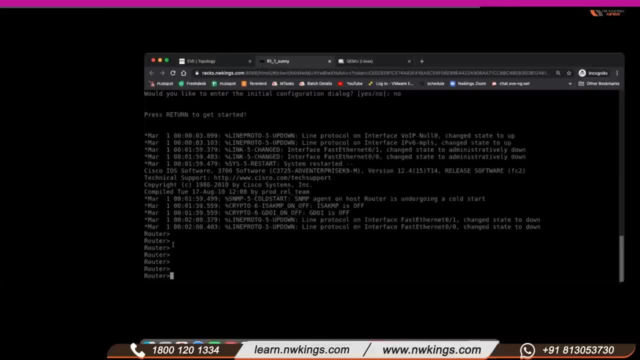 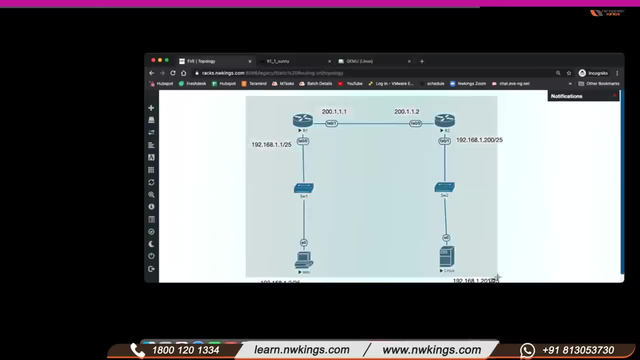 so always say no so that you can type the commands. okay, so this is my lab. let me take a screenshot. so this is my lab. okay, so i am going to type the configuration here. so what would be the commands? so i am. so this is a notepad. okay, this is a software which i am using for my notes that. 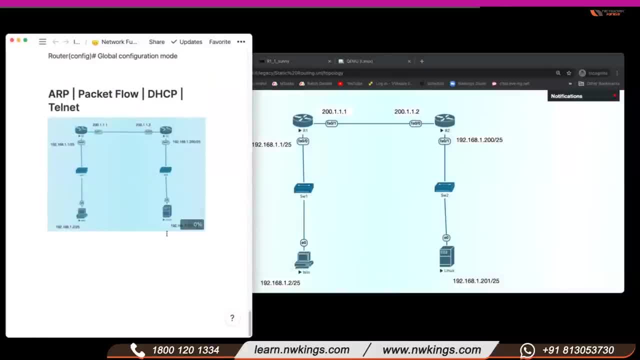 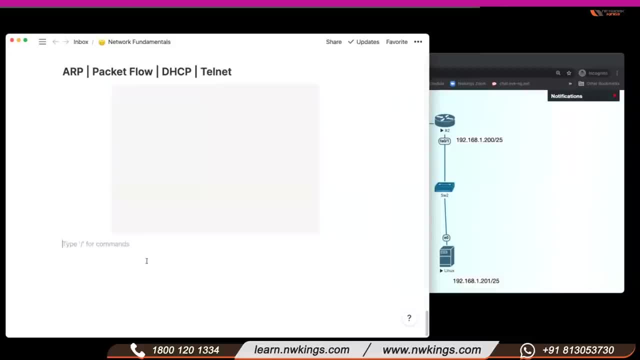 is a notion so you can use your hands events for that. if so, then here i am just writing among these european words here: um, essentially, if, if the country is your, your country language should be here regular pm. it will create your ownили. it is somewhat general. 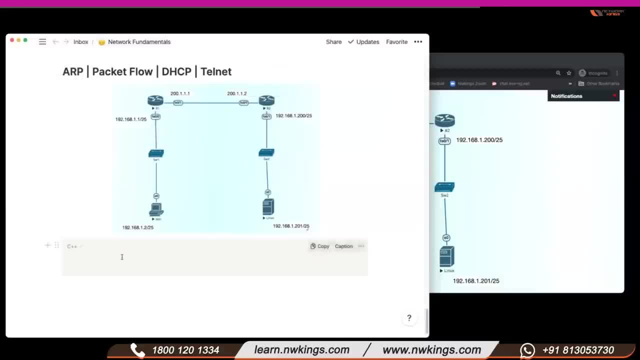 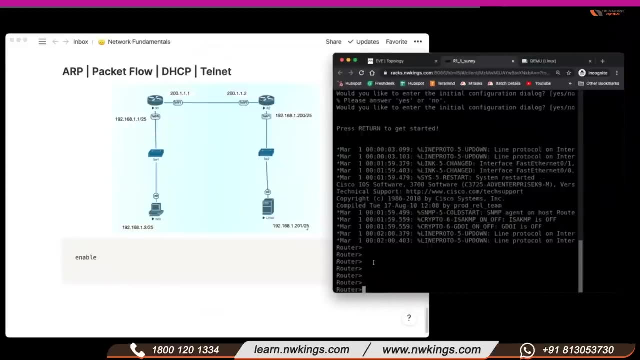 it is also not desirable. 여, you can use it for free. okay, so that is. i am first of all to go inside the router. i need to type one command that is enable. so i'll show you here also the commands and i'm going to type the. 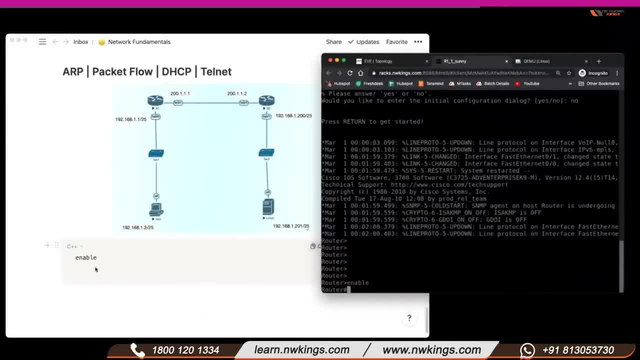 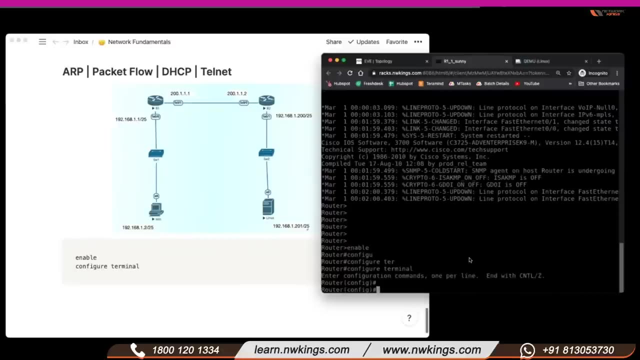 nodes for you. so enable. so once you go enable, you need to type configure terminal. this is the second command to go to the upper level, so that i have already discussed, i think in second day, videos. so now we are inside router global configuration so we can change the router name. 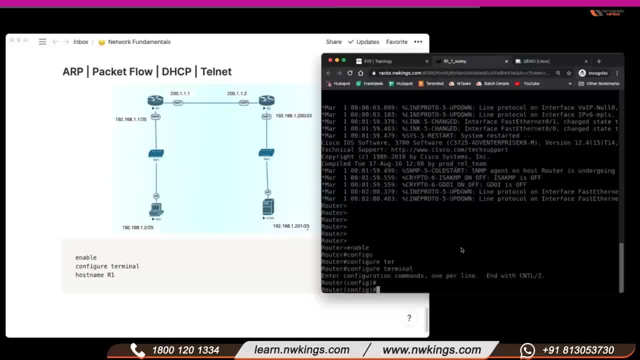 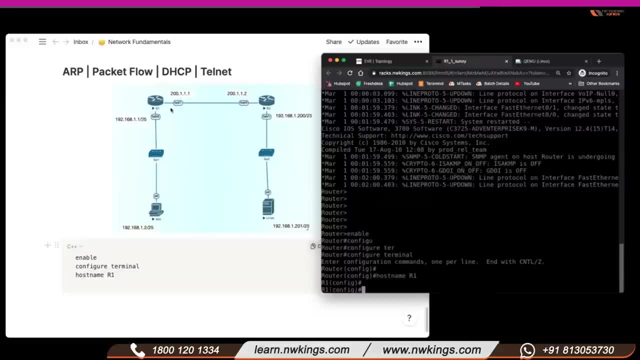 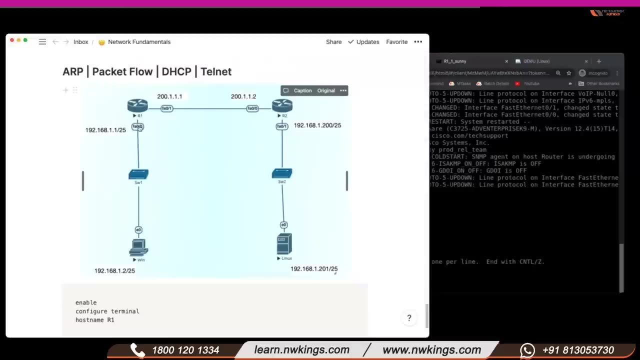 host name r1. host name r1. so you can see we have r1 now and you can see i have two interfaces. one is fa00, if you can see here, if it's visible to you. so fa00, that is fast ethernet 00, it's a port where my switch is. 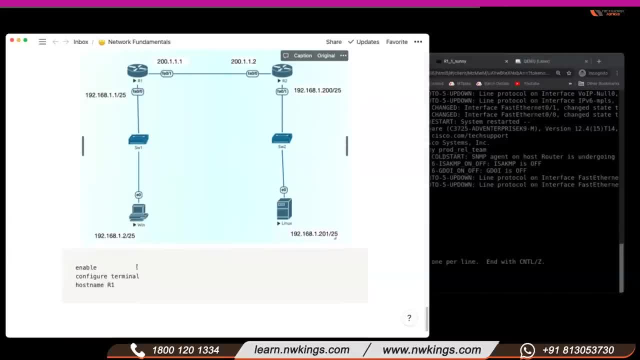 connected and fa01. that is another port. so inside my fa00, fa00, i need to give ip address. what is the command ip address? 192.168.1.1- 255.255.255. by default it's zero, but we have done subnetting and what is the subnet mask of slash 25, 255.255.251.28, if you. 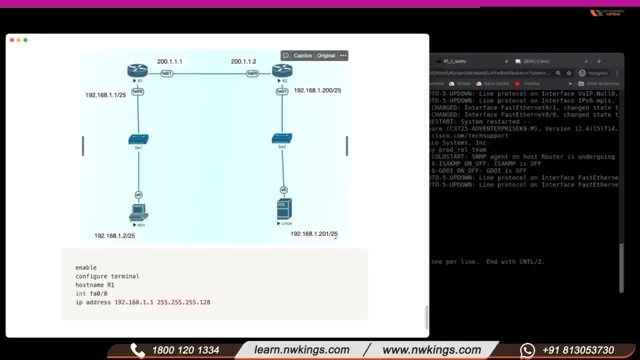 don't know this. just watch yesterday video means you need to learn all, all three sessions. then only you will understand day four. also, if you are skipping those sessions might be you will not understand. so no shutdown. okay, and on fa01, i need to give ip address and then you need to. 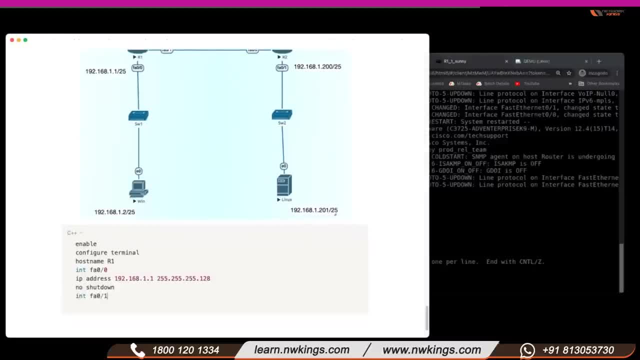 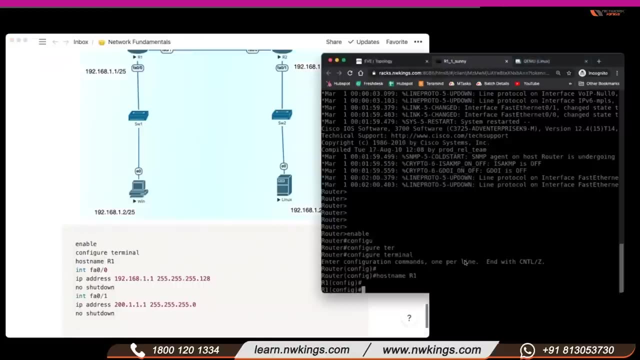 give 200.1.1, so interface fa01, ip address, 200.1.1.1, no shutdown. so we here. i am not doing any subnetting, so tell me, guys, if you have any problem in this. i'll share this notion link, don't worry. 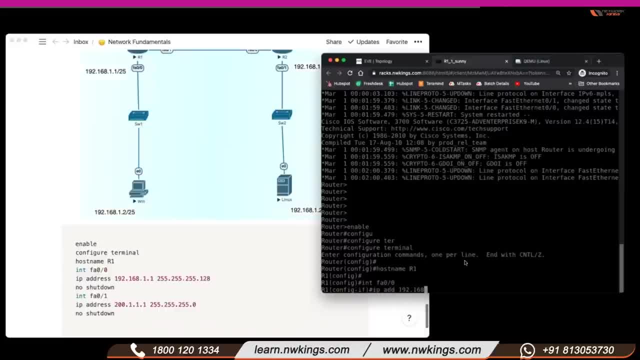 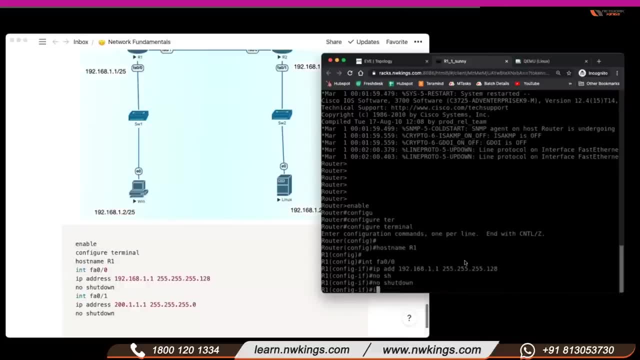 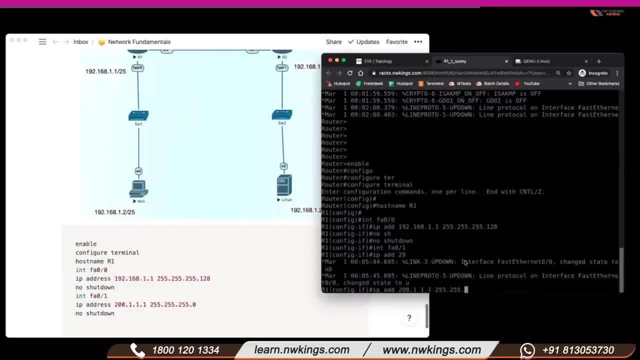 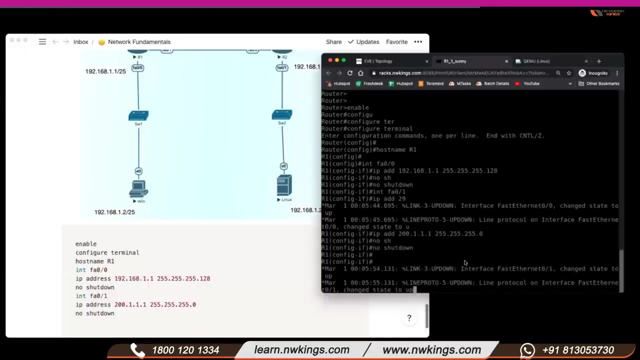 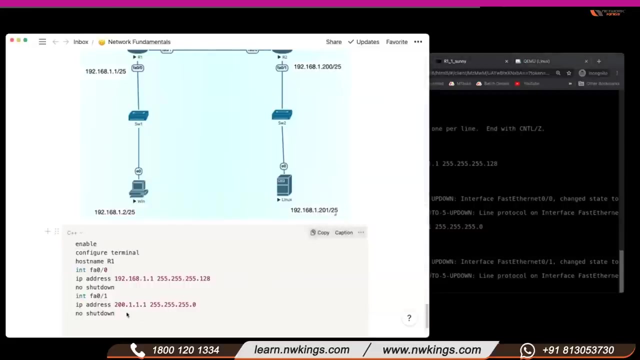 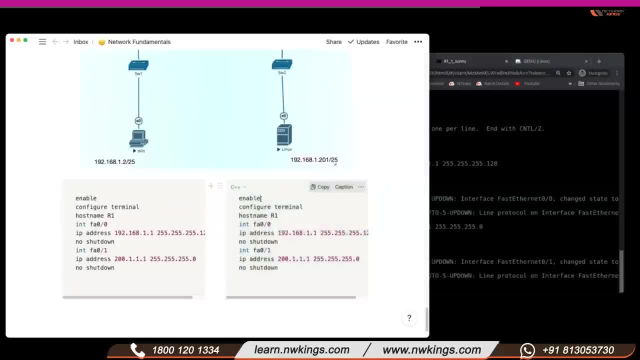 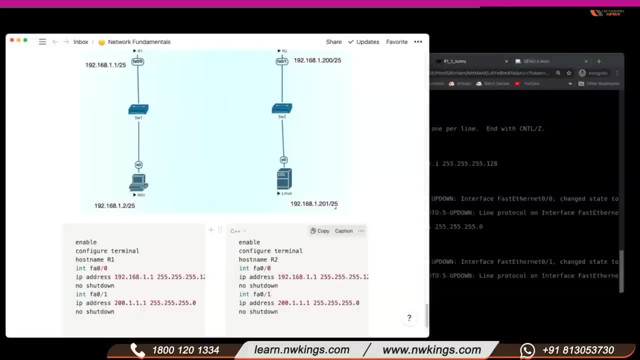 make a duplicate of this and i'm going to make a duplicate of this and i'm going to do this and i'm going to give just add here. so here i'm going to type for r2 on rii, fa00 is 201.12. 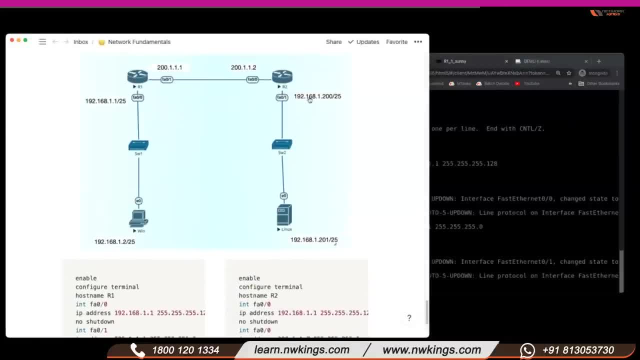 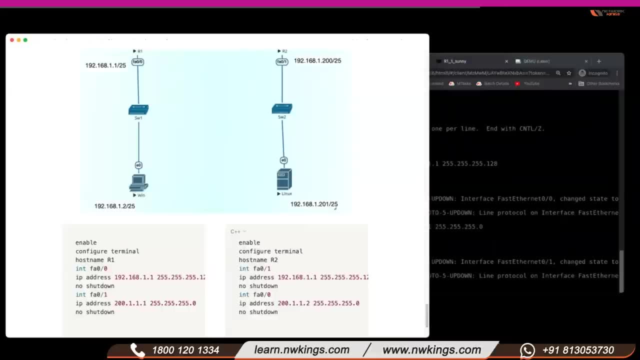 and on fa01 i am going to have what ip, Symf í, merely width, and I'm going to have one, and on fa01 i'm going to have one dot 200, rest. all commands are same. so just i have changed the ip address, change the host name and rest all. 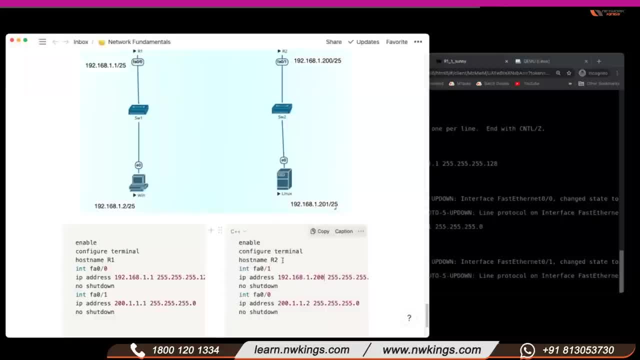 thing side is okay. so now I have shrimp WordPress also soывew wall id. also change the ip address, change name and rest. all thing side is okay. so I am going to set my name here as r2 best davOut pin just bolted in l'host. translate is good. now all commands are same, so just I have changed. 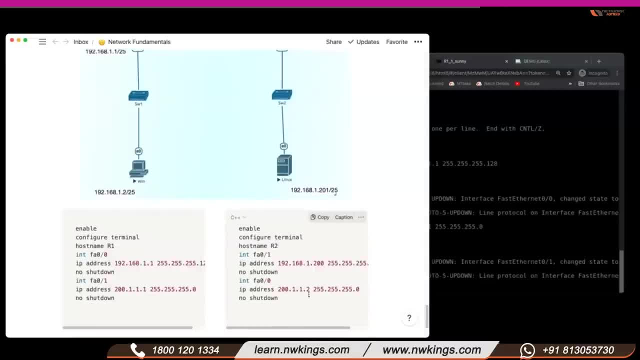 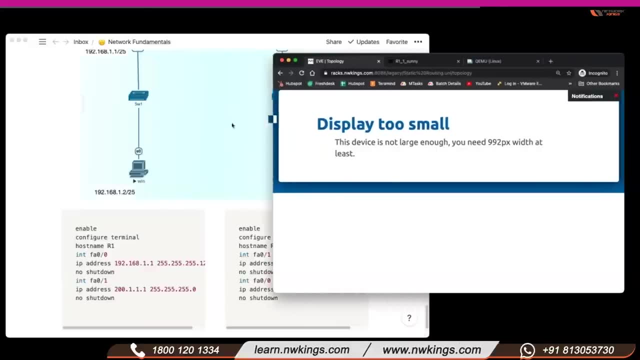 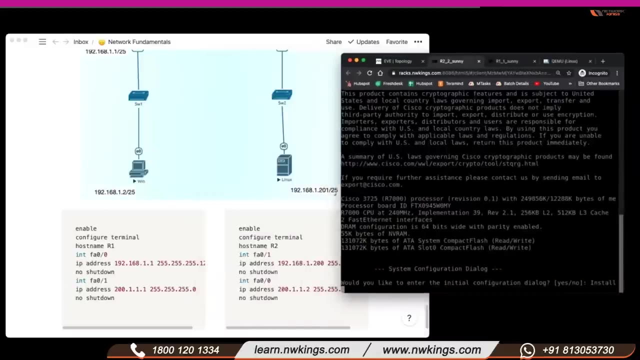 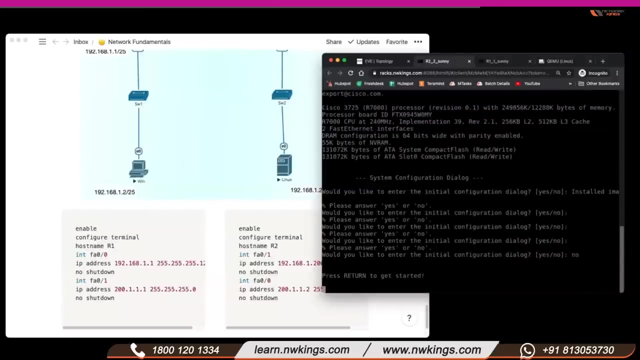 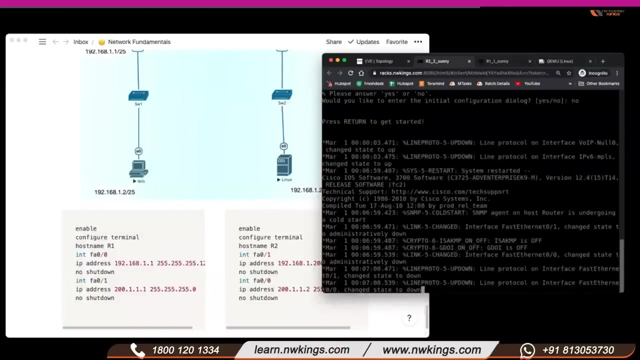 the host name and rest. all things are same. okay, so let's go to router 2 now. so this is router 2 and i'm going to say no. so give yourself a score out of 10. if you understand whole, just type 10. and if you understanding a little bit, just give 3, 4 score to yourself. 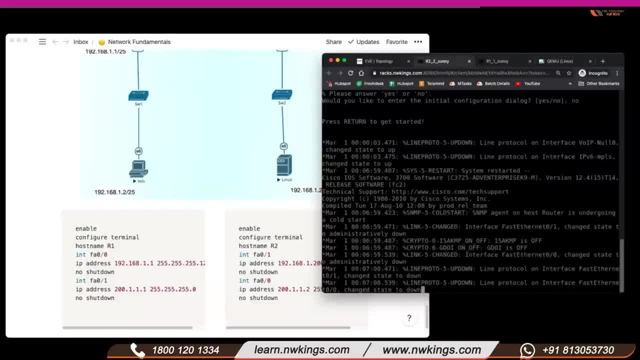 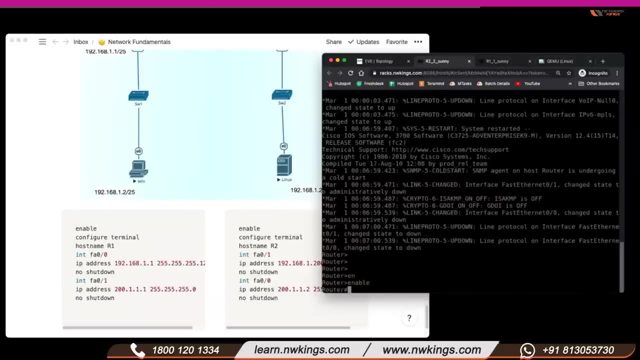 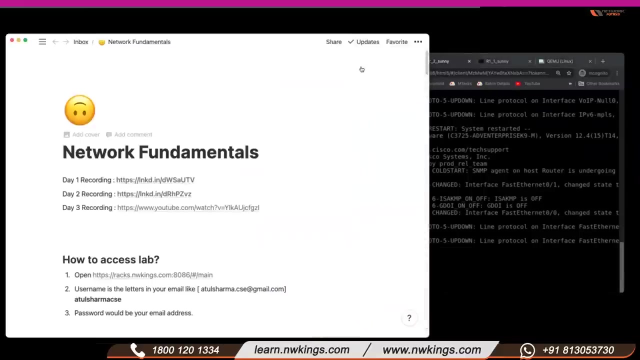 okay, great, okay, don't worry, i have already shared this. i'm going to share this link again with you. just watch these three videos first and you will understand, and you will also get 10 out of 10. okay, chintanji, you are watching from day one and you are still saying 10, sorry, 8. 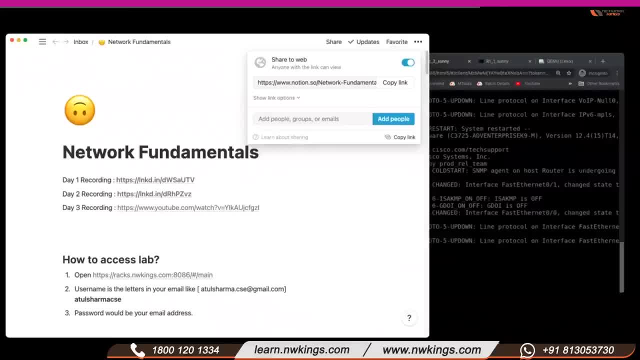 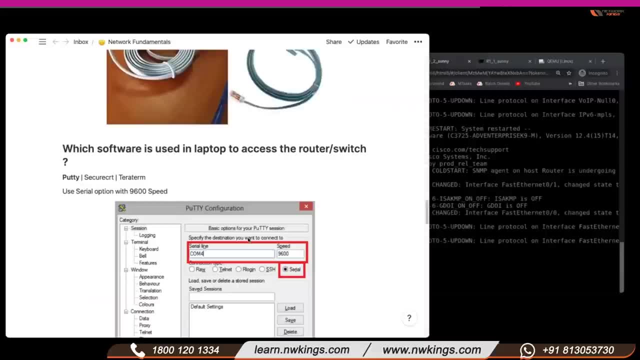 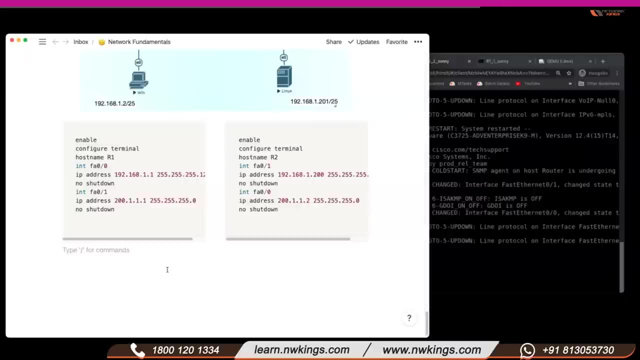 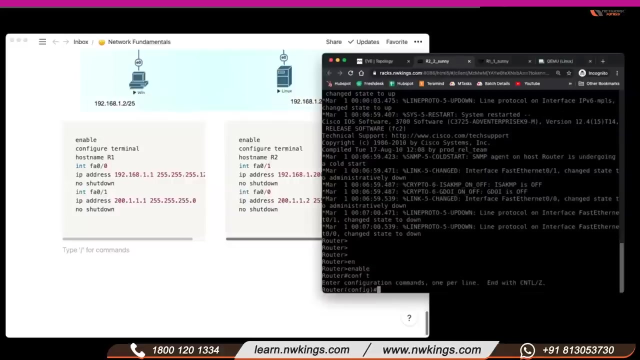 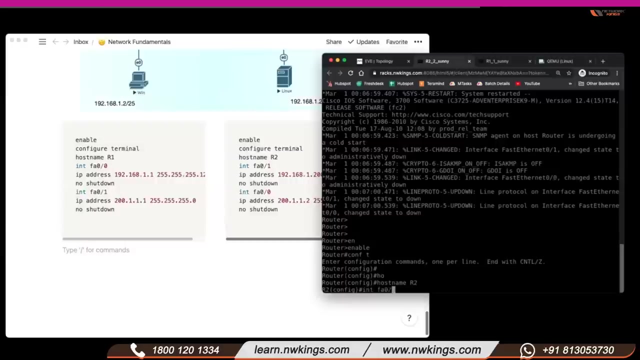 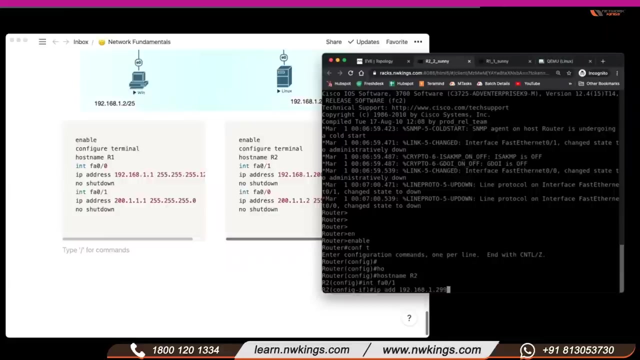 you need to keep revise the things. okay, rahul, you are my old student man, i remember you right, so how? okay, don't worry, okay, okay, so we have given ip address and let's go with config t, okay. host name: r2, interface fa 0: 1. ip address: 192, 168, 1.200. if you don't understand, just copy it first time you. 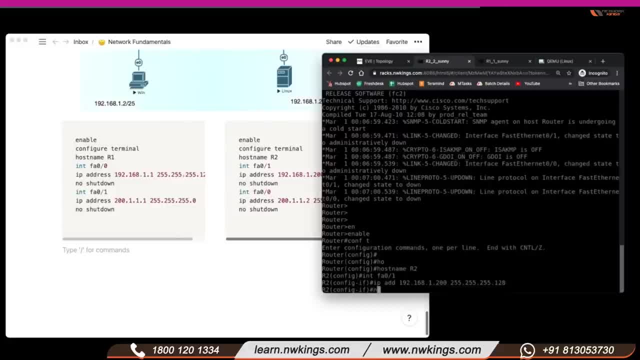 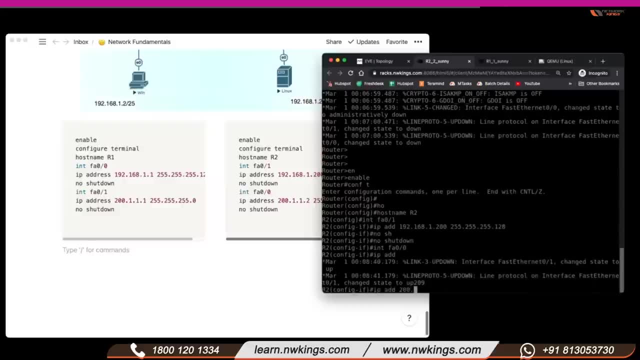 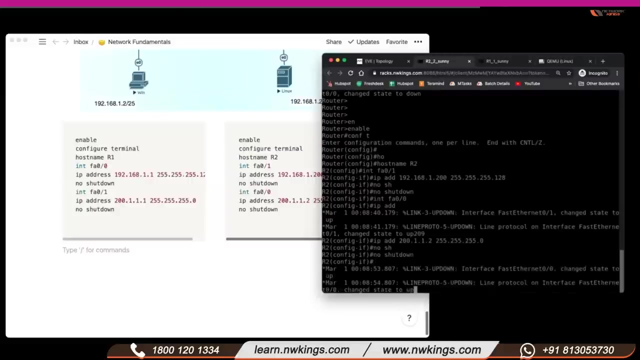 do practical by just checking the nodes and after that try to implement from your own, okay, okay, you know what is the best thing about learning? networking like you are doing something and if you do something it actually motivates you, that it actually rewards you that you are doing something. and when the practical gets successful, 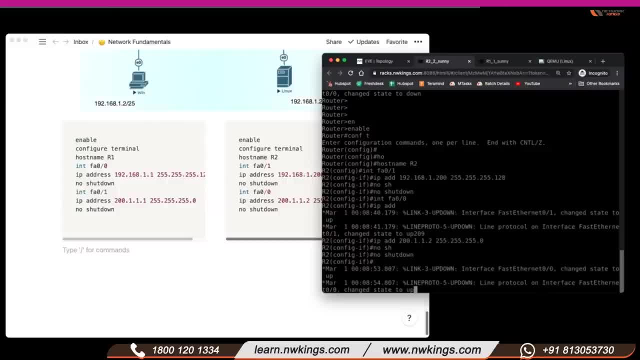 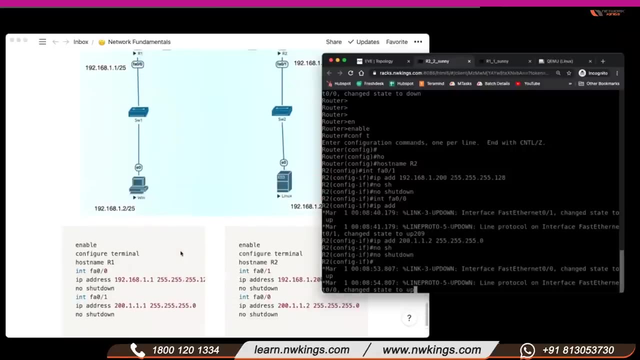 so it motivates you to do more and more. so whenever anybody thinks that we will only check the books, we will only check the videos, or you will learn that by videos it's it is not going to work for you in this it when you do it, then actually you get motivate to learn more. 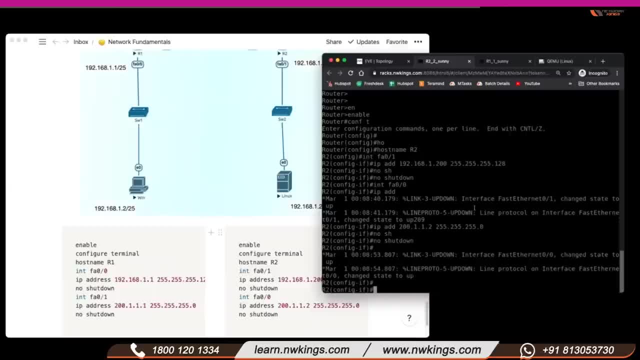 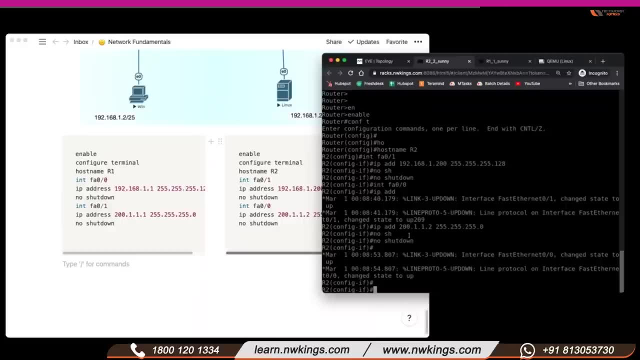 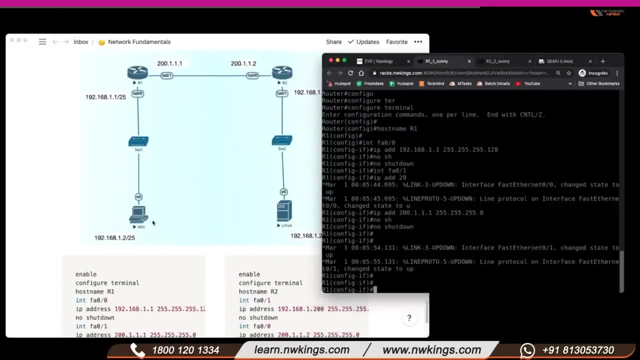 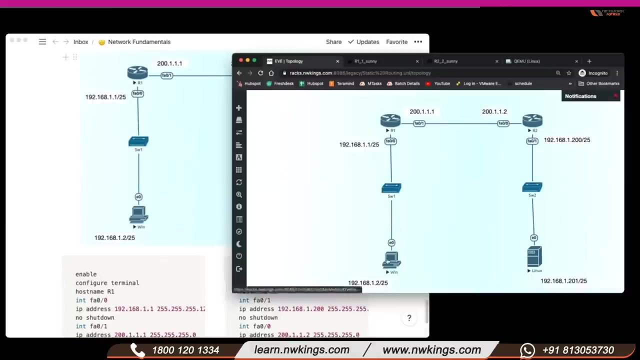 okay. so, rather than just learning, learn with by doing it. okay, so we have given ip address- r1 and r2- right? so tell me, let me give ip address to my machines now and let's check if they will ping each other or not. so what do you think without doing anything? 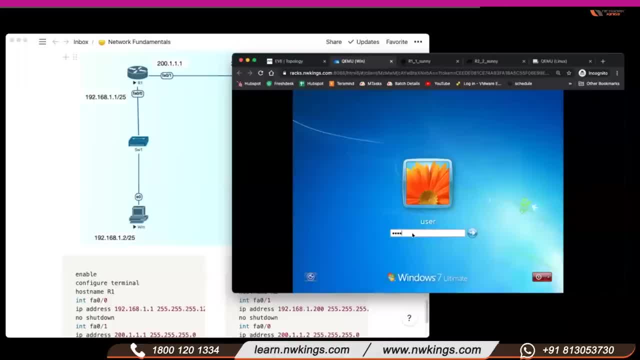 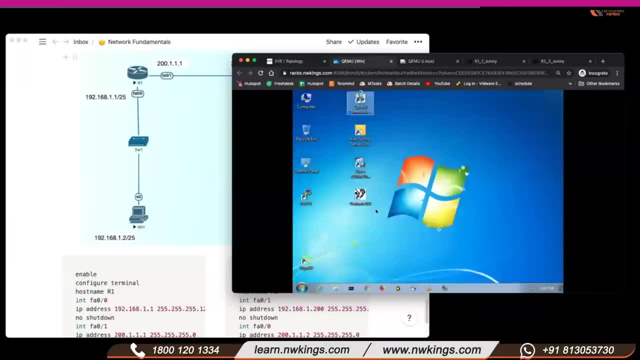 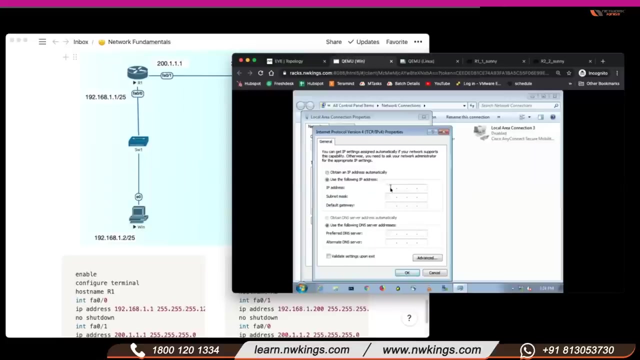 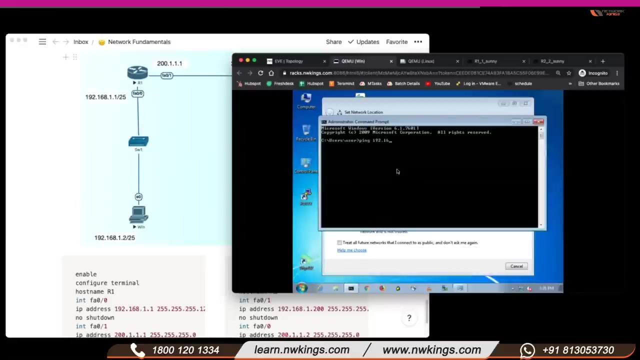 are they going to ping each other or we need to do something routing or something? 192.168.1.2. so we want this computer to connect with the gateway. so let's test if my gateway is pinging 192.168.1.1 so you can see i'm getting a reply from my gateway. 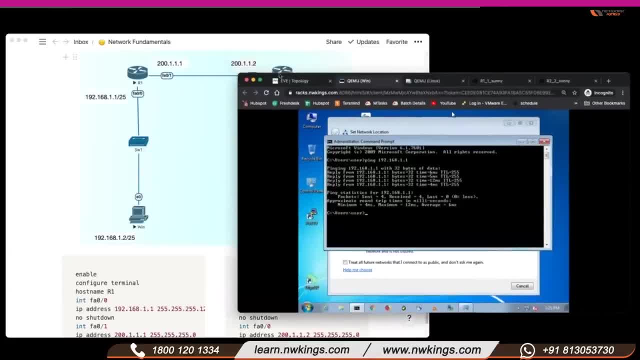 and let's try to ping the another router, which is like 200.1.1.2. we are unable to ping that router. ip, it means your ping. so it means your ping is going from here to here, but this router is not responding. why? why my computer or my? 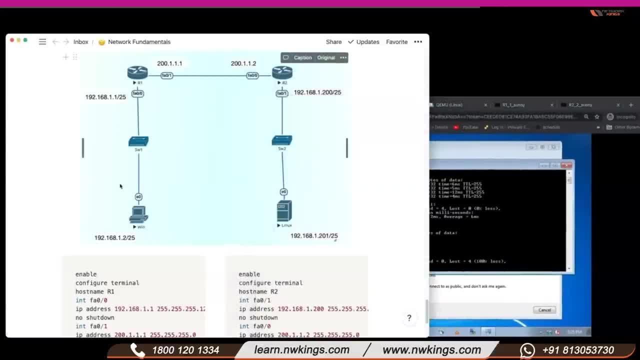 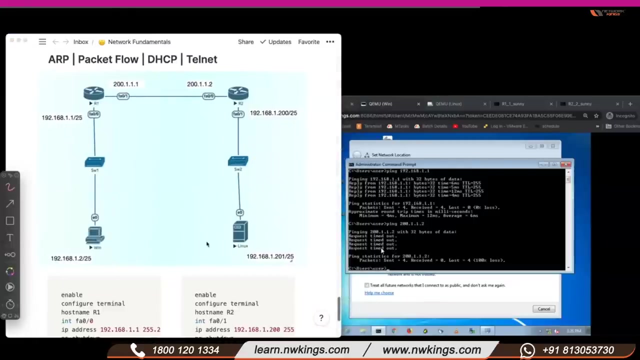 router is not responding. okay, so if i'm pinging to this ip address, this router is not replying me, you can see ping is getting dropped so you can see requested timeout. requested timeout comes when your destination is not replying. you back most of the times. this is the issue. 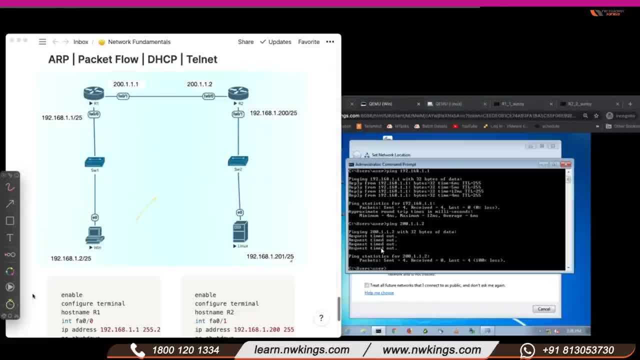 okay why we are getting this? because we don't have route to the destination. what does it mean when you send any information to this router and which ip i am going to? my source is 192.168.1.2 and router 2 does not have this ip information. 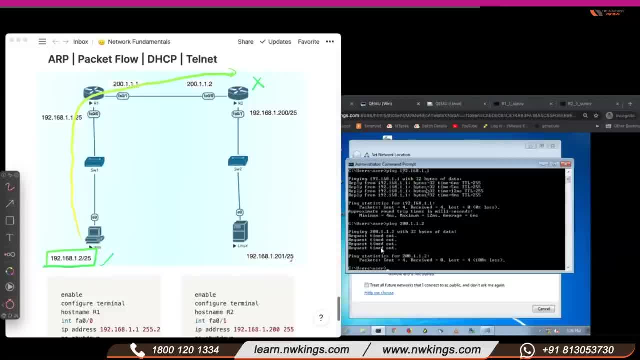 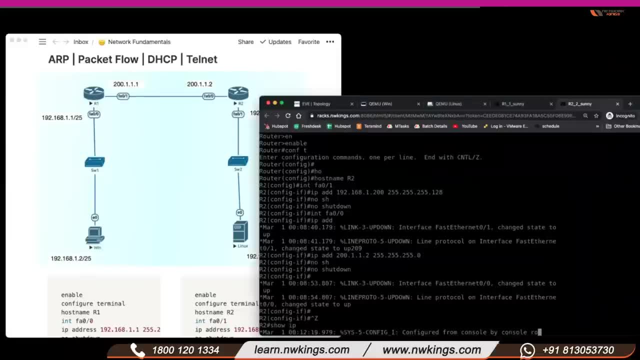 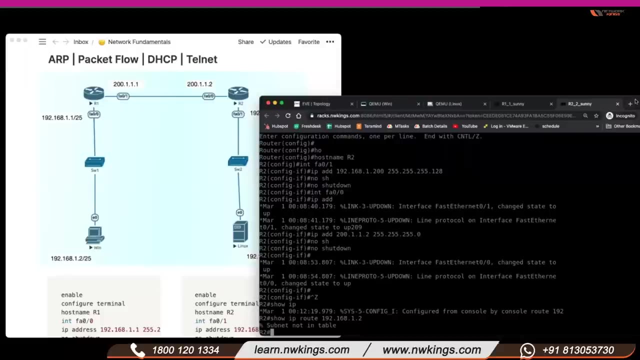 this router does not have any information. so let's check our router. so let's go to router 2 and check one command: show ip route 192.168.1.2. so what exactly router is showing me? this show ip subnet, not in table, it means 1.2. 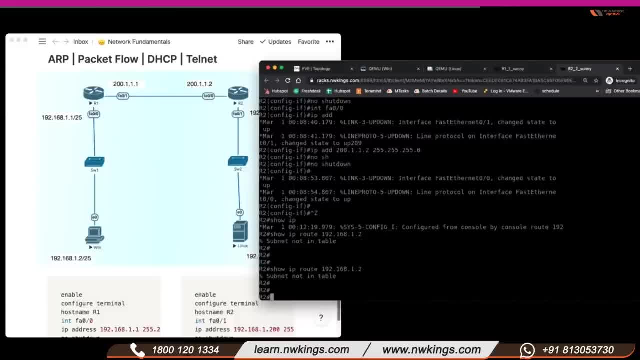 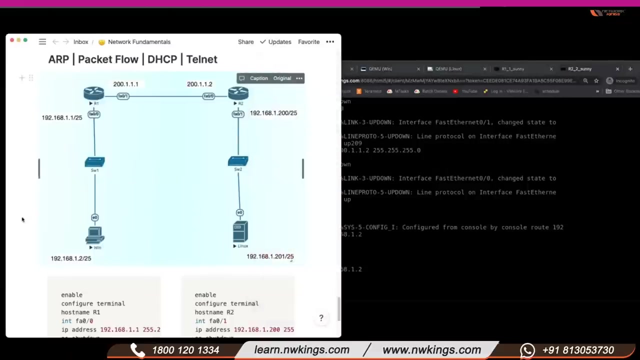 is not having any route to reach 192.168.1.2. i don't have any route, okay, so this is the problem. so here what we have to do, because remember this term- that router only have its directly connected information. it means router will only have its links information. 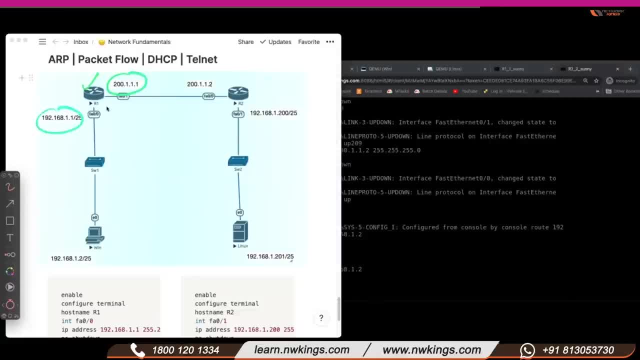 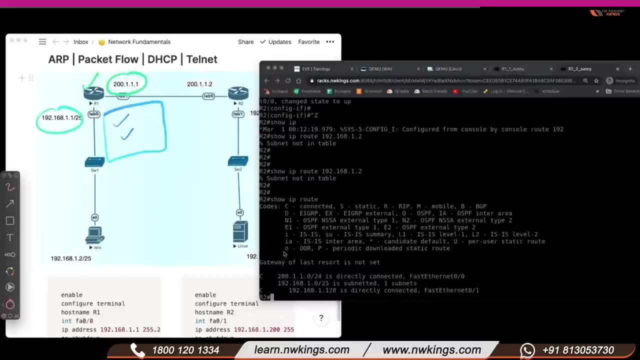 router 1 is connected with this link and this link. so router 1 will have only these two networks in the routing table. let's test. so let me go to r1 and let's check with the command show ip route. so can you see i have only two networks: 192.168.1.0. 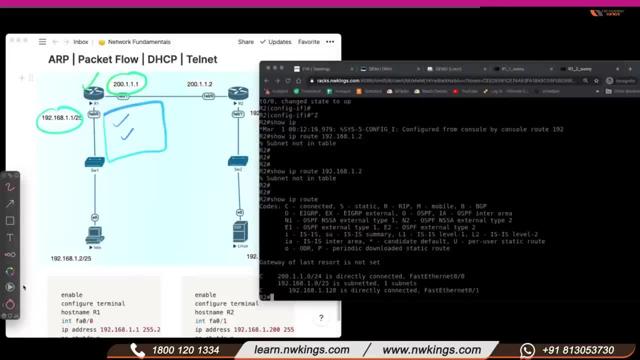 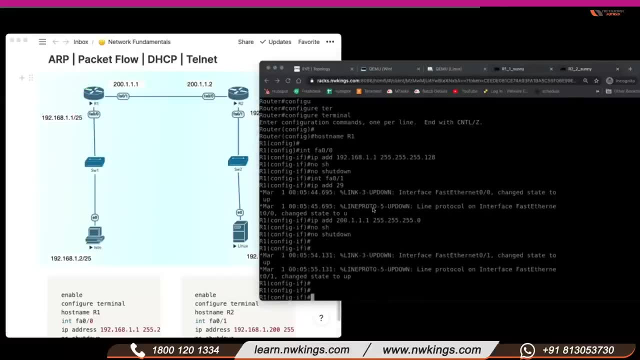 25. sorry, this is r2. OK Now if r2회 connect 1.28. but I queued up to r2 but I cannot connect r2 at the moment, so r2 and I cannot connect my data there and start R1 at this time. 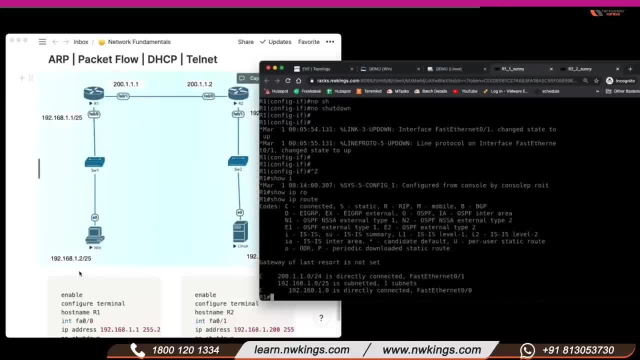 so I requested through router two links. so now let's first connect home it and connect r2, and the r1 and r2 can go one mão here. so let me check here. show ip route has. you can see r2 has 192.168.1.128. this is the subneted network. but this router only has 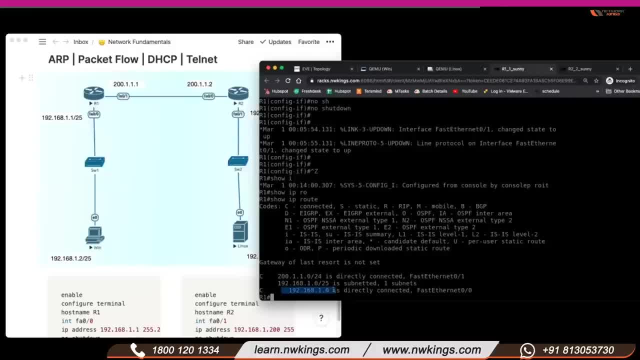 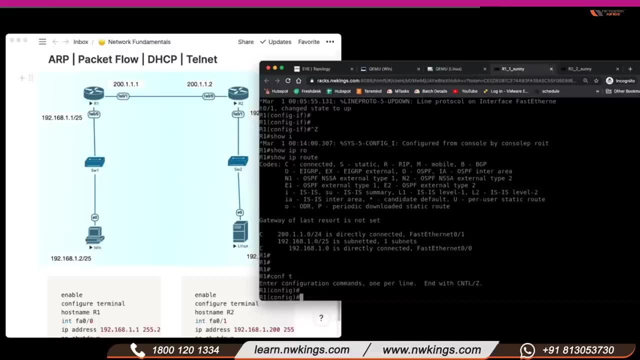 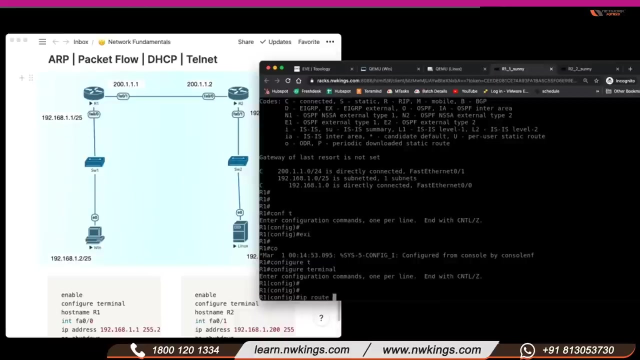 192.168.1.0. it means we need to create a route, we need to set up a manual route. that is known as static route. so s stands for static. it means i am going to add that route manually. so how to add? so go to configure terminal and i am going to type ip- route. and what is the ip? 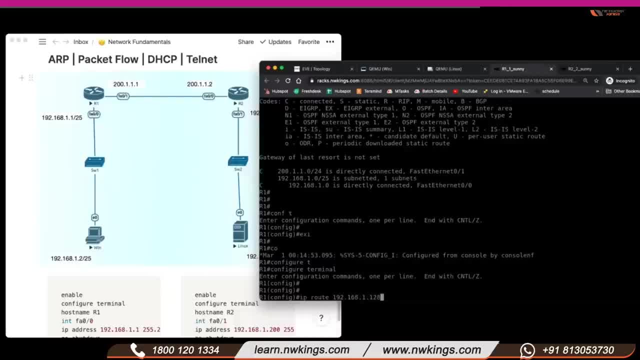 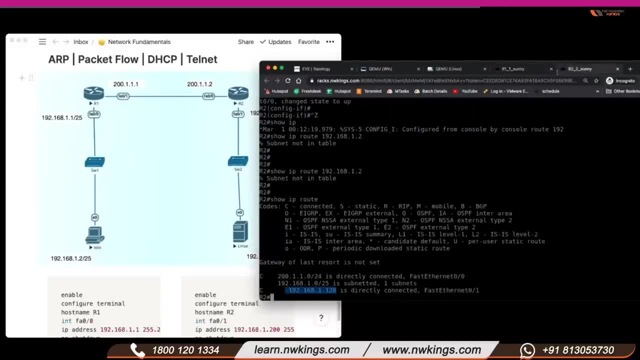 address 192.168.1.28. why i am giving 192.168.1.128? because that is my network id. and if you don't know what is the network id, just check the another router and you will find that network network id here. so this is my network id, the first ip. 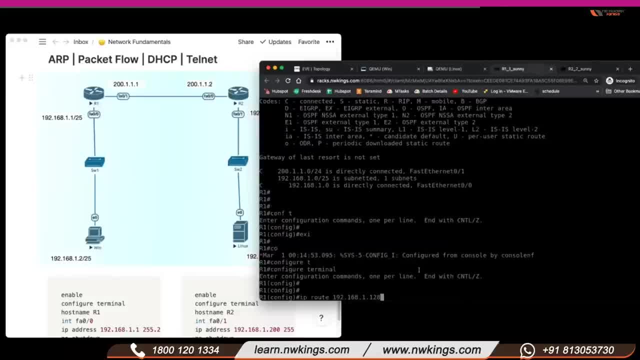 address of any subnet is known as network id. always remember, when we give static route, we always give network ids in most of the scenarios. this is not a language, this is the just simple commands. this is not a language. so, ip route: 192.168.1.128. i am going to type here: 255.168.1.128. 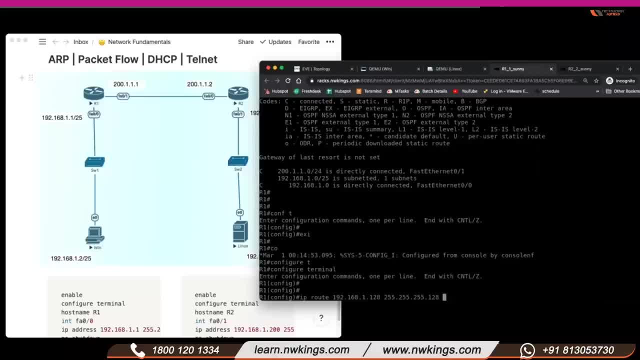 now router 1 is going to this network with the help of router 2. right route if router 1 wants to communicate with this network. router is going from 200.1.2 means router 1 wants to go to 192.168.1.128. 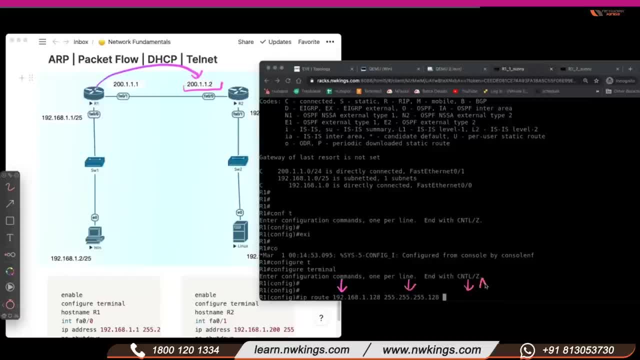 and this is the subnet mask. here i have to add what next hop. so first we always type network id, here i always type subnet mask and here always i give next hop. next hop means the neighbor router. okay, the neighbor router is my next hop ip address. so my neighbor router ip is i am getting the next hop ip address and i am going to type. 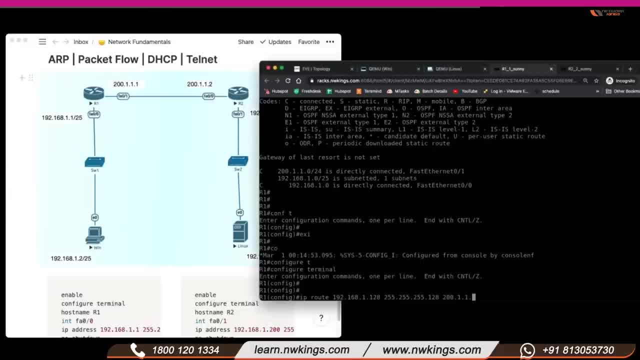 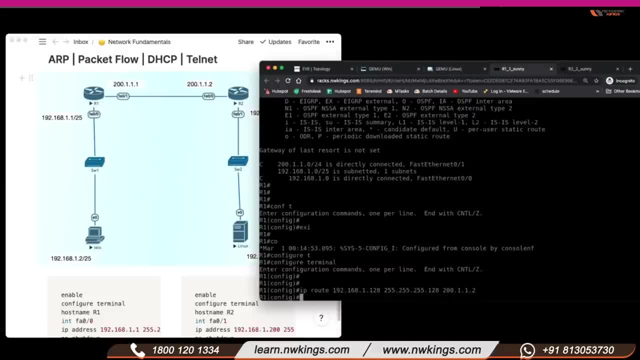 this route from where i am getting this ip, or route from router 2, so that is 192.168.1.128, 255.255.255.128, 200.1.1.2, so in router 2 also. so when we have static route, now my computer is. 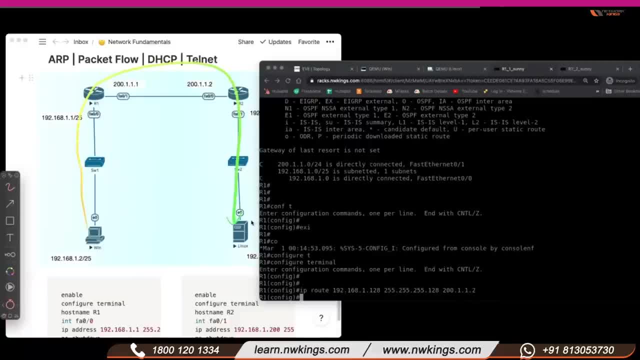 going to send information to this machine and when this machine is replying back now, router 2 needs to send information to this machine and when this machine is replying back now, router 2 is this ip address. so now router 2 does not have any entry, so router 2 also should all router 2. should also know this network. that is 192.168.1.0. so on router 2, i am going to type ip address of router 1. so what is the ip here? 192.168.1.0. so on router 2, i need to create a static route. 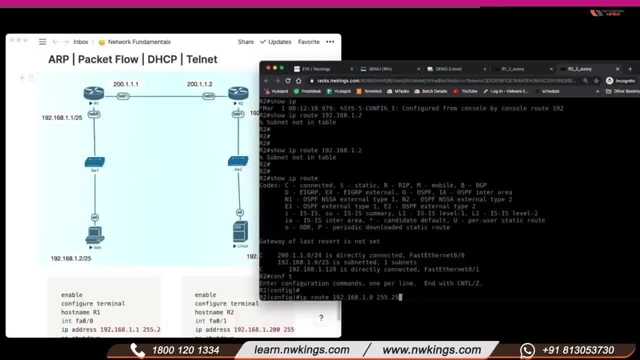 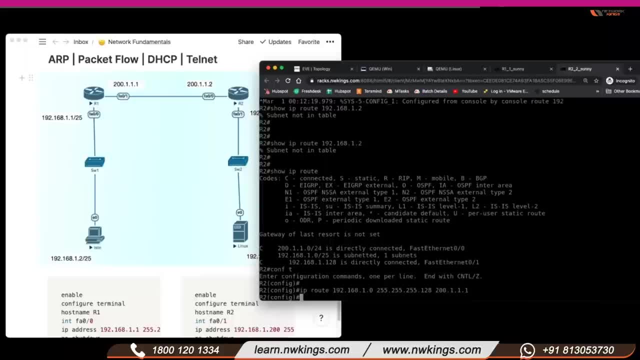 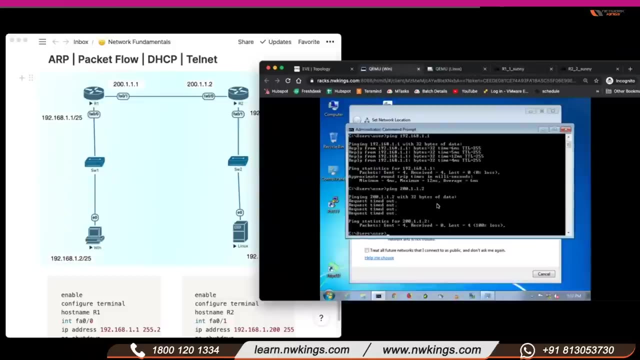 192.168.1.0, 255.255.255.128 and my ip address neighbor ip address is 1, so these are the two static routes you need to create on r1 and r2 and let's test if we are getting the ping. 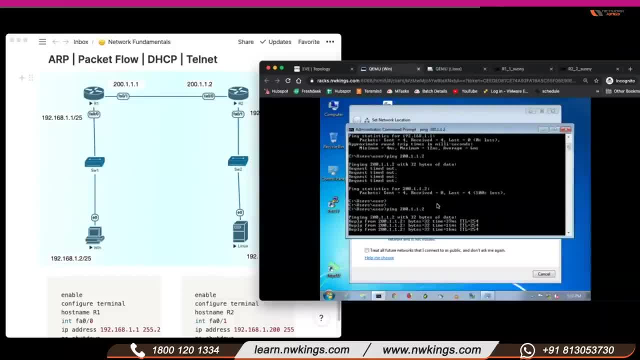 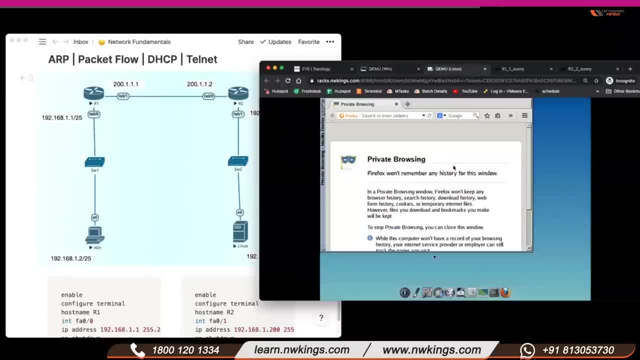 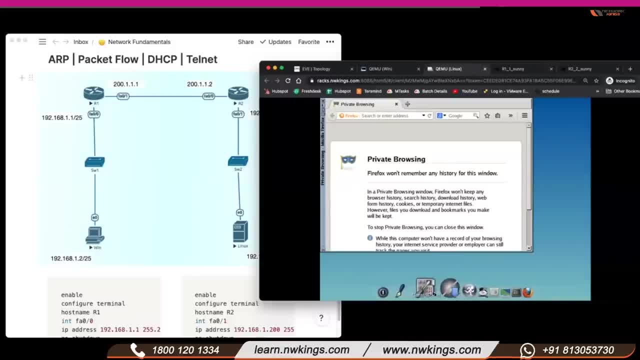 control panel or maybe network. yeah, from here we can give ip. so ip addresses 192.168.1.201, something okay, and my gateway is 200, i think, and apply, i think, 201, yes, so let's test if my machine is pinging 192.168.2.0.1. 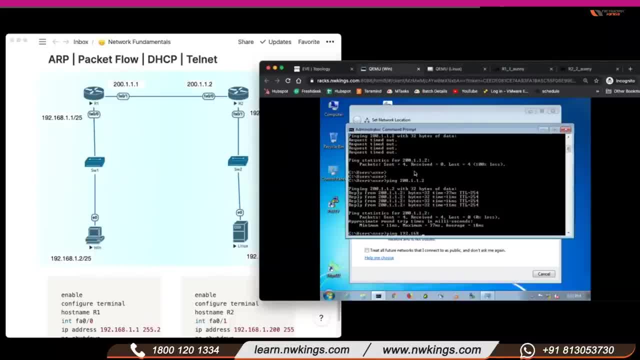 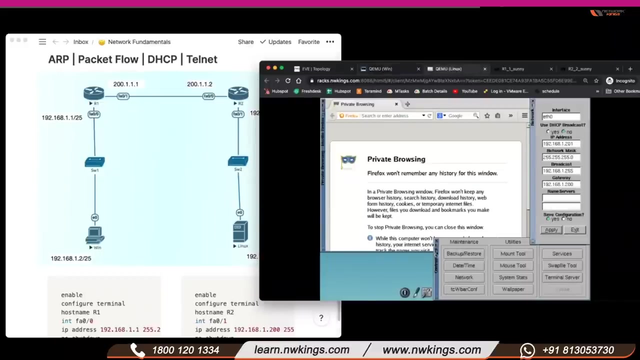 so 192.168.2.1.2.0.1. yeah, so we got the ping guys. can you see that my linux machine is connected? can you see now so you can give the command on linux with the terminal also? but that is a little bit complex with if config command. okay, 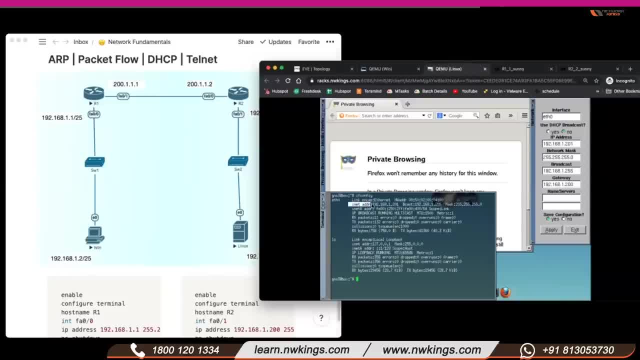 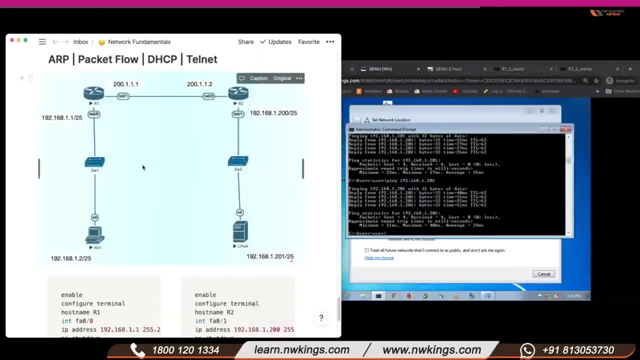 so here you can see i have given here inet address: 192.168.1.2.0.1. okay, so now my windows machine is pinging my linux machine and you can see both the networks are in different locations. so i have given the command on linux with the terminal also. 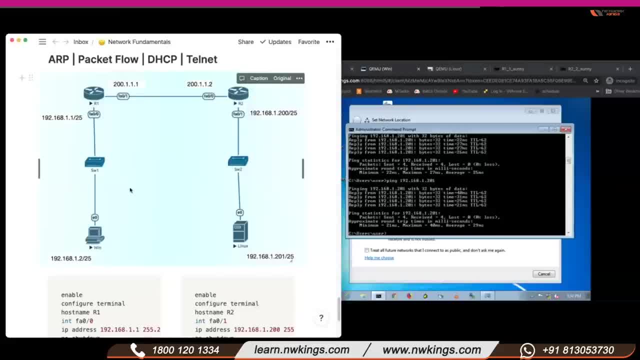 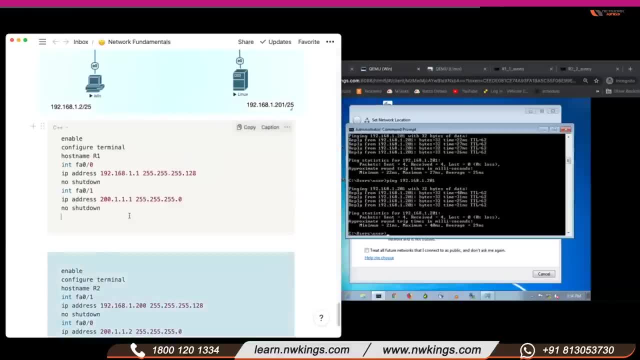 okay. so now my windows machine is pinging my linux machine, maybe, or you can see that both different networks are connected, so i'll type here static routes. maybe you are getting confused how to give. let me repeat it on r1: r1 has only 192.168.1.0 network and 200. 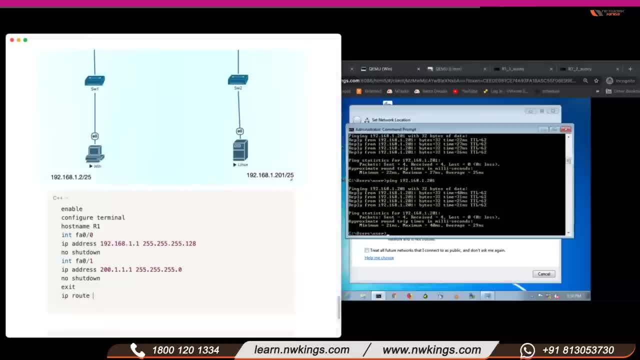 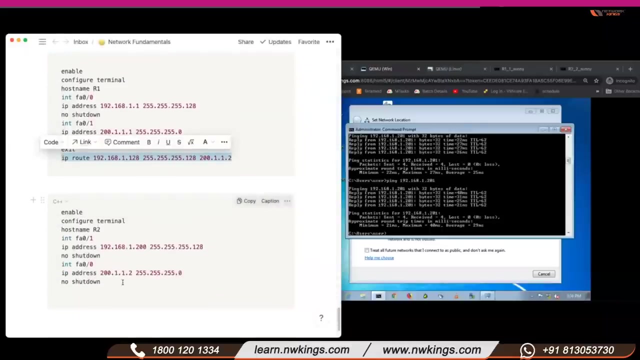 so it means router does not have 192. yeah, so router does not have 192.168.1.120 subnet mask. and the next hop, ip, means router to ip address. so this is the route. on r1 i have to give okay and on r2 i need to create the reverse static route. 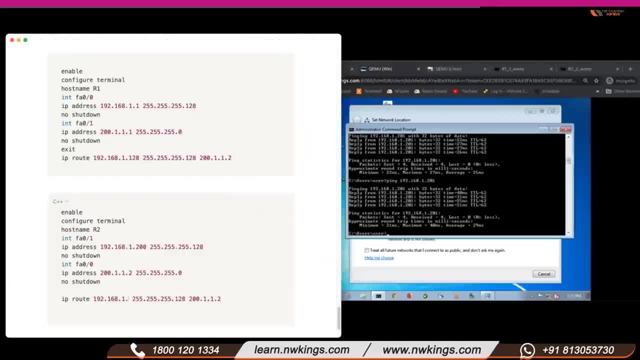 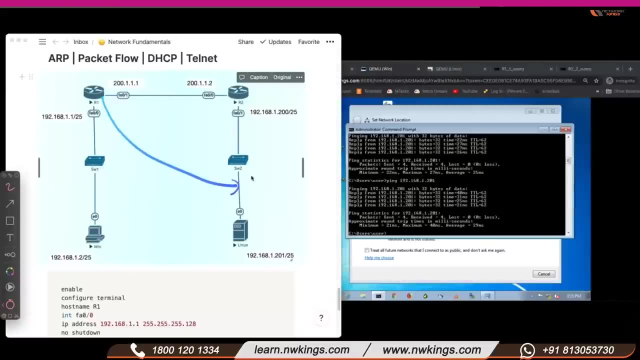 so reverse static route means instead of 128, because 128 is his own directly network. here i have to give 200.1.1. so router 1 will create a static route for this network and router 2 will create a static route for this network. this is i have done. 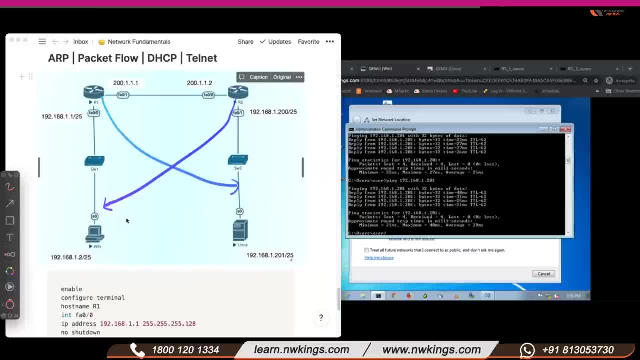 okay, just understand my why i have added static route. because when traffic is going from this computer, router 2 is not forwarding the packet to 192.168.1.2.0. because we don't have to forward the packet to 192.168.1.2.0. 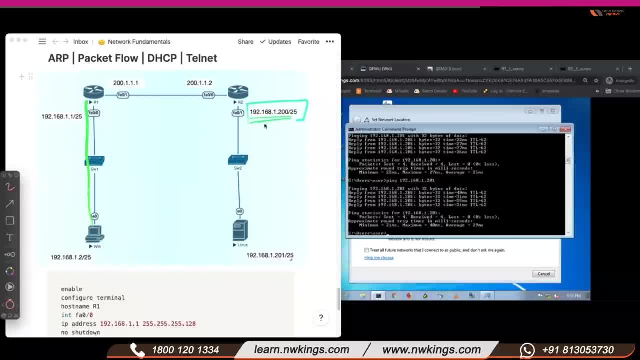 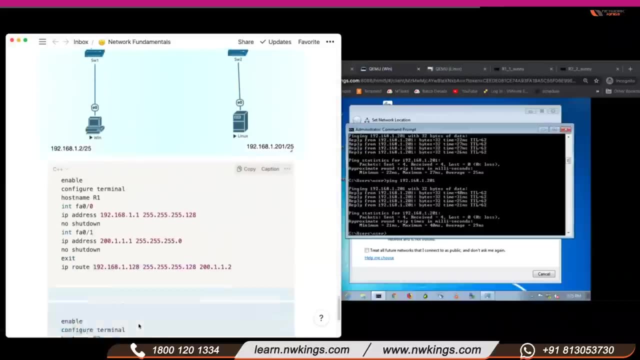 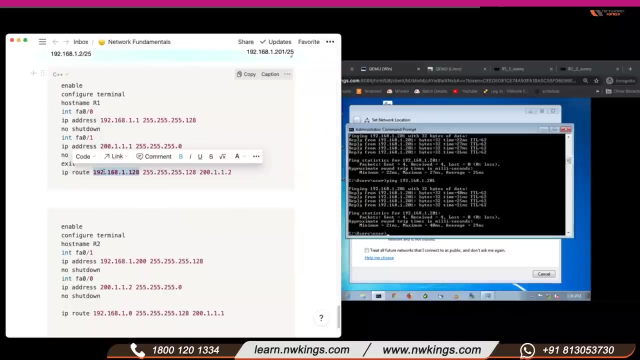 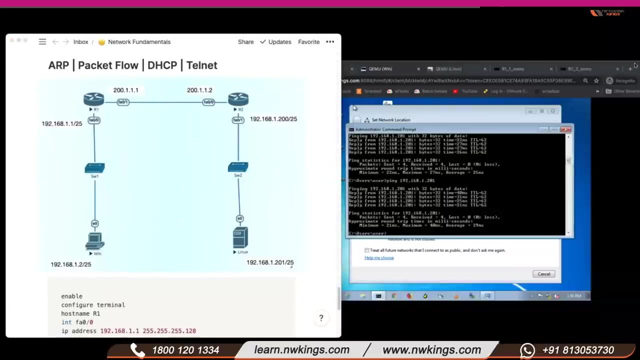 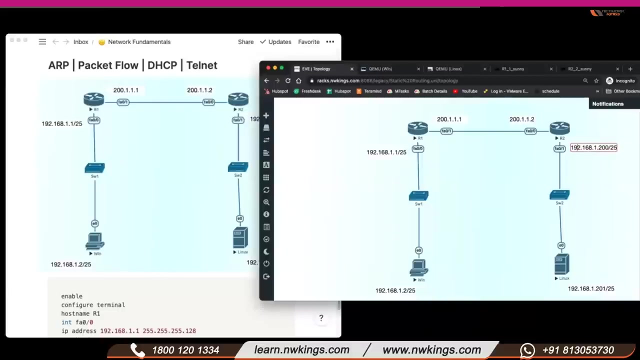 or have information of this thirst the advantages ofッ dead intelligent network. so this is the reason we have added respected 192.162.. address: if you are getting confused, okay, so you can change the ip over here also. like if i can give here 2.1, okay, so you can change ip 2.1 here. okay, so you can do like that also. but i'll keep. 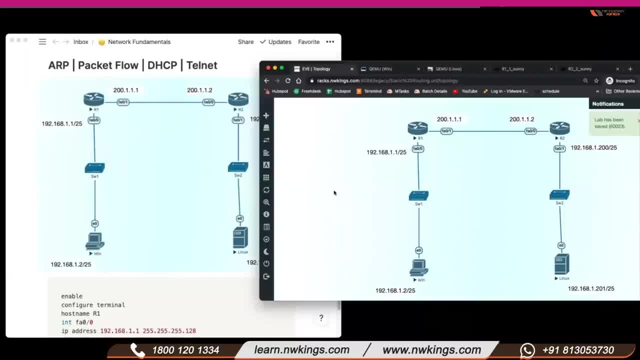 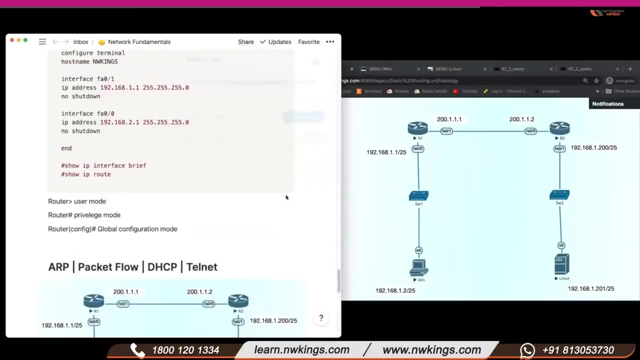 this so you can do it on yourself. okay, so this lab is already in your system. i'm not saving or anything here, so you have to complete this lab and i have already shared the notes with you. okay, and before i stop these devices, let me show you how. 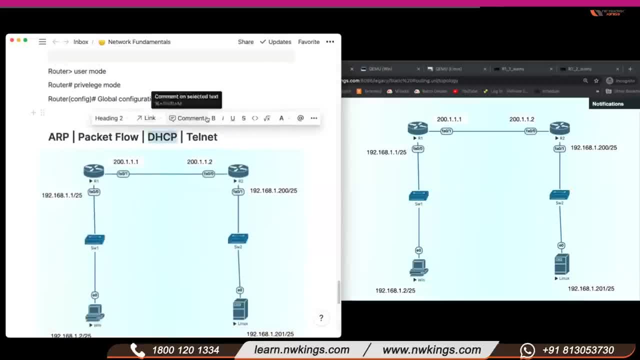 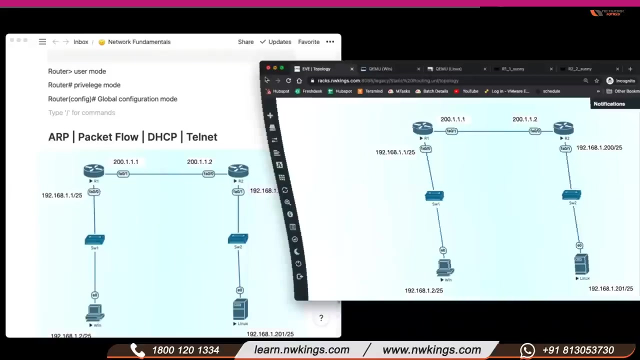 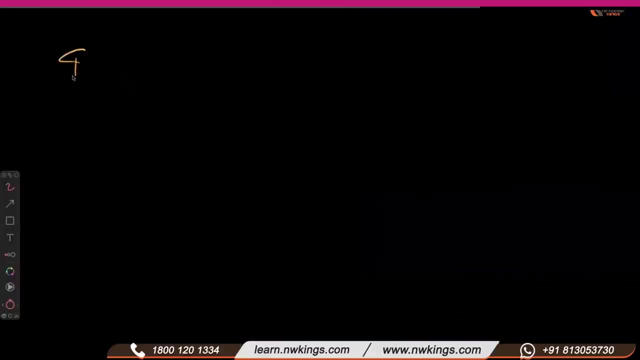 to configure dhcp. so what is dhcp when my computer gets ip addresses automatically? and let's understand what is dhcp, okay. okay, i'm audible. okay, so let's go ahead. okay, so let's understand what is dhcp. okay, so dhcp stands for dynamic host configuration protocol. so when you want that, your router should give ip address to your 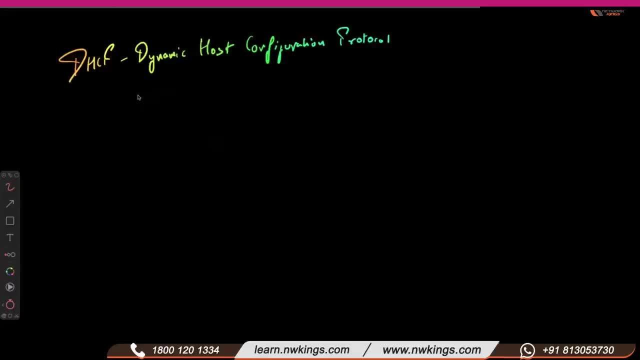 computers automatically. so dhcp is a protocol which assigns, assigns ip addresses automatically. okay, so in dhcp what happens? so suppose this is my computer and this is a dhcp client, okay, and your server could be your windows server, or maybe you can have a router as a your dhcp. 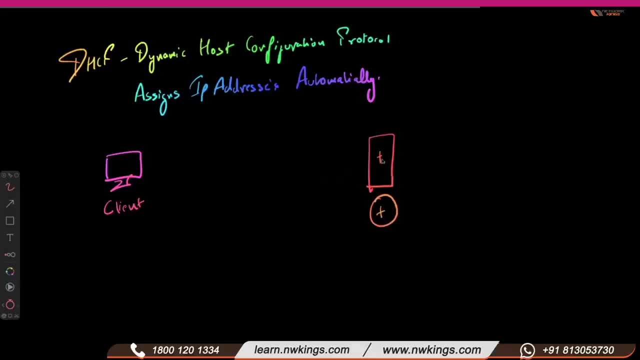 server. so it depends on company to company. some configure on servers and some configure dhcp pool on router also. okay, so if you have a very big company, you can configure dhcp pool in a server and when you are a small- medium scale enterprise, you can configure on a router also. 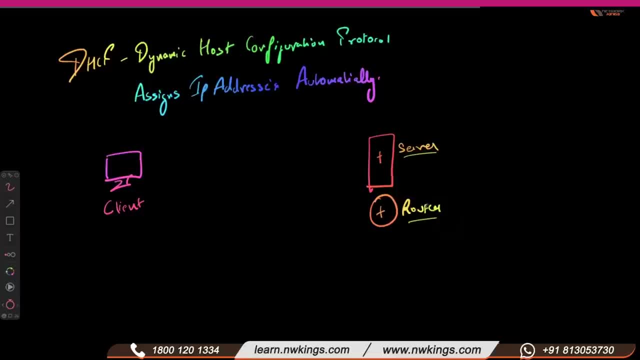 and in our home connections we use router as a dhcp server. so these are my servers. okay, so they will work as a dhcp server, both the devices and this will be my dhcp client. so there is a concept known as dora. what is dora? so first i'm 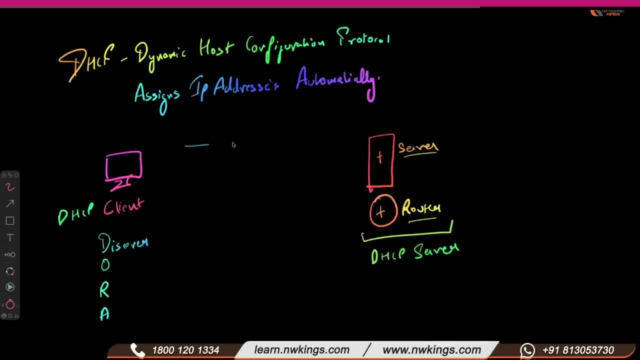 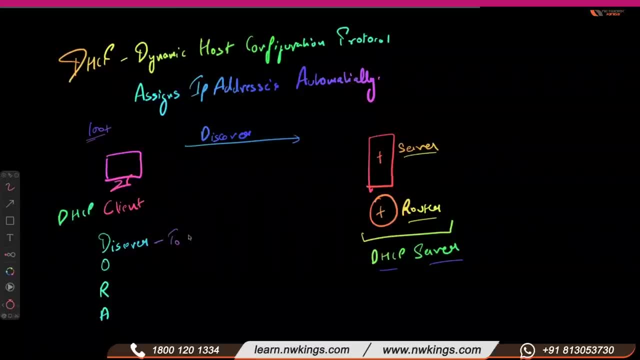 packet to search, to find dhcp, to find dhcp server. okay, and now server will, or router will, check its dhcp pool table. there is a table known as a dhcp pool table where all the ip address are written and it will be like that all ips are free or assigned, so whatever ips are free. 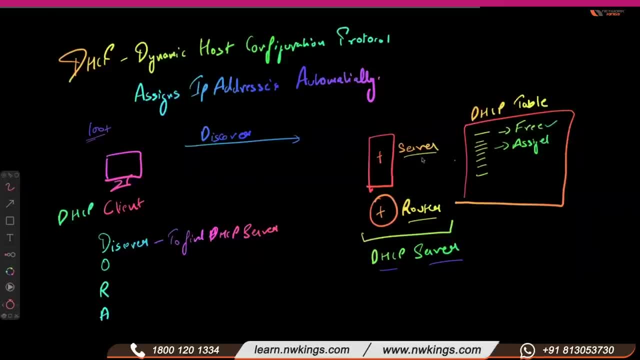 means they are not used anywhere. it is going to send one free ip, which is not allocated to client, with the offer message: offer message of any ip, maybe this computer has one. 53 0000000 to 168, 1.2 now offer messages to allocate instead of allocate. you can see that, so server is going. 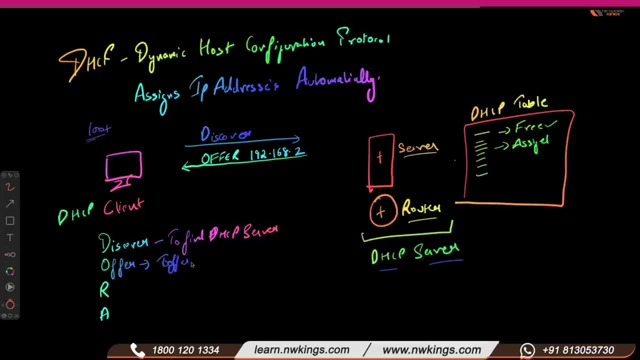 to offer. offer ip address from the pool. what does pool means? pool means like a group. okay, maybe it has a pool of around 250 ips, so one ip address is going to allocate to this client. so now, if everything is okay, then client is send a request packet. okay, give me this ip. 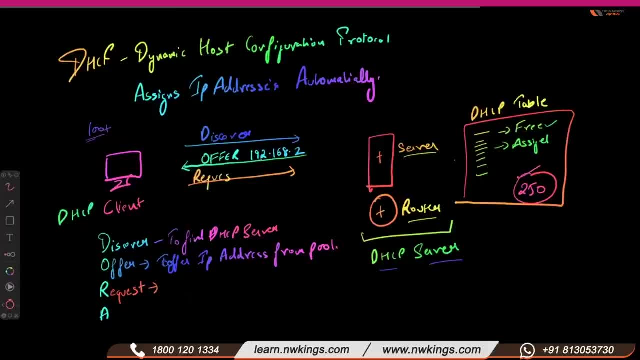 so here i am just showing, i am just offering: are you okay with this ip 1.2? and request means yes, i am okay with this ip. please give me this ip so in which packet we get all ip configuration. in the last packet, acknowledgement: send me ip configuration. so request packet is to get the ip configuration. 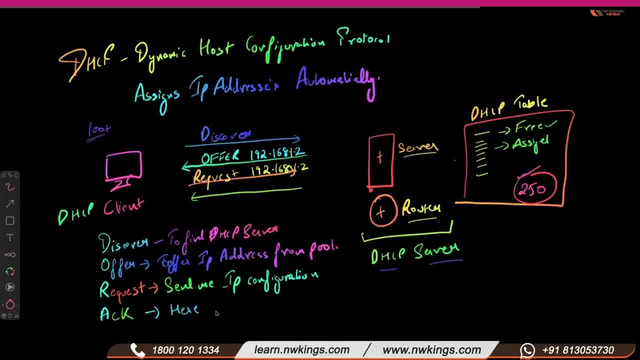 and in acknowledgement you get the. here is the configuration, here is the configuration. so in acknowledgement packet the server will send the ip configuration details. yes, offer is unicast. discover is broadcast packet. offer is unicast packet. okay, so again i will repeat: so client is going to send a discover packet. 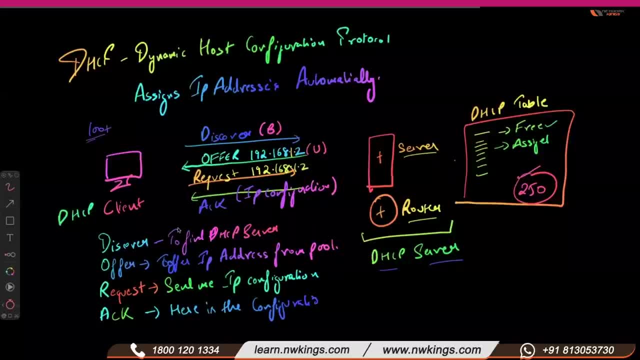 packet to find. suppose i am a server, okay, and you all guys are clients. so first you are going to send a discover packet to me and i'm going to give ip addresses from this pool. so this is dhcp table. so i'm going to send you all one ip address. so all you have different, different ip address. 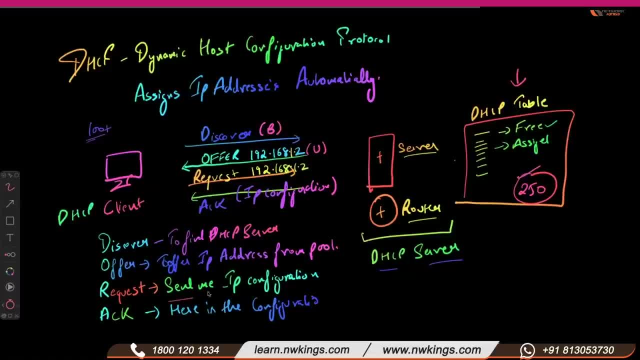 and if you like, the ip address and all. so you will request me send me the ip configuration and with the acknowledgement packet i am going to send all the details in. in acknowledgement packet: see acknowledgement. request will be unicast and rest. you can check with the like some packet capturing tool like wireshark and all. 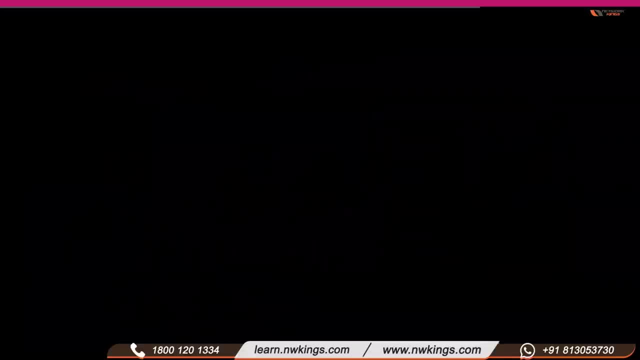 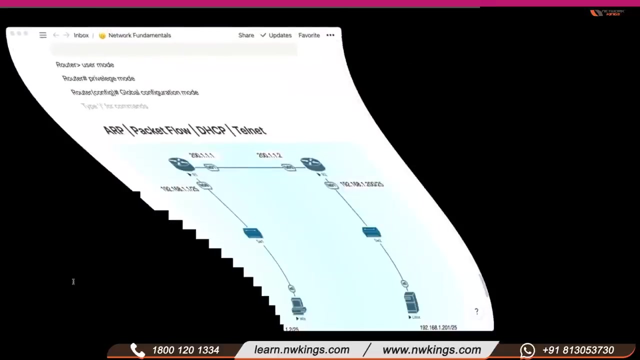 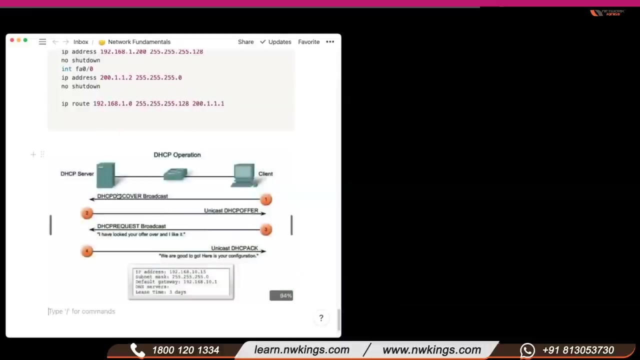 so i'll add one screenshot in your notes so that you will understand dhcp. yeah, so you can see here. so this, so this, so dhcp discover is a broadcast packet according to this image and then we get offer as a unicast again, computer does not have any ip address right in this packet. also, we don't have any ip. 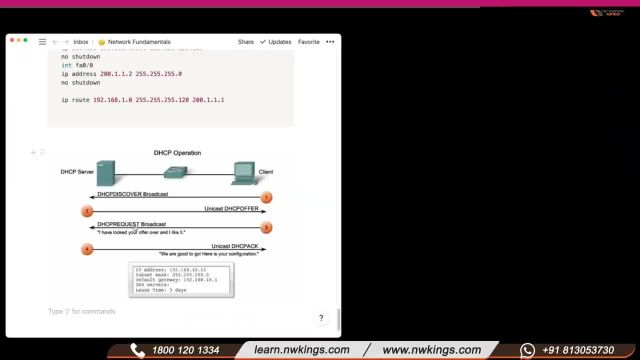 so, still, we are going to send the request to the as a broadcast to the server because it will have dhcp server ip and it is going to send unicast. okay, so you discover, messages from client is always broadcast and messages from server is unicast. okay, so you want me to configure dhcp server in our practical 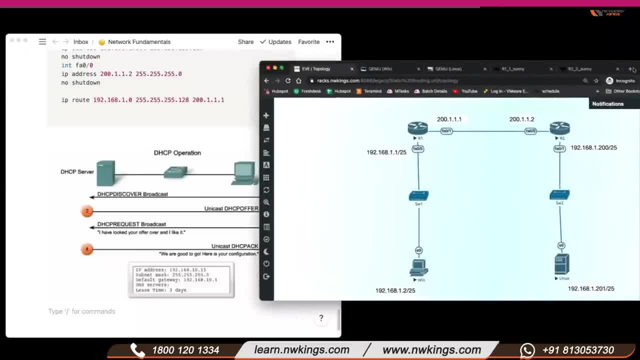 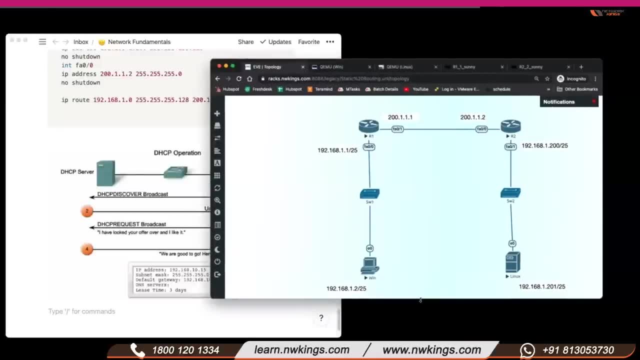 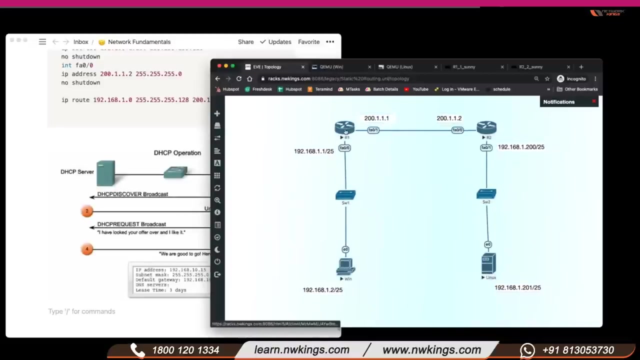 I will do it a little bit late, but it is ok. one of the things this method will give you is some definition that you can see here. that head is not going to. wants you no, then why you are here, man, somebody saying no, you can take leave. 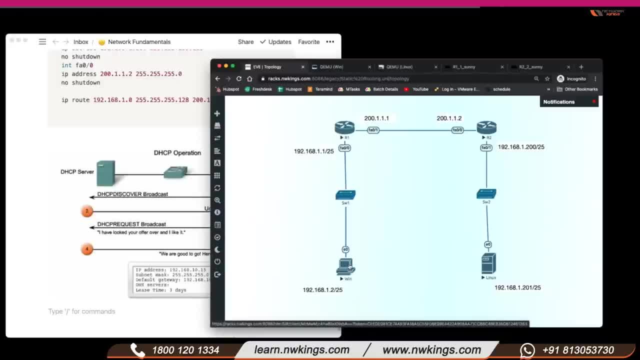 yeah, yeah, I'm going to configure a dhcp server. okay, so I'm going to configure a dhcp server in this R1 so that my window machine will get access to it. machine will get IP address automatically. Adil, I will explain ending process. trust me, I am going to explain. 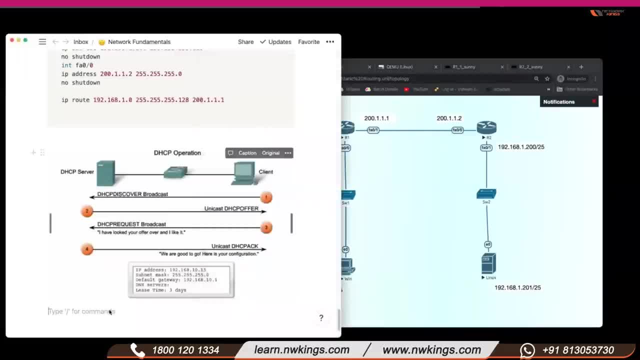 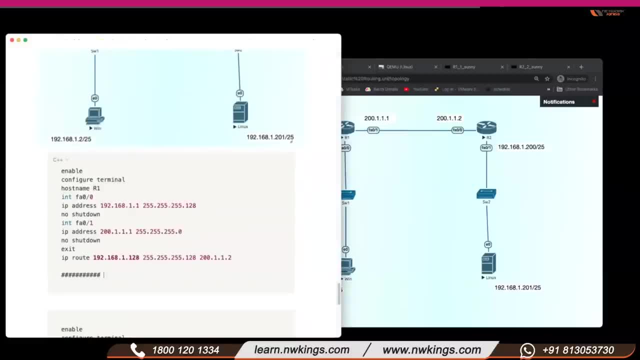 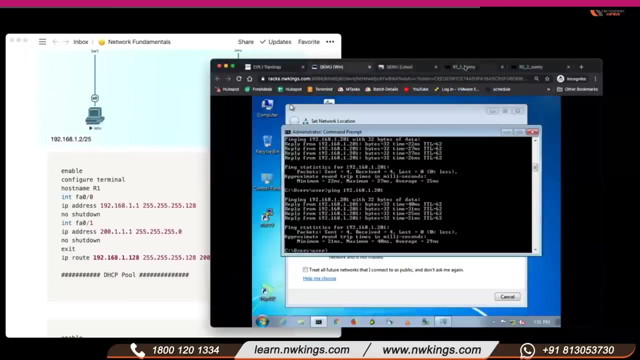 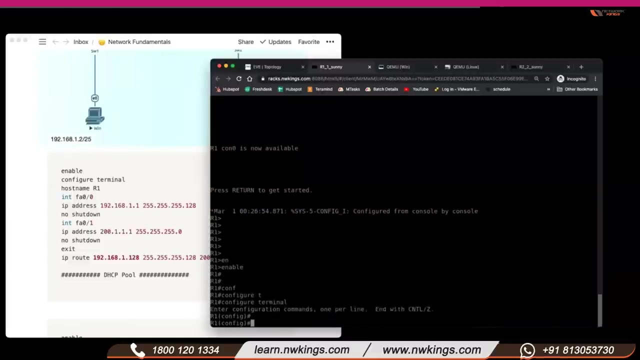 So let me configure DHCP on it. So on R1, I am going to configure a DHCP pool. This is not the last session. we will have last session tomorrow. So DHCP pool. how to configure? It's very simple: go to R1, and in the enable, configure terminal, and I'm going to type: 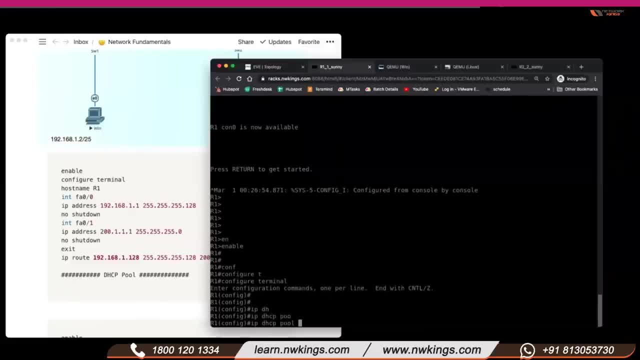 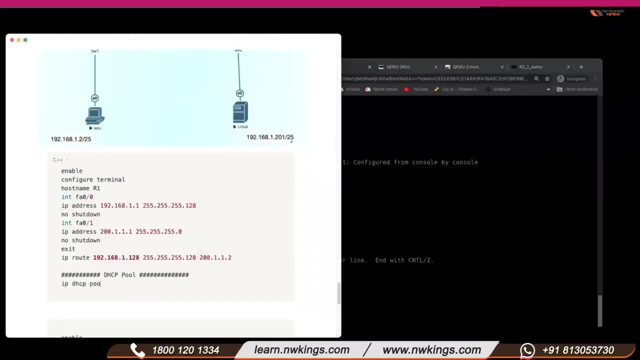 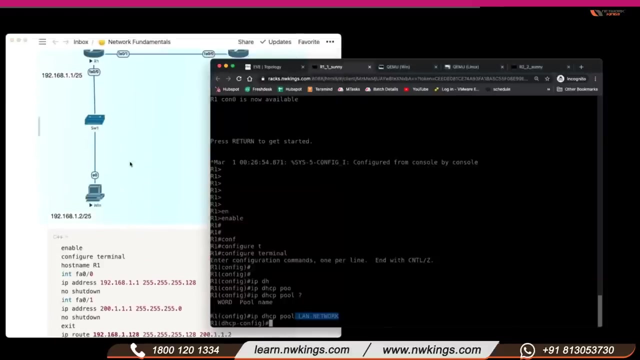 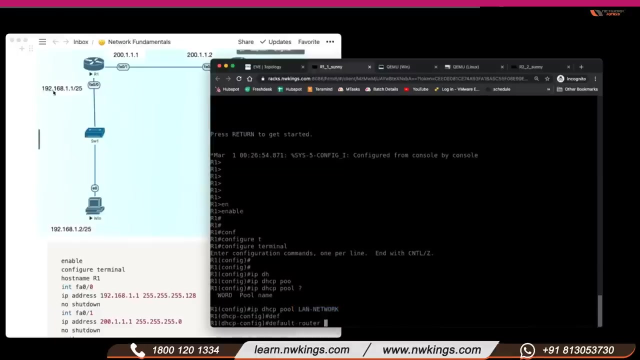 here IP, DHCP, pool, And we can write any name here. So suppose lanphp network, So you can give your name also here. So we will create a pool, IP DHCP, pool, LAN network or anything, any name, And then we will type the IP address of a router: default router. who is the router? 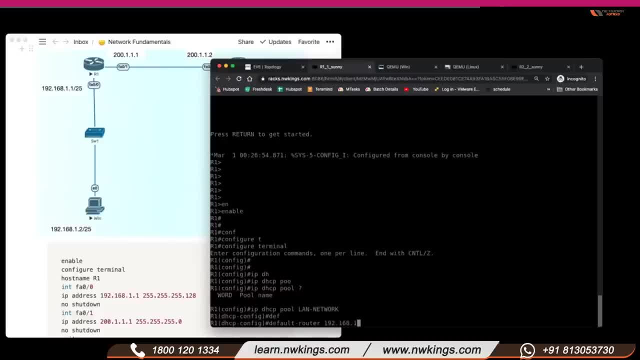 Router IP would be 192.168.1.1.. And for which network We need to give IP 192.168.1.0.255.255.255.128.. Here we are assigning the pool. the IP addresses from this pool will be assigned to your machines. 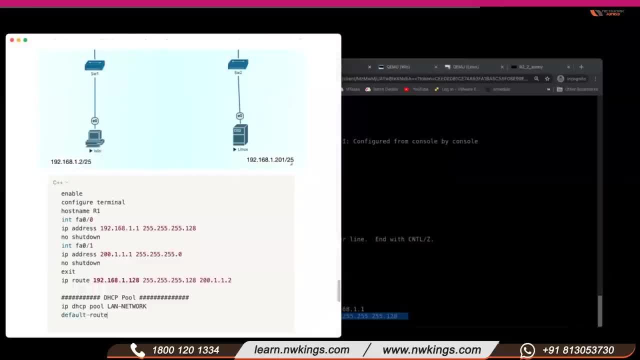 So here I'm making a pool. I am giving here default router 192.168.1.1.. This is my gateway for all my devices. And what is the pool? Pool is give IP addresses from this pool. It means the block of this IP, 1.0 to 1.127, where we have done submitting. 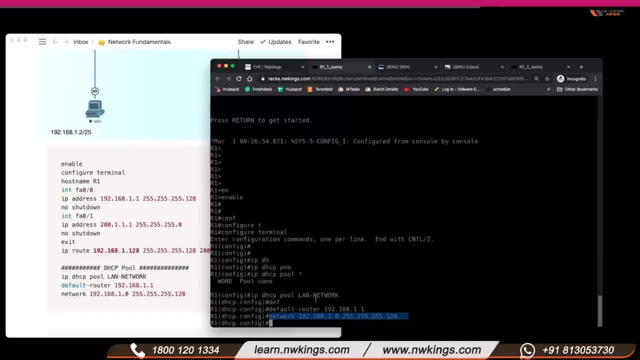 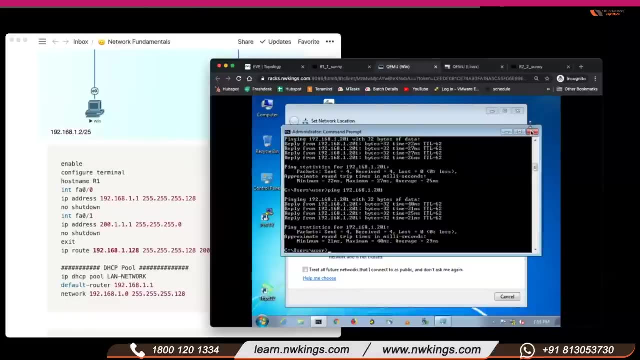 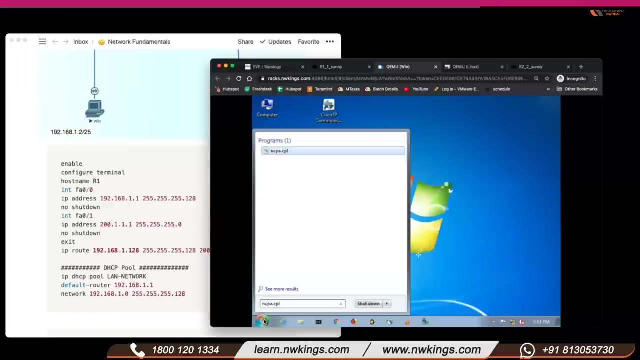 So we are going to assign IP addresses from here. Source Mac would be the computer Mac address, right? So let's see if my window machine will get the IP addresses automatically or not. So how do I do that? So how to choose a DHCP? because we have given static IP, we need to change the properties. 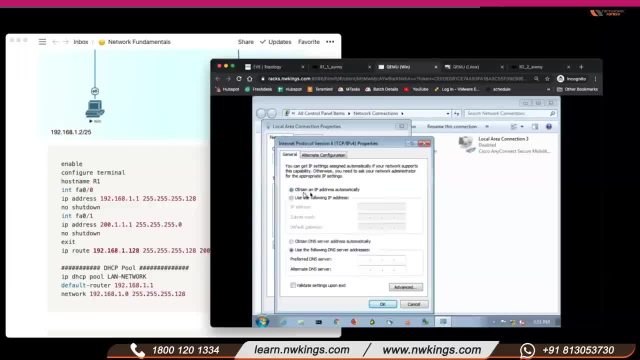 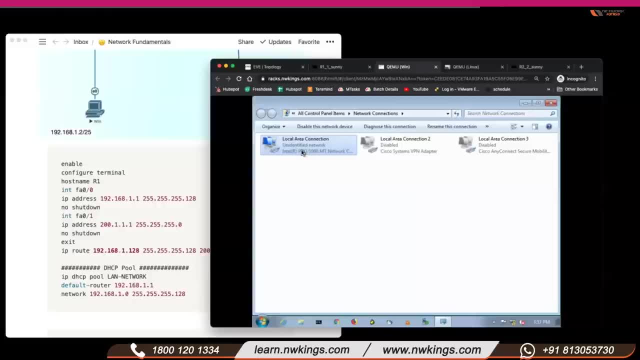 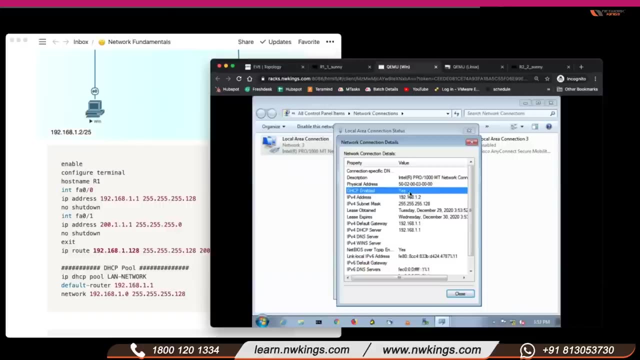 with the DHCP- And by default all your machines have this options enabled- obtain an IP address automatically. So let's check if the computer will get any DHCP IP status detail. yes, we got the IP guys, DHCP is enabled And we got the IP address 192.168.1.2.. 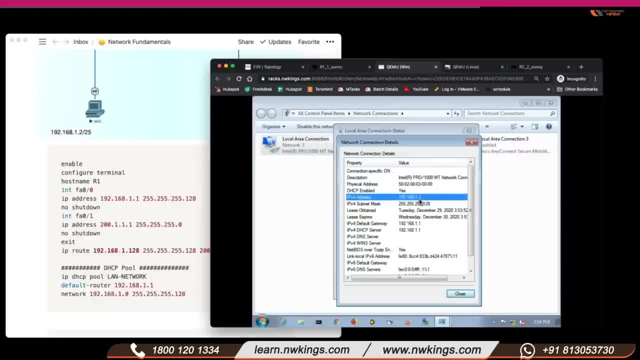 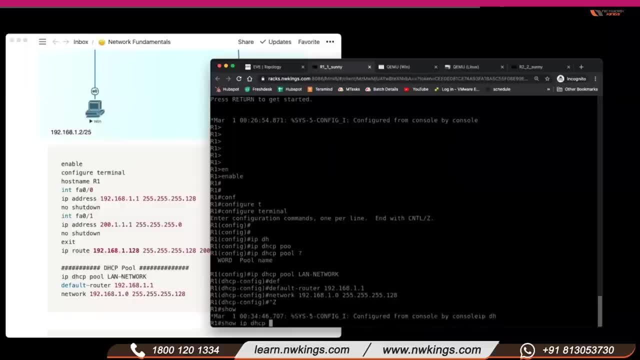 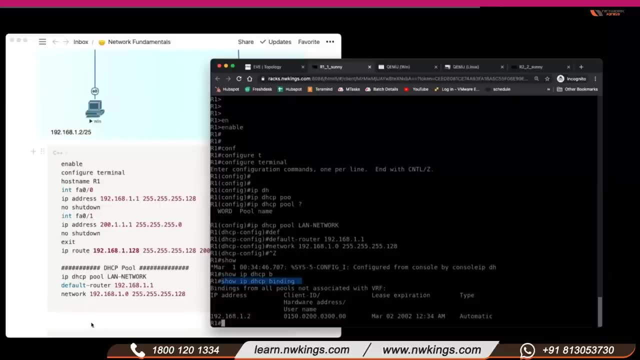 The same IP which we have given in static And in R1, let's check: show IP DHCP binding. So this is the pool. So this is the pool. How to check the pool: Show IP DHCP binding. So what is the command? 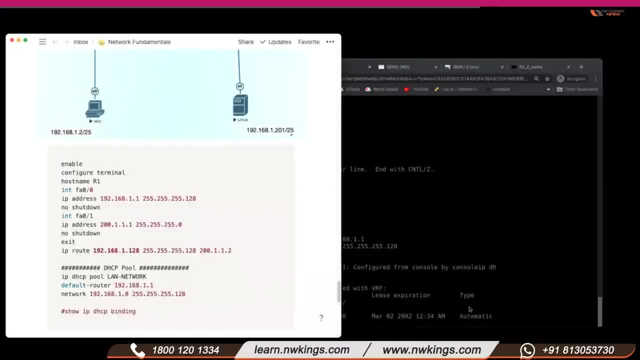 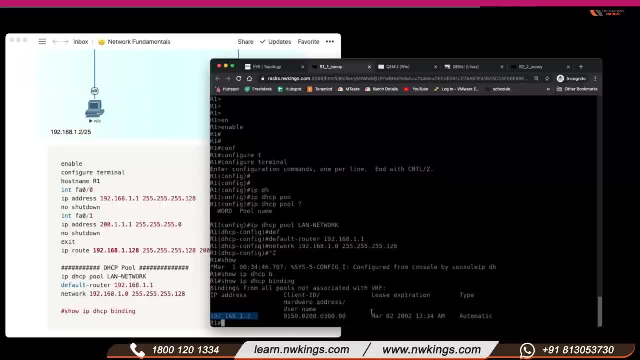 Show IP DHCP binding to check the pool. So you can see, on 192.168.1.2, I have given IP addresses, IP address 1.2, and the lease expiry means this IP address will be given till March 2, 2002.. 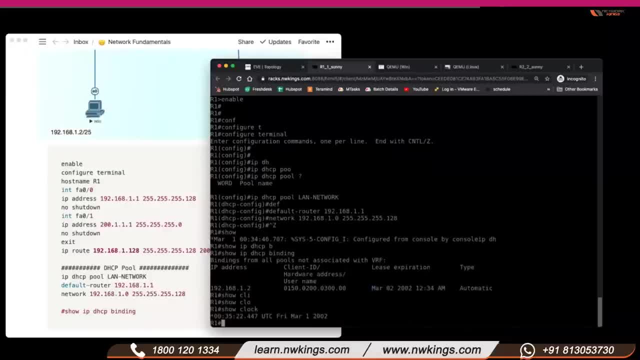 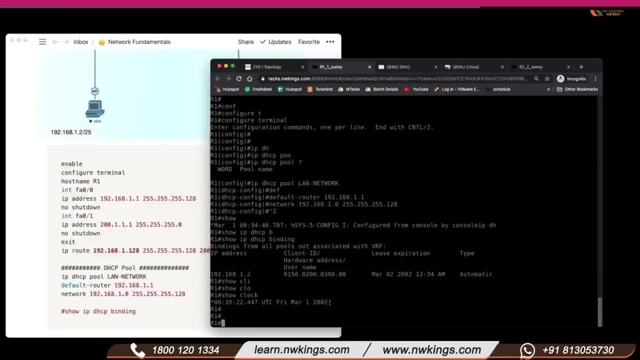 Maybe the router have incorrect time right now. Yeah, it's. these routers are like 18 years old, maybe. No, that. actually that clock is Yeah Not set properly. So you can see in my router it's March 1.. 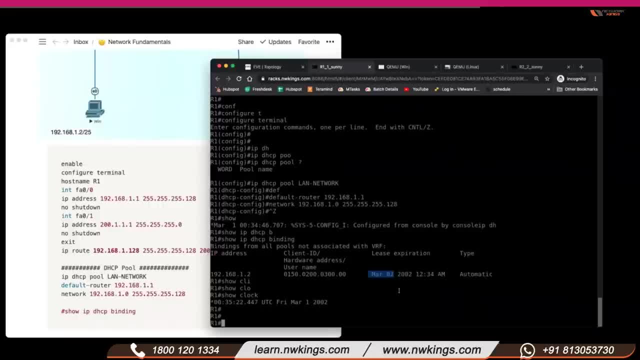 And here I'm giving IP till March 02,. it means 24 hour lease time. Lease time means that this IP address will be allocated to this machine. This is the hardware or the Mac address kind of thing of that device. So if your computer, if you turn off this device and you turn on the device in one hour. 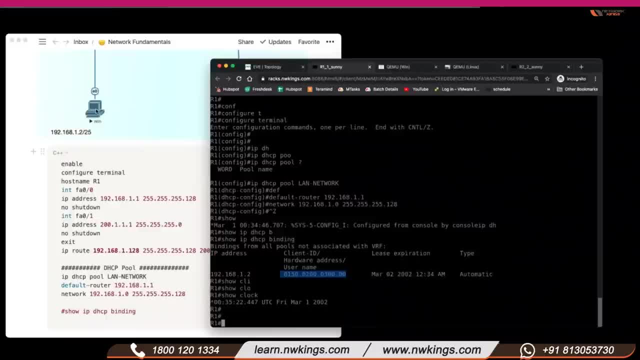 two hour, Three hour. the device will get the same IP address. But if you turn on this device, maybe after two days might be there is a chance you will get another IP from the pool. Okay, clear, Okay. This is how you configure DHCP. 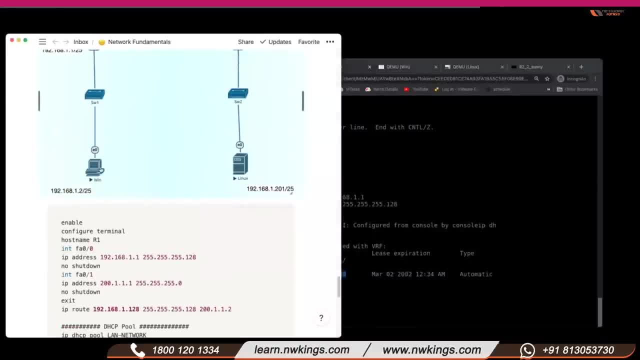 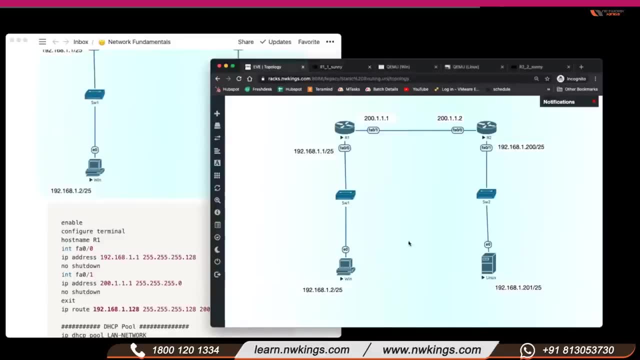 Okay, So all of right now, in my practical I have used only one PC. So you can use multiple PCs over here And so that you can connect and check if computer is getting the IP. Yeah, Linux also same like that. You need to just choose the DHCP service. 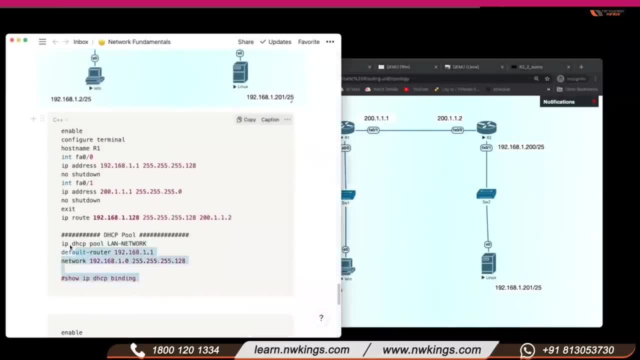 We can configure on R2 also. Let's configure on R2 for bad through practice on R2.. My default router would be 1.200, router Right IP and pool would be 1.128.. This would be the network ID. 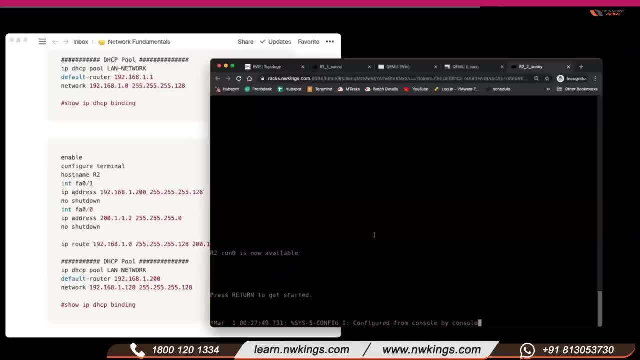 So on R2, I have to configure like this: So enable configurator So you can use the same name on another router, because this is locally significant Means if I'm creating a pool here, so it is not related to R1.. 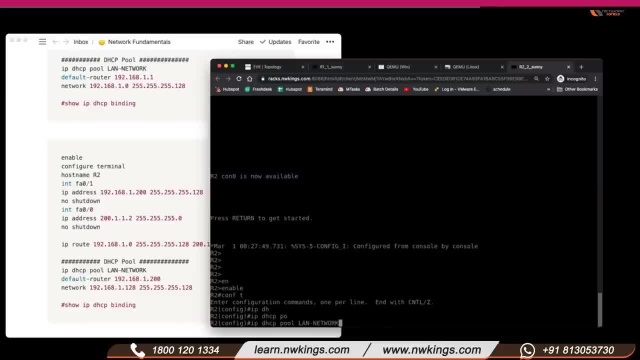 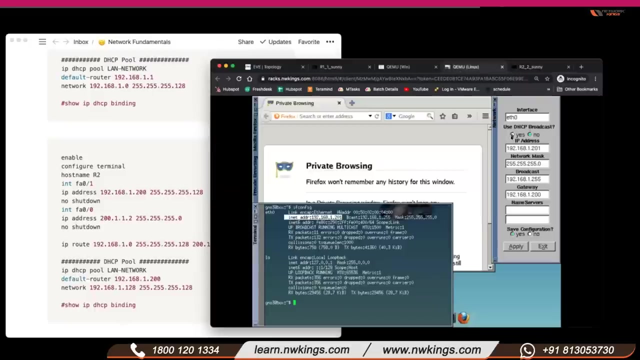 So you can use the same pool name here also. Okay, It should not be different. So it's your call. You want to use the same name or you want to use the different name? Okay, And on Linux machine we need to use this. 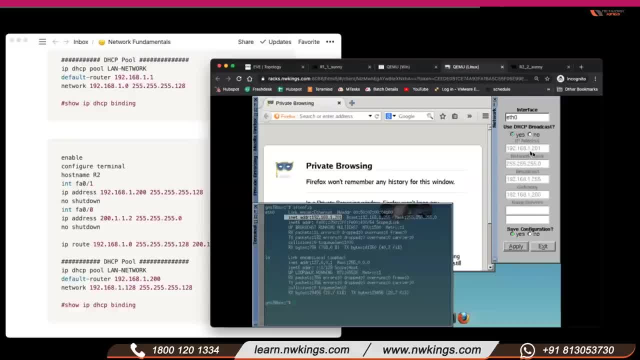 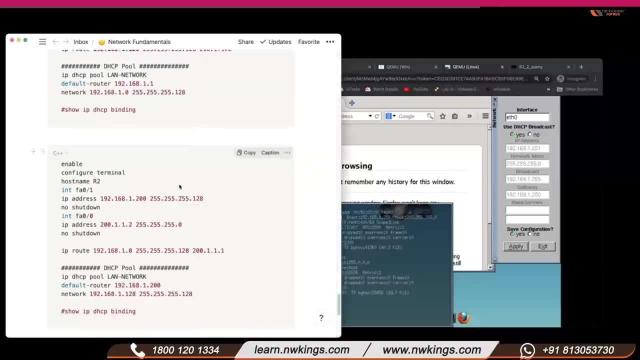 Use DHCP. Okay, Apply. So you can see here. I got the IP address 1.201.. Can you see that? The same config I got in Linux also, Kaleem. actually we have made our router as a DHCP server. We have made this router as a DHCP server. 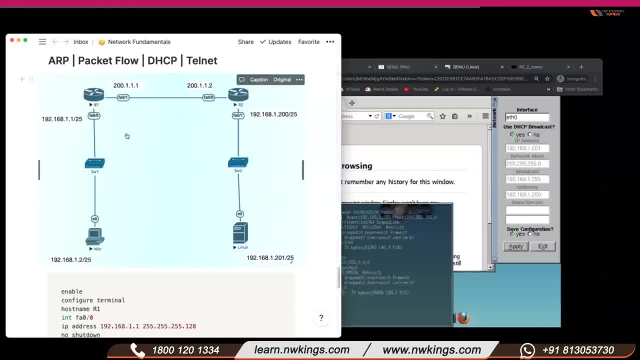 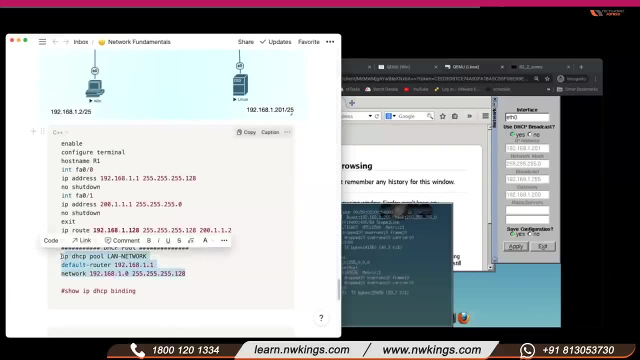 You don't need a DHCP actually server. So just this is just a terminology. We can create a DHCP server. We can create a DHCP server In our router. this is what we have done, So most of the companies are using this terminology. 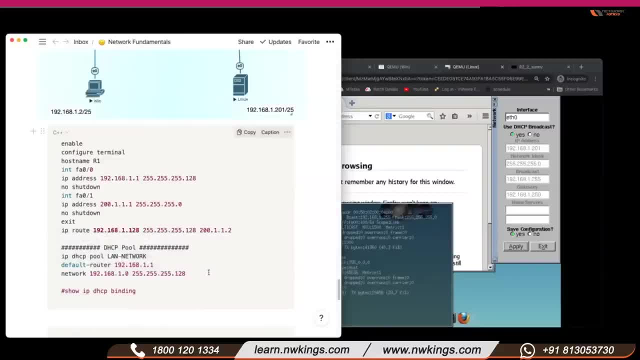 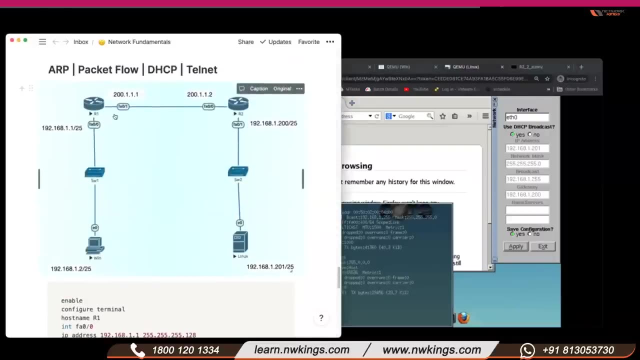 Just take an example: at your home broadband connection. Do you have any server at your home to get the IP address? No, right, So you have your DHCP pool inside your router, Okay, Okay, same thing we are doing on this cisco router, so you can. you can configure on any company. 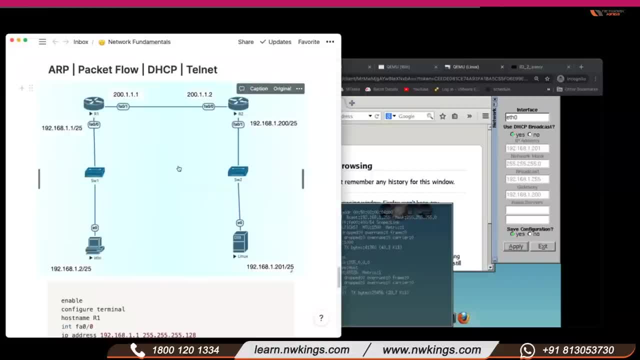 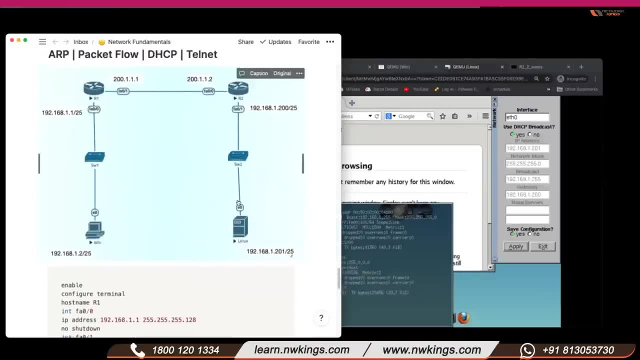 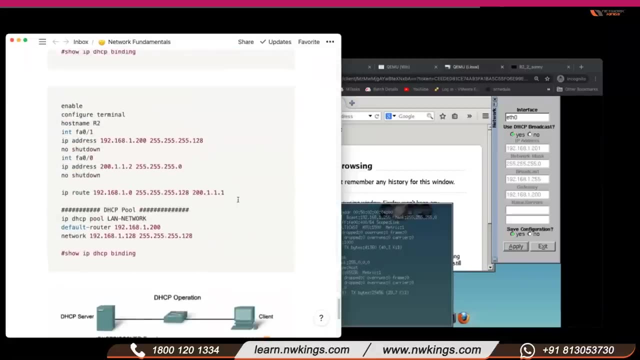 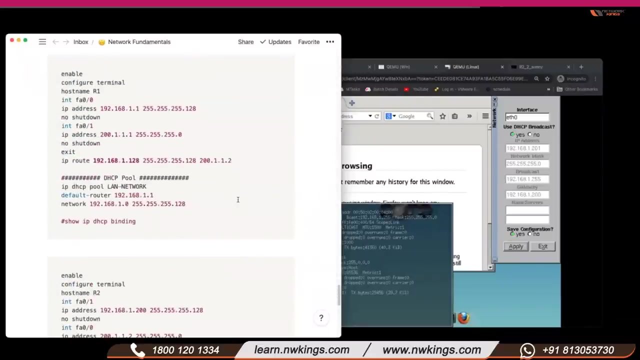 or any vendor device, also like juniper, hp, aruba, any company. so just you need to figure out what are the commands. okay, see, these are network fundamentals, but i just don't want to stick with the theoretical knowledge. i'm just giving you that practical knowledge. at least you will get an idea if you learn. 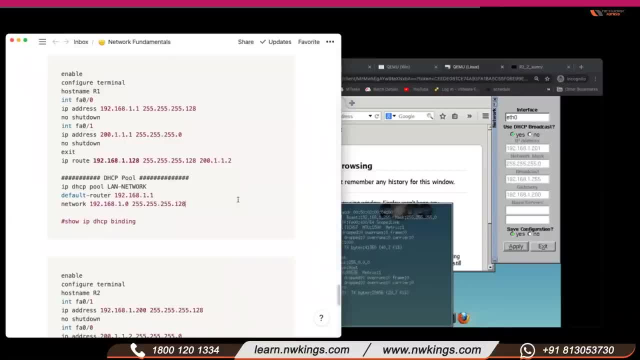 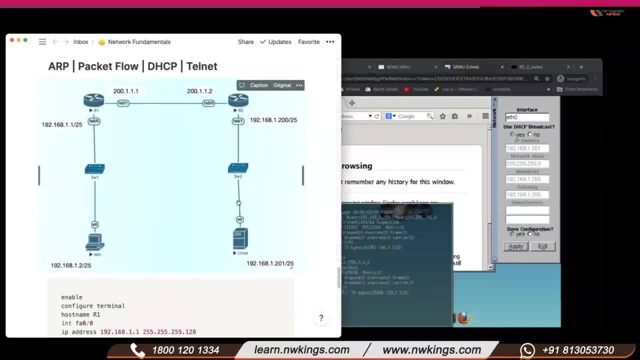 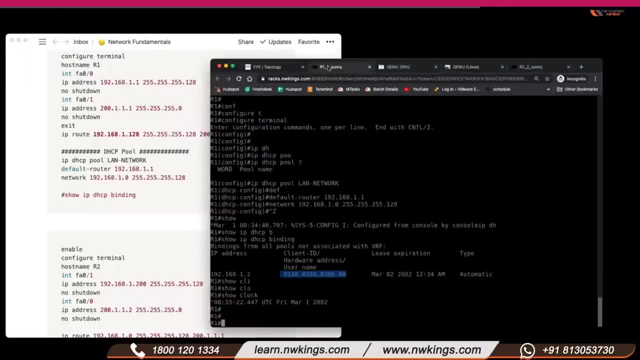 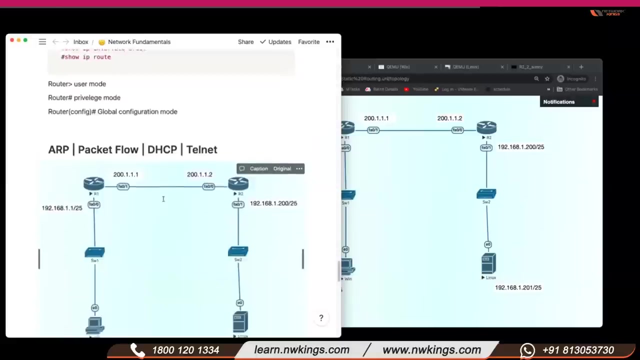 networking. if you go ahead with ccna, ccnp, what exactly and how? you will understand, because we have limited hours here. okay, but you need to practice more and more. okay, you can't be expert in five days, right? so this is just. you need to understand how.